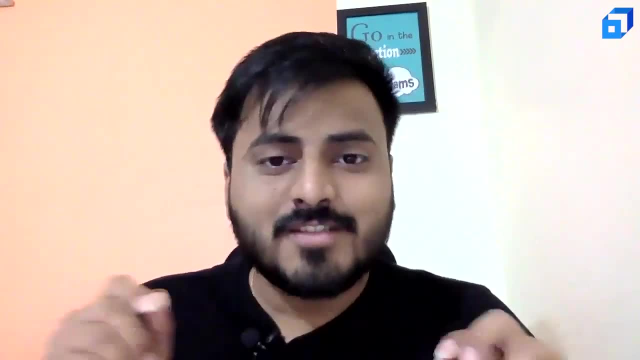 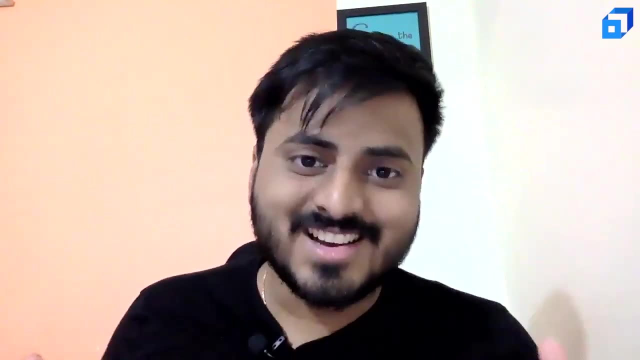 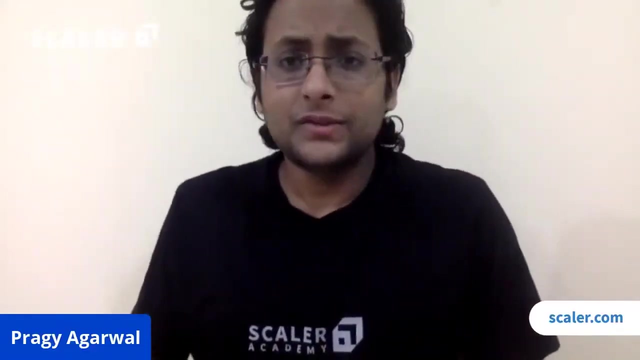 bind research. Finally, under which scenarios we can apply bind research. All these things will be covered in this 3 hour Snyder Cut. So watch, learn, have fun. Thank you. So hello everyone. So the topic for today is going to be Snyder Cut. 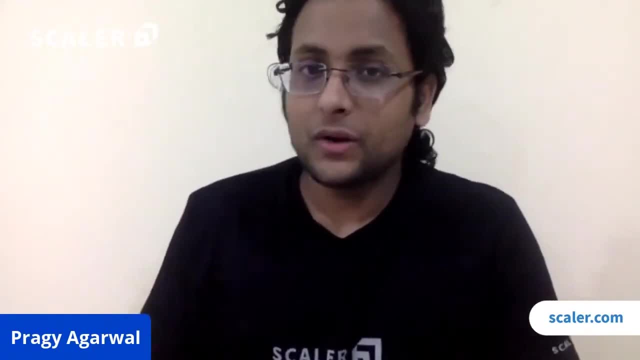 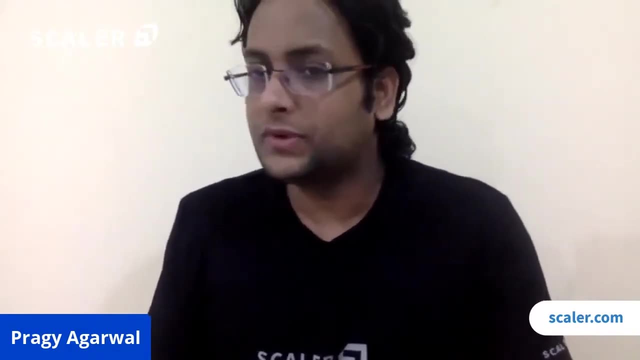 So we are going to look at different searching algorithms. We will start with linear search and then we will move on to binary search. We will look at ternary search and we will solve some problems related to binary search. Okay, Now, as always, after the class, we 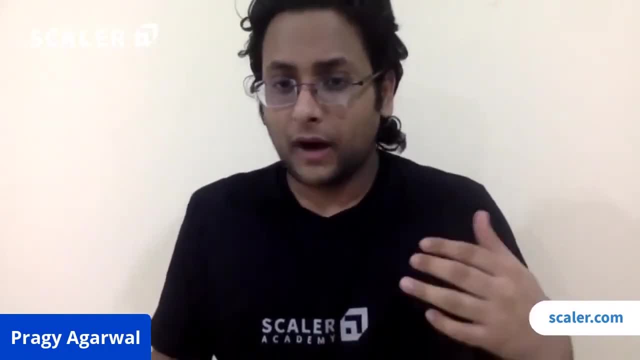 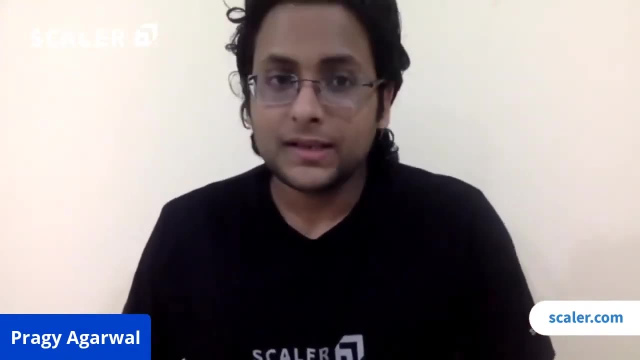 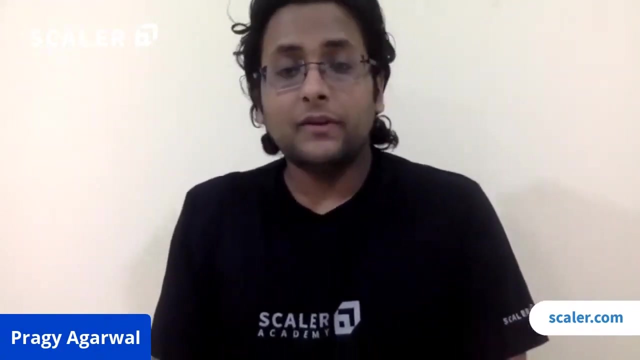 will have an assignment for you guys. So after every class you are given an assignment so that you can actually apply what you have learned in the class and solve problems, so that you can solidify the concepts. The link for the problem set will be in the video description. Apart from that, there 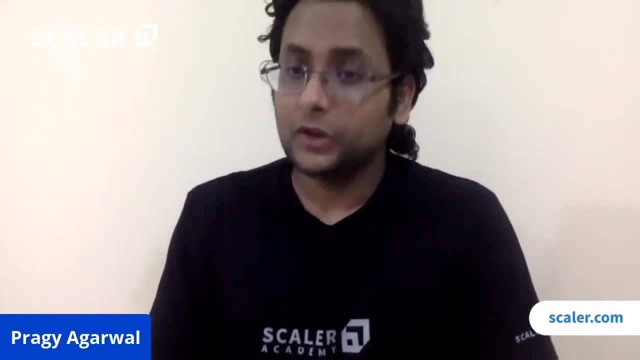 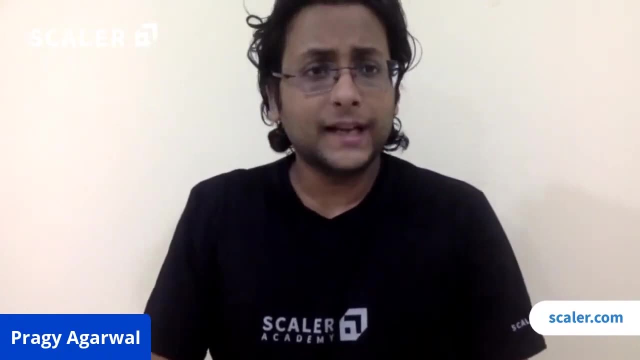 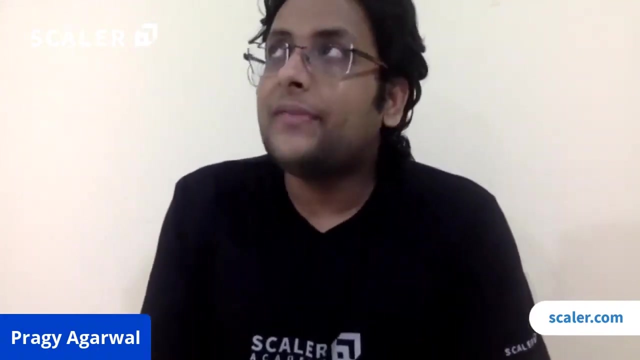 will also be a link for a chat forum so that you can talk to your peers and discuss any issues that you face while solving problems. So that is for today. There is one more announcement that I would like to make, which is that a lot of students come to us and they say that: 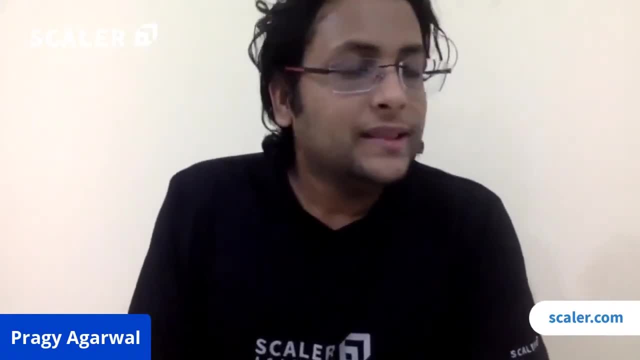 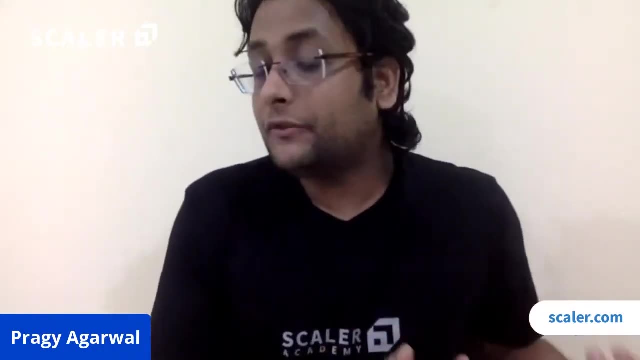 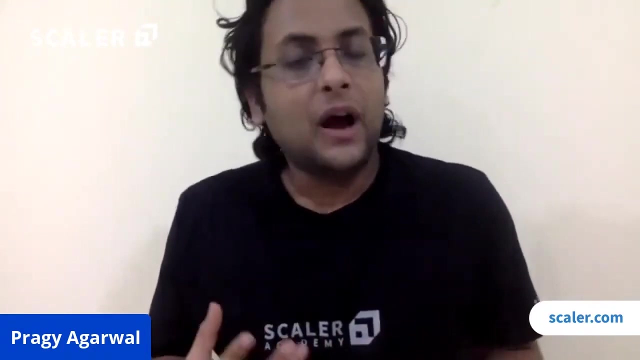 Hey, I need help with interviewing Right. So they tell us that they somehow get nervous during interviews, And a lot of students say that when I'm doing competitive coding online, I am able to solve problems, But when I'm in a face-to-face interview, I somehow get nervous or I'm not sure what. 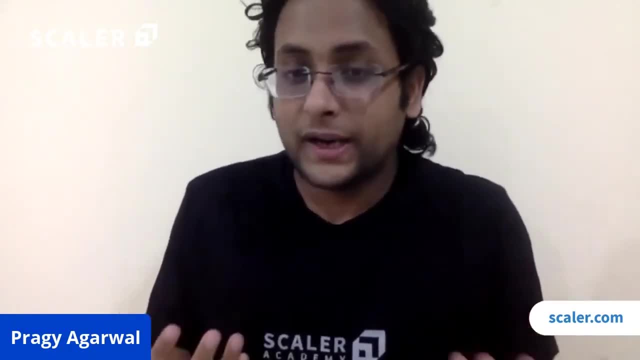 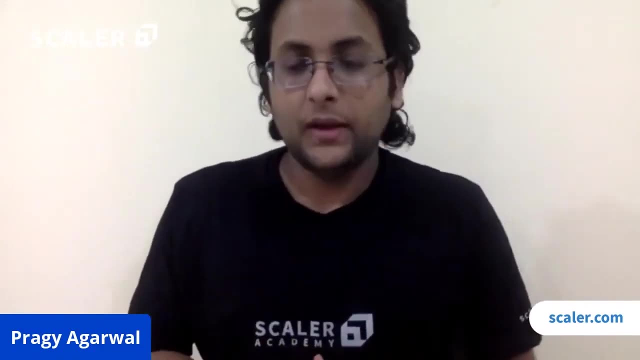 the correct approach, or what correct approach should I take while solving the problem in the interview? So, to handle that, we have organized a mock interview for you guys today, Right? So suppose that you wanted to see how an ICPC world finalist, right? Someone who? 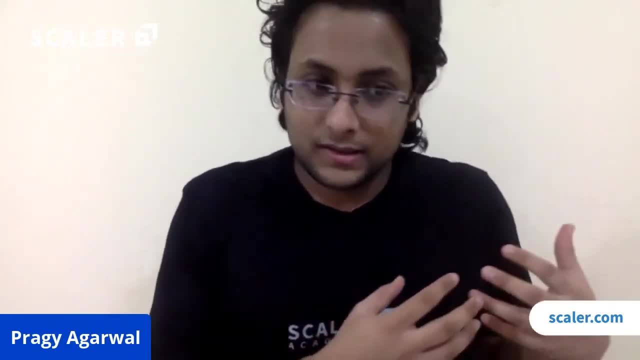 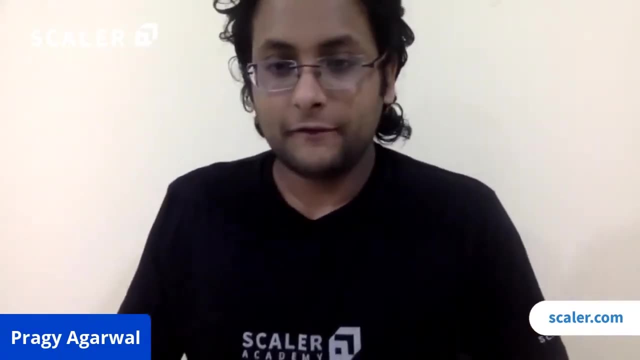 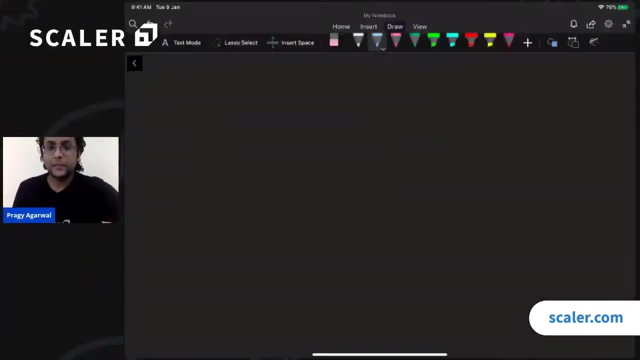 is very strong at data structures and algorithms. how such a person would behave, would approach a problem in a Google interview. All right, Without further ado, let us dive into today's lecture. So let me just share my screen, All right. 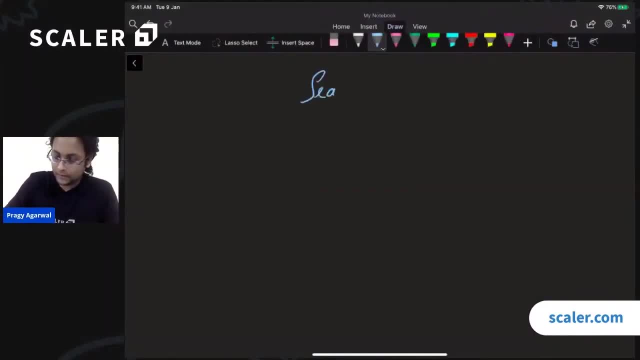 I hope that this is visible to everyone. Can someone just conform These Perfect, Perfect, Perfect. So I assume that most of you would be familiar with some sort of searching right. Suppose that you have a collection. suppose that you have a haystack and you are looking. 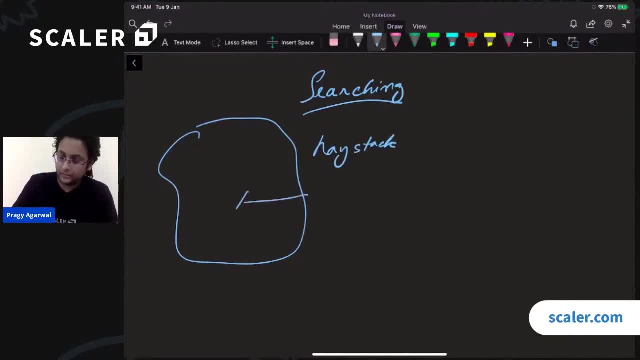 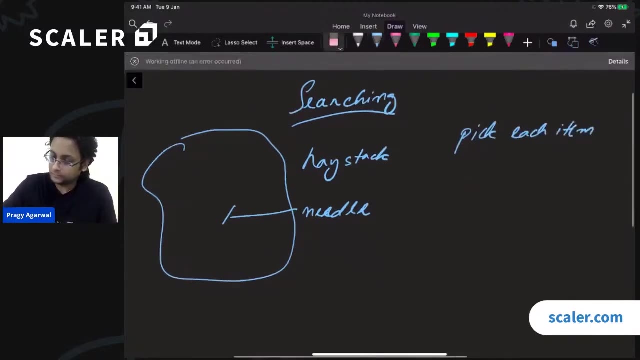 for something in this haystack right, Suppose a needle. then how do you usually search? Well, the way we usually search is: we pick each item one by one. pick each item one by one, one by one, and we inspect it right. 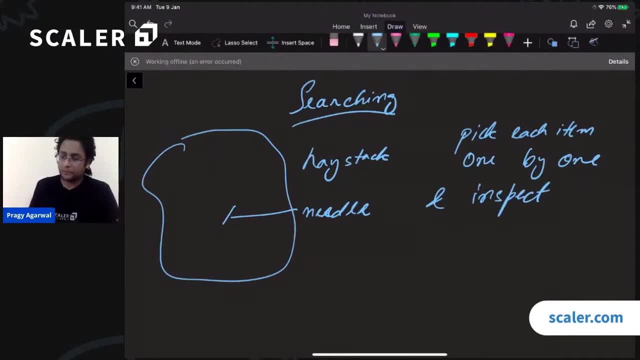 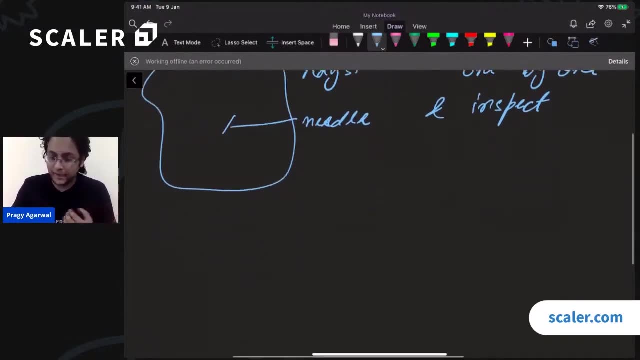 We see if this is the correct item, if this is the item that we are looking for Now. this can be very, very time consuming, right? So just to prove this point, let us play a very simple game. okay, So I want you all to play this game. 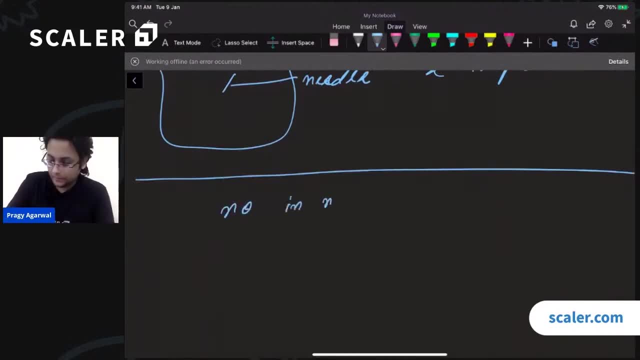 So I have a number in my mind, right, And I'm telling you that the number is between 0 to 1000, okay, Now what you're supposed to do is you're supposed to guess what the number in my mind is. 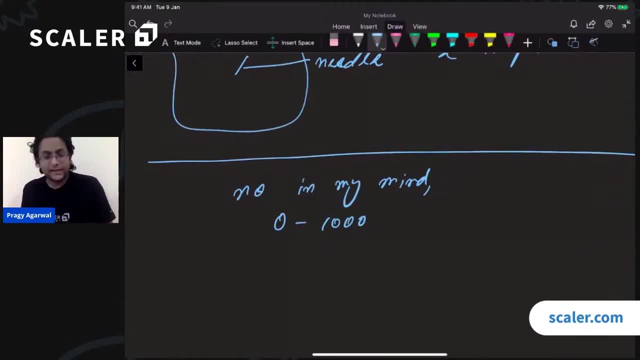 I'm not telling you the number right away. So you're supposed to make guesses between 0 and 1000.. So if you could please start spamming in the chat. just tell me your guesses in the chat and whenever I see the number that I'm guessing, that is in my mind, I'll let you guys know. 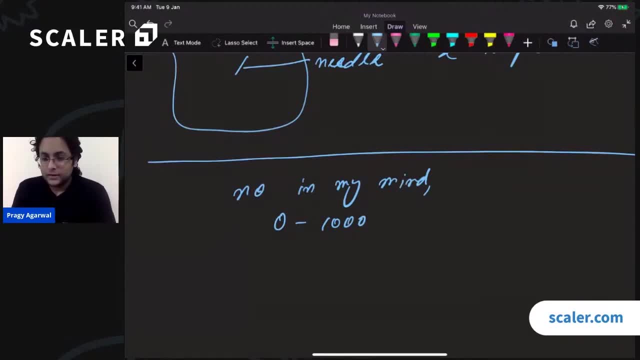 All right. So can you guys please start? I have a number between 0 to 1000 in my mind and you have to guess that number. So start basing in the chat. What do you think the number is? You have no other information. 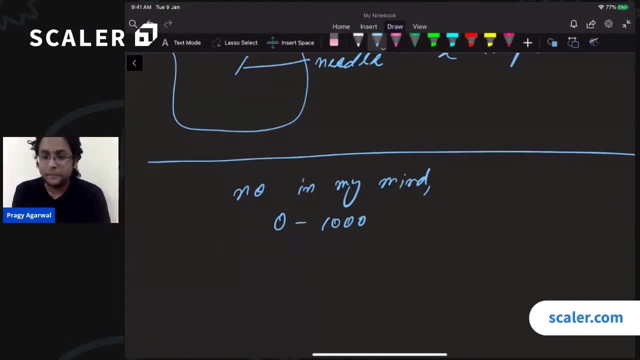 786, not really. That is not what I had in my mind. Oh, okay, I got 52,, 3, 0, 91, 900, 100, 99.. No, none of those. A lot of zeros. some 500,, some 304,, 300, 6, 6, 6, 7,, 8, 9, 10,, 11,, 12,, 13,, 14,, 15,, 16,, 17,. 18,, 19,, 20,, 21,, 22,, 23,, 24,, 25,, 26,, 27,, 28,, 29,, 30,, 31,, 32,, 33,, 33,, 34,, 34,, 35,, 36,, 37,, 36, 37,. 38,, 40,, 41,, 42,, 43,, 44,, 45,, 46,, 47,, 48,, 49,, 50,, 51,, 52,, 53,, 54,, 55,, 56,, 57,, 58,, 59,. 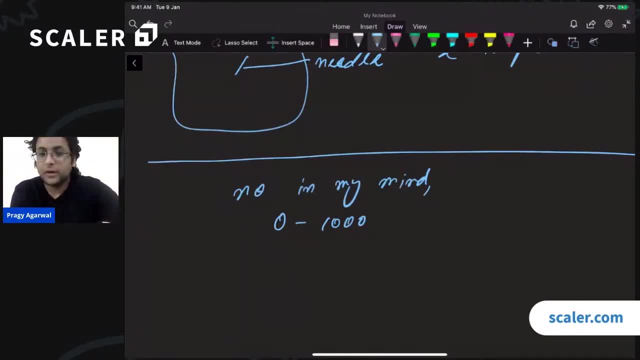 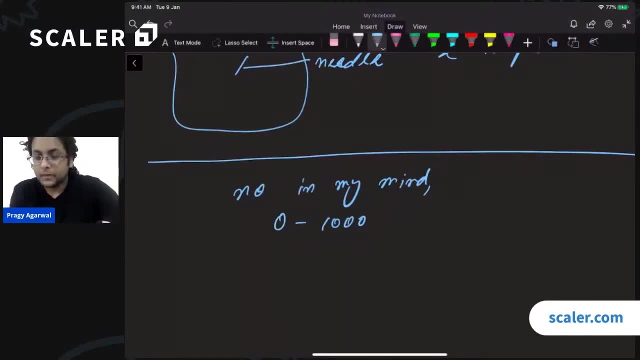 90, 80,, 80,, 80, 80.. Please give some hint. So the show has a very important thing over here. Tushar says: if you could give us something, then we will be able to approach that particular. 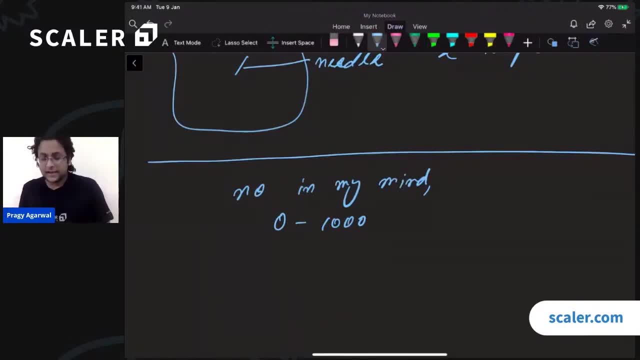 particular solution much faster, perhaps, Right? So we see that if you have no information, if you have no information, information about how to search, then your best chance is to randomly check, randomly guess, Right? Or if you don't want to randomly guess, your best chance is to basically check each possibility. 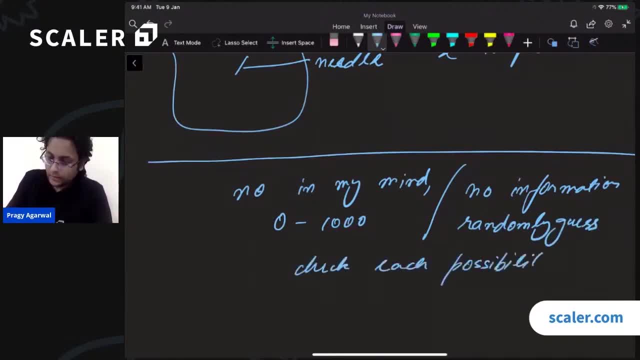 Possibility Right. So it could happen that first you say that, okay, you are guessing the number one, then you move on to number two, then you move on to number three, and you keep doing that, you keep making guesses, till I say that yes, your guess is correct. 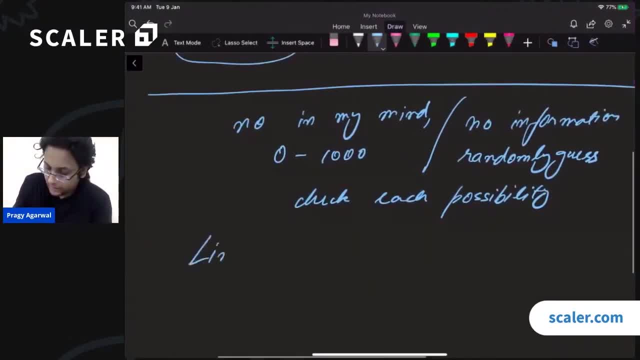 Right? So this is an example of something called linear search, Right? Why linear? Why linear? Because you're going over each item item linearly, right? basically, you're going over each item once. So this is this is called linear search. 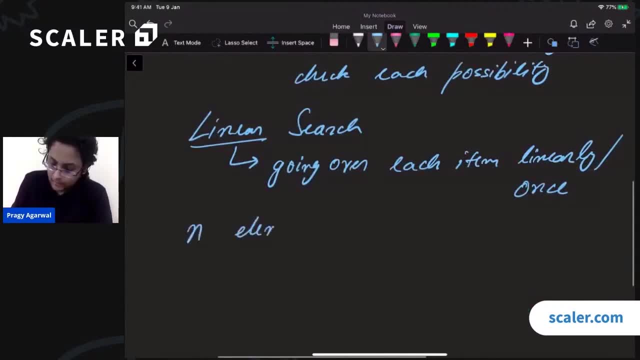 And let us suppose that you have n elements, that you have n elements and you're looking for some value, you're looking for some key in this set of n elements, then how much time, how much time will linear search take us? 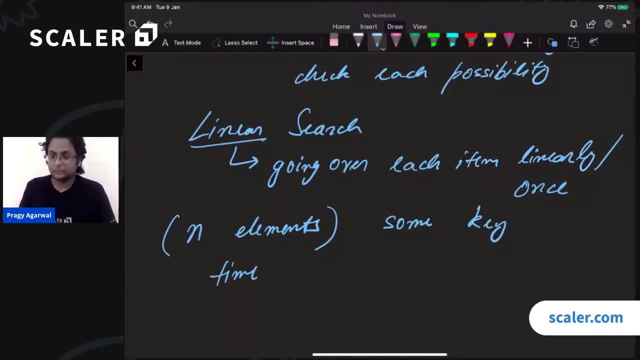 So what is the time complexity of linear search? It is, yes, it is order of n time, Right, And while we're at it, let us also quickly discuss the space complexity. So how much space does it take you to do a linear search? 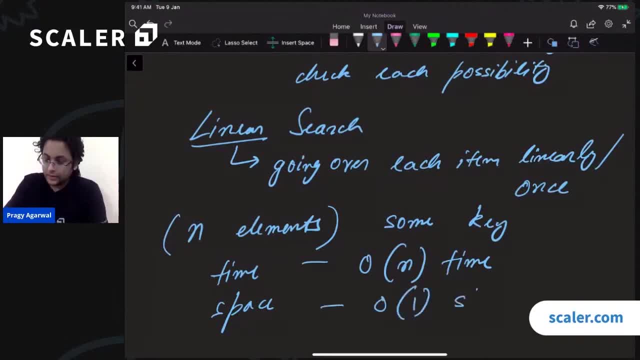 Well, this is just order of one, Right, Because we don't really have to store a lot of memory. We can just use a couple of temporary variables and perform the linear search, Alright, So I assume that everyone is familiar with this linear search. 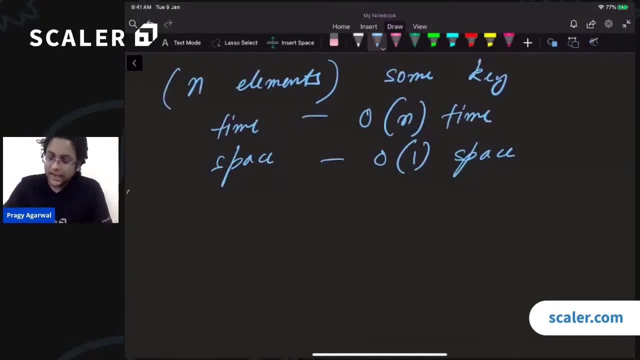 So linear search is very inefficient. Now the question comes: can we search faster? Can we search faster? Right, What do you think the answer to this is? So this is the question. Now I'm asking you: what do you think the answer will be? 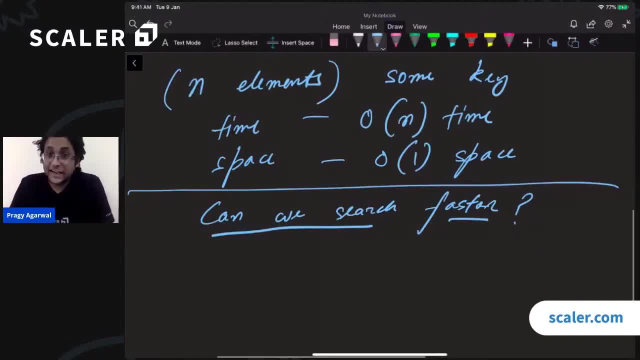 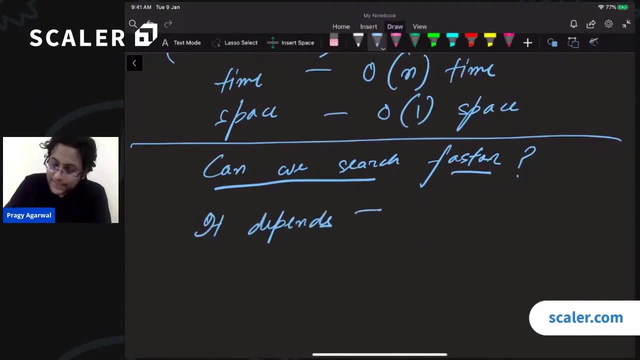 Now, as most things in life, the answer is: it depends, Right, It depends. Well, it depends on what It depends on. is there some pattern, some pattern in the data that we can exploit, That we can exploit? 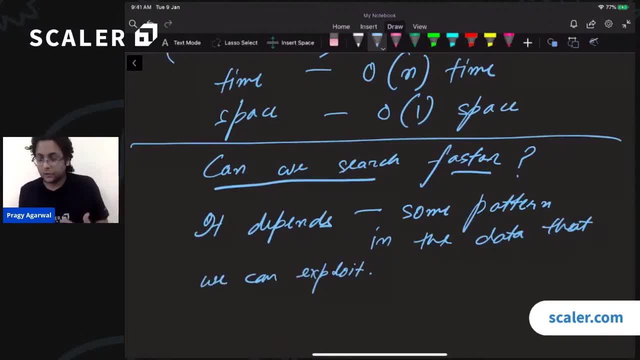 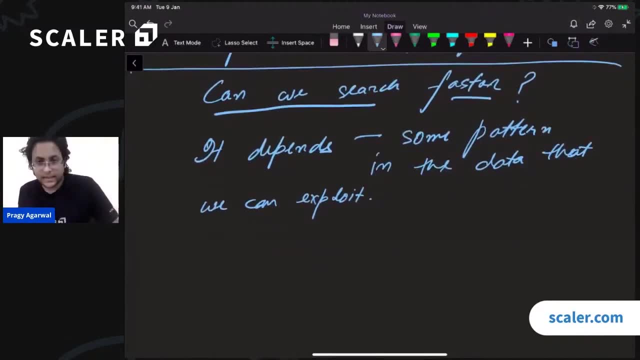 Right, If we have some pattern in the data that we can exploit, then perhaps we could search faster, Right? Does that make sense? For example, let us play this game once again. Right, Let us play this game once again. I am going to guess. I'm going to have a number from 0 to 1000 in my mind. 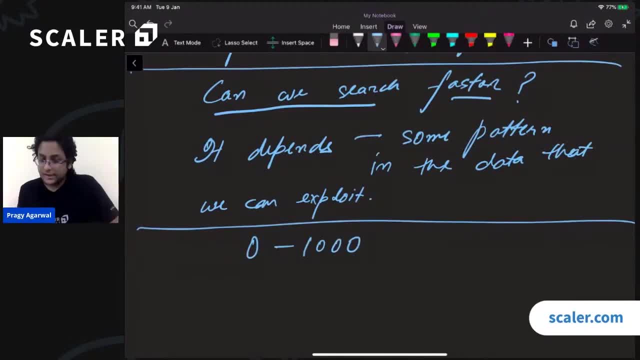 And you are supposed to guess that number once again. However, this time, whenever you make a guess, I'm going to tell you if your guess is too high or if your guess is too low. Alright, Cool, So let us begin once again. 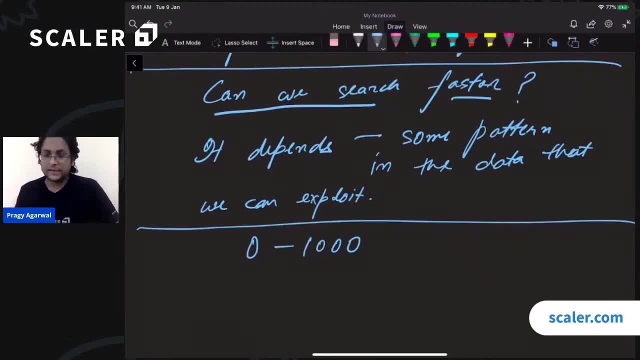 I have a number in my mind And could you start guessing please? So Mudasir says 2.. Well, 2 is too low. Then Mudasir has guessed 34.. 34 is too low once again, Then the next guess is 123. 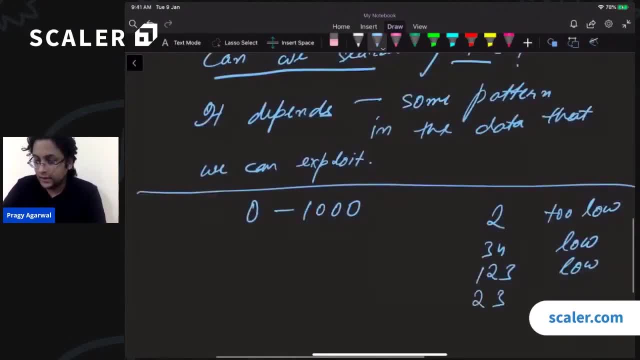 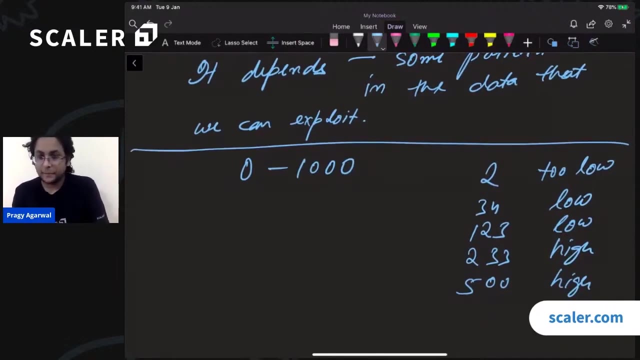 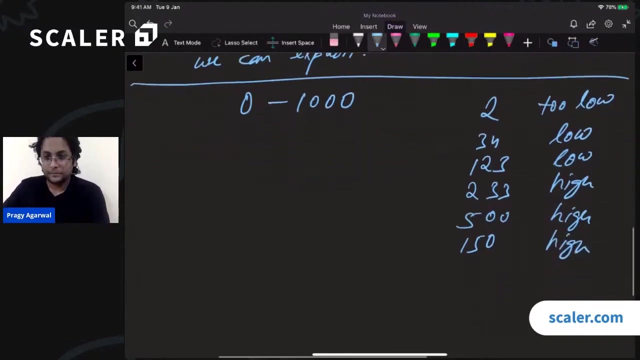 It is too low. The next guess is 233.. That is too high. Sahil says 500.. That is too high. Alright, Keep them coming. Keep the guesses coming. The next guess is 150.. This is too high. 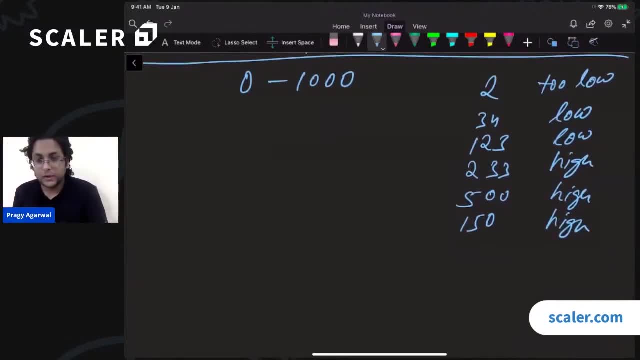 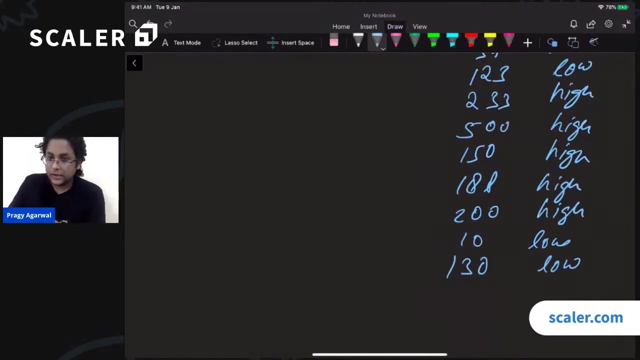 Then what is your next guess going to be? So 188. No, 188 is still too high, 200 is still too high, 10 is way too low. Yes, so 130, 130 is too low. and then what do we have? alright, so 130 is too low, can? 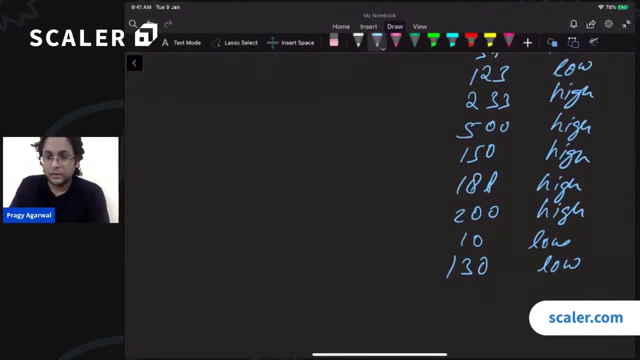 you make more guesses now. 143, right? someone guessed 143 and that is exactly the value that I was thinking of, right? this was my guess. this is correct. alright, so we see it took us some time. right, it took us some time. it was not that we were able to guess. 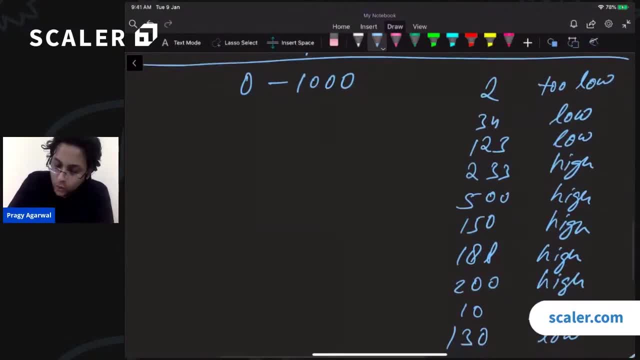 the answer immediately. however, we were able to hone in on the answer, right. so you have. you know of homing missiles, right? the homing missile doesn't really know where the target is, but as it moves forward it will get closer and closer to the target. 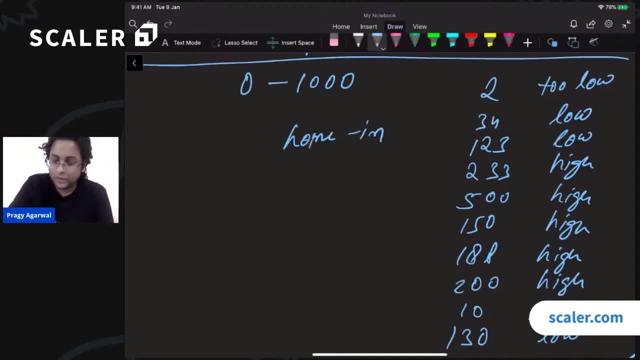 right. that is what we were able to. we were able to hone in right, hone in on the answer. why were we able to do that? because there was some pattern in the data that we could exploit. the pattern was that we were able to figure out whether our guess was too low. 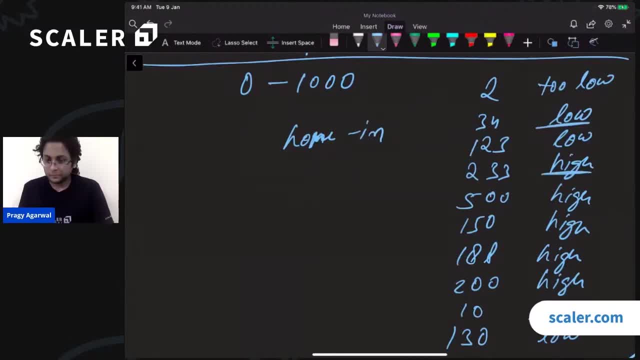 or whether our guess was too high. right now, a lot of you think, a lot of students think they have this misconception that some sort of a binary search- right binary search- can only be applied when the data is sorted, and that is not the case. the data has the 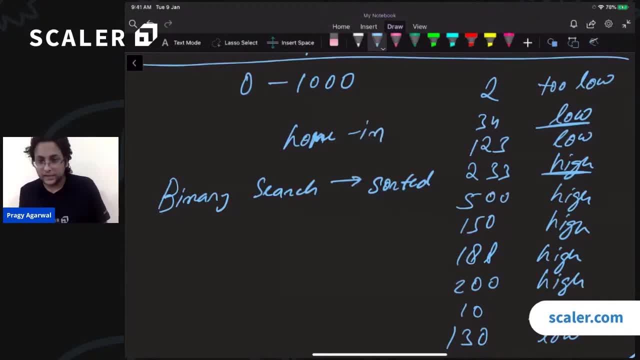 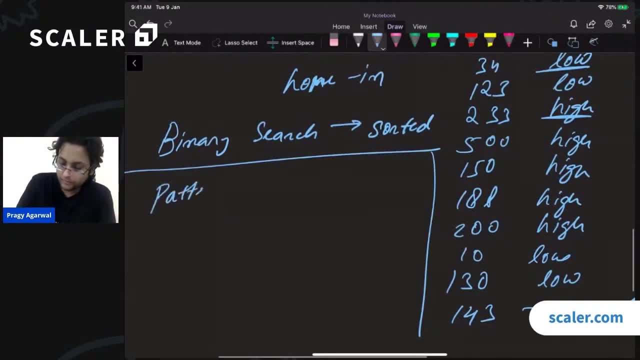 data need not be perfectly sorted for you to be able to apply a binary search, right? so what we are looking for in the data is: we are looking for some pattern or some sort of ordering. okay, so let us define some nomenclature over here. let us define some theoretical. 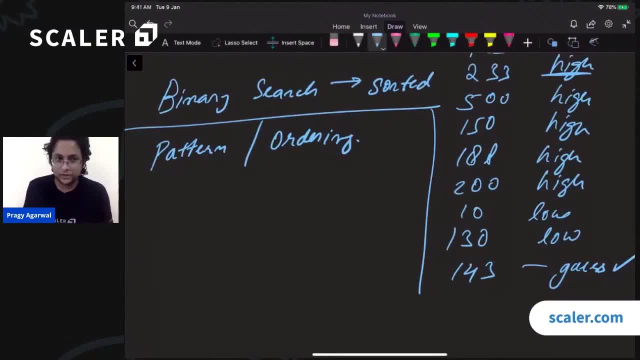 nomenclature over here so that we can make concrete progress over what binary search is right. so suppose that you have some search space, that you have some search space right, and let us represent the search space like this: in the search space there is a- this: 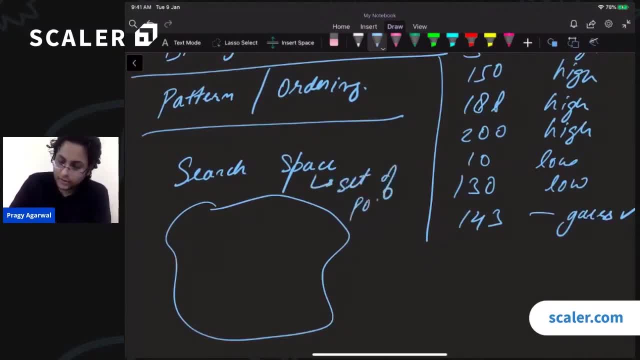 search space is basically a set of possibilities, of possible answers, right? so there's there's one answer possible over here. so this is another possible answer. this is another possible answer, another possible answer, perhaps another possible answer, and so on. 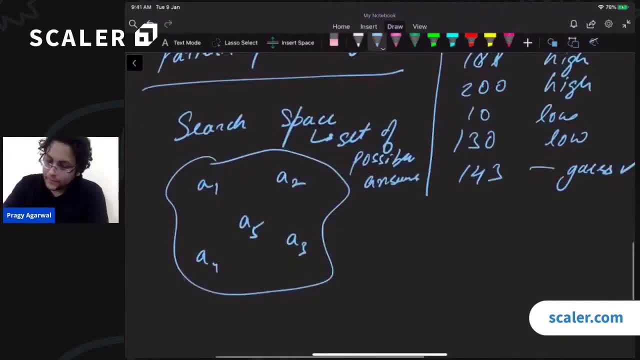 What binary search says is that when you make a guess- let us suppose that you made this as the guess- When you make a guess, if you are able to eliminate, if you are able to eliminate a large fraction, a large fraction of your search space, search space, then you can search. 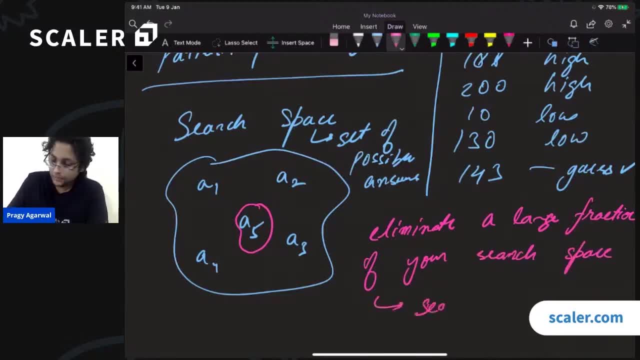 efficiently. if this is the case, then you can search efficiently. right, let's look, let's see how. so let us look at the previous game that we played. in the previous game, whenever you came up with an answer- let us say that you came up with an answer- that, hey, the guess is 200. then all I told you was whether the 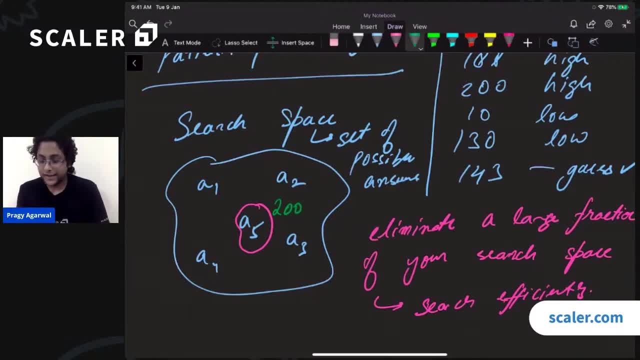 guess was correct or not right. all I told you was whether the guess was correct or not, and that basically allowed you to eliminate this possibility itself right. so you made a guess 200. I told you it is not correct, so you can eliminate this possibility. can you eliminate any other number, can you? 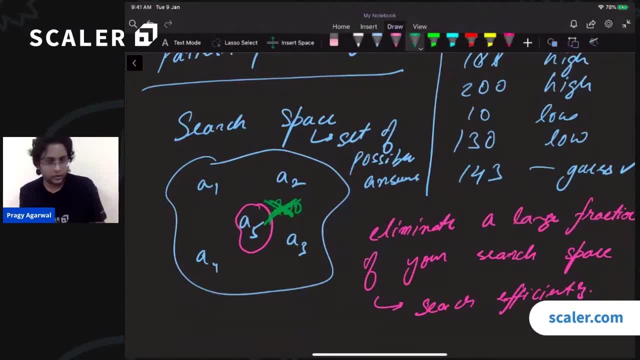 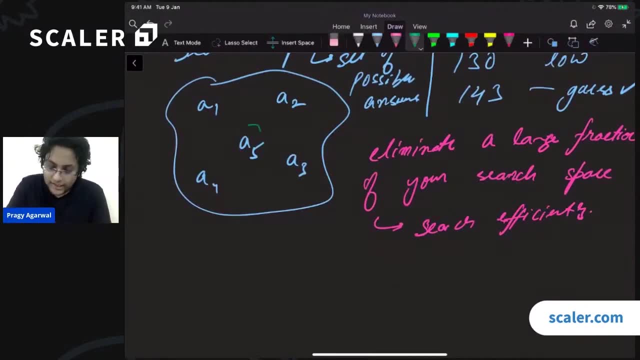 eliminate any other number. did you get information about any other number? you did not. on the other hand, in the second version of the game, in the second version of the game, suppose you guessed 200 and I told you that it was too high. then you could have eliminated every number. you could have eliminated all these numbers. that 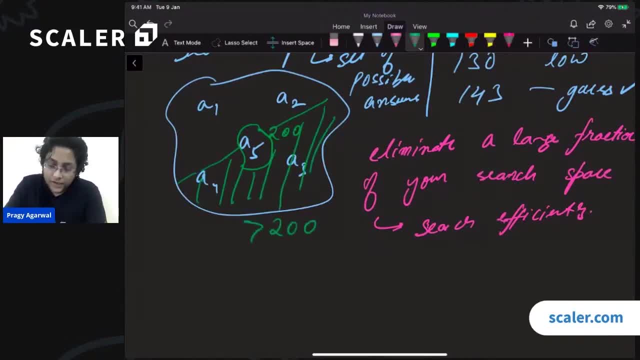 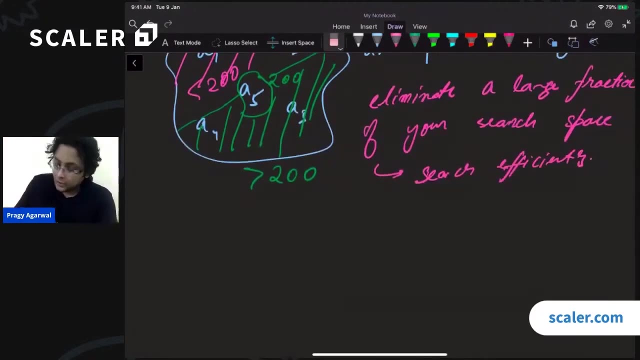 were greater than 200 and your search space would only remain with the numbers that are less than 200. right, does that make sense? yes, so this is something that we will try to exploit in INF rejoice. so, basically, binary search. binary search can be applied whenever you can. you can remove, removed or prove a lot. 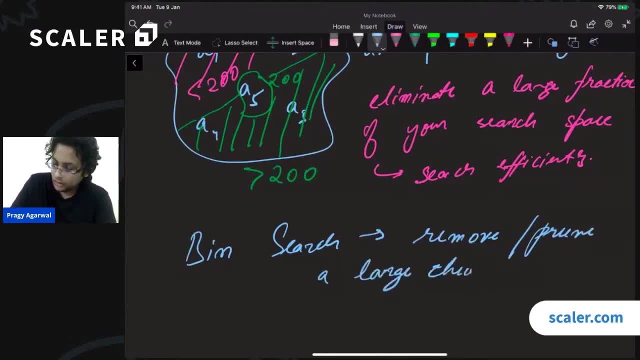 chunk, chunk of your data, of your search space, search space with every guess, all right, all right. so now let us see how you get it from your jaguar. Heather, we have a 否, All right, cool. So let us look at a more concrete example of this. 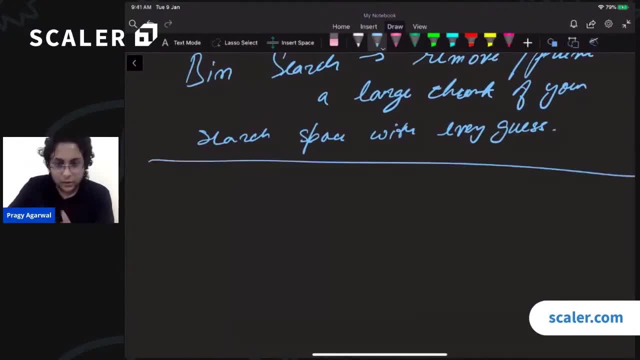 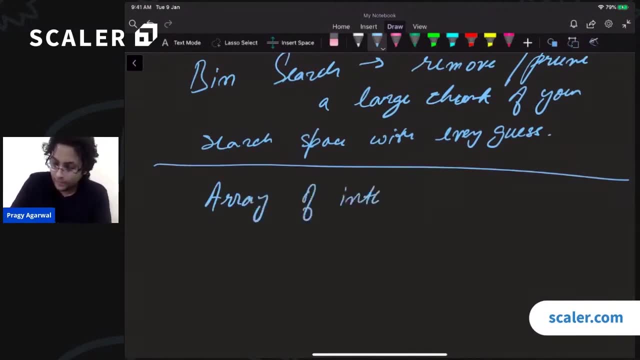 So, mostly when we are talking about searches, the first thing that would come to our mind is that we have an array, right, We have an array. suppose we have an array of integers, right? This array has multiple values. Let us say that the size of this array of size, n, the size of this array is n and we. 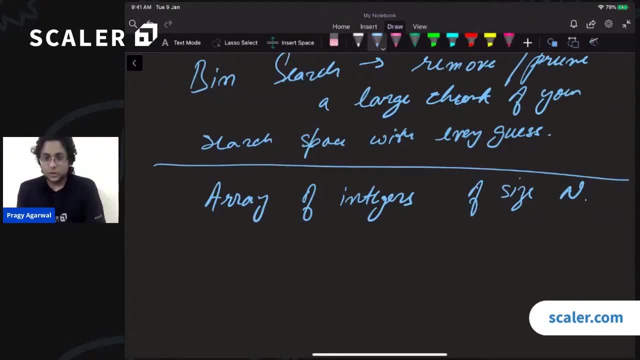 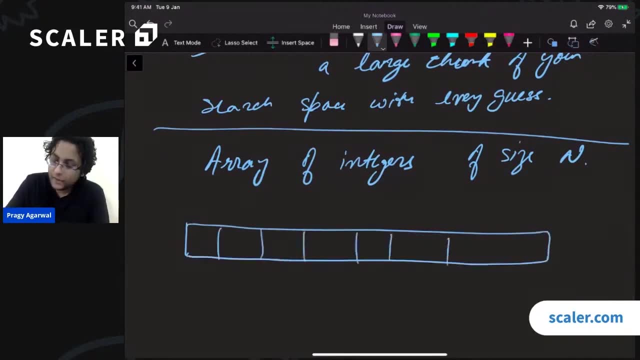 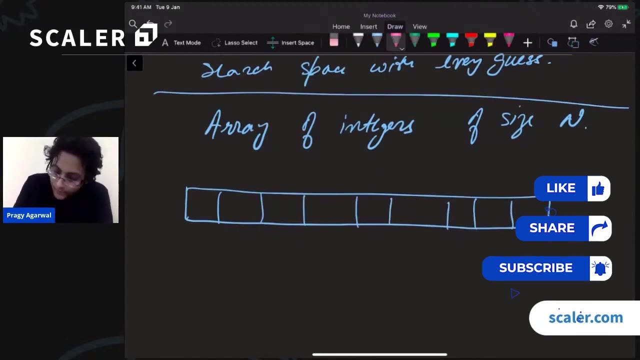 are supposed to search for a particular value in there. So, given an array, given an array, what type of things are we able to binary search for? What type of things are we able to binary search for? So whenever we try to binary search, we try to come up with a proposition. 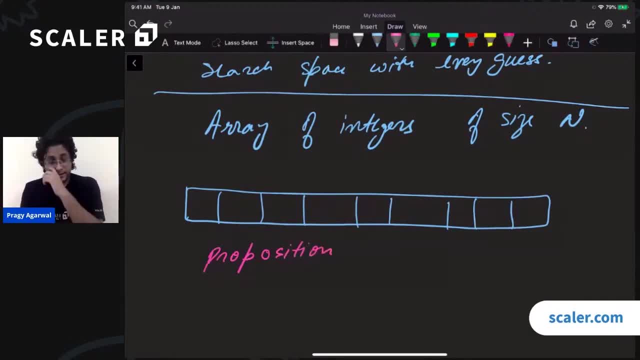 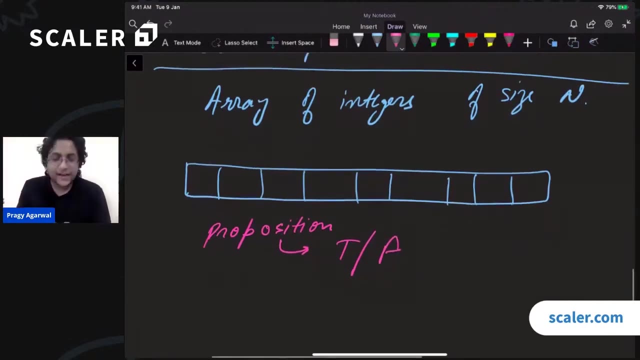 Does everyone understand what a proposition is? Yes, a proposition is something that takes two values- any of two values- right. A proposition can either be true or it can be false. Now, if you can come up with a proposition, if you can come up with a proposition such 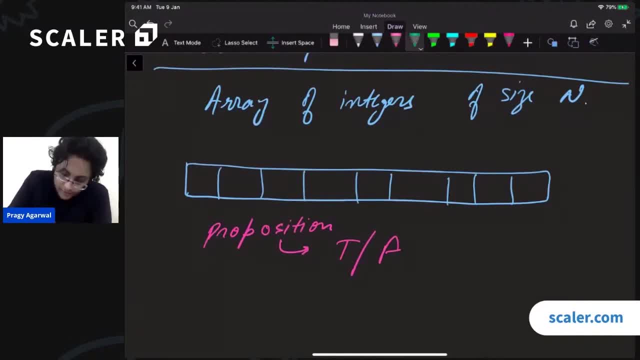 that your array starts looking something like this: that for this particular element, the proposition is true. For this element, the proposition is true. For this element, the proposition is true, and so on. At some point the proposition starts becoming false right. 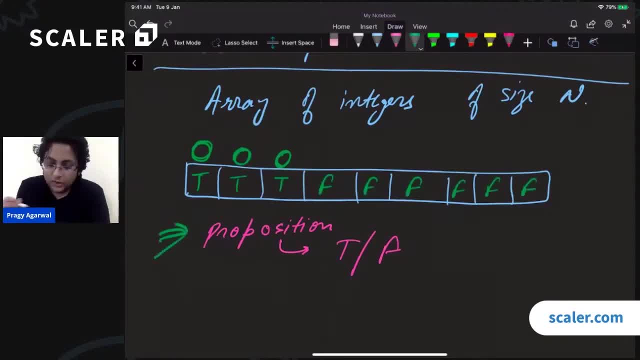 If you are able to come up with a proposition that can make your array look like this, and then you are able to perform binary search on this array, and what will that binary search give you? That binary search will give you this boundary point. 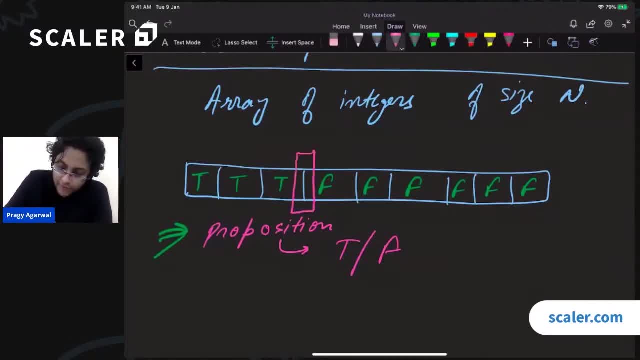 That binary search will give you this point where the proposition flips. All right, Is that clear? So we will look at a little more concrete examples of this. We will look at a little more concrete examples of this. Cool, So let us once again go back to this game of guessing the number. 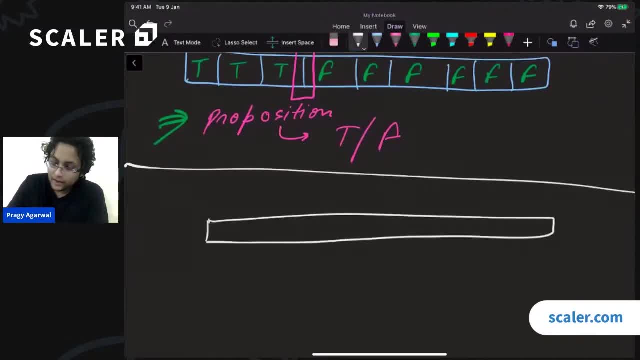 Let us suppose we have a binary search. Okay, So let us suppose that I gave you an array from 0,, 1,, 2, all the way till 1000, right, All the way till 1000.. And I had a guess. 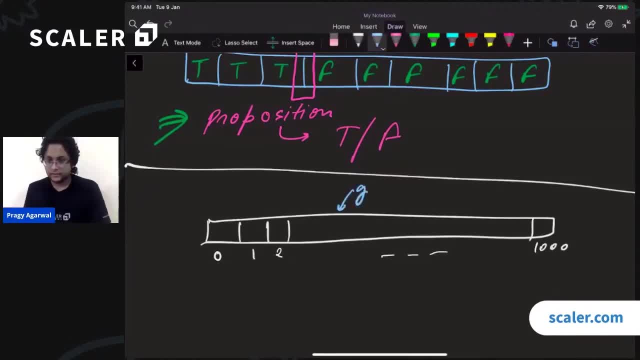 Let us say my guess was this number G. The correct answer was this number G. Now, what is my proposition over here? What is my proposition over here? So, what is the proposition that makes sure that everything to the left of G is true and 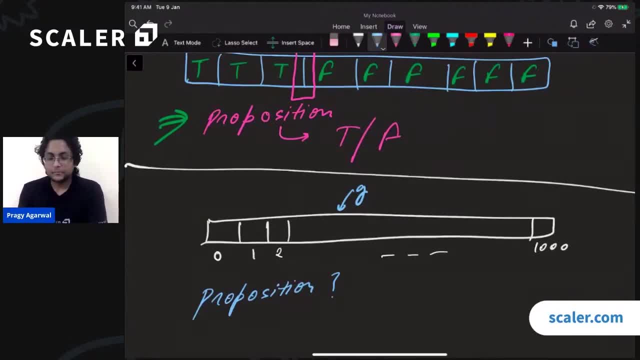 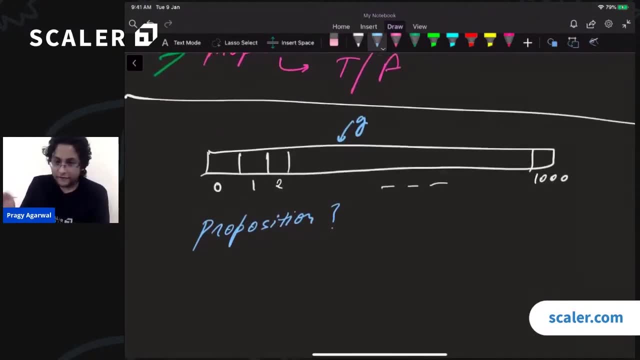 everything to the right of G is false. Can someone tell me that? So what proposition should I make so that everything, every number to the left of G should result in false, while every number to the right of G should return it true, Exactly? 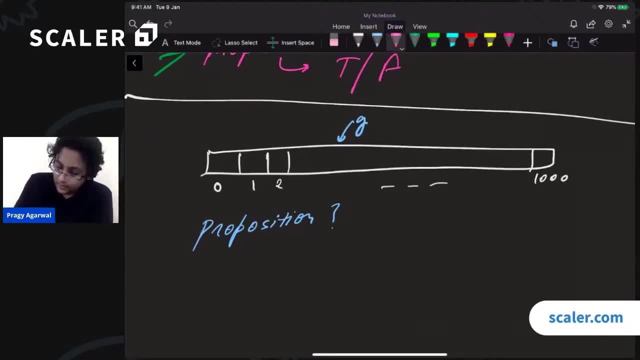 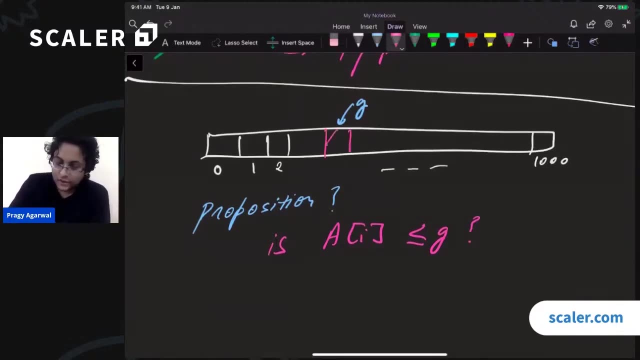 So the proposition can be as simple as: is A of I less than G, Right? Is A of I less than equal to G, Right? What happens in that case? So if G is my guess, if G is my guess over here, then every value to the left of it. 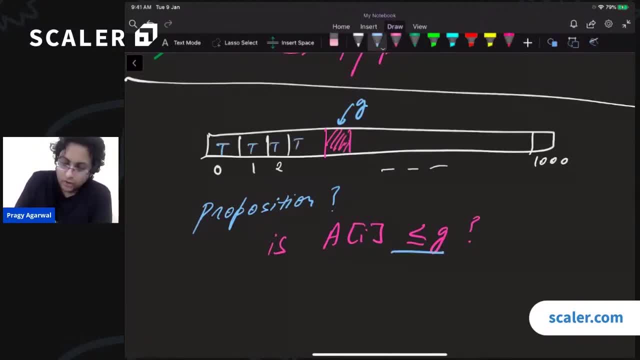 yes, it is less than equal to G. So all these values will be true. All these values will be true. On the other hand, on the right hand side, all these values will be false because they will be if the array is sorted. all these values will be false because they will be. 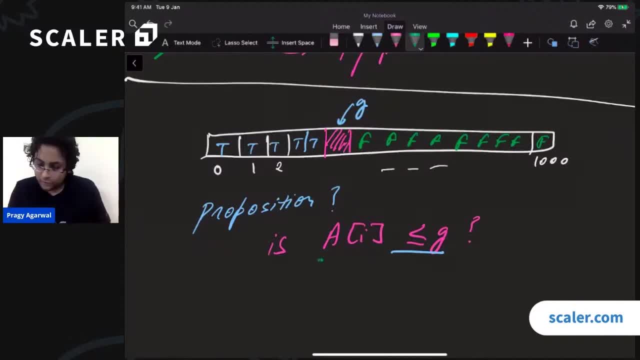 larger than G. So if, if I'm able to come up with this proposition, then binary search will allow me to find this junction, It will allow me to find this point where the true flips from true to false. Is that clear, All right? 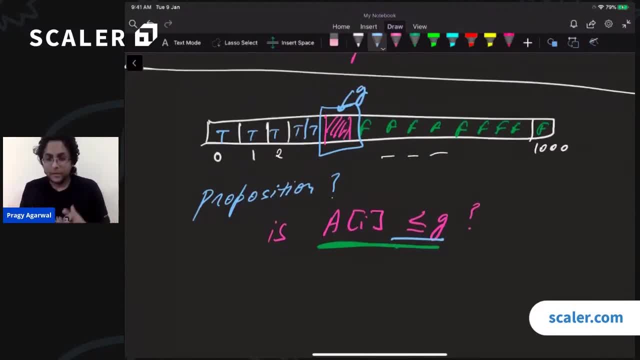 And now the now. we have basically. now we have basically come up with the final definition of binary search. Binary search does not require you to have a sorted array. That is a misconception that you need to have a sorted array array to perform binary search. 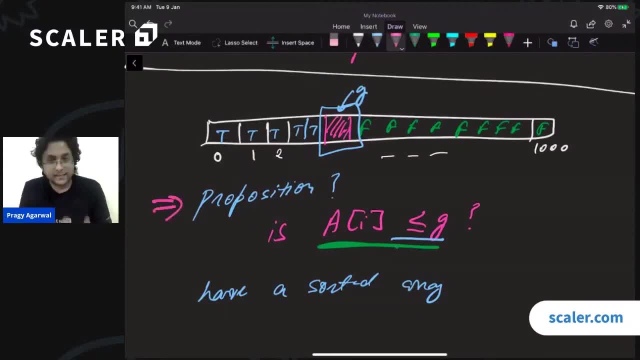 What you really need is you need this proposition. If for any search space you can come up with such a proposition, then you can apply binary search on that search space, irrespective of whether that search space is sorted or not. All right, perfect. 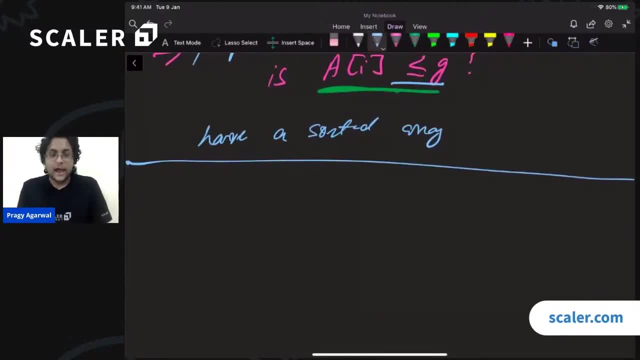 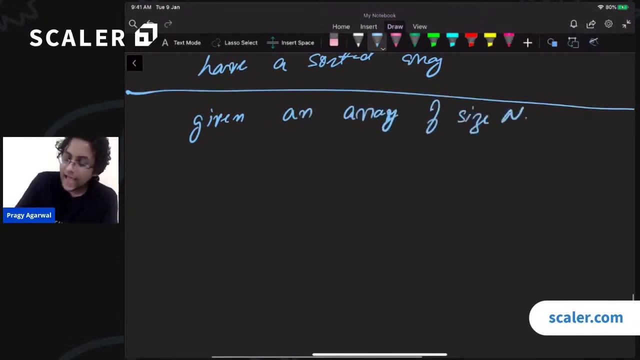 So let us let us dive into some more concrete things and let us try to look at the implementation of binary search Right. So, once again, suppose that we have been given an array Right Of size n, and this array is of integers, of integers right. 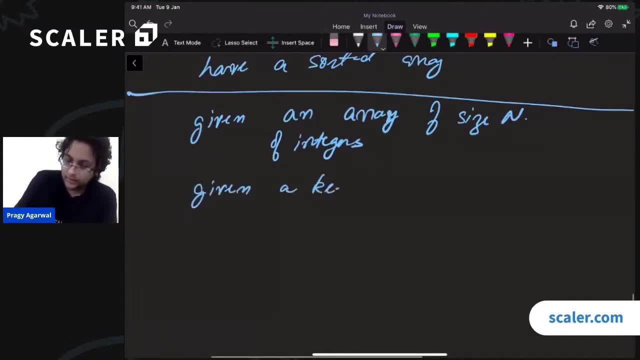 And we are also given a key, suppose k, that we are looking for, that we are looking for, And for now, let us suppose that the array is sorted in ascending order. Right Then, how then? what we have to do is we have to search the element. we have to find, find. 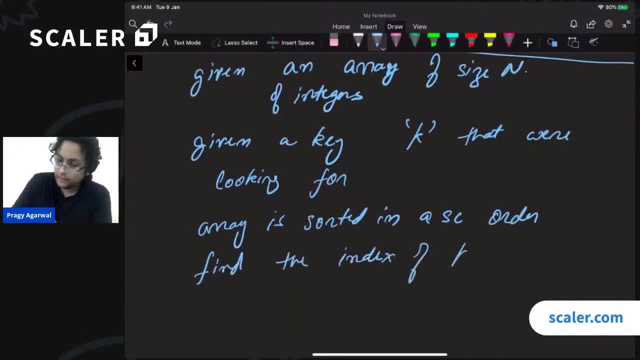 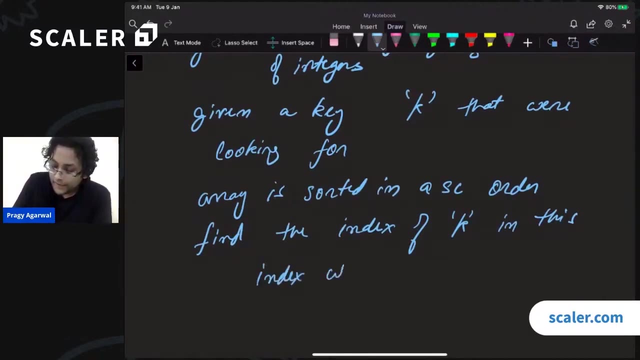 the index index of k in this array. if it exists, right. If it exists in the array, then we are supposed to find the index and return the index. otherwise, what we are supposed to do is we are supposed to return the index index where k should. 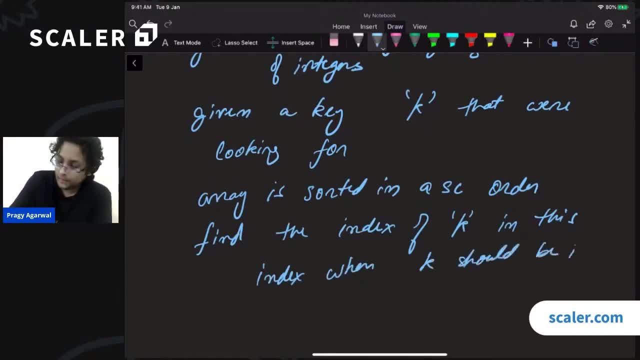 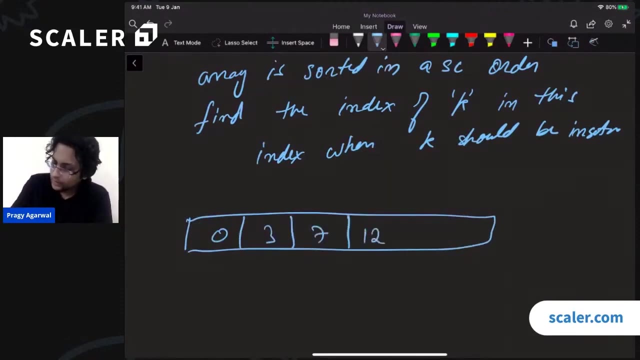 be inserted. k should be inserted Right Inserted in the array. Is that clear? Yes, Is that clear. So, once again, suppose that we have an array that looks like this: 0,, 3,, 7,, 12,, 15,, 16,. 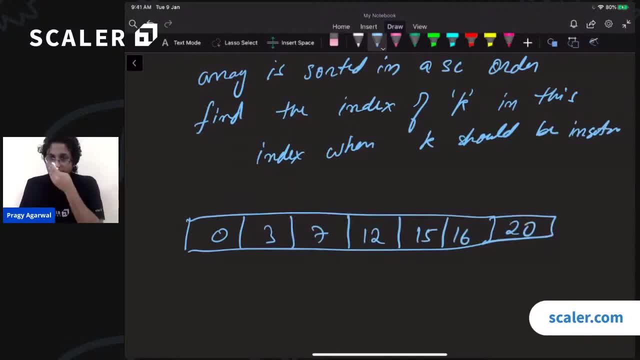 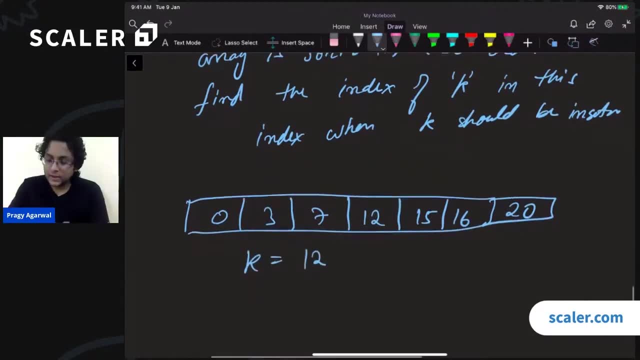 20.. Right, And I give you the key. let us suppose 12, right? So in this case, what are you supposed to do? So let me give the index as well. This is 0, 1,, 2,, 3,, 4,, 5,, 6,, 7,, 8,, 9,, 10.. 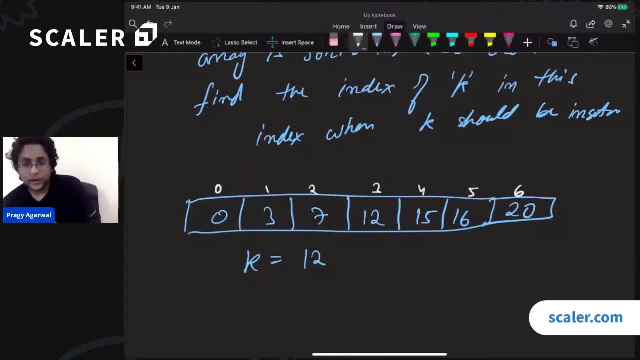 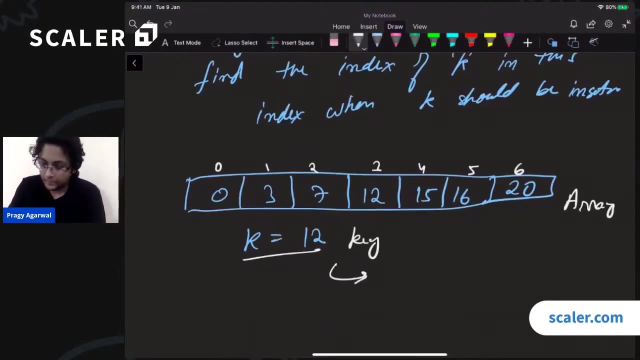 3, 4,, 5, 6.. So, in this case, what are we supposed to return? If this is the array and this is the key, then what value will we return over here? The answer we are supposed to return over here is the index 3, because 12 is at the 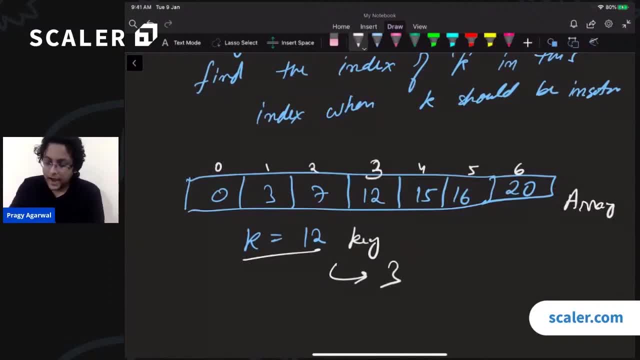 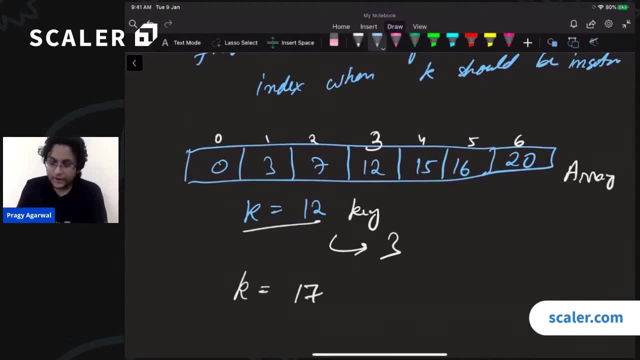 index 3. Right. On the other hand, if I ask you to find the value, let us say k equals to 17,. if I ask you to find the value, k equals to 17,. then what are you supposed to return? 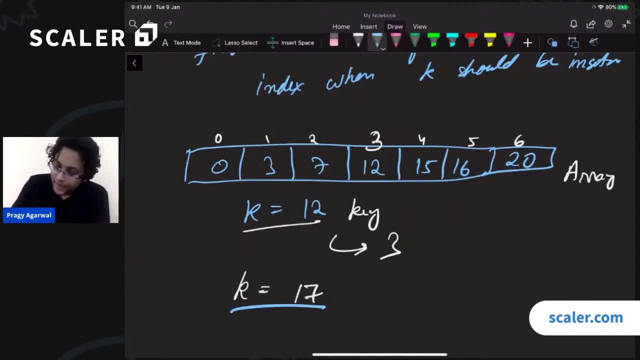 So there are multiple variants, right? In some cases, I might ask you to return minus 1, because 17 is not present in this array. I might ask you to return minus 1,, but that is what we are looking for over here. 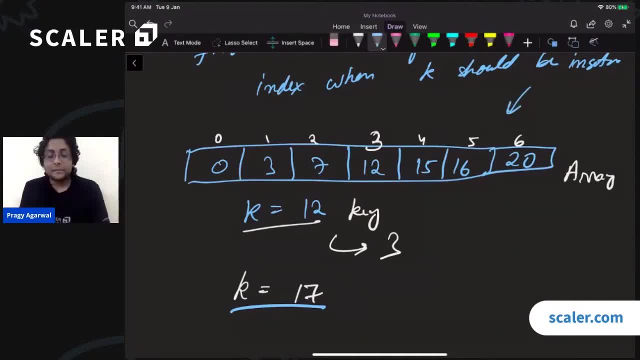 We are saying that if the value is not present in the array, then tell me the index where that value should be inserted, Right? So if 17 was inserted in this array, then what value, what index should it be inserted at? Should it be inserted at this location? 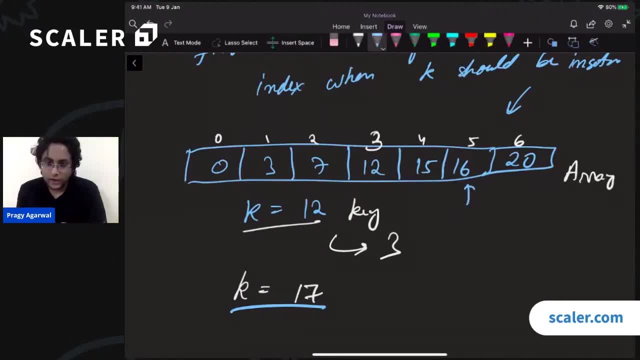 Should it be inserted at this location? No, it should not be right, Because 16 is less than 17.. It should be inserted at 20's position and 20 should be shifted to the right. Yes, 17,. if 17 was inserted, 17 would come in the sixth position and 20 will be moved. 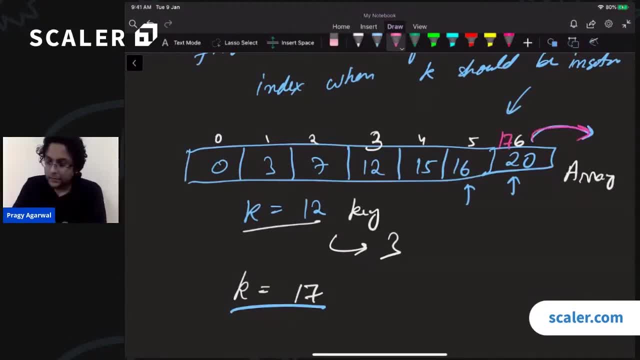 to the right Right. So if the search key is 17,, then you are supposed to give me back the answer. index equals to 6.. Is that clear, Right? Yes, So this is the classic. this is the classic problem of binary search. 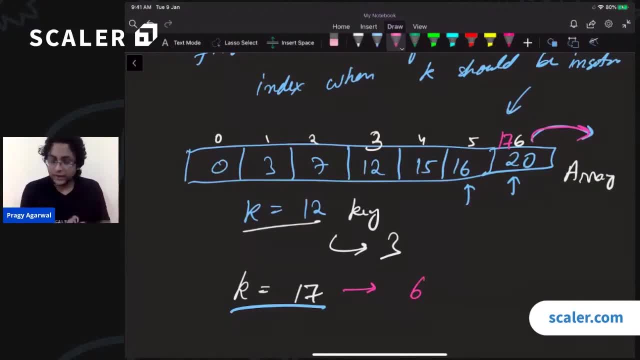 We have been given an array. we have been given an array which is sorted and we have been given a key and we have to search this key within the array Right Now. let us first look at the implementation of how we would do this binary search and 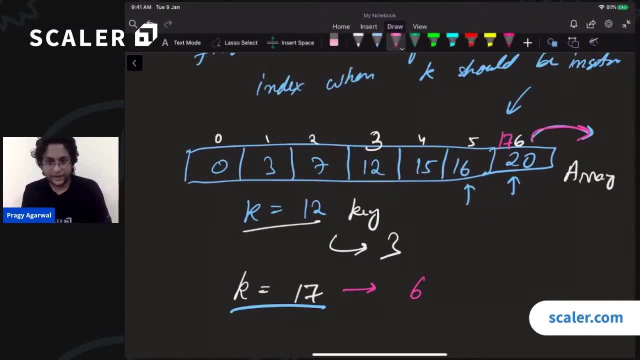 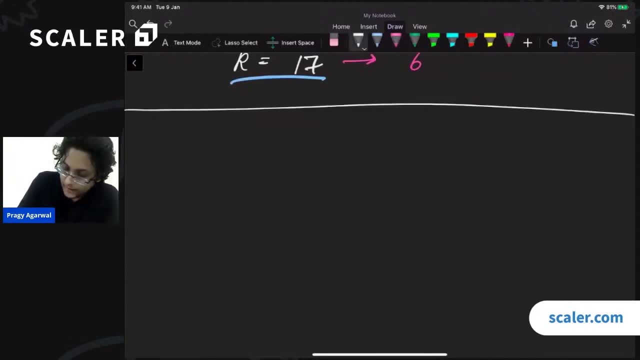 then we will discuss the time, complexity right and the corresponding analysis. Alright, So let us start with this thing. So suppose that we have this function: end, End Binary search And in this we are receiving a vector. We are receiving a vector. 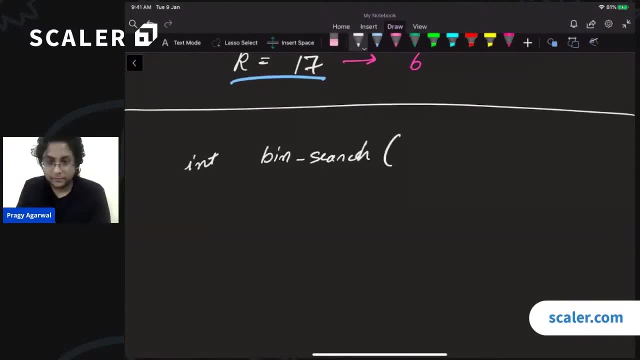 So we can say that, okay, we have a vector, a vector of end. Right Apart from that, we also have the key, So we have an end. So this is not a semicolon, this is a comma. We have an end key. 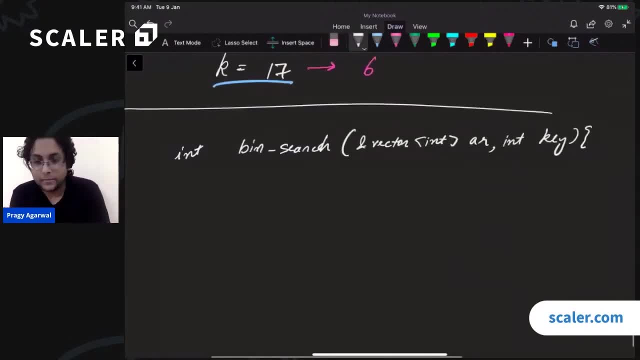 Alright, This is the function that we are going to write. Yes, Shukrata, Yes, in this case we are accepting a sorted array. Alright, we will come to binary searching over non-sorted arrays in some things. We are starting with the most simple thing. 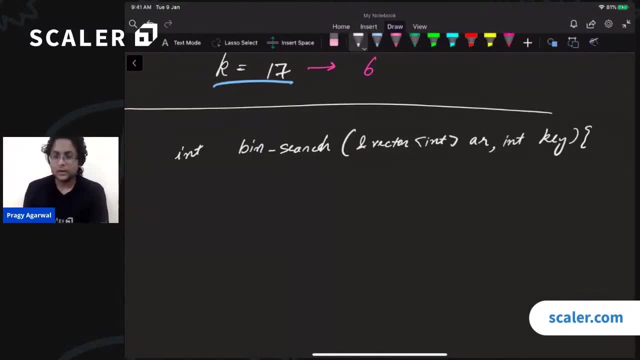 that the array is sorted, Alright, Cool. So how would we write this particular piece of code? So, when binary searching, when binary searching, there are certain things that we would like to identify. There are certain things that we would like to identify If. 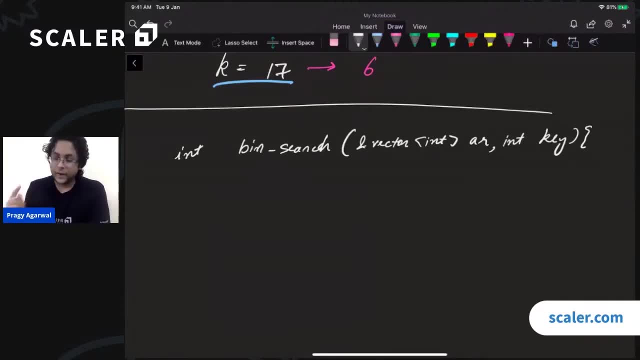 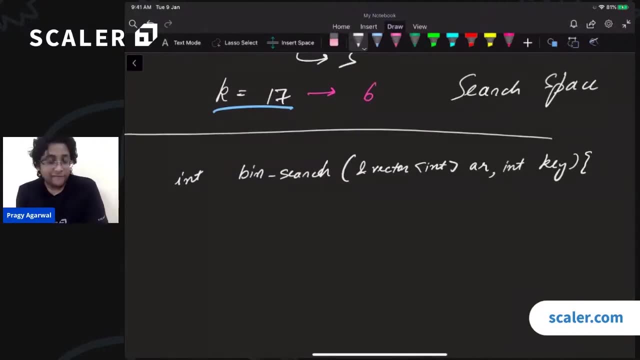 we are going to search. if we are going to search, then the first thing that we need to identify is our search space. Right, Is our search space? Now, if we have an array? if we have an array, then what do you think the search space is going to be? If we have? 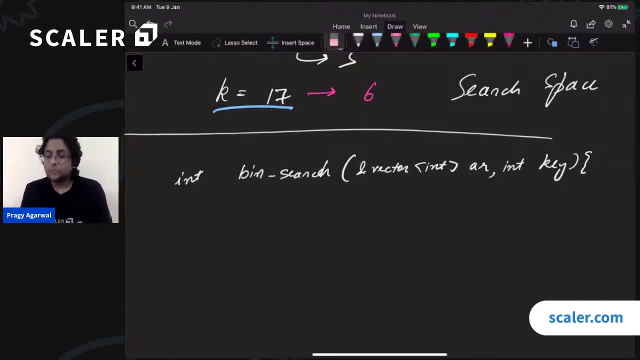 an array. then what is the search space? Well, the search space is all the possible different indexes in the array. Right, The value could be at index 0,, the value could be at index 1, and so on. the last index, so the search space is the indices of the array. well, what is the minimum value of? 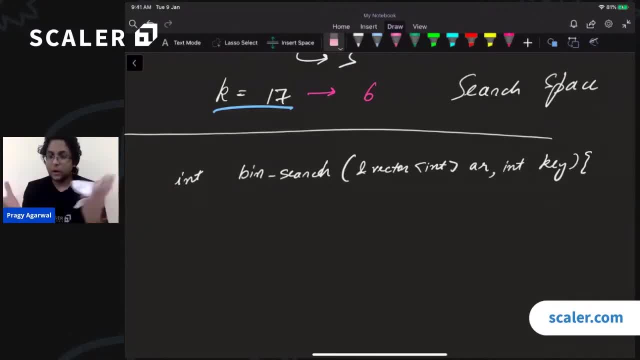 that search space and what is the maximum value of that search space? so can we somehow bound some? can we somehow draw a boundary? can we draw a boundary around that search space? yes, right, so in this case the boundary is from 0 all the way to n minus 1. 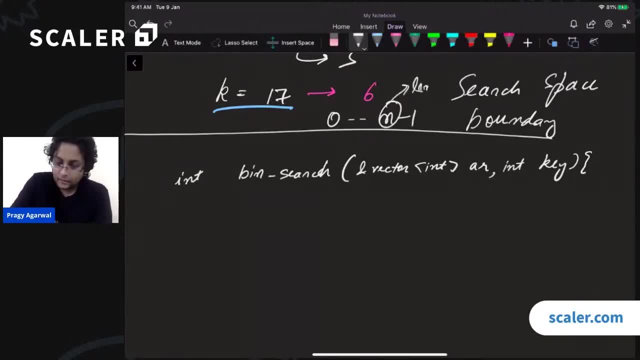 where n is the length of my array. is that clear? all right, so when i'm defining the boundary, i will, i will encapsulate, i will basically wrap my search space around this within this boundary. so i will say that, okay, let us suppose that we have some low right and that is the minimum possible value in my search space, and i also 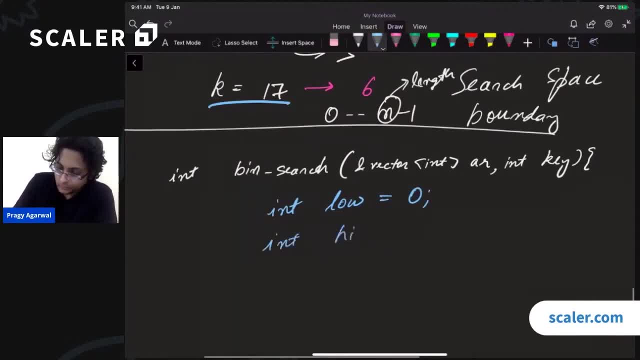 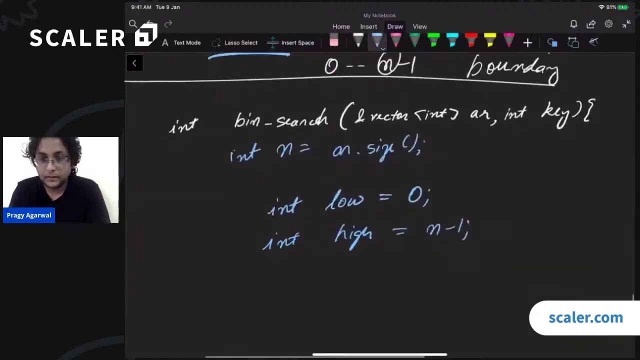 have some high and that is the maximum possible value in my search space. okay, and i can write over here that n is perhaps n equals to ar dot size. all right, cool, now that we have the boundary. now that we have the boundary, we are supposed to perform. 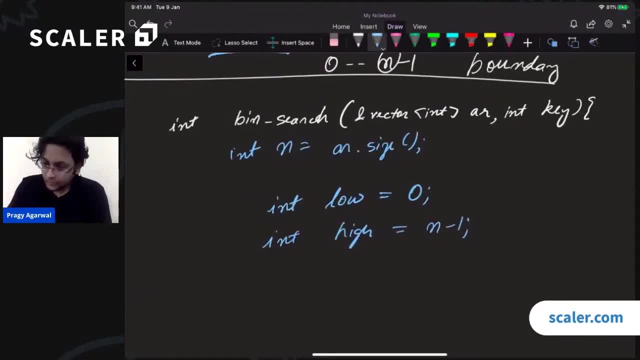 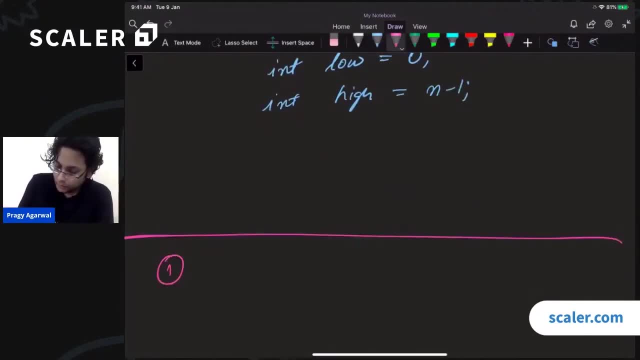 the binary search. okay, so there are. this was the first step of binary search. the first step of binary search was to to bound or to establish. establish, OK, the boundary of the search space. right, the second thing, once you have established the boundary. the second thing is to make a guess, to make a 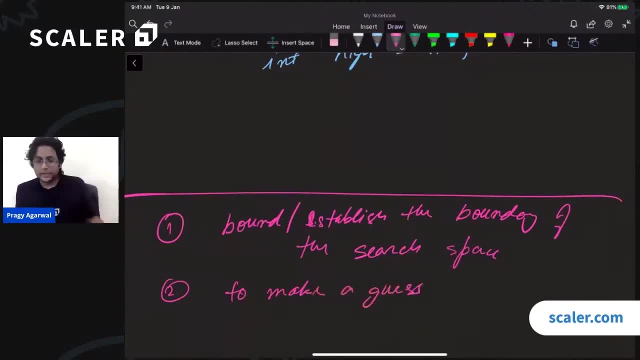 guess. so how do we make a guess? let us suppose that we have some search space and we want to make a guess. what guess do you think we should make? what guess do you think we should make? so we can make any guess, right, we can make any guess, right. 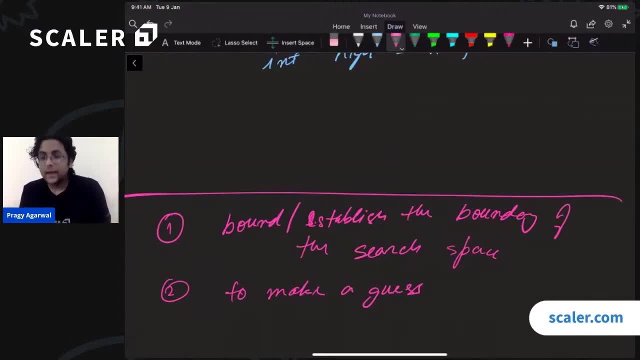 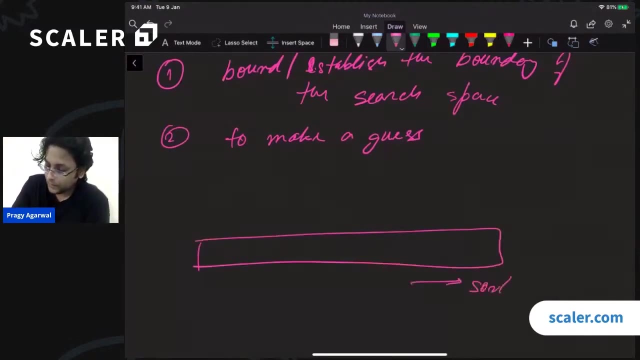 any guess. however, we should try to make a guess that allows us to eliminate a very, very large chunk of the search space, right? does that make sense? so, if I have this array, if I have this array and this is sorted right, and this is my low, this is my low and this is my high right, if I make this guess, if I make a guess, 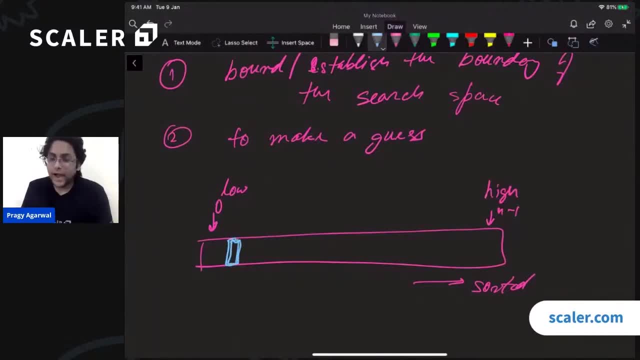 over here. then what will I be able to eliminate? what will I be able to eliminate? I will either be able to eliminate this part or I will be able to eliminate this part. yes, I will either be able to eliminate this left half- if my guess was too high, right- or I will be able to eliminate this right half. 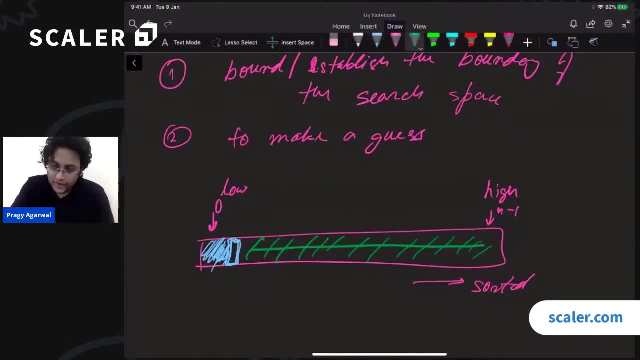 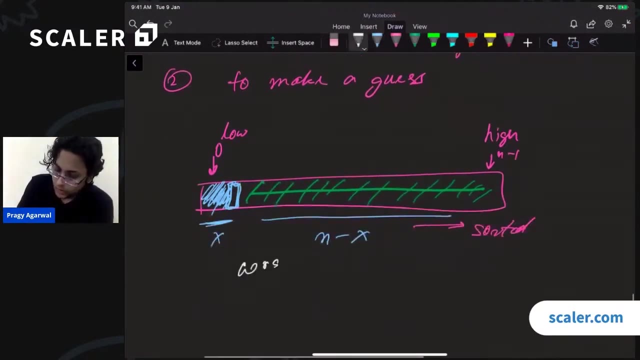 entirely, if my guess was too low. now, what is this value? what are these values over here? what are these values over here? let us say that this is X, then this will be n minus X. right now, the question is: in the worst case, in the worst case, worst case, right, if I'm very, very unlucky, then 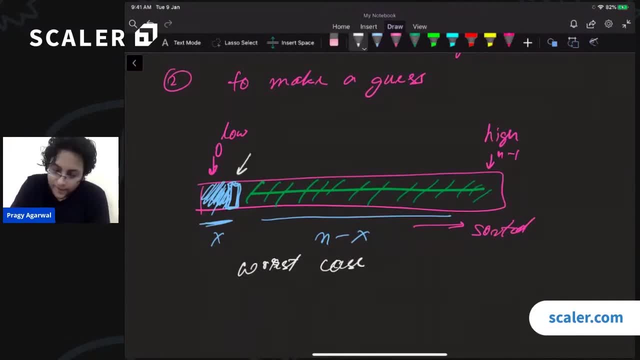 my guess will be: on this side, I will be able to eliminate a smaller value. I will not be lucky. I will not be able to eliminate a very large value, right? so I should try. I should try to make it so that. I should try to make it so that X. 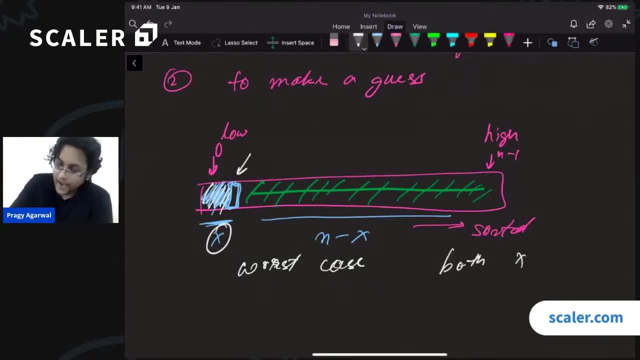 is as large as possible. right, both X and n minus X are as large as possible. right. so that? so that, no matter whether I'm lucky or not, I am able to eliminate a large chunk of my search space, right? so what? what guess should we make over here? we should. 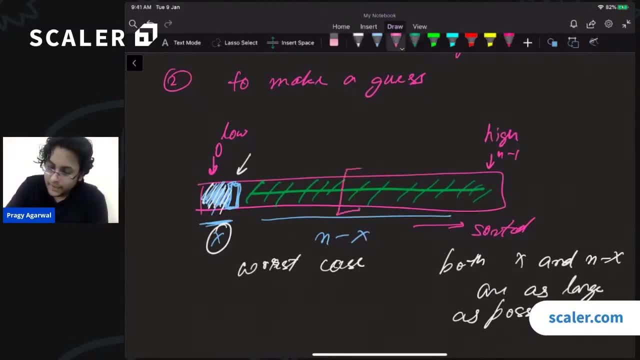 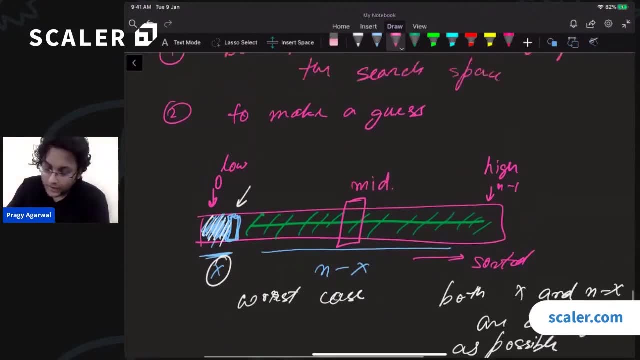 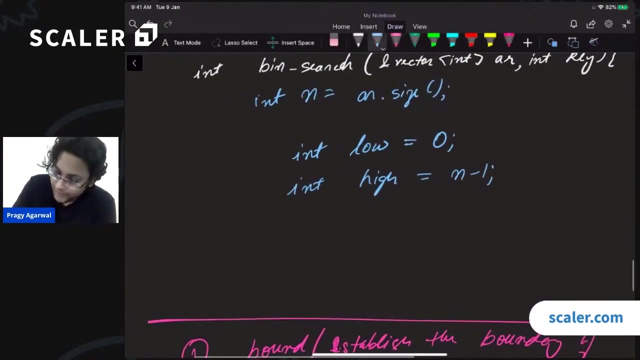 perhaps guess the middle element. we should perhaps be guessing the middle element. is that clear right. so this is the second thing: once we have, once we have decided the search space, once we have the low and the high, now we are supposed to find a mid right. so we will guess a mid. so we 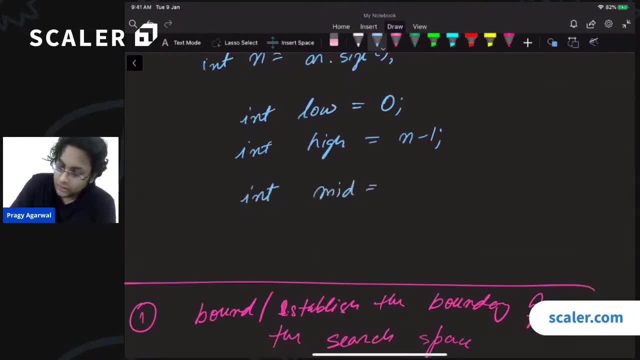 will say: int mid equals to low plus high by 2. right, and notice that this is integer division. this is integer division, all right, cool. so is this part here? is this part here? so is it in this part here? is this part here. so let us analyze the. 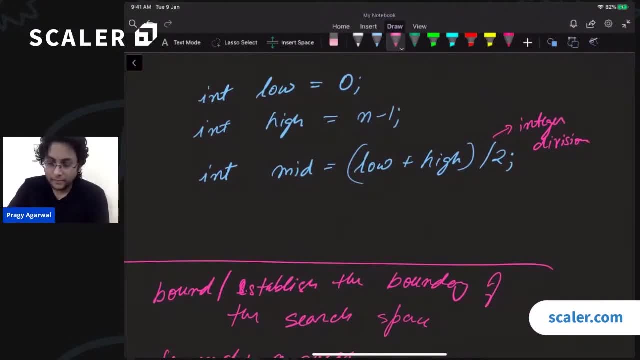 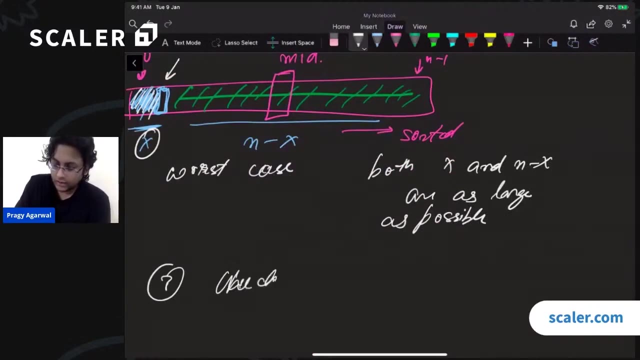 this part here is this part here. so let us analyze the that we calculate the mid on it. once we have the main, once we have the mid, then what do we do? once we have the main, then what do we do? the third step is to check the proposition. check the proposition, proposition and through right and prove. 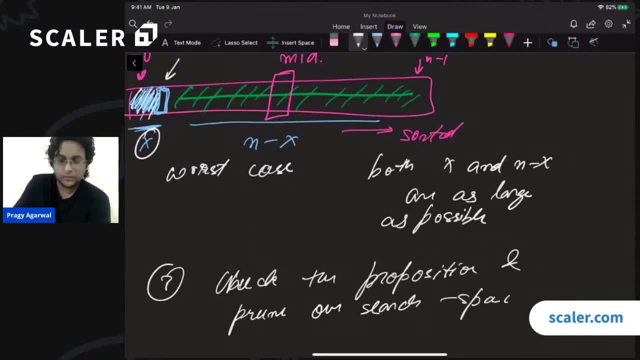 our search space. now the proposition can. the proposition can be either true or false. the proposition can be either true or false. however, in most of the cases, we can have three values. we can have three values: either my guess is too high, or my guess is true, or my guess is exactly correct. so let us let us look in this: 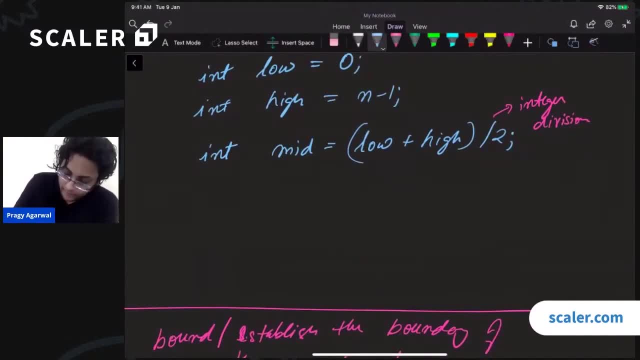 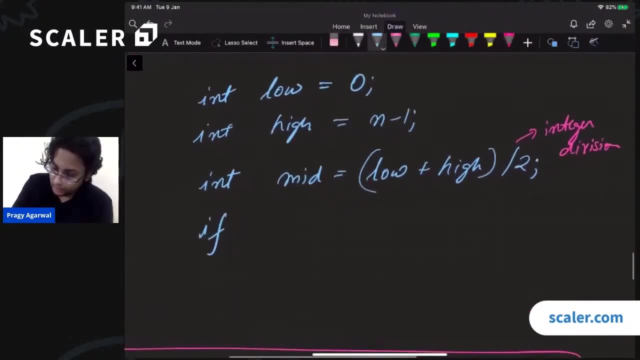 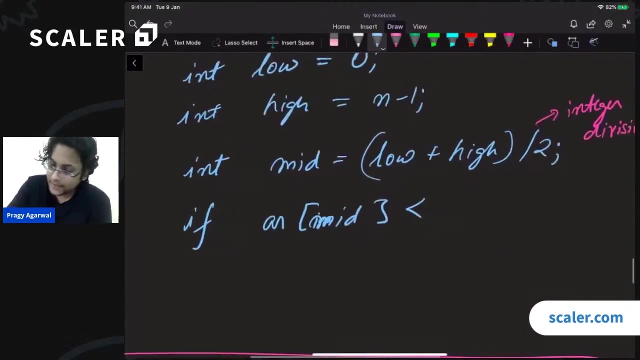 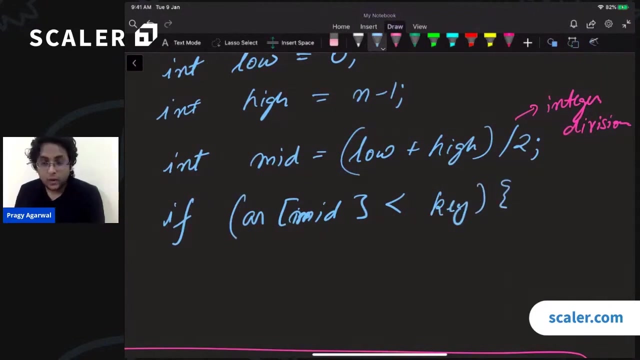 case. let us look at that in this case. so, if so, what possibly can I have over here? what possibilities can I have over here? if AR of mid, if AR of mid is less than the value I'm looking for, is less than the key, if AR of mid is less than the key, then what does that mean? is my guess too high, or? 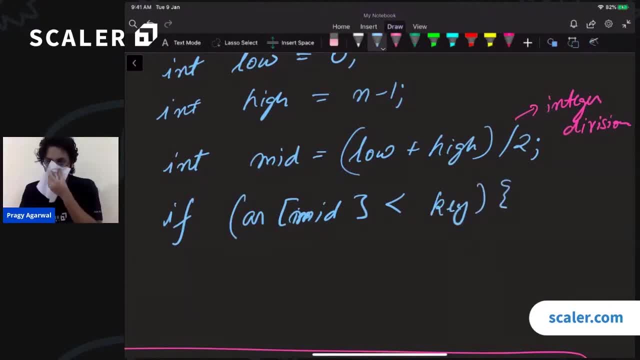 is my guess too low. if the location that I'm looking at, I'm looking at the location mid, if the arranged relation was less than the key, then is my guess, is my guess too high. I'll is, like us two, low when the element was less than the element I was. 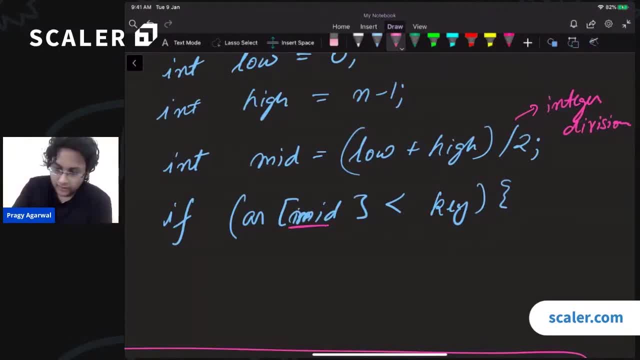 So the array came from iCard. now this is pretty secure and I can try to use it looking for. so I am sure that since the No is sorted, since the array is sorted, any value, any value that is at AR of, let's say, zero or AR of mid minus one. 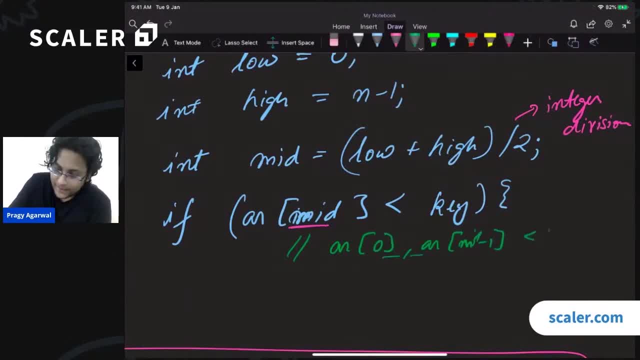 any value, any value, any value that is at AR of, let's say, zero oar, AR of mid, minus one, right, but minus one. all these different value are going to be less than the case. well blessed, because the alcoholic so many bet, is my thought. so my guess was to make. this was two row, so all these 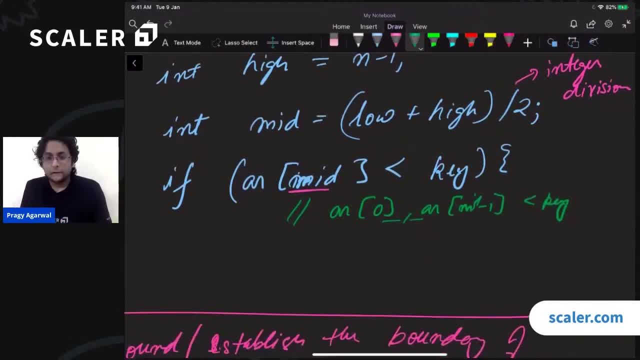 that's what I have. so, all right, there is my guess, so I like of my guess. because there is my guess, so I like of my guess. if to get this comments back then where guess was too low. so what should we do? we should adjust something right. we should adjust the source. 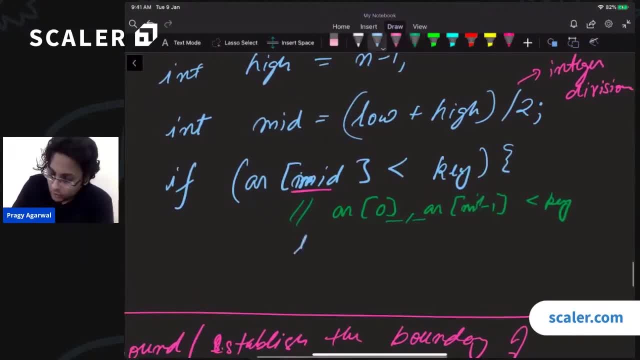 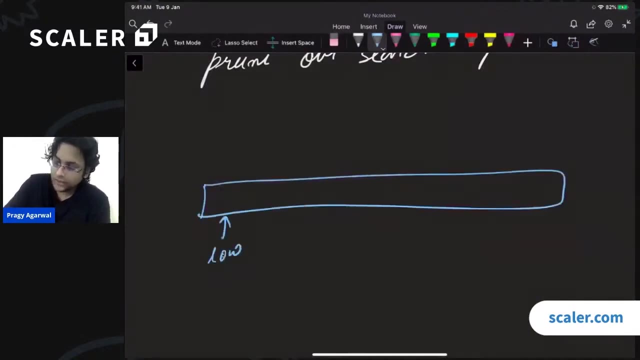 space. how should we adjust the search space? we can say that low equals to mid, this one right. mid, that's one right. so basically, earlier this was the search space, this was low and this was high right, i made the guess admit. i made the guess admit and i found out that this guess was. 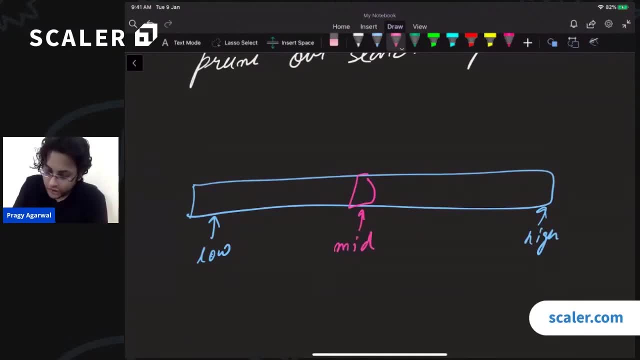 too low. right, this guess was too low, so what should i do? i should, i should shift this low. i should shift this, though, to the element just right of it. right, so this element should now be low, and basically, by doing that, i am eliminating all these different possibilities, right, i am? 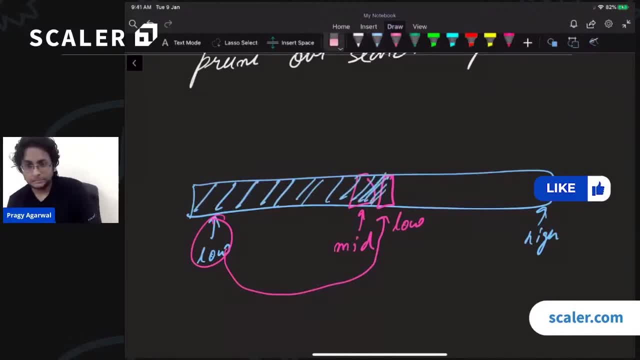 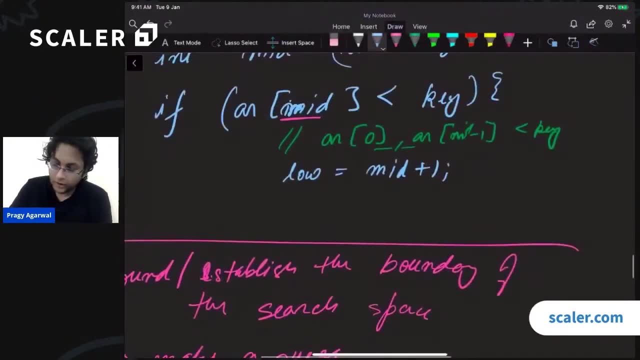 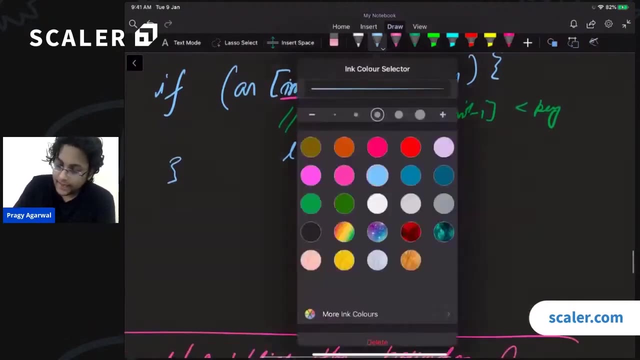 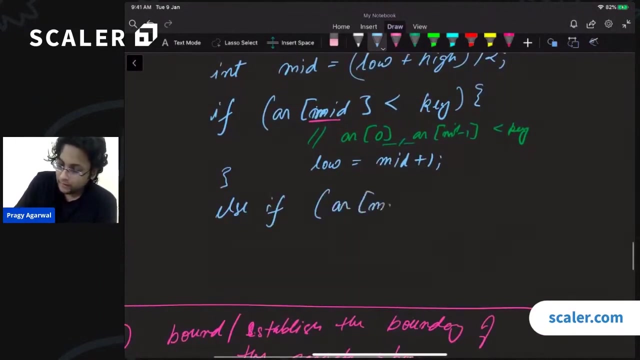 eliminating all these different possibilities. is that clear? so we should move up the loop. is that clear? we should increase the low. all right, so that is one case. so what other cases can we have? what other cases can we have else? if else, if ar of mid was greater than key right, if ar of mid was greater than the value i am looking for, 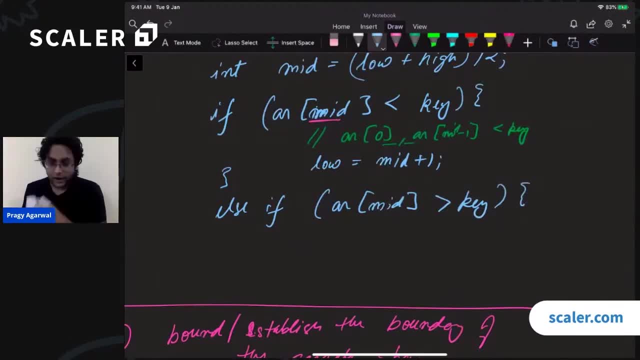 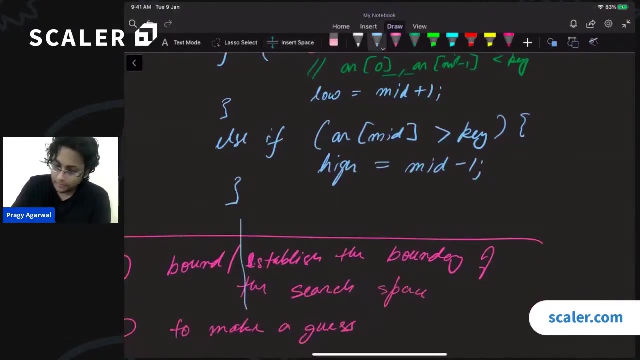 then what happens when my guess is too high? and by the same argument, now i need to decrease the high, and now i need to say: high equals to mid minus one right. otherwise, if even that is not the case, then what possibility remains? if it is neither too high, if it is neither too high nor too low, then what possibility remains? 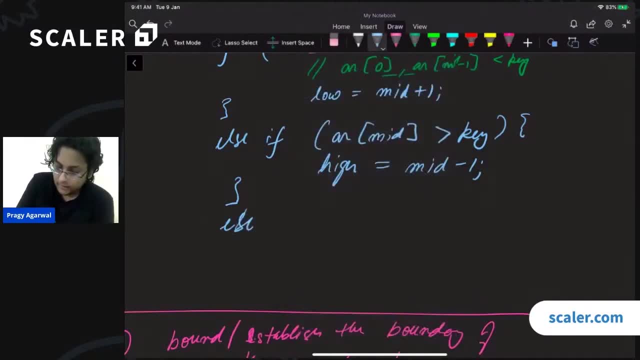 then it must be exactly correct, right, else else my guess was exactly right, right, i guess the perfect answer. so in that case i can just return. i can just return the index right, because i i looked at this particular index, ar of mid. i looked at this particular index and i found a value that was exactly equal to the key. 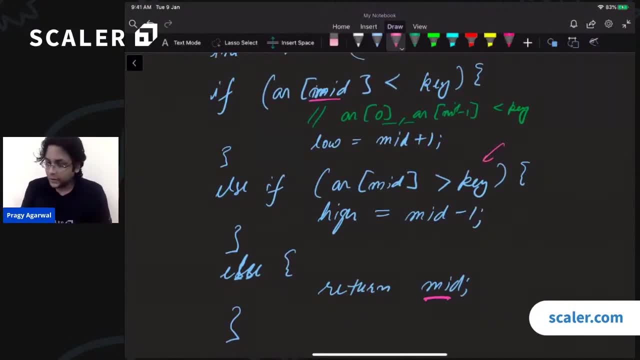 right. it was neither greater than key, it was not less than key, so it must be exactly equal to the key. so i can just return this index, because this is the index that i am looking for. is that clear? yes, perfect, now, let us now. let us look at the code that we have and let us see if 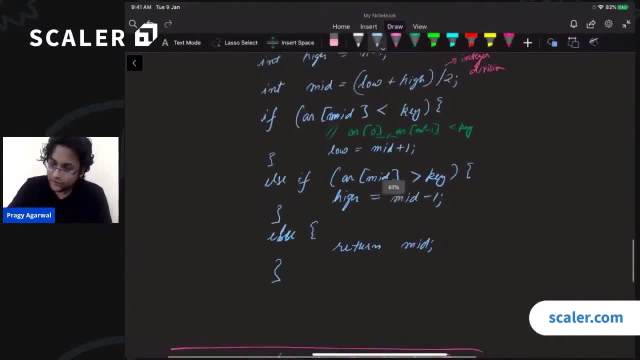 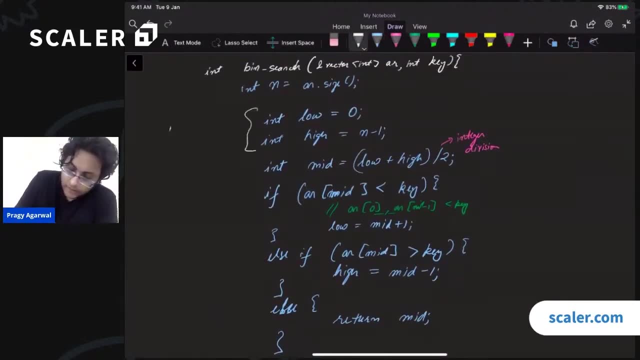 there is something missing over here. let us see if there is something missing over here, right, let us see if there is something missing over here. so, once again in the code, what we are doing is we are saying: let us initialize the search space, initialize space. right, then we 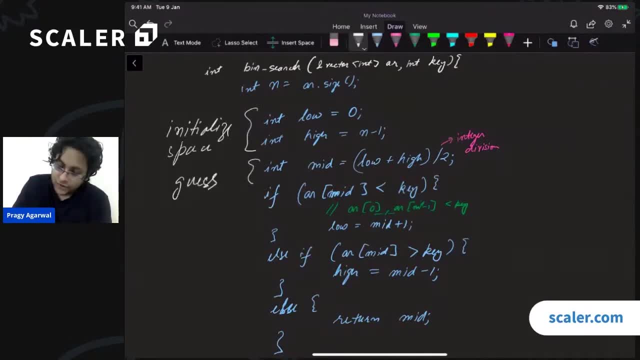 make a guess. so this is our guess, and based on the guess, we adjust the search space. so will we be able to after one adjustment? after one adjustment, will we be able to reach the answer? will we be able to reach the answer after just one adjustment? no right, we have to continuously adjust our guess. 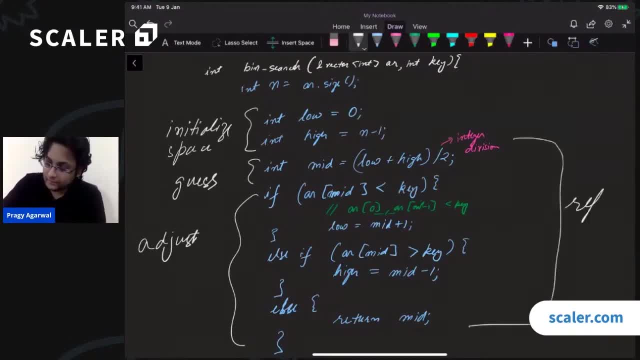 right. so we have to do this entire thing again and again. we have to repeat this, right? we have to repeat this entire thing. so how should we repeat this entire thing? let us put it inside a loop. let us put it inside a loop, so let me add some space over here. 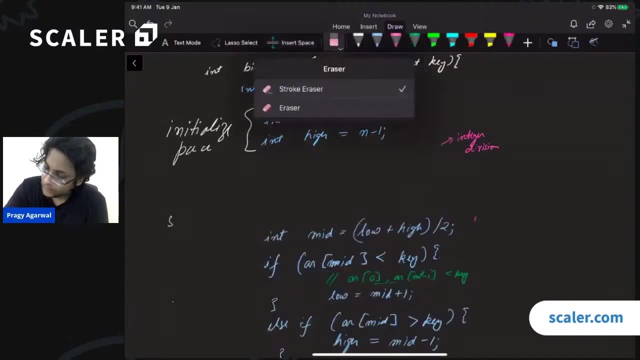 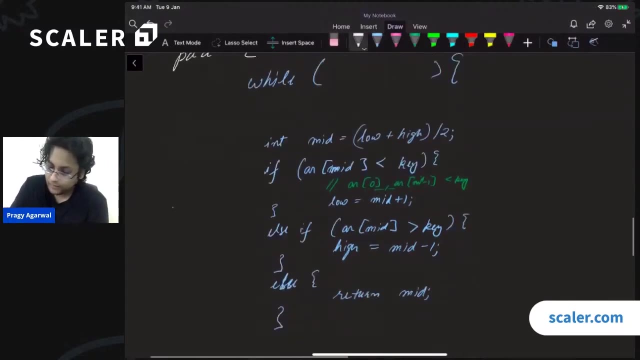 and let me say: right, let me say i will loop. let us say i loop forever, right, while some condition. so i don't really know what this condition is, but as long as this condition is true, i will keep looping. right, i will keep looping till this condition is true. is that clear, right? so we 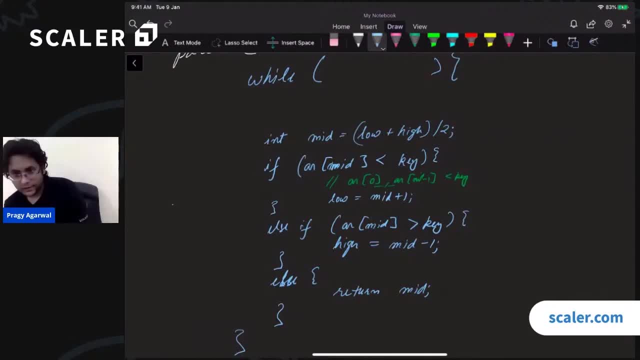 could have done several things over here. we could have called this function recursively as well, right, based on the adjusted case. we could have called this function because of the as well. but recursion will have a lot of different issues with itself, so it will. it will use a lot of. 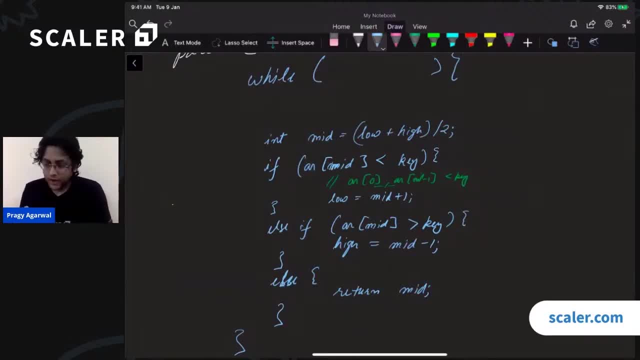 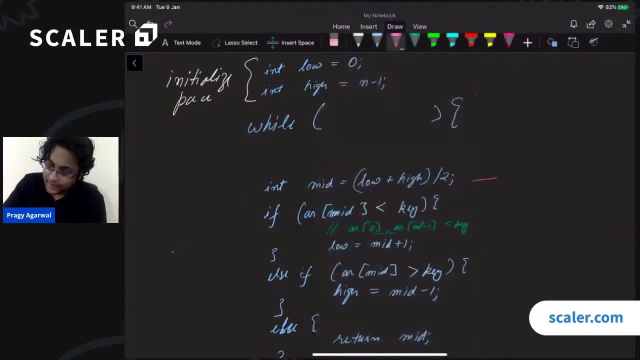 memory because it will use the recursion stack, so we'll keep looping till this condition is true. So let us not do that. Let us go with the iterative approach. So once we have made a guess, once we have made a guess, and we check the guess after. 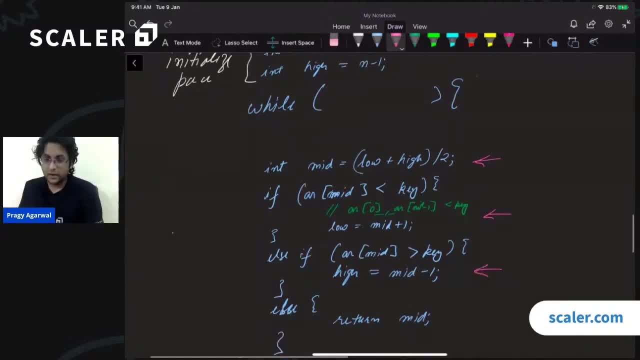 we check the guess, we will adjust our search space. Now, once we have adjusted the search space, what do we have to do again? We have to make the guess again. We have to make the guess again and again. But till what time should we continue this? 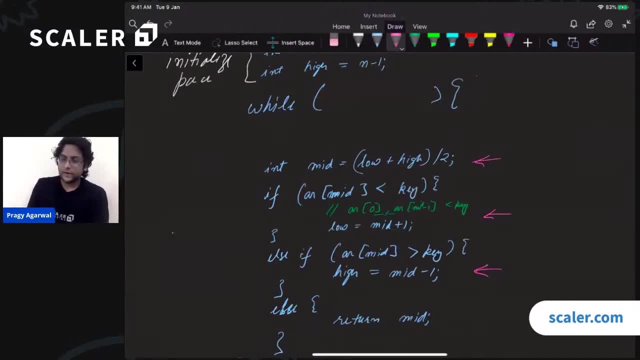 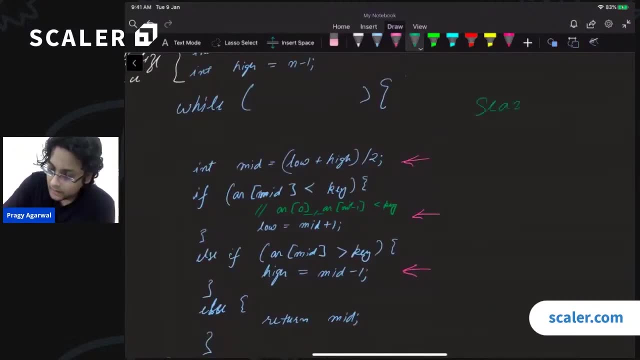 Should we continue this forever and never? No, we should only continue this as long as our search space has elements in it, If our search space has elements in it. So basically, if our search space is empty, then it does not make sense to keep looking. 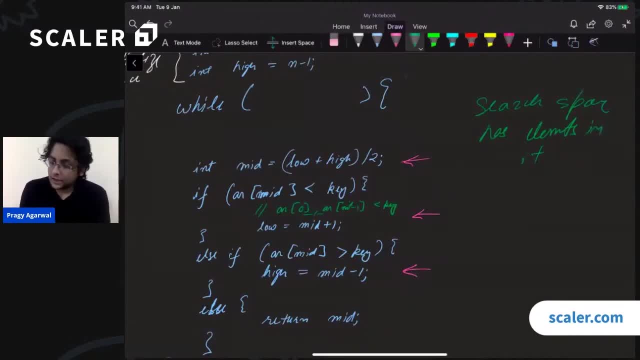 inside that search space. If our search space is empty already, then it does not make sense to keep looking inside that search space. So when will our search space be empty? When will our search space be empty? Let us suppose that this is my array. 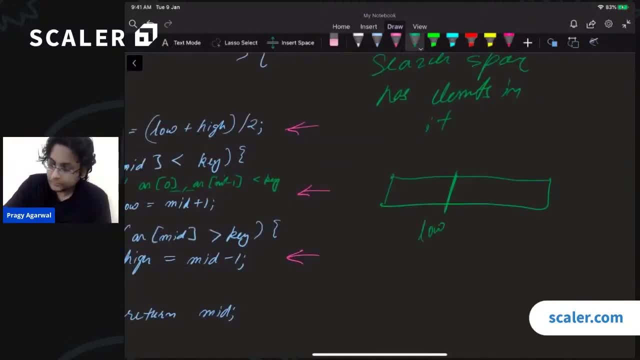 Let us suppose that this is my array, This is the low and this is the high. At what point would I say, for what values of low and high? would I say, that my search space, that this particular area, this particular range over here, this is empty? 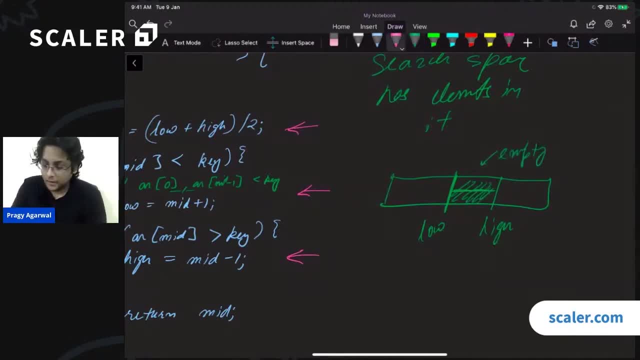 When will I say that? What happens when low equals to high, When low equals to high, When low equals to low and high are the same? What happens when low and high are the same? Well then, my search space is not empty. 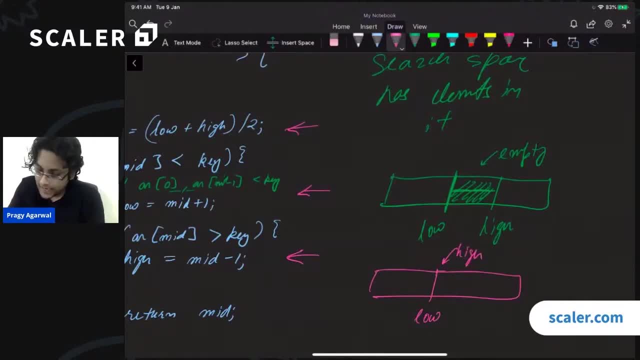 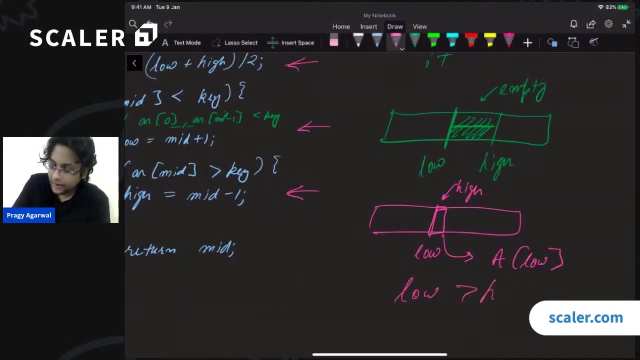 Then my search space has one element which is A of, which is A of low. If low equals to high, then my search space has one element which is A of low. So when will my search space be empty? When low will be greater than high. 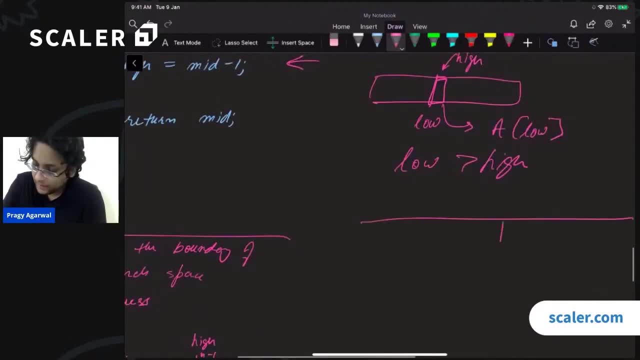 Yes, As soon as this happens, as soon as this is my low and this is my high, then my search space will be higher. Then I am saying that the search space is everything that starts from low and goes till high. Well, it cannot go till high. 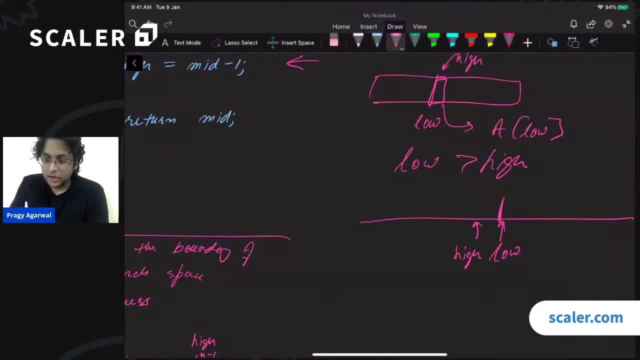 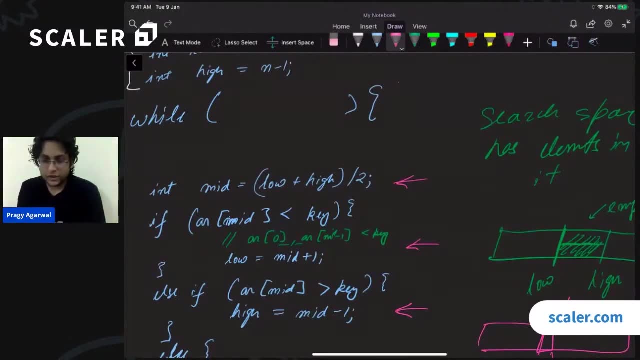 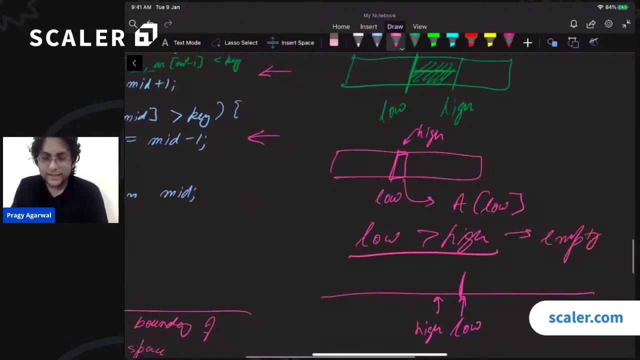 My search space is empty. now Is that clear? So I am supposed to continue this loop till my search space is not empty. So what will be the opposite condition over here? What will be the opposite condition over here? So if this tells me that the search space is empty, then how do I check if the search 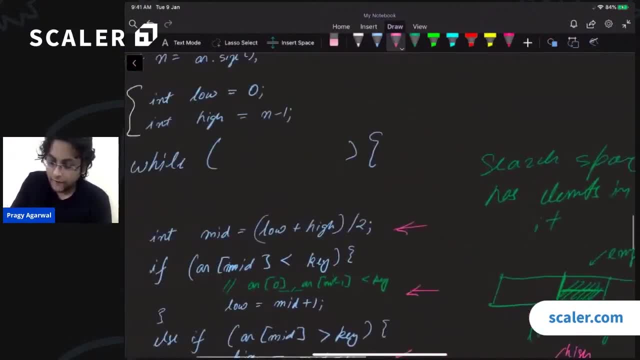 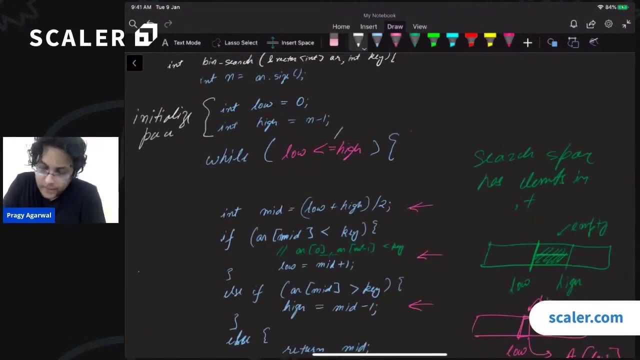 space is not empty. I will check it by saying: while low is less than or equal to high, Is that clear? Yes, Right, And this is very important, right. If you miss this equal to, if you miss this equal to you, might, you might get an incorrect. 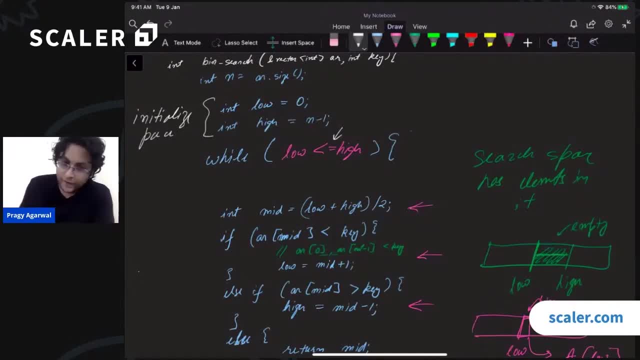 answer right, Or if you. if you do something else, you might run into an infinite loop. So it is very, it is very crucial that we have this condition right, Because this condition tells us when to terminate. It tells us when our search space is empty. 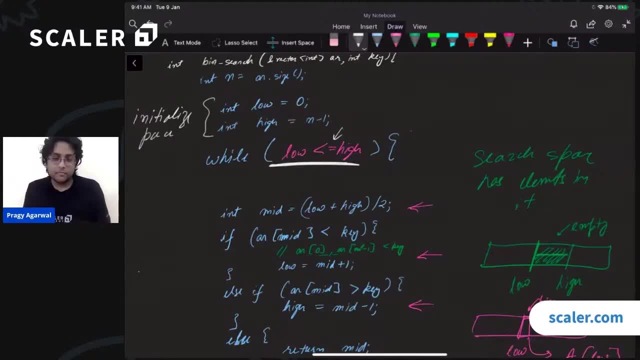 Okay, And I mean. a lot of the times people are worried that, okay, I don't really know how to, how to determine what condition should go over here. So here's the trick, once again, to determine what condition should go over here. you have. 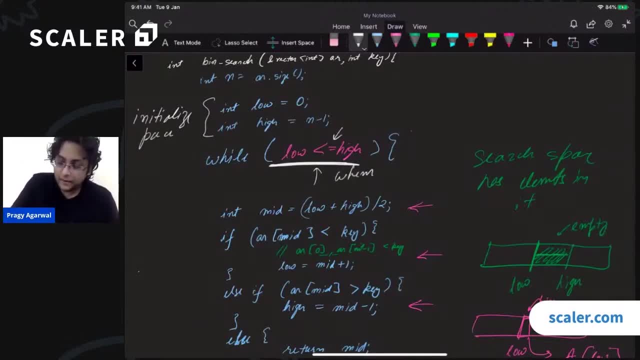 to ask yourself: when will my search space be empty? When will my space be empty And, based on that, you will be able to come up with a condition. Right Cool, So this is basically the code of binary search. This is basically the code of binary search. 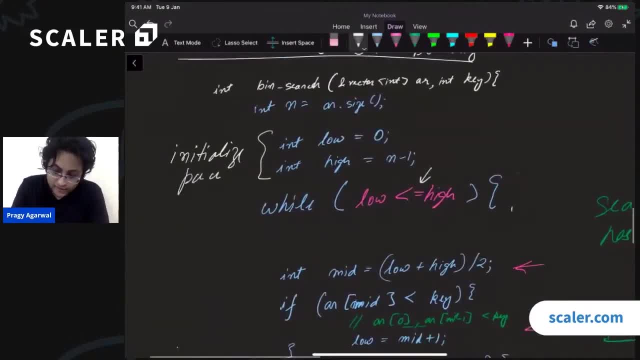 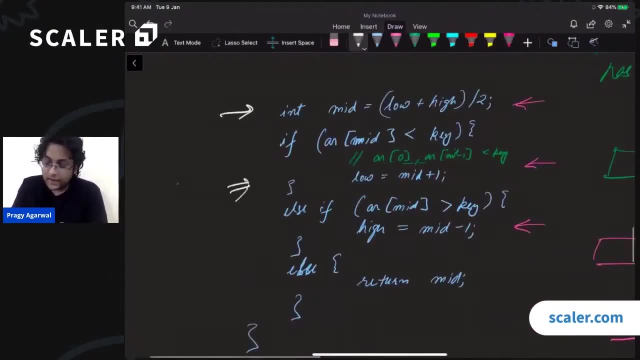 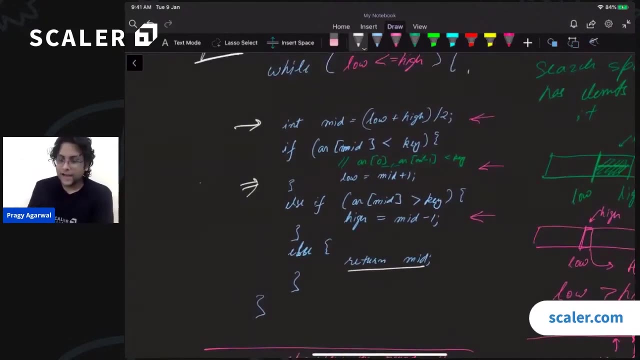 We started with. we started with a search space repeatedly, while the search space was not empty, We made a guess and we adjusted that to guess right. If our guess was perfect, we simply return that guess. we simply return that guess. But what if? what if we did not find that element? 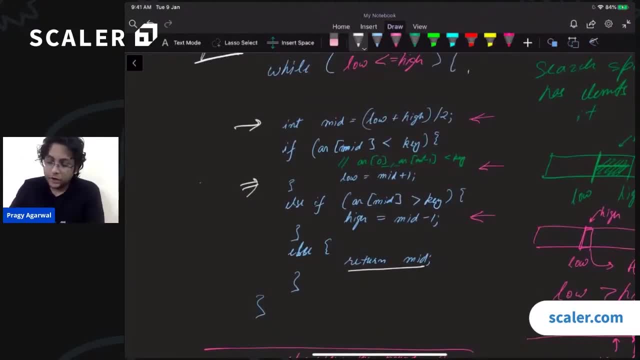 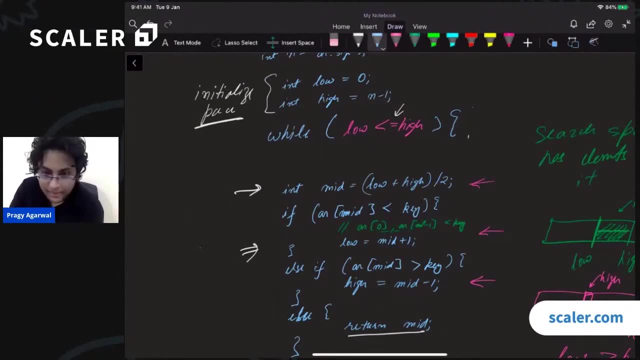 What will happen then? What if we did not find that element at all? What will happen then? Well then, we'll keep on looping. we will keep on looping till the point our search space becomes empty, Right Till the point our search space becomes empty. 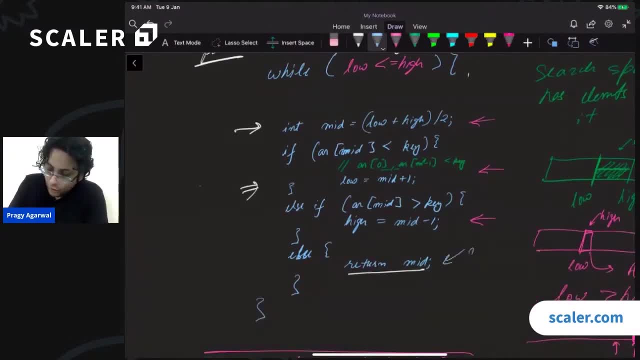 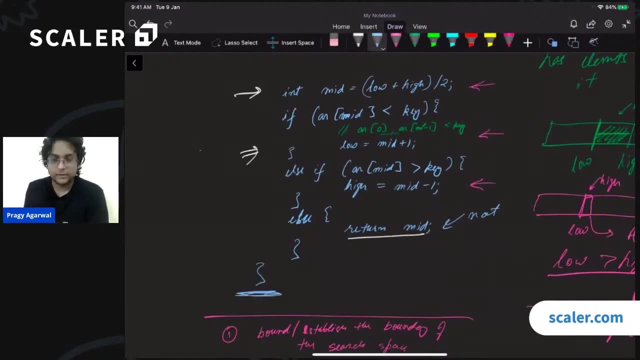 So what will happen is we will not be able to return over here. we will not be able to return over here. However, we will come out of this while loop. so we will come out of this while loop. we will be over here at this point. 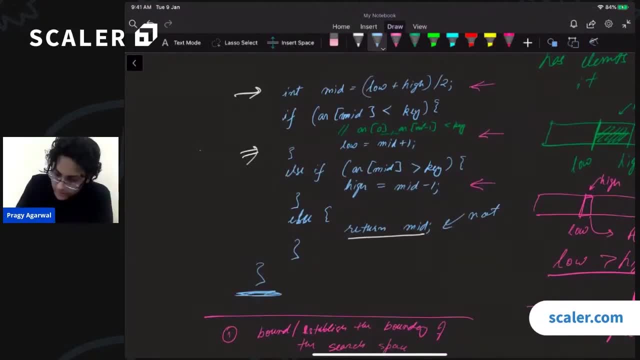 And what values of low and high will we have? We will have a value such that low will be equal to high plus one Right. That is when our search ends. Right. And what is this location? Can you tell me what this location is? 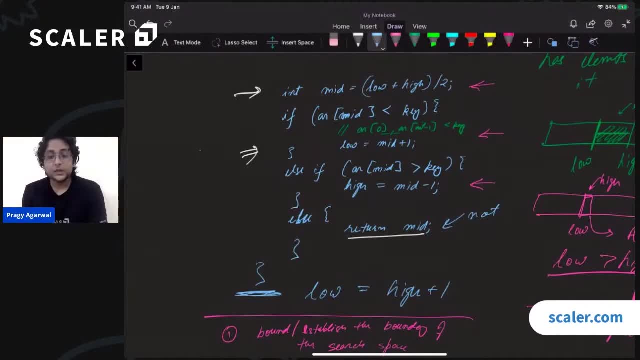 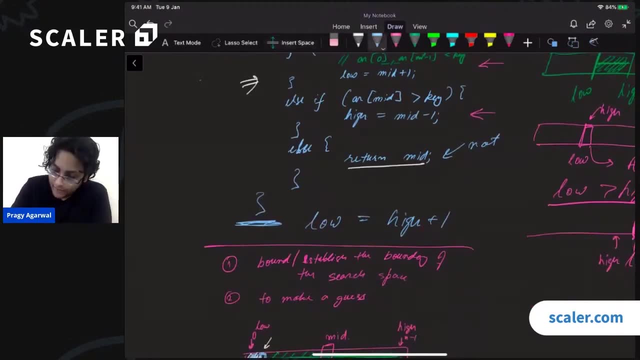 This location is exactly the location where I should insert this element. If I were to insert this element, this is exactly the location where I should insert this element. So, when I am at this point, just give me a second. when I am at this point, when I am, 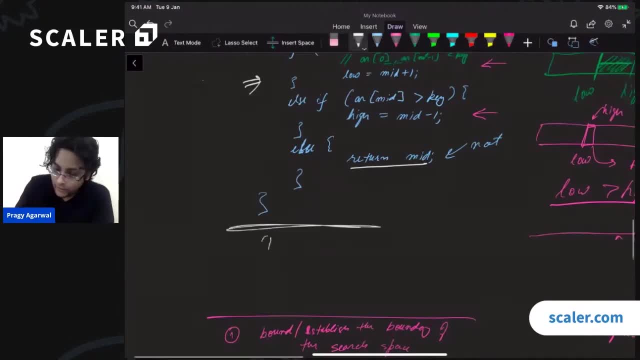 at this point, I know two things. I know two things. The first thing I know is that low is the index, the is the index where I should insert it. If I was going to insert it, then low is the location where I should insert it. 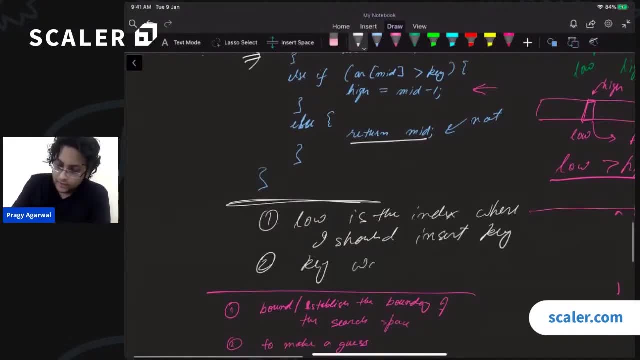 Second thing I know is: key was not found in my array. Key was not present, present in my array Right. Is that clear? Now, once again, if we were to suppose, if we were to simply find the index of the, if, 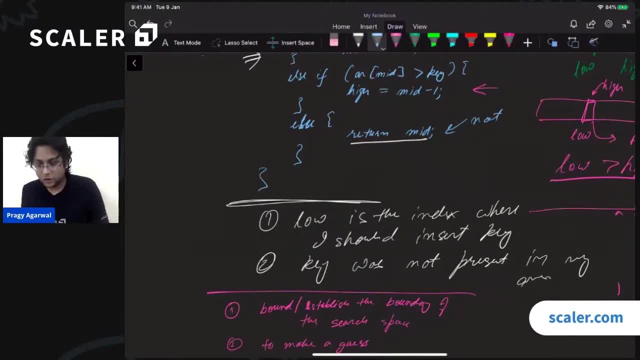 we were supposed to find the index of the key and return minus one. if the key was not present, then over here we will return minus one Right. On the other hand, more practically, whenever I see you, you see a library implementation. 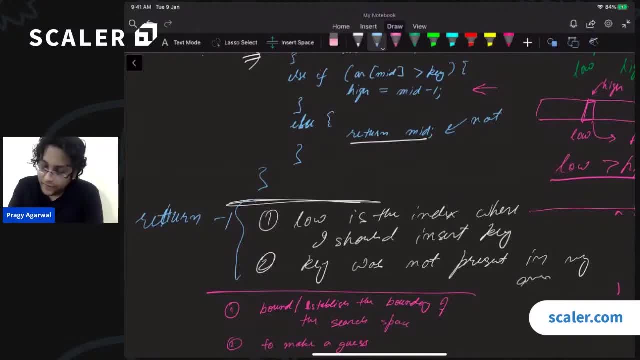 we don't usually return minus one. Instead, we return the index where I should have inserted the key Right. So over here we can also return the low, return the low value right, Because this is the location where I should have inserted the key. 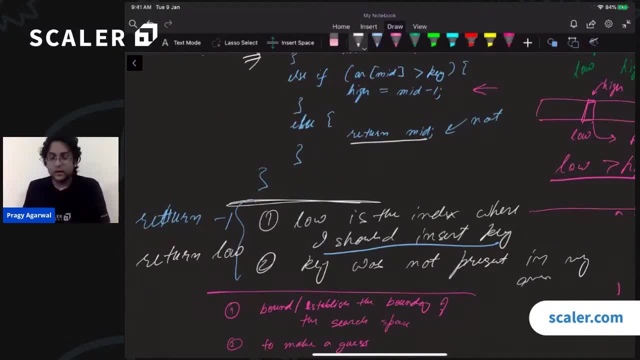 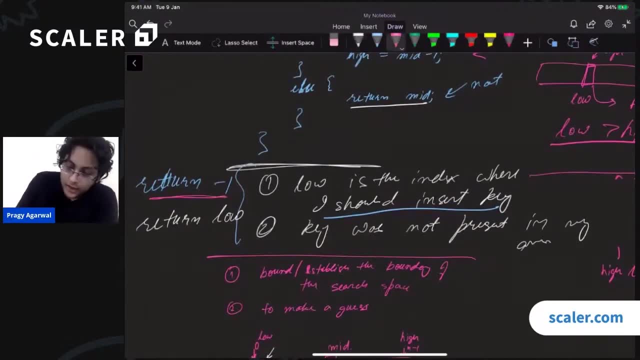 Is that clear guys? Yes, Now one common question is. One common question is: if you are returning minus one, if you are returning minus one, then your caller knows, then your caller knows that the element was not present, right? 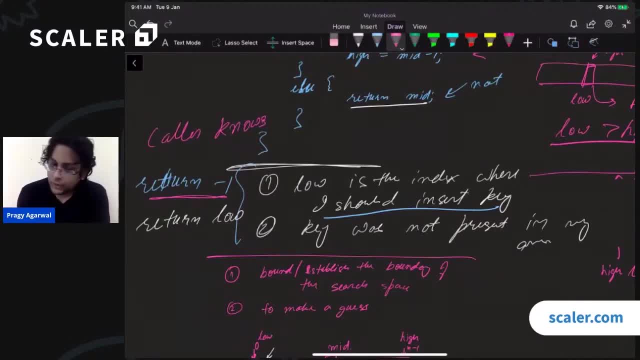 Because, hey, index cannot be minus one. Index of a particular value in an array cannot be minus one. Indexes go. indexes start from zero, right? So in this case my caller knows that the element was not present, but what if I return? 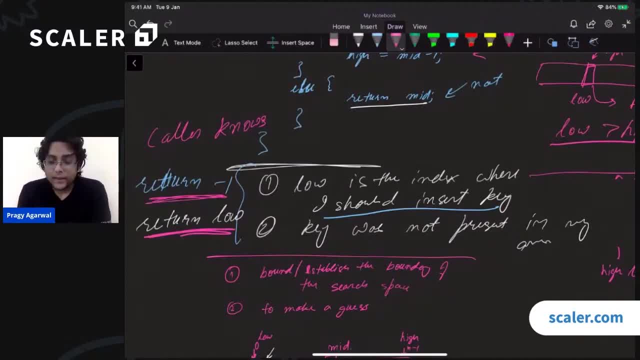 low. What if I, instead of returning minus one, what if I return low? How will the caller find out that the element was not present? How will the caller find out if the element was present or not? Yes, the caller has to be able to make that distinction, whether the element was present. 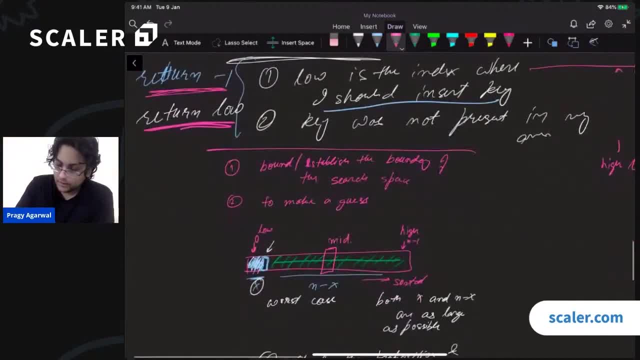 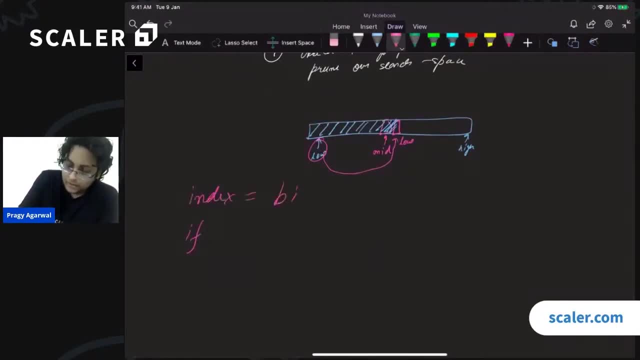 or not. So how will the caller get to do that? Well, the caller can check, the caller can simply check. So it will say that, okay, index equals to binary search, the array and the key right, And the person can check. 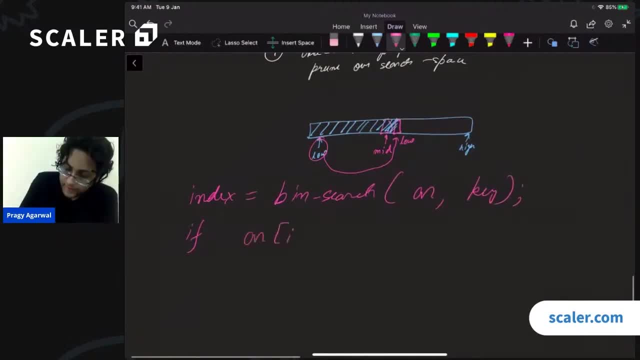 The caller can check. The caller can check if ar of index equals to equals to key right. If ar of index equals to equals to key, then we found the key right. Then we found key, found key at index right. 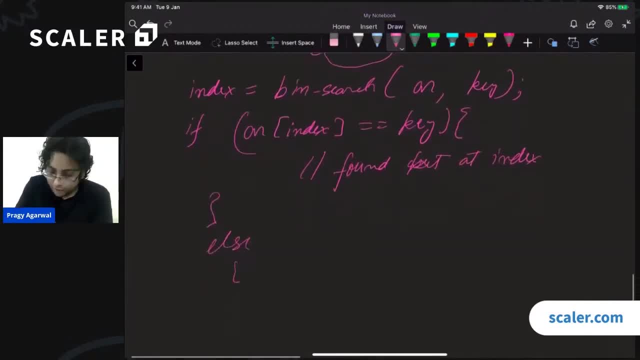 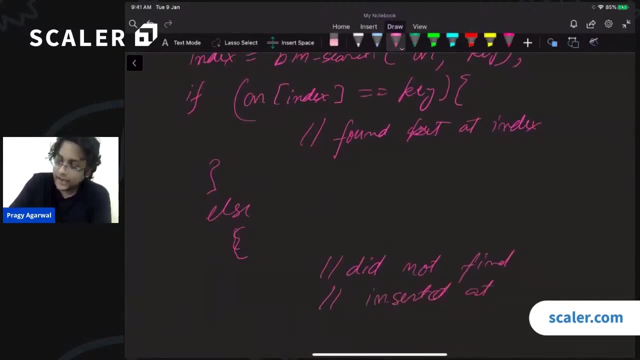 Otherwise. otherwise it means that we did not find the key, but this index is the location at which we are going to insert it, if we were to insert it. So we can say, did not find, did not find the key, But if we were to insert it, it should be inserted. inserted at index. 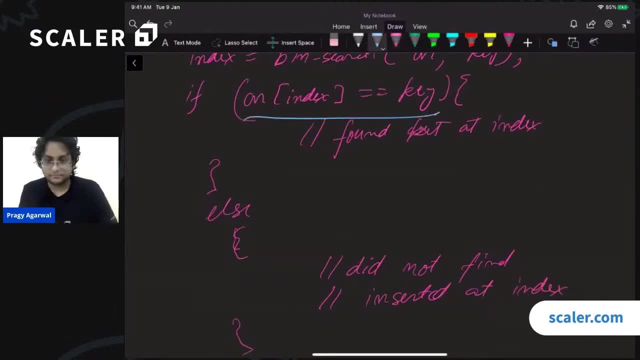 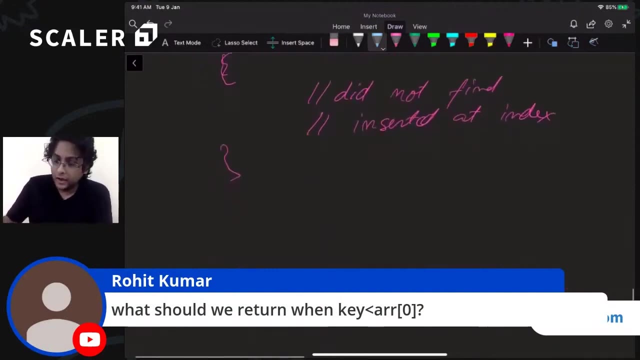 Is that clear? So the caller will have to make this additional check. Is that clear, guys? Yes, Okay. So Rohit has a question over here. Rohit says: what should we return? What should we return if key is less than ar of zero? 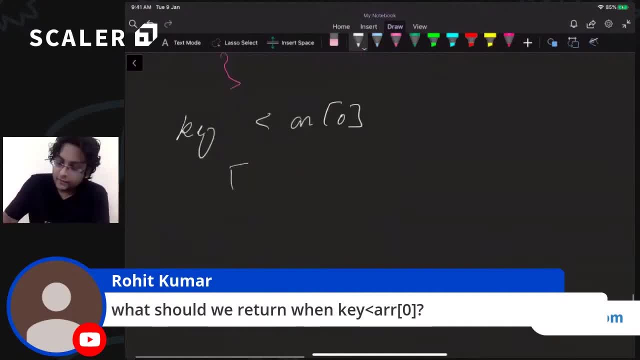 Right, That's a very good question. So suppose that we have this array. Suppose that we have this array: This is the index zero, This is the index one, And so on. Right, Let us say this: This value is 10.. 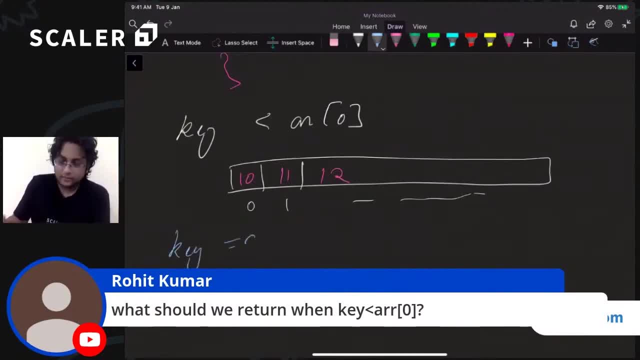 This value is 11.. This value is 12.. And let us say my key was nine, Or let us say my key was five. So, first of all, is my key in the array? Is my key in the array? No, it is not in the array. not present, not present. 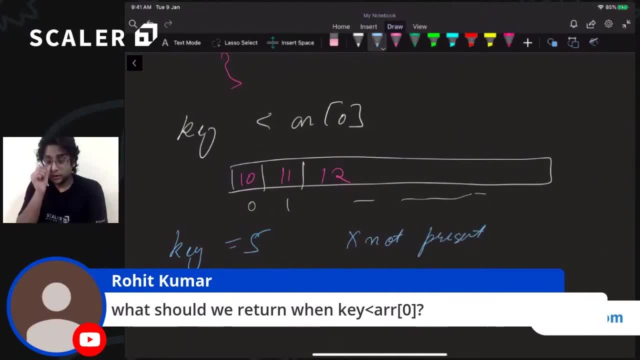 If I were to insert this value, Where should this key go? If I were to insert this value in the array, where should this key go? Can the key go at location minus one? No right, There is no index minus one in the array. 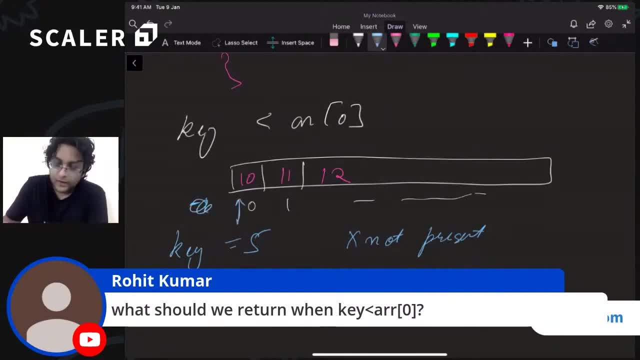 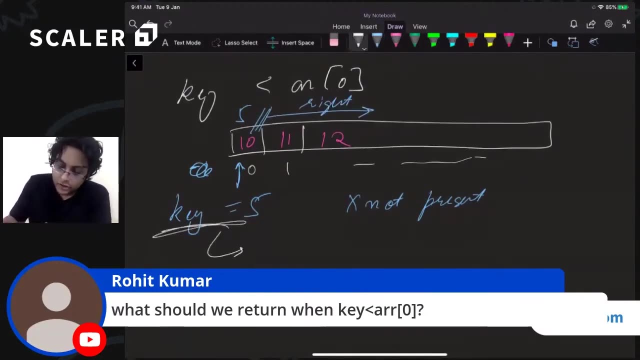 So where should this key go? This key should go at index zero. The five should be inserted over here And everything, that is, everything in the array, should be shifted to the right. shifted one to the right. Does that make sense? So, over here, a binary search. when I search for key equals to five, my binary search should: 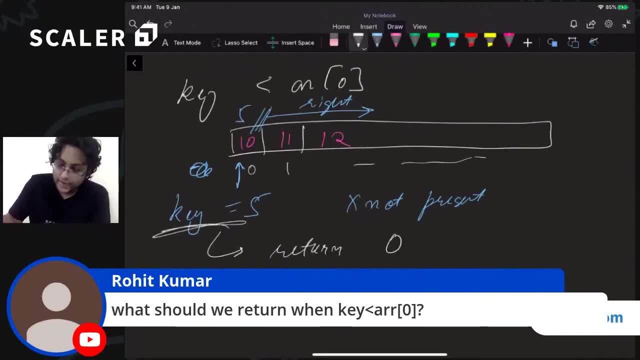 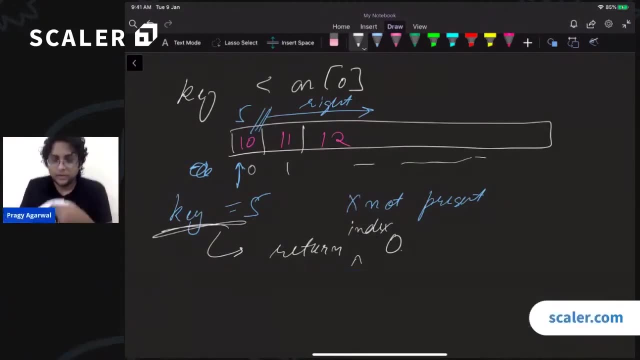 return value zero. it should return the index zero, And that is exactly what our code will do. That is exactly what our code will do. Is that clear? Okay, so let us move on. So I hope that the code and the implementation of binary search is clear to everyone Now. 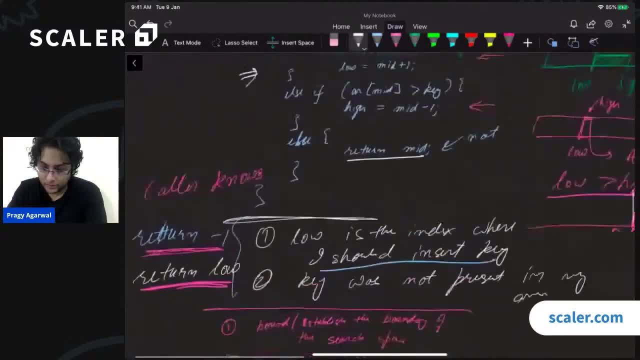 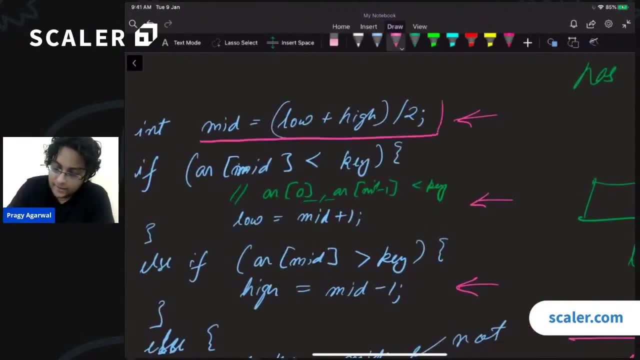 let us look at some improvements that we can make on our code. So one of the most important improvements is that we never try to calculate. we never try to calculate the mid like this. Right, And you might have seen this a lot of times. you might have seen this a lot of. 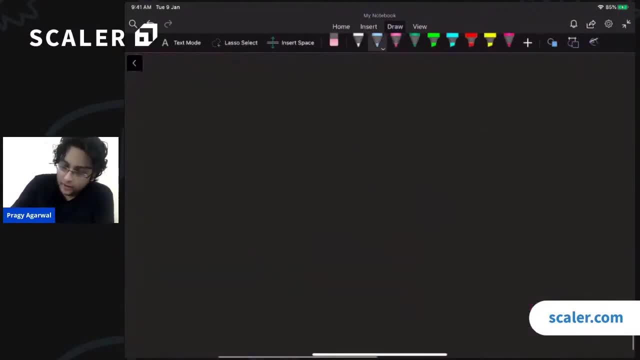 things, People do the following people: instead of saying, instead of saying int mid equals to low plus high by two, high by two, they do something else. They say: int mid equals to low plus high minus low. Let us hi minus low by two, Right? So can someone tell me the difference between these? 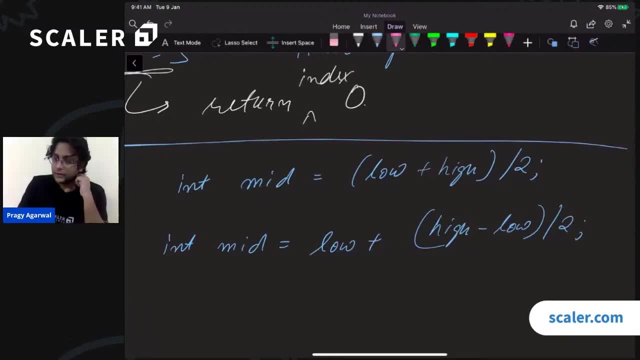 two. Can someone tell me the difference between these two? Why do? why do some people do it this way? Why do some people do with this? But let us try to look at the mathematics. Let us try to look at it mathematically. So if I have low plus high by two, This is this. 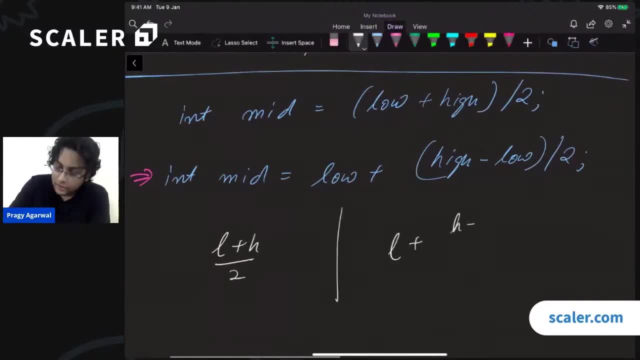 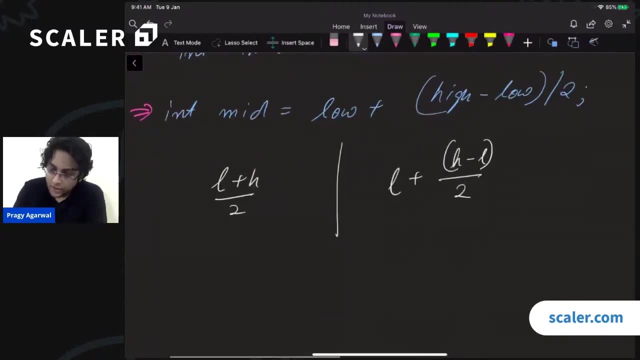 is one thing Or the other, then I can have low, high, minus, low by 2.. Let us see that if there is a difference between these two, Let us see if there is a difference between these two. So what I can do is I can take the denominator 2 common over here. 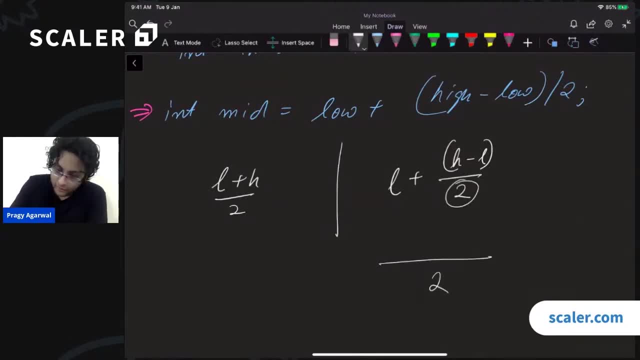 I can take the denominator 2 common over here. So what will happen? This will become 2L plus H minus L. This will become 2L plus H minus L. What is that? That is simply so. 1L will cancel out. 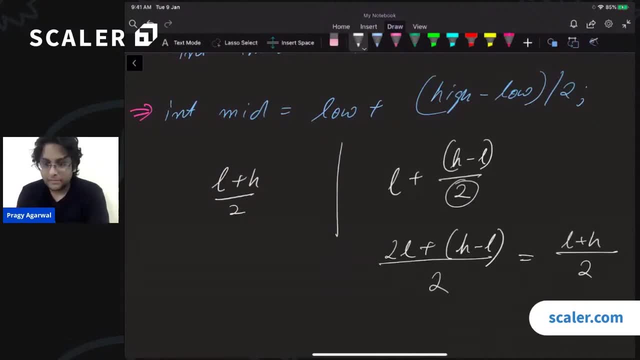 This will simply be low plus H. This will simply be low plus H. So we see that the left-hand side and the right-hand side are equivalent. From a mathematical point of view they are equivalent. So what really gives? Why do people do this? 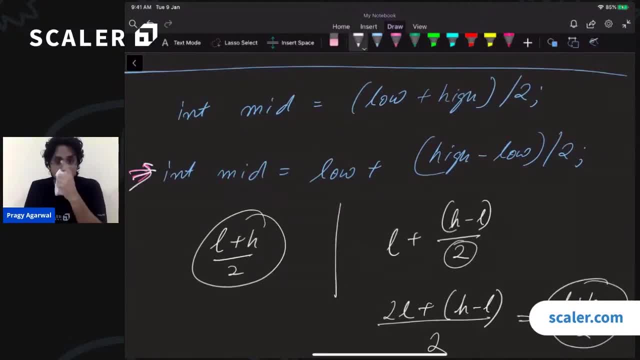 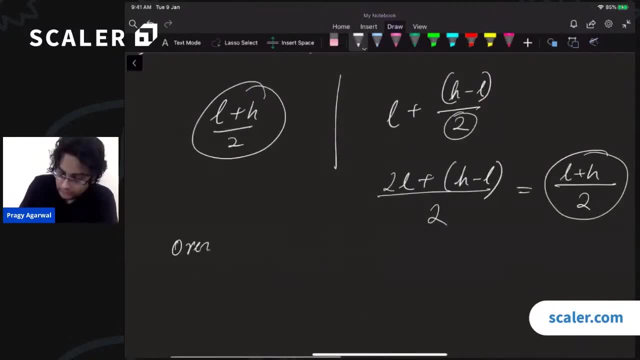 This is more complicated, right? The reason why people do this is even though they are mathematically equivalent. when we are dealing with computers, we can run into an overflow. When we are doing addition, we can run into an overflow. For example, let us suppose that our integer 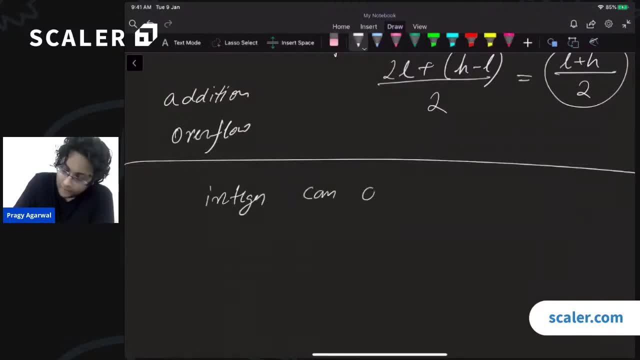 that our integer can only store. so let us suppose that the largest value our integer can store is, let us say 10 to the power 9.. Let us say 1 billion. Let us say that our low is 5 into 10 to the power 8.. 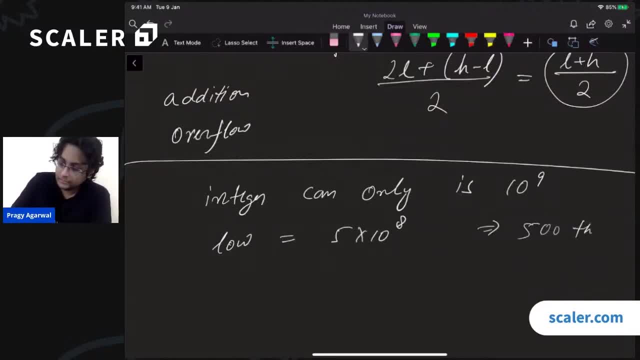 So our low is 500,000.. Let us say that our high is 8 into 10 to the power 8,, which is 800,000.. If I have something like this, what will happen when I try to calculate the mid? 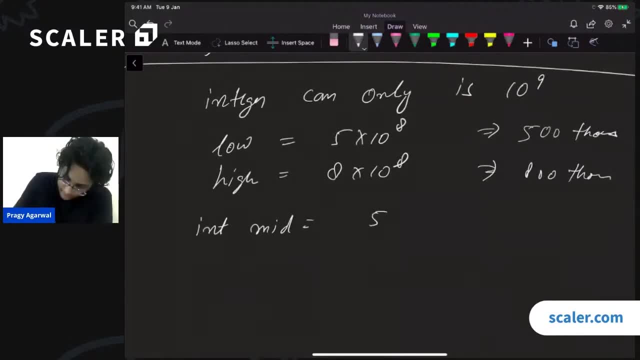 What will happen when I try to calculate the mid. I will be doing 5 into 10 to the power 8, plus 8 into 10 to the power 8, right, This will be low plus high, and then I will divide it by 2.. 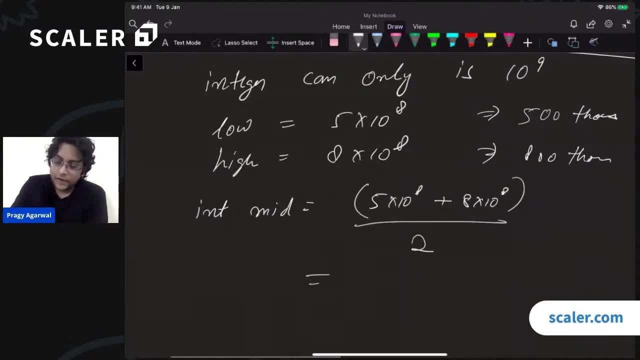 Yes, then I will divide it by 2.. But what will happen over here When I try to add these values? when I try to add these values, this will be 13 times 10 to the power 8, right, And we just saw that. 13 into 10 to the power 8, this cannot fit in my integer. 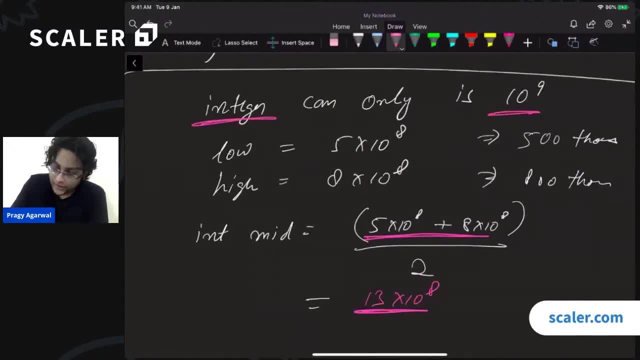 My integer can only be up to 10 to the power 8.. This is greater than 10 to the power 9, right, This is what. This is: 1.3 times 10 to the power 9, right, So this value over here. this will overflow. 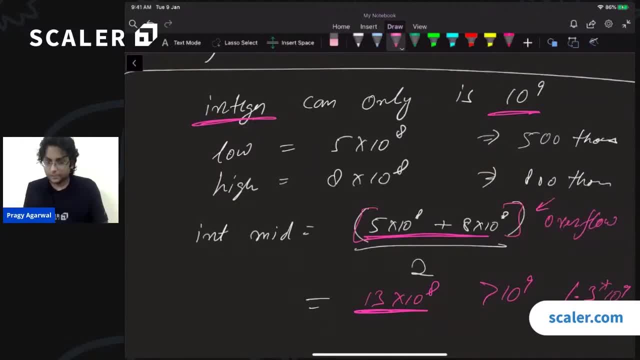 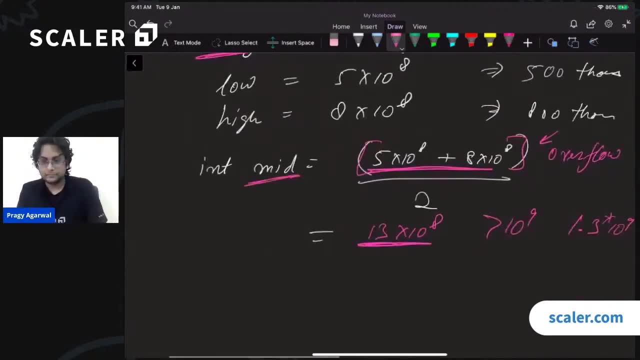 This will overflow And the value that I will get over here will be garbage. right, It will give me a wrong answer And then I divide the wrong answer by 2. I will eventually get a wrong value of mid. Is that clear? 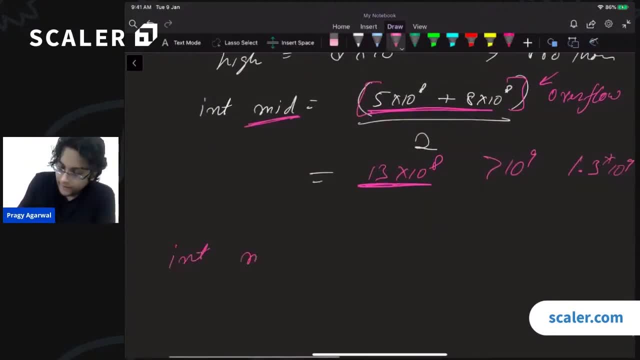 Yes. On the other hand, if I do it the other way, if I do it the other way, if I say low plus high minus low by 2, right, If I do it this way, then what happens? Then this will be 5 into 10 to the power 8. 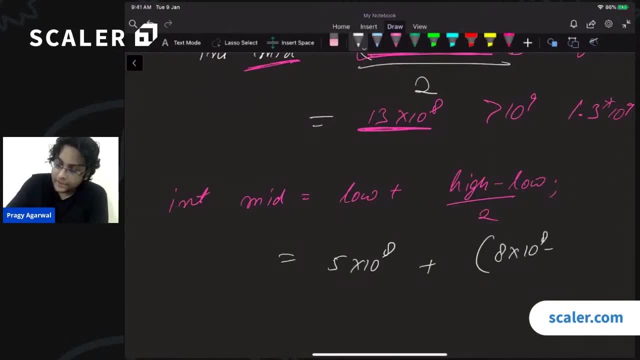 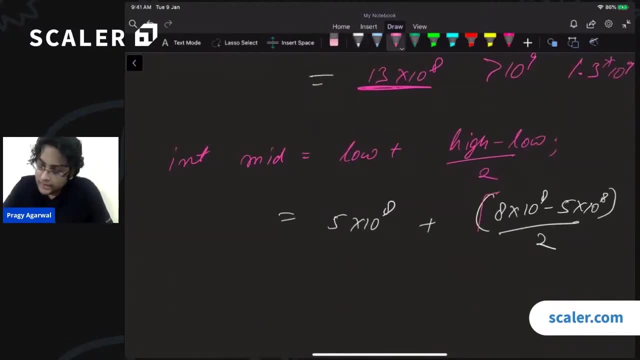 plus 8 into 10 to the power 8, minus 5 into 10 to the power 8 by 2, right, And is this operation going to overflow? Is this operation going to overflow? No, I am subtracting things, right. 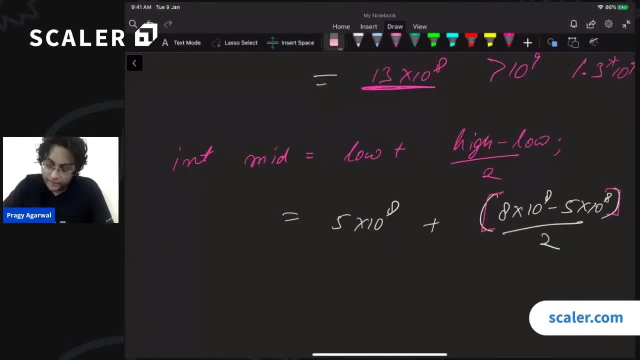 I am subtracting things. The answer over here: It will be less right. The answer over here will be less than this value: Yes. So what do I get over here? I get 5 into 10 to the power 8, plus 3 into 10 to the power 8 by 2, right. 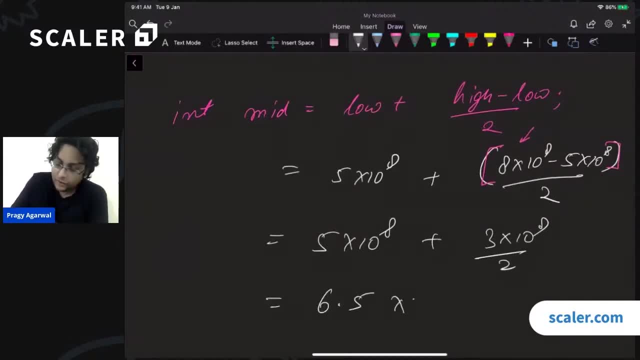 And then I can. then this will give me the correct answer: 6.5 into 10 to the power 8.. Is that clear? This will not overflow. This will not overflow, Whereas this approach will overflow. Is that clear? 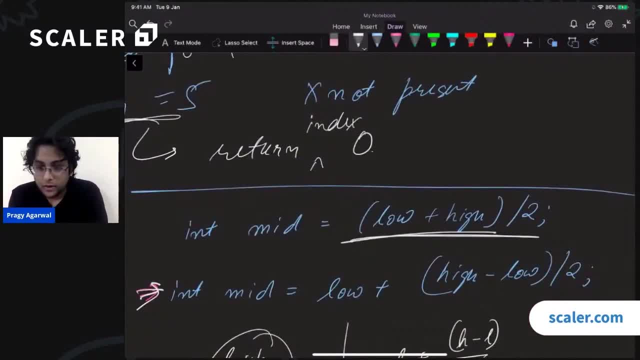 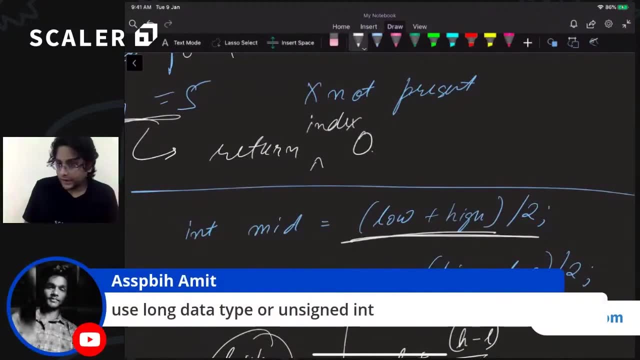 This approach will overflow, All right. So Amit over here says that hey, we can just use a different data type, right? If you're dealing with an integer, maybe we can switch to a long data type, right. But I mean, what if you were using a long right? 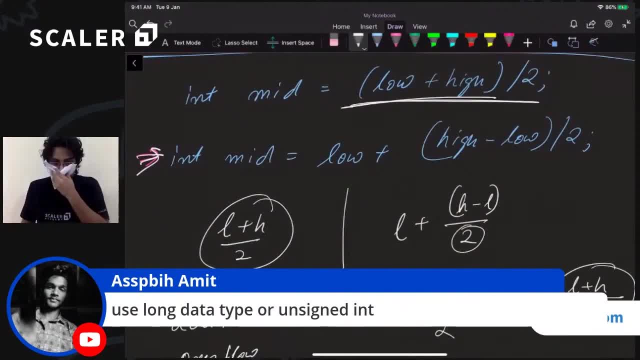 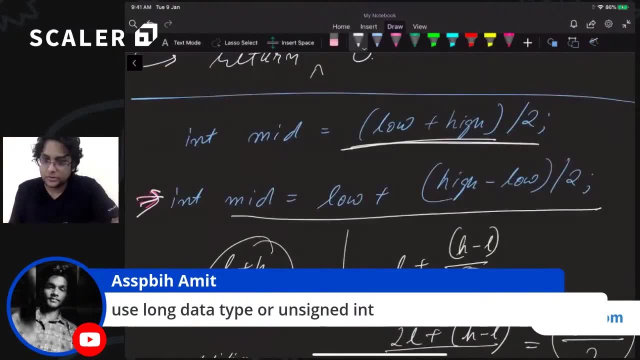 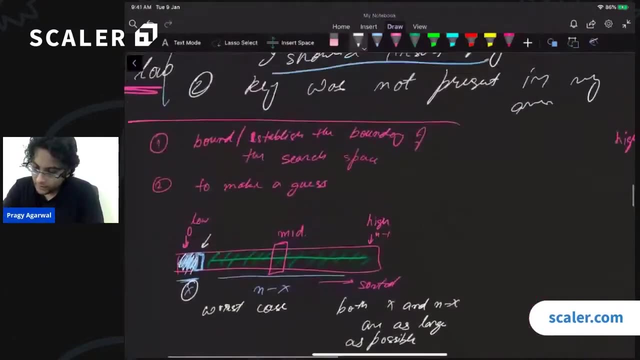 I mean, the problem is, what if you were using a long? what would you do then? So, in general, it is a good idea to implement implement a mid calculation via this particular approach. Okay, All right, So that is the improvement we are going to make over here very quickly. 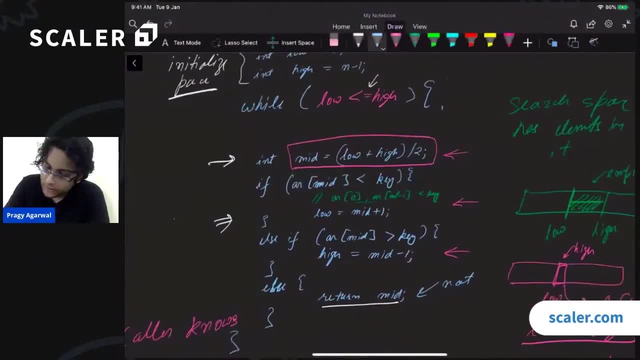 We are going to code 1, a code of binary source. We are going to remove this and we are going to improve it. We are going to say: int mid equals to low plus high minus low by 2.. All right, Perfect. 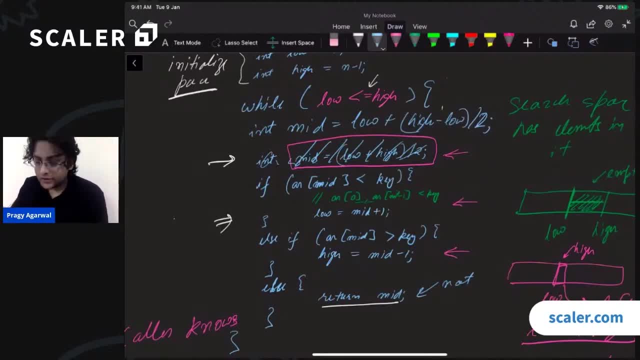 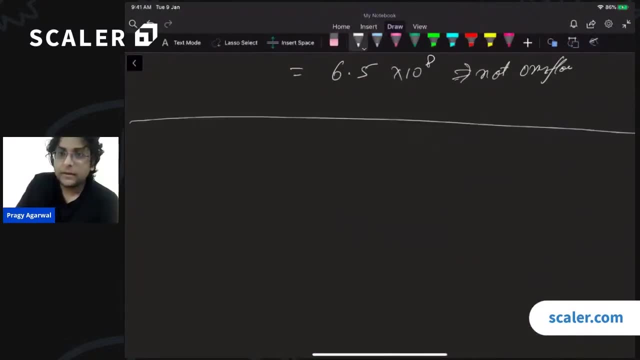 Okay, I hope that everything is clear till now. Now let us try to. now. let us try to analyze the time complexity of binary search. All right, Let us try to analyze the time complexity of binary search. time complexity- All right. 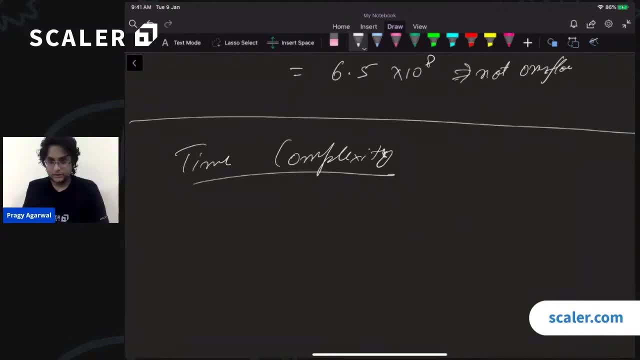 So how do we talk about the time complexity of binary search? So what is really happening is, initially I have the search space of size n, right. Initially I have the search space of size n and I guess the midpoint, I guess the midpoint. 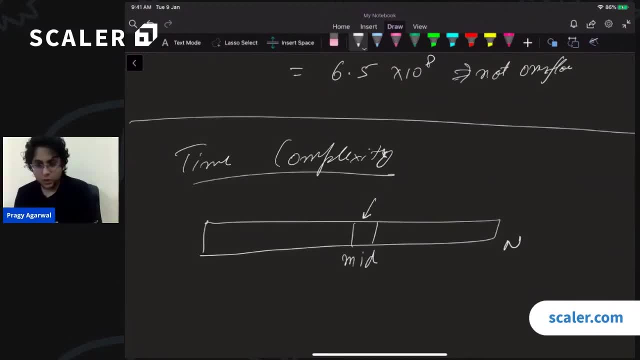 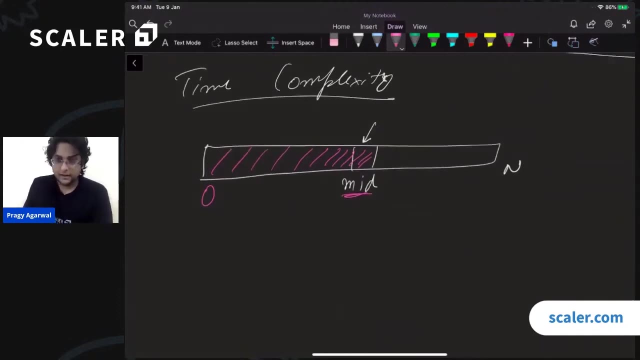 as my guess. If my guess is too low, if my guess is too low, then I am able to remove these elements. Right, I am able to remove these elements. How many elements was I able to remove? So, if this is 0,, this is mid and this is n, then after one guess, if my guess was too, 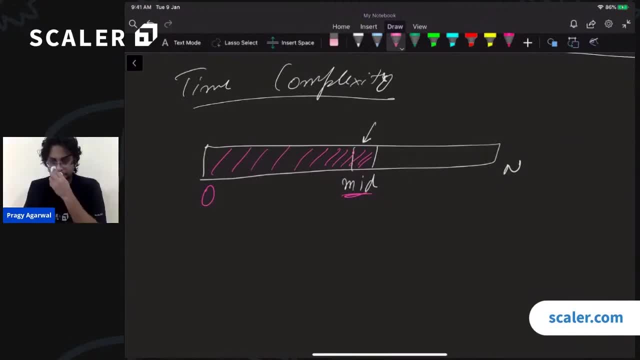 low, then how many elements was I able to remove? I was able to remove n plus 1 by 2 elements, Right, Yes, Yes or no. On the other hand, if my guess was too small, then I would be able to remove all these different. 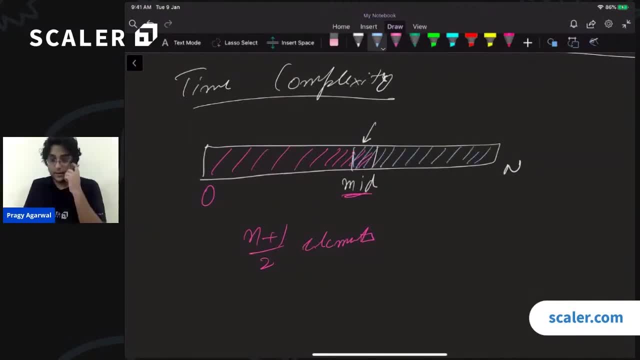 elements. Right, Everything from mid all the way till n, n minus 1.. Right, Even then, I was able to remove n plus 1 by 2 elements. Right, I was able to remove n plus 1 by 2 elements. 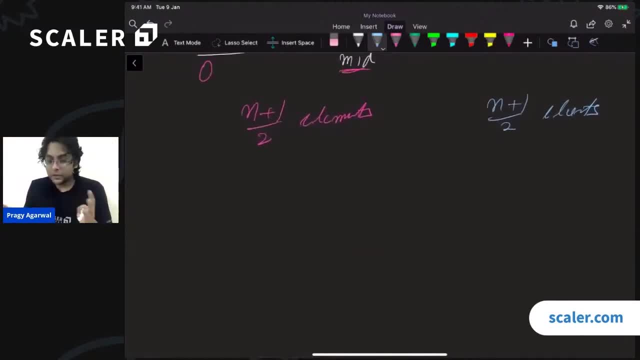 So what really happens is, every time I make a guess, I am reducing the search space by half. Right, I am halving, Halving the search space by half. So I am reducing the search space, space, with every guess, Every guess. 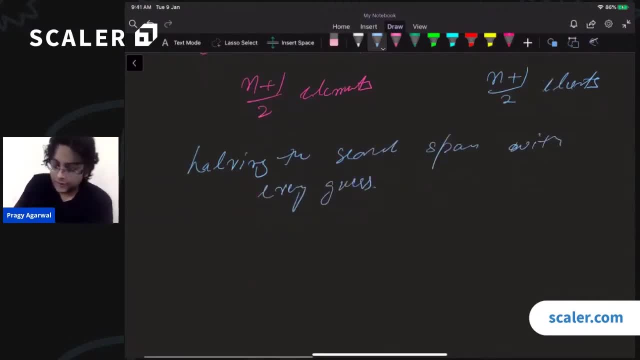 Right. So suppose we started with this guess n. we started the search space of n. After one guess, I will have a search space of n by 2.. After one more guess, I will have a search space of n by 4.. 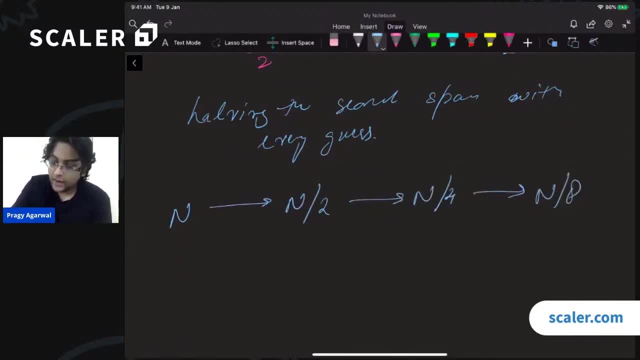 One more guess. I will have a search space of n by 8.. Right, And when will I end? So, finally, the search space will reduce down. the search space will reduce down to just one element. Right, This search space will reduce down to just one element. 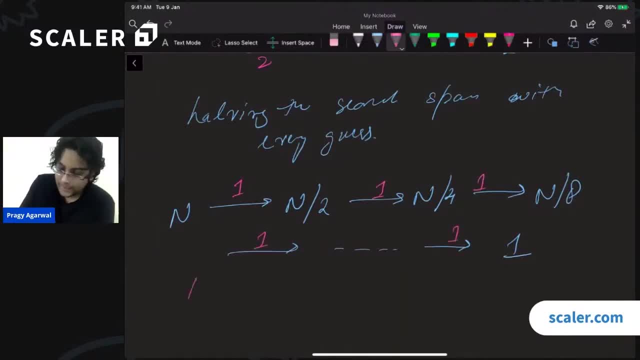 So the question is: how many guesses did it take? So it took me one guess over here, one guess over here, and so on and so forth. So how many guesses did it take, Right? How many guesses did it take? So, no, guys, it did not take me n plus n by 2, plus n by 4.. 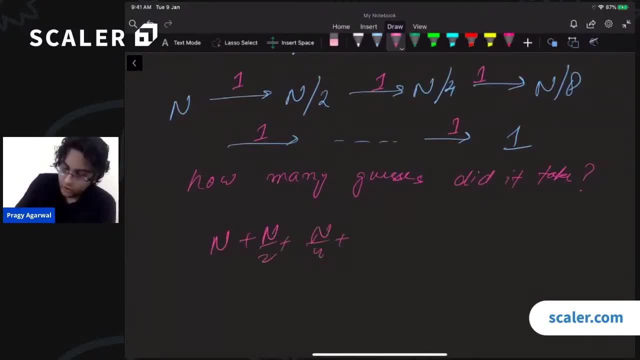 It did not place the filter. bastard by two plus n by four, all the way till one. no, this is not how many guesses i got right. this isn't correct. so remember that when we are moving from this search space to this search space, i am making 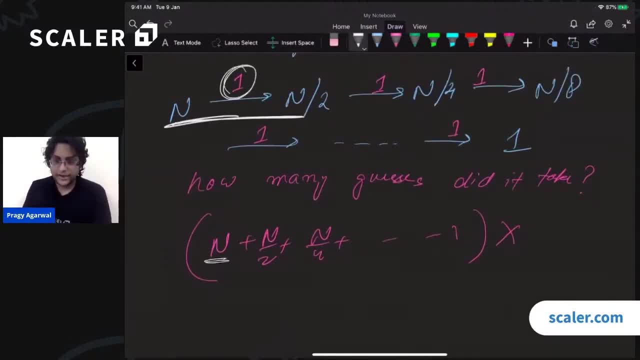 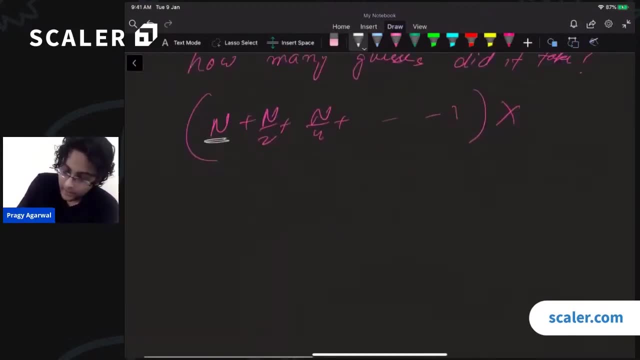 one guess. i am not making n guesses over here. right, i made just one guess and i was able to reduce my search space from n to n by two. right, so basically at the zeroth guess, when i have not made any guess, my search space is of size n. after first guess: right after first guess, my search 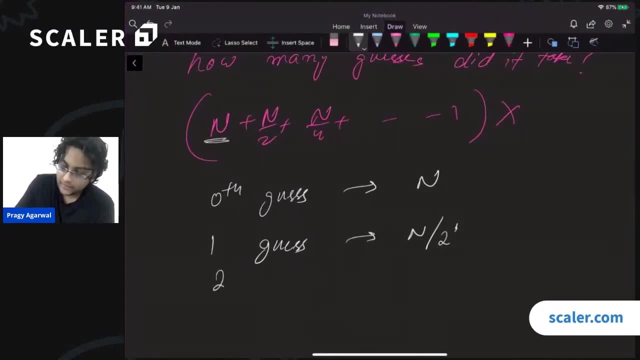 space is of size n by two to the power one. after second guess, my search space is of size n by two to the power two. after the ith guess, my search space will be of the size n by two to the power i. right now. the question is at what value of k? at what value of k will this thing become equal to? 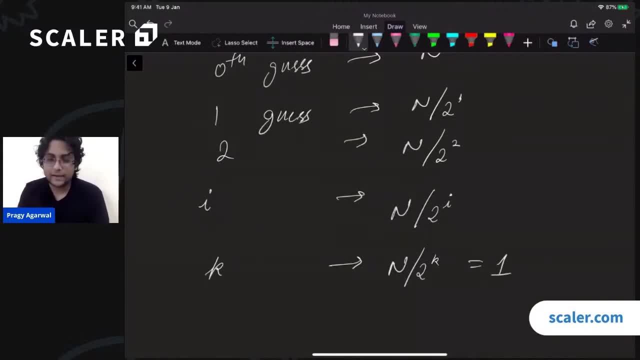 one, at what value of k, with my search space reduced to one signal element? that is the question that we are asking ourselves. so this is the equation that we get right. so at the kth, at the kth case, our search space will be this, and we want the search space to have just one element. 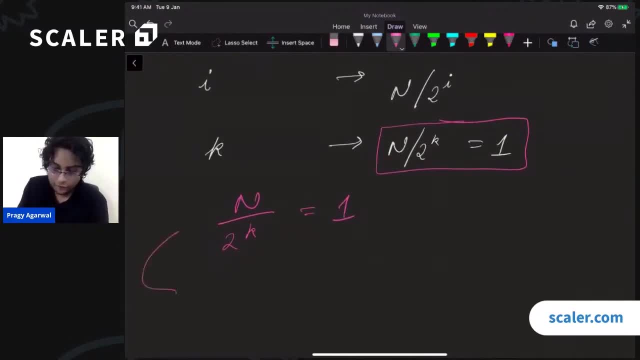 so can we find the value of k from here? can we find the value of k from here. so what can we say? this implies that n equals to 2 to the power k, which implies that i can take log on both side. right, i can take log base 2 on both sides. log base 2 of 2 to the power k. 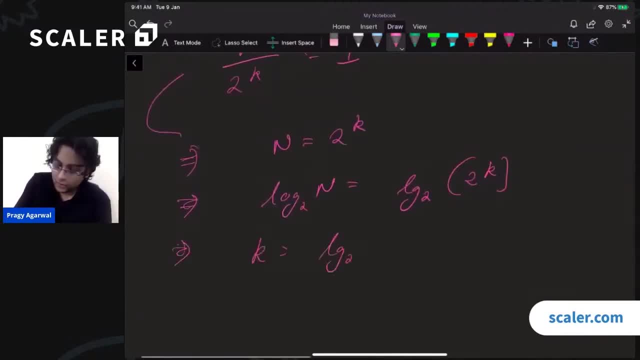 right, which implies that k equals to log base 2 of n. is that clear? yes, so i am. i am taking order of log n guesses, i am making order of login cases, right, and that is the complexity, that is the time complexity, complexity of binary zone. so that is typically one, one of the biggest questions that we get and that is consider. 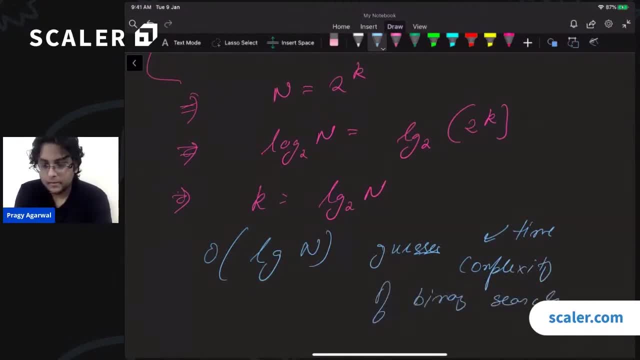 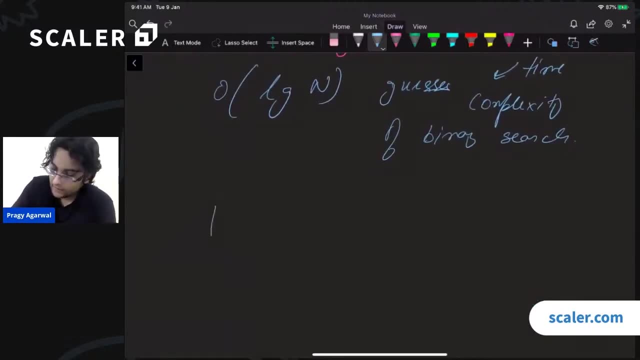 that this refers to our parameter theomial range of the parameter assez, is that clear? yes, is that here, guys? so basically, we started with an array of size n. then, after first guess, we were able to reduce it to half the size, to reduce it to size one. well, it will take us log base two of n guesses. 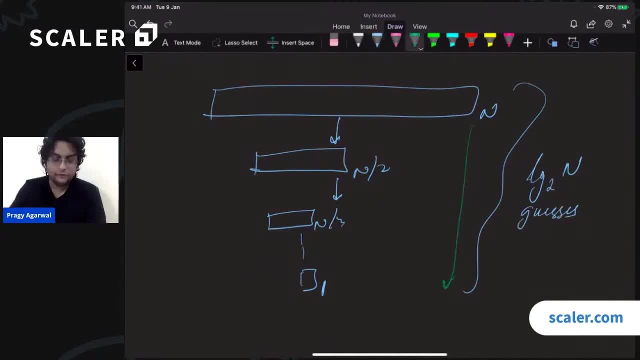 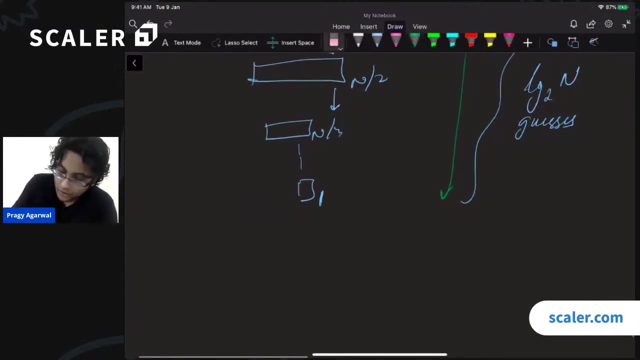 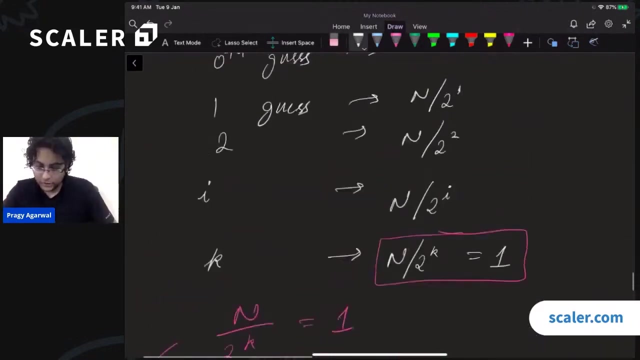 right, the depth of this tree, the depth of this is log base two of n. is that here, right? okay, what about the space complexity? what about the space complexity? right? so let us go to the code to analyze the space complexity. let us go back to our code. 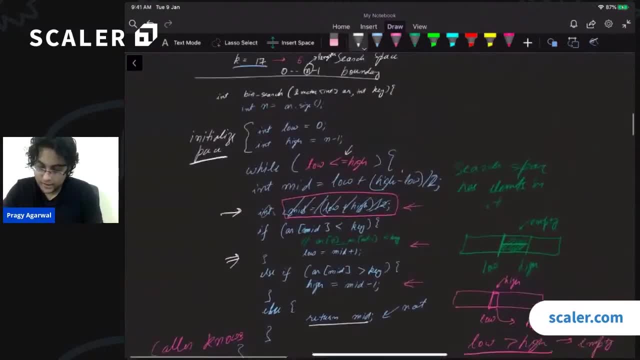 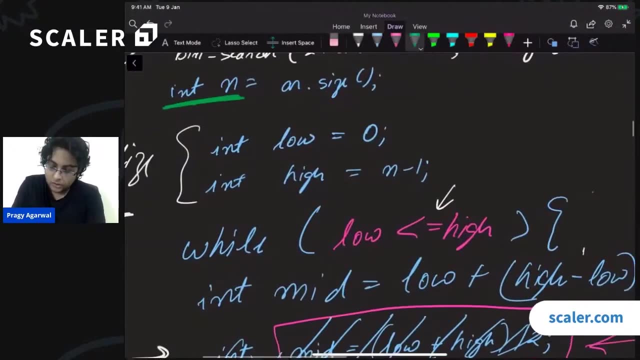 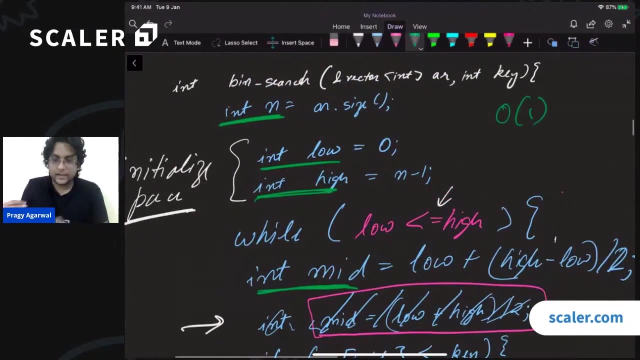 and let us see what variables we are using. so this is, this is our code. let us see what variables we are using. so we are declaring a variable over here, n, we are declaring a low, we are declaring a high and we are declaring a mid right. all of these, all of these take constant space. they are just. 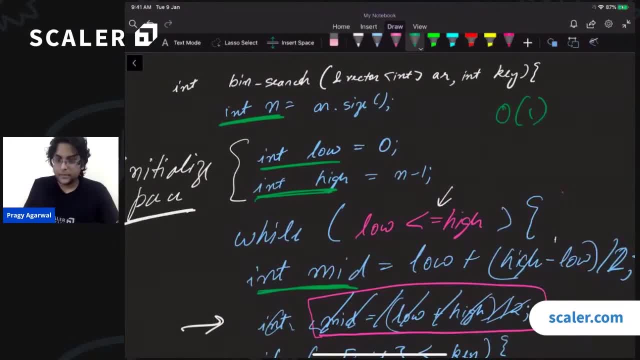 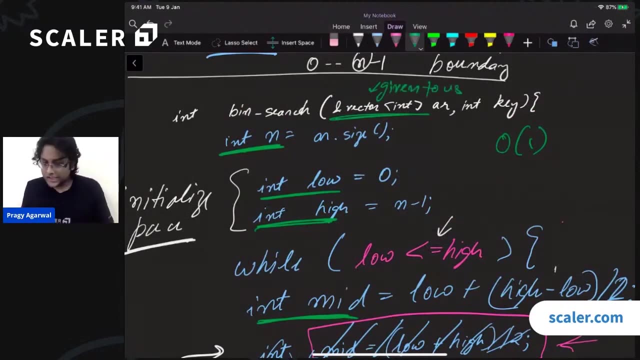 integers. so, overall, our space is just constant, right, we are not allocating space that is dependent on the input. we are just allocating a constant space, right? notice that this is this vector. we are not allocating this. this is given to us, already given to us. since we are not, 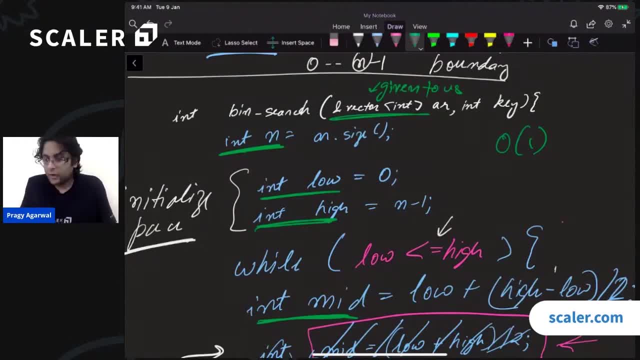 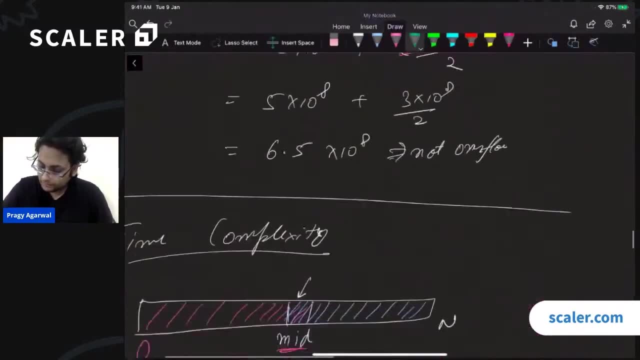 changing this array at all. we are not changing this array at all, so we don't have to allocate the space for the array. all right, the array is given to us. so the space complexity of binary search is going to be the space complexity of binary search is going to be simply order of one. 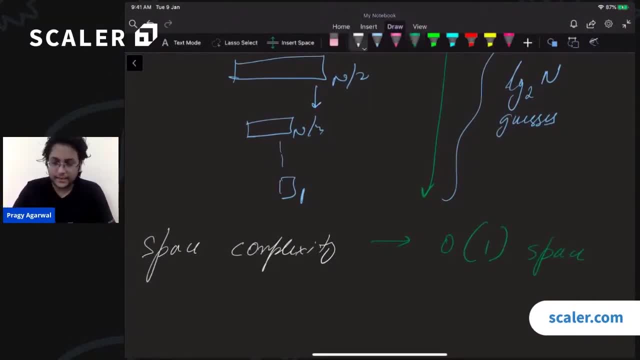 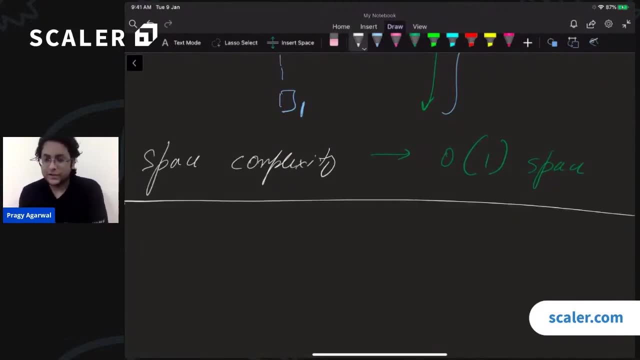 right, constant space. is that here, guys? perfect, perfect, perfect. now let me ask you a question. let me ask you a fun question over here. so this is called binary search, right, this is called binary search, binary search. why is it called binary search? because we are splitting into two parts. 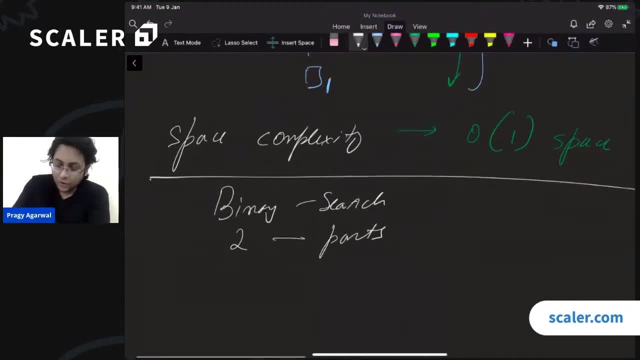 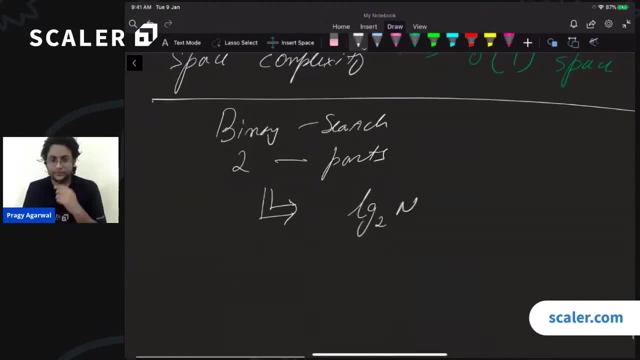 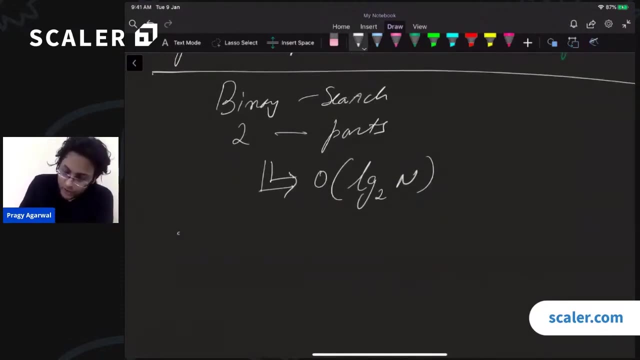 two parts with every guess right. and we saw that when we do binary search. when we do binary search, our complexity turns out to be log base 2 of m. right, our complexity turns out to be log base 2 of m. what if, instead of binary source, what if i try to come up with something like toner research? 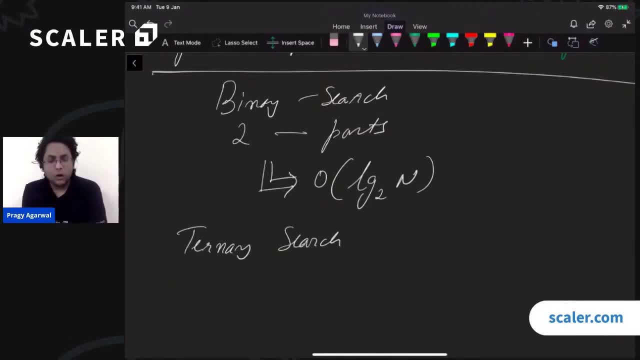 what if i try to come up with something like turner resource? so, first of all, how would the research even work? right, how would the research even work if i have this particular array? then now i have to guess two values. i have to get mid one and i have to get mid two. right, this is my 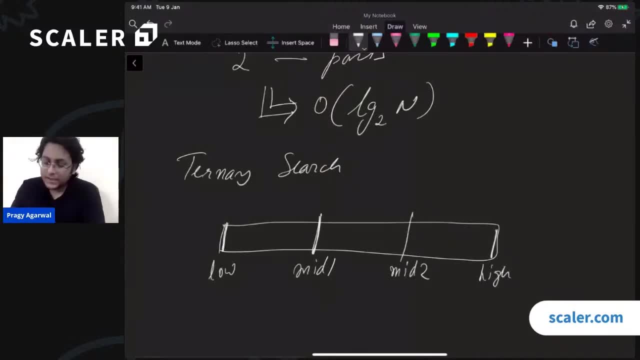 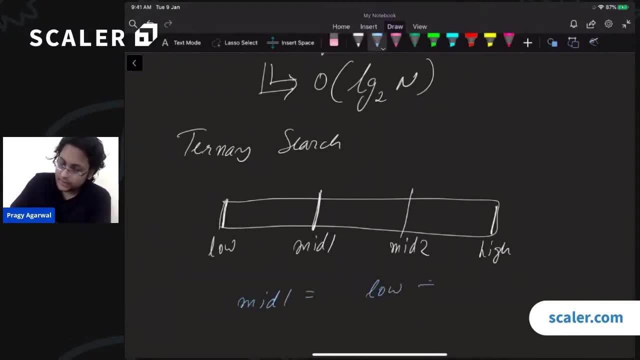 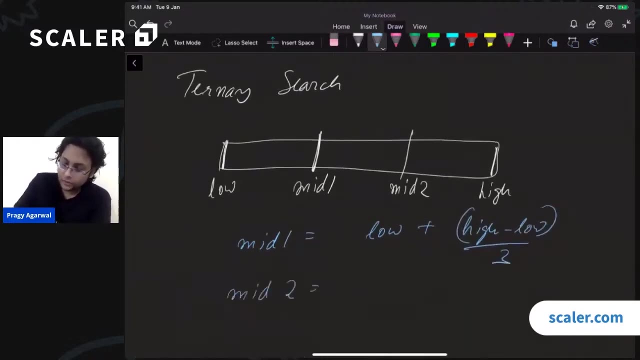 this is my height in the research. what i can do is i can make two guesses right. i can make two cases. i can say mid one equals to low plus high minus low by three, right. and i can say mid two equals to low plus two times high minus low. 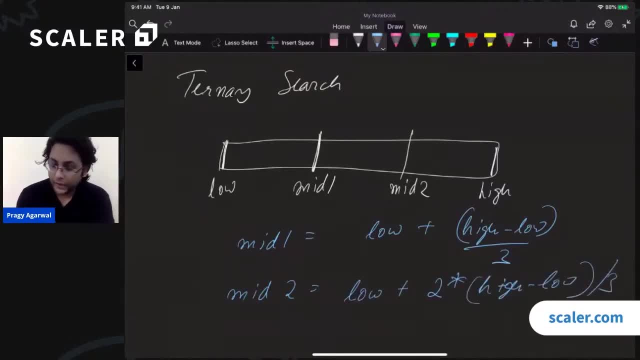 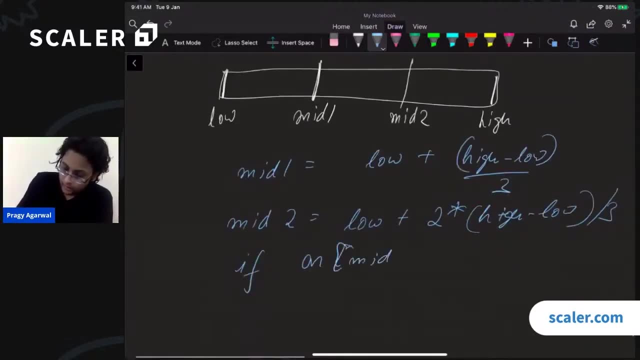 by three, yes or no? can i do that? and then i can compare right, then i can compare. so i can compare ar of mid one with my key, i can compare ar of mid two with my key right, and what will i get? what will i get either. 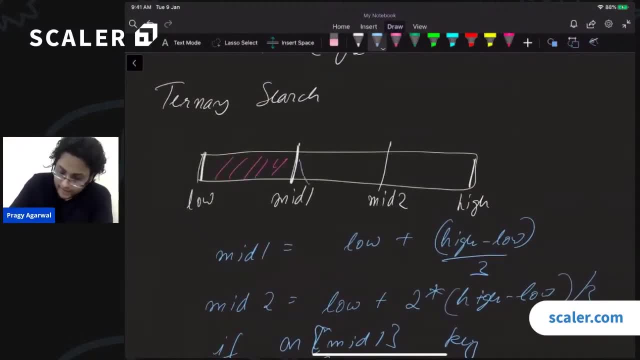 either my key will lie in this area or my key will lie in this area, or my key will lie in this area. yes, that is. that is. that is all the possibilities, right? my key cannot lie in both these areas at the same time. right, my key cannot lie in both these areas at the same time. does that make sense? so 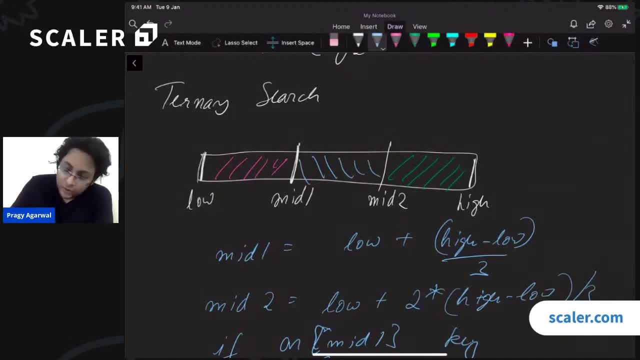 after one guess. after one guess, we were able to reduce our search space by one to one. right from n we could go to n. by three right, we could eliminate a larger chunk of our search space. does that make sense? this is called ternary search, this is called ternary source and in 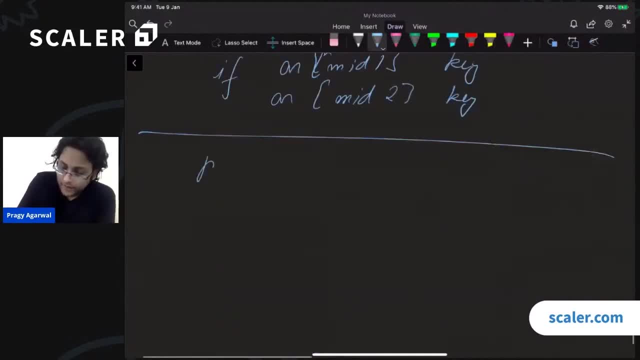 general. you can extend this idea. you can extend this idea. you can define something called a key research, you can define something called a k research. and in k research, what you will do is you will calculate mid one, mid two, all the way till mid k minus one right, and then we'll compare. 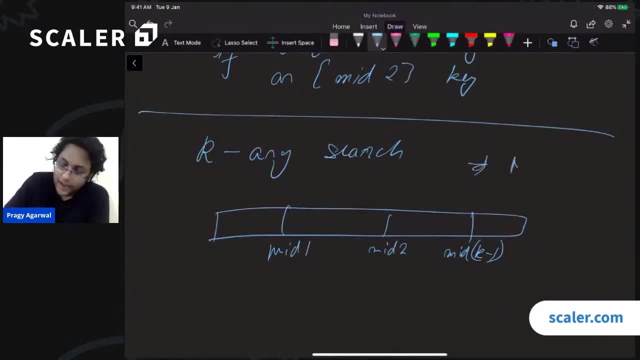 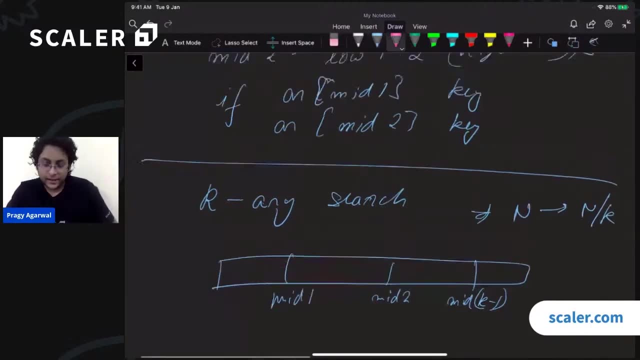 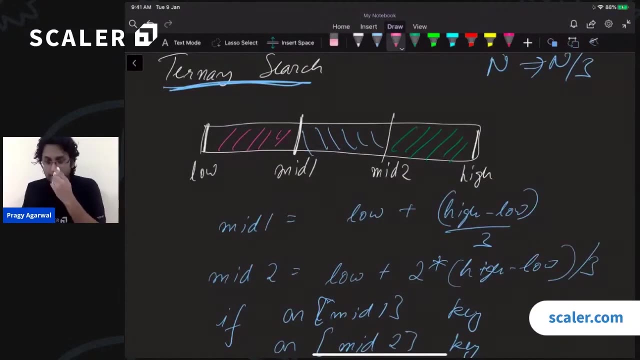 with all that will allow us to. in one case, it will allow us to go from n all the way till n by k, right? does that make sense? yes, ternary means three divisions, binary means two divisions, carry means k divisions. all right, is that clear example of ternary search? well, the example is very simple, right we? 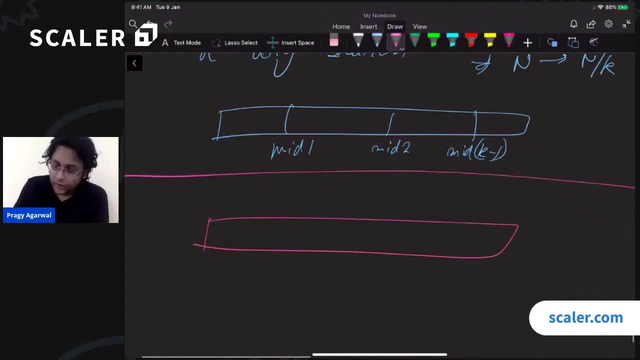 given an array. given an array, what i am going to do is i am going to make two guesses, right, instead of making one guess at any point. i am going to make two guesses and, based on these two cases, i am going to decide whether i should be looking over here. 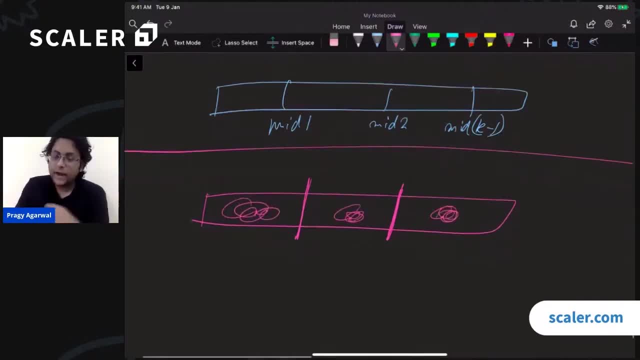 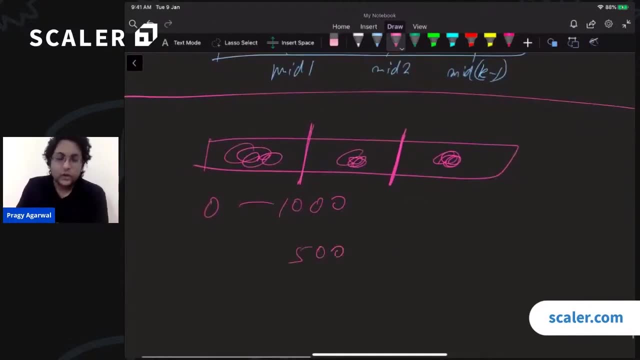 or i should be looking over here, or i should be looking over here, right. going back to our original, then we were supposed to guess between zero and one thousand, right? instead of instead of you giving me a guess like 500, you could have given me two guesses at the same time. you could have given. 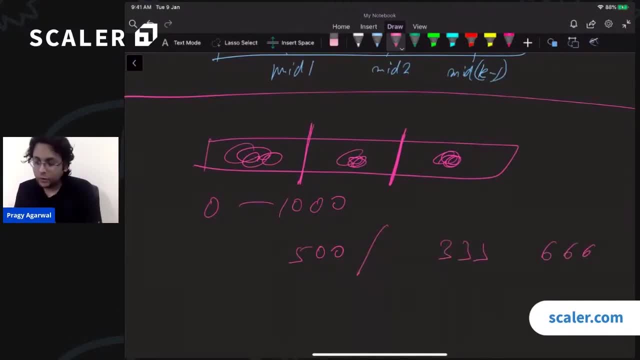 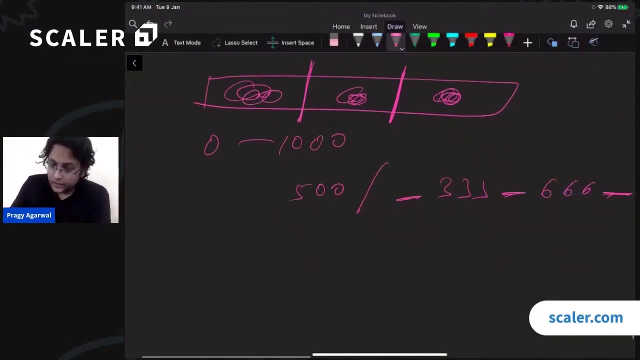 me three, three, three and six, six, six, right. and then i could have told you that, okay, it is less than three, three, or it is between this or it is above this. does that make sense? yes, does that make sense, right? so the time complexity of ternary search. ternary search. 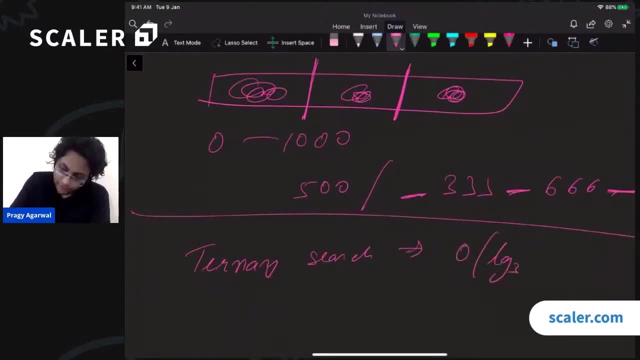 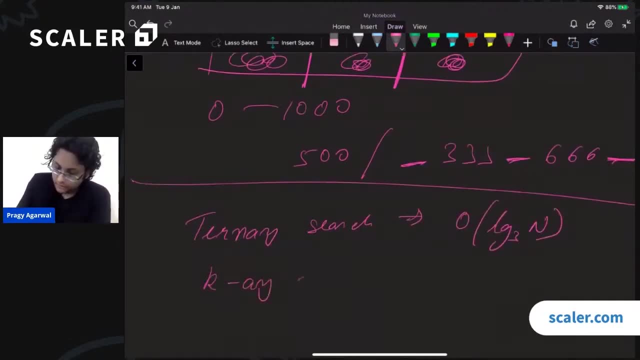 it seems that the time complexity of ternary search will be: order of log base. three of n- right, because we are dividing by three every time. similarly, the time complexity of k research would be: order of log base. k of n. yes, now, which is greater? which do you think is greater? is log base 2 of n more or is log base? 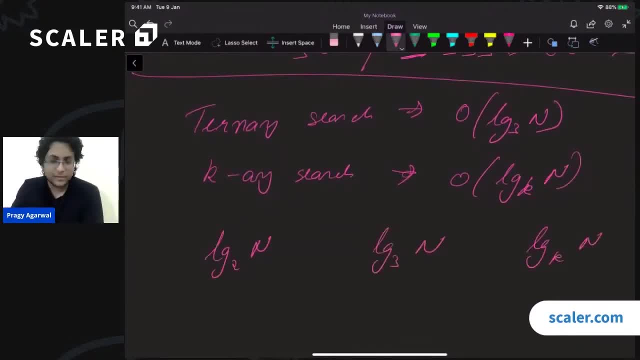 3 of n more, or is log base k of n more right for some large value of k? which value is more? which value is smaller, right? so which value is larger? which value is smaller? well, if we divide by 2, if we divide by 2, then it takes us certain number of steps to reach. 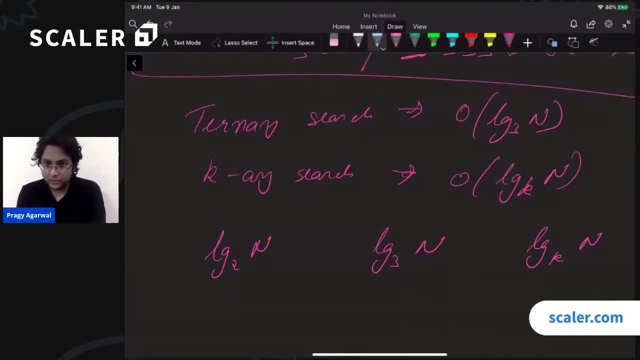 one. if we divide by 3, then it will take us less than steps to reach one right. if we divide by three, then it will take us, let us, lesser steps to reach one. so log base 2 is greater than log base 3, n, which is greater than log basis k, ent. 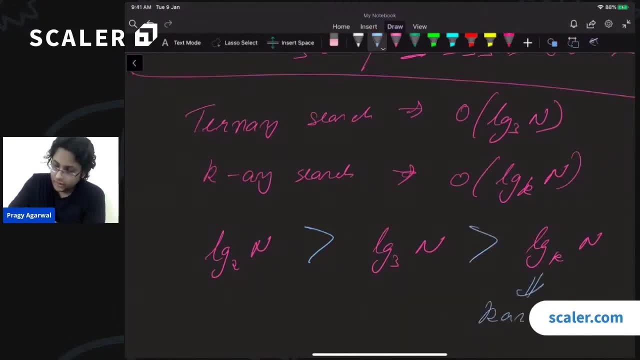 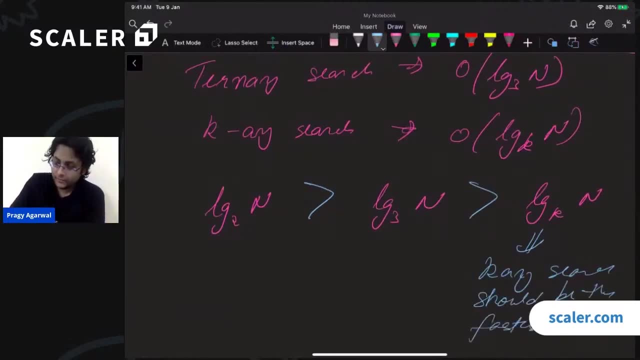 Okay. so this it seems like k research. k research should be the fastest, should be the fastest right. So why do people still use binary source? Why do people still use binary source? Why don't we always have k research? k research seems to be very fast. 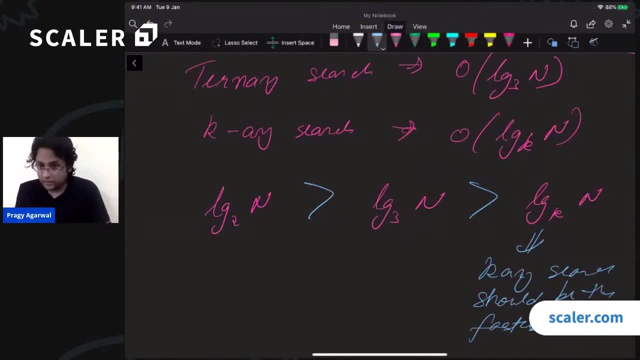 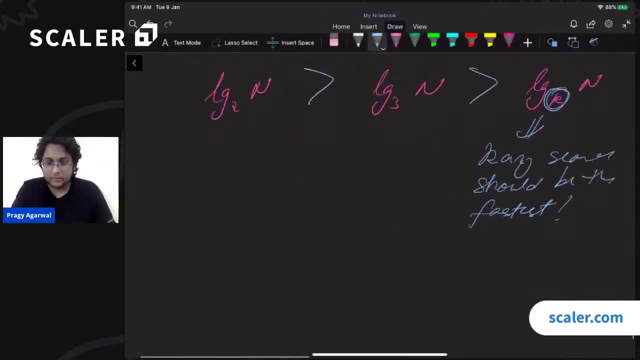 Right, And it seems that I can make it as fast as I want. right, I can just increase the value of k to make it as fast as I want, Yes or no? Yes, Well, let us see what is the fastest value I can have. 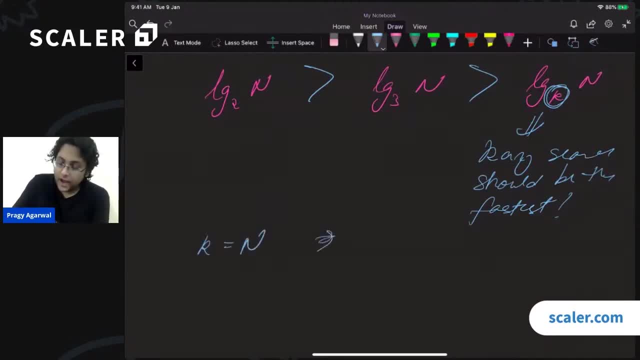 So maybe when k equals to n, when k equals to n, I will get log base n of n, which is simply one, So I will be able to find the answer. find the answer in just one guess. That is amazing, Right. 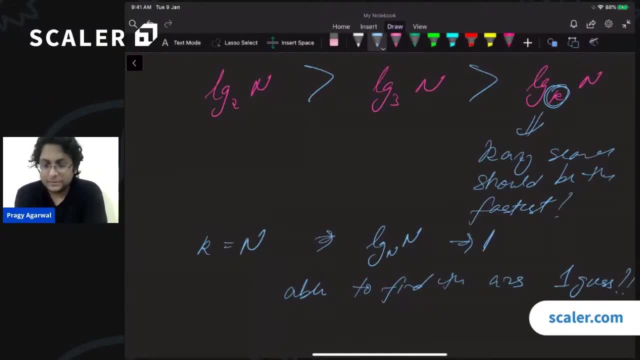 I will be able to find the answer in just one guess. That's very, very weird, right? I was able to find the answer. I was able to search the element in the array in just one guess. if k equals to n, 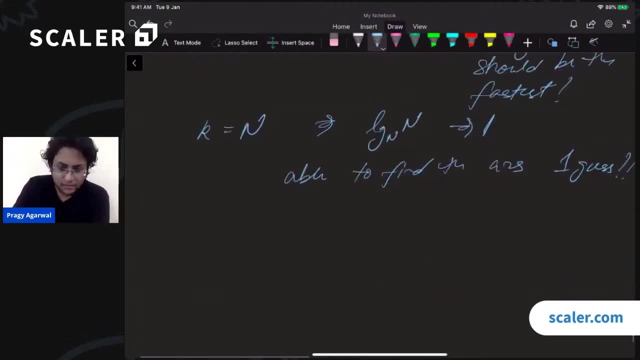 Is that correct? Is that correct? Yes, but there's a catch over here. Right Now. what really happened was we had this array and we made every element. we made every element as a guess. we made every single element as a guess, and then we check if our 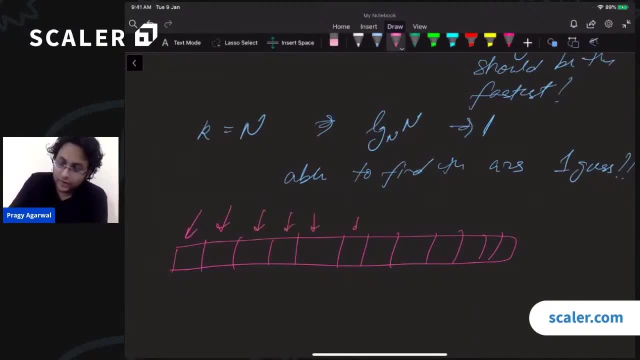 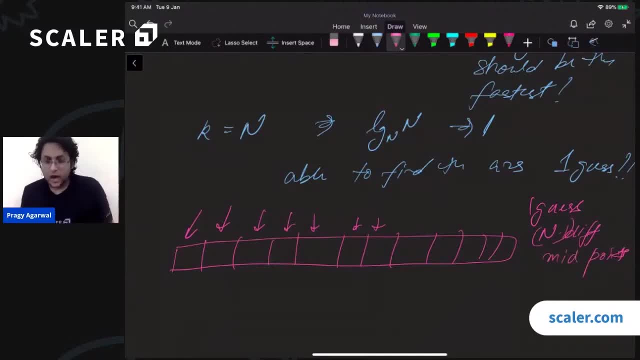 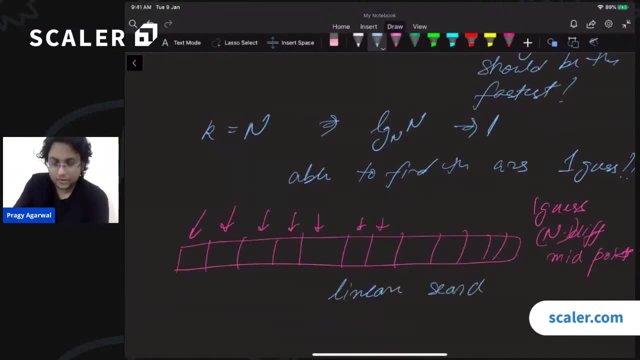 So are we really? are we really doing an efficient search over here? Are we really doing an efficient search over here? No, this has reduced to the linear search Right. This has reduced to linear search. So it turns out that when k equals to n, we were expecting it to take just one guess. 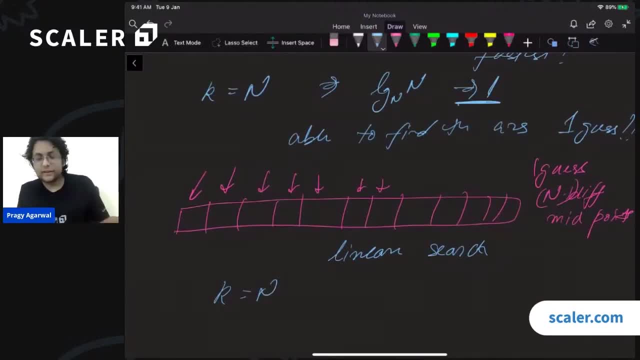 it did take just one guess, But inside that single guess it didn't take just one guess. Inside that single guess we were doing a linear search, Right? So this is the worst thing that we can do. Does that make sense? 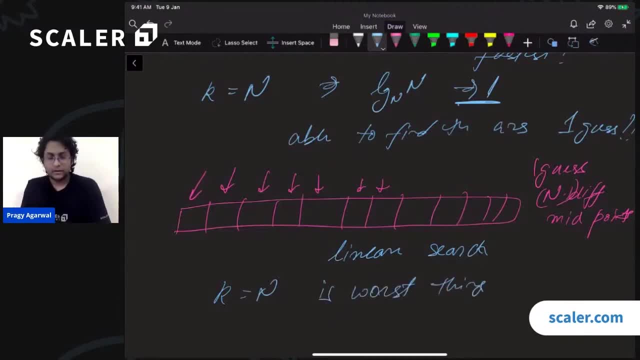 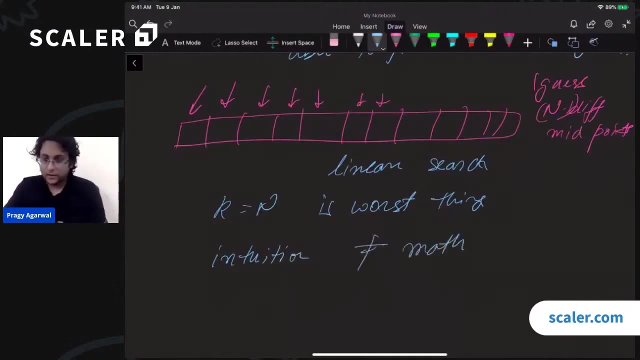 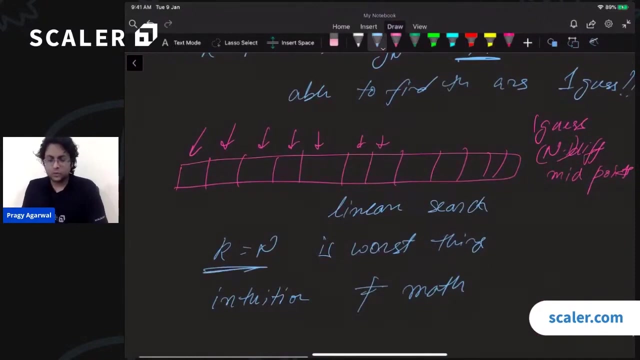 k equals to n is the worst thing that we can do. So what? what really gives? We see that our intuition, intuition does not equal our math over here. Right, Math says, math says that this should be faster, But intuition says that this should be slower. 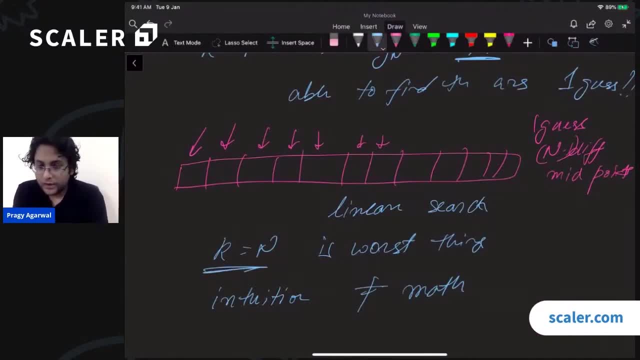 So what? what really gives over here? What really gives over here? Well, there's a catch, There's a catch. right, There's a catch in the fact that this is bigger complexity. There's a hidden constant factor. There's a hidden constant factor. 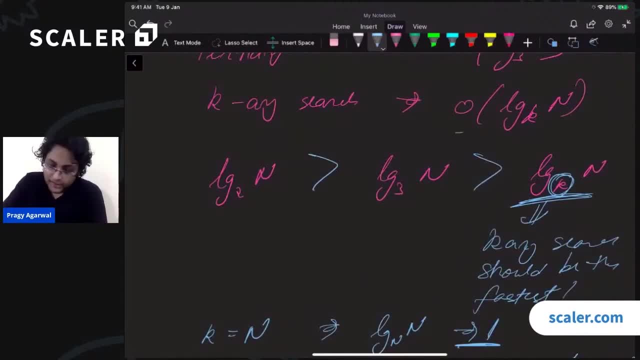 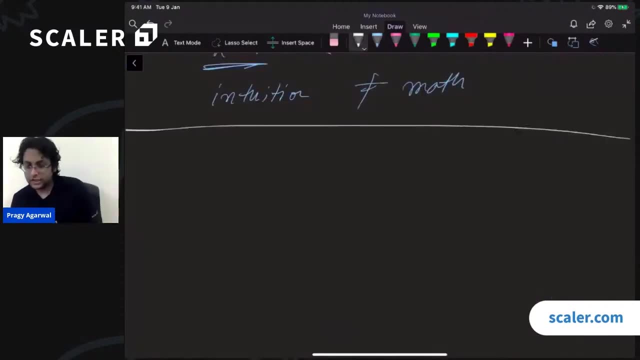 Let us look at the exact complexity of searching. Let us look at the exact complexity of k research. If I'm doing binary search, if I'm doing binary search, then I have one guess, right, I have one midpoint. Yes, Yes. 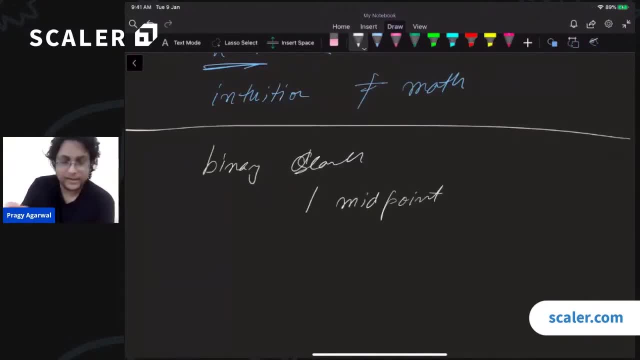 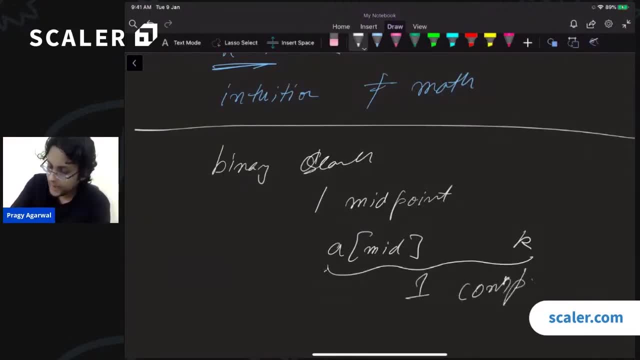 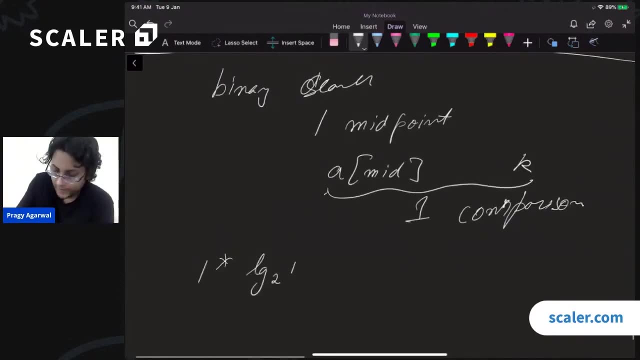 This is one comparison. This is one comparison, Right? So my complexity, my actual compact complexity, is one times log base 2 of n. This is in the case of binary search. On the other hand, when I have ternary search, when I have ternary search, I will guess two. 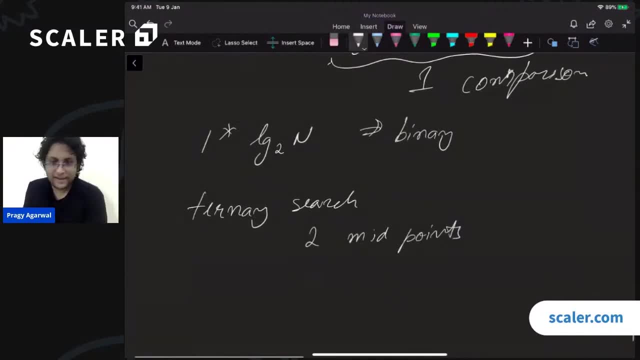 midpoints. Right, I will be guessing two midpoints. And then what comparisons do I have to make? I have to compare A of mid 1 with K. I have to compare A of mid 2 with K, Do you agree? 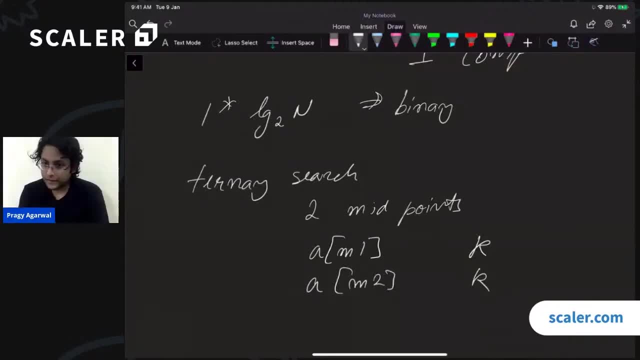 Yes, I have to compare A of mid 1 with K And I have to compare A of mid 2 with K. So how many comparisons is that? This is in fact two comparisons. Right Now, you see the hidden cost. As we increase the value of K, as we increase the value of K, the number of comparisons 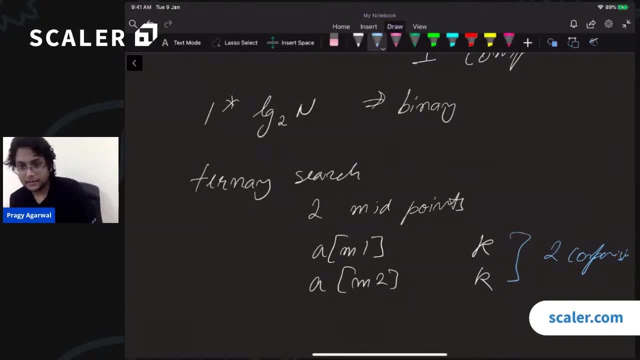 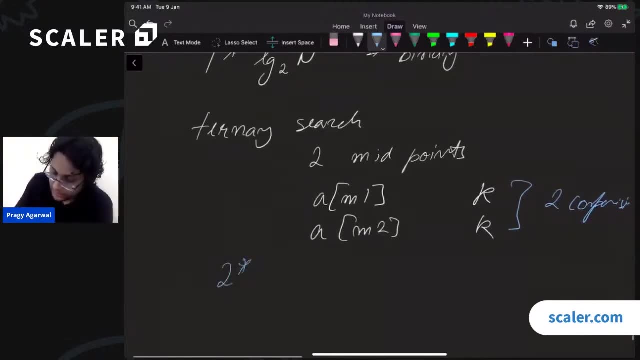 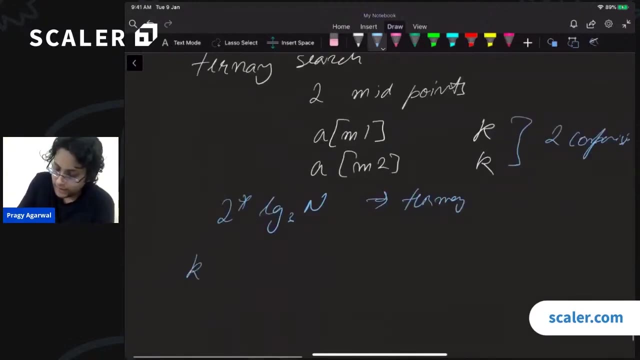 for each guess increase. Does that make sense? Yes, guys. So for ternary search our complexity is 2 times log. base 3 of N. This is for ternary search, Ternary search And in general for K research. 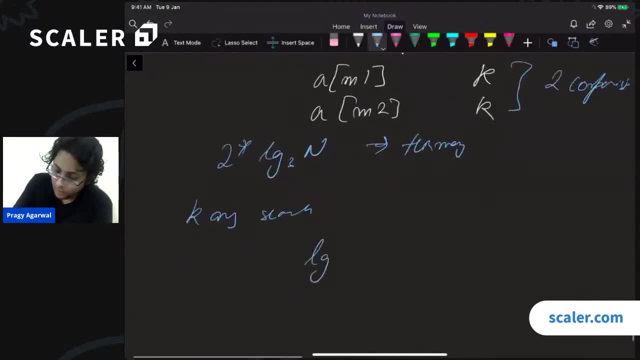 our complexity, will be log base K of N. But for every guess we will have to make K minus 1 comparisons. Right, We will have to make K minus 1 comparisons. Now let us ask this question again: What do you think is larger? What do you think is larger? Is log base 2? 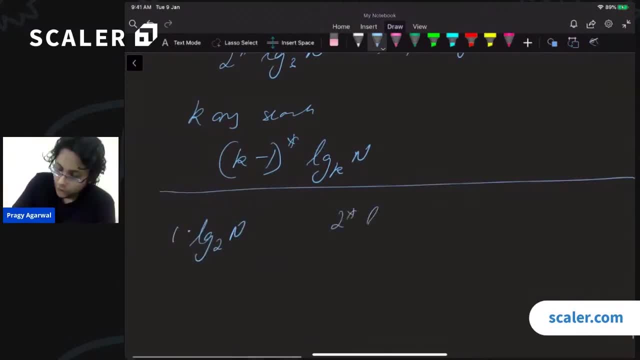 of N times 1 larger Or is 2 times log base 3 of N larger Or is K minus 1 times log base K of N larger? Which one of these is larger? Well, now we know. Now we know that actually this is the reverse, the other way around. 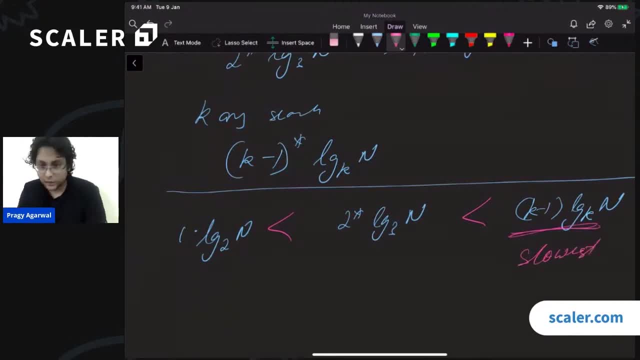 This is the slowest, This is the largest value, So this is the slowest And in fact binary search is the fastest. Is that clear? So we can totally do K research, We can totally do a ternary search, We can totally do a K research, But practically binary search will. 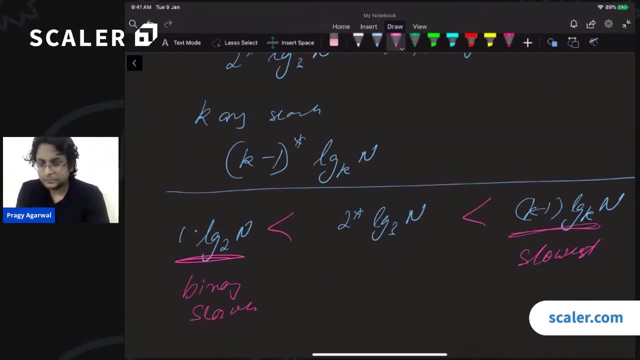 work much, much faster. Is that clear, guys? Yes, Is that clear? Binary search will work much, much faster. Right Cool, Now there is this question. Now you might be thinking that okay, you told us about ternary search, You. 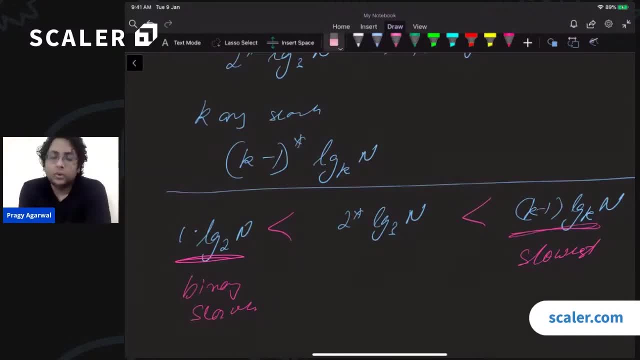 told us about K research And then you said that, okay, those didn't, those don't really matter, Right? Why did you even tell us in the first place? Why did you tell this to us in the first place? The reason is that in certain situations, in certain situations, 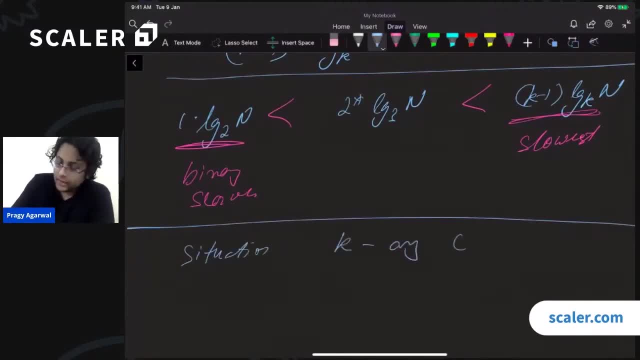 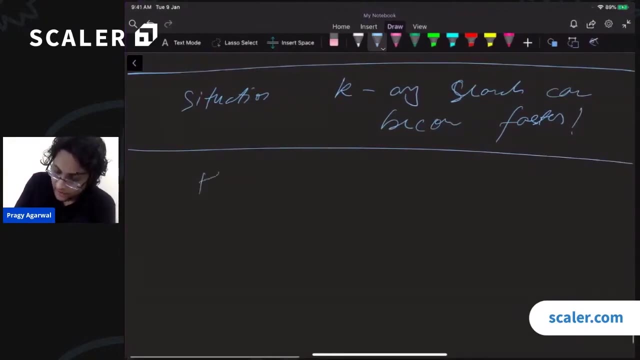 K research. K research can become, can become faster, K research can become faster. Let us look at how. Let us look at how. Suppose suppose that we are dealing with some sort of a disk, right Hard disk. Suppose that we are dealing with some sort of a hard disk. 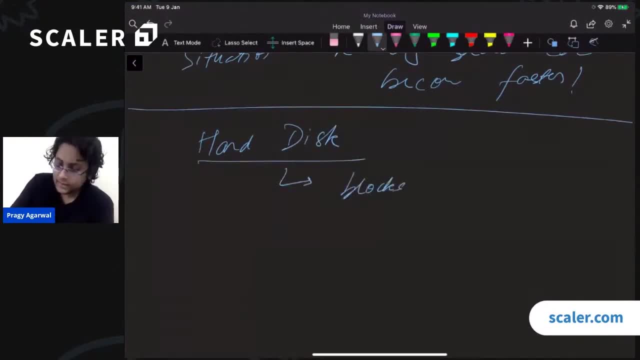 Do you know that hard disk is split into blocks and sectors and tracks? Yes, So basically, we are talking about a spinning hard disk over here. We are not talking about that- the new SSDs over here. We are talking about that spinning hard disk over. 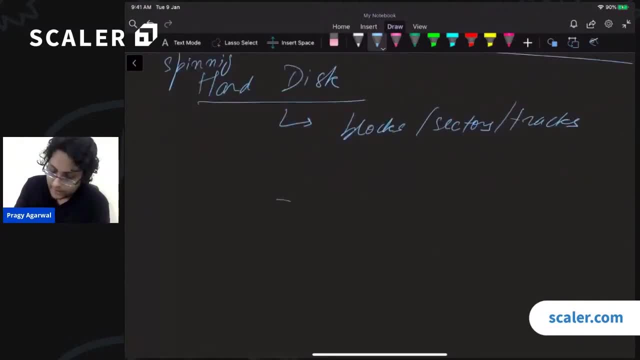 here the magnetic hard disk. So what really happens is in a magnetic hard disk you have several platters, You have several platters And for each platter you have a readhead. You have a readhead That is at a particular platter, That is tracking a particular track. 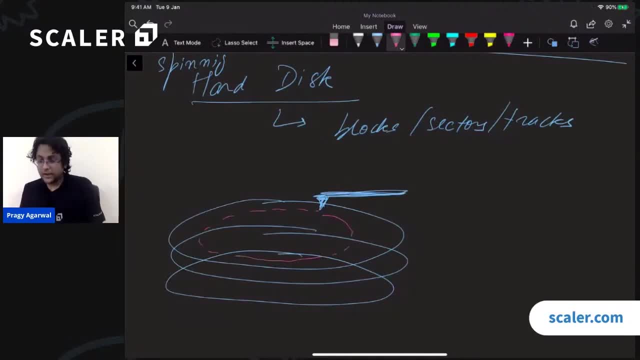 That is, tracking a particular track on this platter. Right Now, what you have to do is this: this one track, information across this one track is given, is, let's say, called a track And let us say this is one block. So usually this, this can be something like: 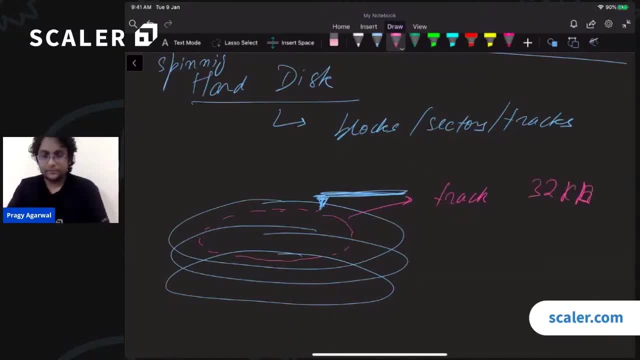 32 kilobytes. This could be 32 kilobytes, All right. Now what happens is, if you have to read, if you have to read any value within this, then that is very fast. Right, Then, that is very fast because your disk is spinning, Your magnetic disk is spinning at 1000 RPM. 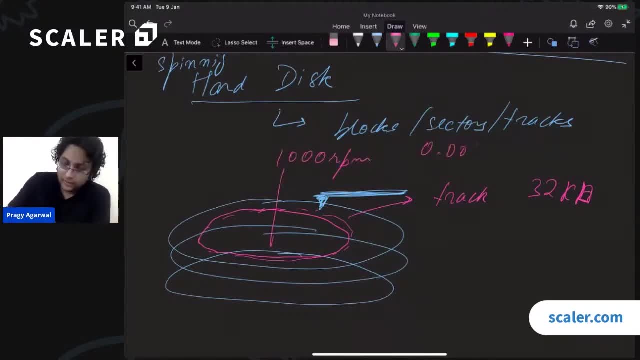 Right. So within within 0.001 second you can read this entire 32 kilobyte. you can read this entire 32 kilobyte block. But if you have to change blocks, if you have to move from this sector, if you have to move from this track to perhaps this outer track, if you 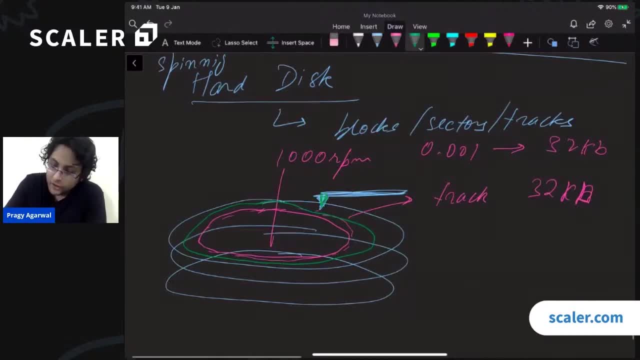 have to do that, then what you have to do is you have to move this head, You have to move this readhead, So you have to unplug this readhead. You have to run the motor to move it back, Then you have to plug it back, And that takes some time. So that that that 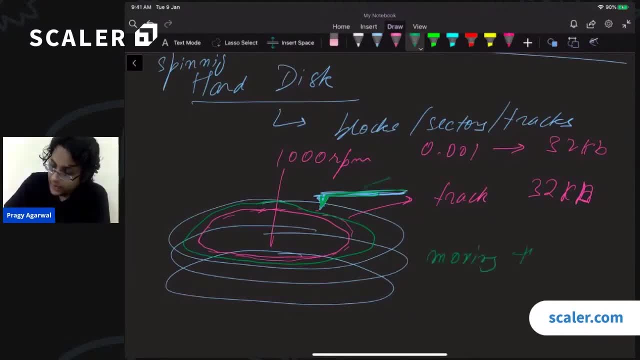 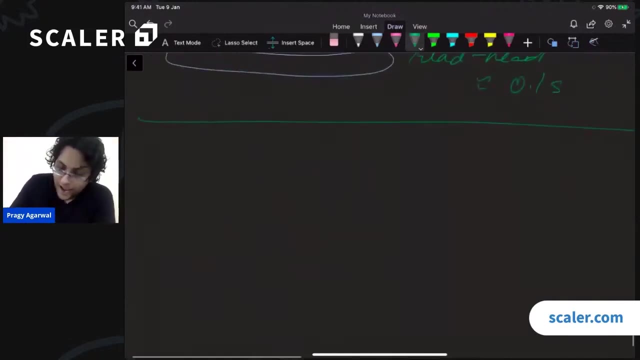 that thing that moving the readhead. moving the readhead can take a lot of time. It can take, say, let us say, 0.1 seconds of time, Right? So that is very, very slow. Is that clear? So it turns out. it turns out that what really happens, it turns out that what really happens. 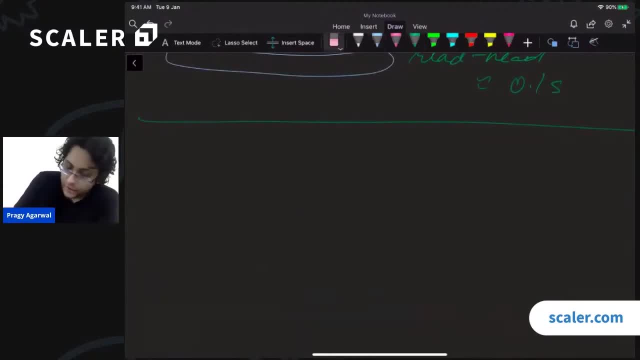 is. it could be the case that, due to this thing, due to this thing, it could be the case that making comparisons, making comparisons, Okay Okay, Making comparisons is fast, All right. You read 32 kilobytes of data in the memory And 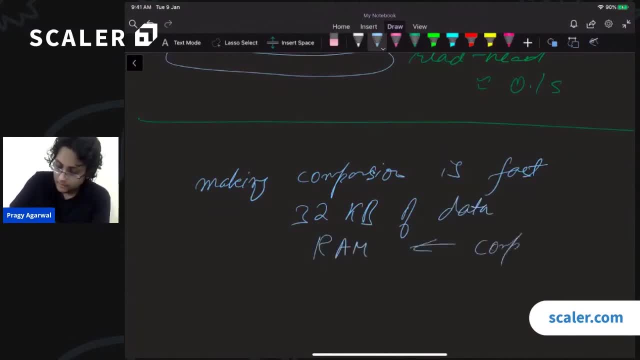 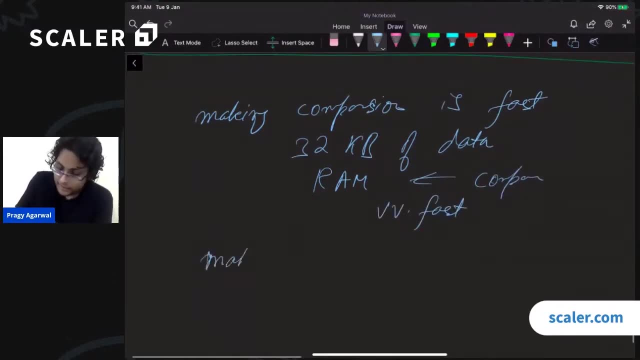 then, once the data is in your RAM, you're making comparisons in the RAM Right, And RAM is very, very fast, Very, very fast. On the other hand, making a guess is making a guess is slow. Making a guess is slow Right, Why? Because for every guess, for making a guess. 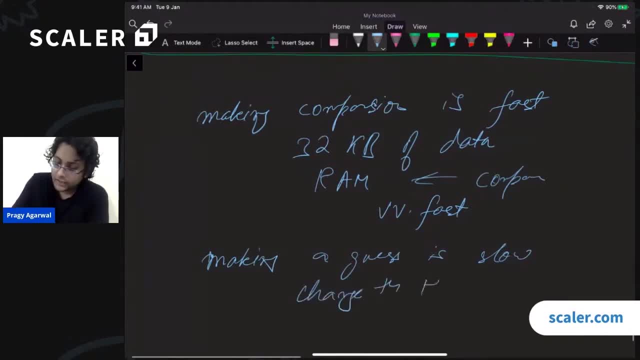 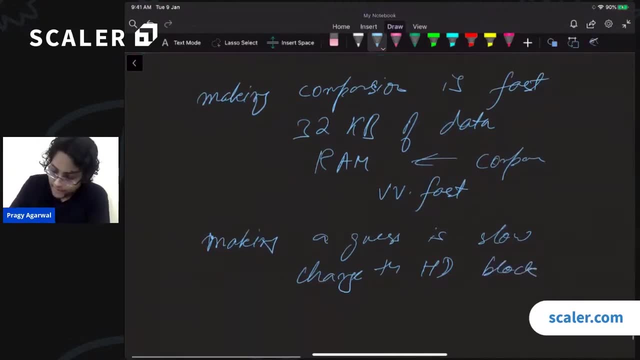 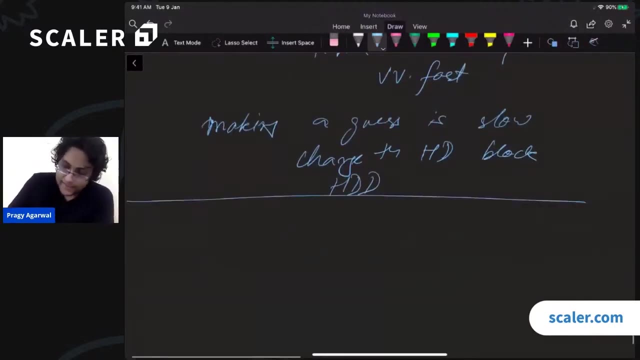 you have to change the block, You have to change the HARD vog And you have to move that. you have to move that read manually high, because this is this is happening at the hardest level. This is not happening at the RAM level. So what really happens in this case is making a guess. I want to reduce the guesses. I want. 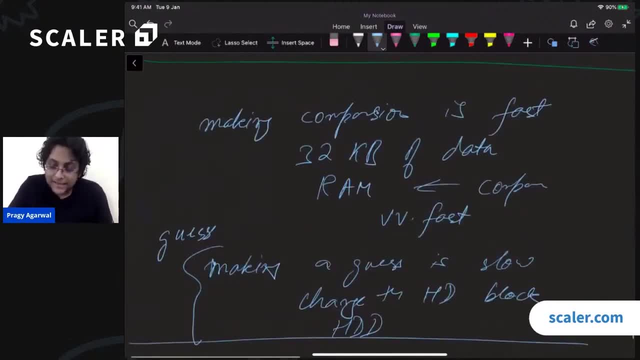 to reduce the number of guesses I make. I don't really care about the number of comparisons because the comparisons are happening in the RAM very, very fast. So in this point, in this sort of scenario, I want to reduce the number of guesses I make. I don't really care about. 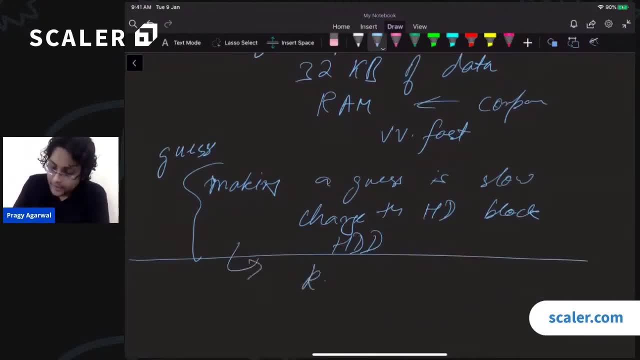 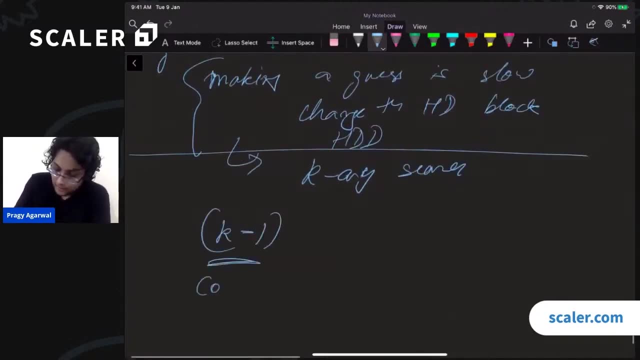 the number of comparisons Right. Now let's look at this part of the problem. For instance, let me talk about the prefer to use some sort of a k research, right? i would prefer to use some sort of a k research because in a k research, this is the number of comparisons, right, and this is the number. 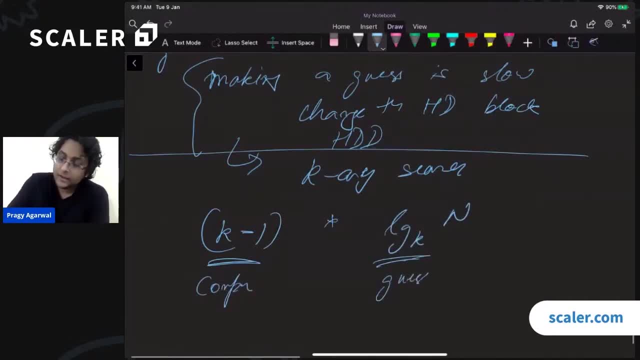 of guesses. this is the number of guesses. the larger the value of k is, the lesser my guesses will be right. the larger the value of k is, the lesser my guesses will be. so, basically, to maximize my efficiency, i choose a k which is equal to the block size. 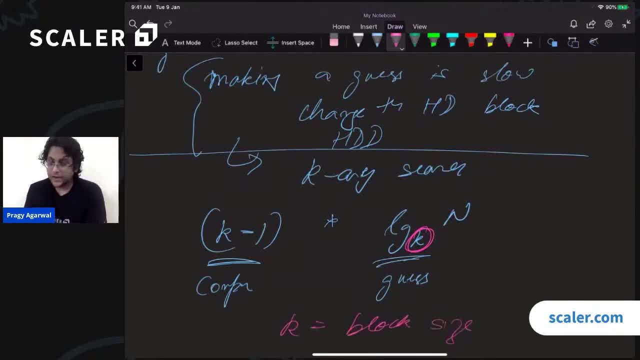 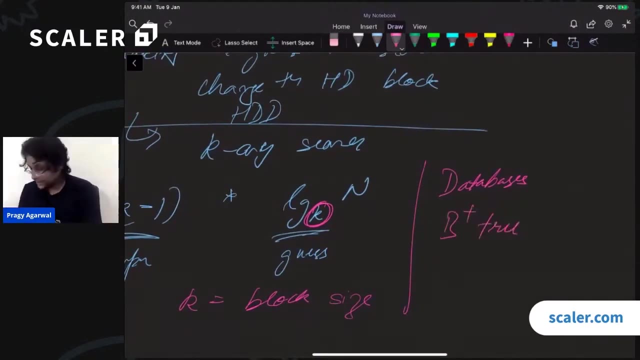 I choose a key which is equal to the block size and this thing, right? this thing is used all the time in databases. whenever you are using a database, the database internally is storing the data in some sort, in a thing called a B plus tree. right, it's something called a B plus tree. 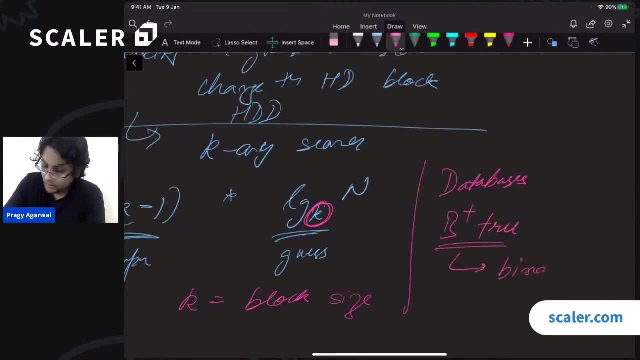 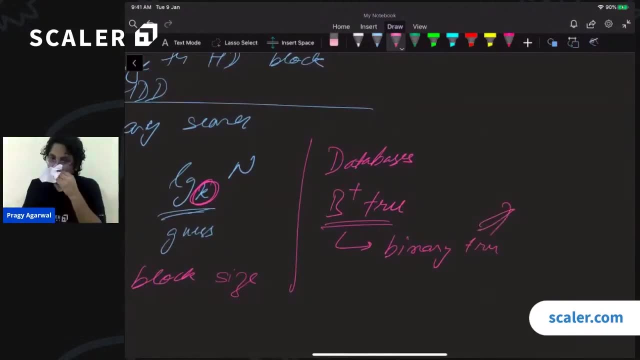 and a B plus tree is simply a binary tree- binary tree that has been extended. so so binary tree works in the binary search manner. right on a binary tree you can have a binary search tree and you can binary search on it. on a B plus tree, you can do a k research. you can do a k research. 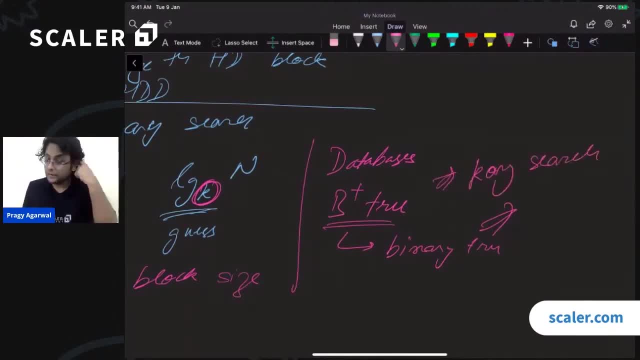 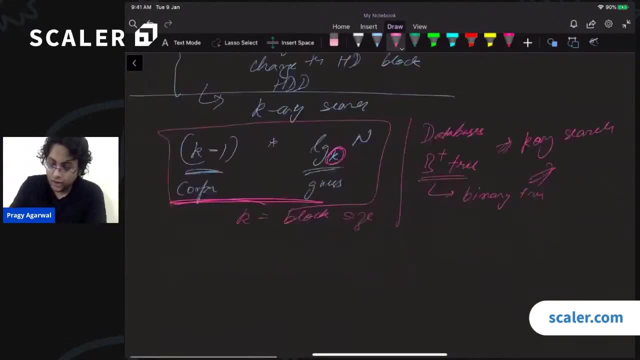 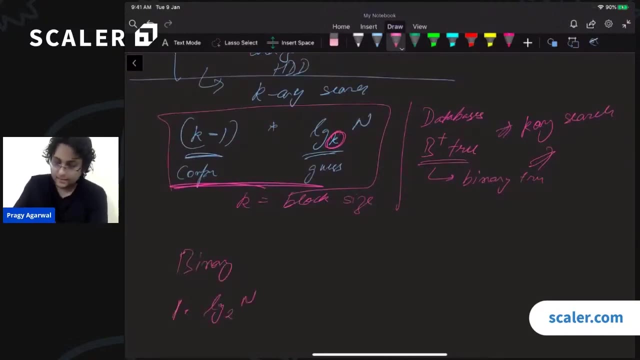 on a B plus tree. all right, how did you come up with this formula? so this formula is what we just saw, right? this formula is what we saw for binary. for binary search, we have one comparison and log base 2n guesses. for ternary search, we have two comparisons and log base 3n guesses. for k research, we have k minus 1 comparisons. 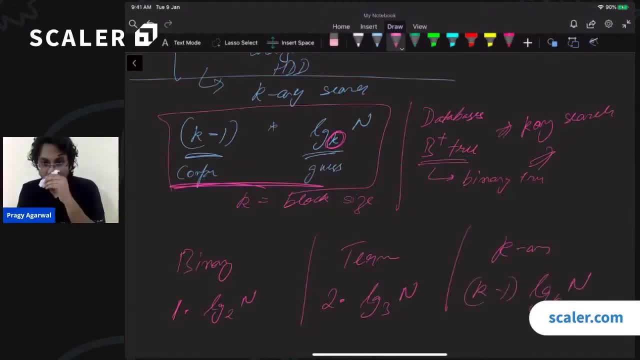 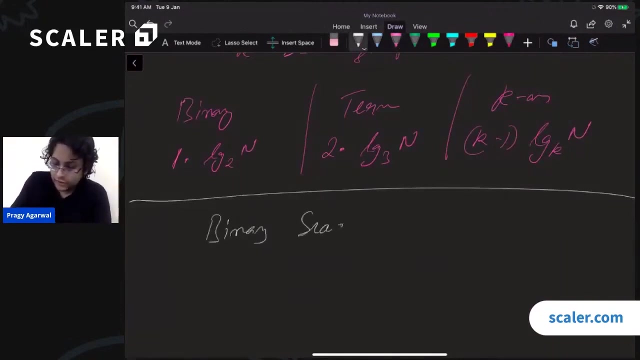 and log base k n guesses. all right, is that clear? this is multiplication. is that clear, guys? all right, so i think we are going to leave it at this. right, we are already above the time. so today we basically discussed binary search, binary search. we saw how to implement it, right, we saw how to implement it and we saw that this 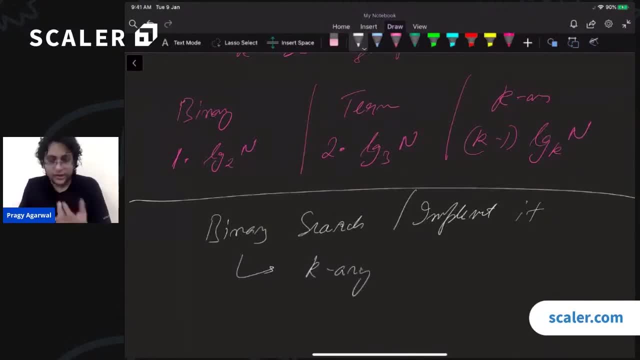 idea can be extended into a k research, into a ternary search or a generic k research. k research is generally slower, right. generally we would like to do binary search, but there are cases. there are cases, for example, databases, in which k research is very, very valuable. okay, cool. now i would want each of you to, once this lecture is over, to find the link in the video. 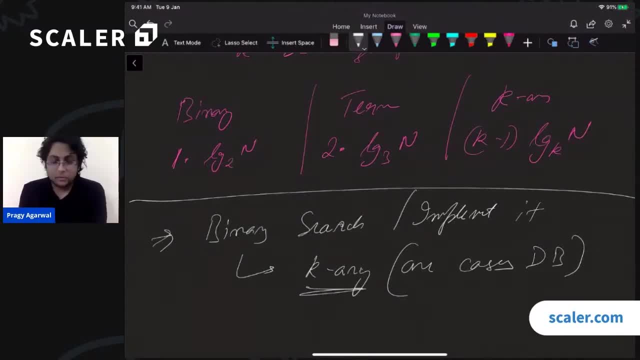 description or there's a link to the assignment right today's assignment. so please go over there and i mean try to try to solve those problems. so those problems will be on basic binary search. there are some things that we were not able to discuss, like binary search on a rotated 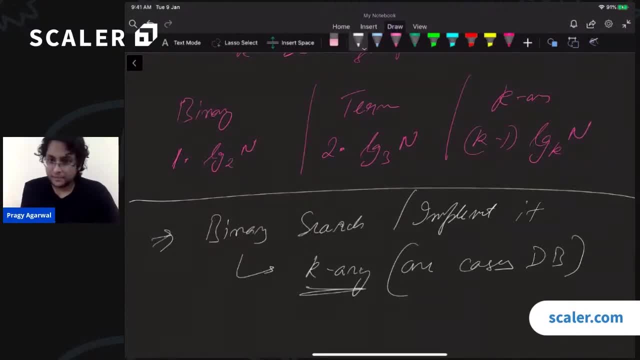 array, like finding the peak element. we can discuss it in the next class, all right, all right, guys cool, will we cover interview? interview with problems from your website? yes, reshma, so all these problems. so that is why we give you the assignments. right, we are discussing the problems. 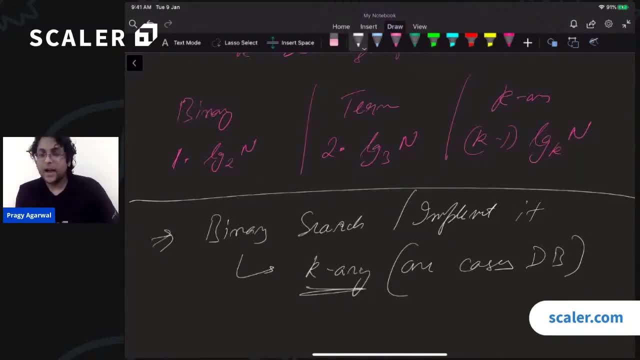 that are part of those assignments. okay, i mean, of course, when we are actually doing a scalar class, i mean when someone joins an academy, we usually have three hour classes, right, and i mean we have classes every single day for three hours. so that gives us a lot of you know a lot of. you know a lot. 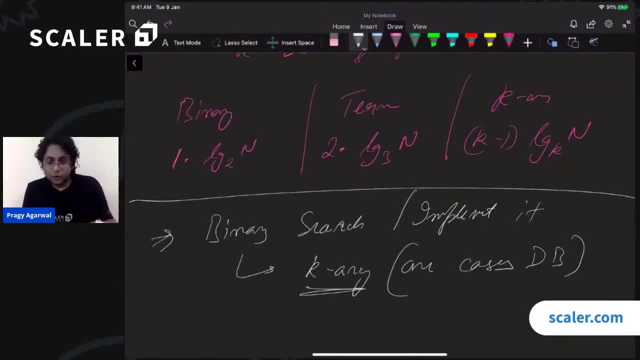 time to work with the student, right, so they are able to solve many more problems. we won't be able to do that on youtube, right? so i understand that you won't be able to get the exact same experience as killer, but that's to be expected, right, because this is on youtube. all right, then, so please make. 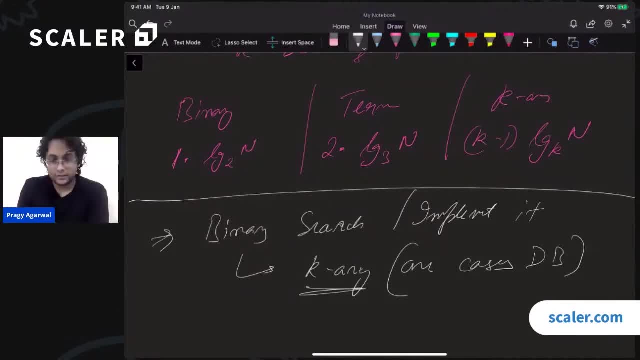 sure that you solve the assignment. please make sure that you are taking notes while you are studying the lecture and see you in next class. in the next class i will continue. we will continue with binary source and you will be looking at more advanced problems on my research. okay, perfect, uh, if you want to join. 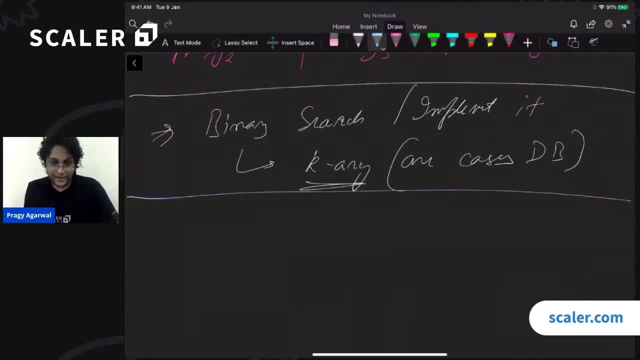 scalar. well, uh, we don't really announce the dates during lectures, so whenever, if you are, if you are trying to join scalar, just go to scalarcom, right, and any announcement, any announcement about a new batch, announcement about a new batch will be made over there, right? so please, please, monitor the. 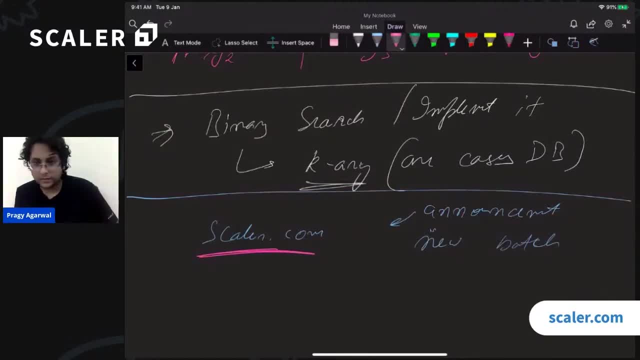 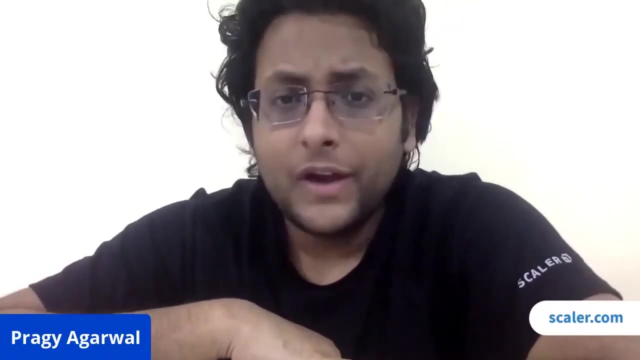 scalarcom website and any announcement about any new upcoming batches will be made over there. right? so let us end the lecture then. all right, bye, bye, guys, have a nice day. we are back with another lecture today. we are going to continue binary search. we are going to 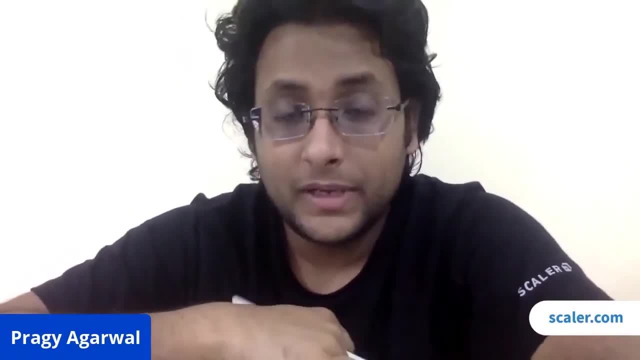 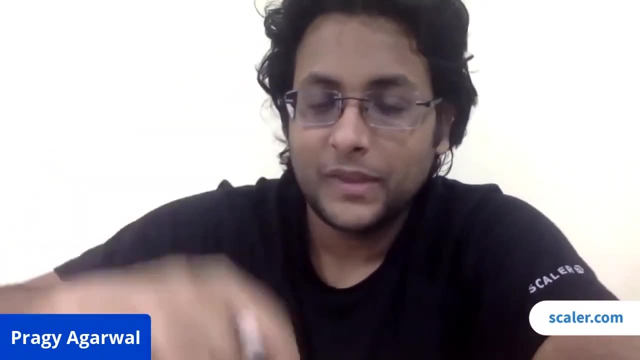 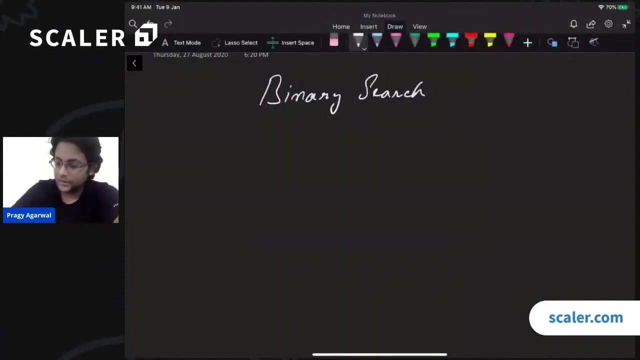 look at some questions or that have been asked in companies, or in some of the top companies right, regarding buying research. now, without further ado, let us start the class. so let me just share my screen, all right, i hope that everyone can see the screen and whatever i am writing over here. 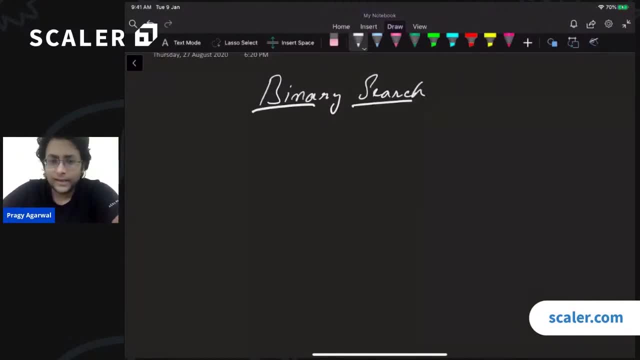 cool, so let us start with a question directly. so we had yesterday. we had looked at what binary search was and how to implement binary research. let us dive into one question today. okay, so suppose that you have been given an array right and this array has n integers. 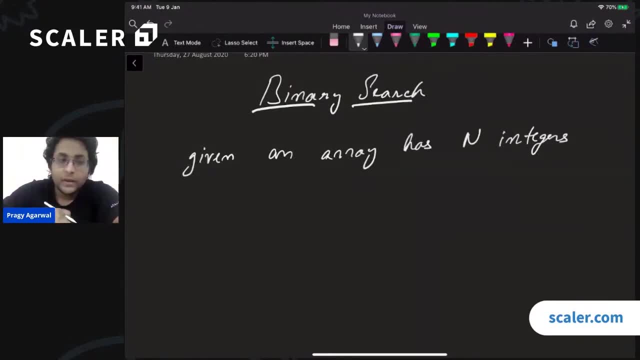 all right. now it has also been told to you that in this array, all elements but one come twice, come twice. all right. also, it has been said that the array is sorted, array is sorted. So let us first take an example of such an array. Let's look at such an example. Let's say that we have 0, 0. We have 4, 4, minus 1.. We have, let's say, 5.. We have 5 over here, suppose. Then we have, let's say, something like 7, 7. And we have 8, 8.. 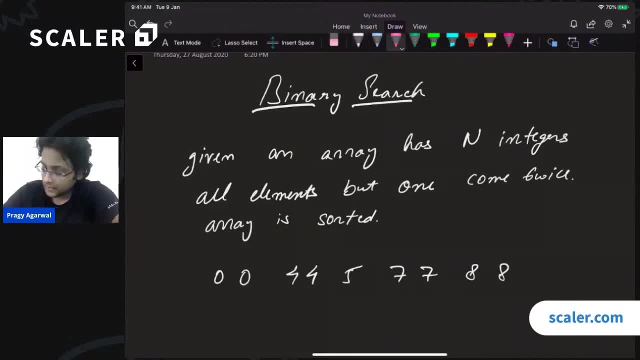 Right. So in this array we see that every element has been repeated twice. There are 2 0s, there are 2 4s, there are 2 7s, there are 2 8s, except for one element. Except for one element, every element is repeated twice. Also, this array is sorted Right, So it is sorted in ascending order. I hope my voice is clear. 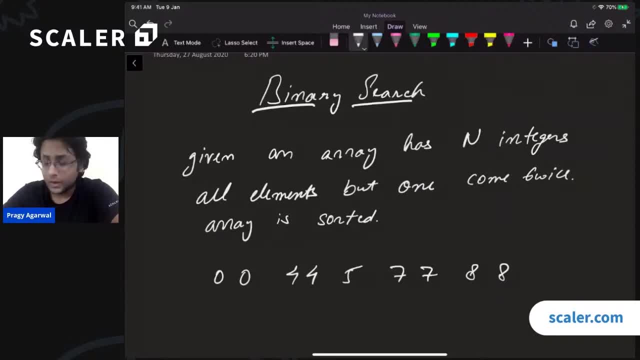 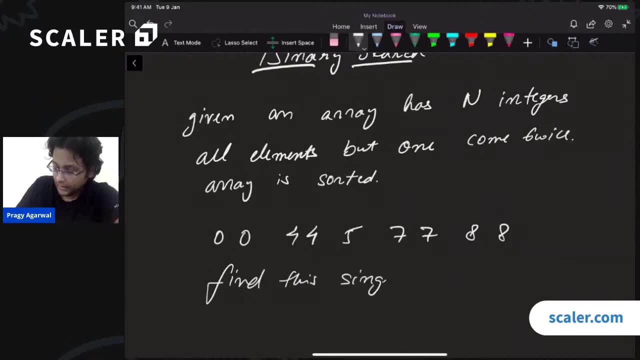 All right, Cool. Now the question says you have to find. you have to find this singlet element, Right, You have to find this element, which occurs only one time. So if this was the array that was given to you as input, then you are supposed to return 5.. Is the question clear? 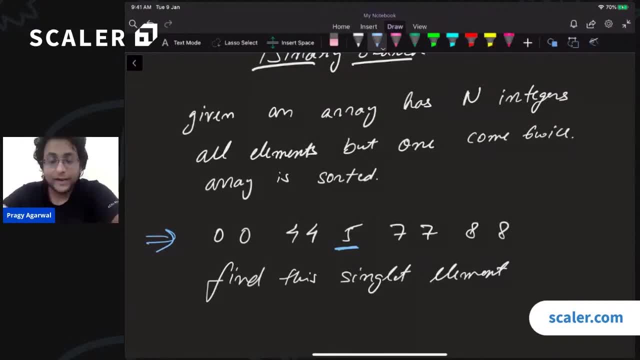 Yes, So we have been given an array, It is sorted. Every element in the array occurs twice except for one element, And we have to find that one element that occurs only once. All right, So let us see some approaches. Let us see some approaches. 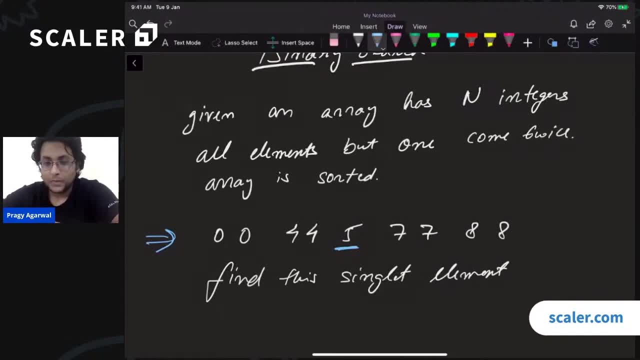 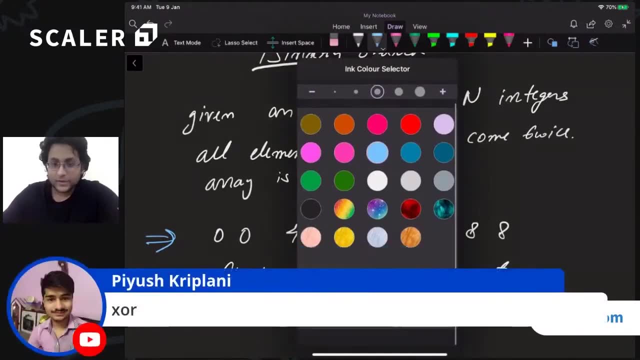 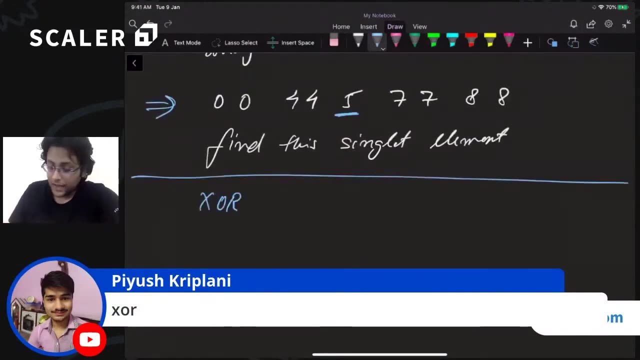 Hmm, So Piyush has a very nice idea over here. So Piyush has a very nice idea over here. Piyush says: let us try XOR Right Now. we all know the property of XOR. We have seen that in the bit manipulation class That XOR acts like a lock and key. Lock and key. 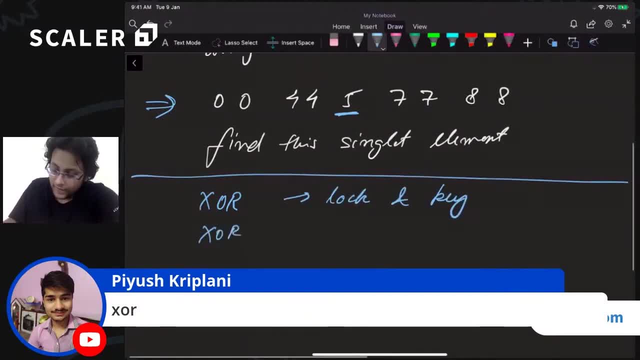 Right. Basically, if I XOR the entire array, if I XOR the entire array that is supposed to give me that, That element that occurs only once, Right That element, I am supposed to get the correct answer. because all these things will cancel Right 0. XOR 0 will cancel 4. XOR 4 will cancel 7. XOR 7 will cancel 8. XOR 8 will cancel And I will be left with 5.. 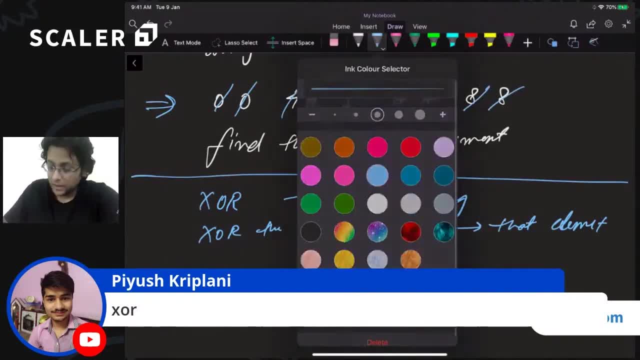 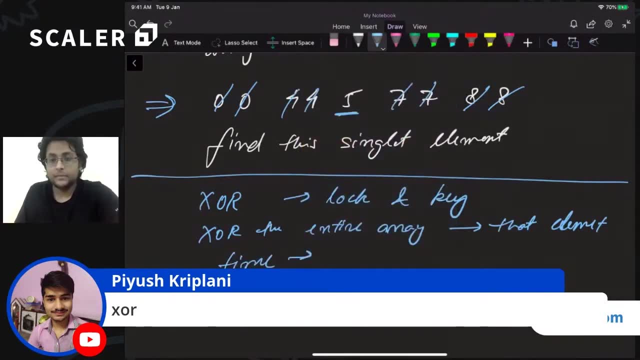 So, yes, that is a valid approach. That is totally a valid approach. What is the time complexity of this? How much time will this take? How much time will this take? This will take an order of N times. have to go over each element and check. right, we have to exhaust each element. all right, cool enough. 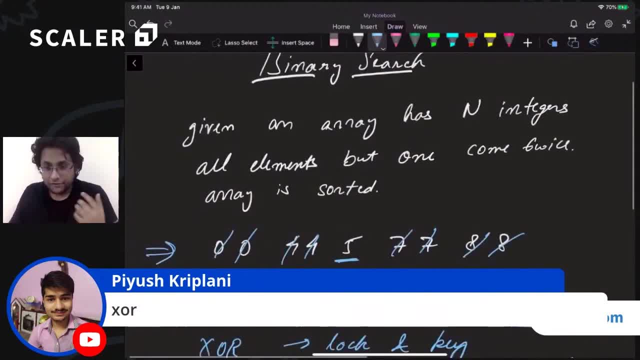 can. can we do better in this? using this exotic, are we first of all making use of this property? we know that the array is sorted, right, we know that the array is sorted. so either if we use xor or if we use a map to keep account, then we are not really using this sorted property, right? 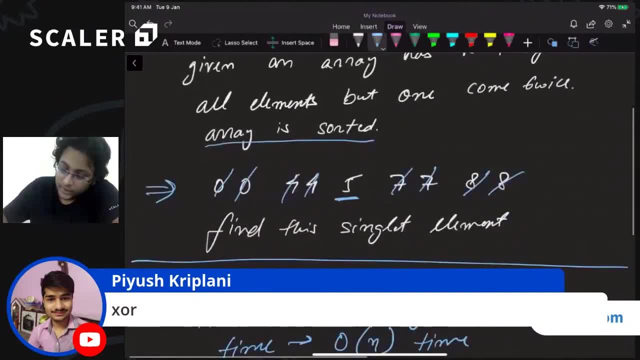 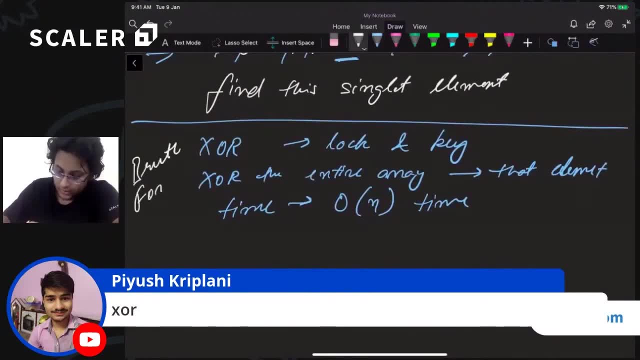 they are going over each element. so let us let us try to make use of the sorted property and see if we can reduce the 10 comments. so this is a this is a valid brute force approach. this is a valid brute force approach, but let us come up with an optimized solution. 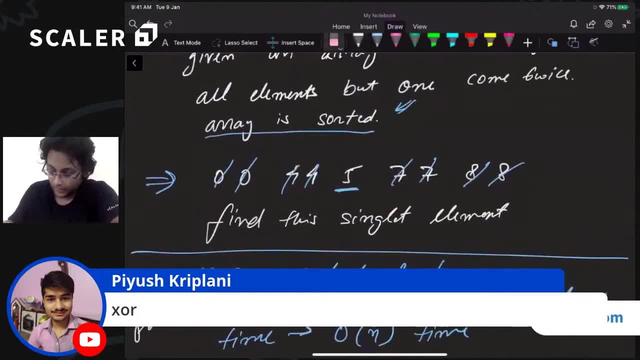 that exploits the property, that the array is sorted. yes, let us see if we have some other approaches. all right. so yes, a binary search would be the answer here. but what exactly are you going to do with the binary search? how exactly are you going to search it? 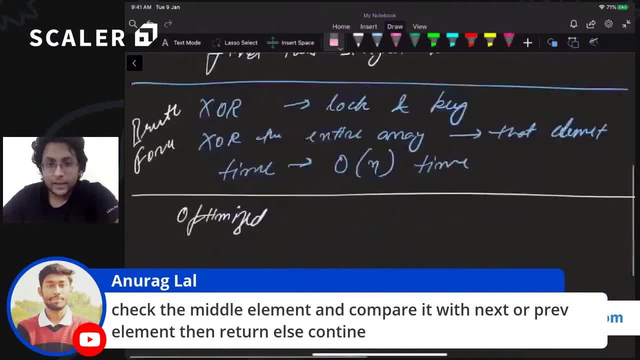 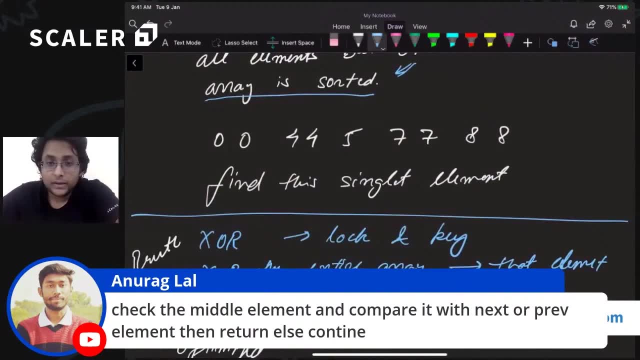 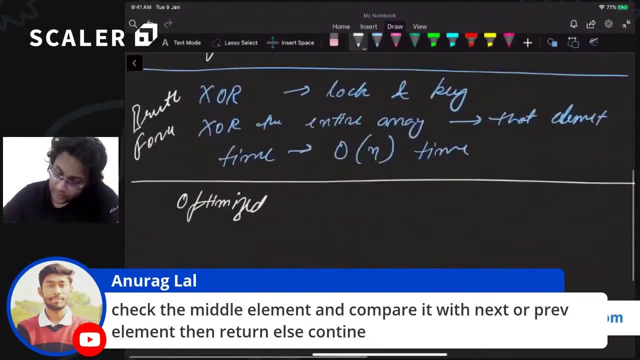 all right. so anurag over here says that let us check the middle element. let us check the middle element, all right. let us suppose we have some middle element and what anurag is saying is: let us compare it with the previous or next element, right. and then return. well, let us suppose that this array was a little longer, right? let us say: 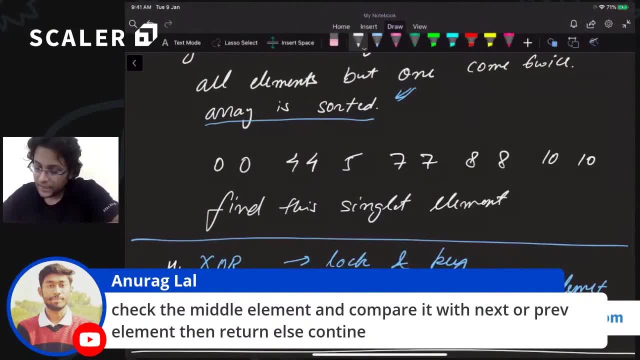 that we had 10 over here as well. so when you find the middle element, let me just let me just add the 1. this is zero. one, two, three, four, five, six, seven, eight, nine, ten, right, so what will be the middle element? this will be the middle element right now. if this is the middle element, then we compare it. 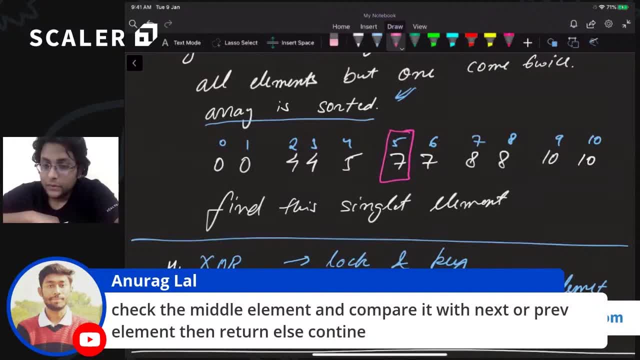 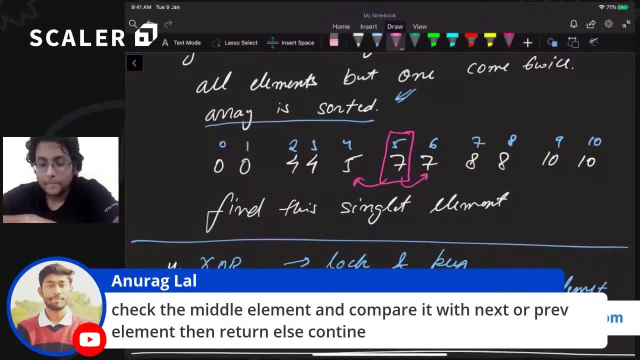 with the left and right element, and what exactly do we do? what exactly do we do? so? we look at both neighbors. we look at both the neighbors. all right, this is five and this is seven, so how does that help us? how does that help us? it doesn't really help us, right? hmm, okay, so what? what can we do then? 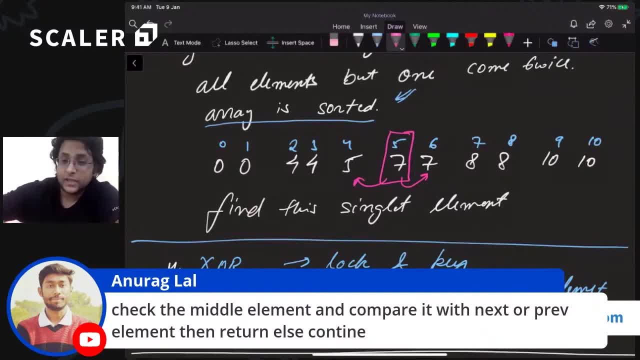 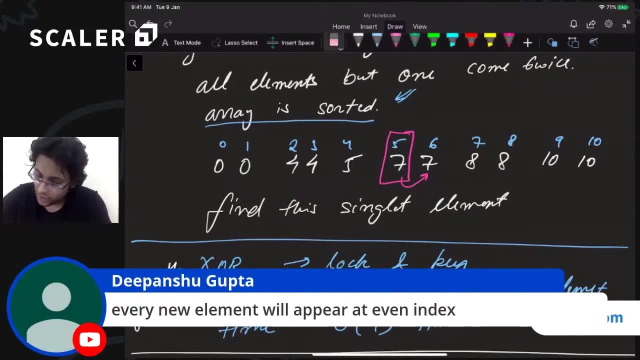 yes. so dipanshu has a nice idea over here. let me just show dipanshu's comment. so dipanshu says that let us observe one thing. let us observe one thing: that whenever a new element comes, whenever a new element comes, it always comes at an even position. 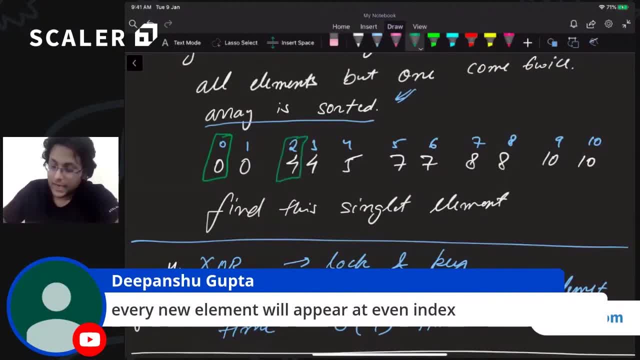 right. whenever a new element comes, it always comes at an even position. yes, is that correct? until and unless? until and unless that middle element comes, after that, every new element comes at an odd position. do you all agree? yes, the first occurrence of any element is on an even position on the left. 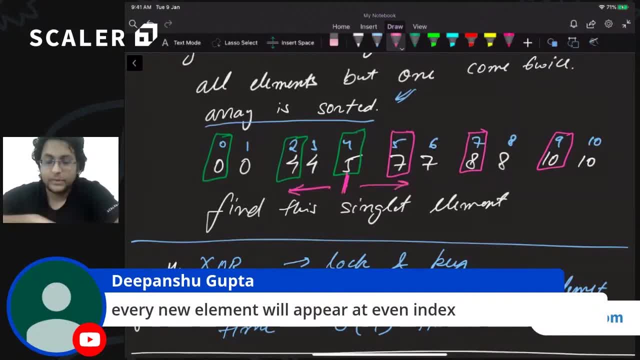 side of the smith and is on an odd position on the right side of the smith. do you guys observe that? so we are going to use this property, we are going to use this observation to find out what the what, the single occurrence element is right. so suppose that we do something like this. suppose that we do something like this: 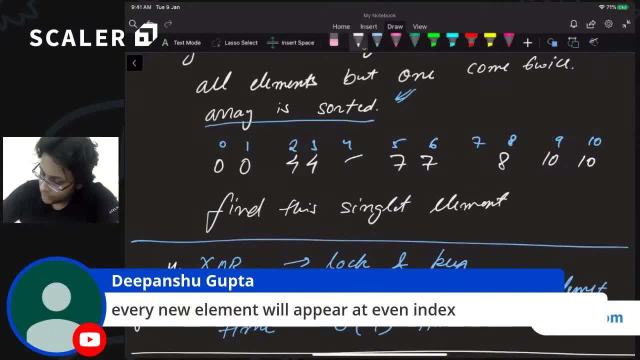 we, we pick. so we have a high and we have a low. so this is five and this is eight. we have a low and we have a high right. let us calculate some mid right. let us calculate some mid. what we will do is this mid will be, let us say, a of smith. 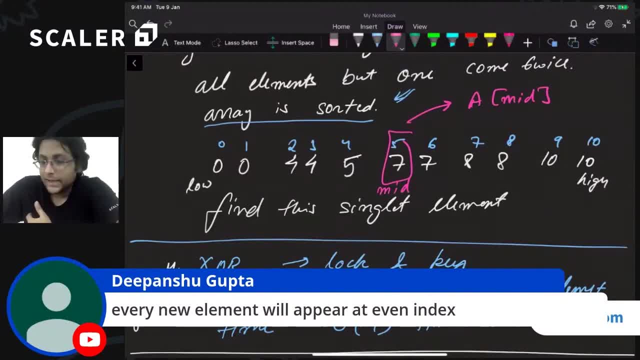 this a of mid. it might be the first occurrence of this value, or it might be the second occurrence of this value, right, we don't really know. this seven, this seven that we landed on, this could be the first occurrence of seven, or this could be the last occurrence of seven, right, we don't really. 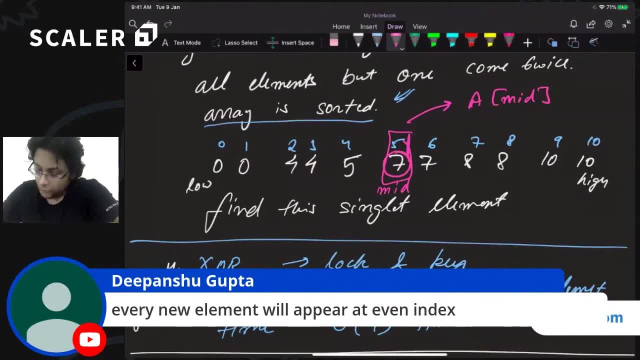 know. so, if so, what we can do is we can find the first sequence of seven. suppose that we landed on this bit, suppose that we had laden of this bit. then we can compare it with the previous element and always find the first occurrence. first occurrence, occurrence of a of mid. 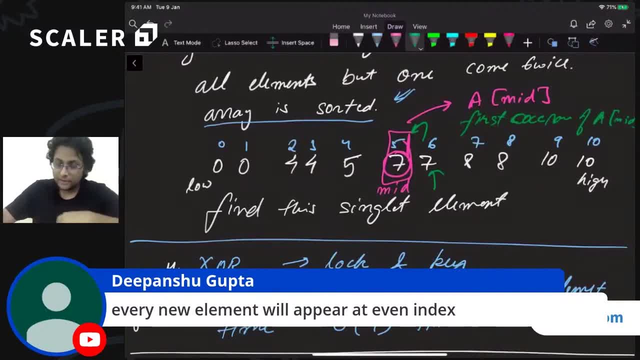 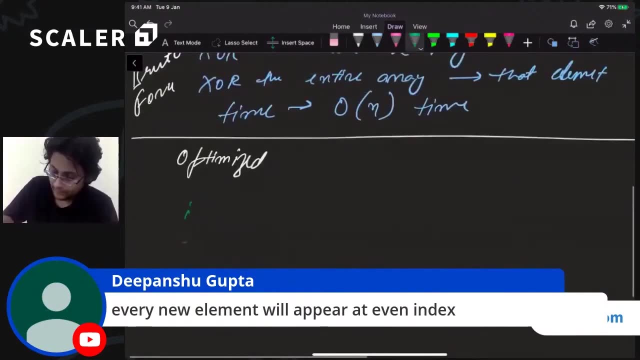 can we do that? yes, given a mid number, can we find a of mid? and then can we find the first occurrence of the output? it will either be that element itself or it will be just the previous element. right cool now. once we have that, once we have that, we can check if the index, if the index of 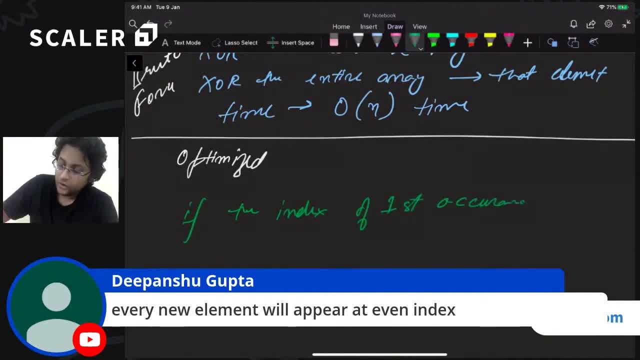 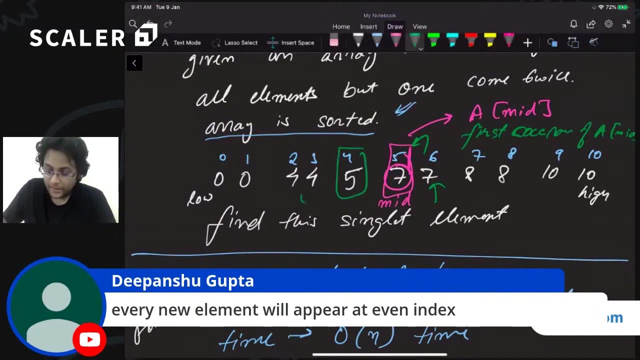 first occurrence, occurrence of a of mid right. if this is what, even if this is even, then what does that mean? what does that mean? that the element, that the singlet element lies to the right of me, right whenever i, i find the first event occurrence at an even position. 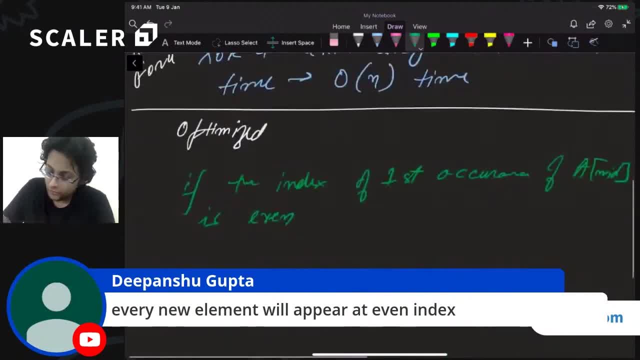 that means that a single singlet element lies to the right of me, so i will move right in this case, right on the other hand, if this is not the case, if it is odd, then i will move left. yes, and i will also have to stop at something, right? 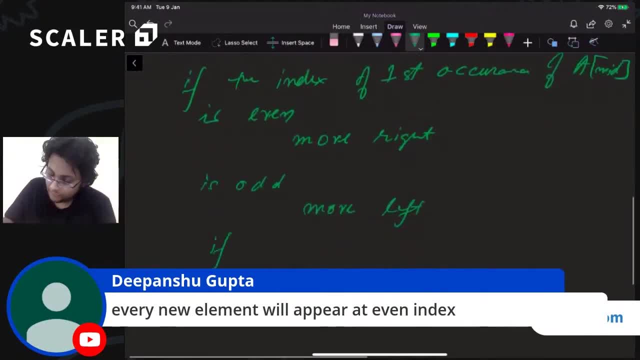 i will also have to stop at some point so i can check. i can check: if a of mid is the first occurrence, first occurrence and there's only one occurrence, right, so a of mid plus one, mid plus one is not equal to a of mid, then i know that i have found my singlet element, because 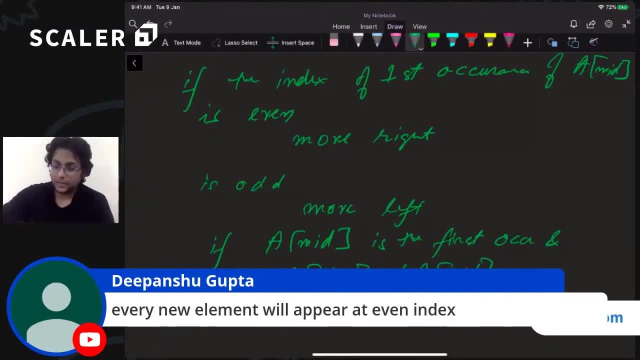 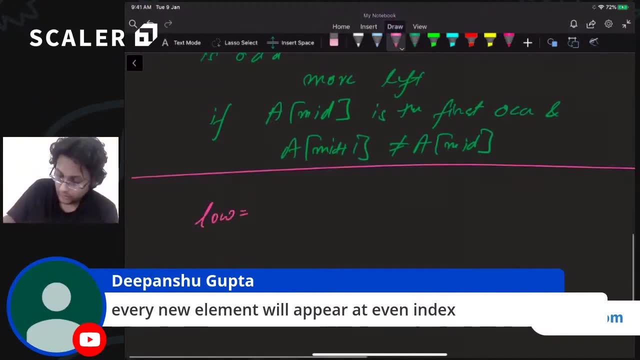 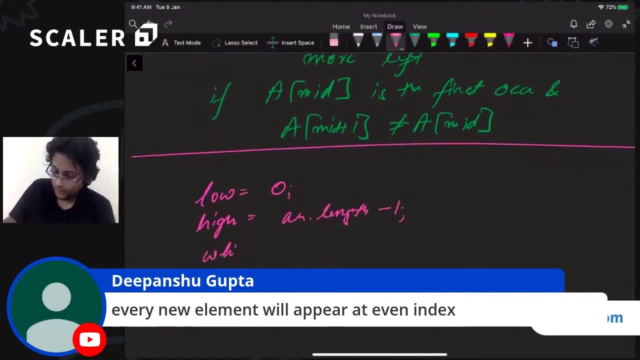 it occurs only once. does that make sense? yes, so what will be the very quick pseudo code for this? so we will have: we will start with low equals to zero. we will start with high equals to length of so ar dot length minus one right. then we will loop while low is less than equal to high, right. what will we do? 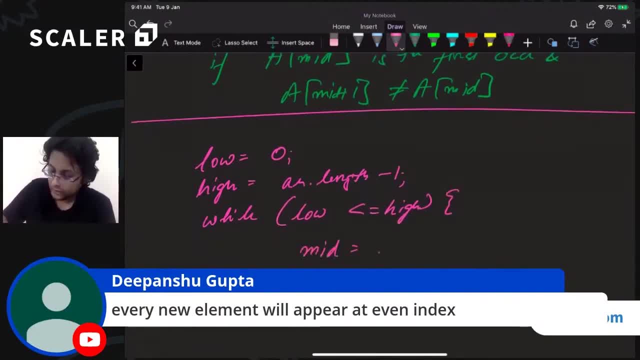 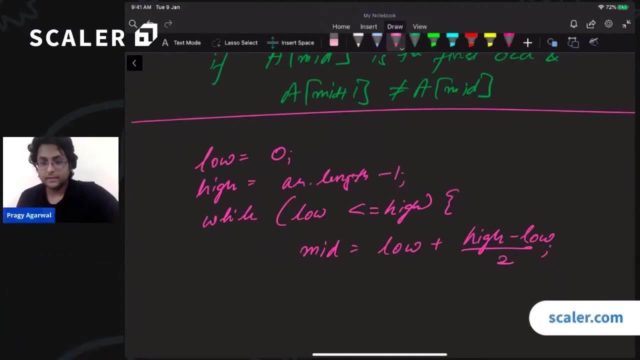 so we will calculate the mid force. so we will say: mid equals to low plus high, minus low by two. yes, we just calculated the mid. the bool say express twin command, surely? uh, yes, cool, all right, so we calculate the mid, then we can check. so we will first check. so we know that. 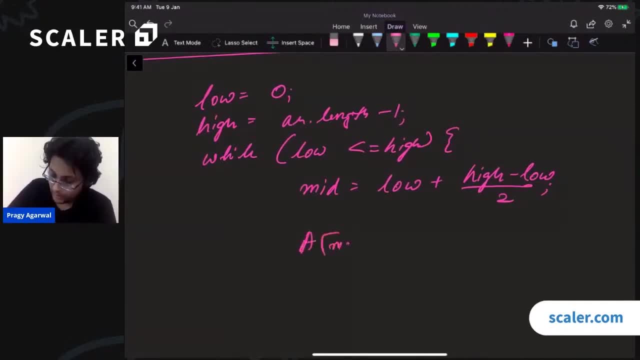 we know that we have to find the first occurrence of a of mid right. how do we find the first occurrence of a of mid? well, we can check over here. we can check if a of mid minus one equals to a of mid right. if this is the case, then a of mid is the second occurrence and not the first occurrence. 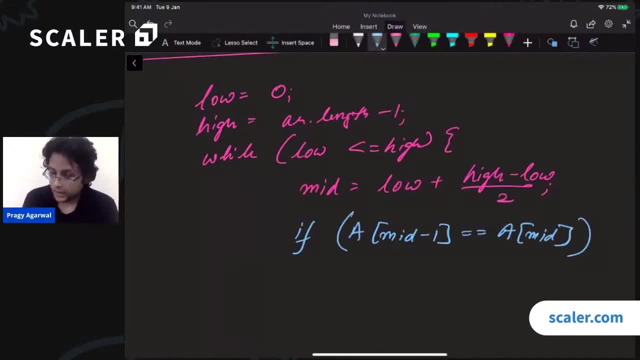 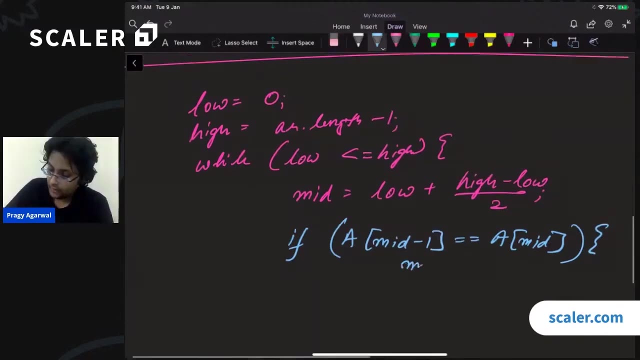 do you agree? yes, if a of mid minus one is equal to, equal to a of mid, then a of mid was the second occurrence, because the previous element is also equal to. in this case, what is the first occurrence? the first occurrence is mid minus one, right, in this case, the first occurrence is mid minus one. 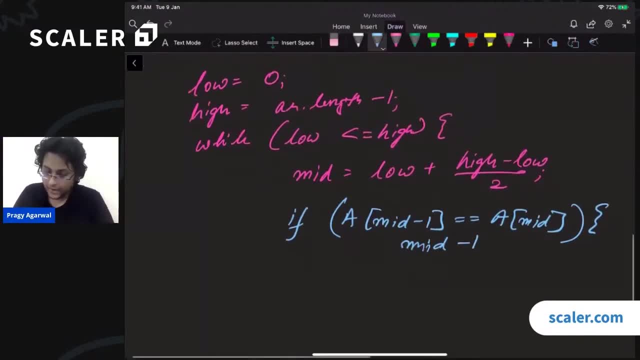 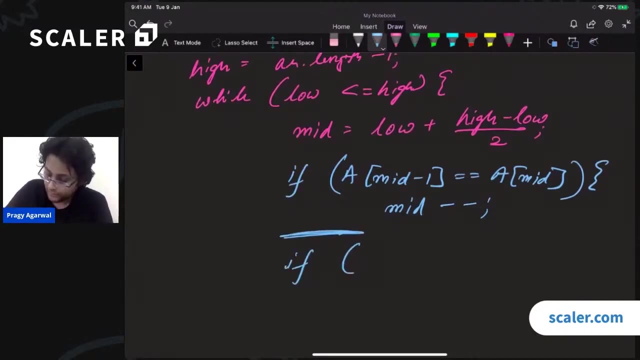 otherwise the first occurrence is mid itself. right, all right. so what, what i can do is over here is i can do mid minus minus, mid minus minus. and then over here, my mic contains the index of the first occurrence. now i can check. now i can check if mid is even or odd. so if mid 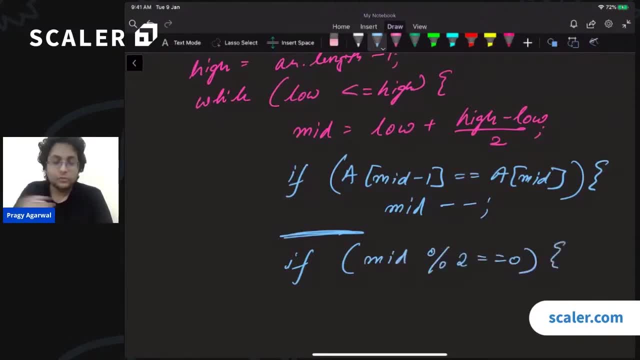 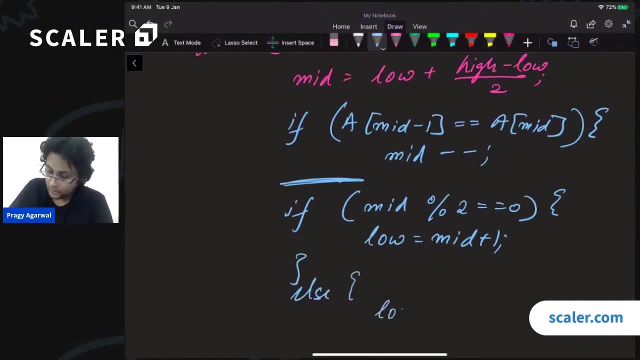 is even what two equals three equals to zero. then i have to move towards my right. yes, i have to move towards my right. how do i move towards the right? i say low equals to mid plus one right. otherwise else i move towards the left. i say low equals to- oh sorry, high equals to mid minus. 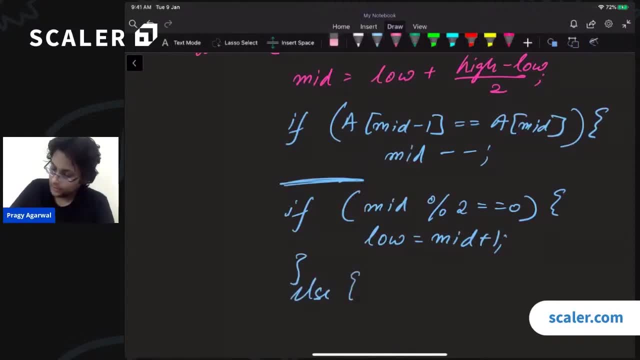 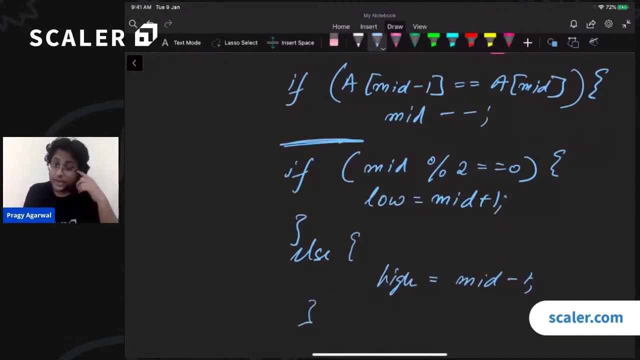 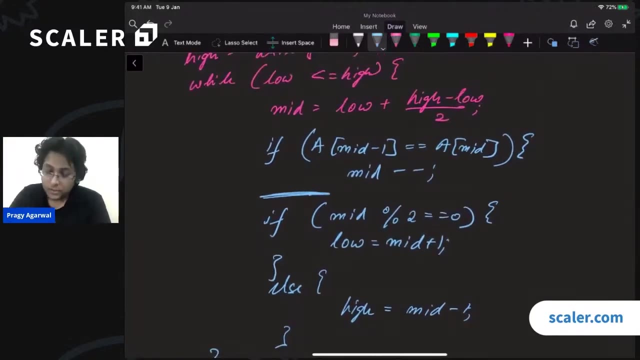 one. i simply say: high equals to mid minus one right, perfect. but that does not really tell me when to stop. right, that does not really tell me when to stop. so i have to make some other checks as well. also, there is one more problem over here, that what if? what if this mid turned out to be? 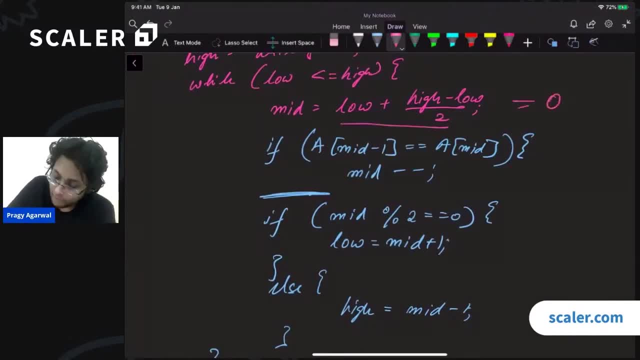 zero. what if this mid turned out to be zero? then this a of mid minus one will give me an index error, right? i will be trying to index at a negative value. that is not good, right? so i have to take care of these things. so, first of all, what i can do very quickly over here is i can first 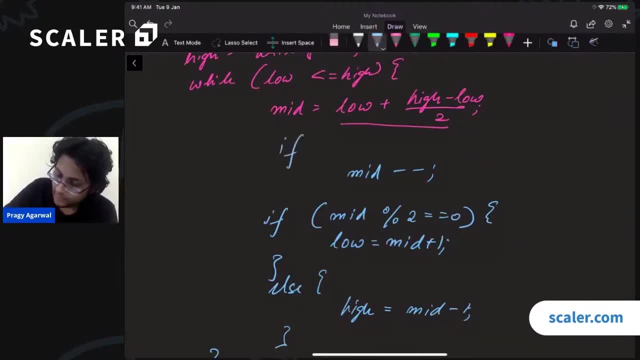 confirm this right. i can first fix this thing. i can say: if mid is greater than zero right and a of mid minus one is equal to equal to a of mid right, then do mid minus minus, then do mid minus minus. so after this point, over here at this line. 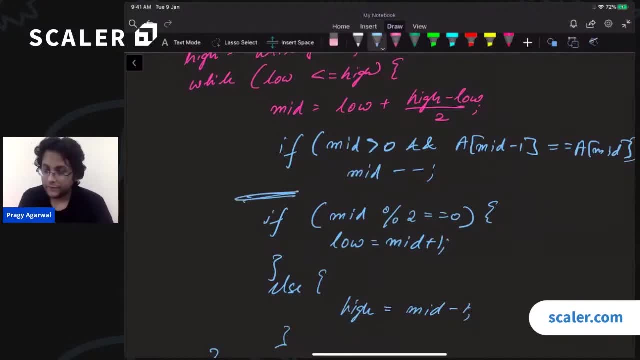 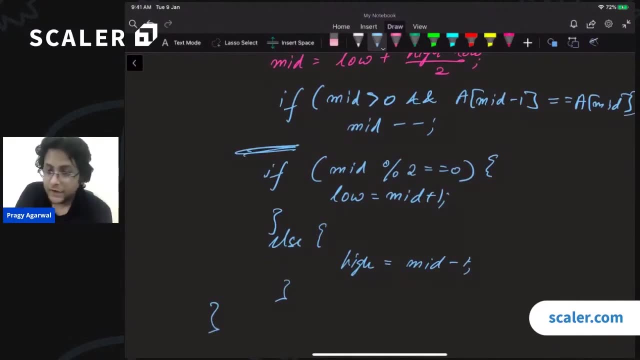 mid will be the first occurrence of a of mid right. min will be the first occurrence of your. now, if mid is even, we do look as we increment the low, else we increment the high. but once again, when do we stop? once again, when do we stop so we can check over here, if a of mid plus one right, if a? 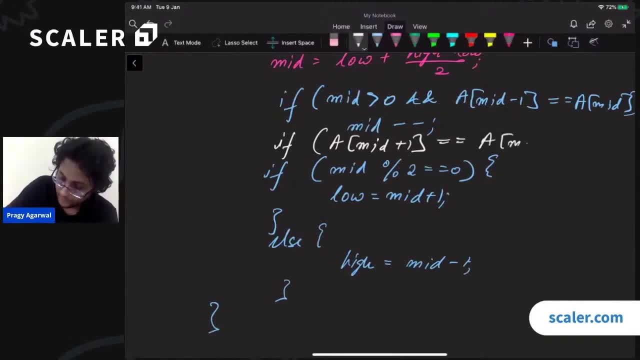 of mid plus one is actually equal to a of mid. is is not equal to a of mid, my bad, so we we have the first occurrence of this element, right, we have the first occurrence of this element, and if the next element is not the same, then we have found the correct location. right, then we have found the. 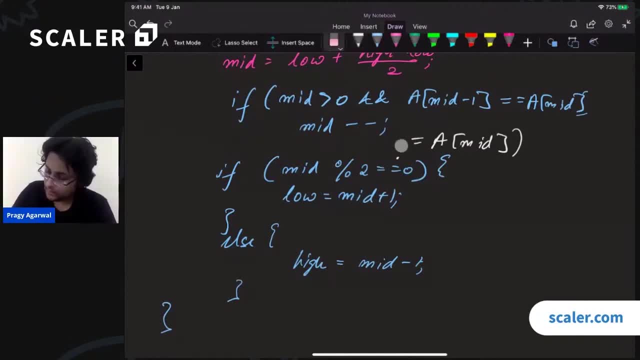 correct location. so what? what i can do over here is let me just erase this and write it properly. and also, we will have to make sure that we check the boundary condition right. so we will check if mid is less than you is less than n minus one, and a of mid plus one is not equal to a of mid. 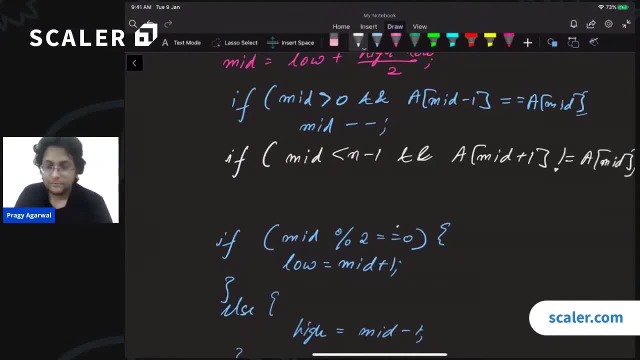 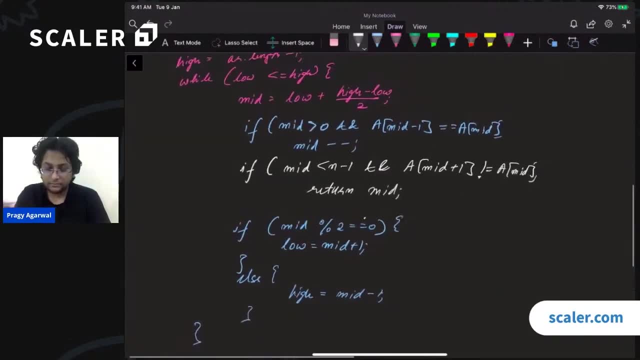 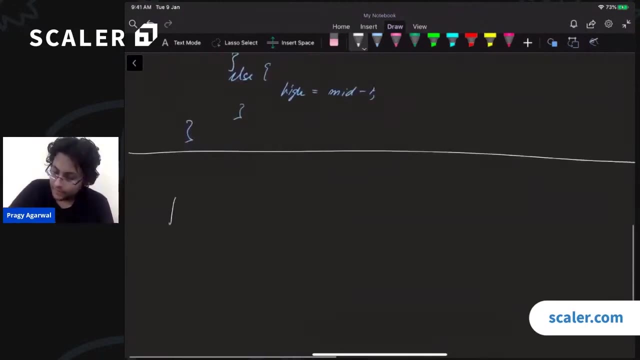 then what do we have? we can just return. we can just return the mid, because this is the correct answer. is that clear? yes, is the approach clear? so the approach is very simple. the approach is just saying that once you have these elements, once you have these elements, all the elements. 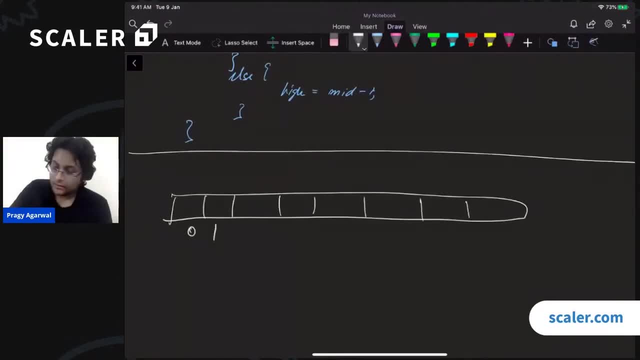 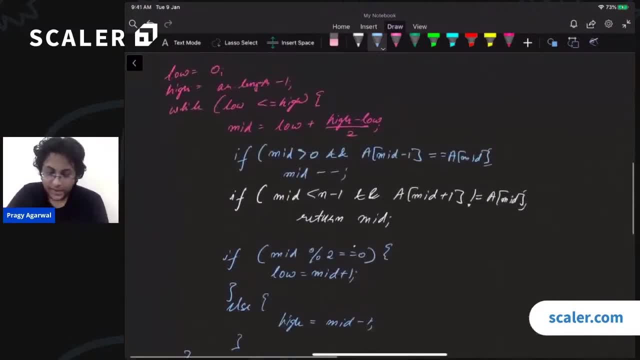 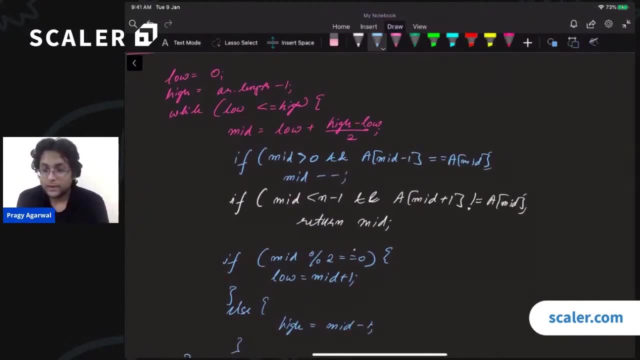 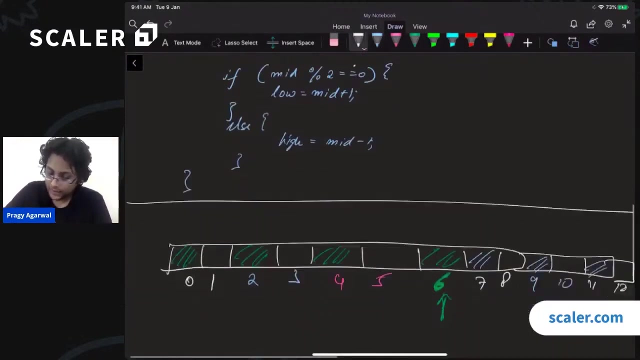 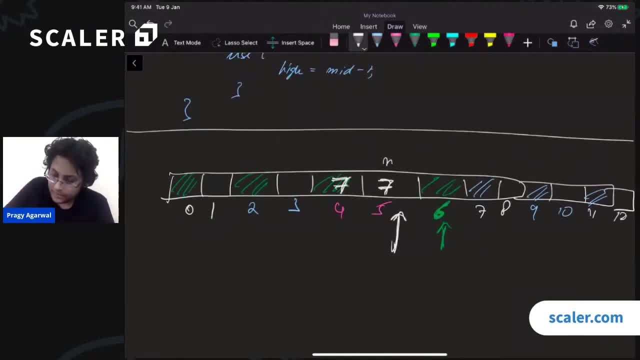 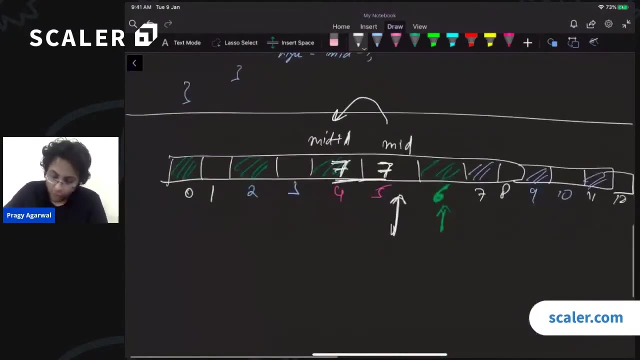 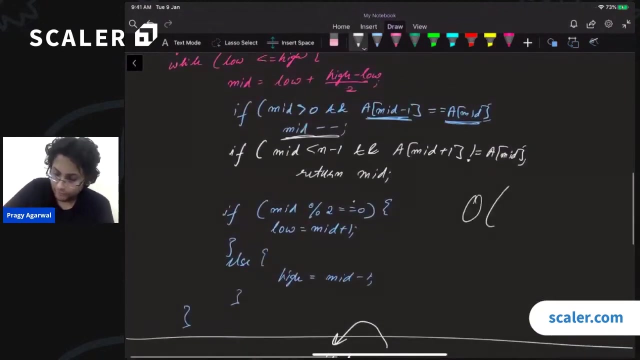 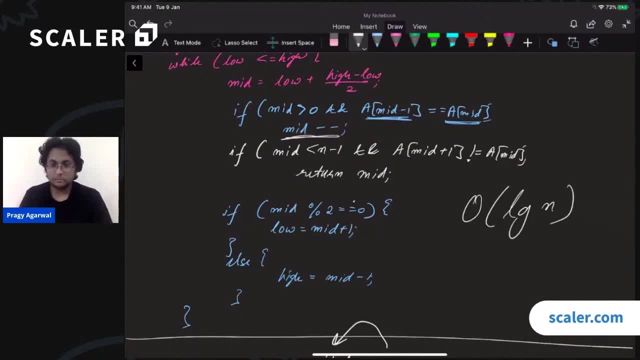 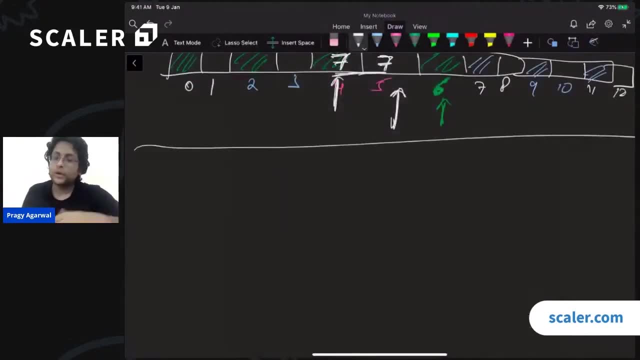 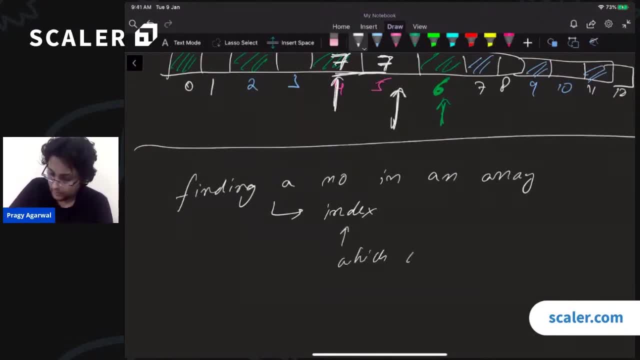 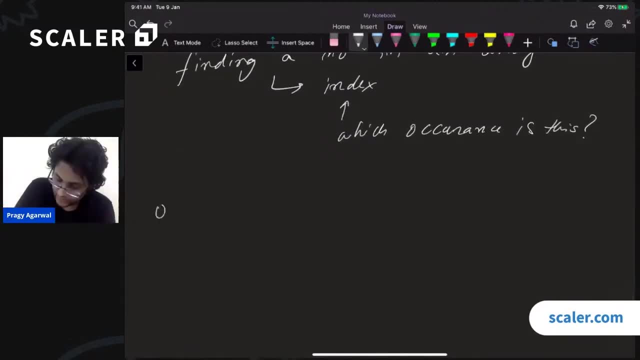 What occurrence is this? Which occurrence is this? Which occurrence is this? Basically, what I'm saying is suppose that I have a sorted array- 0, 1, 2, 2, 2, 2, 2, 3, 4, 5, 6. It's suppose that I have this sorted array. 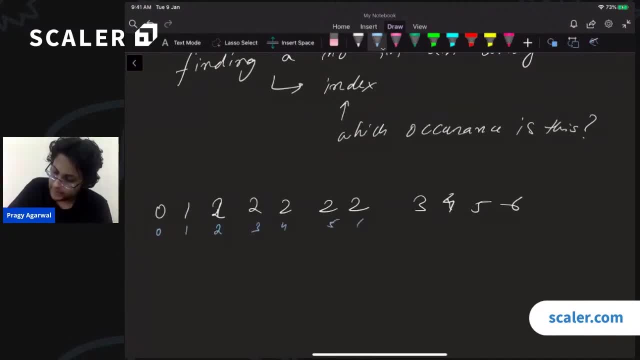 Right, So this is index 0, 1, 2, 3, 4, 5, 6, 7, 8, 9, 10. Now suppose I want to find the value 2. I want to find the value 2 in this array. So when I'm searching for the value 2, the value 2 occurs at more than one indices. 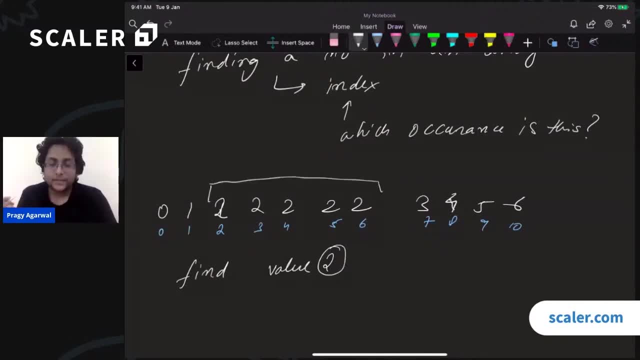 It occurs at all these different indices. So what index should my binary search really return? That is the question, Right? So yesterday we saw that, okay, We were, we were returning an arbitrary index, right. as long as we found the index, It doesn't really matter what occurrence we were looking for. 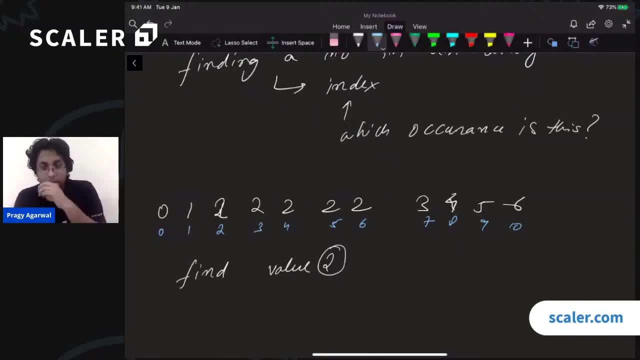 Right. So I mean that is perfectly fine. But usually what you will do Is you will try to return either the lower bound. You will try to return either the lower bound Right, which is basically the first occurrence Right, or you will return the upper bound. 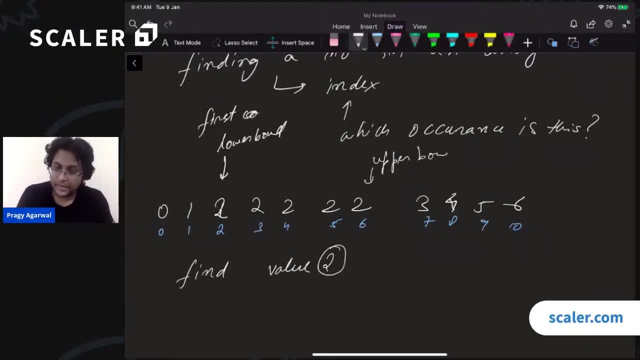 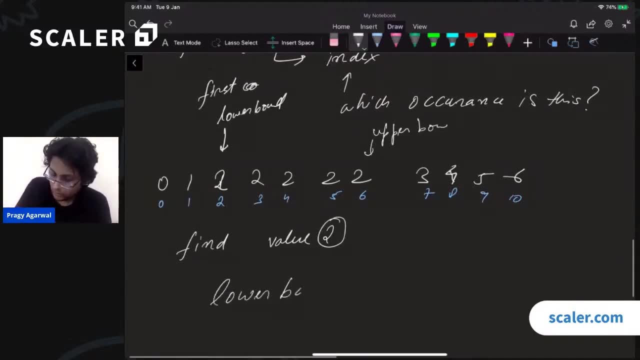 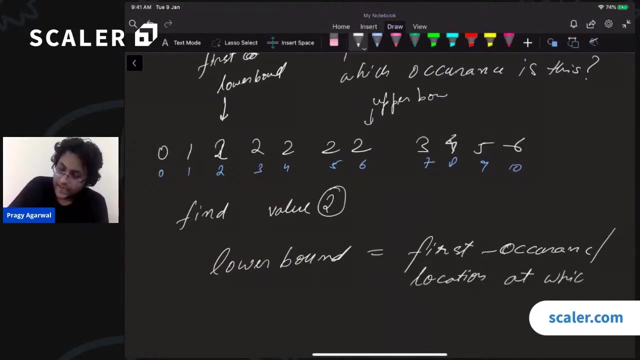 Upper bound right, which is the last occurrence. Does that make sense? Yes, what? what if the array is not present? so, lower bound, Lower bound, is the first occurrence, Right, or if the element is not present, it is the. it is the location. It is the location at which I can insert the element. I should insert the element. 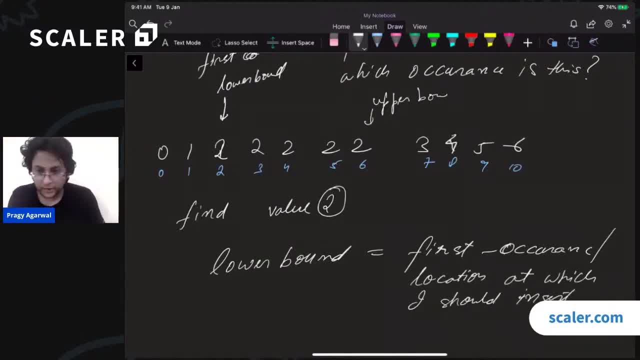 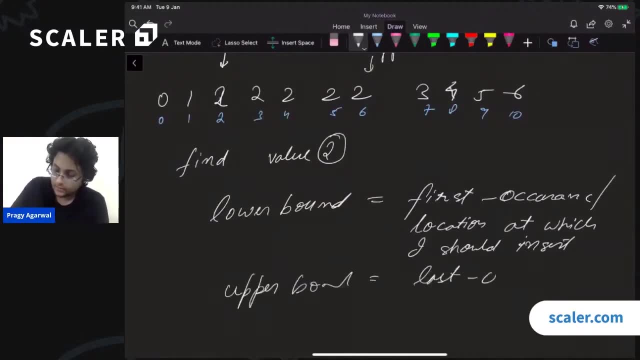 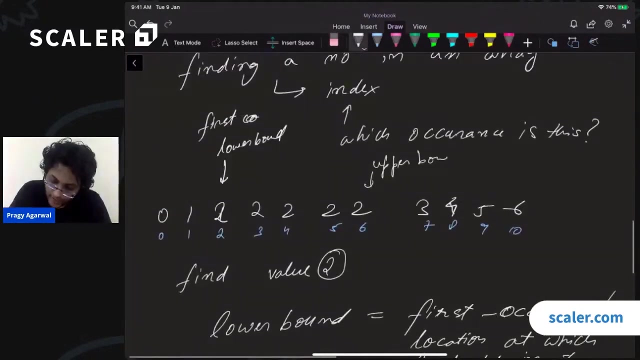 Insert the element to keep the array sorted. Yes, Similarly, the upper bound. Upper bound is the last occurrence, Right? Is that clear? Yes, Yes or no? All right, cool. So basically, the question now is that, if you have been given this, if you have been given an array like this, 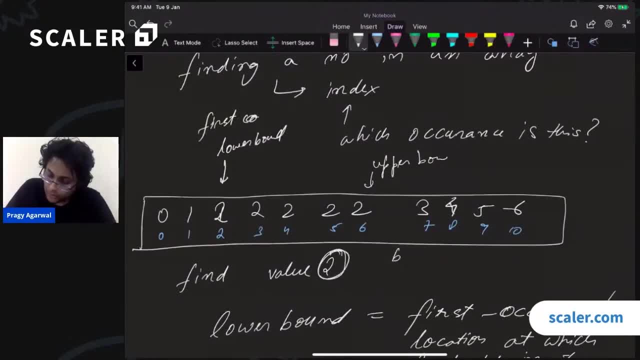 And I ask you that, given a value, you have to return both the first occurrence And the last occurrence of this element. then how will you do that? Right? how will you do that? What if lower bound equals to equals to upper bound? Well, that simply means that simply means that the 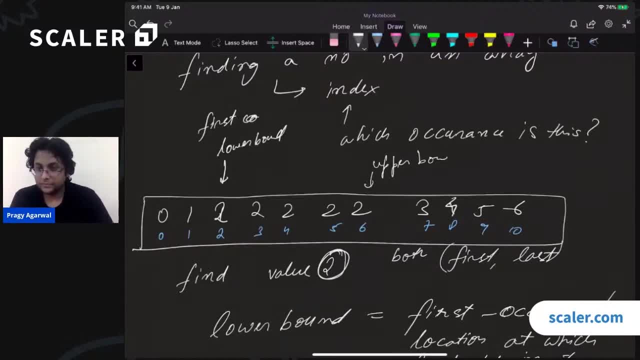 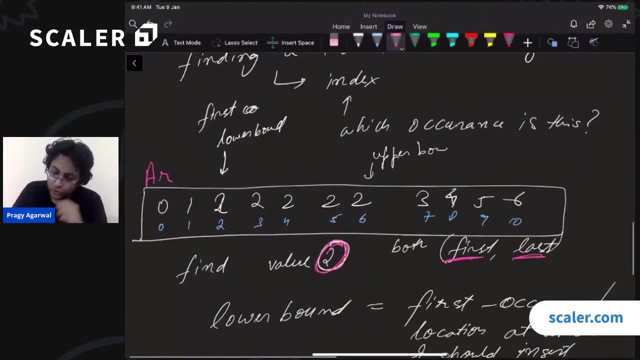 element occurs only once. Right, Trishma? that simply means that the element occurs only once. So suppose that the question is that, given this array, Given this array and this value 2, you have to find both the first occurrence and the last occurrence of this array. So basically, if I give you 2, you have to return 2 and you have to return 6. 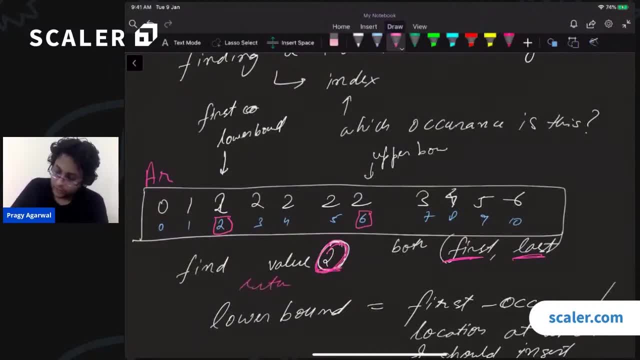 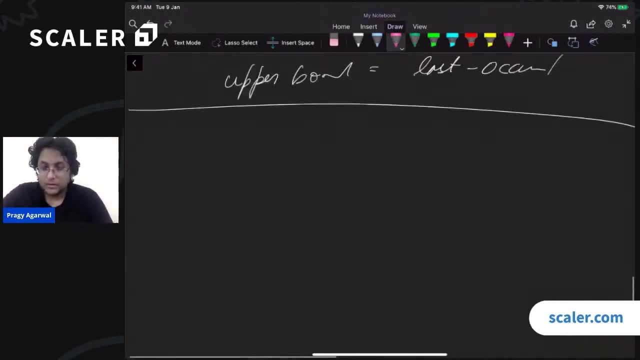 So if the input is this array and 2, you have to return 2 comma 6, Right? so how will we do that? Yes, Yes, so this is very simple, right, This is very simple. We just have to make sure that we tweak a little bit of those minus ones and plus ones. 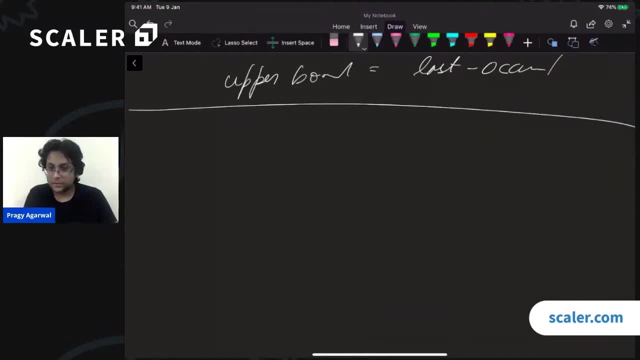 We just have to make sure that you tweak a little bit on those minus ones and plus ones. Okay, so usually what we do is we write the loop like this: So while low is less than equal to hi, Right. and then what do we do? We say if 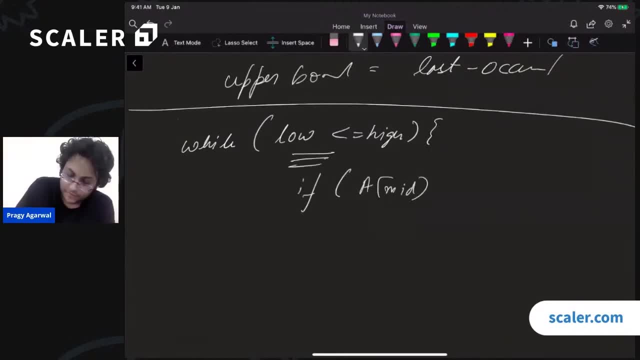 array of mid. So we have mid calculation over here. We have something over here. you say, if If array of mid is less than key, if array of mid is less than key, then what do we do? We do lower bound, we do low equals to mid plus 1, we do low equals to mid plus 1, otherwise. 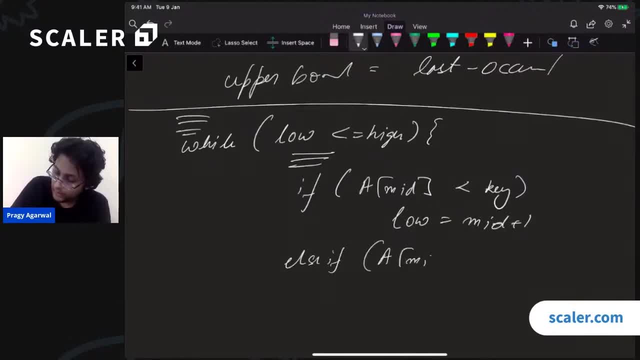 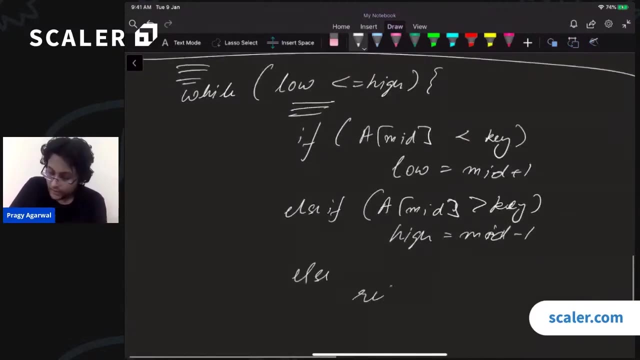 if a of mid is greater than key, then we do. high equals to mid minus 1, mid minus 1, otherwise, if it is exactly equal. in the last class we saw that we can just return the mid. we can just return the mid because we have found the location, but now we can't just return. 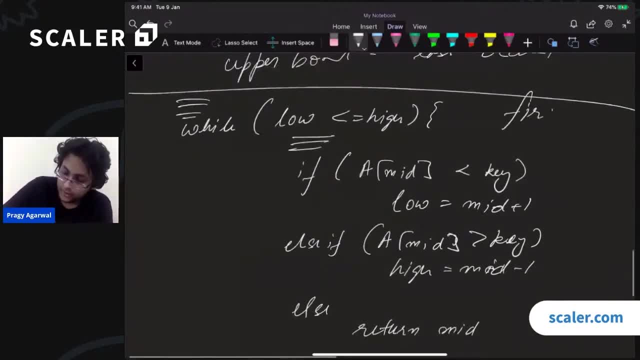 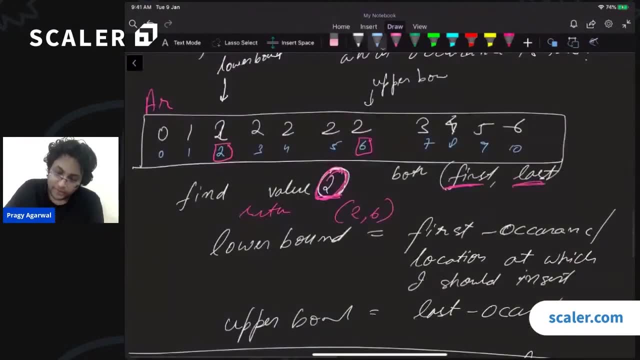 the mid. now, if we are looking for the first occurrence, suppose, if we are looking for the first occurrence, can we return the mid arbitrarily? No, because what could happen is, when we calculated the mid, suppose we landed at this particular location, we found the 2, but we cannot return it because this is not the first. 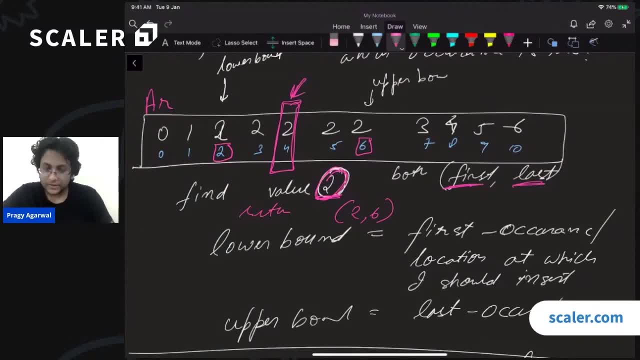 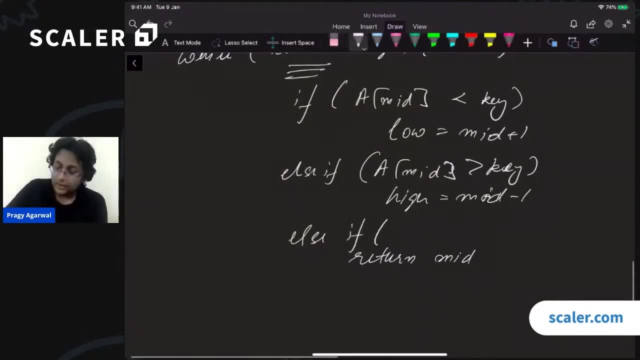 occurrence. this is not the first occurrence, so how do I ensure that this is the first occurrence? I will have to check over here that first of all. that first of all else, if mid should be greater than should either be 0, if the mid is equal to 0, then it is my first occurrence. 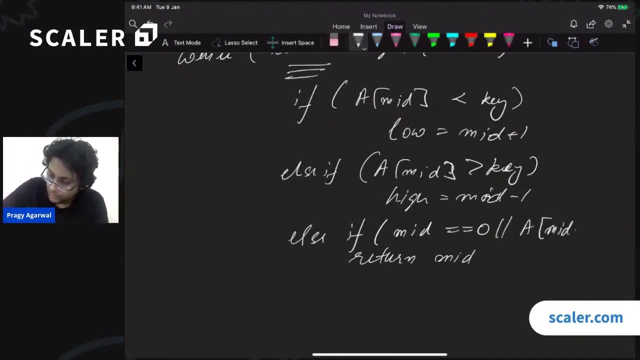 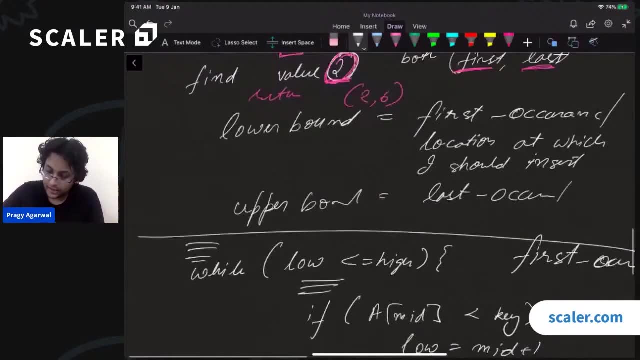 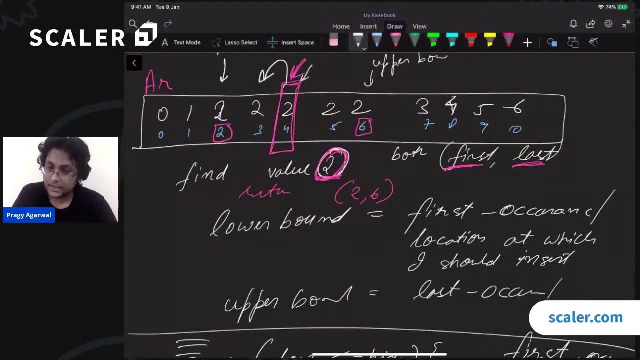 or a of mid minus 1, minus 1 should not be equal to a of mid. should not be equal to a of mid, because if the previous element is equal to the same element, then this mid is not the first occurrence. does that make sense? yes or no? alright, that is fair enough. 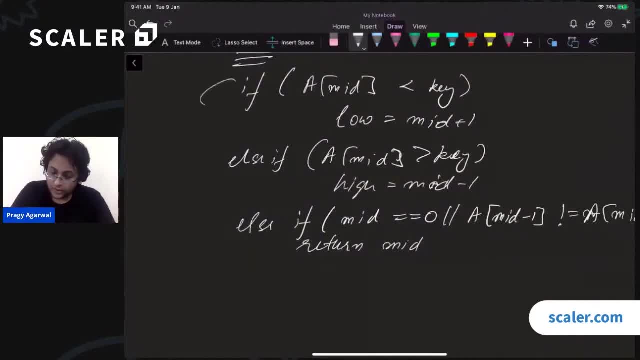 but then what does really happen then? if I write this code, there is a condition remaining, right, There is some condition remaining over here. yes, there is some else condition remaining over here, right? So what do I really do in that else condition? 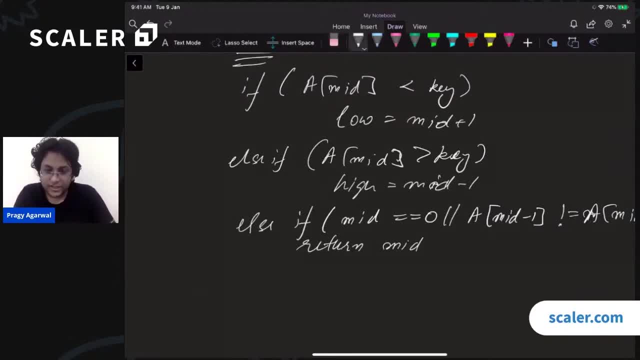 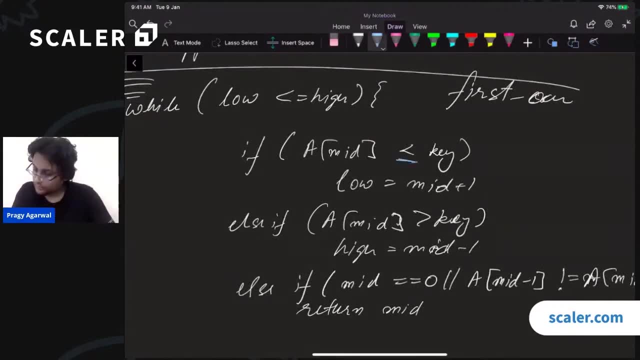 Well, I have to absorb that else condition. it will have to absorb that else condition somehow. so, basically, what I need to do is I need to make this thing. I need to make this thing less than or equal to key. oh sorry, I have to make this thing. I have to make. 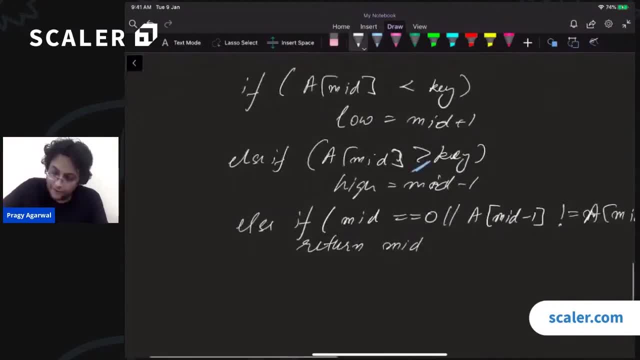 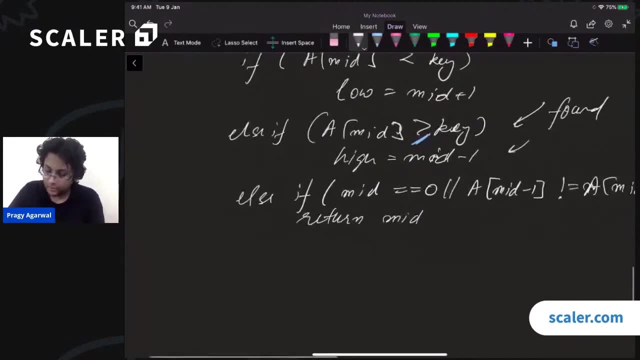 this thing greater than or equal to key right. Basically, if I have found, if I have found the element, but it is not the first occurrence, then I will still decrease my height, right, Suppose I found the element. I found the element over here, but it is not the first occurrence. 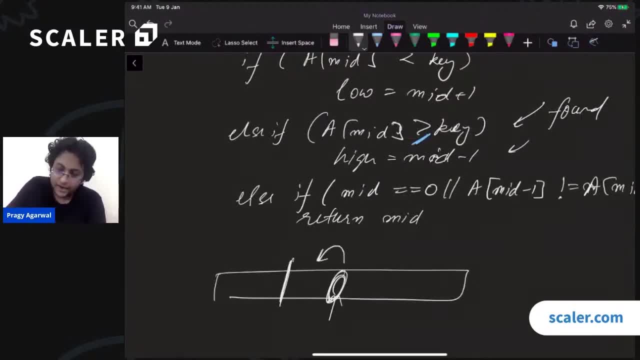 the first occurrence occurs over here. then what should I do? I should move left, I should decrease my height, is that clear? But once again, the moment I do this, something else happens. right Another issue arises. what is that issue? 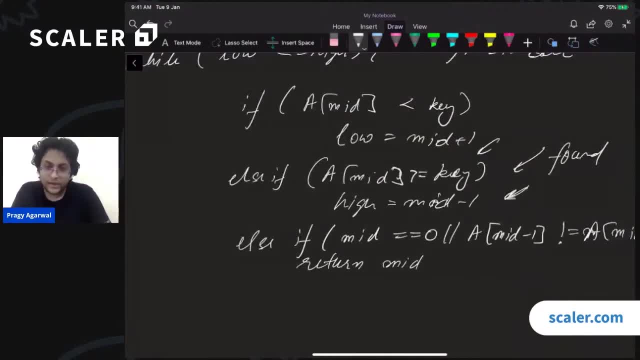 That issue is that if I have this condition in my else, if I will never come into the else, right, I will never come into the else. so what I will have to do is I will have to move this particular condition on the top. yes, do you guys agree? do you guys see the problem? 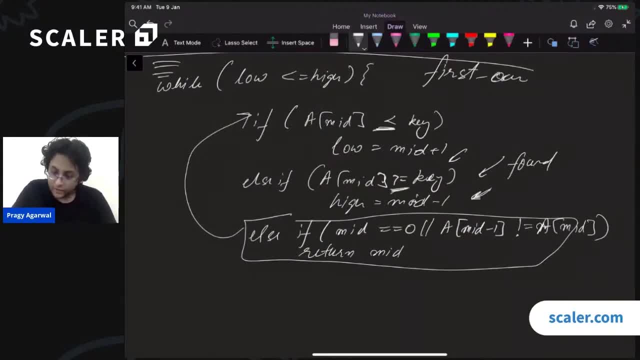 Because if I have less than here and if I have greater than or equal to here, then I will never go into that else. condition right, These conditions are exhaustive. yes, so I will have to move this up. So what will my actual code look like now? 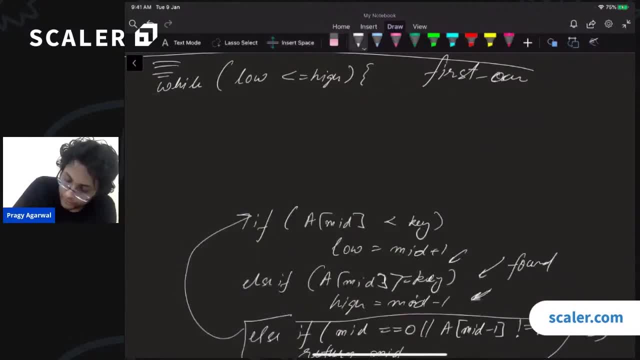 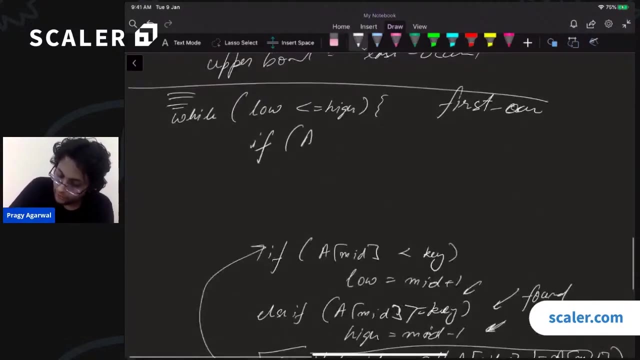 What will the correct code look like now For finding the first occurrence? what I have to do is I have to check first: if mid is zero, right. If mid is zero, sorry. if. if, if A of mid equals to equals to key, right. 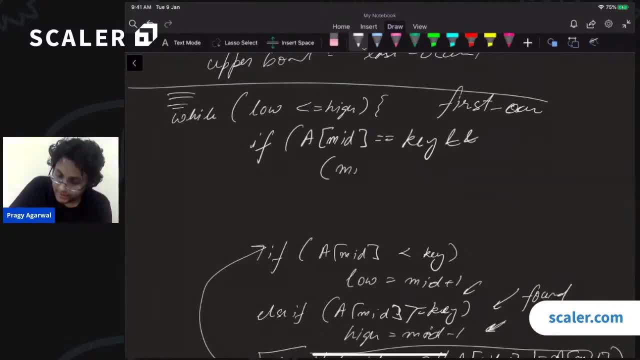 If I have found the value and either mid is zero or A of mid minus one is not equal to A of mid right, only then, if I have found the element- and it is the first occurrence- only then can I reduce it. 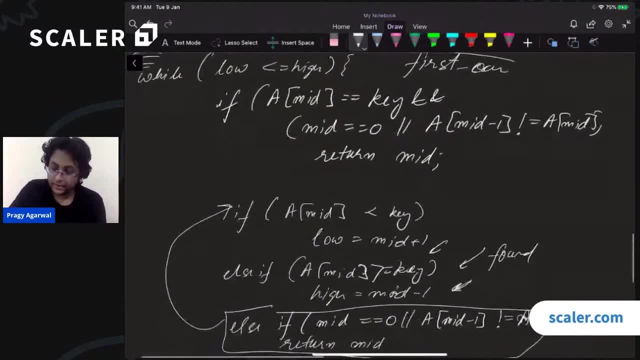 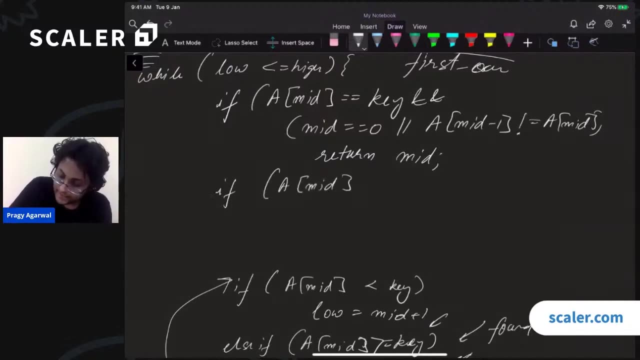 Only then can I return the mid right, Only then can I return the mid Otherwise. so let me just put it over here. otherwise, if A of mid is less than the key, then I have to move up right, So I can say: low equals to mid plus one right. otherwise else I can simply say: 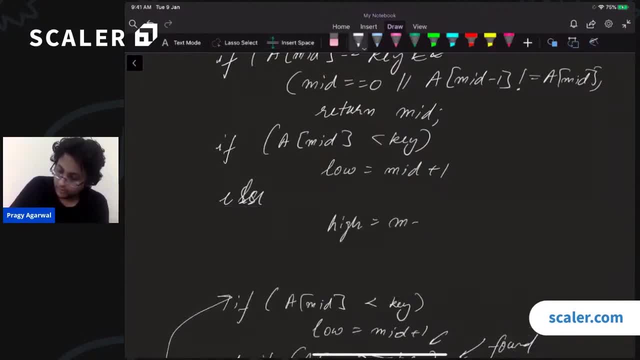 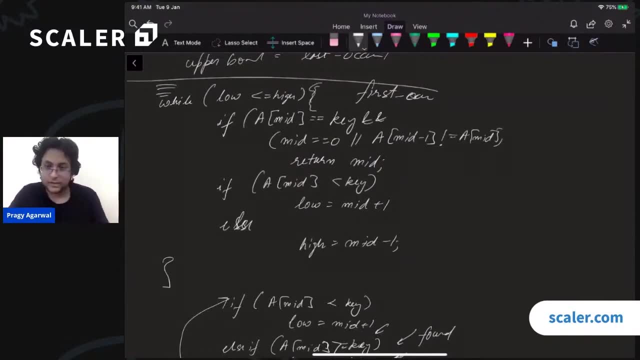 High equals to Mid minus Right, and this is what my correct code looks like now. This is what my correct while loop looks like now, And this is for the first occurrence, Right, this is for the first occurrence, So this code is incorrect. This code is incorrect. 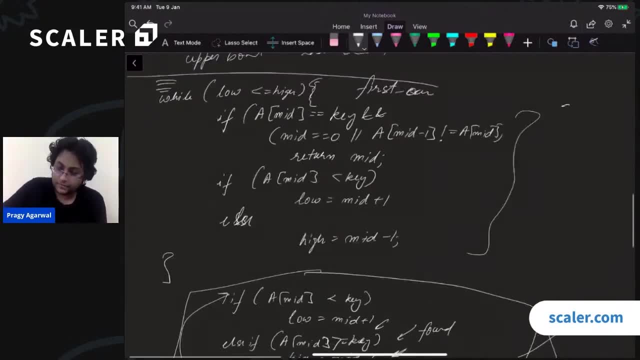 Right, and this is the final correct code for the first occurrence Of occurrence. Can you similarly do? can you similarly find the last occurrence? Can you similarly find the last occurrence? Can you similarly find the last occurrence, Yes or no? Yes, you just have to do it the other way around. you just have to do it the other way around. 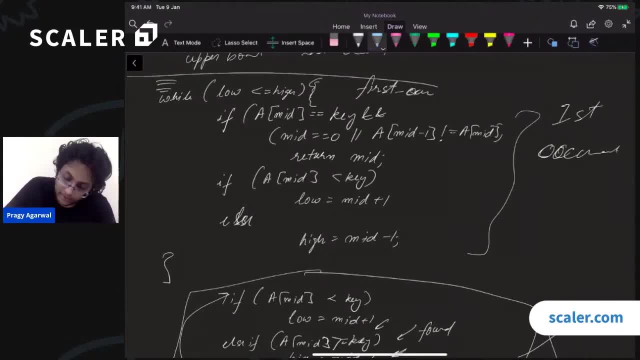 basically, you have to make sure that A of mid equals to key and mid is equal to. Either mid is equal to n minus 1 or A of mid plus 1 is not equal to A of mid. Right, that way we find the last occurrence. and when we are finding the last occurrence? 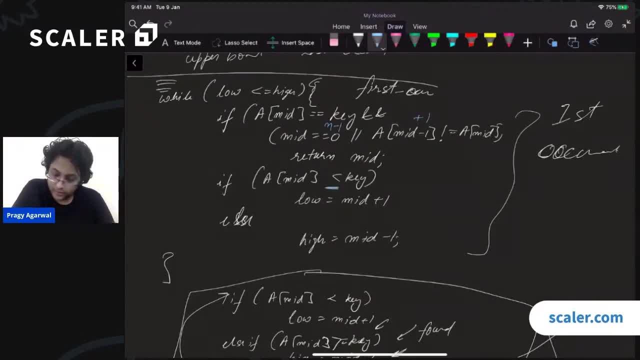 This will be less than equal to and this will not be. this will be less than equal to right. This will come in less than equal to over here. So that is very simple. It is very simple to find the first and last occurrence of an element in an array. 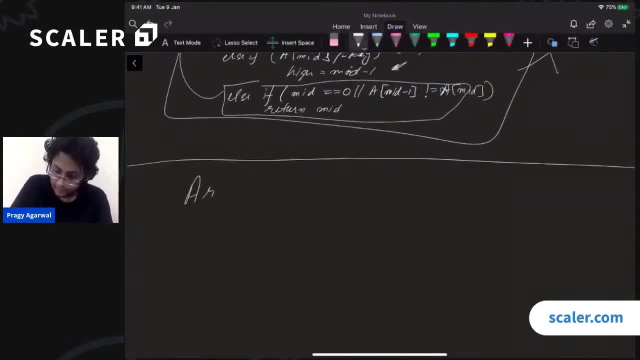 All right. Now suppose that I have an array which is sorted and has size n, has Size n and I tell you that, given a value X, given a value X, you have to count the number of occurrences, occurrences of X, in this array. then what will we do? 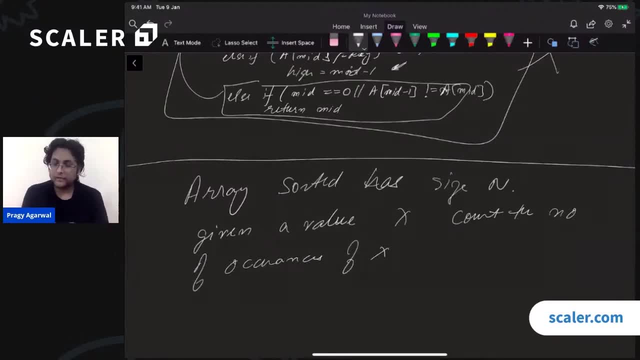 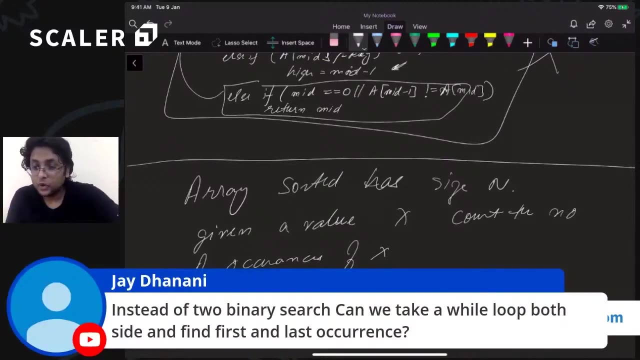 If we have to count the number of occurrences in this array, then what will we do? Yes, JSA is. instead of two binary searches, Can we take a value Both side and find first and last occurrence? Yes, totally, Jai, We can totally do that. 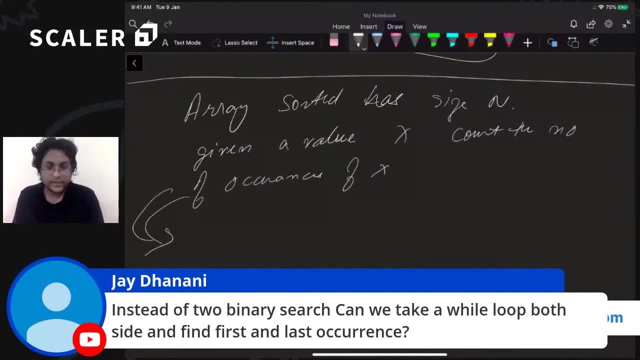 So let us, let us, we are going to explore that and via this question, We are going to explore that via this question. Suppose that we have this array. It suppose that we have this array. This element is X, X, X, X, and all the way till this location, It's X. 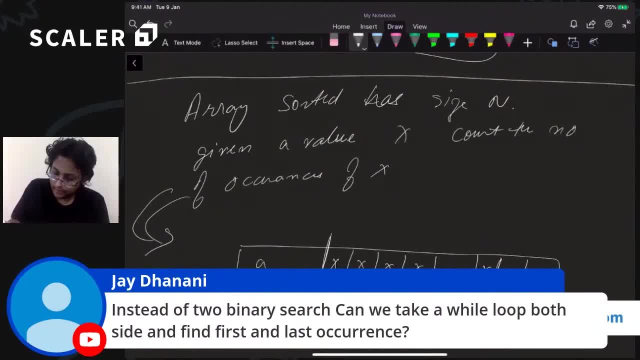 Then this is something else. This is Y, Y, This is AA. so if I am supposed to find the count of X's, If this is a sorted array, If I am supposed to find the count of X's, then I have two options. either I can find the first occurrence, 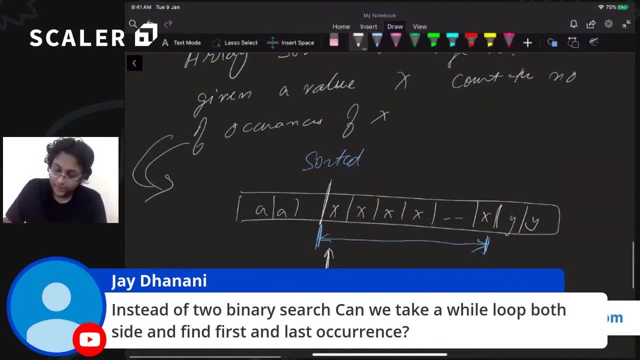 Either I can find the first occurrence, then write off value, then write a for loop Right till the last location of X, Yes or no. I can find the first occurrence and then I can increment the count one by one. I can. I can go one by one and till till I reach the last occurrence of X and I can do a count plus plus. 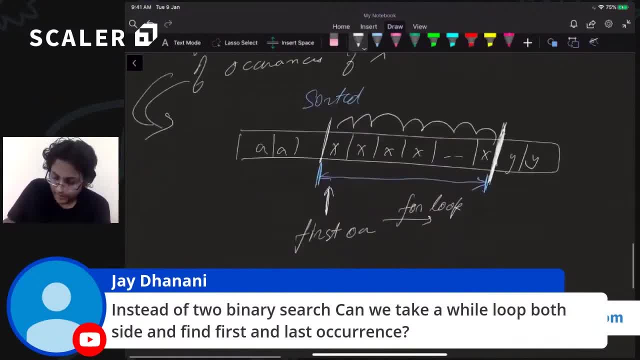 I can do a count plus plus. If I do it this way, then what will be the time complexity? What will be the time complexity of this way, When to find the first occurrence? it will take me order of log n time. but after that, after that count each of these values, I will have to count one by one, again and again. 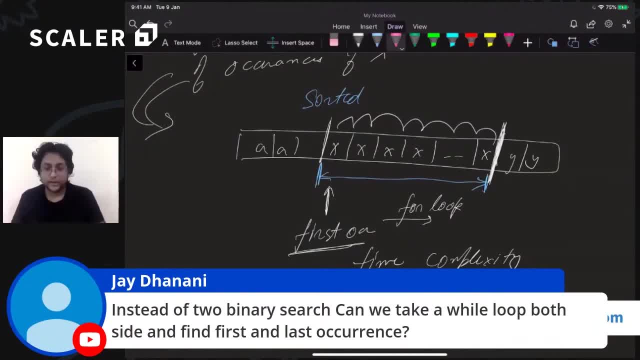 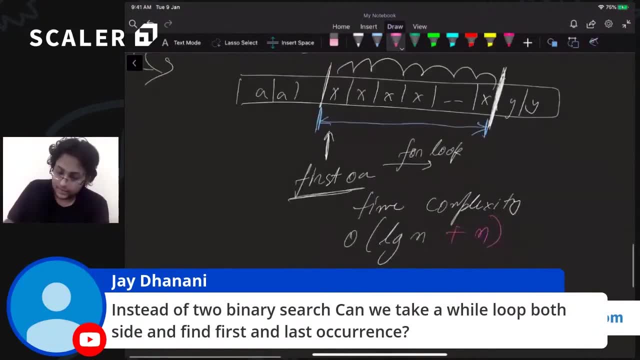 One by one, again and again. so it will take me order of n time for the counting. in the worst case, What if the entire array was full of the same values? Does that make sense? So in this case, this approach will be linear. this approach will be linear. 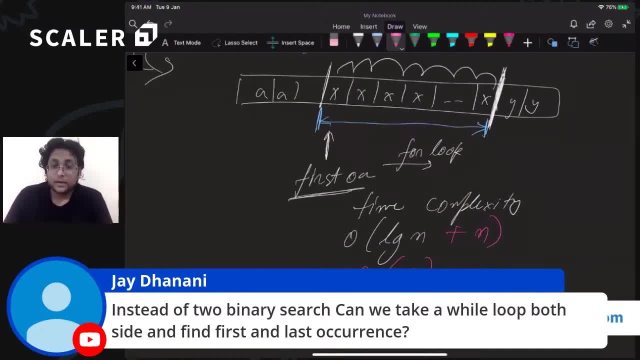 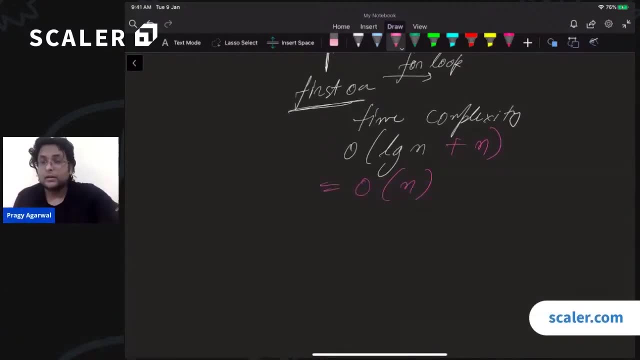 On the other hand, can I do something better? Can I do something better? Let me just clear the banner, just give me a second. yes, can we do something better? Right, So we can. what we can do is we can simply find the last occurrence, we can simply run. 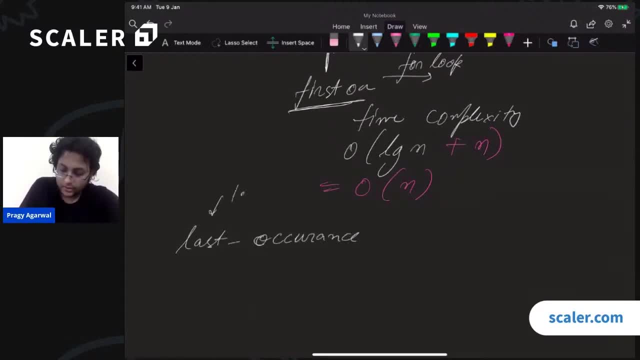 a binary search to find the last occurrence right. This is one binary search, binary search, and we can also use another binary search, one more binary search right to find the first occurrence right And then we can simply return. we can simply return last occurrence minus the first occurrence. 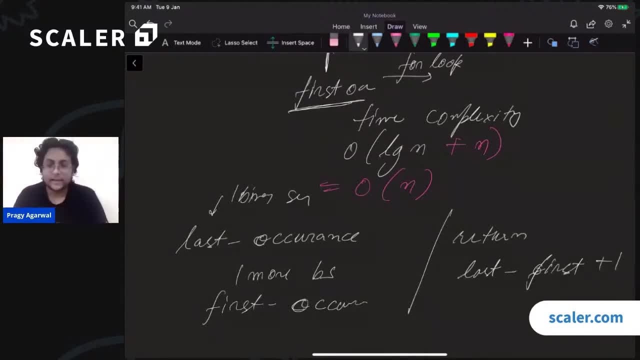 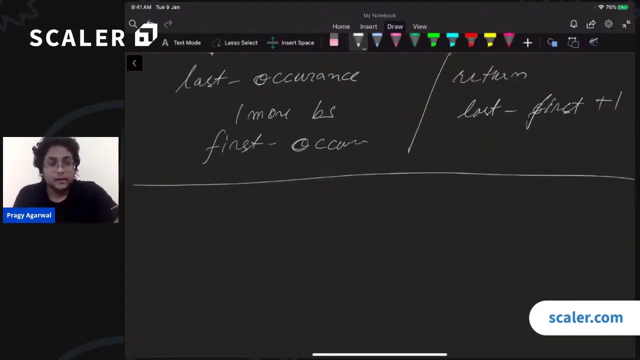 Yes, is that correct? Plus one, exactly right. last occurrence minus first occurrence, plus one right, And that will basically give us the count of that element. is that clear? Yes, all right, perfect, cool. So I hope this is clear because this is very important. first of all, because I mean whenever 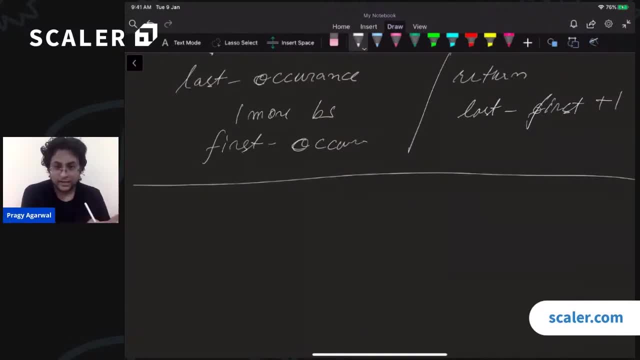 you do binary search, you have to understand that you are either going to be finding the last occurrence or the first occurrence. you are not going to be returning any arbitrary occurrence. Also, because in all of the further questions, in all of whenever you are doing binary search, 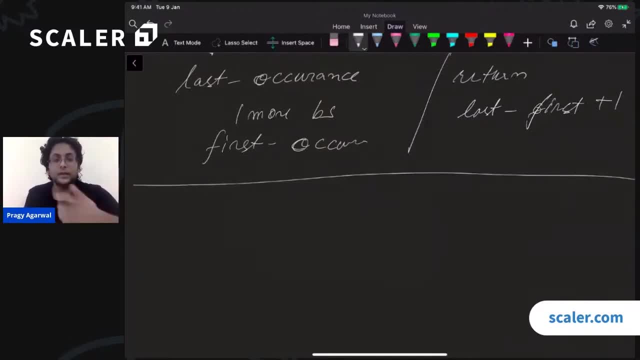 this is going to be very important for us. it is going to be very important for us, So let us look at another question. let us look at another question. So suppose that we have been given two sorted arrays. right, This is a very, very famous question. I mean, this question has been asked in all sorts. 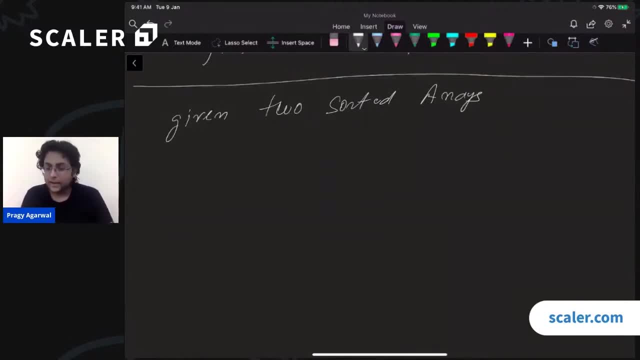 of companies, right, Be it Google, be it Amazon, be it Facebook, be it direct type, all the companies have at some point asked these questions. This particular question and this question is very, very, very frequent, right, And even if you, even if you try to search on YouTube, you will find hundreds of videos. 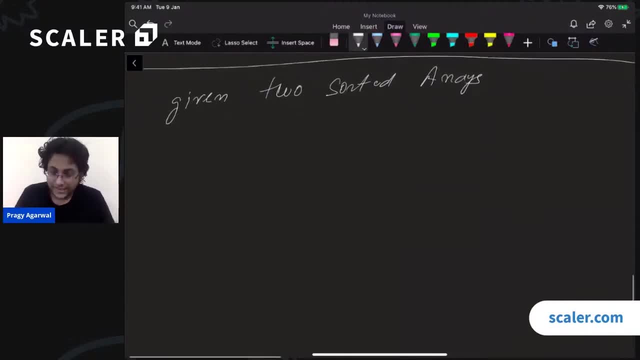 about this question. So this question is very important. The question is that you have been given two sorted arrays of length: length n and m respectively, right, Right. So you have been given two sorted arrays. one is of length n, one might be of length. 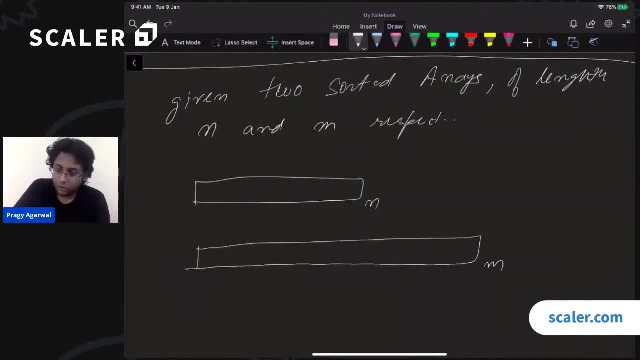 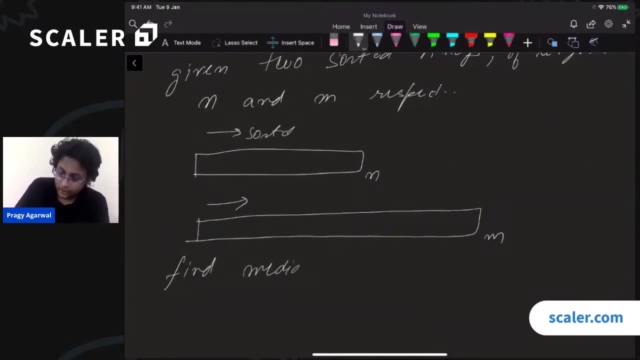 m. We don't really know which is larger, which is smaller, And both are sorted. Both are sorted. The question is, we have to find the median of both the arrays. both the arrays combined Combined, We have to find the overall median. 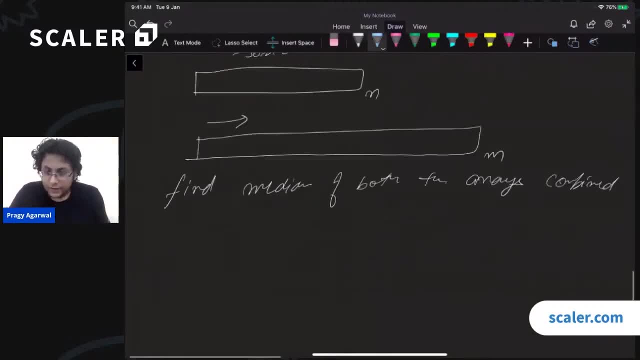 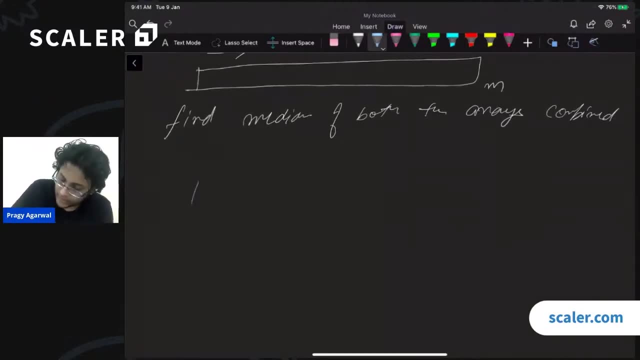 Yes, Right. So first of all, let us look at what median is. First of all, let us quickly look at what the median is. So suppose that I give you this particular thing. Suppose that I give you this array: 1, 2,, 2, 3,, 5,, 5,, 6,, 8,, 10, right? 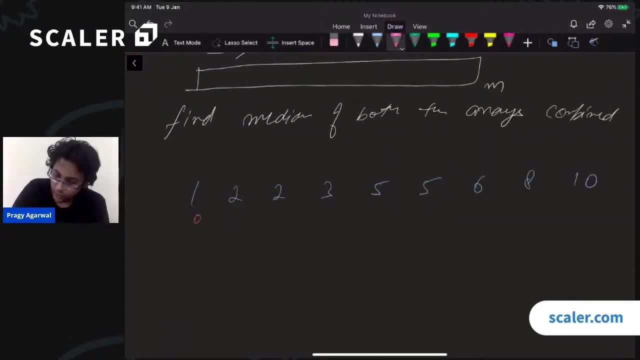 Suppose that this is my array, And let me put the indices as well. right, So 0, 1,, 2,, 3,, 4,, 5,, 6,, 7,, 8, right, So what is the median defined as? 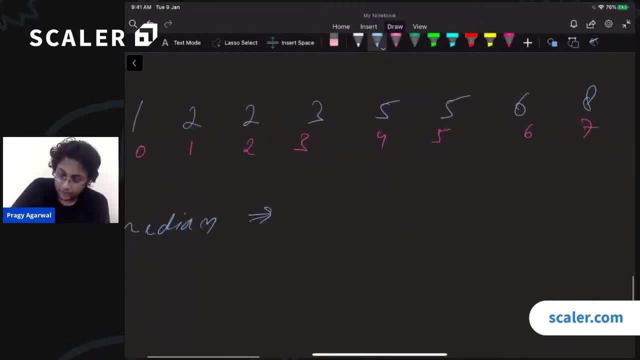 What really is the median? So median, basically, is another term for the middle element Right. This is a loose definition. This is not the exact definition, But median. you can think of median as the middle element Right Of a particular, of a particular collection. 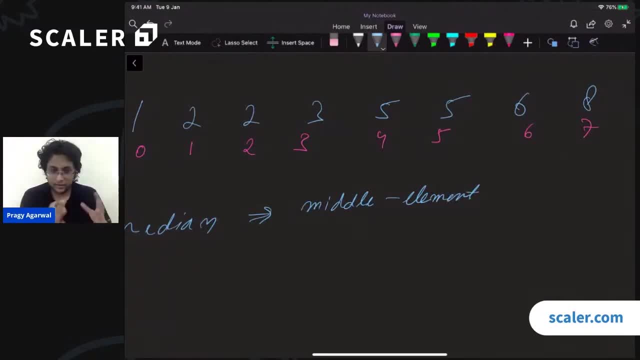 Now, what do you mean by middle element? If you are talking about the middle element, we should have some sort of order. We should have some sort of ordering. Yes, So that is why we are talking about a sorted array. So we are saying, if we sort a particular array, 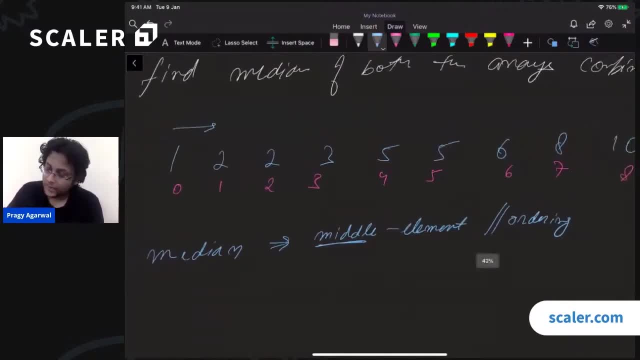 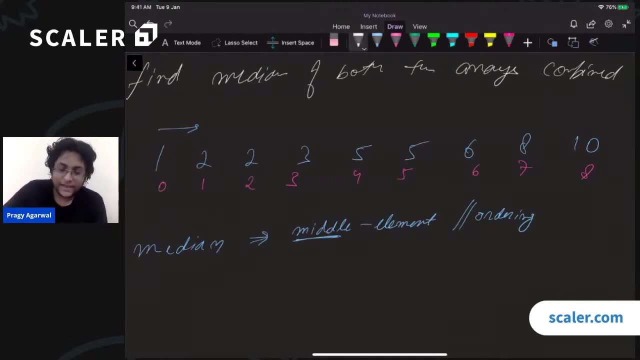 And then we look at the middle element, And then we look at the middle element. So, in this case, do I have a middle element? In this case do I have a middle element? How many elements do I have middle element? how many elements do i have? i have nine elements in total. right, i have nine elements. 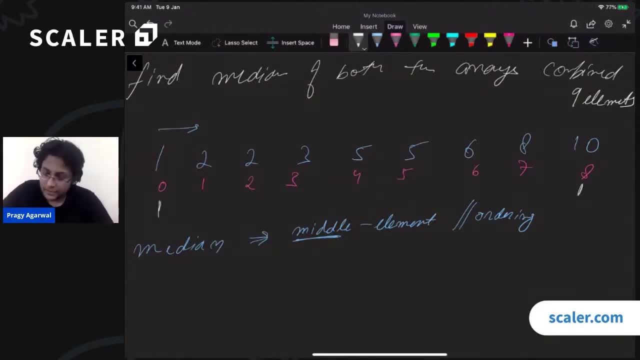 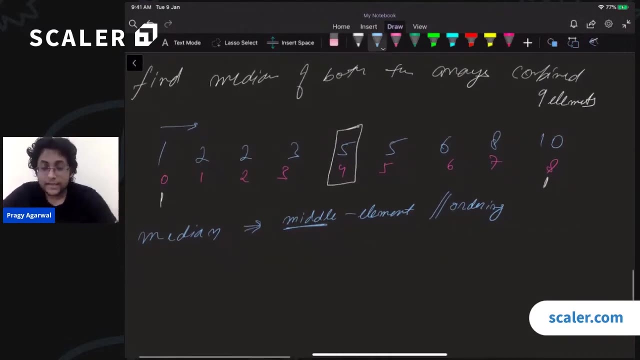 in total, from zero all the way to eight. so what will be my middle element? this will be my middle element. yes, this will be my middle element. okay, so basically, this is what a median is. now some of you might ask: all right, well, what if the number of elements is even? what if the number of elements 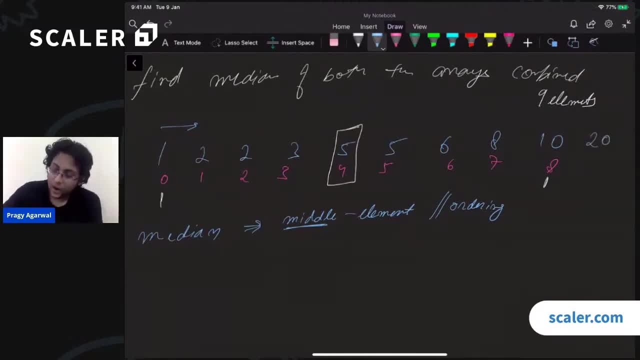 is even so, let us say that i add up 20 over here. right now. i have 10 elements. now i have 10 elements, right. this is no longer nine, this is 10 elements. now there is there is no middle element, right. the middle element does not exist. now there are two middle elements. both this and this are middle. 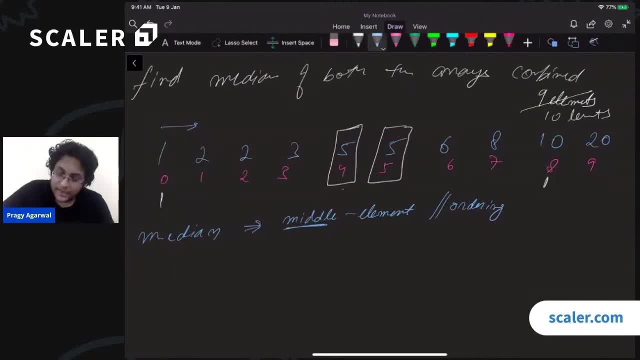 elements. yes, then, what is the medium? well, in that case, median is the average average of both of these. so, in this case, this is both five and five, so the median is just five. on the other hand, let us let us try to change the values. so let us say: this is, this is nine, this is nine, and let us say this was. 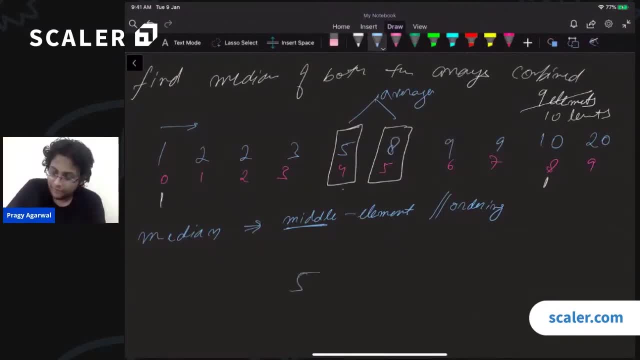 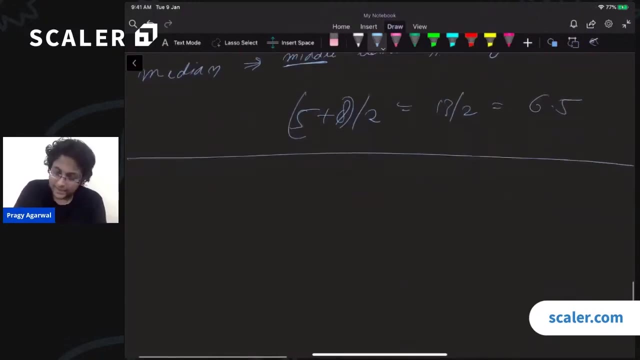 eight. if this was eight, then what will the median be? it will be five plus eight by two, which is 13 by two, which is six point five. all right, is that clear, cool? so this is what the median is. now the question says that you have two arrows. you have two. 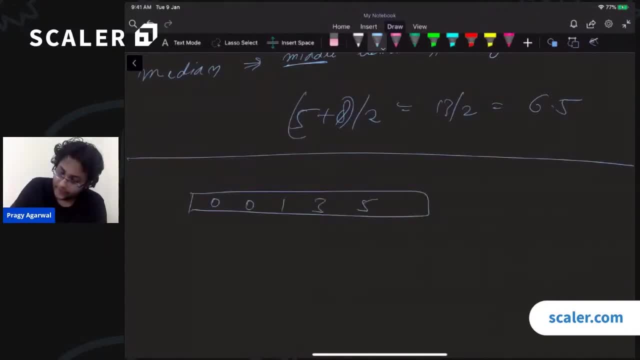 arrows. let us suppose zero, zero, one, three, five, eight, And you have another array. Let us suppose 4, 5,, 6,, 7,, 8,, 9,, 20,, 30.. Let us suppose that we have these two arrays. So let me put the indices very quickly: 0,, 1,, 2, 3,, 4,, 5, 0,. 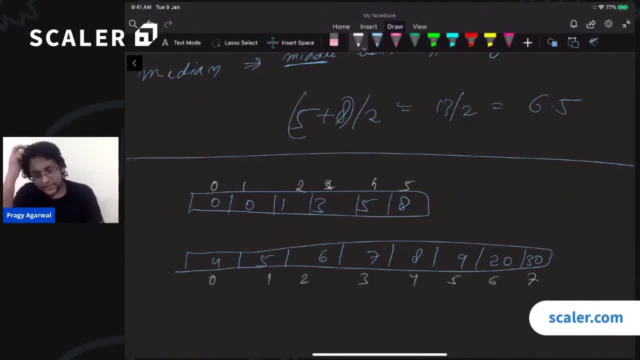 1,, 2,, 3,, 4,, 5,, 6, 7.. Now, the question is not asking you to find the median of each of these arrays. That is not what is being asked. What is being asked is the median of the overall. 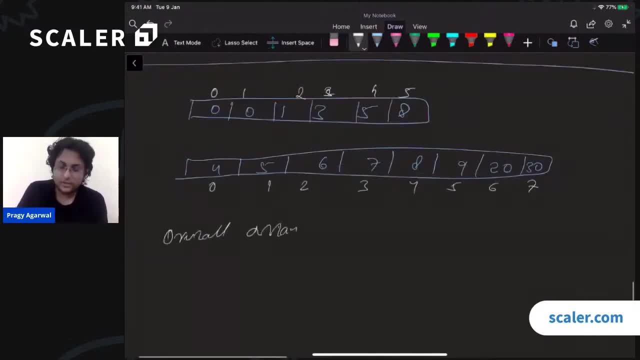 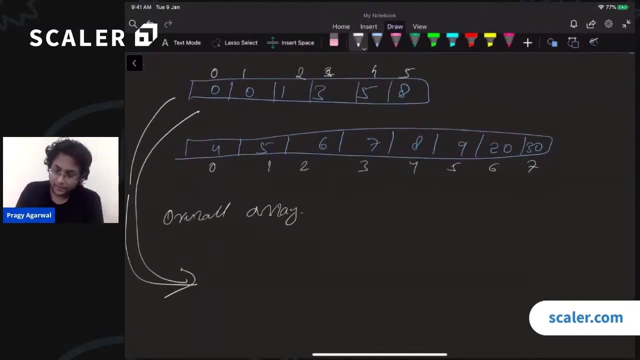 array of the overall collection. So, basically, if I were to take all these elements, consider all these elements and sort them, then what will be the median? So what will be the median in this case? What will be the median in this case If I write both the arrays in sorted? 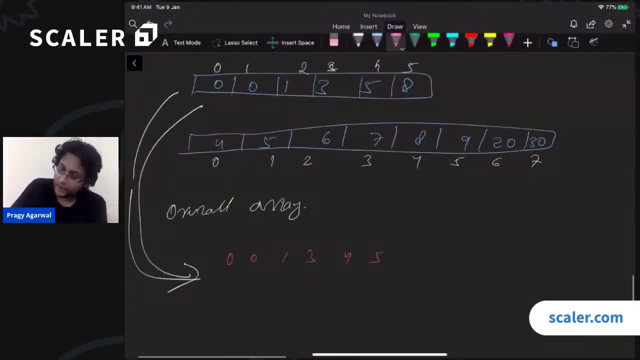 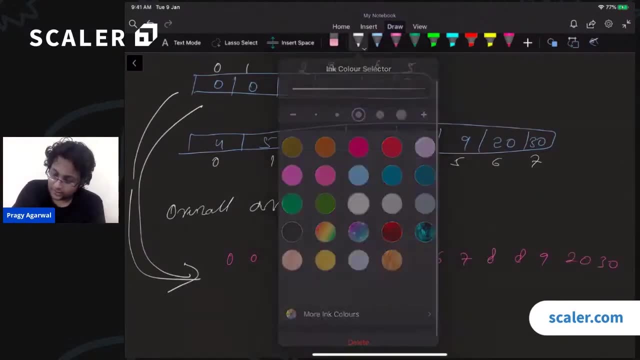 form. I have 0, 0,, 1,, 3,, 4,, 5,, 5,, 6,, 7,, 8,, 8,, 9,, 20,, 30. Right, Yes or no? And this is 0,, 1,, 2,, 3,, 4,, 5,, 6,, 7,, 8,, 9,, 10,, 11,, 12,, 13.. Right, That's. 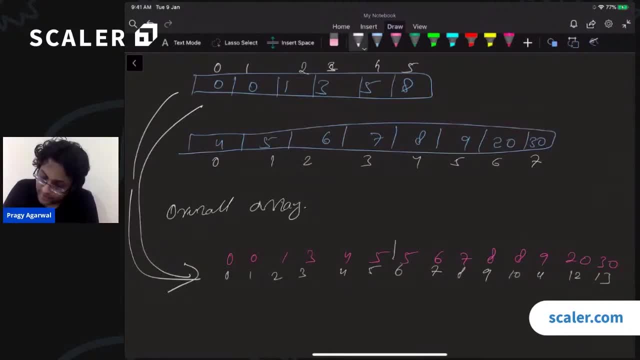 an even number of elements. So the elements what The elements 6 and 7.. So the median will, over here, be: the median will be 5.5.. Is that clear, Yes or no? Is the question clear? We have been given two arrays and we have to find the overall median of the two. 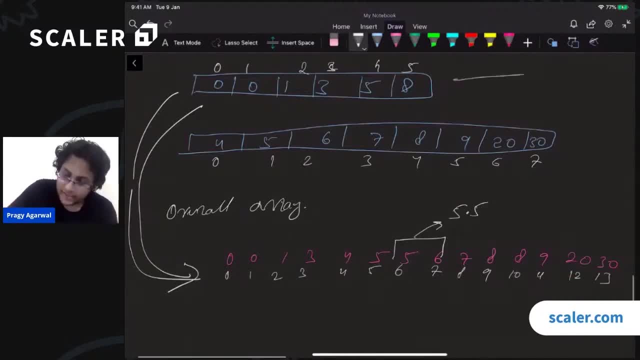 arrays. Is the given array sorted? Yes, Both the arrays are individually sorted in ascending order. Both the arrays are individually sorted in ascending order, But I mean relatively. they are not sorted. So it is totally possible that this element is greater than this element. That's totally fine. Okay, There's no relation. 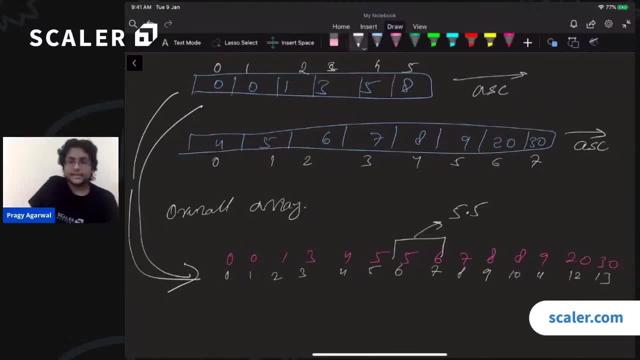 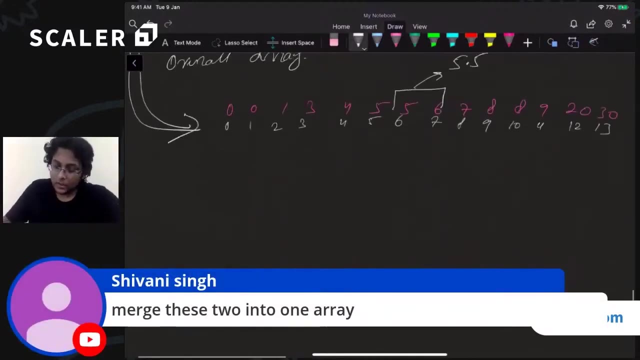 between the two arrays. It is just that they are individually sorted. Yes, So, yes, Shivani has a nice approach over here. Shivani says that let us very quickly merge the two arrays. So where did our comment go? Yes, So Shivani says over here that what we can do is we can. 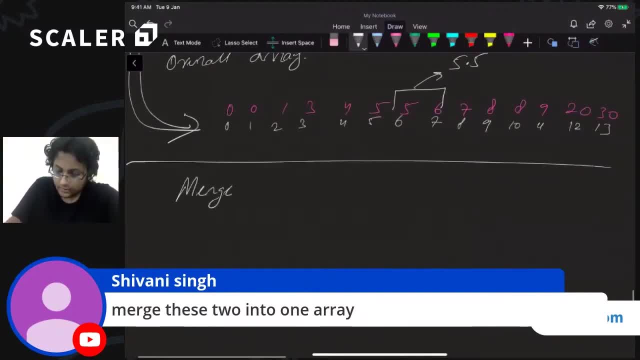 merge the two arrays. So when you are doing the merge sort class, you, you read this merge algorithm, right, Merge algorithm. What does this merge algorithm do? Given two sorted arrays, it created a sorted array. Yes, And how much time did it take? How much time did? 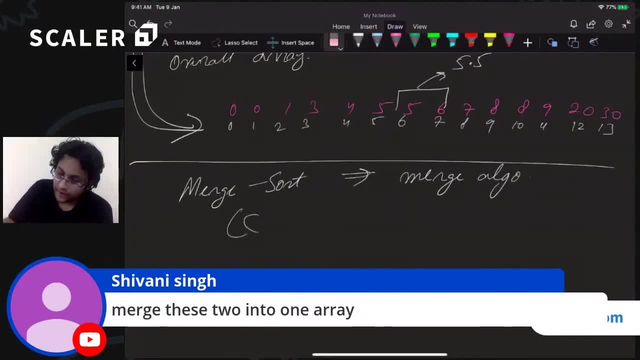 this merge algorithm take. So if, if I have, if I have total of total of total of two arrays, n plus m elements, if I have n plus m elements, then usually if I do, if I, if I just do sorting, if I just do sorting in a naive way, then how much time will sorting? 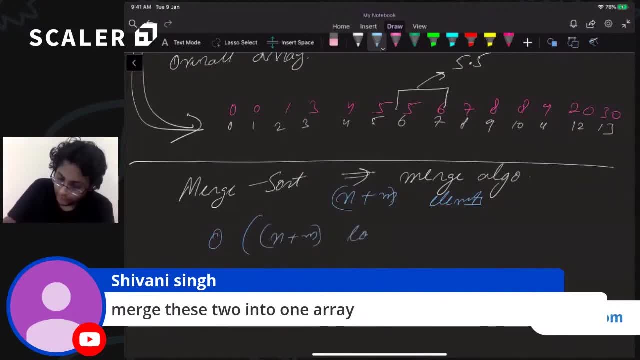 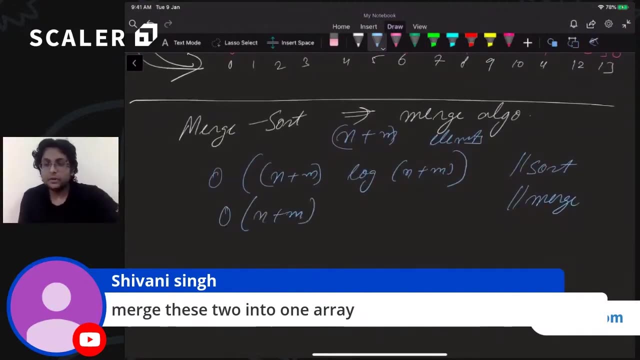 take me. It will take me n plus m. log of n plus m. This is how much time sorting will take me. However, if I use the merge algorithm, given that both the arrays are sorted, then I can do it in order of n plus m time. Yes, I can merge the arrays in order of n plus. 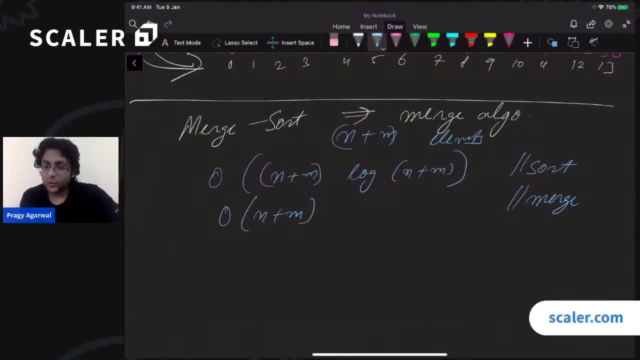 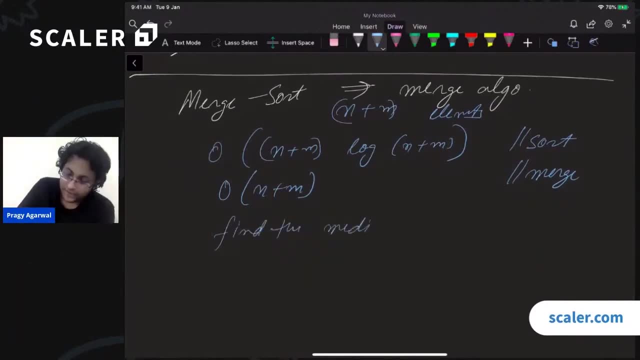 m time. Once I have merged both the arrays, then I can very quickly find the median. Yes, I can very quickly find the median. Find the median. How much time will it take me? If I have merged both these arrays? how much time will it take me to find the median? So suppose, 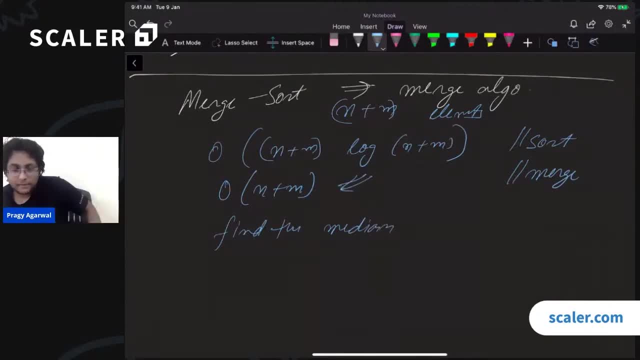 that I have merged both the arrays. After that, how much time is it going to take me to find the median? So is it going to take us order of log n time? No Right. So finding the median, finding a median, is just order of one. You just have to look at A of mid. just have to look at A. 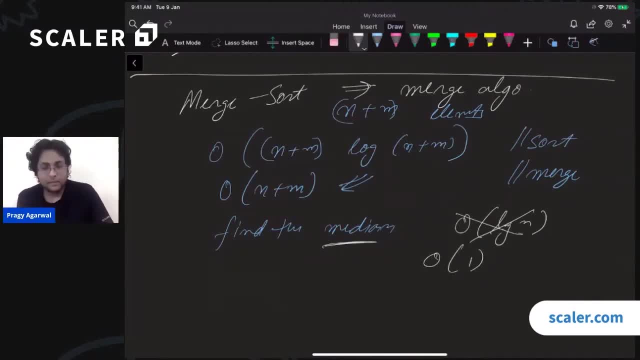 of mid, If the number of elements is even, you just have to get A of mid and A of mid plus one right. So finding the median takes us order of one time, provided that I already have a sorted array Overall, if I do this merge thing. if I do this merge thing, my 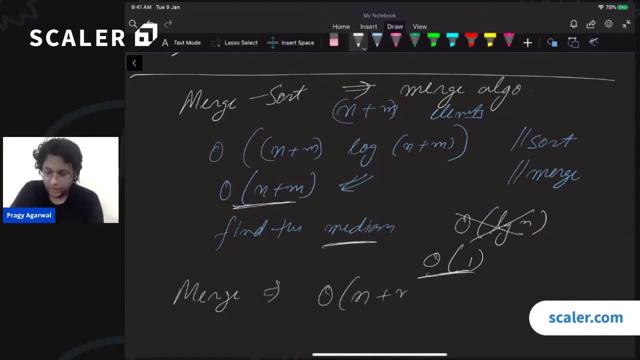 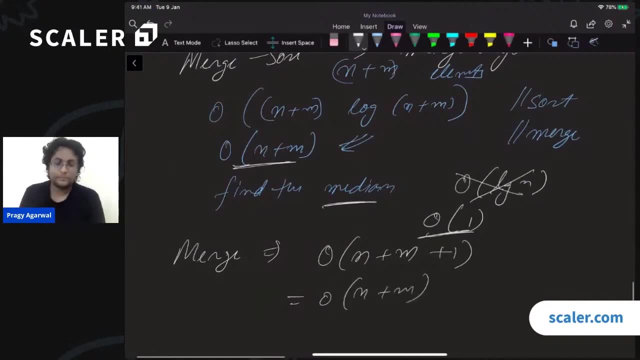 overall complexity will be: order of n. Order of n plus m. to merge all the strings means Merge the two arrays plus one to find the medium. To find the medium, which is just order of n plus m. Is that clear? Order of n plus m. 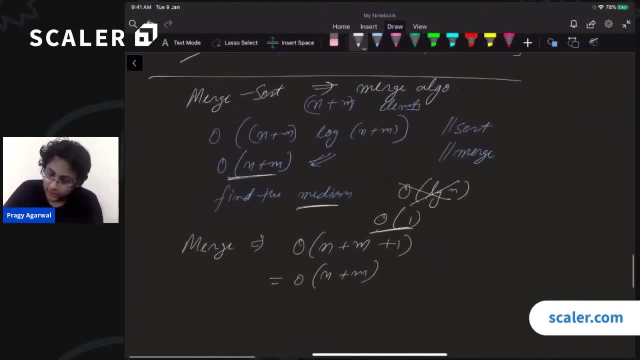 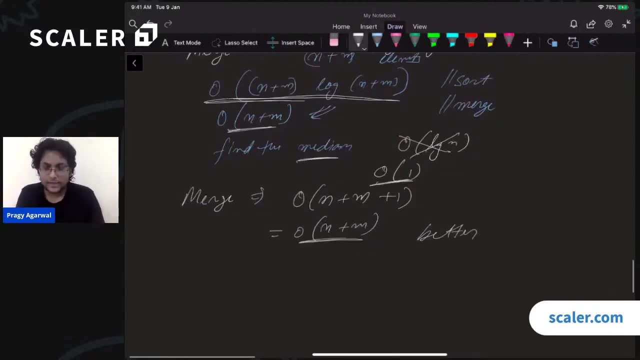 Well, that is fine, that is good. that is certainly better than the naive approach. So this was the naive approach, So this is certainly better, But we can still do better, So this is not the best approach that we can use. 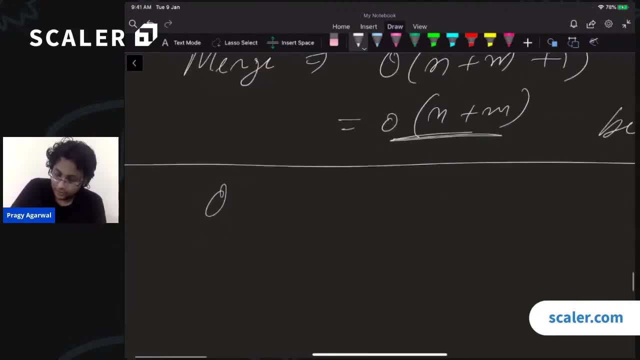 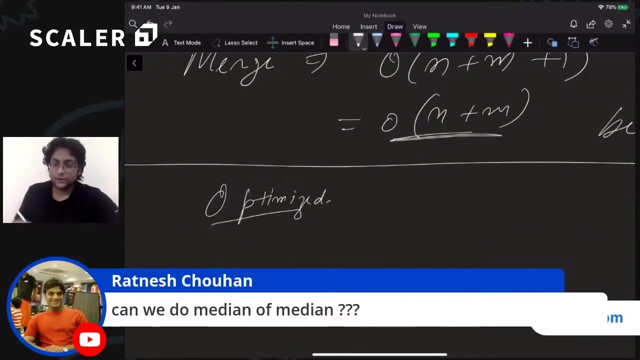 So can we still optimize? Can we come up with an optimized approach now? What other approaches we have? So Ratneesh has a very, very nice question over here. Ratneesh says: can't we just use the median of medians? 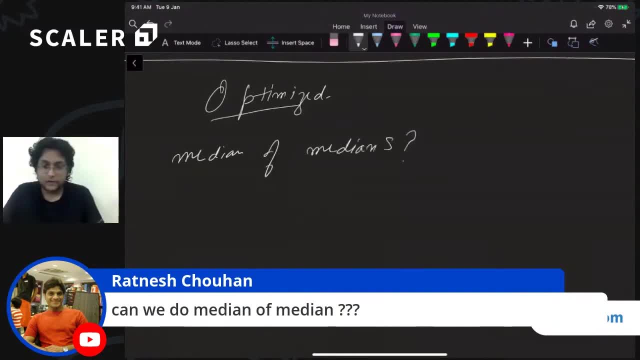 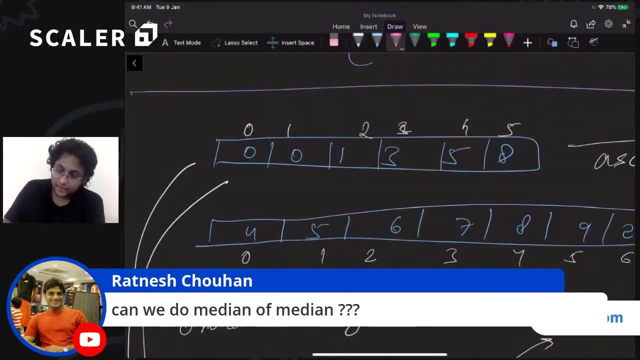 Median of medians, right. What does Ratneesh mean over here? Let us suppose that we consider these two arrays right. Let us consider these two arrays separately. What is the median of the first element or of the first array? 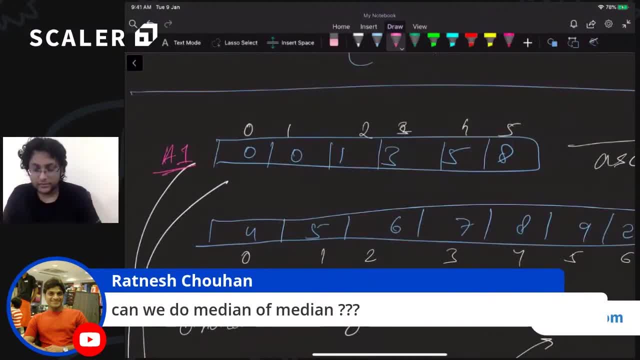 So this is the first array. What is the median of the first array? only? So this array has six elements. So the median will be. The median will be what? So? zero, one, two, three, four, five, right. 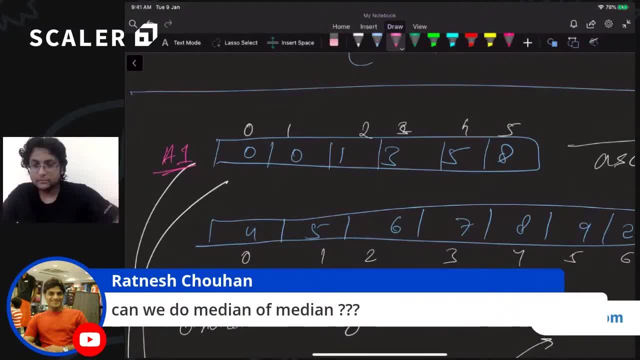 It has six elements. So the median will be at what index? No, no, no. So what Ratneesh is telling us is that let us try to find the median of medians. Let us try to find the median of medians. 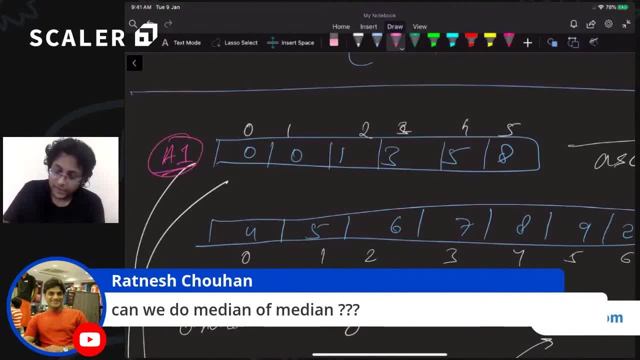 So, first of all, let us consider this particular array A1.. This particular array has how many elements? It has six elements, from this location to this location. So what will be the median of this particular array? It will be the sum of these two. 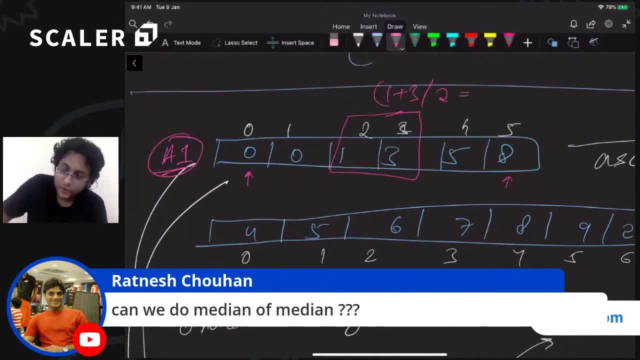 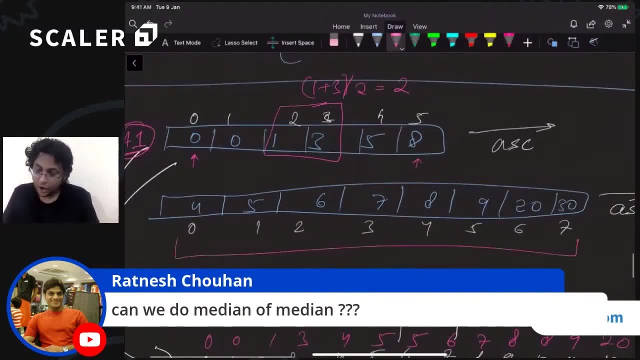 It will be the average of these two, right, It will be one plus three by two, which will just be two, right? Similarly, let us calculate the median of this array. Let us calculate the median of this array. Well, how many elements does this array have? 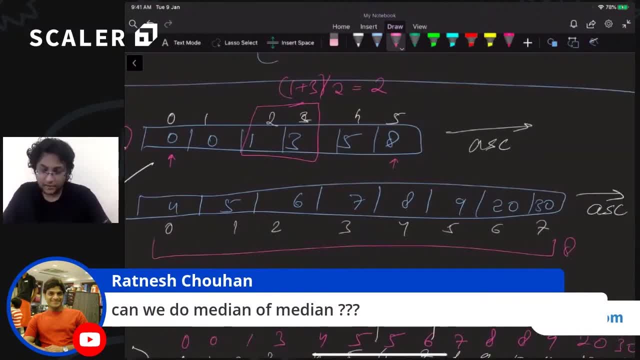 This has eight elements, right? And what is the median of this array, Or this array That will be This: three, This is three plus four, right? This element at three and element at four, So that is seven plus eight by two, which is 7.5, right. 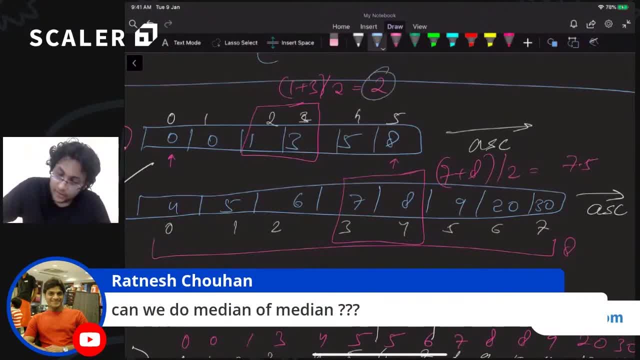 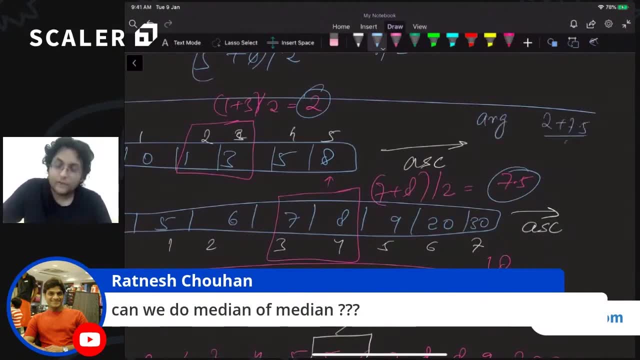 Now Ratneesh is saying: once we have these two medians, can't the final answer simply be the average? Can't the final answer simply be the average of these two, Two plus 7.5 by two? Well, no, that is not going to be always true, right? 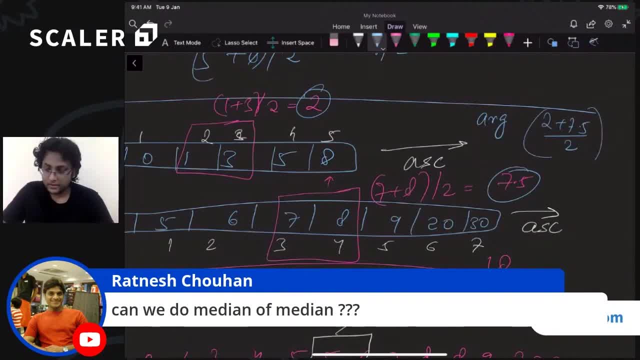 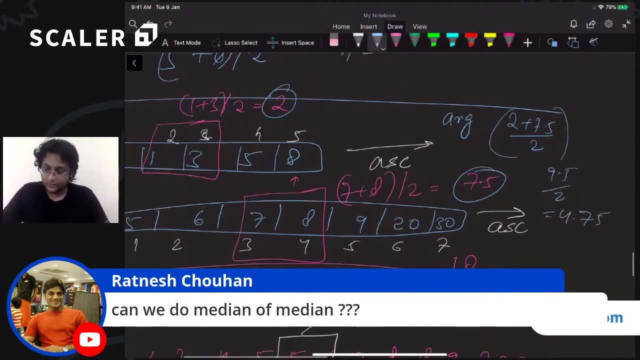 That is not going to always be true. Is that clear, Ratneesh? Over here we see that this does not really work. This is 9.5 by two, Which is 4.75, right, And that is not the answer. 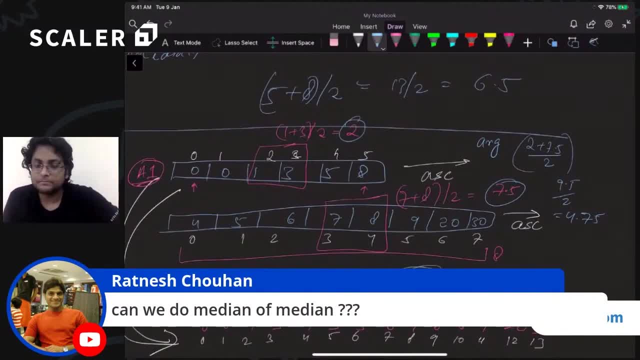 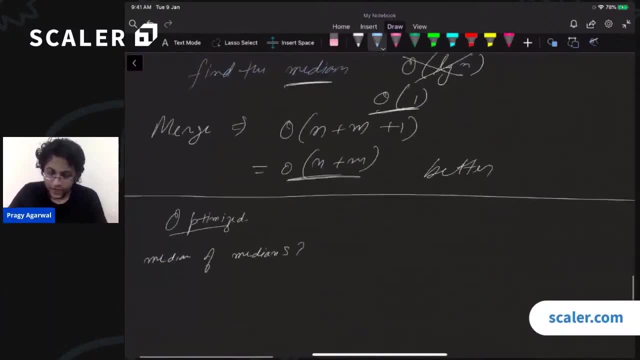 The correct answer is 5.5 over here. So it doesn't really work All right. so let me just remove Ratneesh's comment. So median of medians will not work over here, So we have to do something else. 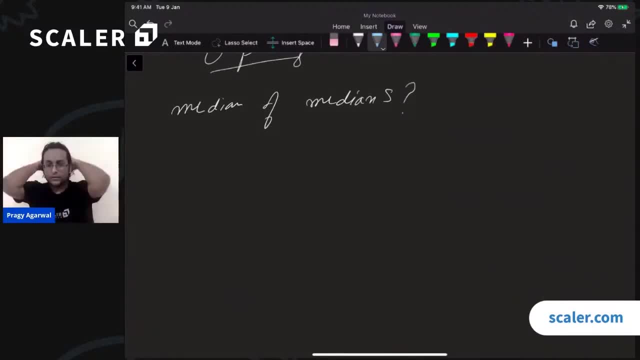 Yes, so what approach can we use? What approach can we use? So now we have to do some sort of a binary search. We can use some sort of a binary search to optimize the solution, right? So what we are going to basically do is: 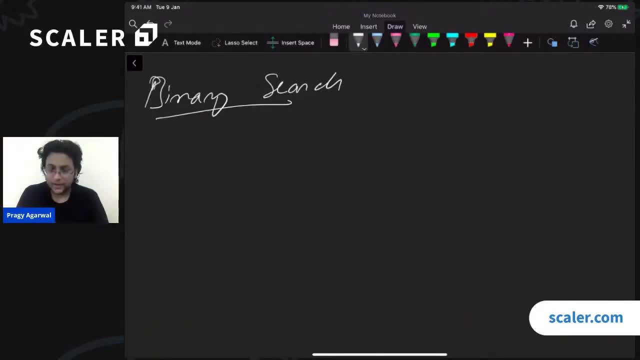 we are going to binary search. There are multiple ways of doing this. We are going to binary search on the index only of. We are going to binary search over the smaller array. Smaller array, right? So first of all, suppose that this is A1.. 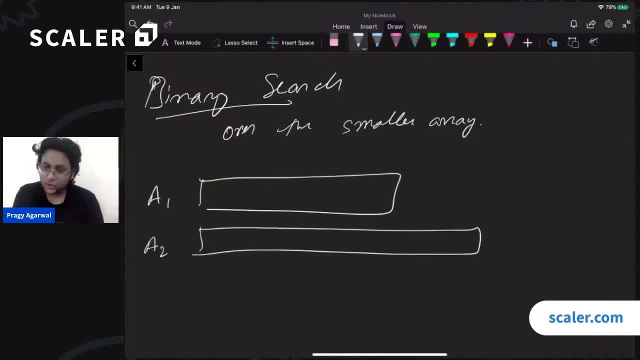 Suppose that this is A2, right, So can I assume? Can I assume that I assume, without loss of generality, that a1 is smaller than a2?? Can I assume that the length of a1 is smaller than length of a2?? Yes, If that is not the case, then I can just swap those arrays. 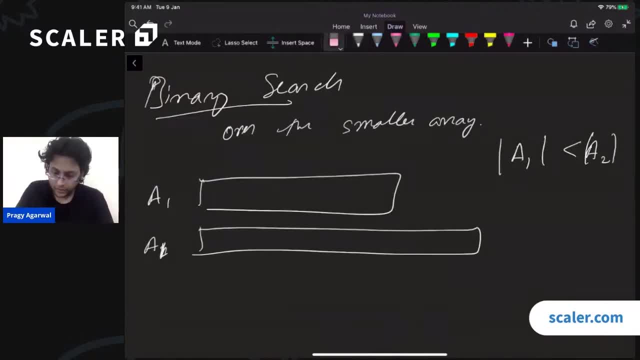 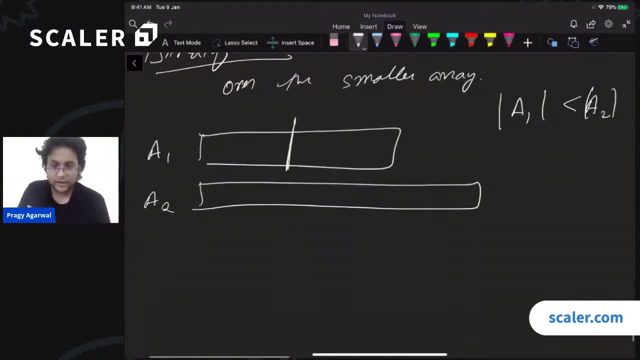 right, I can call this a1 and this a2. if that is not the case, right? So I can let us assume that a1 is the smaller array. So what we are going to do is we are going to binary search in this smaller array. all right, So we will have some low, we will have some high. 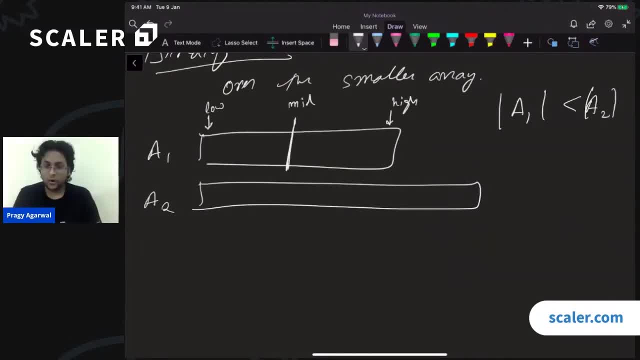 and we will calculate a mid all right Now. once we have this mid, the question is: when will a1 of mid be the correct median? be the answer: What has to be true? What has to be true for a1 of mid to be the correct median? What has to be true? 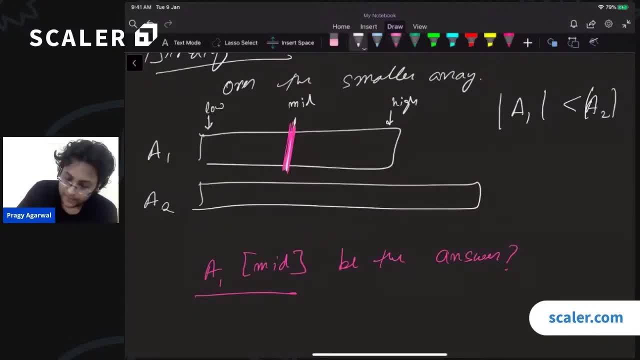 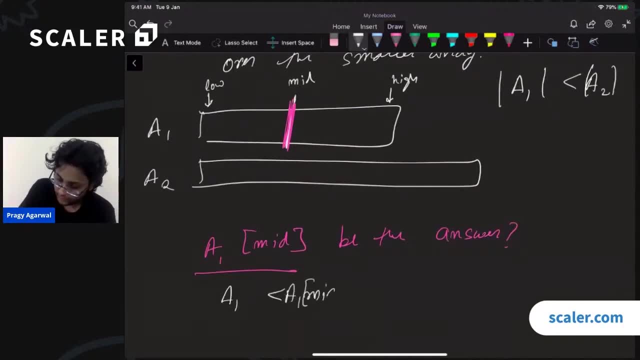 Okay, If A of mid is the correct medium, then how many elements? how many elements in A1, how many elements in A1 are less than mid? A of mid? How many elements in A1 are less than A1 of mid? 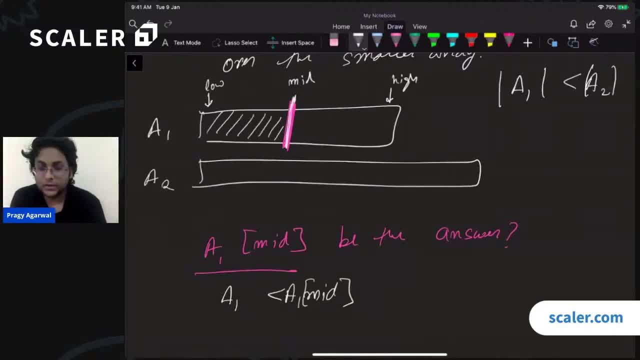 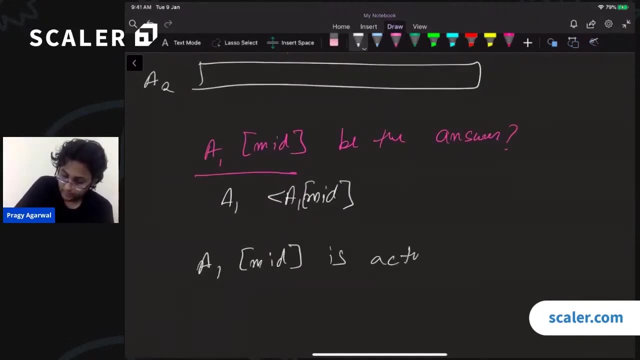 When all these elements are less than A1 of mid. Yes or no, Do you agree? And how many elements are greater than this? Well, all these elements are greater than it. Yes, If A1 of mid, if A1 of mid is actually the medium, is actually the medium, right? 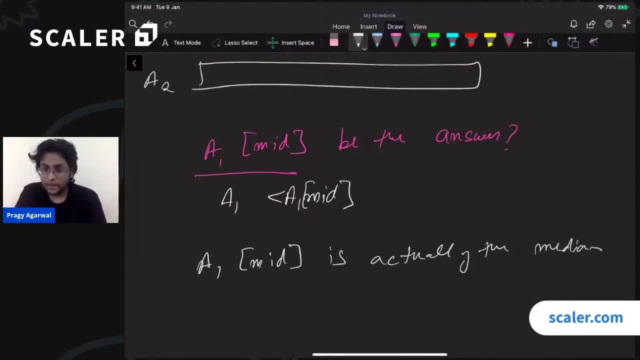 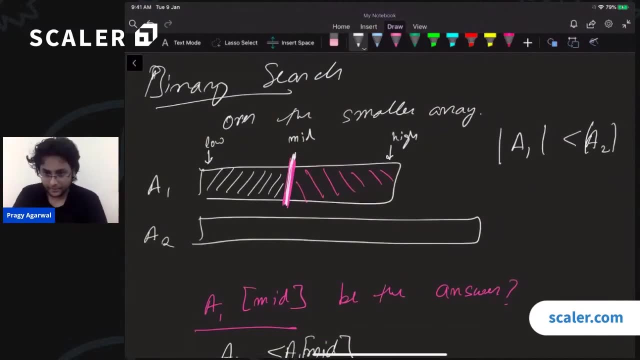 Then what must be true? What must be true Then? half of the elements, right across both the areas. half of the elements must be less than it and half of the elements must be greater than it. Yes, half of the elements must be less than it and half of the elements must be greater. 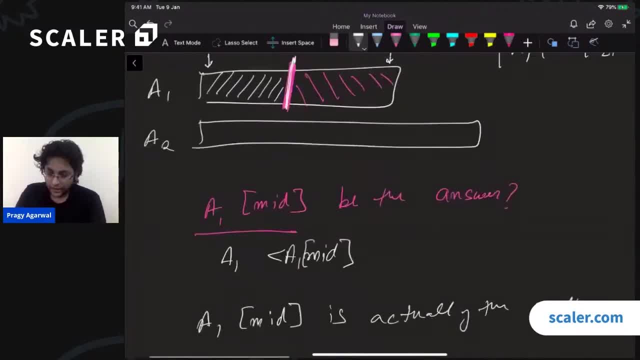 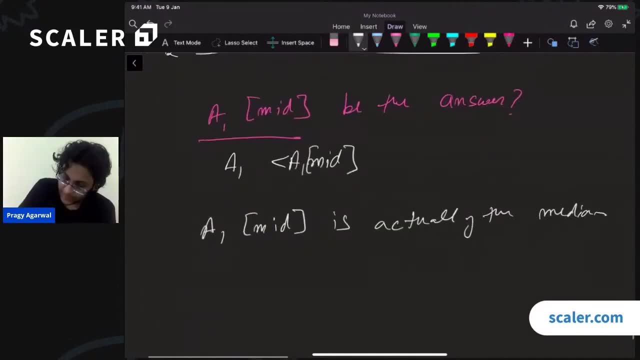 than it Cool. So let us check. Let us quickly check. So if, if A1. If A1 of mid is actually the medium, then how many elements in A2 should be? or if this is the case, if this is actually the medium, then how many elements in A2 should be less? 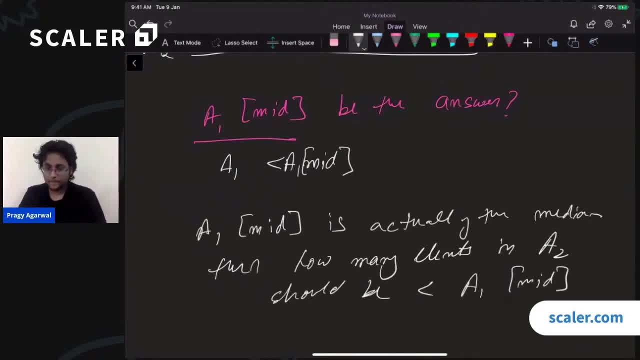 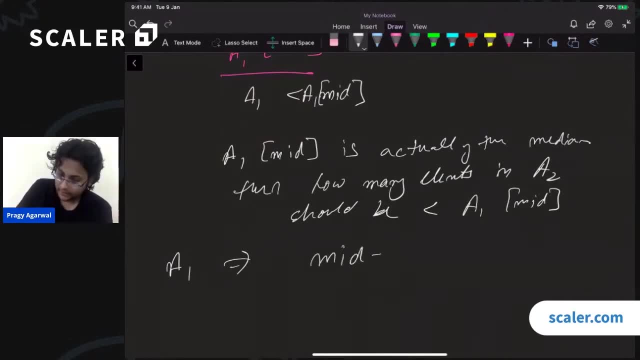 than A1 of mid Right? That is the question, Right. So we know that in A1, there are in A1, there are mid minus one elements, or there are mid elements, mid number of elements. So the the count of elements in A1 that are less than mid is mid, right. 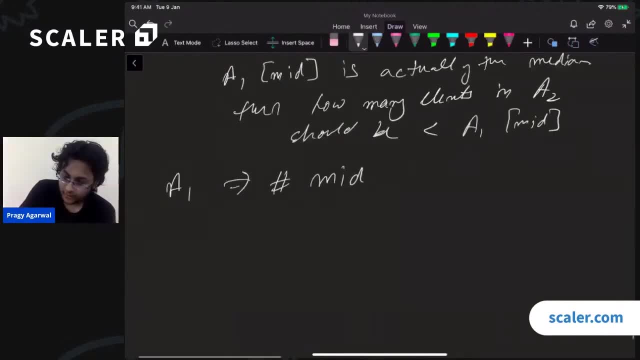 So the count, so the total number of elements that have to be less than A of mid. the total number of elements that has to be less than A of mid should be n plus m by two, Yes or no? Should be n plus m or plus one by two? actually, 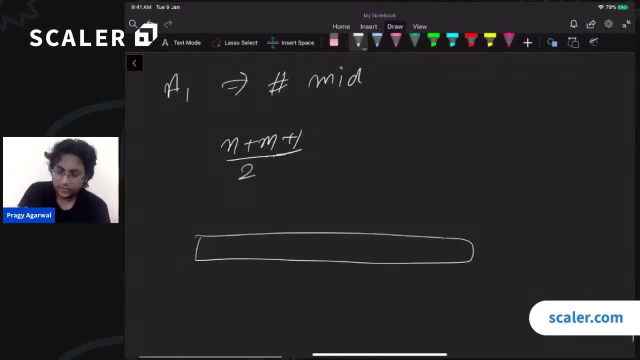 Do you guys agree, If I have this total sorted array, if I have this total sorted array- and this is actually the medium- Then half, Half the elements will be less than it and half the elements must be greater than it. So if this many elements are less than it, overall, overall right. 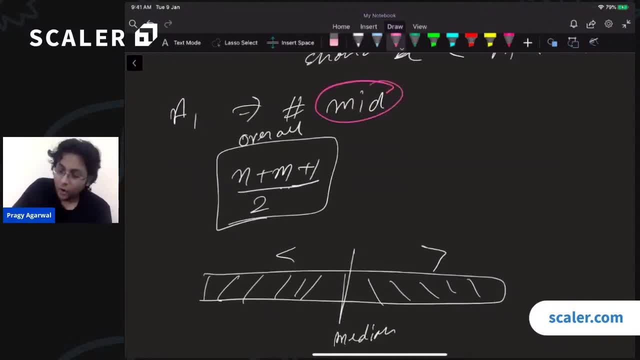 And out of these, out of these, this many elements were already present in A1.. This many elements were already present in A1, then, what is the number of elements that are present in A2, which are smaller than this A of mid? 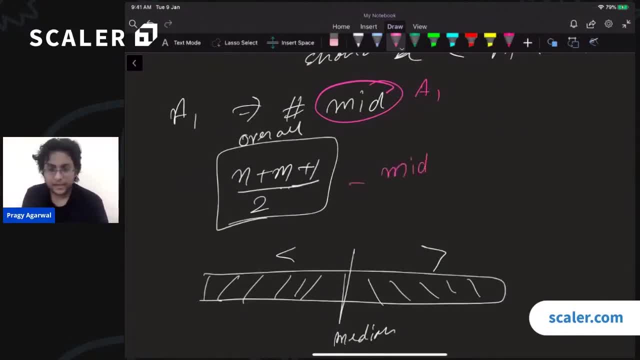 So this many elements, this many elements were already present in A1, so this must be the number of elements. This must be the number of elements. This must be the number of elements in A2, number of elements in A2 that are less than mid. A of mid. 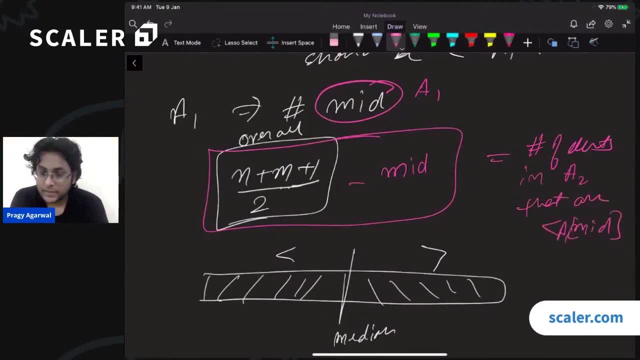 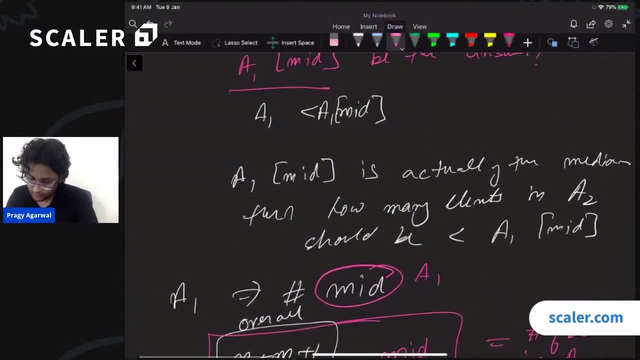 Yes, Does that make sense? How can you say that length of A1 is equal to mid? No, no, no. We are not saying that the length of A1 equals to mid. We are not saying that. We are saying that consider, consider that. assume that mid is the correct medium. 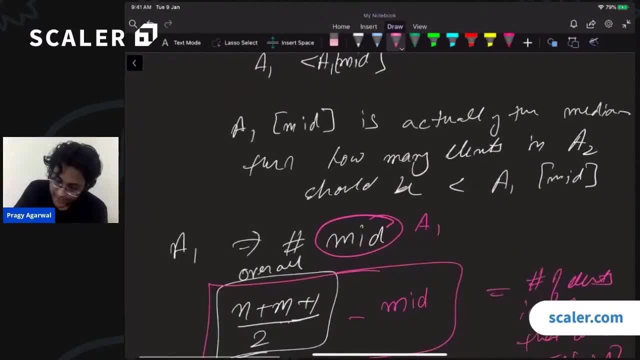 Assume that mid is the correct medium. Assume that mid is the correct medium. Now the question is: do I take a mid Again? this is not to be true. If there are these many elements that are less than it in A1,, then how many elements should? 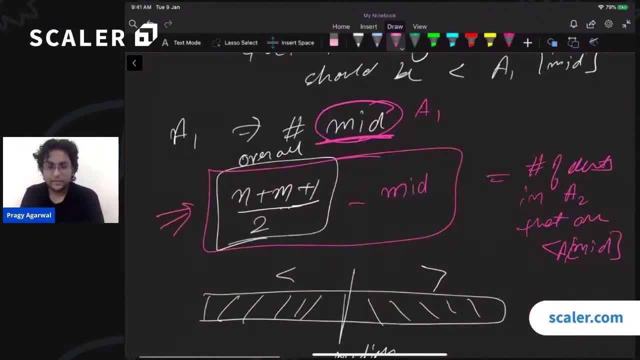 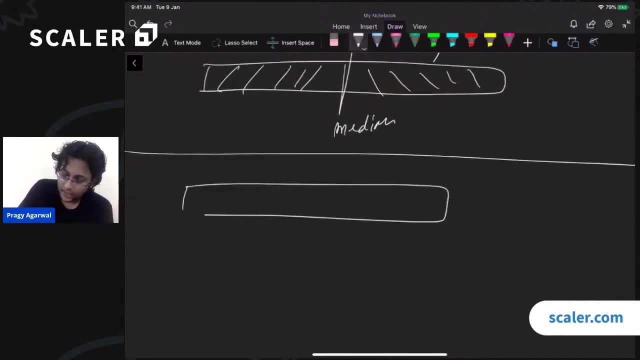 be less than it in it, And this is the answer. This is the answer: These many elements should be less than mid in A2.. So what we can actually do is what we can actually do is we can start with some low over here. 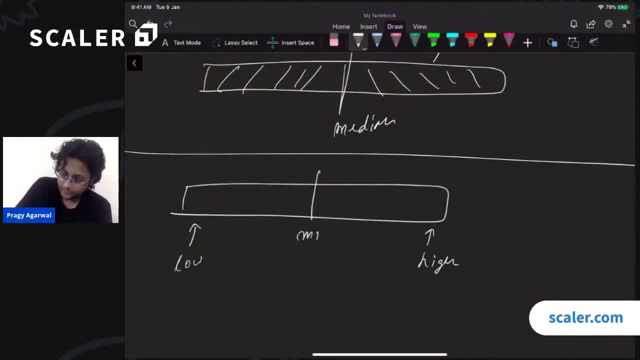 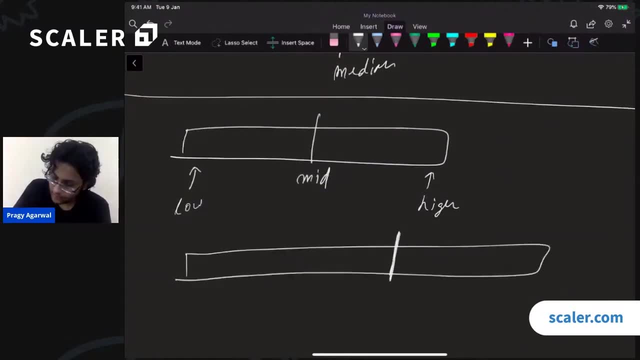 We can start with some high over here and we can calculate a mid. Now what we can do is we can look at, we can put a marker at n plus m Arringten, send plus 1 by 2 minus mid. right, we can, we can look at this particular index. right, we will have four. 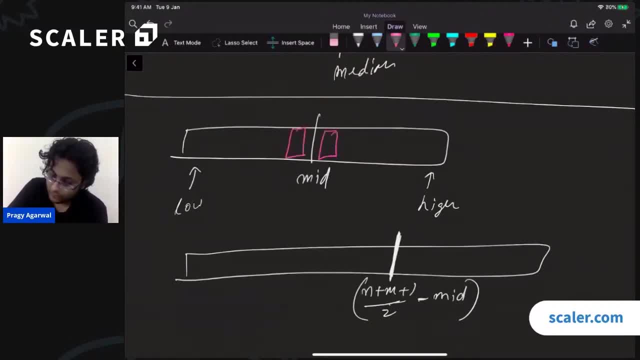 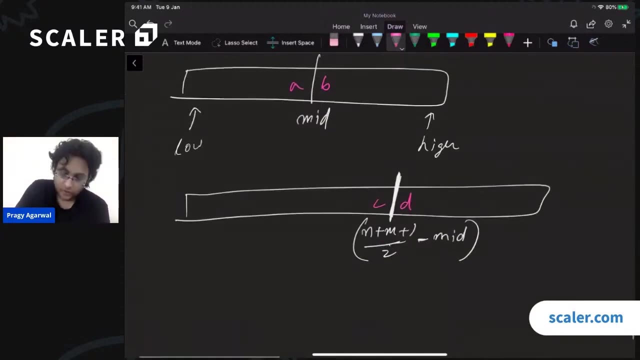 elements. now, we will have four elements. we will have one over here, one over here. one element over here, one element over here, right? so, let us? let us call these elements a, b, c, d. let us call these elements a, b, c d. a b c d, right now. when is this a of mid? when, so? when am i at the correct position? 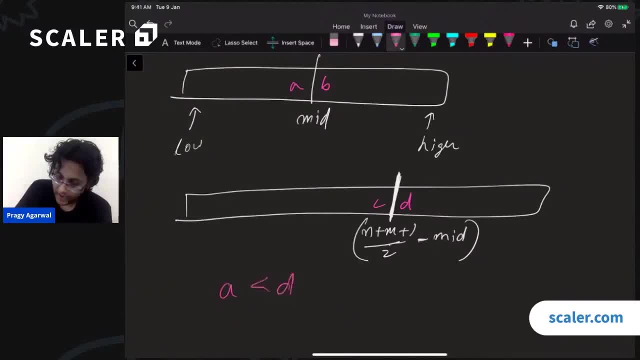 i am at the correct position when a is less than d and b and c is less than b, right, if this is the case. if this is the case, then this marker, these two markers, they point to my median, do they not? yes, do they not point to the median? why do they point to the median? because the number of elements 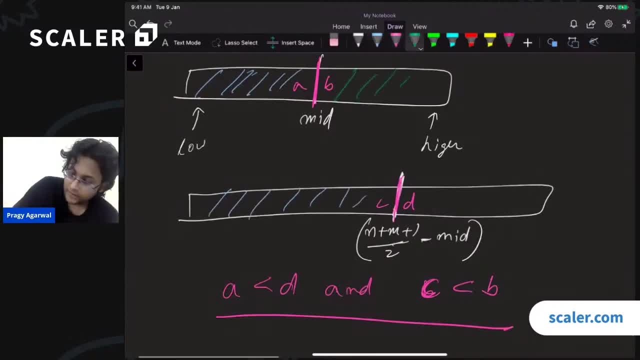 the number of elements over here and the number of elements over here is equal. do you guys agree? the number of blue elements is equal to the number of green elements? yes, and how are they equal? because i have chosen to be right, because i have used this formula. 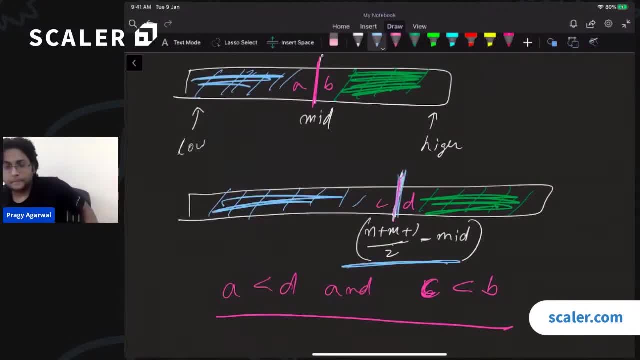 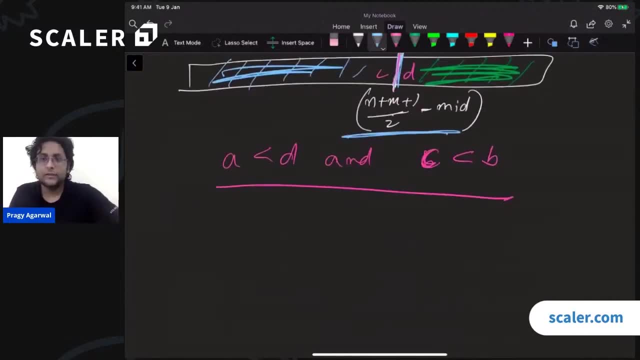 to make sure that i land at the correct spot over here. does that make sense? cool. so, guys, if this is not clear to you at the moment, we will. we will make sure to basically explain this with an example. okay, so we will. we will. we will look at a concrete example. 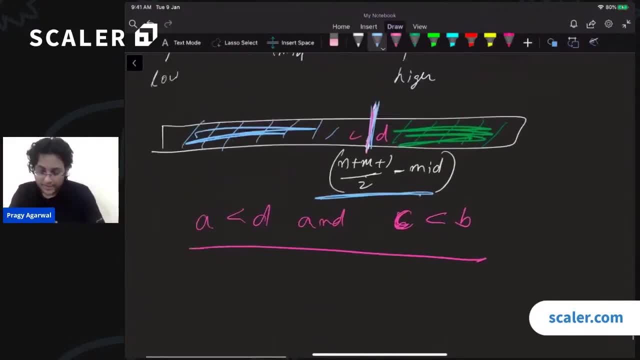 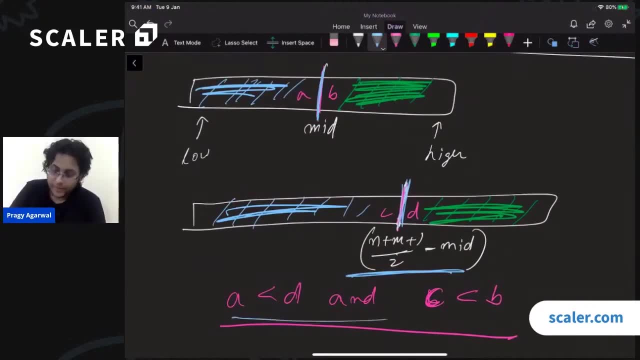 but let me first explain the idea, right, let me first explain. so, basically, what we have to do is we have to binary search for a mid such that the property of the median, such that this property of the median becomes value. all right, now look at a concrete example. let us look at a concrete example. 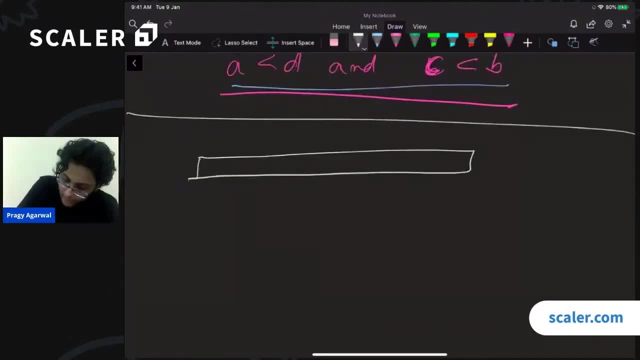 to further establish this. suppose that we have this array: zero, one, one, three, five, seven, all right. and we have another array, suppose four, five, six, eight, eight, twelve, twenty, thirty, all right, let us mark the indices: zero, one, two, three, four, five. zero one, two, three, four, five, six, seven, all. 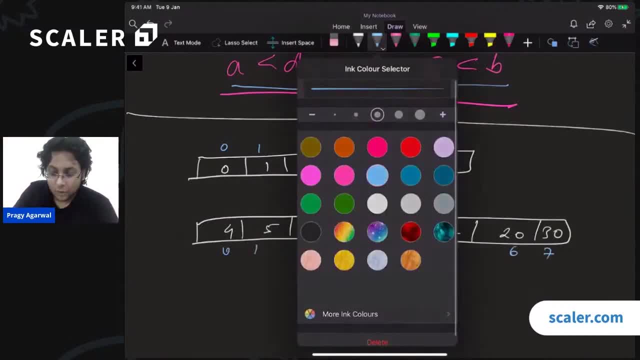 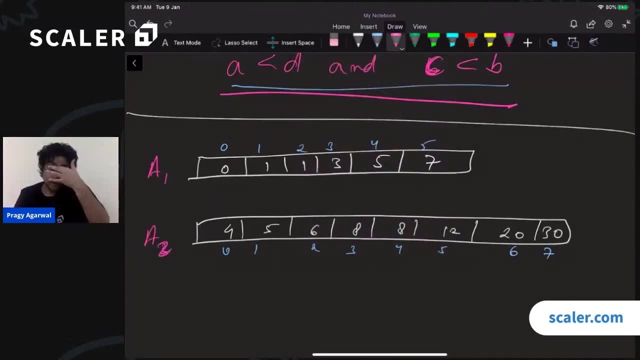 right now which one is a1 and which one is a2, which one is the smaller array? this is the smaller array and this is the larger array. yes, this is the smaller array and this is the larger array. so let us, let us have two pointers: let us have the low pointer and let us have the high pointer. 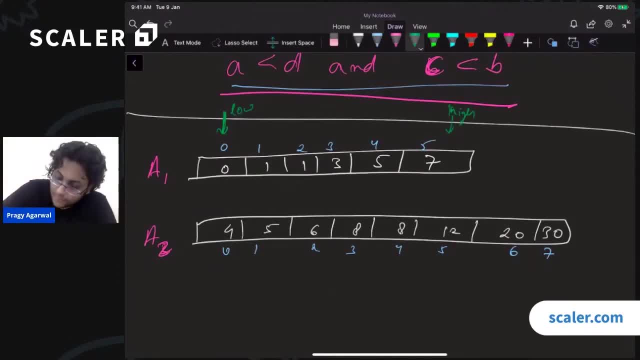 yes, let us have the low pointer. let us have the high pointer also. what is the value of n? the value of n over here is six. and what is the value of m? the value of m is eight. yes, there are six elements in the a1 array and there are eight elements in the a2 array, yes or no? cool, so now we. 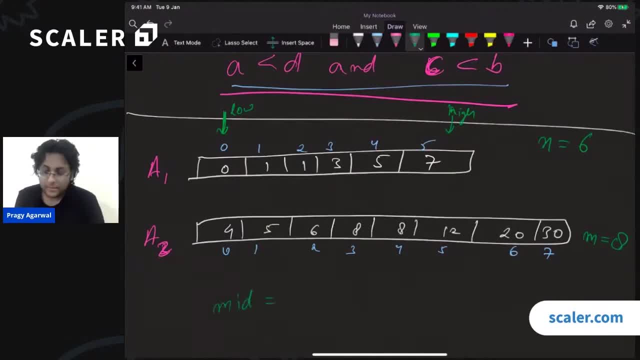 have this low and high, what will be the mid? what will be the mid? mid will be five by two, which will be two. yes, mid will be five by two, which will be two. so this is the midpoint. this is the midpoint, all right, and a1 of mid. 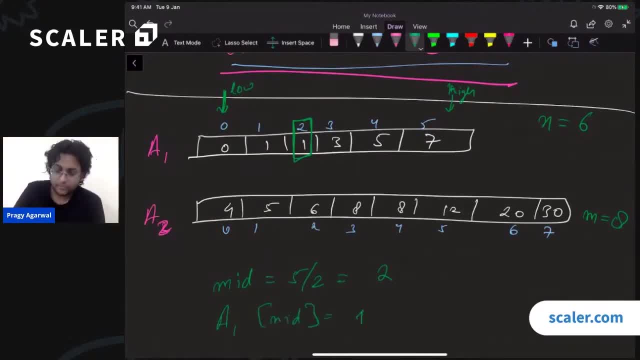 a1 of mid equals to what it is one right now. the question is: how many elements? how many elements in a1 are less than or equal to a1 of mid? how many elements in a1 are less than or equal to a1 of mid? well, these many elements, right, this? 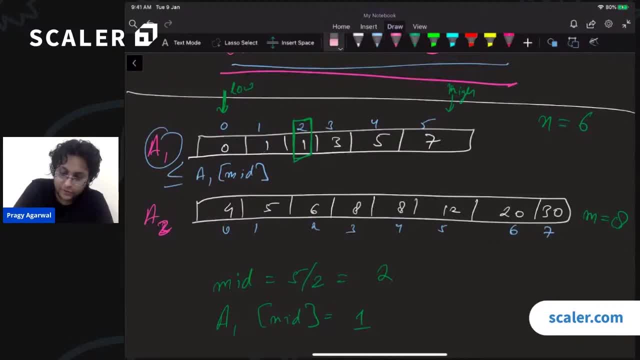 element and this element. yes, there are two elements that are less than or equal to a1 of mid. what is the count of that? well, the count is simply mid right. mid is the count. do you agree? right now, if, if this one, if this one was actually the median, if this one was actually the median, then 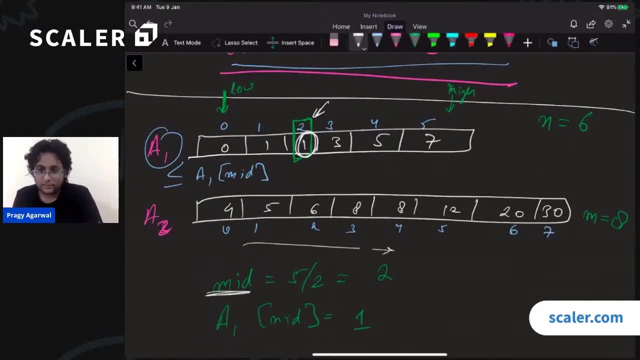 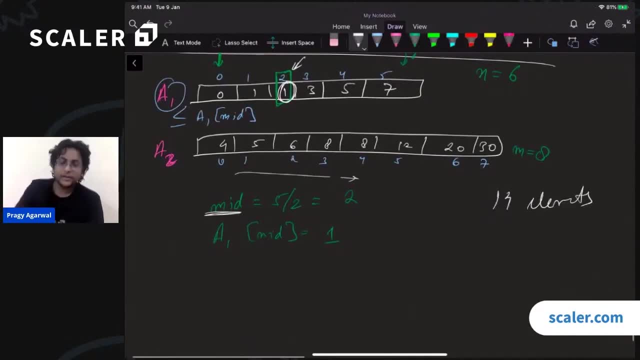 how many elements should in this array should be less than one? right in this array, how many elements should be less than one? well, total, there are 14 elements. right, total, there are 14 elements. so if, if my median, if there is my median, then half of the elements must be less than it. 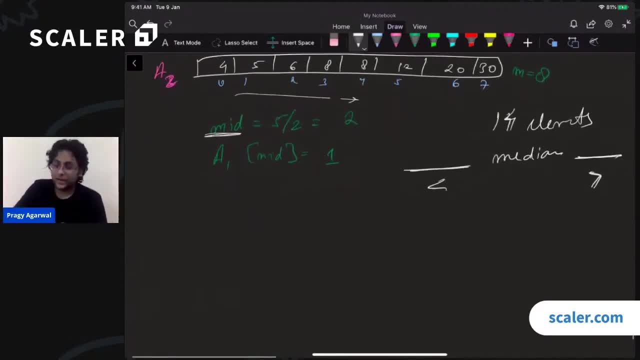 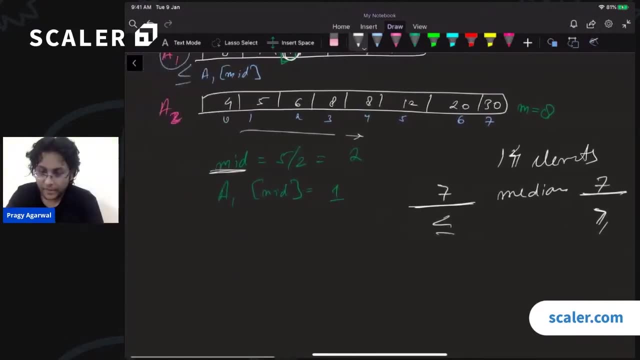 half of the elements must be greater than it, right? so basically, what i am saying is: seven elements should be less than or equal to it. seven elements should be greater than or equal to it. that is the property of my median right, yes or no? cool. so basically, if this is the case, 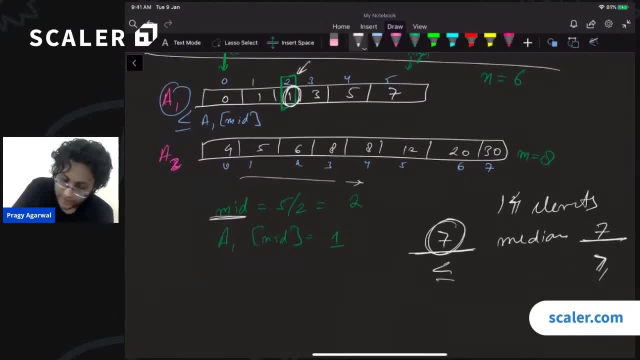 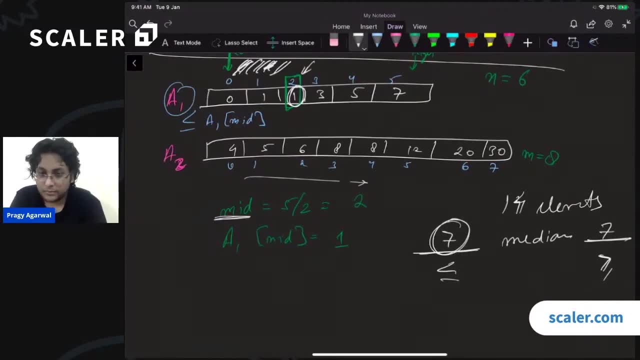 if this is the case, and two of these. so two of these seven elements. two of these seven elements come from a1. two of the lesser elements come from a1. then how many lesser elements should come from a2? how many of the lesser elements should come from a2 when you are from a1? so 5 must be from a2. 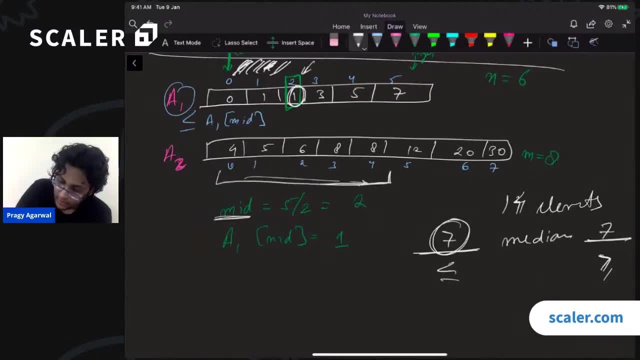 right 5 must be from a2. so all these elements, all these elements should be less than one. it should be less than this one. if one was the median, then all these elements should be less than one. are they less than one? are they really less than one, yes or no? they are not less than one right, so one. 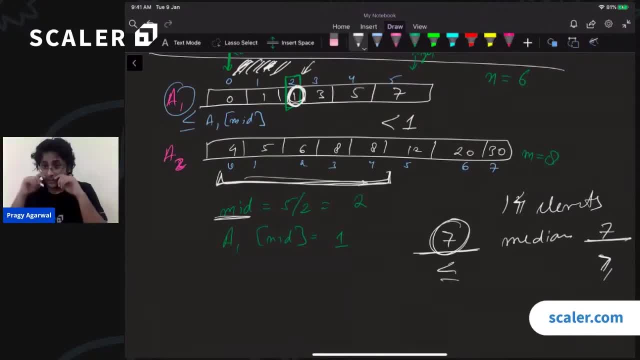 cannot be the median. does that make sense? because because all these elements, they are not less than one, so one cannot be the median. so my median is two small. in that case i have to increase my loop. right, i will try to find the median on the right hand side. is that clear? 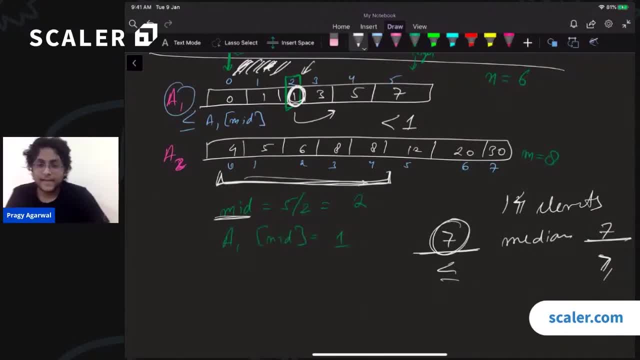 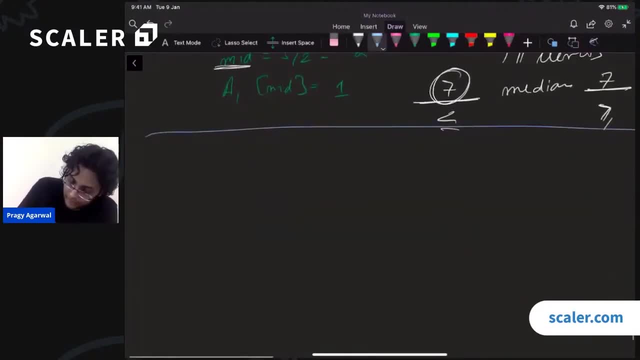 is that clear guys? yes, so basically, what we are saying is. basically what we are saying is that let us say: let us say that we have, we are going to have a low and we are going to have a high, and we are going to calculate the mid as low plus high. 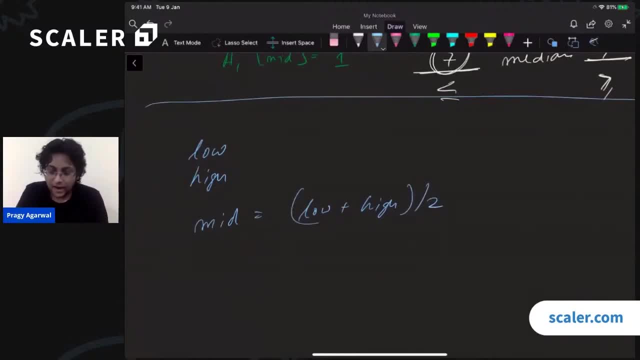 two right now. how many elements are less than mid, e of mid in the first array? well, that is just me. so how many elements should be less than it in the second, and how many elements should be less than it in the second array? that should be what that should be: n plus m plus 1 by 2 minus mid. 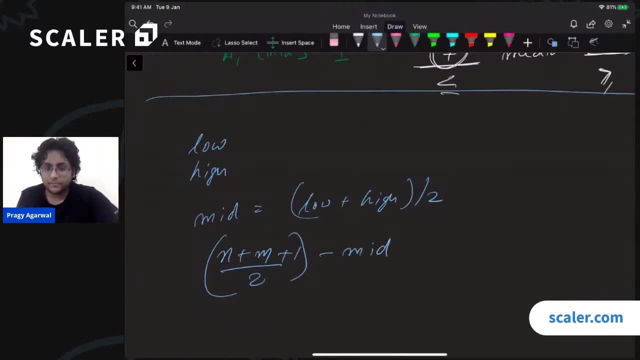 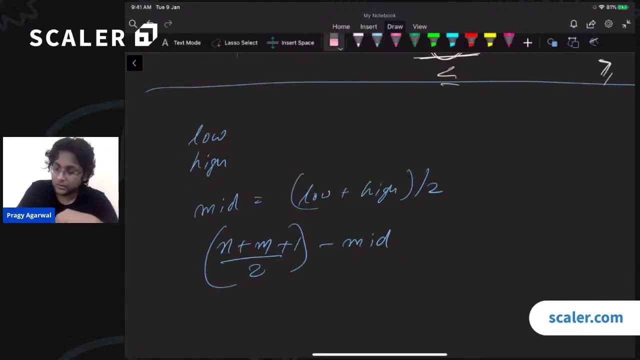 yes, that should be n plus m plus 1 by 2 minus right. so what we can now do is: so this is, this is this is the partition, this is basically the partition partition of a2.. Now we can simply check now. we can simply check. now we have four elements. we have a1 of mid, we have a1 of 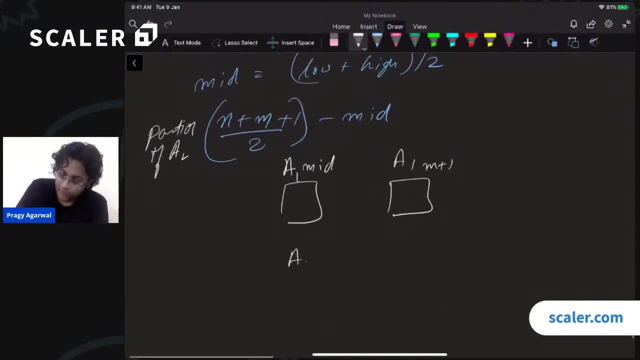 mid plus 1 and we have a2 of partition and we have a2 of partition plus 1.. Right, Is that clear? And we can check if this, if this element is less than this element and this element is less than this element, then our partition is valid and we have the correct. 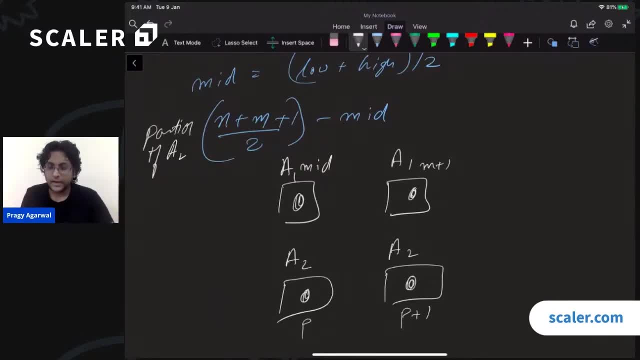 midpoint, Then our partition is valid and we have the correct midpoint Right. Why n plus m? why this plus 1 thing? Well, this is just to make sure that the number of elements, number of elements that are on the left, are greater than or equal to the number of elements. 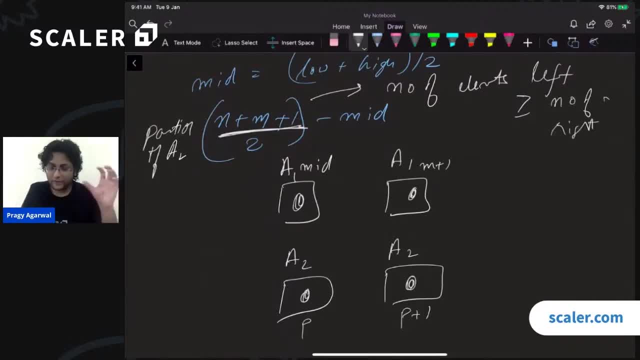 on the right Right. That is just to make sure that the number of elements on the left are either equal to the number of elements on the right or they are one more than the number of elements on the right. Okay, So, if I mean, if the number of elements is even, then there will be a mismatch, right? 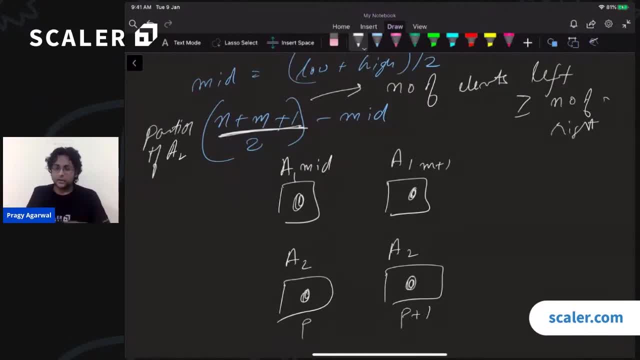 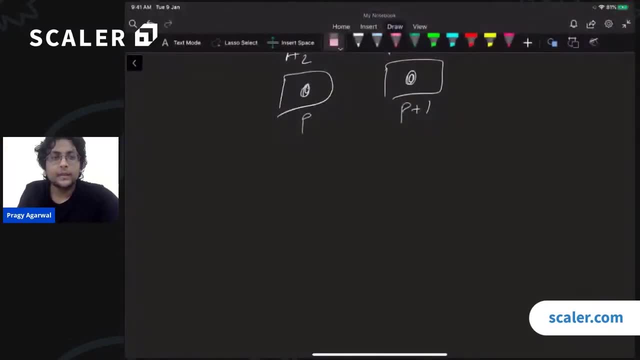 You can't have both the same number of elements on both left and right, So we will have one extra element in the left. Is that clear guys? Just give me a second. Let us look at some code for this. Let us look at some code for this. So what will really happen is: 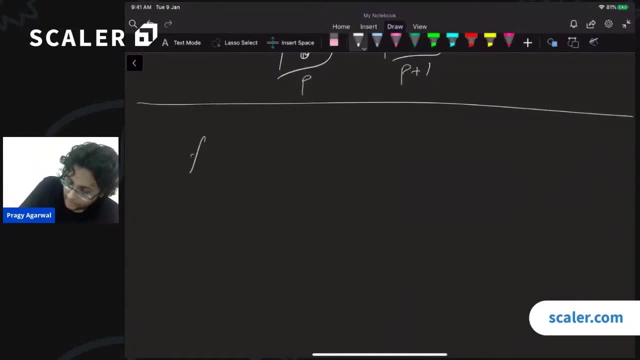 let us suppose that we have two arrays. So we have find median, find median, and we have two arrays. We have A1 and we have A2.. Right, Let us, let us call this A and D, Let us call this the array A and the array B. Alright, for simplicity, Now what we are. 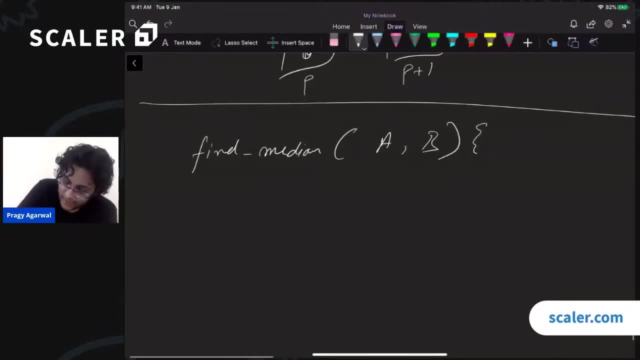 going to do is: we're going to make sure. we are going to make sure that array A is smaller. We are going to make sure that array A is smaller. How can we make sure that array A is smaller? How can we make sure that array A is smaller? 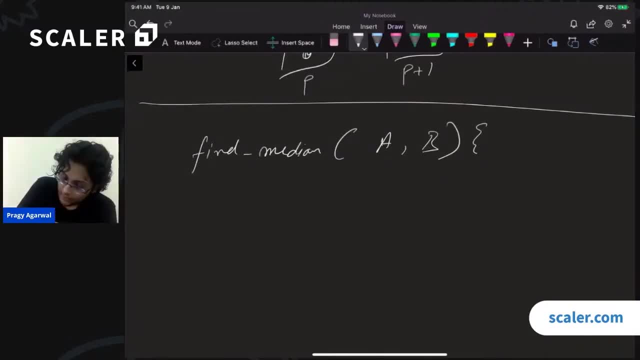 smaller. well, we can, we can declare it over here, right? so we can say: if the length of a a dot length, a dot length is greater than b dot length, if it is in fact larger, then simply swap the values of a and b, right? so this will ensure that the that this particular array is smaller. 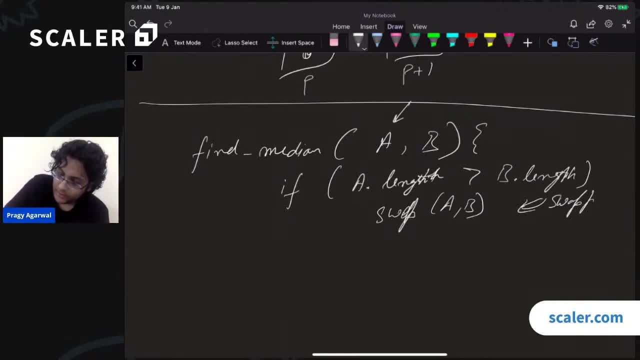 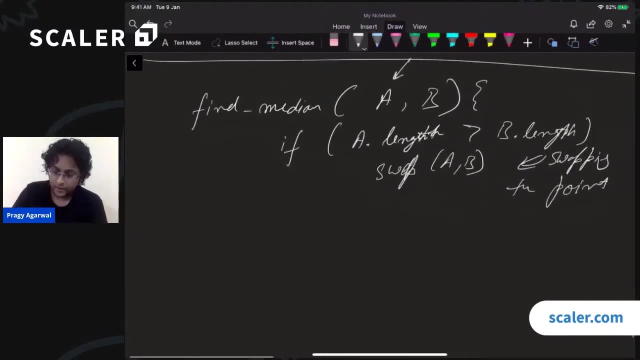 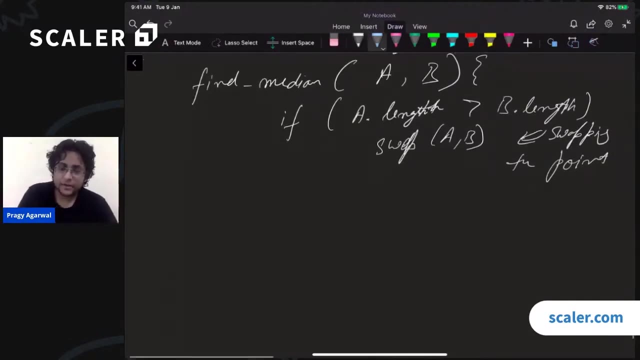 right and notice that this swap is just swapping the pointers. this is just swapping the pointer. this is not actually moving the arrays. this is just swapping the pointers, right. so now that we have ensured that a is the smaller element, so now what we can do is: we can have, we can have a low. 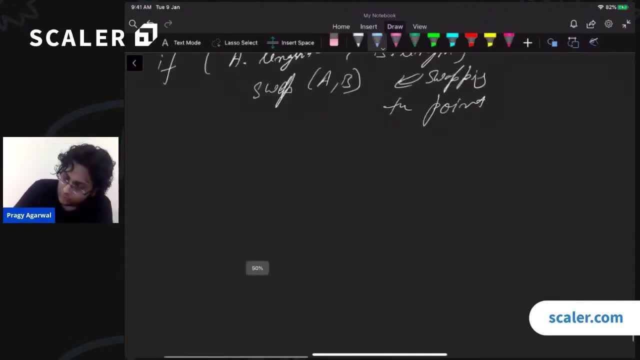 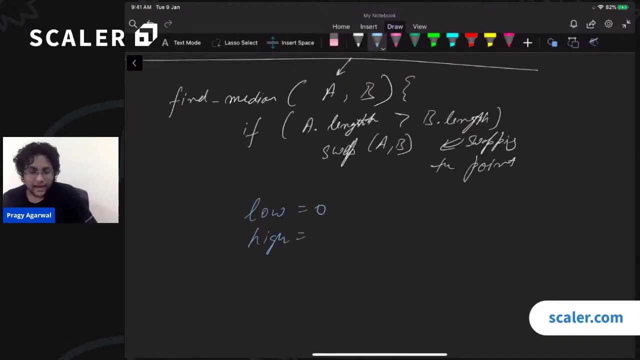 and we can have a high right, so we can say that, all right, low. we can initialize low equals to zero and we can initialize high equals to what. so what array are we searching over? we are searching over the smaller array. we are searching over the smaller array, so we will say high equals to. 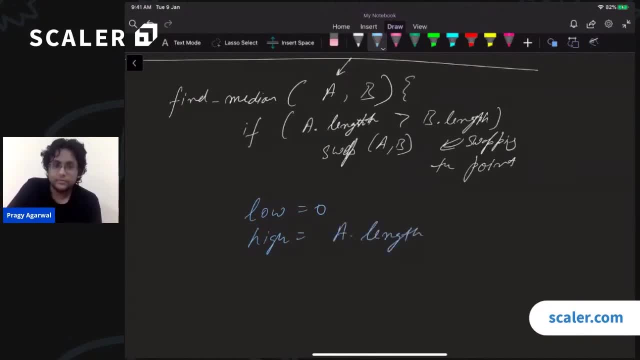 a dot length, it's a dot length, right. and basically, let me let me also do one thing, let me let me also save two values over here, n and m. so let me say, for simplicity, let me say, that n equals to a dot length and m equals to b dot length. b dot length, right, so we have cf the length. 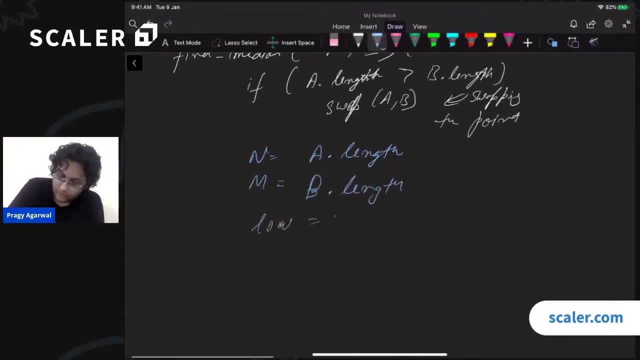 or the length in nm. so now my low will be zero and my high will simply be n. all, right now i can loop. now i can loop, while my low is less than or equal to the high. right now, what is the first thing that i should do? the first thing that i should do is i should 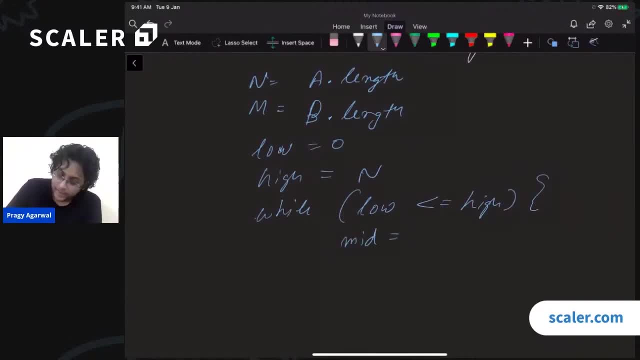 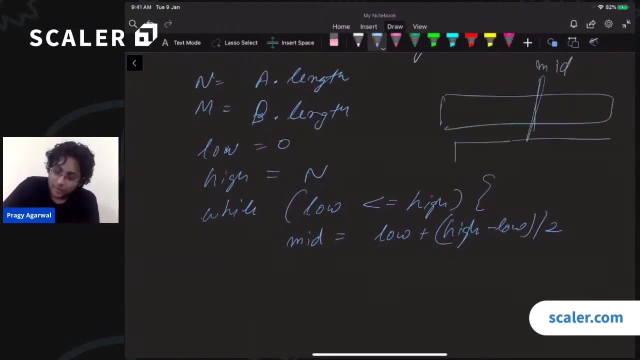 calculate the mid. i should calculate the mid. and what is the mid? the mid is simply low plus high minus low by two. right cool now, this mid. this mid is a marker in the first array. this mid is a marker in the second first array. what will be my corresponding marker in the second? 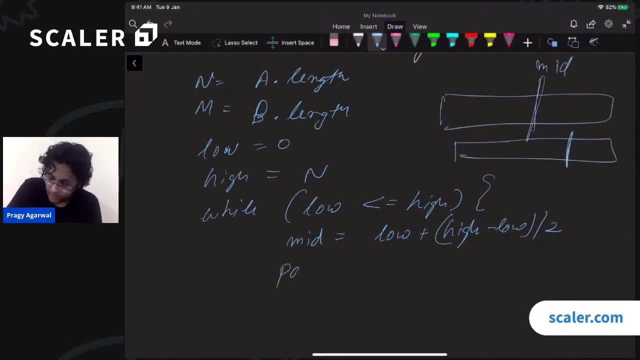 array, as we just saw that corresponding marker. that is called this partition right. this is called partition. this is going to be n plus m plus 1 by 2 minus mid right. is this clear to everyone? is this clear to everyone that this will be the partition? 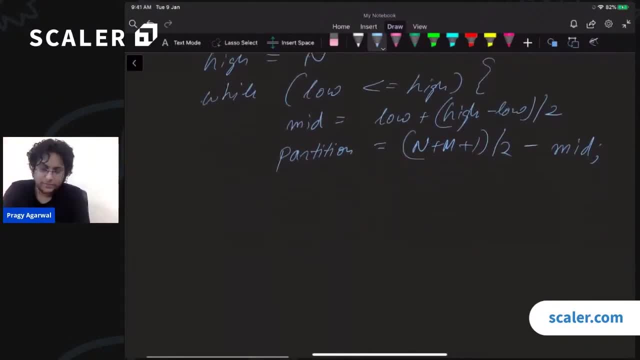 now, what we are going to do is we are simply going to compare values, to compare values. we are going to say that if, okay. we are going to say if a of mid, right, if a of mid is less than or equal to b of partition plus one. 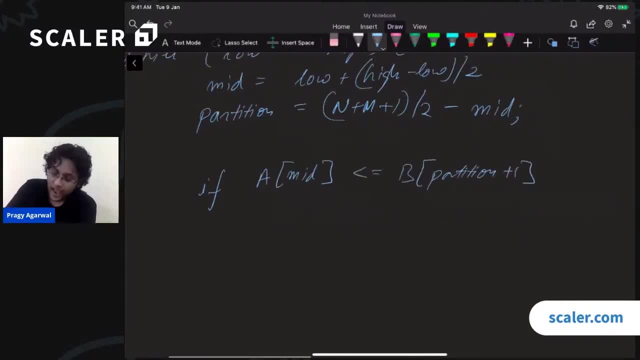 right, if a of mid is less than equal to b of partition plus one and a of mid plus one. or basically, i can write it the other way: i create: b of partition partition is less than a of mid plus one, right? if this is the case, then what do we have? 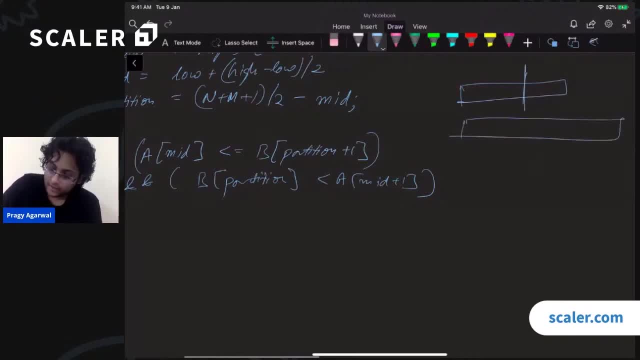 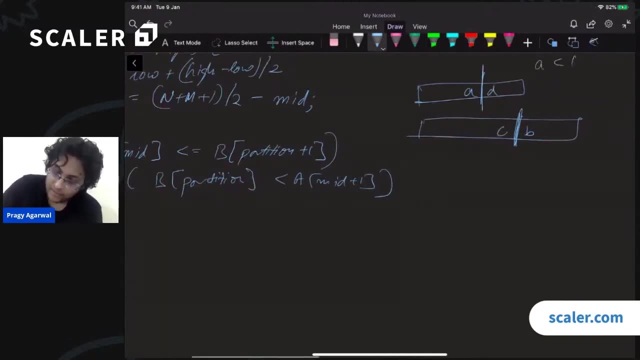 what do we have? we have two arrays. we have two arrays such that this element is smaller than this element right, and this element is smaller than this element right. so a is less than b and c is less than d, right, and we know that the number of elements over here is equal to the number of elements. 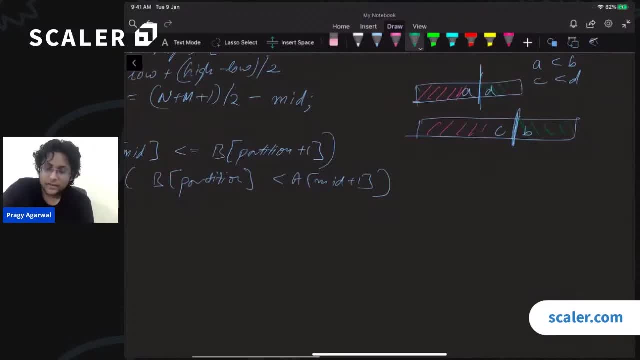 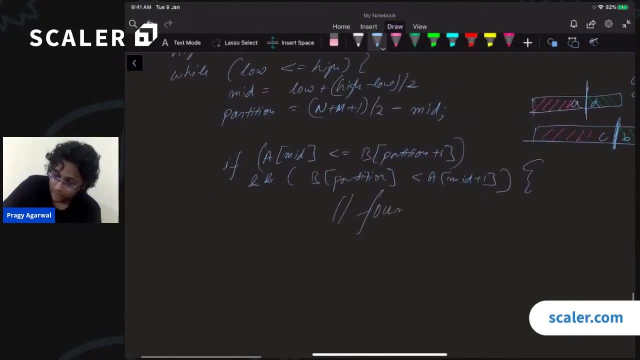 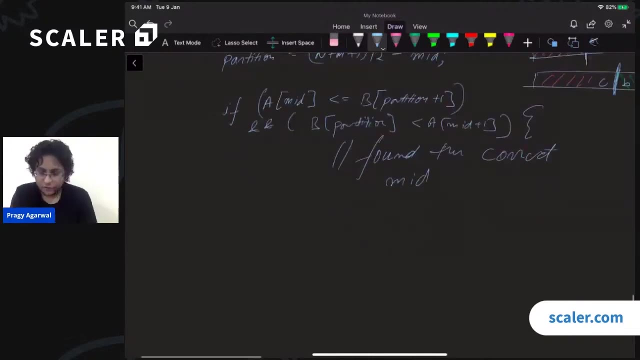 over here, right, if this is the case. if this is the case, then i have found my median, okay. so i have found my median over here, so i have found the correct, the correct midpoint, right, and i will actually return the median over here. so we will have two cases over. 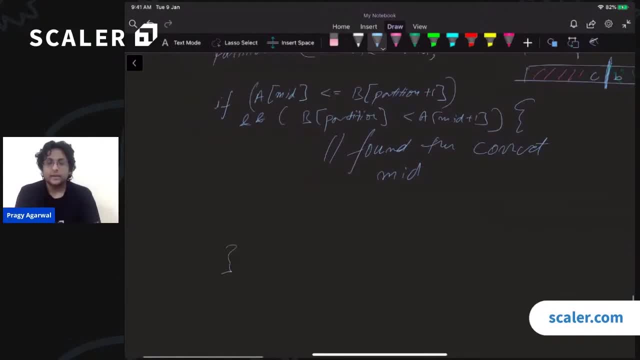 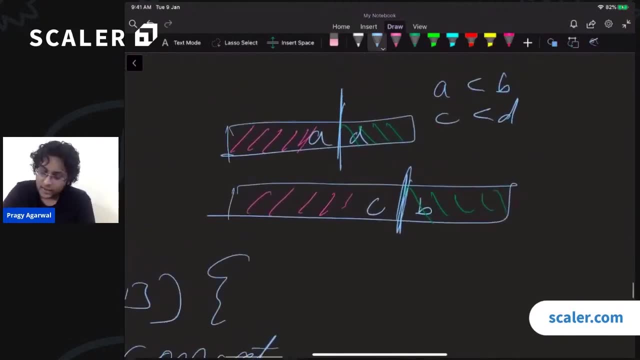 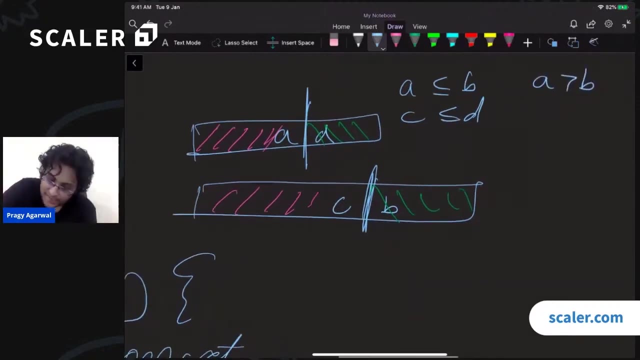 there as well. we will look at that, but if that is not the case, if that is not the case, then some other case will arise. right, then some other case will arise. what case can arise? what case can arise? so, either it can be that a is actually greater than b- right, it can be that a is greater than b- or it could be that c is. 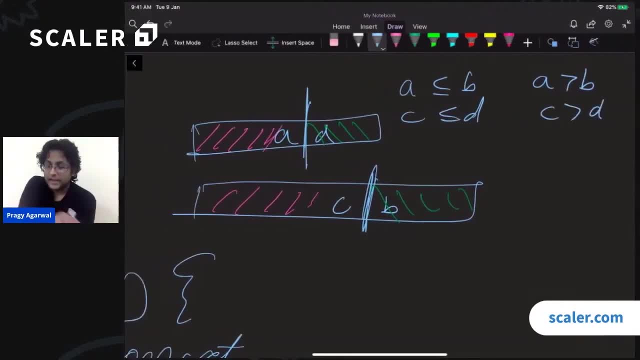 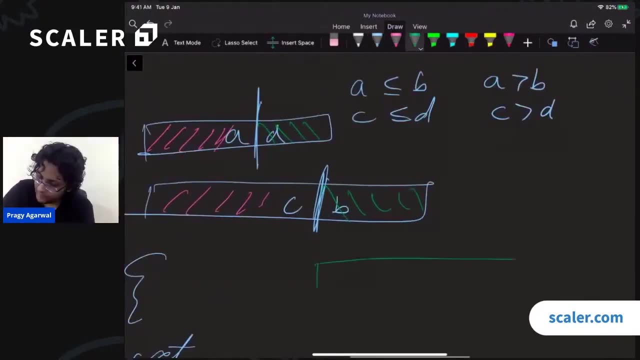 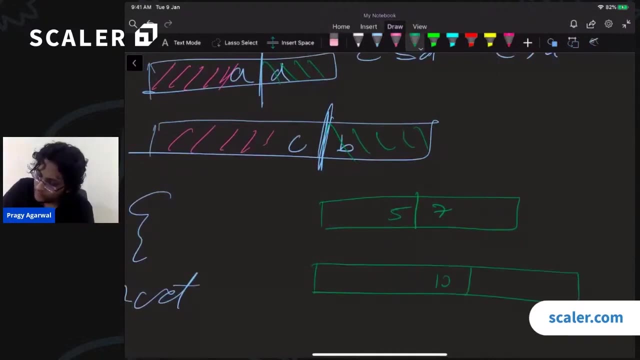 greater than d, yes or no? if a is in fact greater than b, if a is in fact greater than b, let us suppose that i have something like. i have something like 5 over here and 7 over here, right? and i have something like, or let's say, 12 over here. 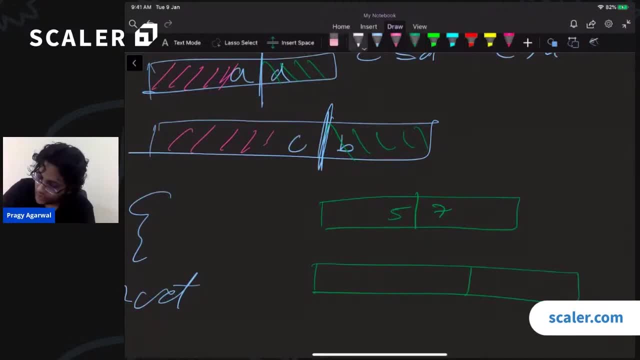 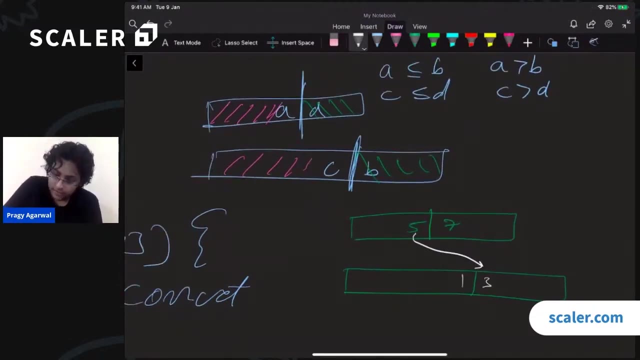 and sorry, not 12. let's say 1 over here and 3 over here, right? so if this element is greater than this 3, then what does that mean? this element happens to be greater than this 3, then what does that mean? it means that my midpoint is too high. this midpoint is too high, right, i have to move left. 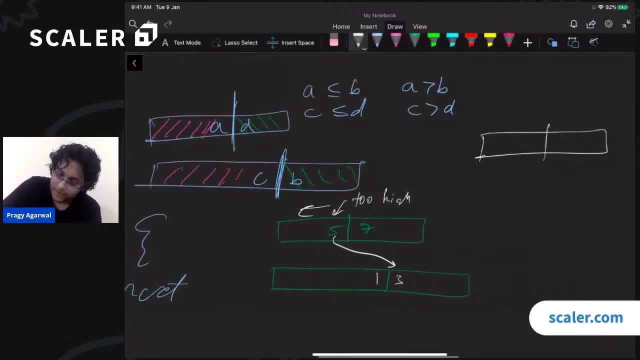 is that here? similarly, if that's the opposite, if i have 5 and 7 over here, right. if i have, let's say, 12 over here, right? so if, if this element is greater than this element, then my mid should be on the right. this, this value, this value: 7 over here, this is too low. 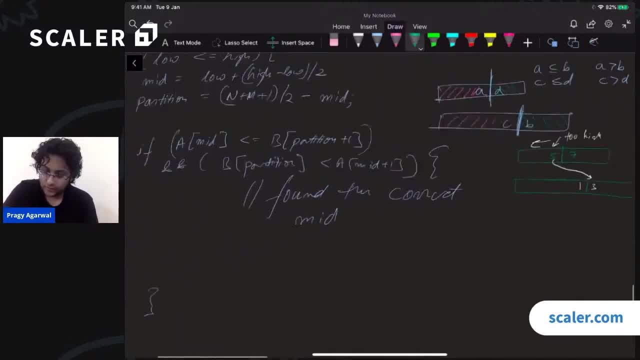 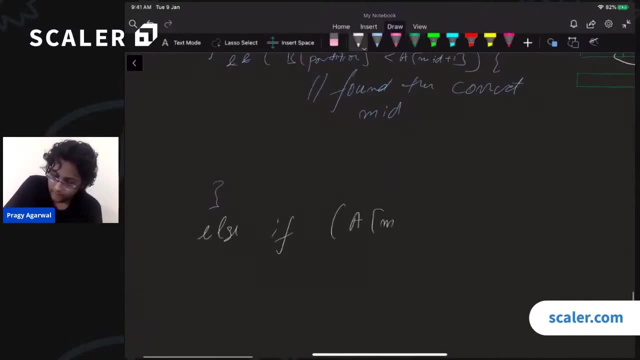 so I should move to the right it. so that is what we are going to do over here. we are going to say else: if else, if a of mid is greater than B of partition plus one, partition plus one, then I have to increase my mate. it's why I have to. 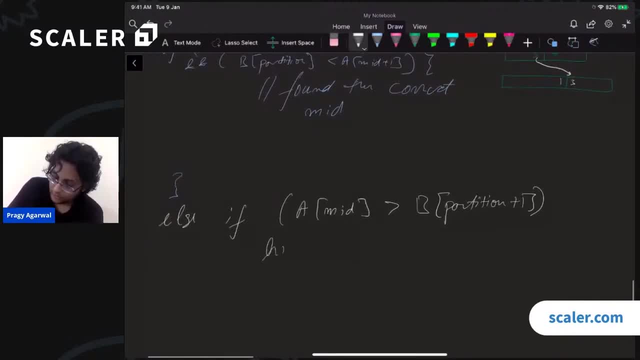 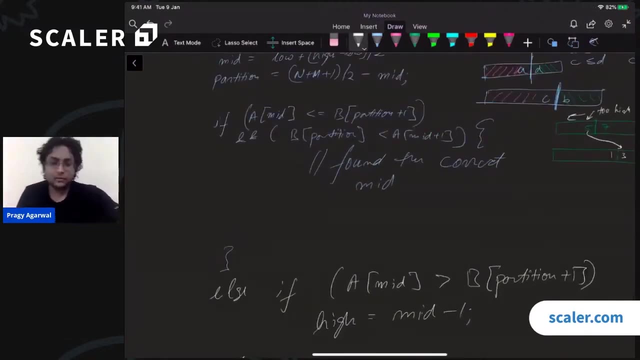 decrease my mate right. so I will say high equals to mate minus one. otherwise I will say no equals to make plus one mate plus one. all right. so this is the main value. this is the main value. now there are some more conditions that arise. there are some more conditions that arise. those conditions are: 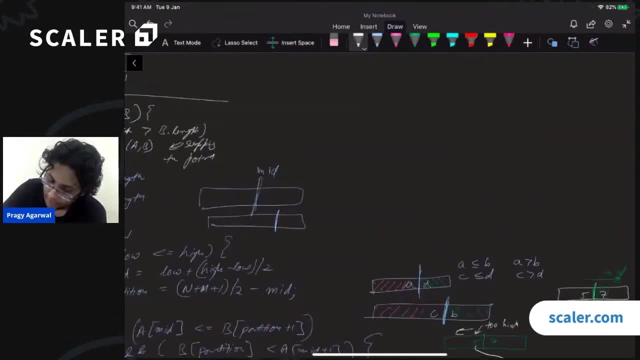 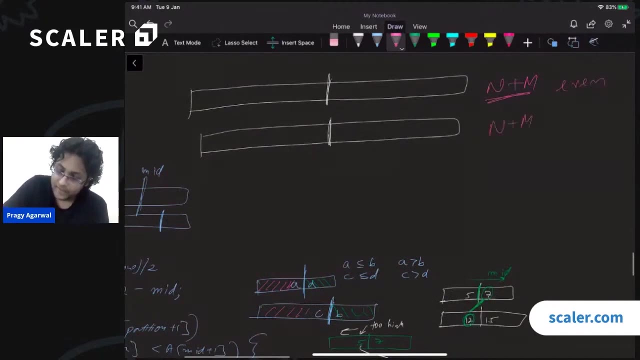 basically, let us let us take one more condition and then we are going to say one more example. let us suppose that we have this particular array and we have this particular array, all right. now we have two conditions: either the combine length, N plus M, either this is even, or N plus M, this is. 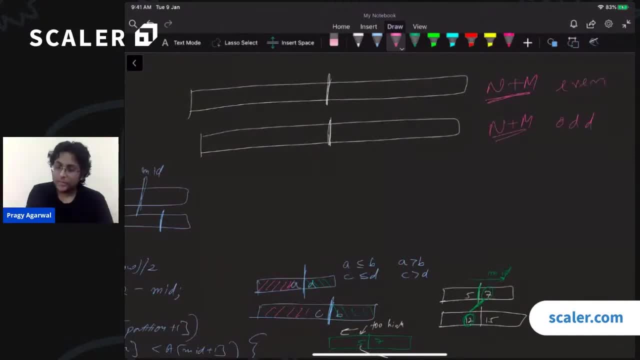 odd. either this is even or this is odd. now, if the length is odd, then what will be my medium? if the length is odd, then what will be my medium? this is a B, CD, right? we know, this is a c, right, then okay, and what will be my modem? fuck, I don't know. 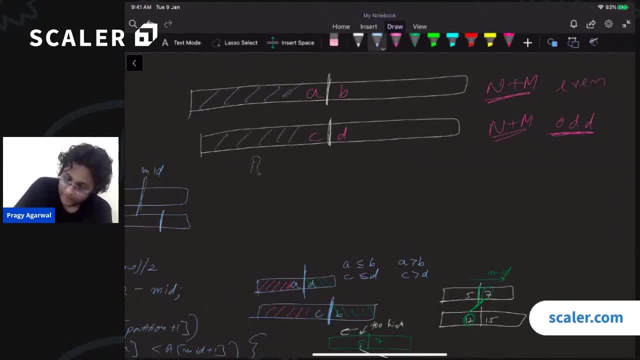 the number of elements over here. so the number of blue elements- blue elements- is either equal to number of green elements, is either equal to number of green elements, or it is equal to green elements plus one right. it is either equal to it or one more time. so if, if i, if, 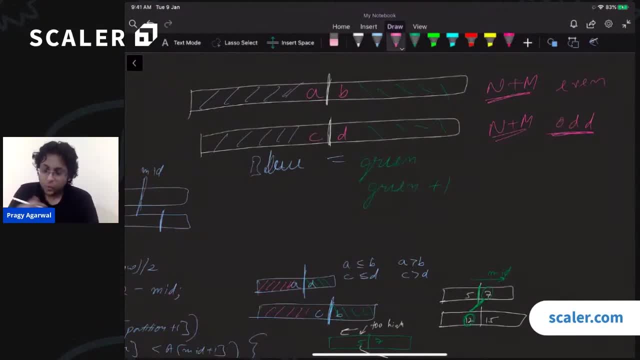 i found the correct midpoint over here, then. then, what can i say about the median? what can i say about the median? the median has to be one of these two things. right, the median has to be one of these two things, yes or no? yes or no, guys? and which one of these is the? 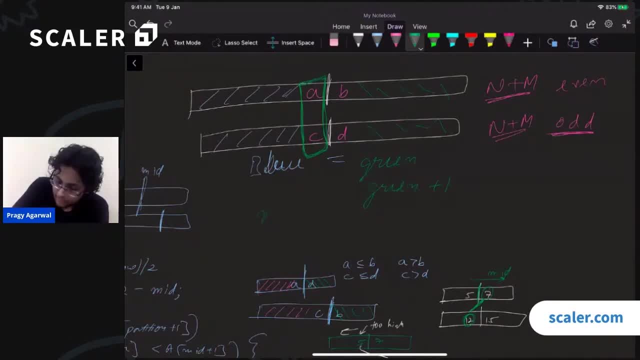 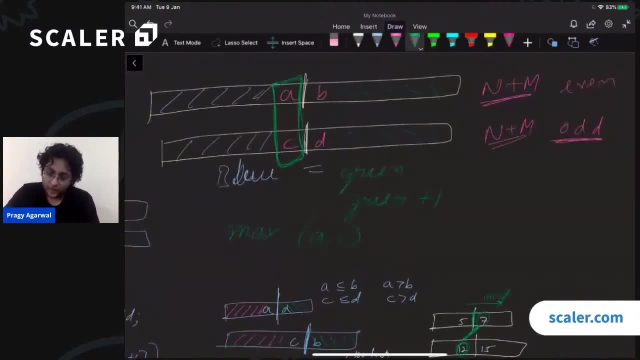 median going to be? is it going to be a or c? well, it is going to be the maximum of a comma c. yes, the median over here is going to be the maximum of a comma c. on the other hand, if the number of elements are even, if the number of elements are even, then the number 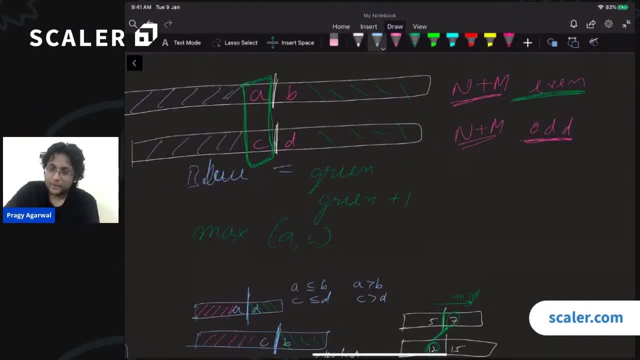 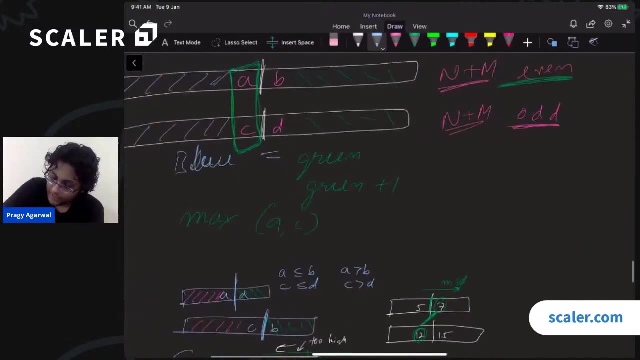 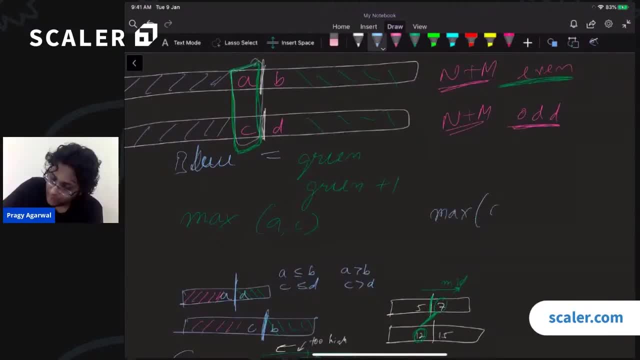 on the left right. i want to find the maximum value on the left, so x of a comma c, and i want to find the minimum value on the right right, so x of b comma p. and i want to take the average of those Because the median 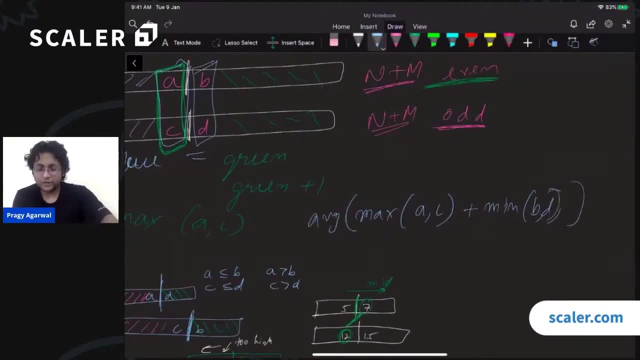 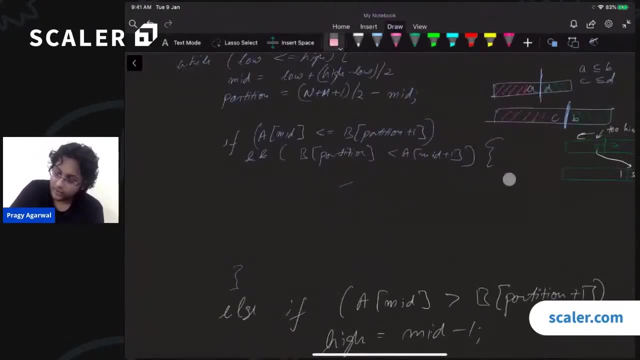 will be average of two different values over here. I have got to take the average of those, Is that clear? So basically, what do I have to write over here? I have to check. I have to check if, if n plus m mod 2. 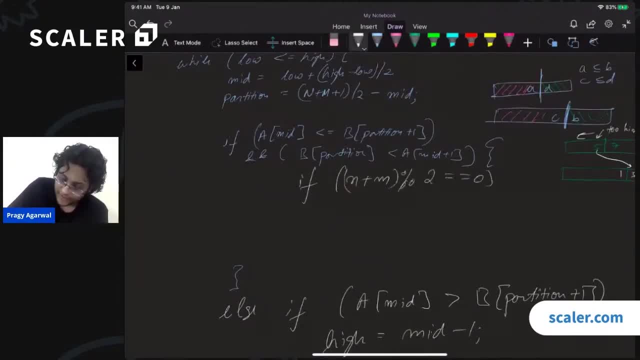 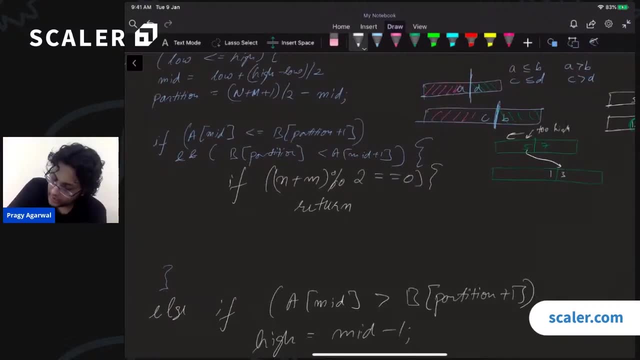 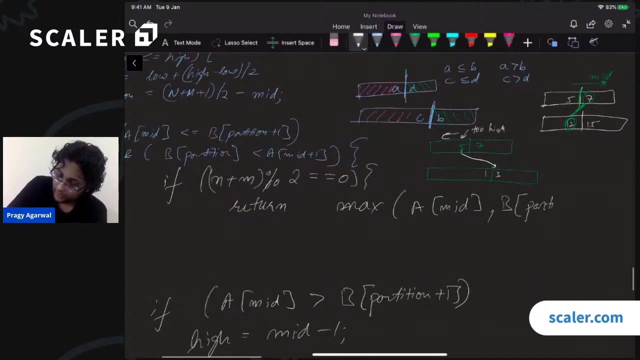 if n plus m mod 2 equals to, equals to 0. If it is, even then I have to return, return basically a of max. So basically I have to return. I have to return max of a of mid comma, b of partition, the max of these two. 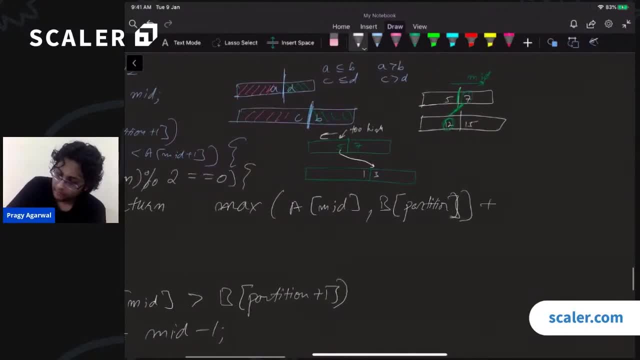 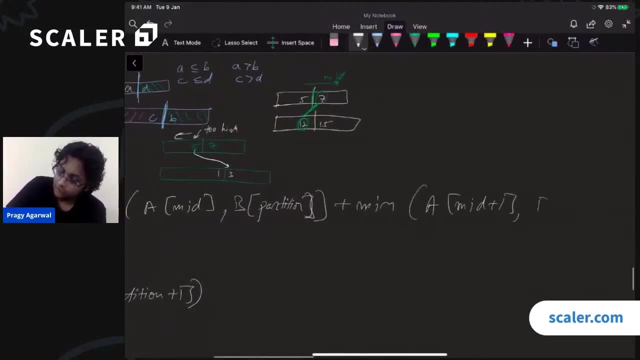 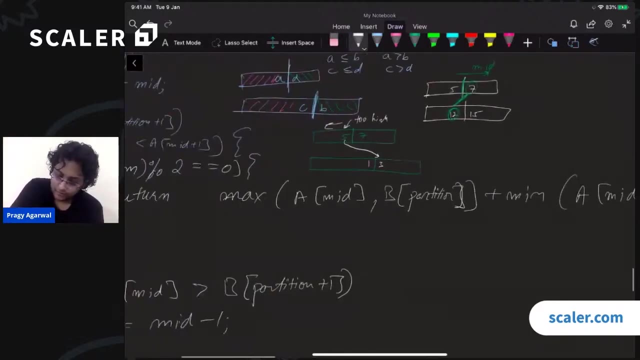 plus the minimum of, plus the minimum of a of mid, plus 1 comma b of partition minus 1 partition minus 1 right, And I have to take the average of these two. So I will add these two up and I will divide by 2.. 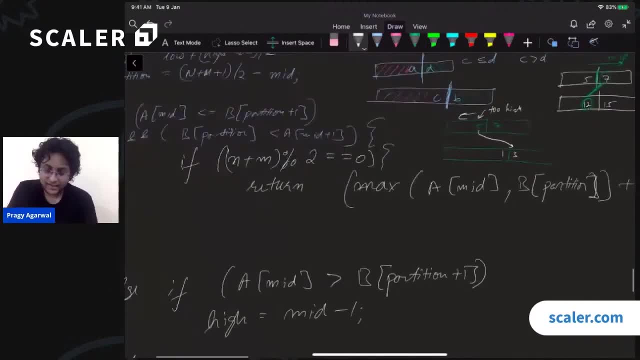 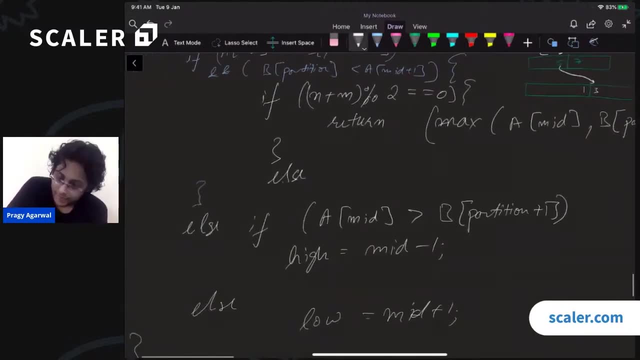 That is a very long line, But I hope that it makes sense. That is the case when my number of elements is even. On the other hand, if the number of elements is odd, then this is very simple. Then this is very simple. I simply return. 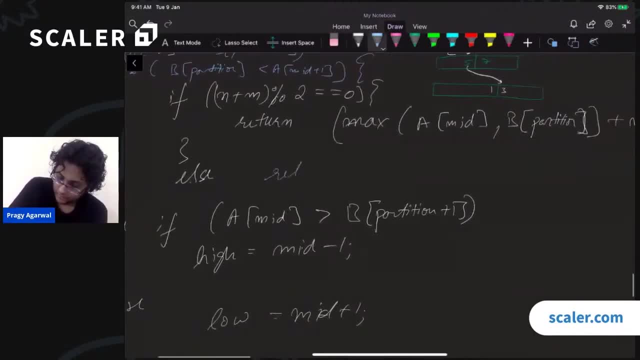 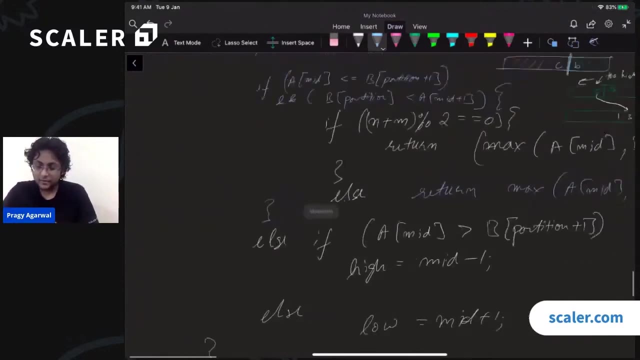 so I can simply return over here the max of a of mid and b of partition. Alright, I can simply return the max of a of mid of b of partition. So this is basically. this will basically be the code for finding the median of two arrays. 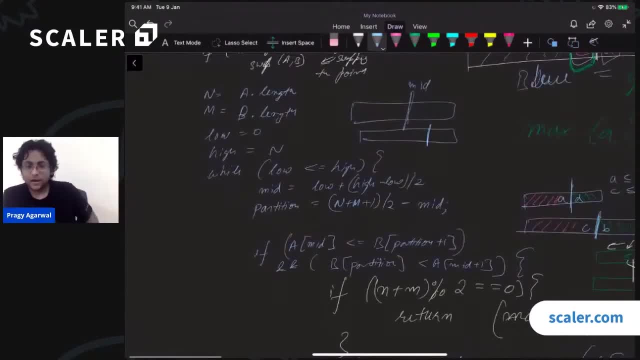 Now, there is one bug over here. There is one bug over here. Can someone catch that bug? This code is not entirely correct. There is one very, very crucial bug over here, And that bug is basically- let us suppose that I was searching in this array- 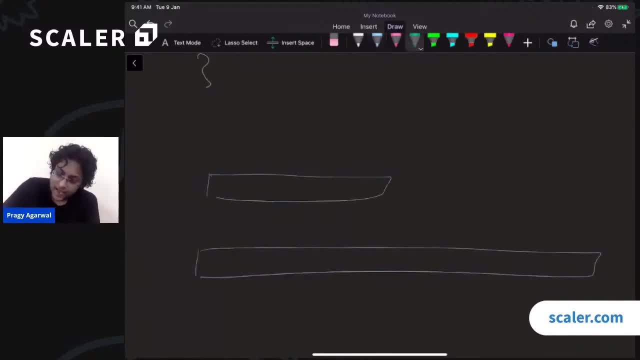 and I was searching in this array. Suppose that while searching this array, either my midpoint became n-1 or, if my midpoint became midpoint became 0. then what do I compare? I don't have anything to compare If my midpoint is this thing. 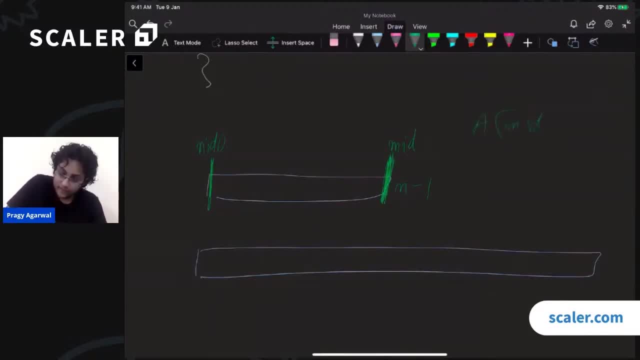 n-1, then I can't compare a of mid plus 1 with anything. I can't really compare a of mid plus 1 with anything, Yes or no. So for that to handle that, we can, very simply we can virtually append infinity and minus infinity. 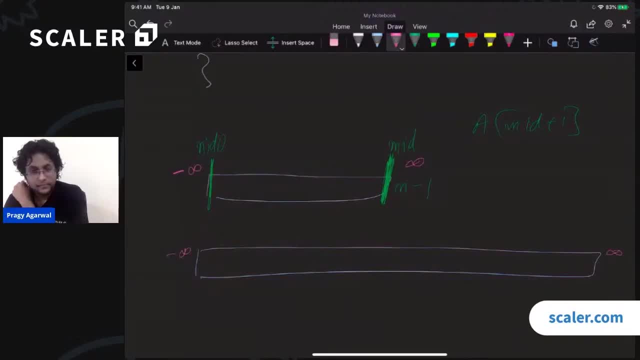 to the left and right of both the arrays. Alright, Yes, exactly. So then, even in that case, if the first array is only of size 1, so we will very quickly exhaust the mid. We will very quickly exhaust the mid, So to handle that situation. 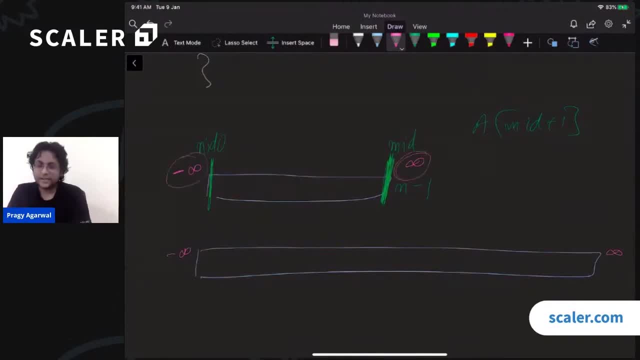 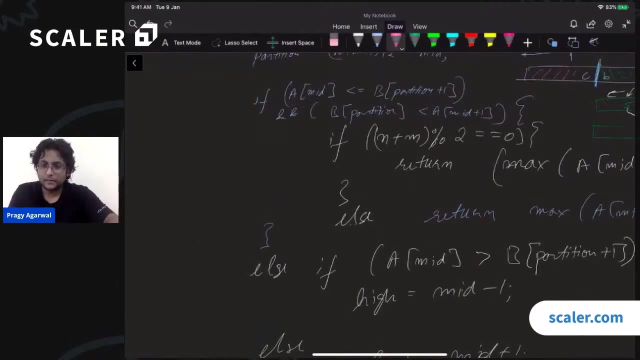 to handle that boundary case, we need to add infinity and minus infinity on the right and left side of both the arrays. Alright, You don't have to actually append it, You can treat it virtually. You can treat it virtually, Is that clear? 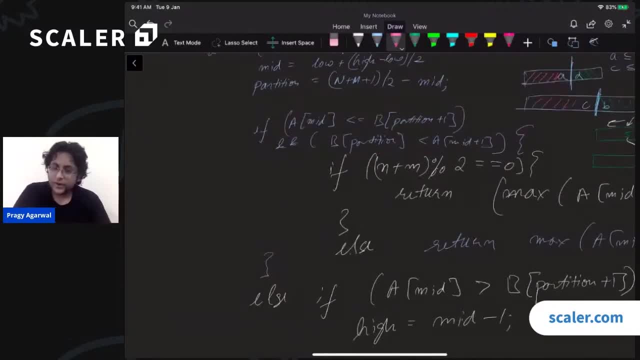 Yes, aaj kud zyada ho gaya. Well, I mean, I would recommend that you actually try and code this up, That you actually try and code this up. When you try and code this up, this will. So I understand that you won't be able to. 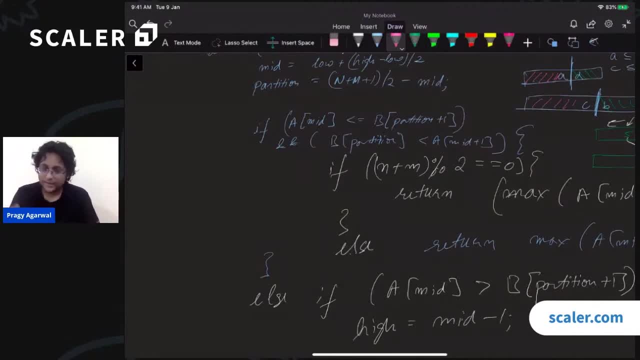 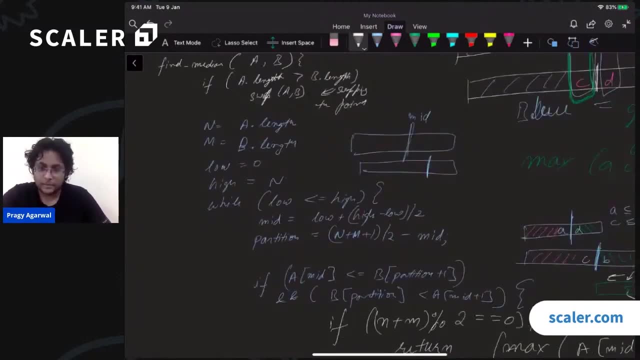 I mean, you will have to get practice on this, You will have to actually try and code this up to properly understand this Right, But I hope that the intuition was clear. The code might not be clear to you, but I hope that the intuition was clear. 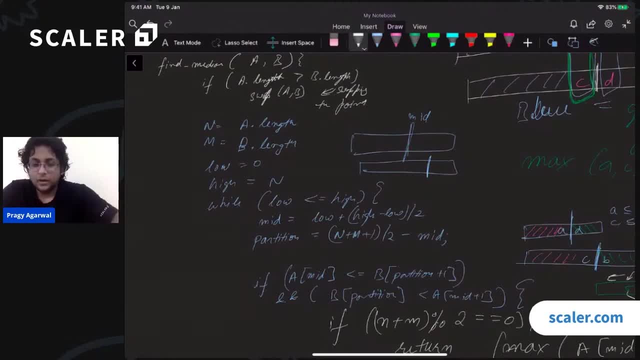 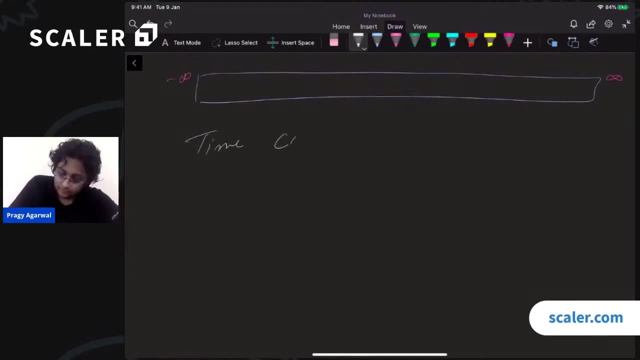 Right, Cool, So Now, what will be the time complexity of this overall algorithm? What will be the time complexity of this overall algorithm? Yes, So we are doing a binary search, right, We are doing a binary search over what? 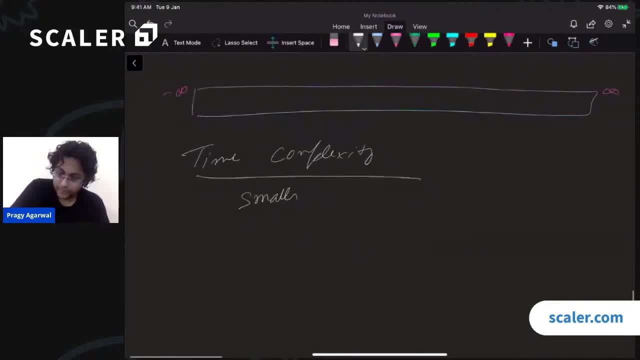 We are doing a binary search over the smaller array. We are doing a binary search over the smaller array. So what will be the time complexity? It will be order of. It will be order of min. So it will be order of log of min of. 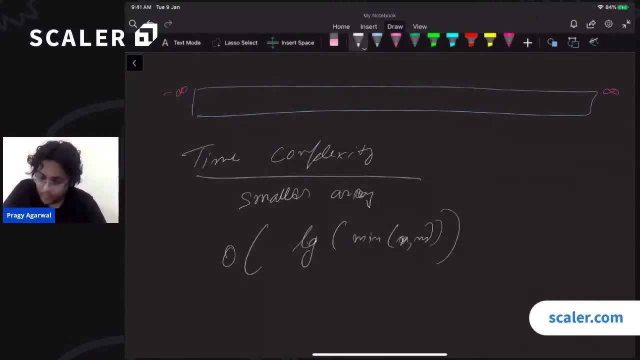 Right, It will be. order of log of min. Is that clear? Yes, There are a lot of edge cases over, So we always have to take care of the edge cases. I mean, the elegant solution is very elegant, but the groups are excellent. 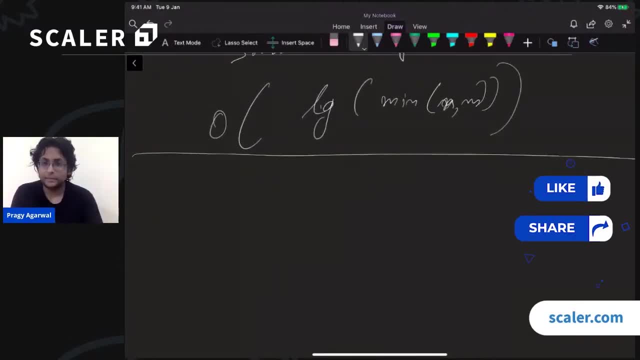 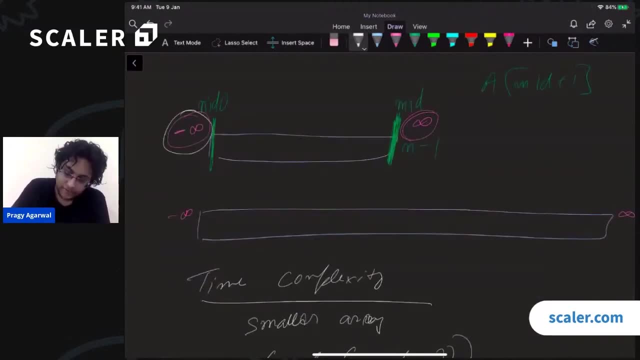 The code only becomes difficult because of all the edge cases that you have to handle. Alright, The chart says: how are the corner cases rectified? The corner cases can be rectified by just adding a minus infinity to the left of both the arrays and a plus infinity to the right of both the arrays. 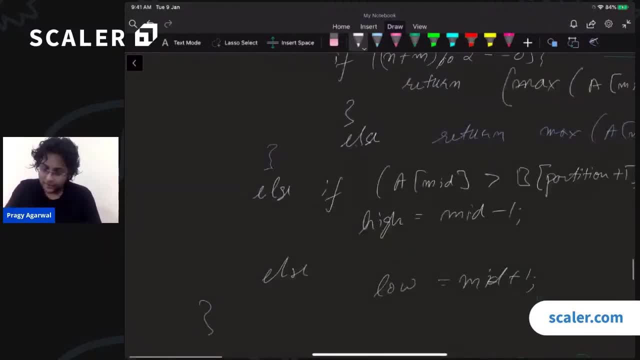 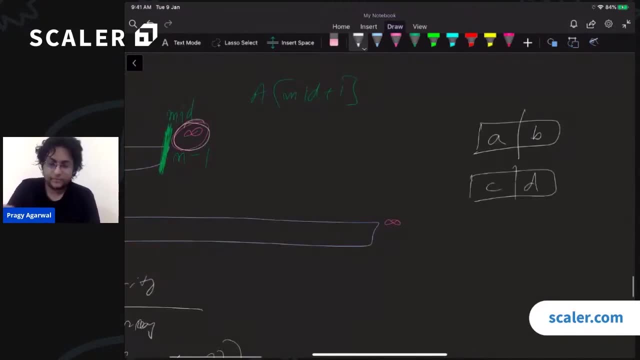 Alright, Basically, you can say that you have four values over here. You have four values over here. You have A, B and you have C, D. You have these four values over here. Well, what if this midpoint, what if this midpoint was equal to n minus 1?? 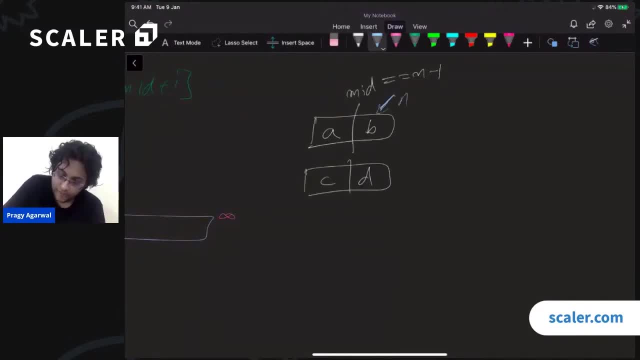 In that case? if that is the case, then there is no A of mid plus 1, right? There is no A of mid plus 1.. So what value should you consider instead of B? There is no B. B does not exist, right. 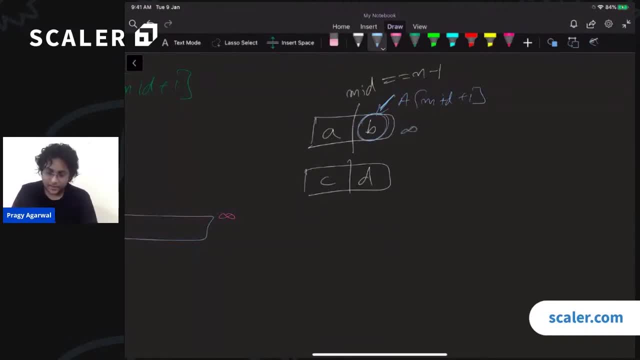 So what value should you consider instead of B? You should consider infinity. Similarly, this value over here, if this is partition, and this is partition plus 1, right. If there is no D element over here, then you should consider infinity in space. 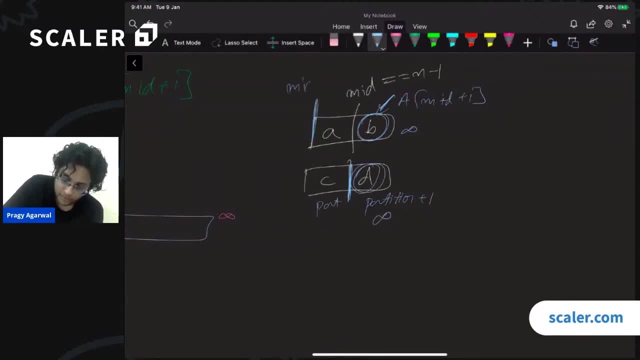 Similarly on the left-hand side. if mid is 0, then on the left-hand side you should consider minus infinity and same for partition. Is that clear? So once you actually try to code this, things will start making sense. 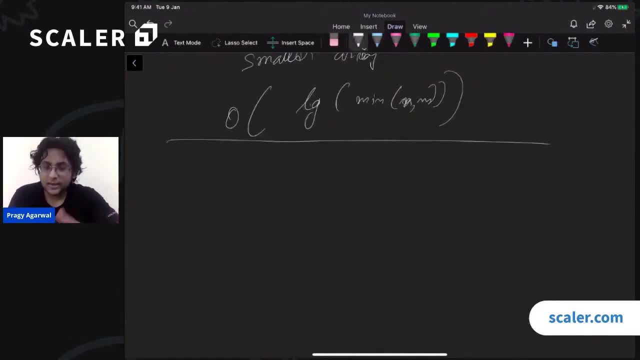 I don't want to give you the exact code right now, because then it will defeat the purpose of us trying to solve these questions. You actually have to code this yourself. struggle a little with the edge cases, and once you figure this out, things will become clear. 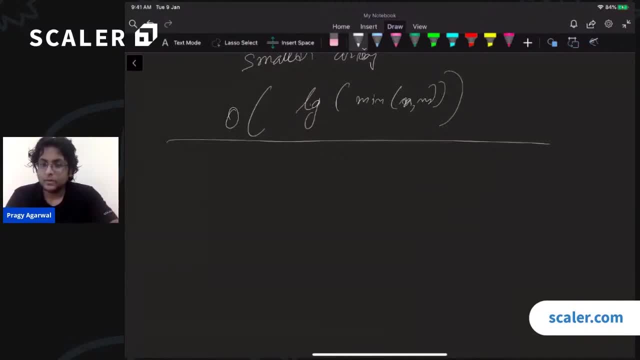 All right, Cool, So let us move on then to the next question, right? So the question was something like this. The question was something like this: that we have an unsorted array. That we have an unsorted array, right. 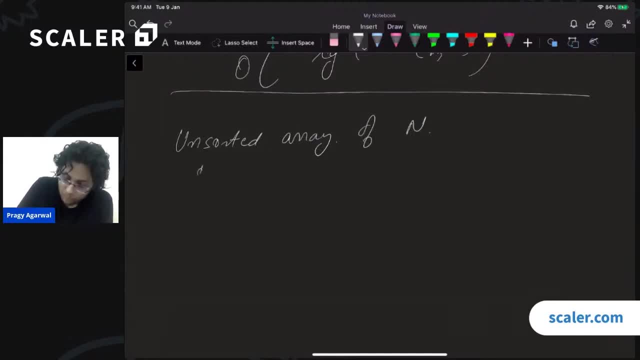 Of size n. right, And this array only has positive integers. Right, We have an unsorted array. We have an array of size n, and this array only has positive integers. Now, we have been given a value. We have been given a value- x- right. 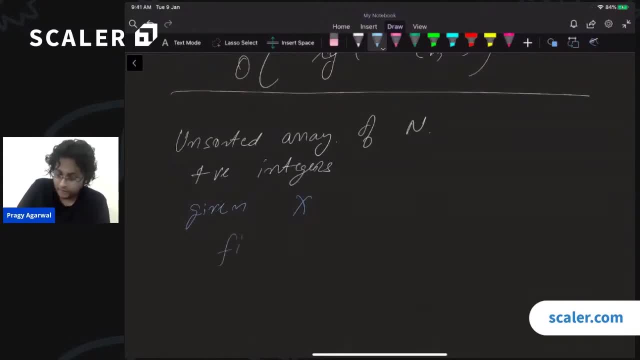 And we have to find the largest value of k, The largest value of k, such that no subarray, no subarray of length, k, k has sum greater than or equal to x, or let us say just sum greater than x. right, So that's a mouthful. 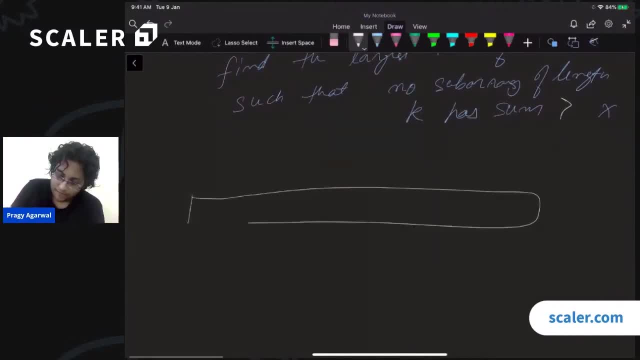 That's a mouthful. Basically, what we are saying is: suppose that we have some array with some elements. We have some array with some elements and we have been given a number: x equals to 10.. Let me also give this array. So this is a 1, 5, 6, 2, 0, 1, 3, 5.. 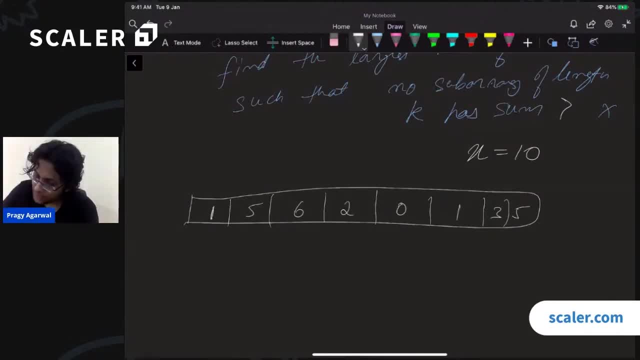 All right, Let us say this is my array And I have been given some x equals to let us make this a little smaller. Perhaps x equals to 6,. right Now we have to find the largest window size. K is the window size. 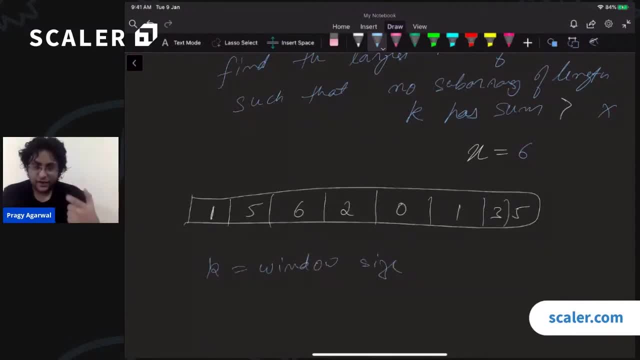 We have to find the largest window size, such that in that window there is no window. There is no window that sums up to greater than 6.. Right, There is no window that sums up to greater than 6.. So, in this case, what will be the answer? 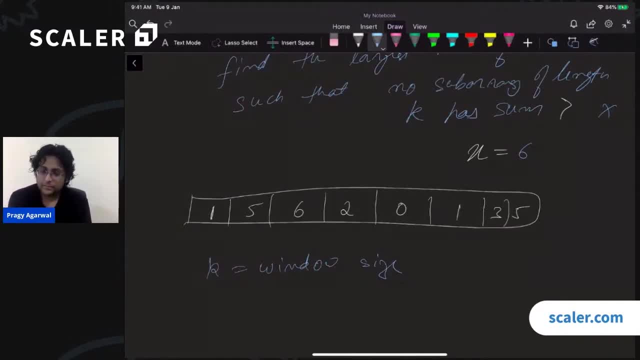 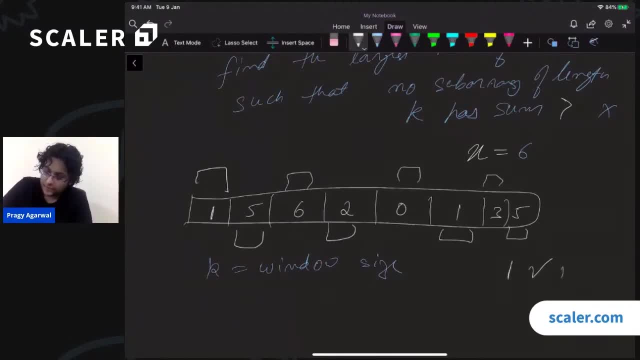 No right. So window of size 1 is valid. Window of size 1 is valid. Size 1 is valid, All right. On the other hand, if I have windows of size 1, this is valid, All right. 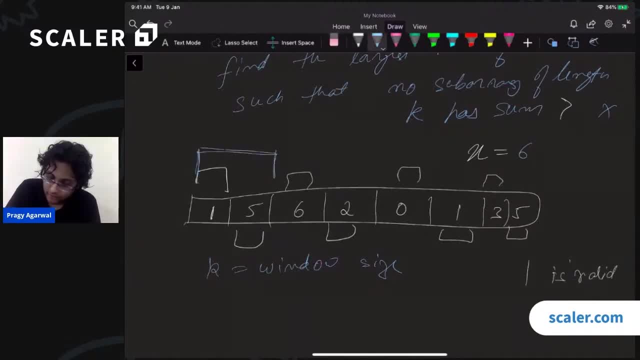 windows of size two. if I have windows of size two, let us say this window, right? What is the sum of this window? The sum of this window is six, right, So six is okay. What is the sum of the next window? Five plus six, The sum of this is 11.. Well, 11 is greater. 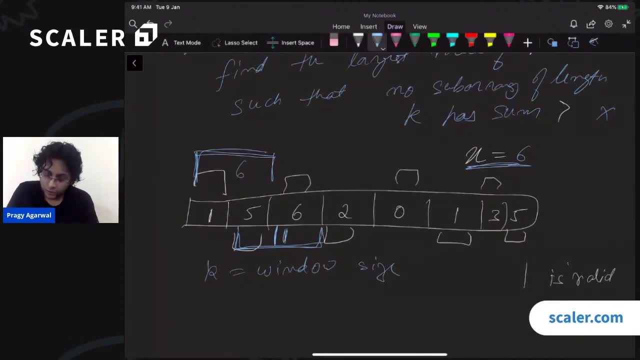 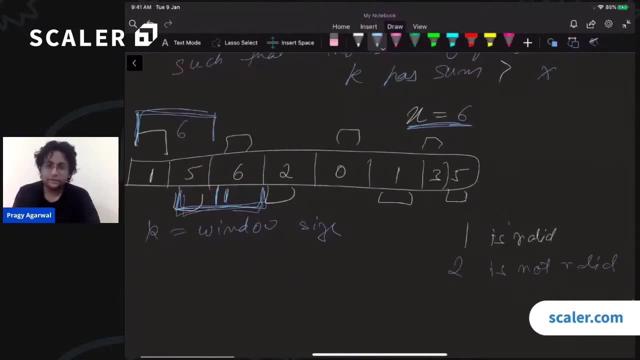 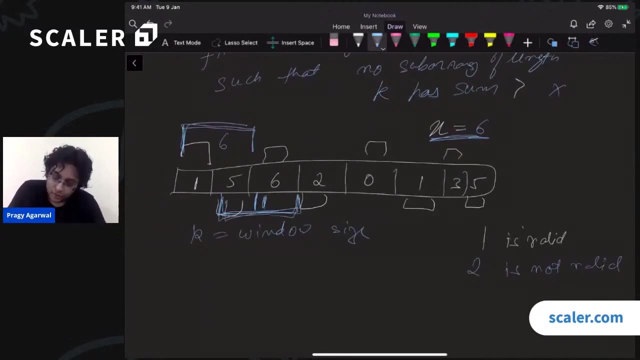 than six. right, 11 is greater than six. So this window is not okay. And because this window is not okay, the window of size two is not valid. Windows of size two are not valid. Is that clear? Okay, so we know, we know that a window of size two will give me. 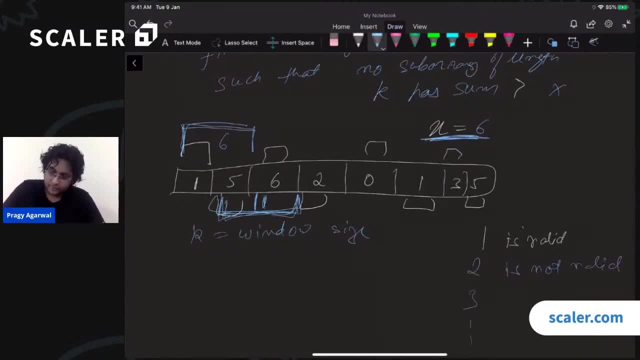 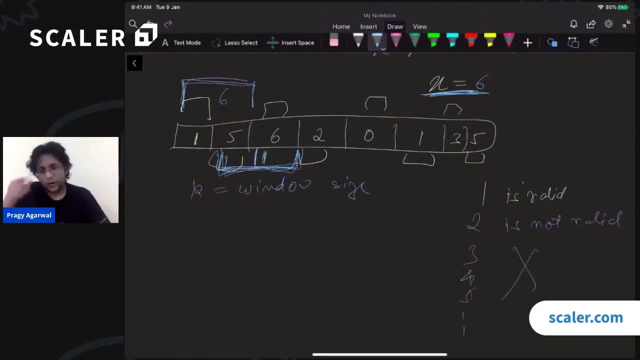 a sum greater than six. So should I try a window of size three or above? Should I try a window of size three, size four, size five, Yes or no? I should not try that right. There is no point in trying them. Does everyone agree? Yes, because we have to find the largest. 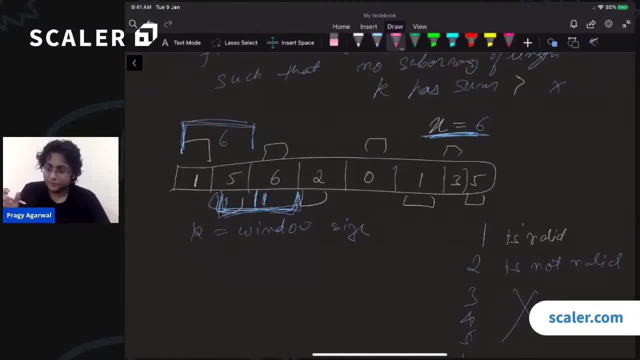 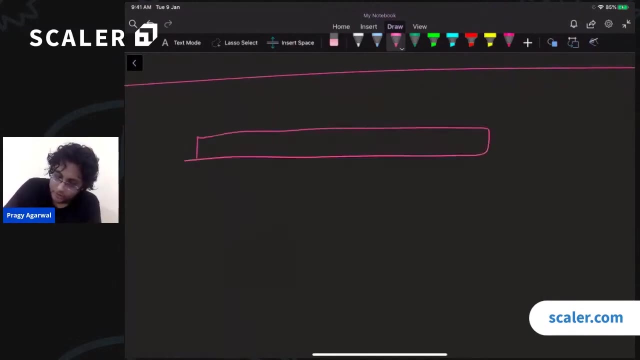 window such that the sum of any, the sum of any sub array of that size is greater than six, must be less than or equal to this summation value over here. Right, Let us take another example. perhaps Let us take another example. So let us take one more array. Suppose this: 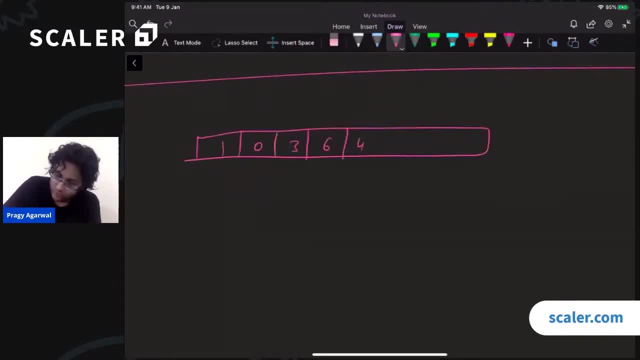 array is 10364270.. And let us say that x equals to 30.. Right, Let us say that x equals to 30. Now, what is the largest window? What is the largest value of k, such that no window of size k is greater than six? 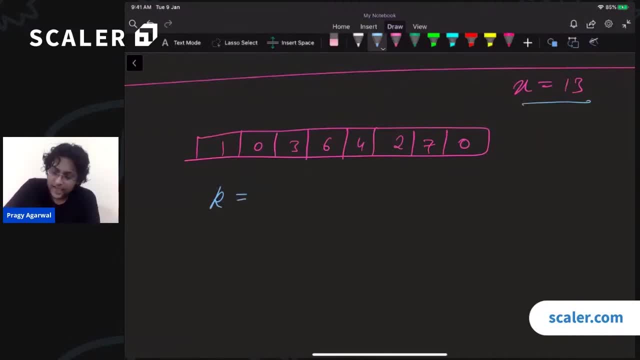 Right. So does k equals to one work? Does k equals to one work? If I have windows of size one, then is the sum going to be greater than 30? No right. So windows of size one, windows of size one- they all have some less than 30. It's a windows of size one- are valid. 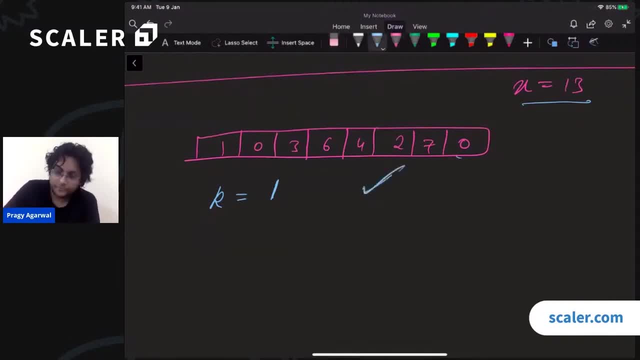 Every window of size one is valid. So size one is valid. This is valid, Right. What about windows of size two? Well, this has a sum of one. this has a sum of three. this has a sum of nine. this has: 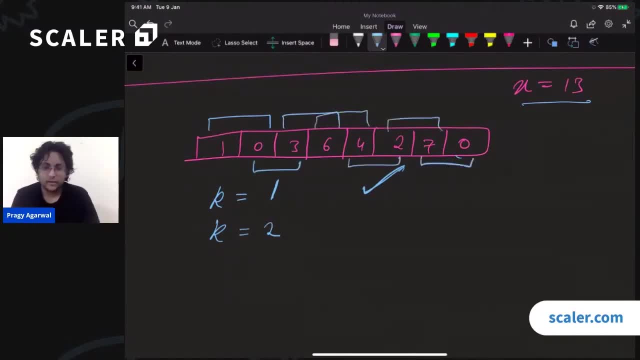 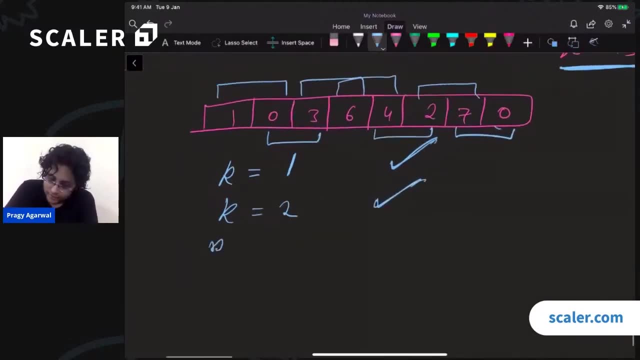 a sum of n. this is six, this is nine, this is seven. right? All the sums were less than or equal to 30. So windows of size two are also valid. All right, let us try increasing the window size. k equals to three. All right, now, what? what do my windows look like now? 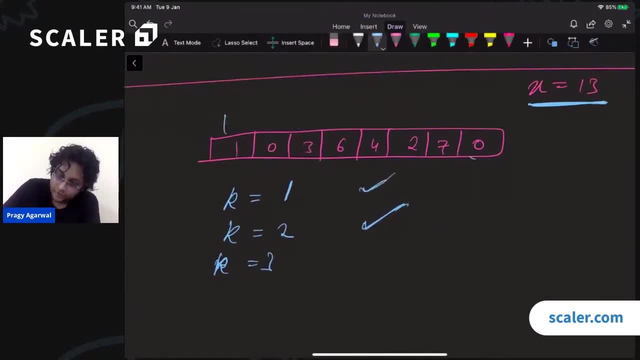 My windows are. so this is my window. first window. What is the sum of this? It is four. This is the second window. This is the third window. This is the third window. This is the fourth window. This has some 12.. This is the fifth window. What is the sum of this fifth window? This is still. 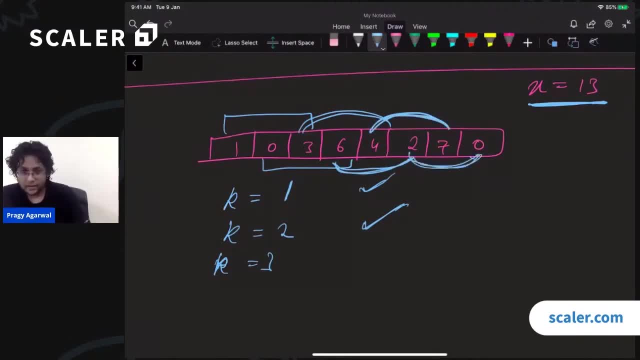 30. This is the last window. This has some nine, It's still. we see that window of size three is also valid. Is that your window of size three is also valid? Let us, let us try to increase it further. So let us try. k equals to four. All right, Now what is the size of? 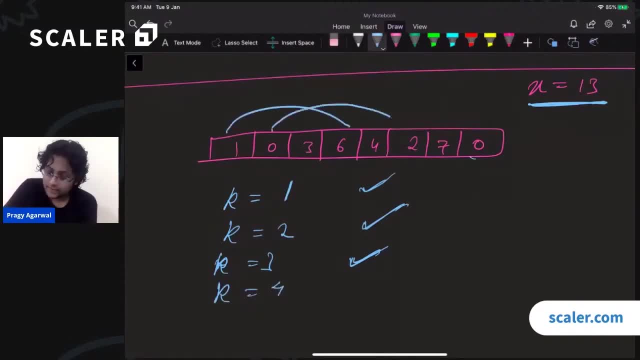 what is the sum of this 10?? What is the sum of this? That is, that is 15, the sum of this particular window is 15, and 15 is already greater than. so windows of size for not valid. Is that clear? Because 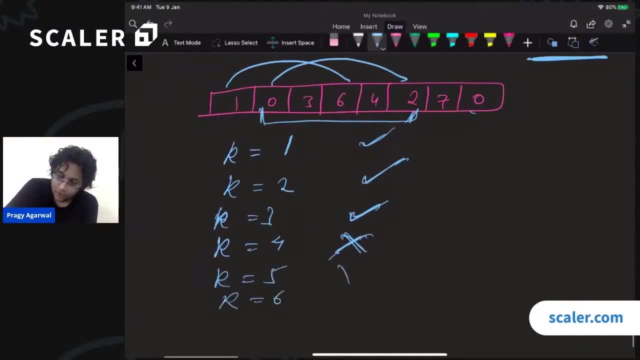 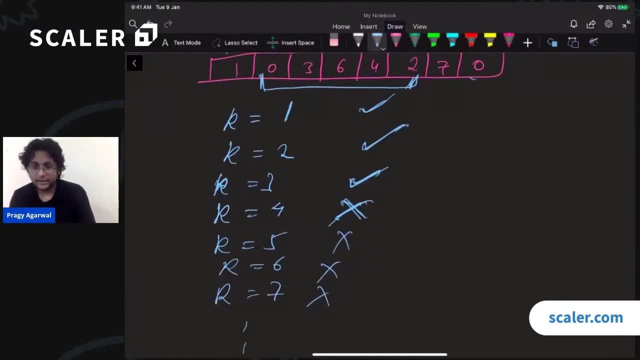 windows of size four are not valid. Windows of size 5, Windows of size 6 will also not be valid. Is that clear, All right, All these will not be valid. Yes, is that clear, All So? if this is my array, if this is the input array and this is the value of x that has, 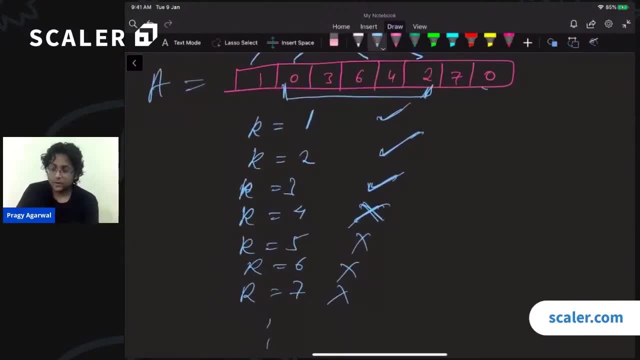 been given to you. then what value of k should you return? What value of k should we return? We should return k equals to 3, because we have to return the largest size of window, so that no window of that size, no window of that size has some greater than x. 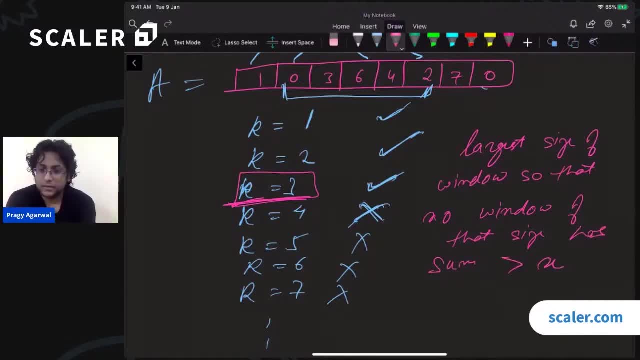 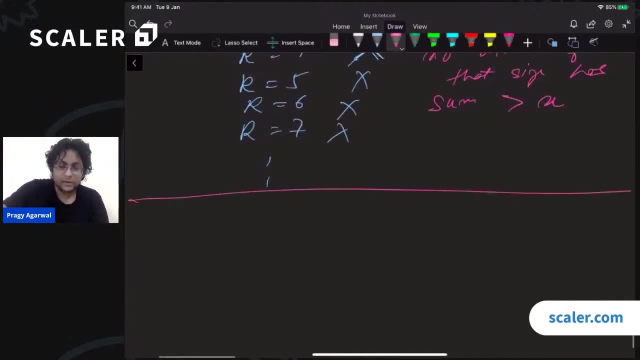 Is the question now clear? Yes, is the question now clear? All right, So how can we approach this particular question? How can we approach this particular question? So, guys, whenever you, whenever you are, whenever you come across a new question, don't forget. 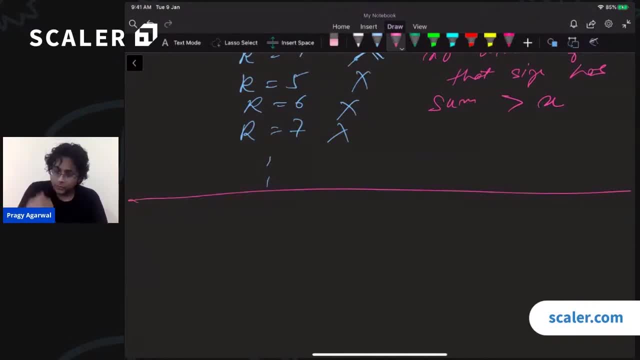 don't try to come up with the optimized approach right away. come up with the most brute force approach First. try to solve the question. Once you have solved the question, then you can try to optimize it, Because some solution, some solution that works but is slow. 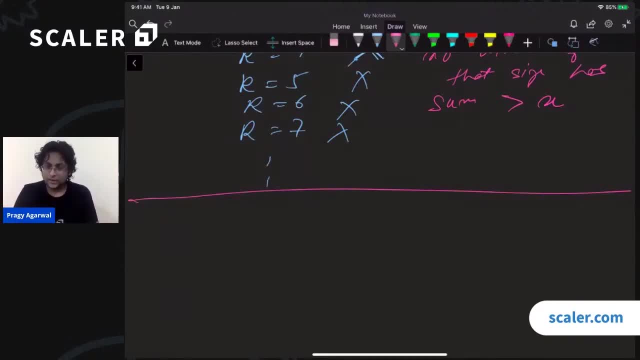 Some solution is always better than a fast solution that you never find. Having some solution at least is better. Let's think about brute force approach first. Yes, So what can we do? All right, So let us look at two questions. Let us look at two questions. 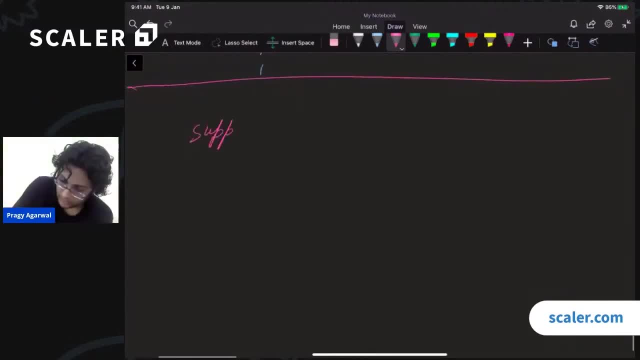 Suppose I have a guess right. Suppose I have a guess, a guess for k, Right? Suppose I say that k equals to, let's say, 5.. Suppose I have this array, Yes, And I have been given a value of x. 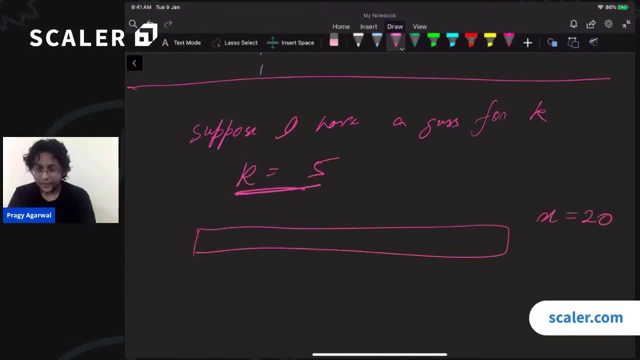 Let's say 20. And I am guessing that k equals to 5.. Then how can I verify, How can I check it? How can I check it? I have to consider every possible window of size 5.. I have to consider every possible window of size 5.. 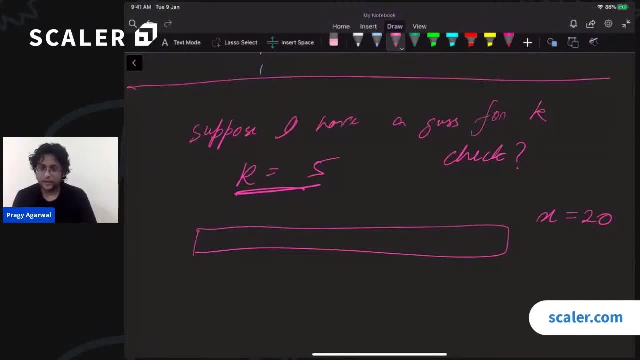 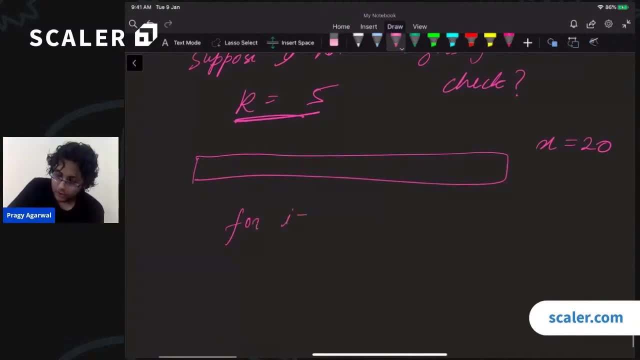 So how can I do that? How can I do that? I can either do two nested loops, So I can either say: for i equals to 0 all the way till n minus 5 minus 1.. For j equals to 0 till 5 minus 1.. 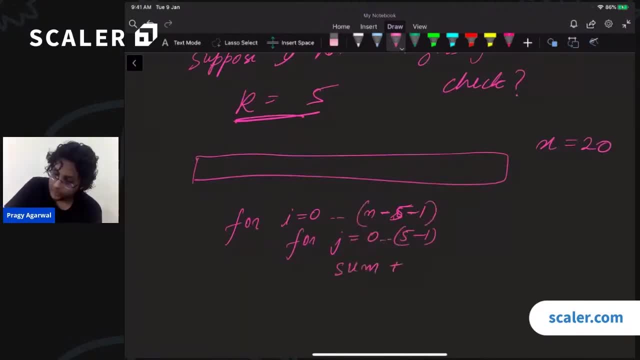 And then I can say: sum plus equals to a of j, a of i plus j, a of i plus j, And initially sum equals to 0.. So, doing this, what will this do? This will give me so sorry over here. 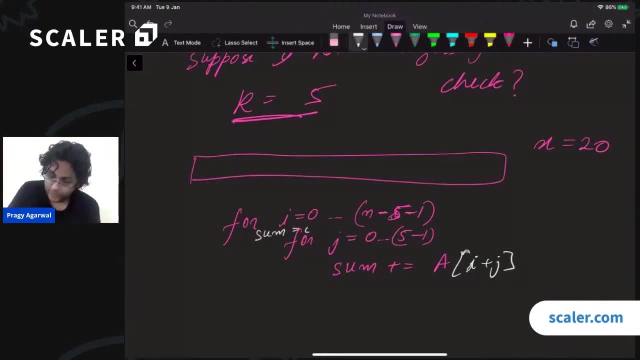 I will have to say: sum equals to 0 over here, Sum equals to 0 over here. So, basically, after this inner loop, in each iteration of this inner loop, I will have the sum of one window. I will have the sum of one window. 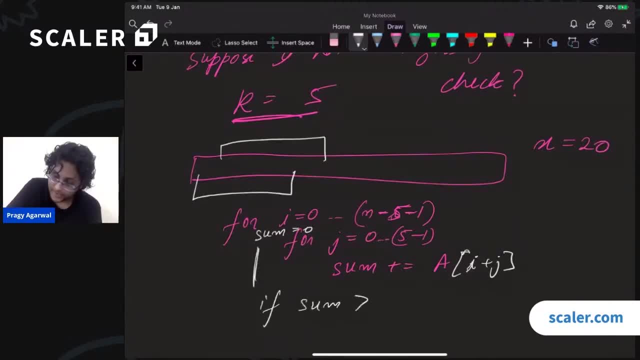 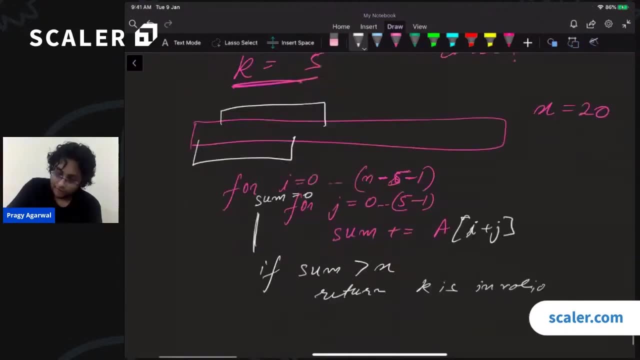 Again and again. So I will have to check if sum is. If sum is greater than x, then return that window size is invalid, right. K is invalid Right. After this entire thing is complete, I can say that k is valid. 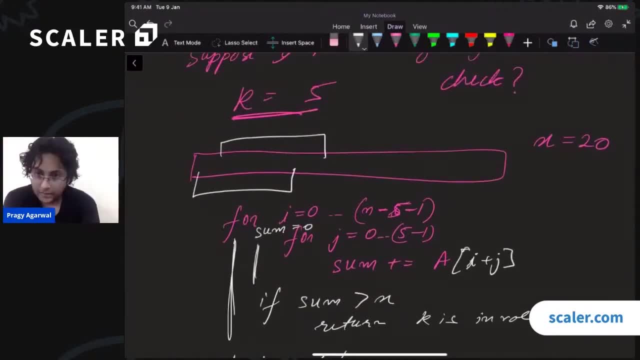 Right. So, given a window size k, this is how I can check it, Yes or no? That seems like a very, very difficult approach to do, right? So can we simplify this a little bit? Can we simplify this a little bit? 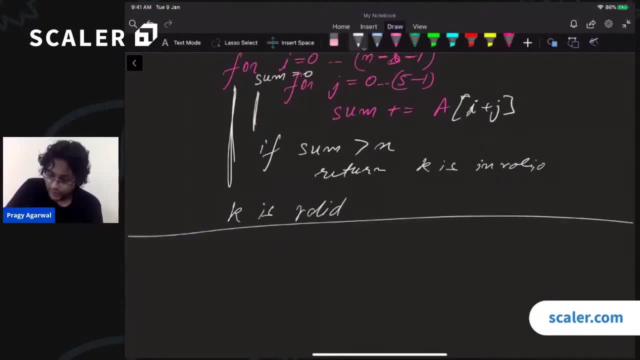 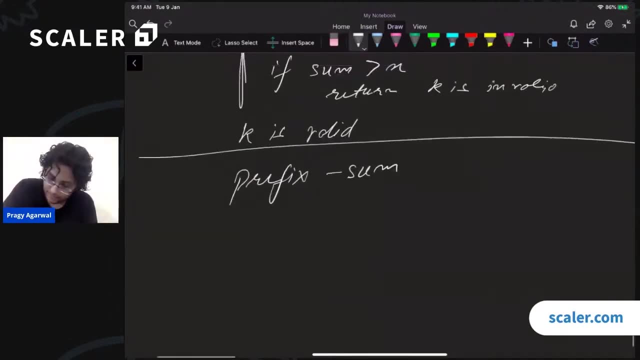 How can we do that? So are you guys aware of prefix sum? Are you guys aware of prefix sum? Suppose that this is my array. Suppose that this is my array and I want to find the sum from some start location to some end location. 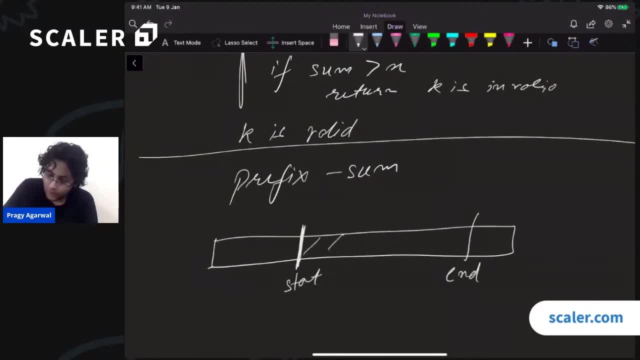 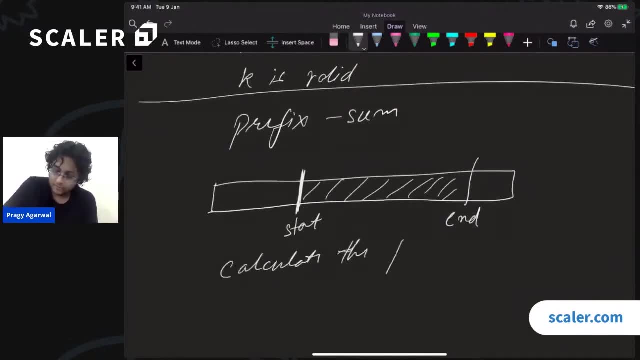 If I want to do many, many queries of such form that find the sum of all these different elements, then how can I do that efficiently? I can calculate. I can calculate the prefix sum, The prefix sum of the array right. Let us say that this is the array a, then the prefix sum of array a will be p of a. 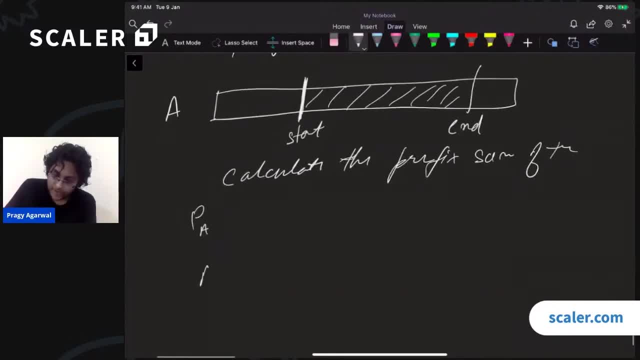 Yes. Now if I were to ask, if I were to tell you to calculate a of i plus a of i plus 1, or plus a of i plus 2 plus all the way to a of j, then how can you express this in the form of prefix sum? 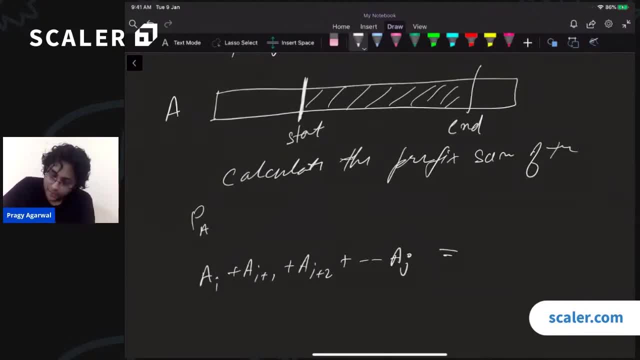 How can you express this in the form of prefix sum? Well, this is simply equal to what p of j, p of j, p of j minus p of i minus 1.. Yes or no? Is that clear, Yes or no, guys? 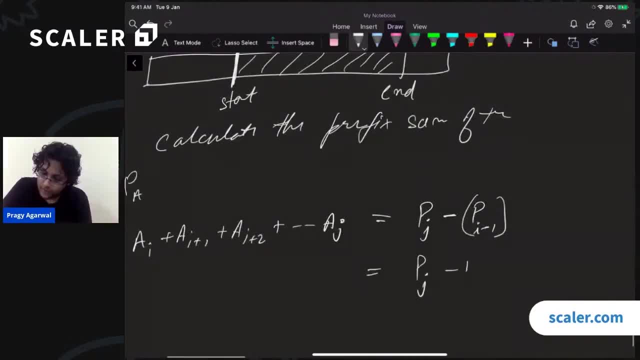 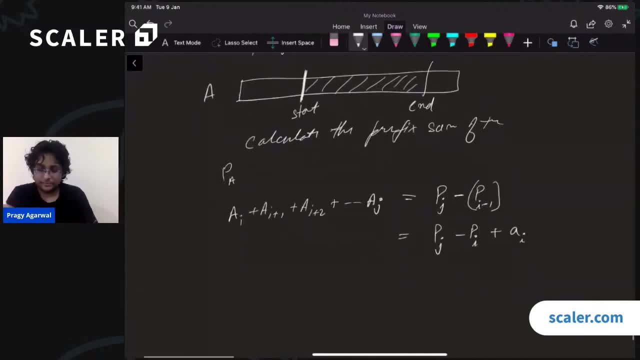 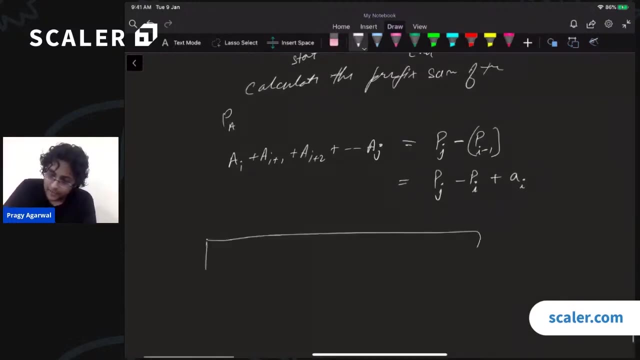 Alternatively, you can also write this as p of j minus p of i plus a of i. You can also rewrite this as this: They are the same thing, All right. So once I have this prefix sum, Once I have this prefix sum, if I tell you that, find me the size of, find me the size of window of size 5, starting from this location, i. 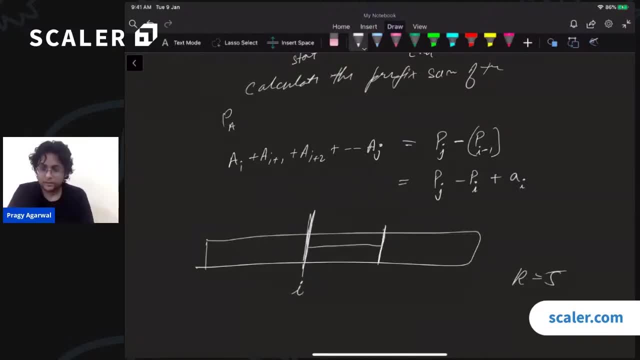 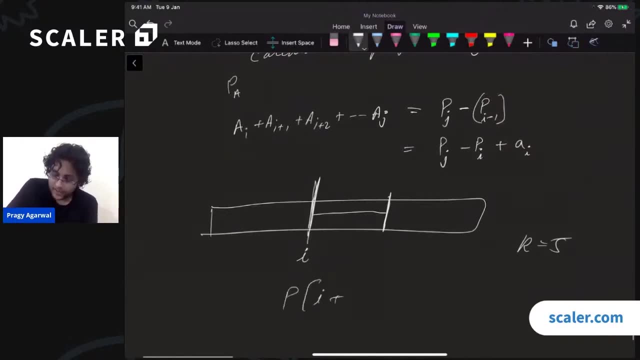 If I ask you to find the sum of this window, then how can you do that? How can you do that? You can very simply do what You can simply do: prefix sum of i plus k minus. prefix sum of i minus 1.. 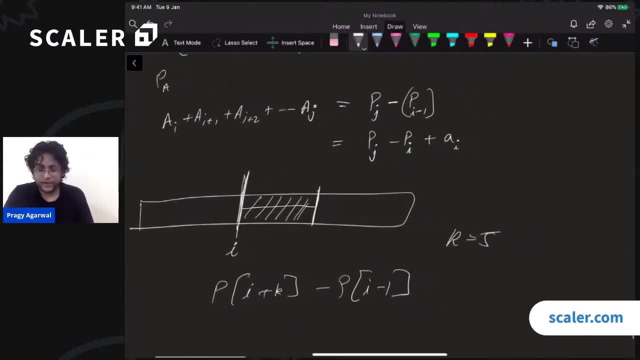 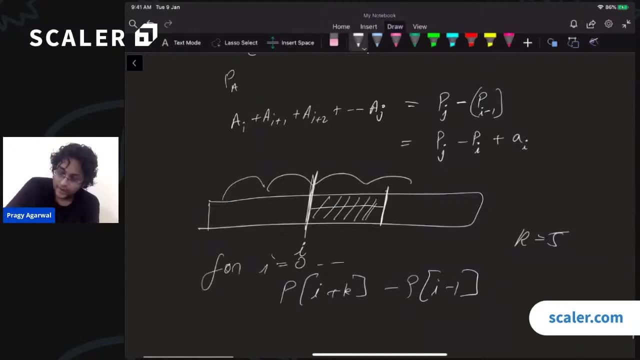 Yes or no. This will give you the sum of this window Right And to go over, To go over all possible windows, you can just write a loop for i equals to 0, all the way till n Right, n minus k, basically. 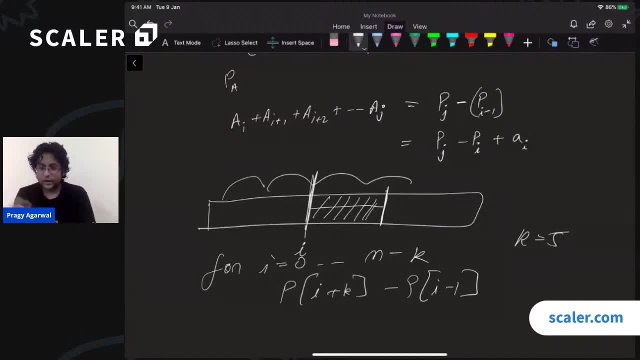 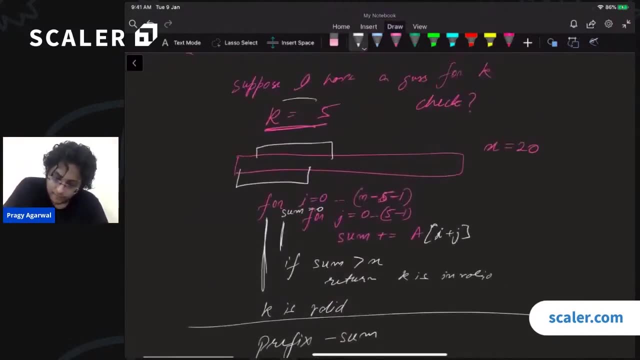 Yes, So that is the first thing that we can do to make our sliding window calculation a little simpler. We can store the prefix sum, But the thing still comes that, all right, given a value of k, given a value of k, I can check if it is correct or not. 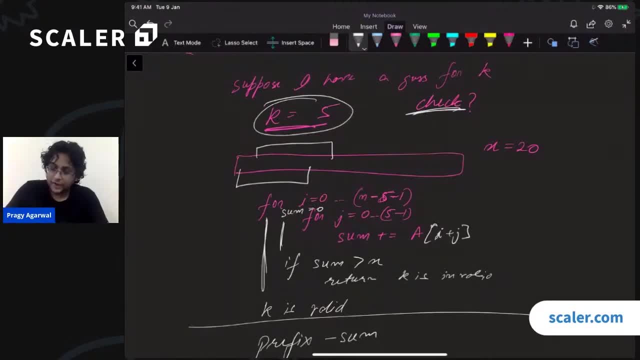 But how do I find the value of k? How do I find the value of k Currently? the approach that I have, Currently, the approach that I have, The approach that I have is start from k equals to 1 and try increasing it. 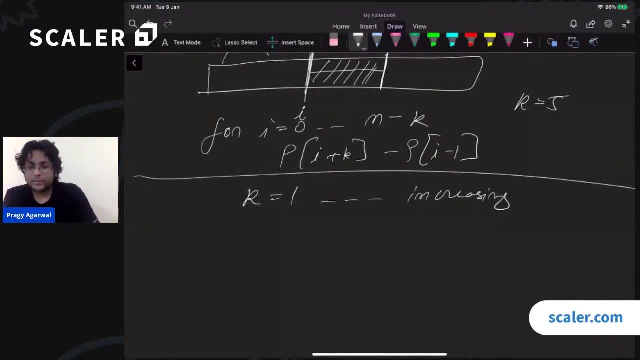 Try increasing it one by one, Right? If I do that, then what will be my time complexity? What will be my time complexity? I will have a loop of, I will have a loop for k. This will run for order of n time. 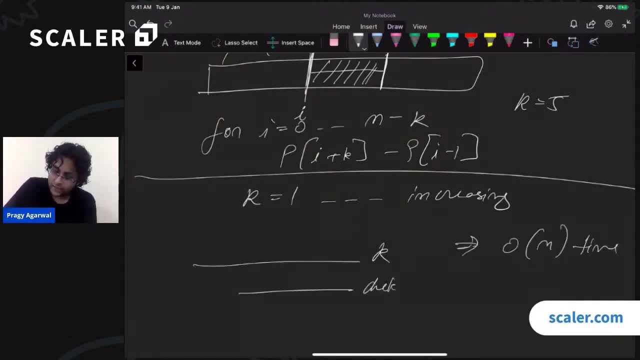 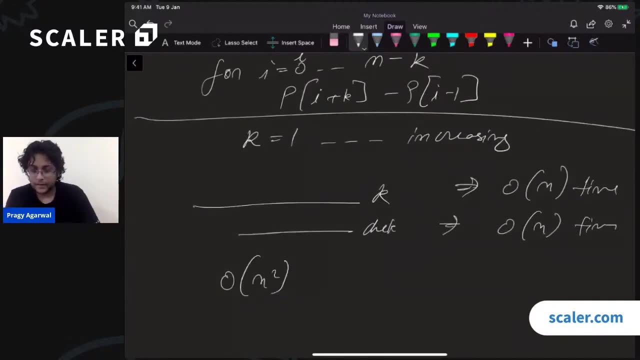 Right, Then I will have a loop for checking, Checking k. This will also run order of n time, So my total time complexity will be order of n squared. Yes, Of course I also have to consider the complexity of the prefix. 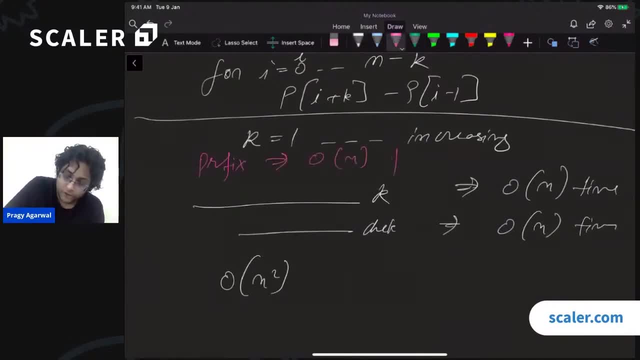 But calculating the prefix sum is just order of n, pre-competition, Pre-competition. So this is actually order of n squared plus n, which is just order of n squared Right. This is my naive, this is my brute force, brute force. 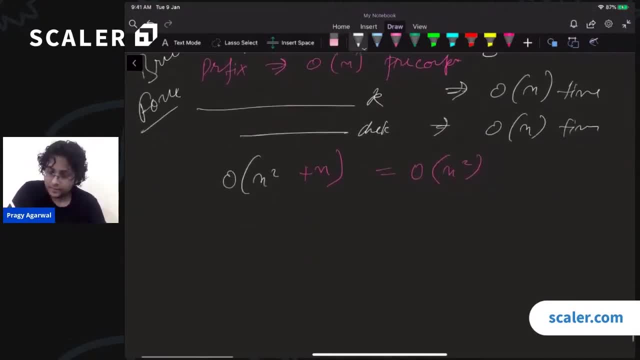 I will go ahead. All right, Can we, can we improve this? Can we improve this? So right, Teju says that we can use binary search. Right, But what should we binary search over? Right, Teju? what should we really binary search over? 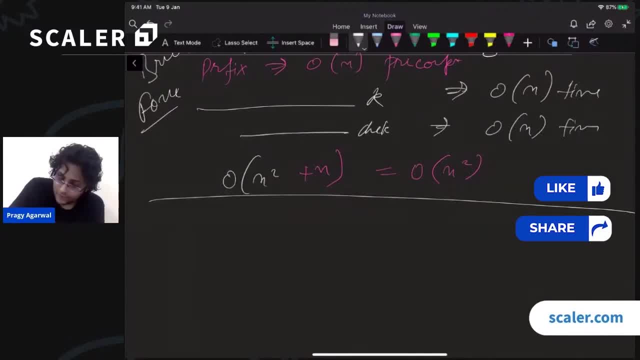 Yes, so Prakash says that we can binary search for the value of k. So we are going to binary search, Binary search for the value of k itself, Right, So how? so what is the minimum possible value of k? 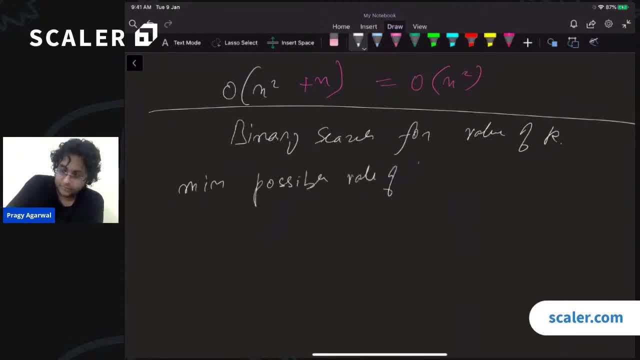 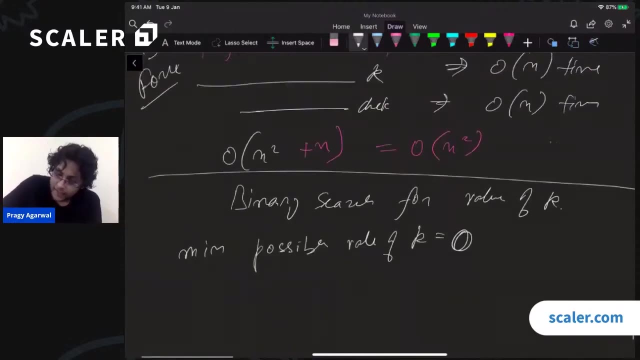 What is the minimum possible value of k? What is that? What is that? What is the minimum possible value of k? guys, It is 0.. Right, It is 0.. Basically, if some a of i, if some a of i itself, is greater than x, then I can't have a window. 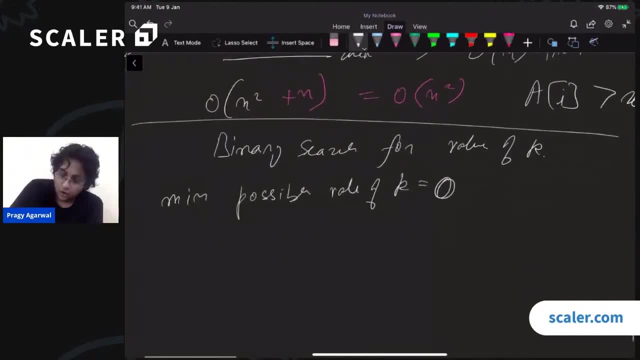 even of size 1.. Right, In that case the value of k will be 0.. On the other hand, what is the maximum possible value of k? Possible value of k? That is n. Right, If I take the entire, if the sum of the entire array is still less than x, then that is the. 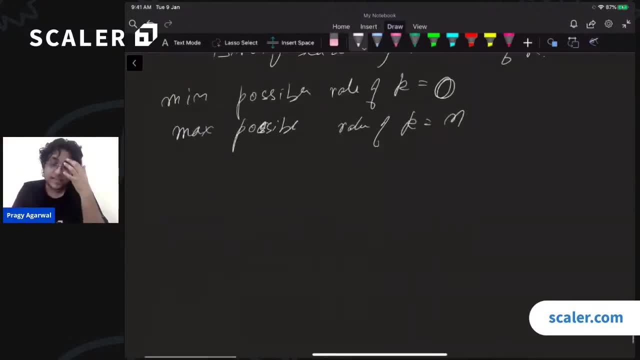 maximum possible value of k. So what I have to do is I have to binary search in this search box. I have to binary search in this search box So I can say: low equals to 0, high equals to n, While low is less than equal to high. 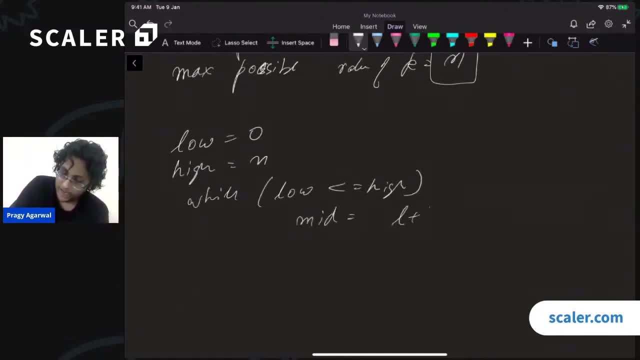 Right, I will say: mid equals to low plus high by 2. Right, All right. Now, once I have the mid, what should I do? What should I do? I should check check window of size mid. Right, I should check window of size mid. and I will have another function over here. 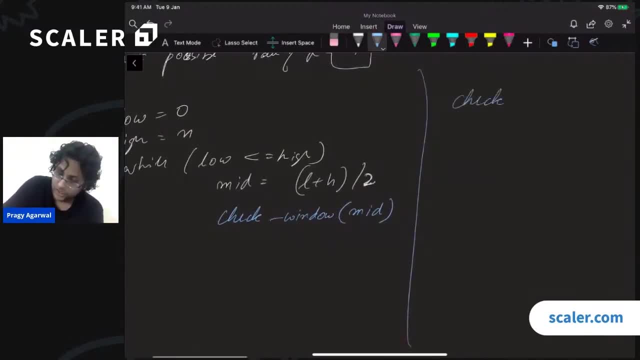 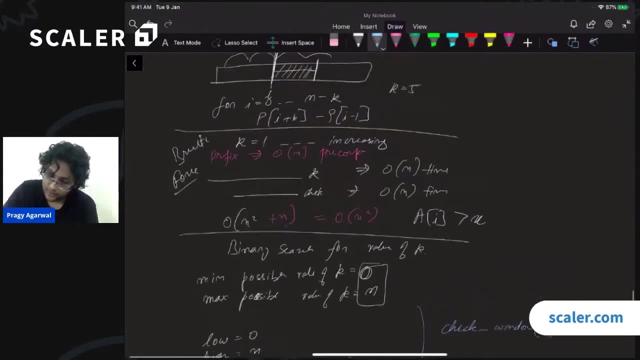 I will have another function over here: check window. check window: right, That takes a value of k and it turns true or false. Right, This check window is going to do exactly this. This check window is going to do exactly this. 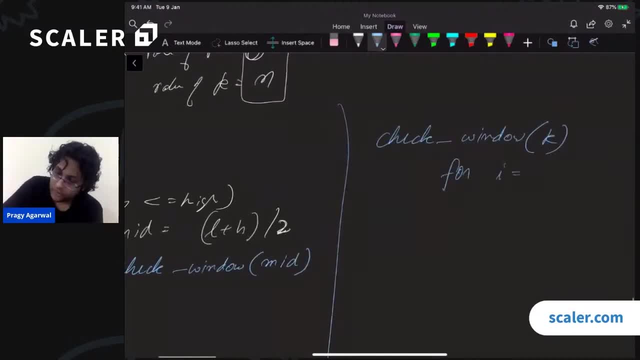 So it is going to loop. It is going to say: for i equals to 0 or the weight is n minus k. Right If the prefix sum of i plus k minus prefix sum of i minus 1.. Right If this is greater than x. if any of this sum is greater than x, then return false. 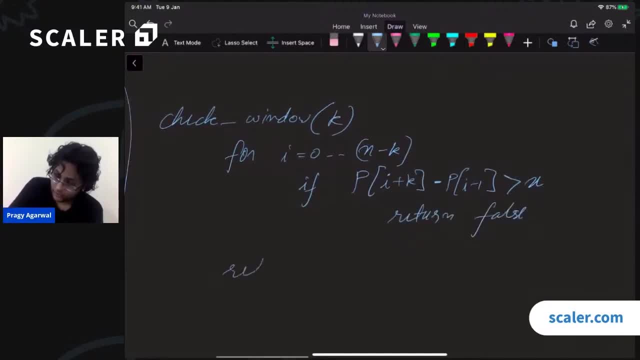 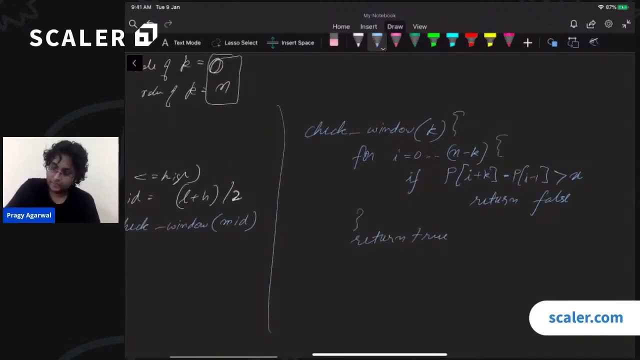 Return false Right. Otherwise, return true Right. If all these windows are valid, then return true Right. This is the check window functionality, Right? Is that clear guys? Cool. So we have a function for check window now. 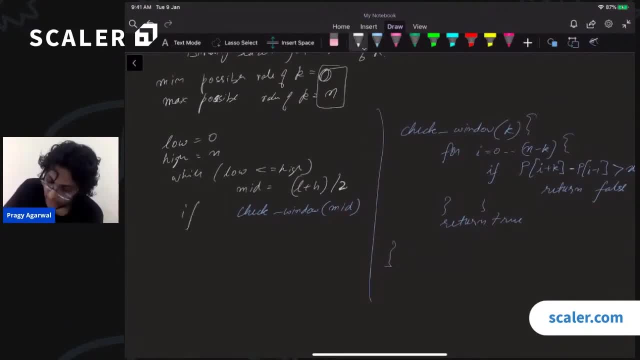 So what can we see over here? What can we see over here? So if I check window, if I check window of mid, and this comes out to be true, if check window of mid comes out to be true, then what can I say? 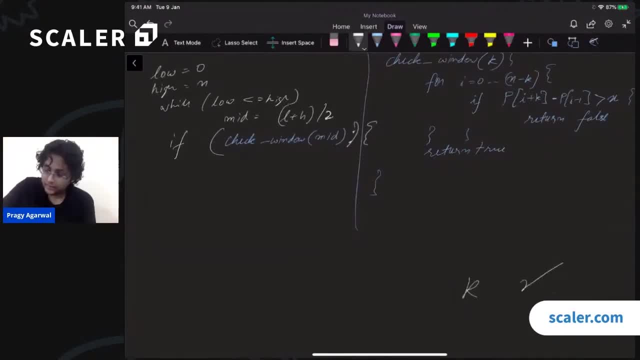 If a window of size k works, then can I return this. If a window of size k works, then can I return that window size as the final answer Yes or no? No, I cannot, Because, yes, this works, but this might not be the largest value that works. 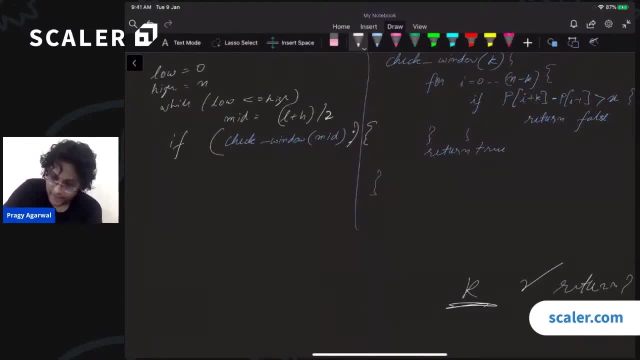 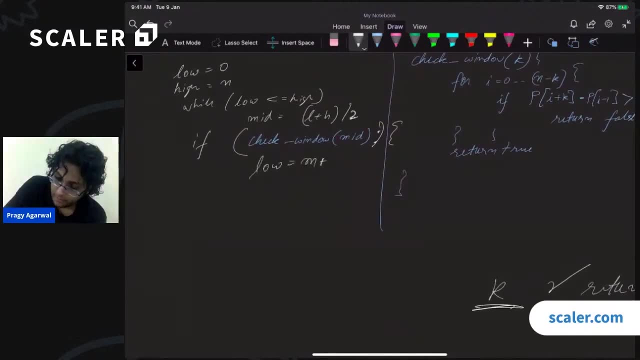 I have to find the largest value that works Right. So if this is the case, then I have to increase my low. So I will say low equals to mid plus 1.. Right: Mid plus 1.. On the other hand, if this does not work, then I have to decrease my value of k. 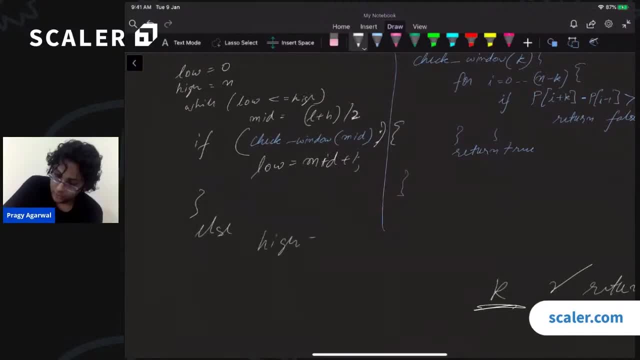 Right. So else I will say: high equals to mid minus 1.. Right, High equals to mid minus 1.. Well, when do we stop? When do we stop? When do we stop? So we can either stop when this loop exits or we can explicitly check. 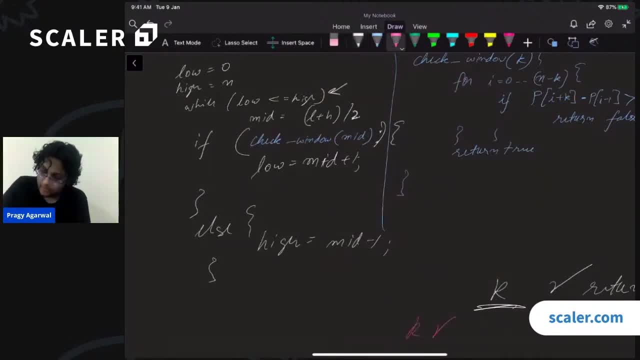 We can explicitly check that k works, but k plus 1 does not work, Right? If that is the case, then we can simply return. Is that clear? Even if we do not do that, that is fine, Because this loop will automatically take care. 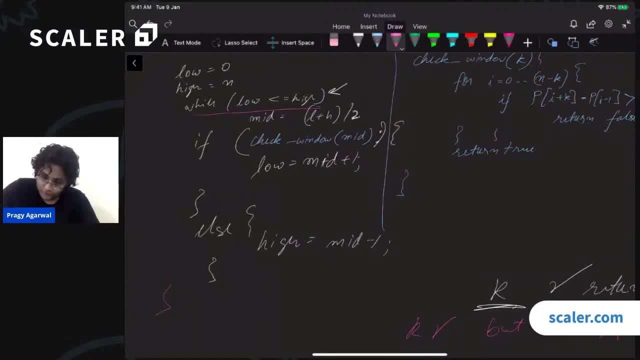 Is that clear? So we will return when we find a position of k which works but the other one does not. If we find an immediate higher position right, k works but k plus 1 does not work, That will be our correct answer. 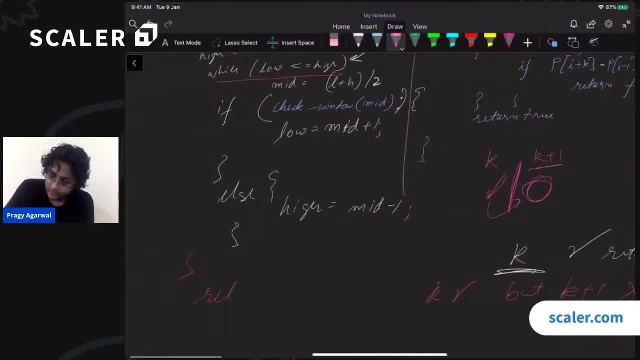 Is that clear guys? So after this loop, after this while loop is over, I can simply return. I can simply return what? What can I return? So this will exit when low will become greater than high. Okay, 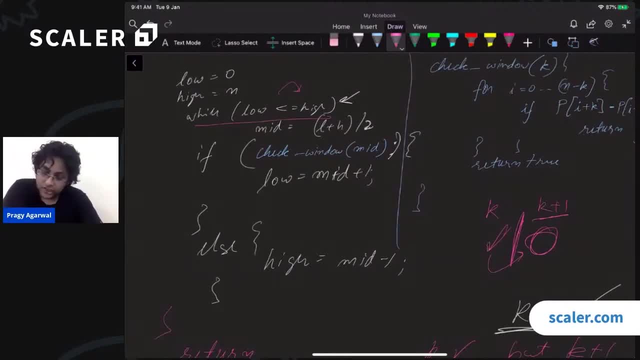 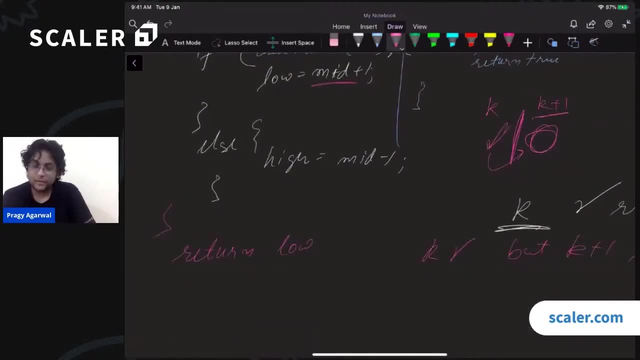 Low will become greater than high. How will it become greater than high When I would just do, low equals to mid plus 1.. So I can just return low over here, Right, I can just return low over here, and that will be my size of the window. 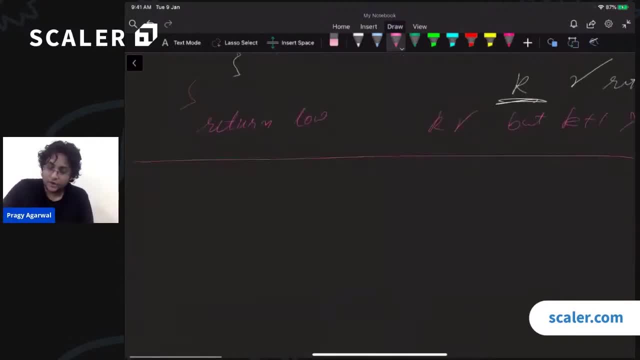 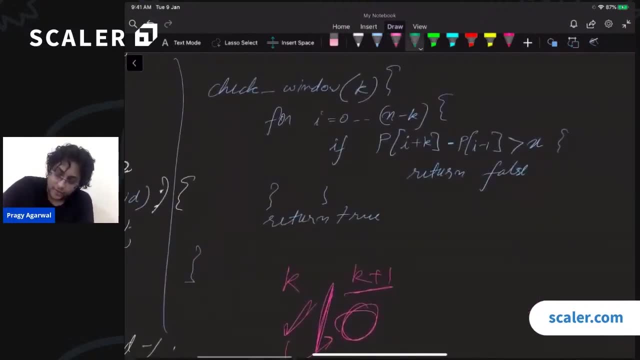 All right, Cool. So what will be the overall time complexity of this algorithm? What will be the overall time complexity of this algorithm? So let us take this step by step. How much time does check window take? How much time does one call one function call one function call to check window take? 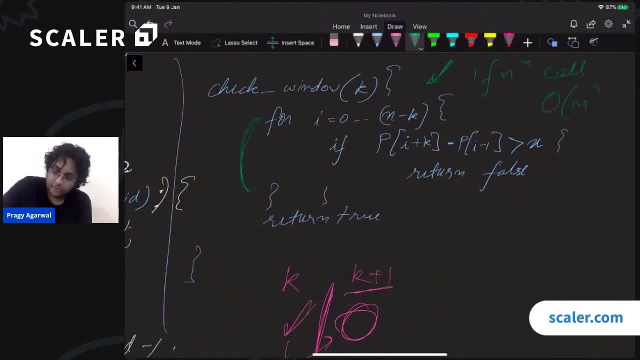 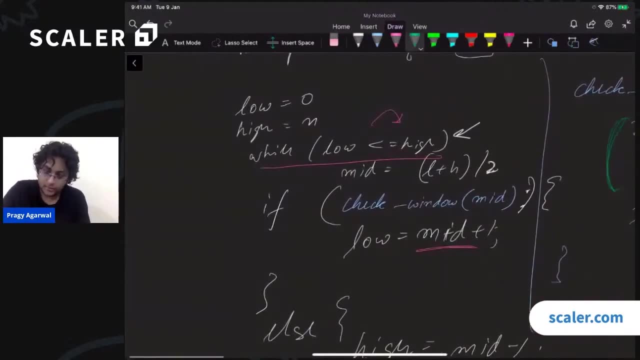 This is simply a for loop Right. This takes order of n time per call. Right, This takes order of n time per call. Well, what about this thing? This is log n search, Right? This is log n search, But inside this log n search, we are doing this order of n call every time. 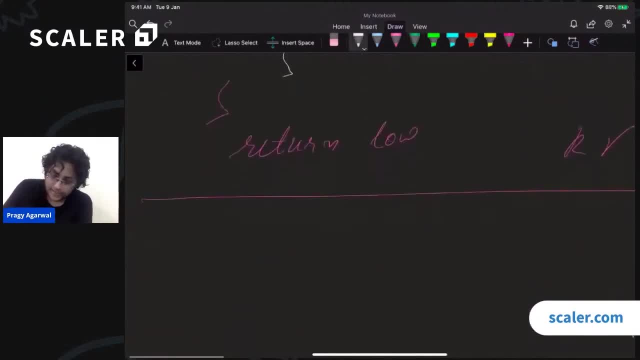 Inside this log n search, we are doing this order of n call every time, So basically the time complexity will be: order of n times. log of n. Yes, Order of n times. log of n. Well, we also have to consider the prefix something. 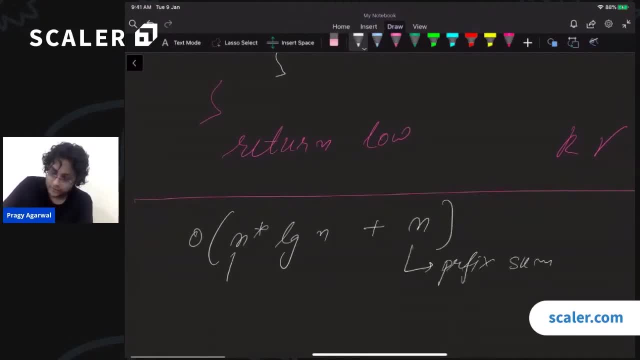 So this is for the prefix sum. This is for the binary search. This is for the binary search. Binary search. Oh sorry, This is for the binary search. This log n thing. This is for the binary search Search. 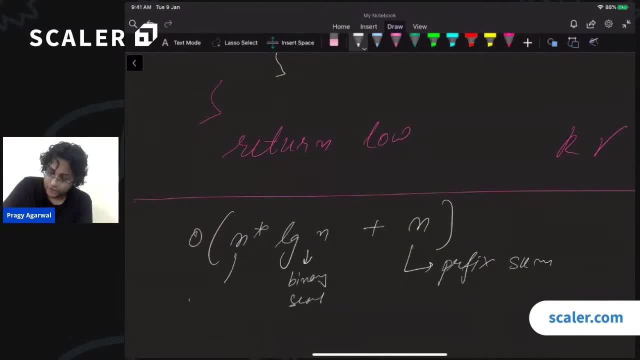 And this is for check window, Check window, Right? So the overall time complexity is just: order of n, log n. Is that clear? All right? So let us end the class at this point. Bye-bye, Have a good day. 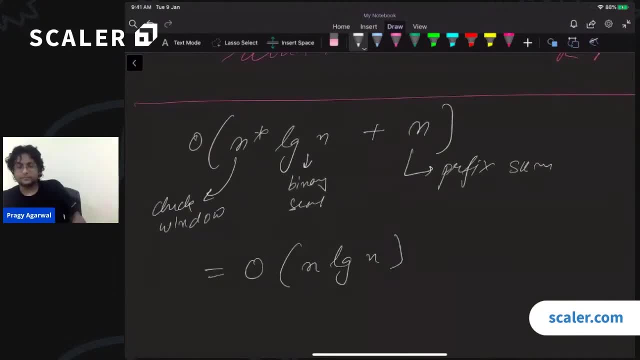 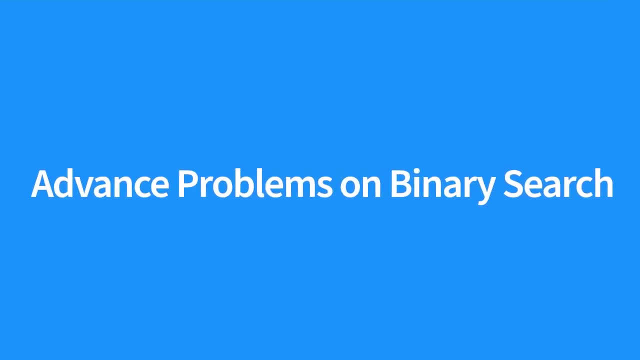 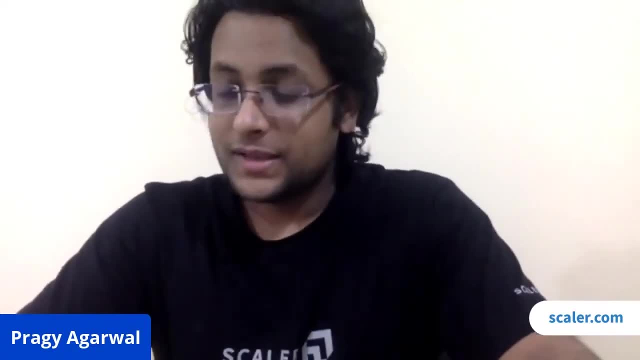 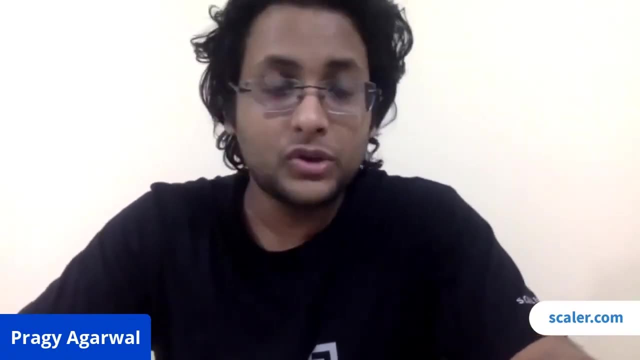 Thank you. Thank you Everyone. So we are back again with another class, All right. So today's topic is once again binary search. So we have been studying binary search in the past two lectures, right? So if you have not watched those past two lectures, please go and watch them. 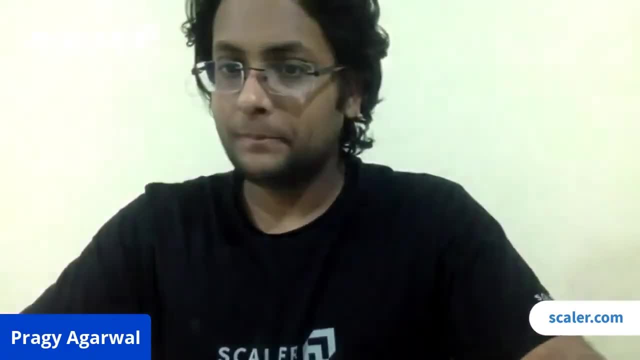 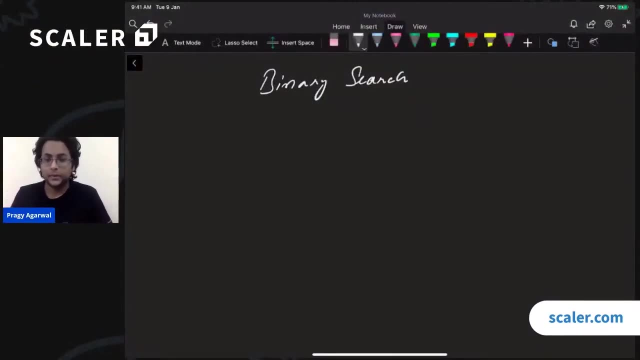 So let us continue with some more advanced problems on binary search today. All right, Let me just share my screen. I hope that everyone can see the screen, All right. So what is binary search? So let us start with a question that you might have seen earlier, right? 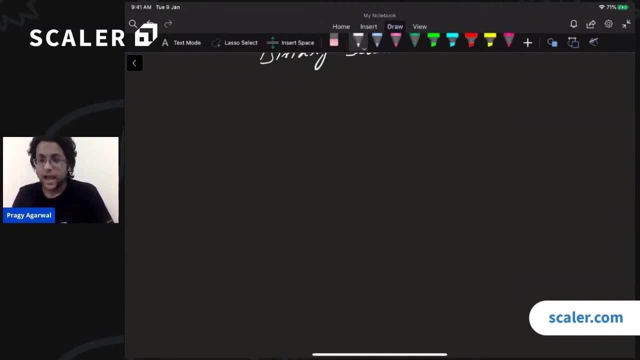 It is a pretty famous question and you might have seen this in the arrays 2D arrays class that we already had right, But this question is relevant to binary search, so let us quickly see it here. once again, Question goes something like this: 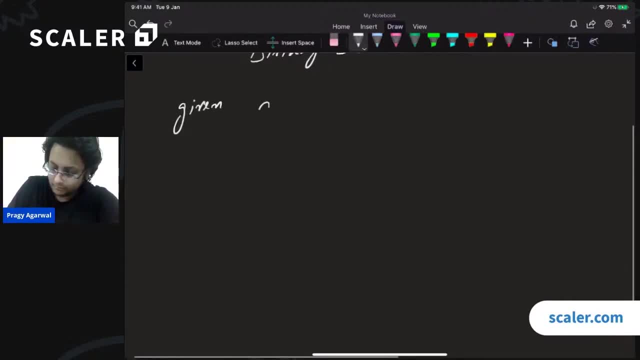 You have been given a matrix. I mean, this is not that matrix movie thing, This is a matrix, It's a 2D array. right Now, this matrix can have a certain size. Let us say that the size is n cross m right. 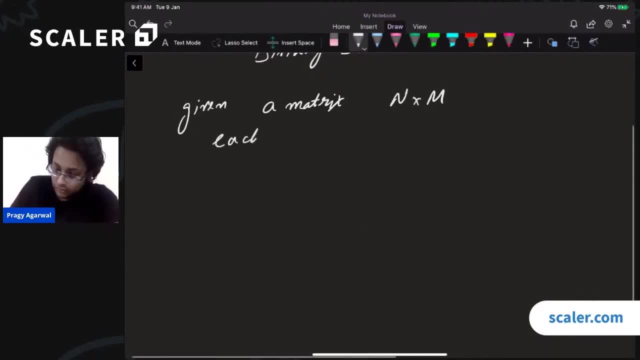 Now there's one property in this matrix: that each row and each column is sorted right. So let us quickly take an example of what such, what such matrix would look like. So suppose we have 10 over here, 20,, 30,, 40,, 50, right? 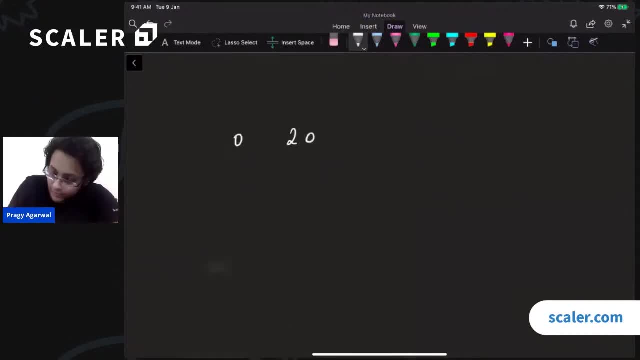 All right, All right, All right. What other numbers can we choose? So let us suppose that we have 15,, 25, perhaps 35,, 45,, 55.. Something else could be 27,, right, 29,, 29,, 37.. 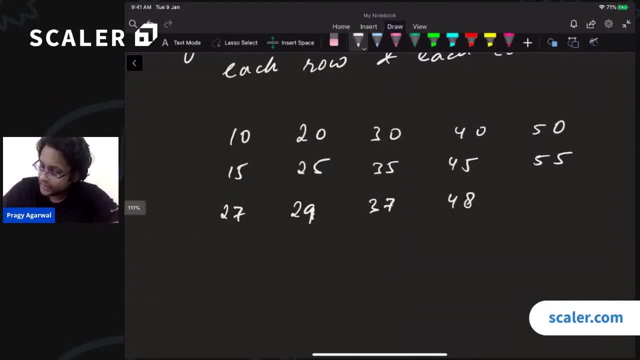 Let us say 48.. And let us say 60,, right? So let us let us just add quickly one more row. So suppose this is 32.. And suppose this is 40. Suppose this is 51.. Suppose this is 60.. 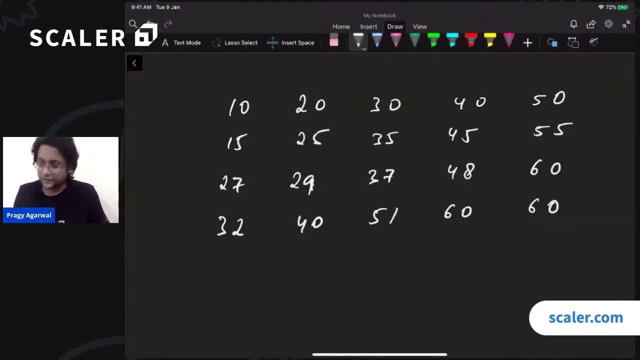 And suppose this is also 60, right? So we see that in this matrix every row individually is sorted, right? Every row individually is sorted, And so is every column. So is every column right. Cool, All right. Now what is the size of this particular matrix? 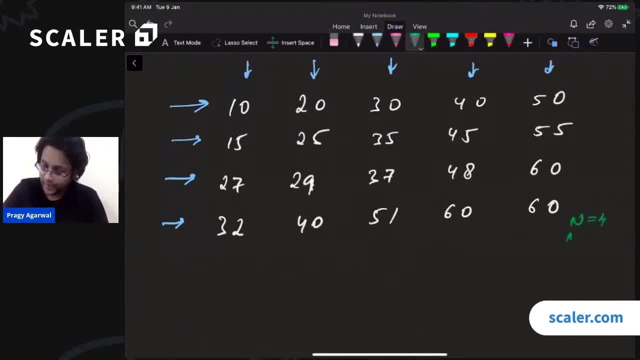 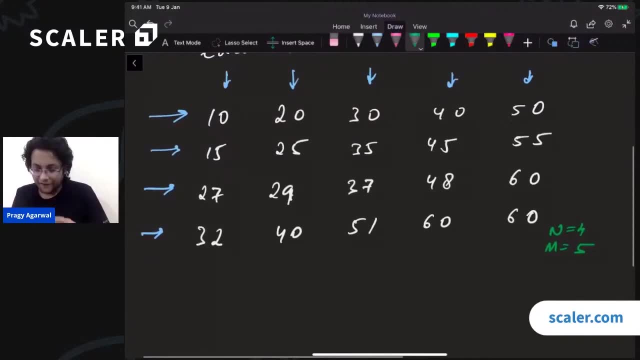 Well, over here we have four rows, So n equals to four And m equals to. we have five columns, So m equals to five. So this is a four cross five matrix. right Now, we have been given an integer. 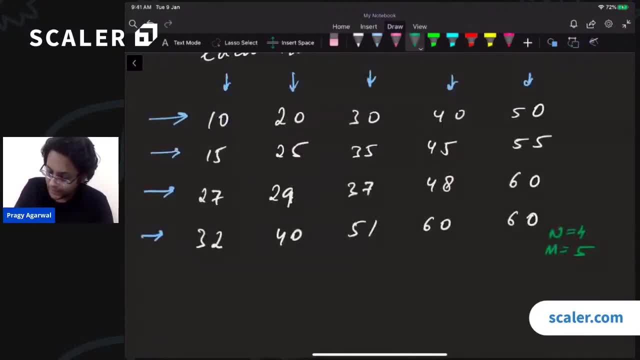 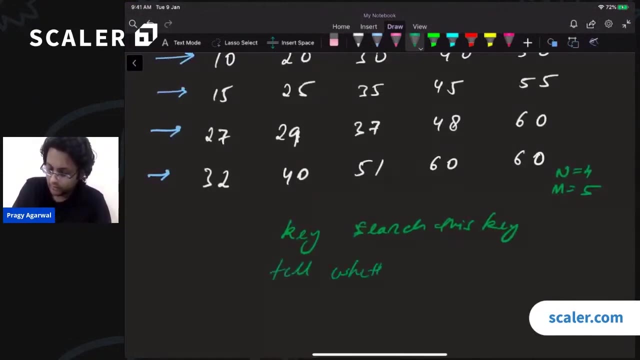 We have also been given an integer k, So k stands for key. We have been given a key And we have to search this key. We have to search this key within the matrix And we have to return. we have to basically tell whether the key exists or not. 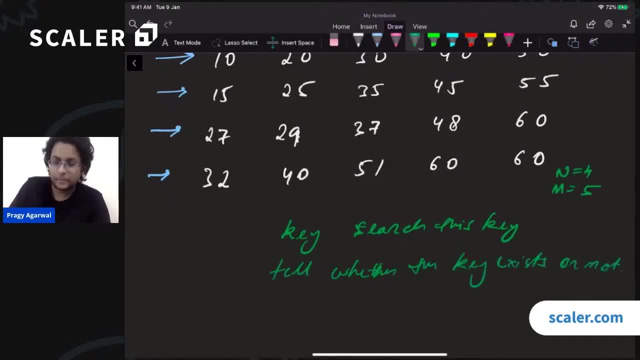 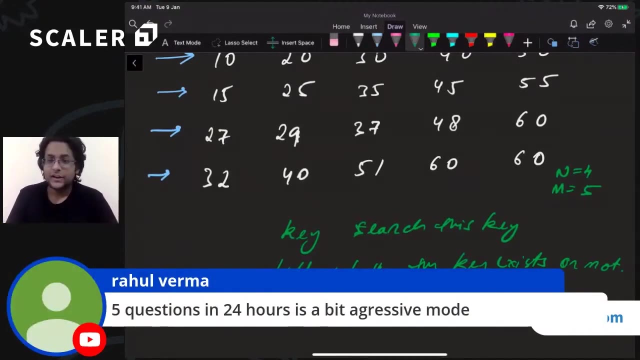 Key exists Or not? Fair enough? Yes, All right. So Rahul has a question over here. Rahul, I guess, is talking about the assignments that were given in the last class. Rahul says that five questions in 24 hours is kind of aggressive. 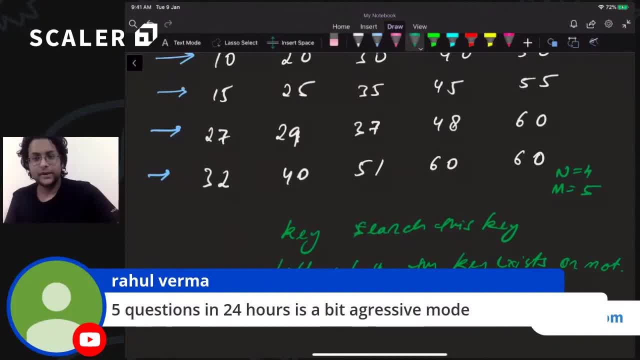 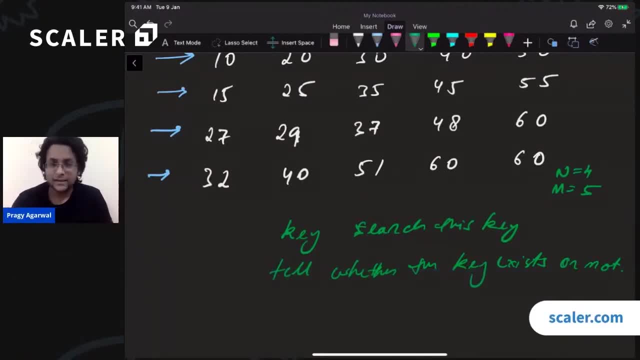 So, Rahul, you do not have to attempt those questions in 24 hours, Right? So, unlike when you are enrolled in Skiller Academy, you will have a lot of guidance. you will have mentors, you will have TAs that will be helping you while you're working through. 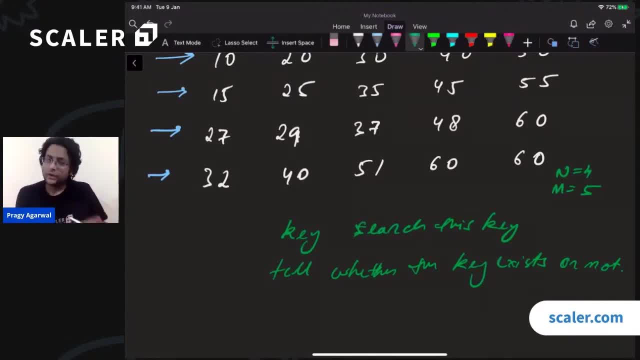 the assignments. We will have remedial classes a lot When we are on YouTube. we just want to give you as many assignments as we can so that you can practice on your own time. So it could be the case that yesterday, after taking the class, you were able to solve two of the problems. 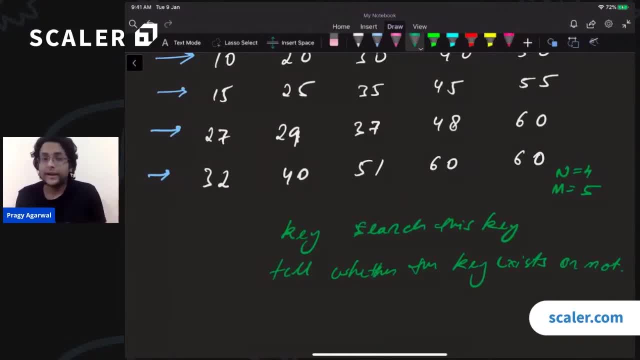 Now, maybe five days later or 10 days later, you want to come back and try it again. So we just want to make sure that you have some new problems that you can still attempt. All right, So do not worry about the time constraint. This assignment is not timed, So feel free to take this assignment. 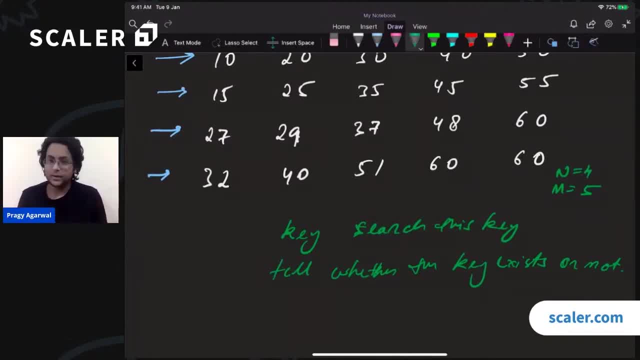 whenever you want, how many times you want, So it doesn't really matter. Just the assignment is just to make sure that you can practice a lot. Perfect, So yes, Sajia is saying that this question has been done in the previous class, So we are going to very quickly move to this question. All right, 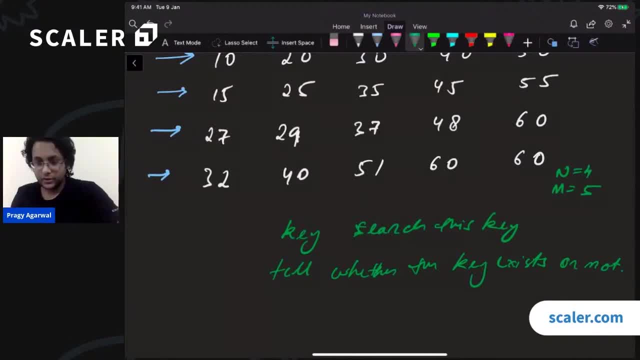 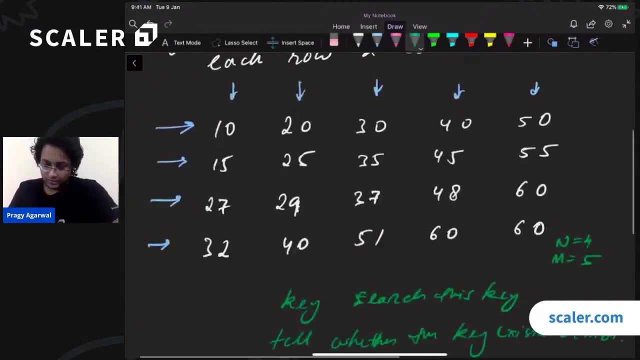 But this is kind of important for bio researchers. So, as you guys already know that this is a bio research question, So let us just quickly recap this. All right, Perfect. So this is a question. You have been given a matrix of size N to a N. 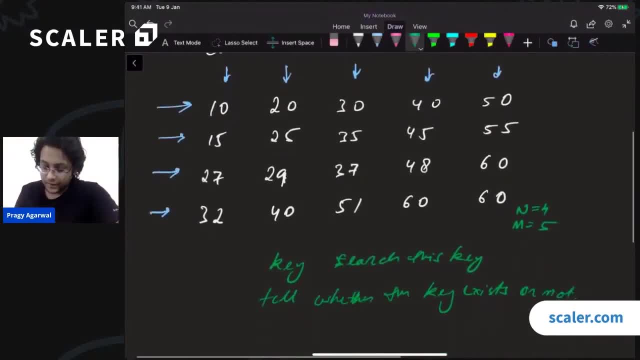 Each row in each column is individually sorted. Given a key, we have to find whether this key exists in this matrix or not. Yes, Perfect. So What approach do we have? Well, one of the brute force approaches. So, whenever we have a new problem, 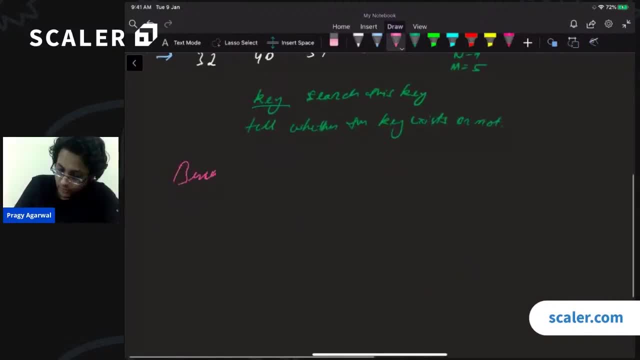 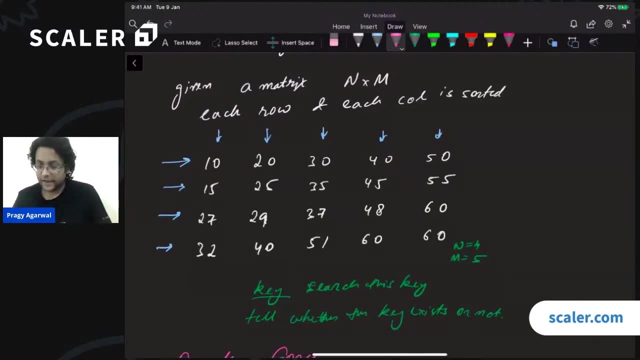 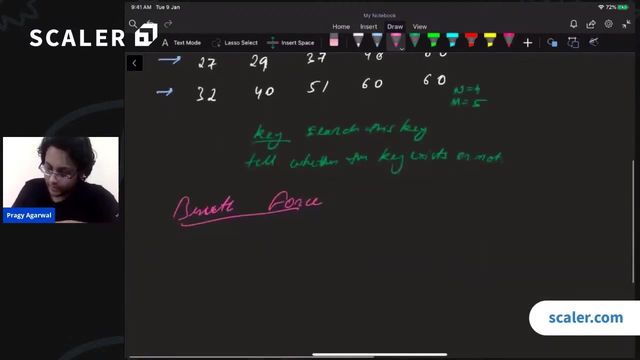 we try to come up with a brute force approach. Brute force approach Right In a brute force approach. we will not be using any extra information that we are given. So what will be the brute force approach? We simply try to linearly. we simply try to linearly. So linear search, Linear search. 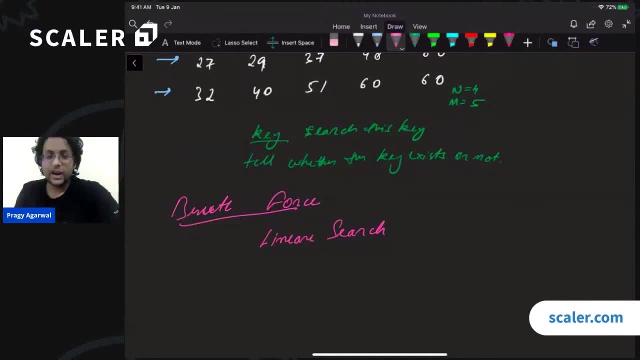 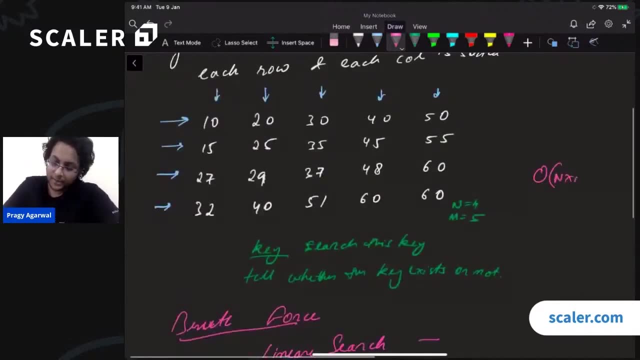 If we search through the entire matrix in a linear manner, then how much time is it going to take? What will be the time complexity? Well, how many elements are there? There are total N, cross M elements. We are doing a linear search, So it will be the complexity, The amount of time it will take. 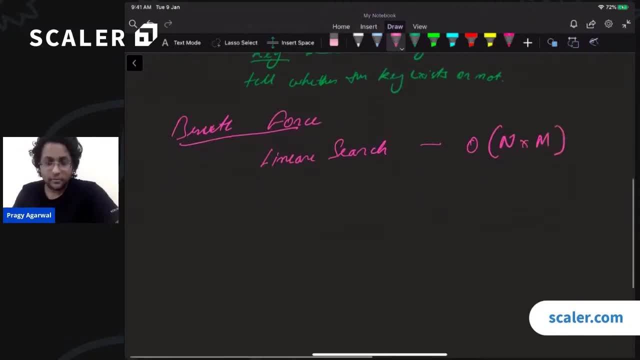 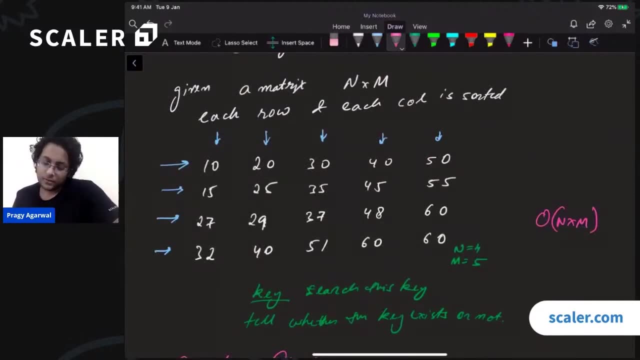 us for linear search will be: order of N, cross M. All right, But we can optimize, right? We know that each row and each column is individually sorted. Interesting Well, let us, let us just worry about the rows. So we know that, because each row is sorted, we can Binary search. We can binary search inside. 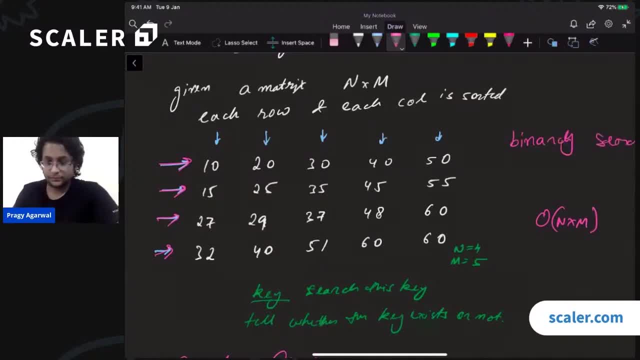 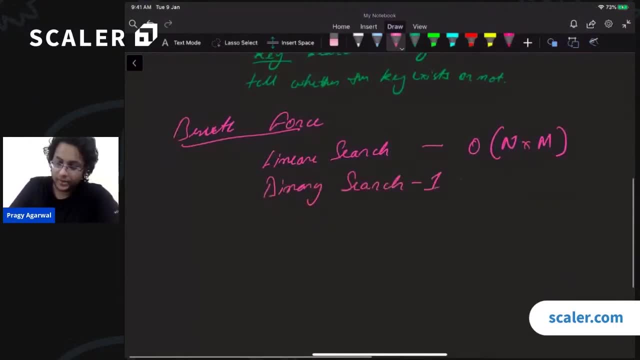 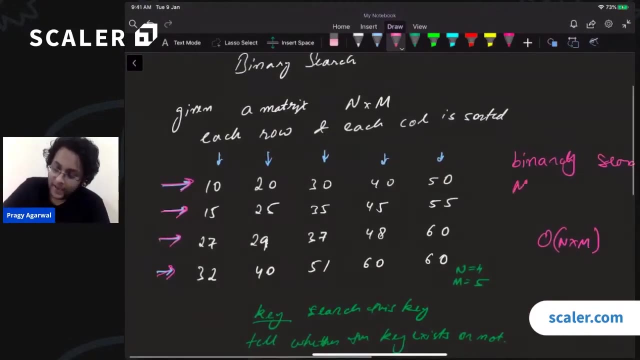 each rope. Is that correct? So if the binary source by research, let us say this, let us call it binary search one, If you binary search inside each row, then how much time is it going to take us for every row When there are elements? Well, they are elements And there are N rows and there are M problems. 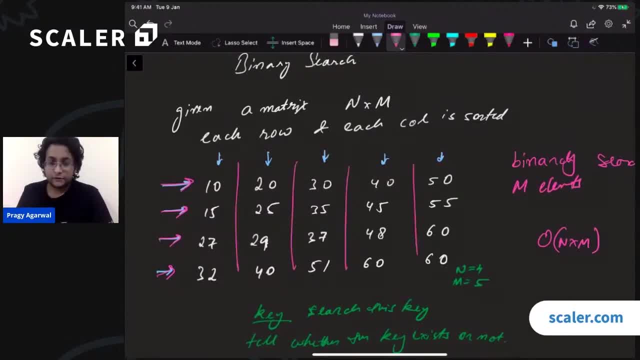 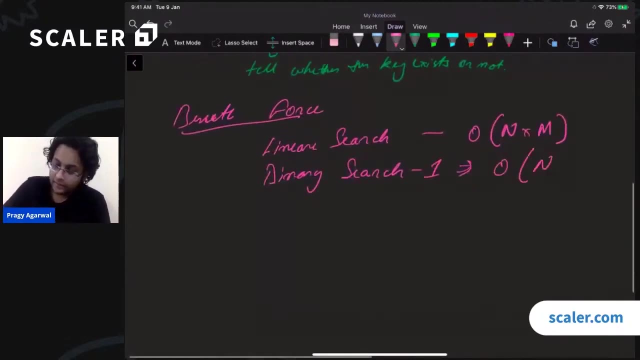 columns. So every row has m different elements. So if you want to binary source among n m elements, it will take us log of m time. Right? This is for one row. Now we have to do this for all of how many rows are there any different? So it will take us order of n times log m. 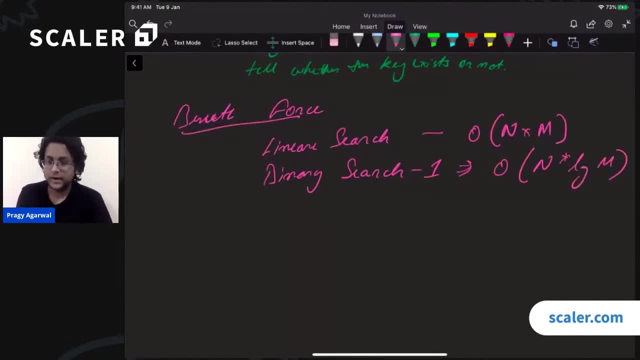 time. Yes, do you guys agree? On the other hand, if we, if we, basically so this is on the rows- if we binary search, binary search, number two on the columns, right, then it will be very simple. So it will be m times log of n, because now we are searching within. 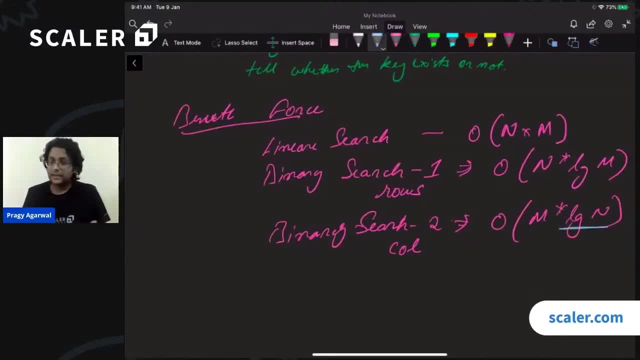 each row. we are searching within each column. And how many elements are there in a column? well, equal to the number of rows. So we can search through a column in log n time and we have m columns to search Right. So if we search through just the rows, we will get 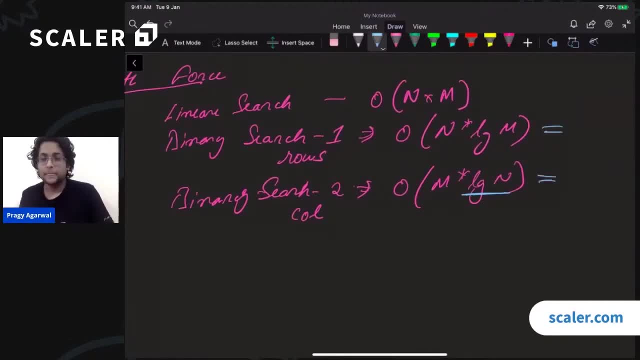 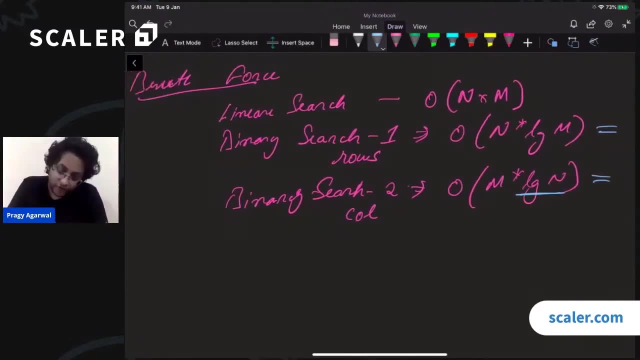 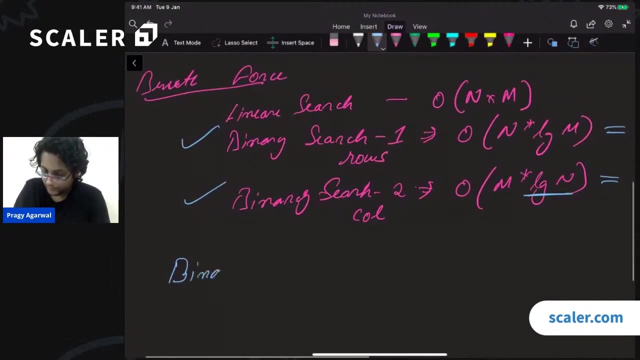 this combination. The question is: can we do better Right Now? this might not be obvious from the question itself. We have already tried binary searches. we have already tried binary searches, But binary search is not always about this binary property. So just because you are saying binary, 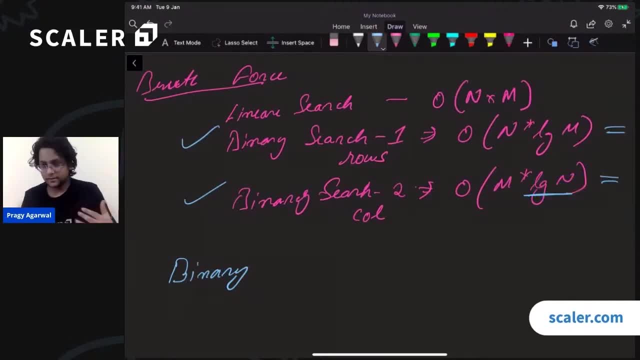 that does not mean you always, always, have to split the array to half. That is originally what binary search means. But binary search has a more important concept, more important underlying concept, And the concept, as we discussed in the previous classes, is what The concept is that given. 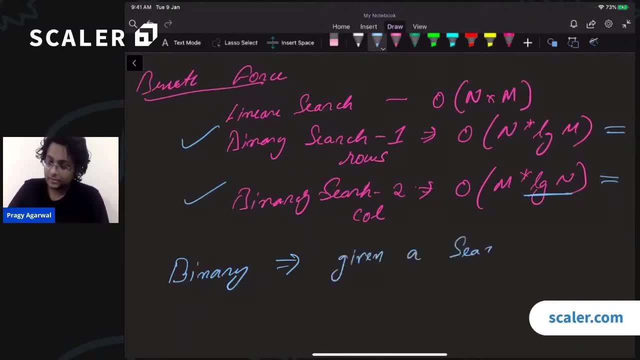 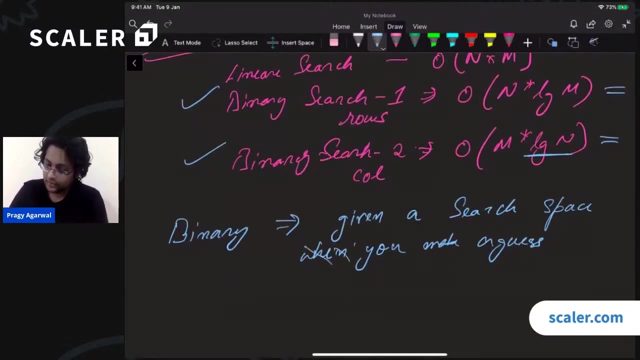 a search space, given a search space, when you make a guess. when you make a guess, you are able to eliminate a large part of that search space, right So? every guess, basically every guess, every guess allows you to eliminate a large part of a search space, right So? 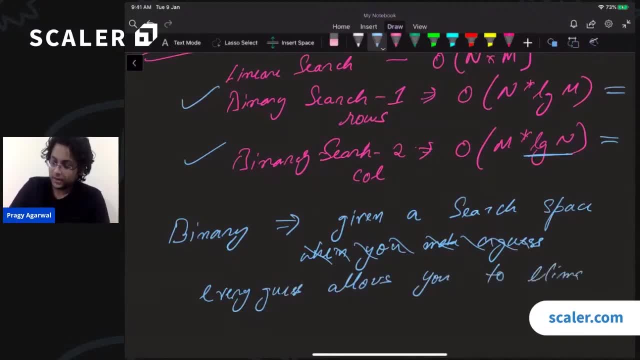 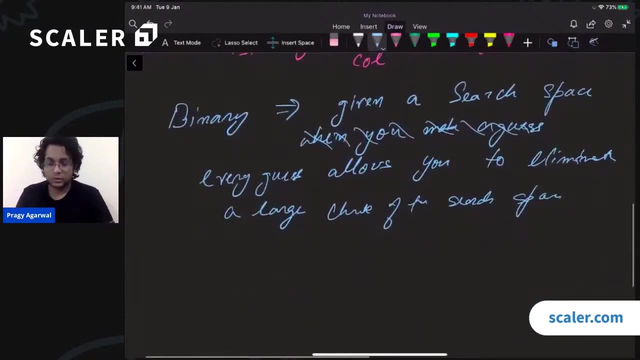 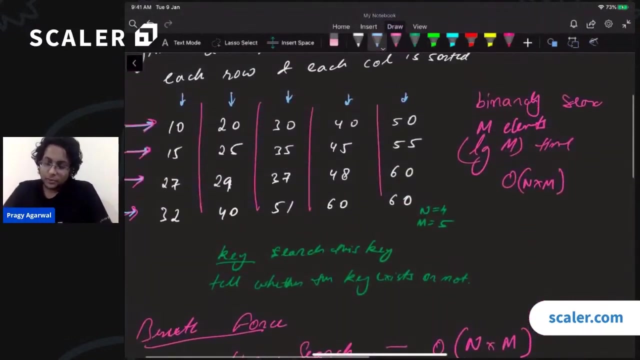 to eliminate. eliminate a large chunk, chunk of the source space. perfect, all right, so that's fair enough. so how can we basically do that? how can you basically do that for this particular question? well, we can observe, we can observe. let us suppose that. let us suppose that we are looking at this. 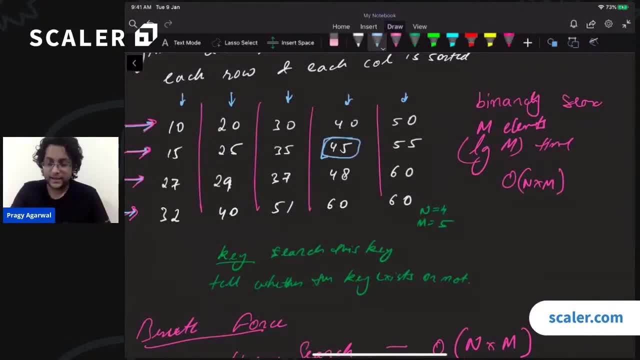 particular element. let us just pick any random element and let us say that we are looking at this particular element. right then, if we determine, if we determine that, given our key, let's say that we compare this key with 45, we compare this key with 45. suppose that the key is less than 45. suppose that we. 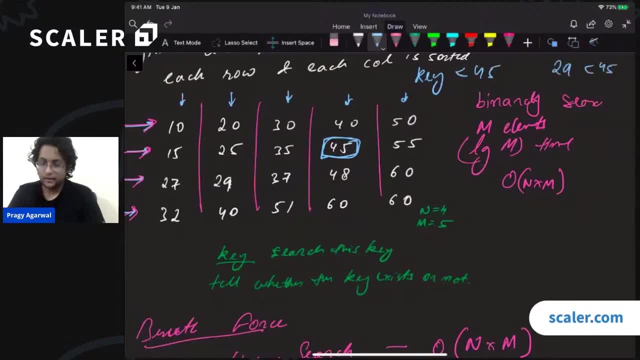 are looking for an element like 29. 29 is less than 45, right, then? what can we, what can we know from here? what can we do from? this key was less than 45, right, so can this key? can this key be over here? can this key be in this area? no, 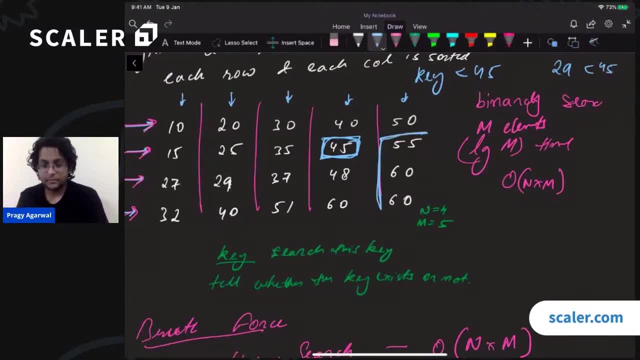 right, this key cannot be in this area. why? why can it not be in this area? in fact, in fact, this particular area? because this key is less than 45 and everything in this area, everything over here in this area, is already greater than 45, right, so the key cannot be over here. similarly, similarly, so I can reduce. 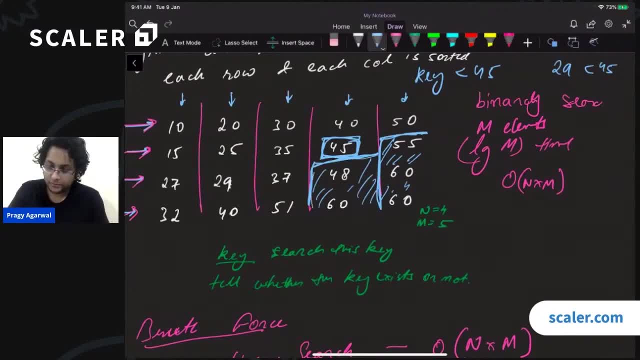 right, so the key cannot be over here. similarly, similarly, so I can reduce my search space by a larger this, this might be a larger. now there's one more property that we get. if we, if we move in a particular order- suppose that we are starting from the top right- then we can also eliminate some more, some more rows. 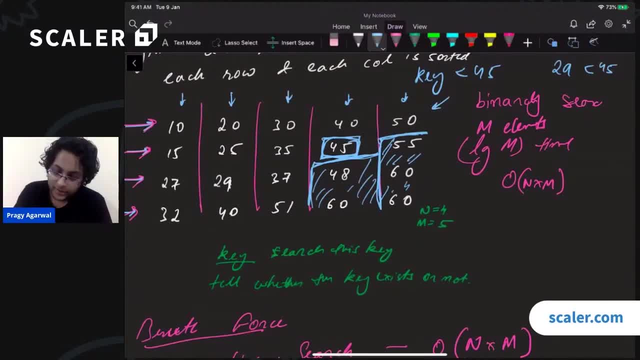 or some more parts. so we will be. we will see that we will be able to eliminate this top row as well. right, so over here there's nothing binary over here. we are not really splitting the search space into half. however, what we are able to do is we are still able to eliminate a large chunk of the search space with every. 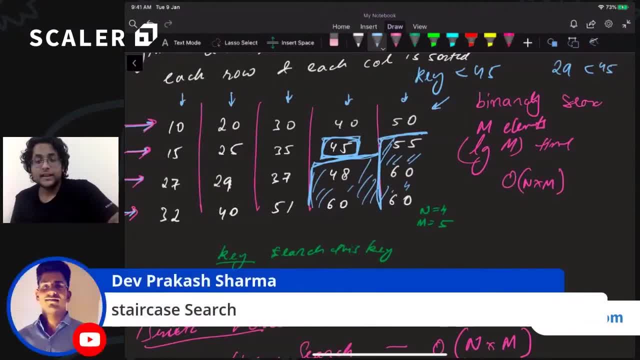 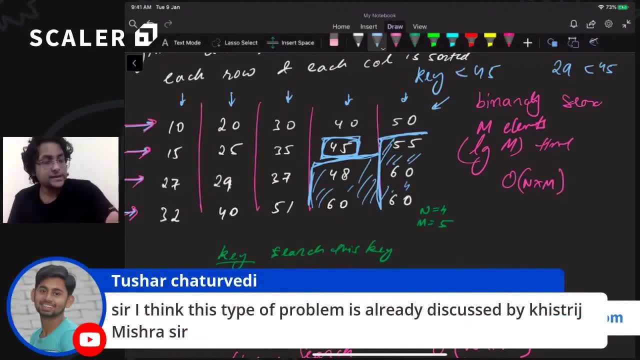 guess, yes. so Dave has a nice name over here. Dave is saying that we can call this staircase search right. and yes, Tushar also points out one thing. so Tushar says that this has already been discussed in a previous class. so yes, it has been. 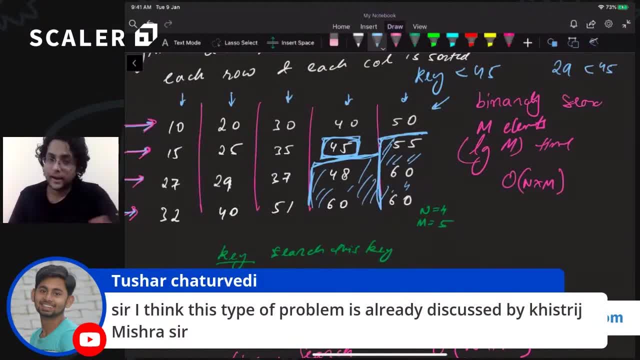 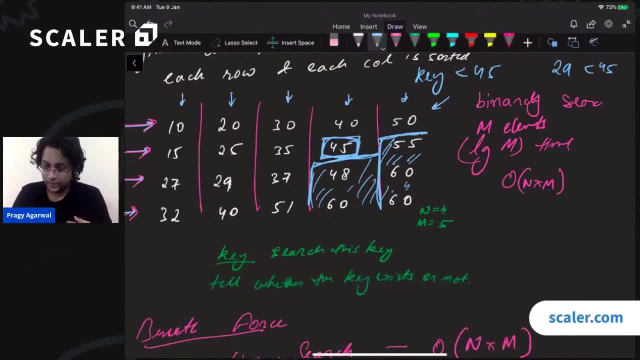 discussed in the array class. however, it is important enough to bring up again in the binary search class right, just to stress the point that binary search is not just always about binary search. right, you can still do sort of a binary search on even though you are not splitting the data into half, right, and 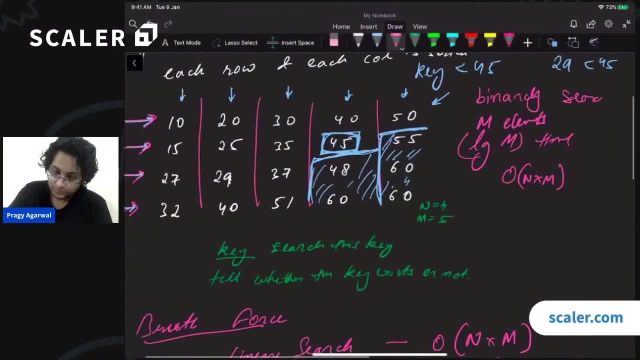 so very quickly. how can we, how can we do the search now? suppose that we start from the top right. so, once again, let us assume that the key we are looking for, the key we are looking for, is 29. we are looking for the value 29. 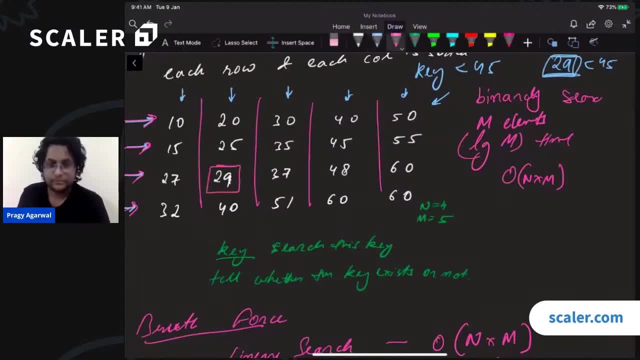 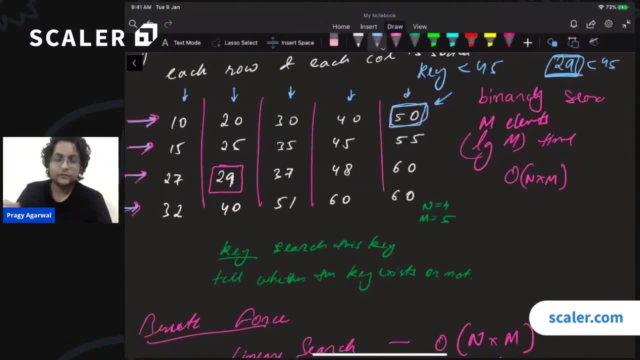 and 29 happens to be over here, right. so we better reach this point. we better reach this point, but for now we don't know where the key is. so let us start from the top right. let us start from the top right and we will compare 29 with 50. 29 happens to be less than 50. 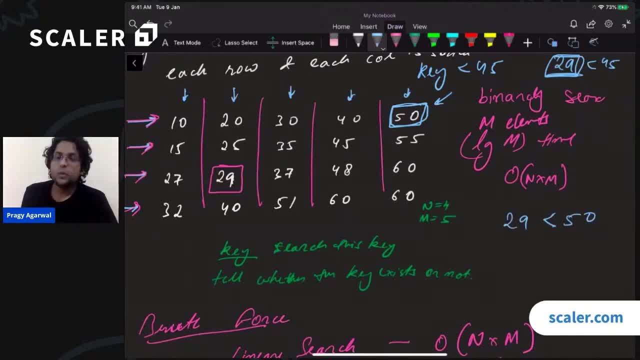 since 29 is less than 50, what can I eliminate? what part of my matrix can I eliminate? so where can 29 definitely not lie? because of this comparison that I have just made, I know that in this particular column, this particular column is sorted right. so over here, in all this column, every element is greater than 50. 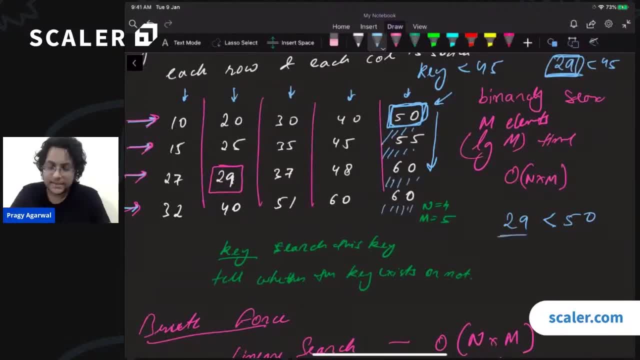 is greater than equal to 50, and we already know that 29 is less than 50. so my key cannot be in this column, right? my key cannot be in this column, So I can eliminate this column, Do you agree? Yes, All right, Once I have eliminated the column. now I have a different matrix, right, I have? 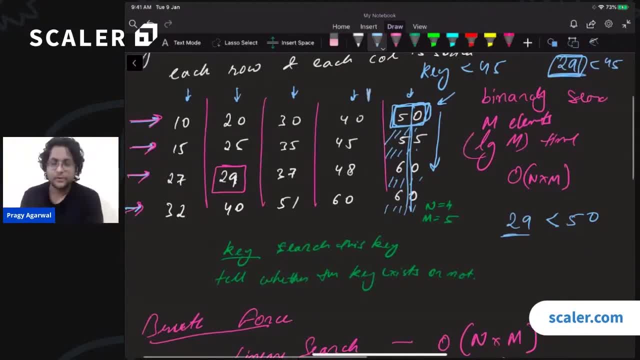 a different matrix. The matrix exists only up to this column right. So what is the top right part now? What is the top right part of the matrix? It is this particular cell. All right, Let us compare once again. So we know that 29 is again less than 40. So once. 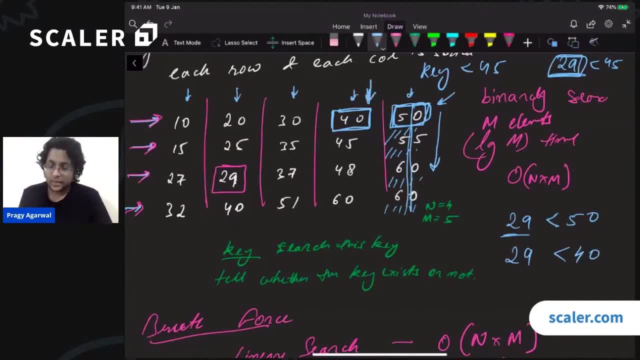 again by the same argument. since this column is sorted, then 29 cannot be in any of these elements, because we know that 29 is less than 40. So let us very quickly eliminate this column as well. Perfect, Let us move on to the next top right element. So this is 30.. 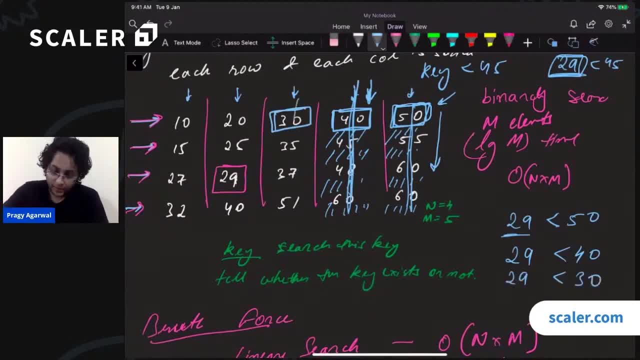 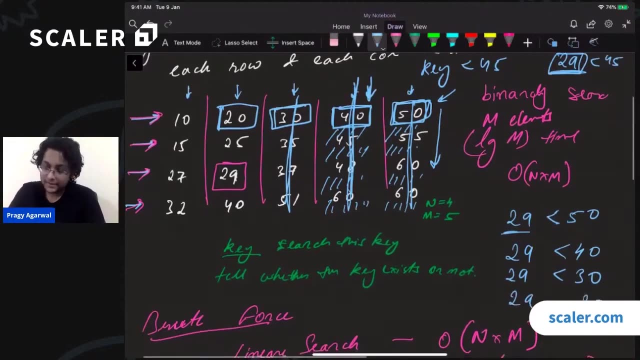 29 is still less than 30. By the same argument, we will be able to eliminate this particular column. Does that make sense? Yes, Let us continue. So now, the top right element is 20, right: 29 versus 20.. What is it? So 29 is greater than 20.. Well, now a different. 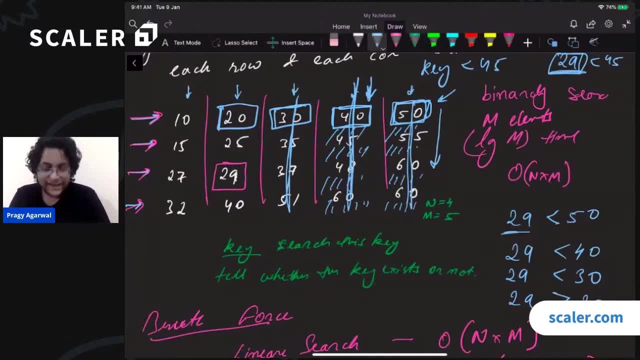 argument appears. Let us look at the different argument. So we know that 29 is greater than 20, right? So if we look at this particular column, if you look at this particular row, we know that everything to the left of 20, everything to the left of 20 over here in. 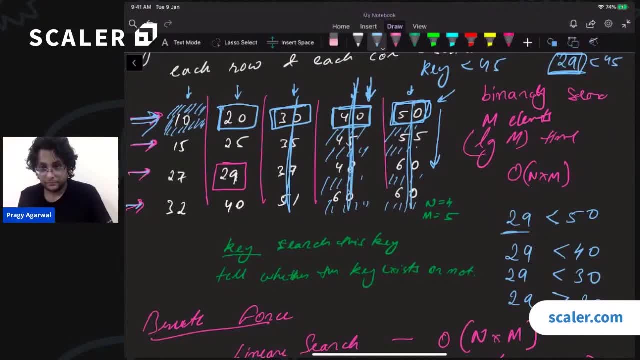 that same row right. that has to be less than 20.. Everything to the left of 20 has to be less than 20.. Because the row is sort of: So 29 cannot be over here. So what we can now do is we can. 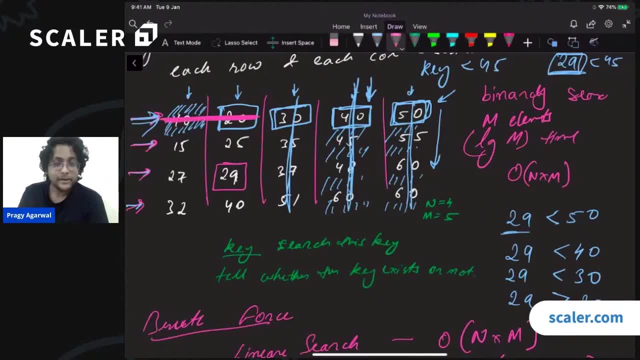 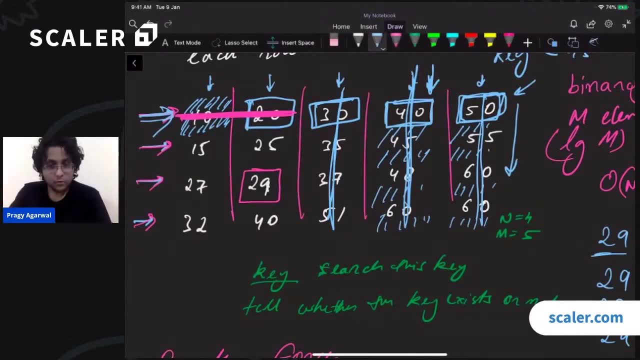 eliminate this particular row. We can eliminate this particular row And notice that these columns have already been. these columns have already been eliminated, right? We move on to the next top right element. So 25 is the next top right element. We compare once again. 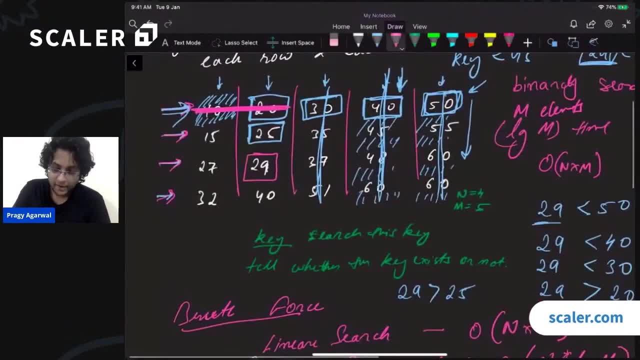 29 happens to be greater than 25.. So by the same argument, we can eliminate this row. Then we move to the next top right element, which is 29.. And now we can return. yes, that, yes, we have found. 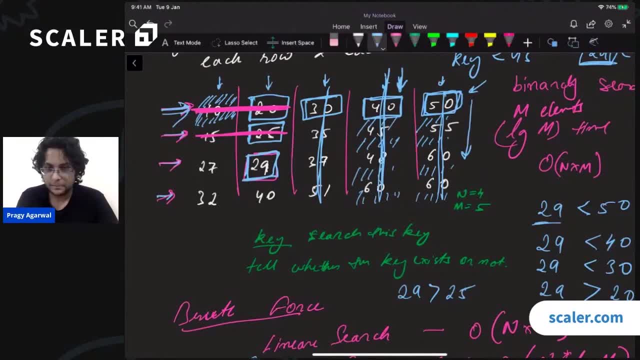 29 and 29 exists in our matrix. Is that clear? Yes, So we are not doing binary search, We are kind of doing a staircase search. right, We are zigzagging around. So in this particular case, we moved along this path. We moved along this path. There's nothing binary about this. 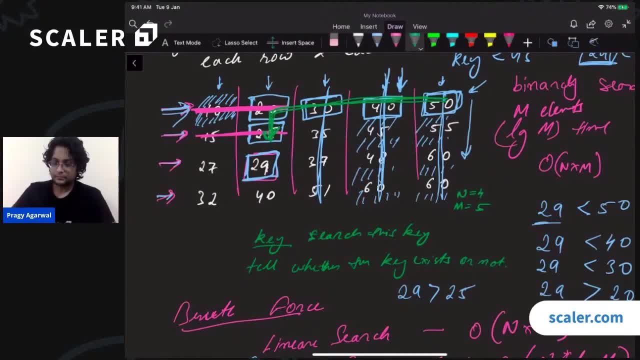 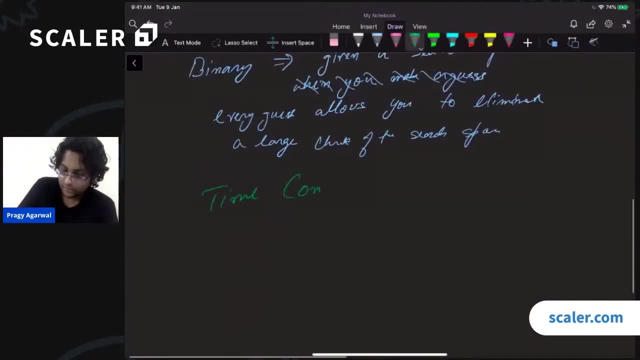 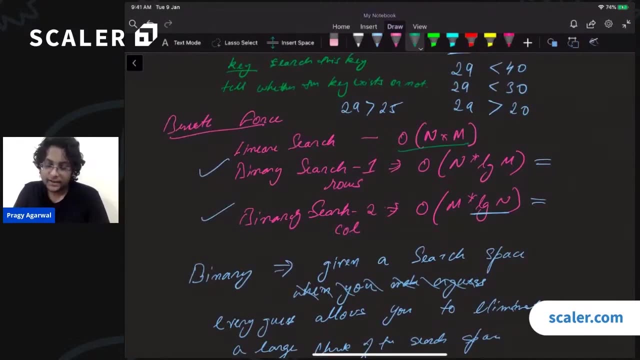 but this is still an example of binary search. Is that clear, Cool, Okay, What will be the time complexity, Time complexity of this approach? So we have already seen that linear search takes this much time. Binary search will take either n login time or 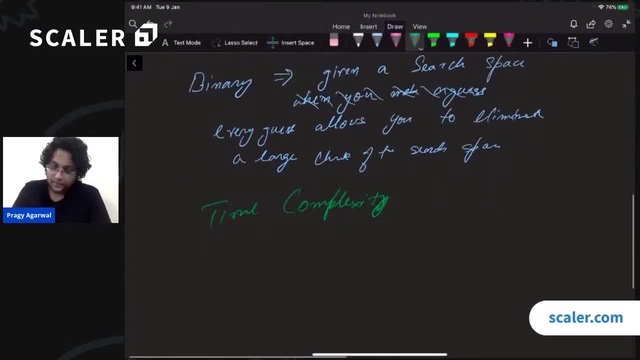 m login time. What about this particular approach? Well, for this approach we can. we have to go from the top right corner, in the worst case, to the bottom left corner, right, From the top right corner to the bottom left corner, And the path does not matter. The path does not really matter. 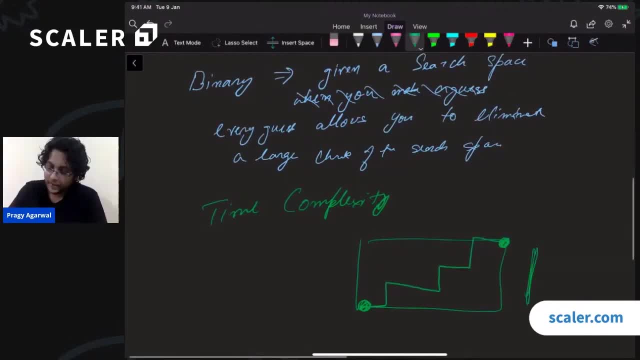 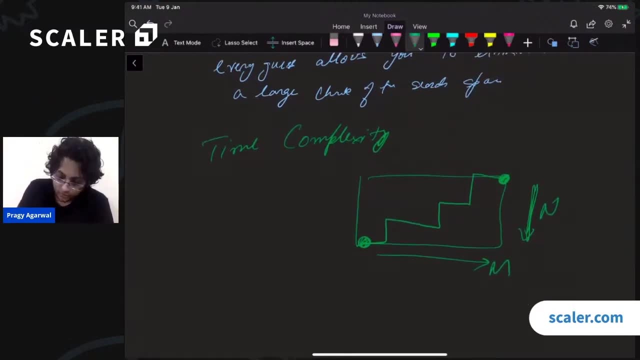 because in both the cases we have to go from the top right corner to the bottom left corner, And this is what we will be covering. We will be covering n different rows and m different columns, So our total path length, Our total path length, is equal to n plus m, irrespective. 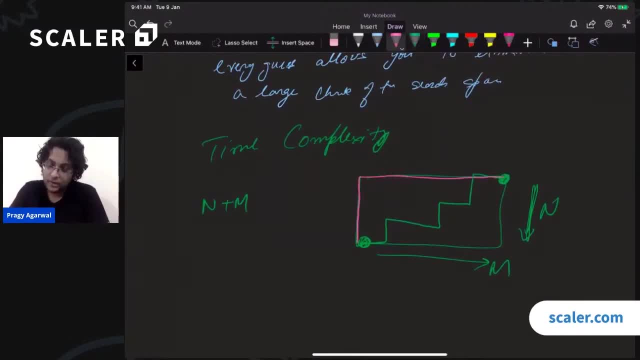 of what path we need. Either we go this way or we directly go over here, or we maybe take this weird way. All these cases have the same path. length of n cross m, m plus n, So the time complexity will be the order of n plus m. Is that clear? So this was a repeated question. 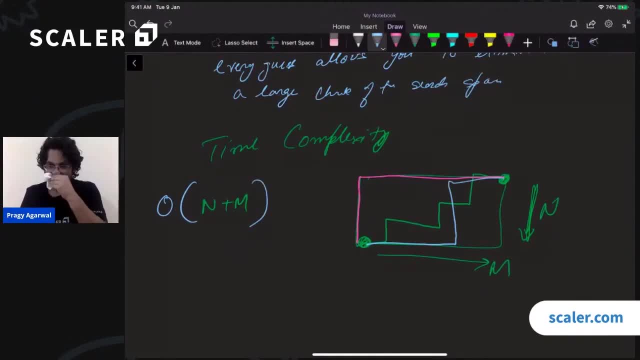 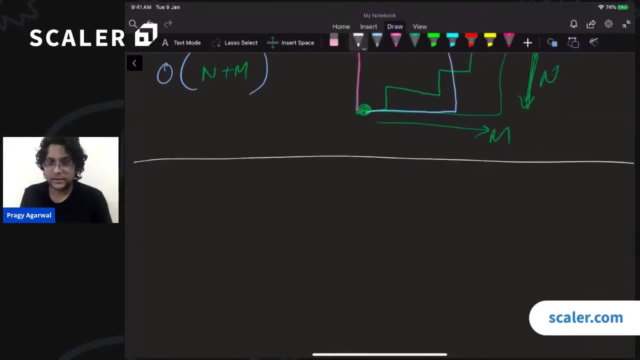 but this was still. we'll just keep going on till the end. So this was a pretty simple, very simple and very relevant to binary search. Let us move on now. So, very quickly for this question, let us move on to the next question. 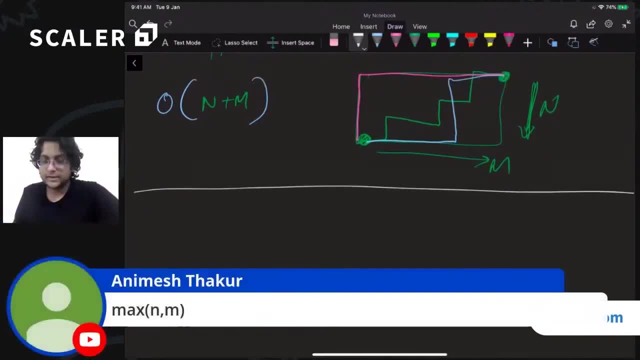 So Animesh over here says: can we rewrite this? So Animesh says that, okay, perhaps we can also rewrite this as order of max of n, m And that is true, That is true. So, as we saw in the very first class, 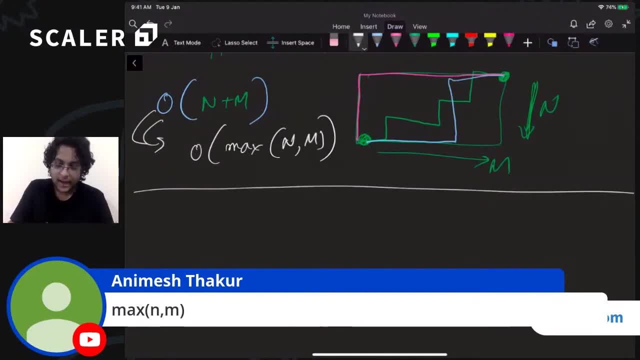 on time complexity analysis, we saw that we can rewrite this part as max of n m, Because asymptotically, these complexities will turn out to be the same. They are related by a constant factor of each other. All right, Perfect. 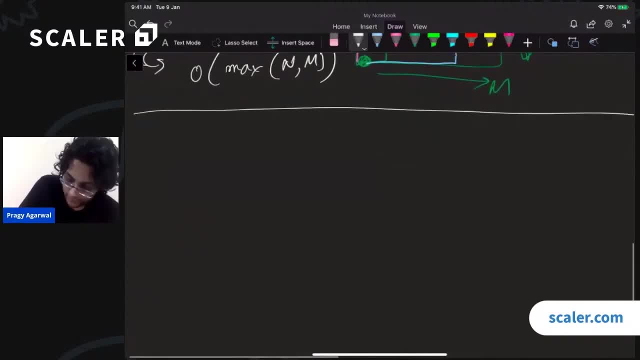 Moving on, let us see a more challenging question. So this question is very famously called aggressive cows. Aggressive cows, I think this question was originally from the platform Sporch right And this question is very, very common. I mean, this question happens to be. 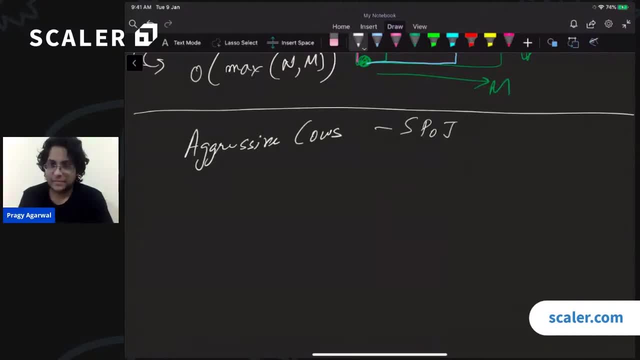 one of the favorites for all the companies. So this question, it has been asked numerous times at Google. This question is still asked very frequently at places like Direct Time and Amazon, And this is a very, very nice question, Right? The special thing about this question? 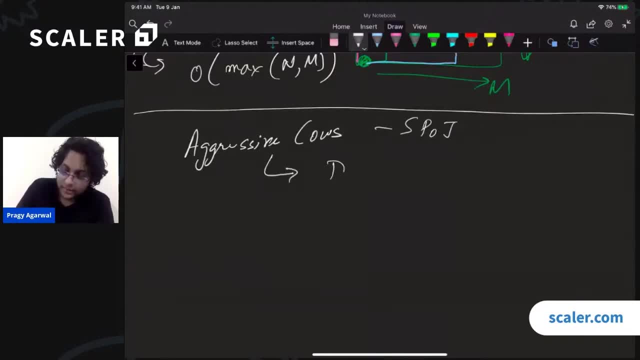 as you will see, is that it has a very nice solution using dynamic programming as well, But it can also be solved using binary search Right. So a lot of the times when a student goes to an interview, they are expecting a difficult interview question. 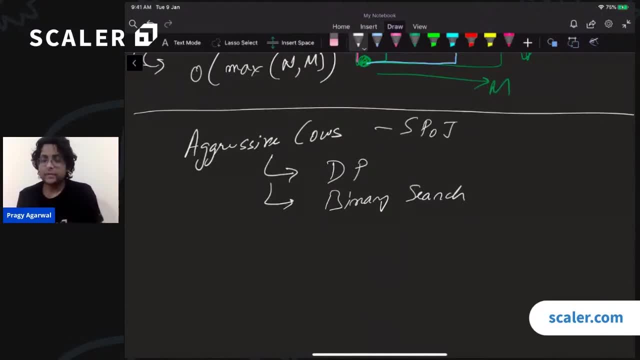 Right, A lot of the students are afraid of dynamic programming, Even though dynamic programming is pretty easy, Right? So whenever they see this question, the natural approach, the natural idea that comes to their mind is: okay, I can try dynamic programming. 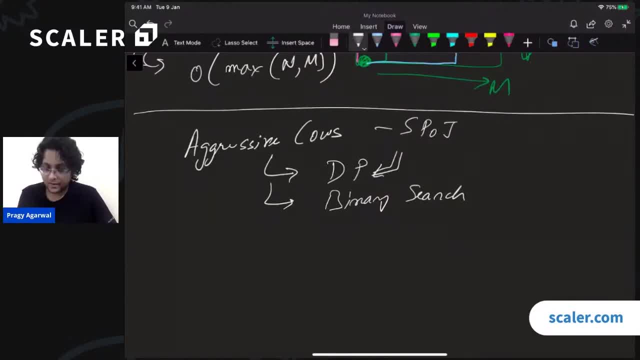 on this particular question. Of course, dynamic programming solves this question, but binary search solves this in a faster manner. All right, So let us quickly see the question. The question goes something like this: that you have n different stalls. You have n different stalls. 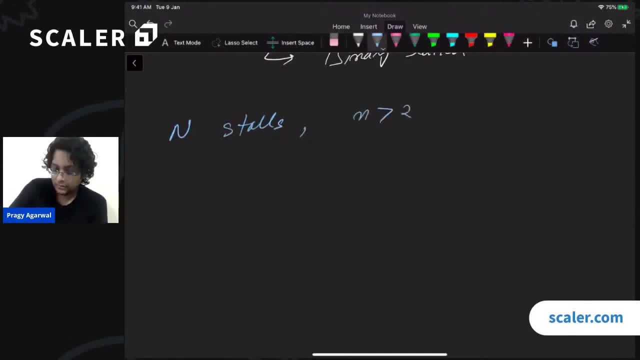 Right And the stalls. so let us say n is greater than 2.. You have n different stalls, You have more than 2 stalls And you have c cows Right. Once again, c is going to be greater than 2.. 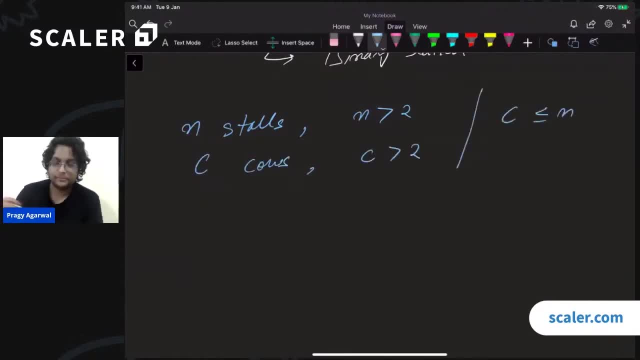 There's one constraint over here: that c is less than or equal to n. Right, We have n different stalls and we have c different cows. Now you have been given the location of these stalls. The location of these stalls has been given to you. 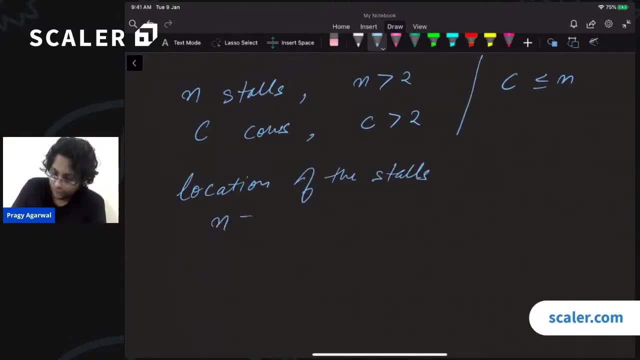 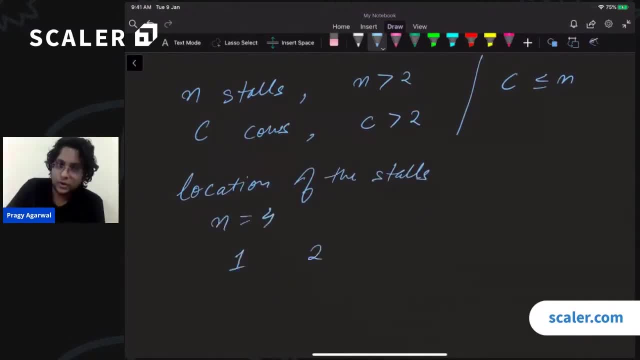 And the location of these stalls are 1,, 2,, 5, and 8.. Right n equals to 4.. And the location of these stalls are 1,, 2,, 5, and 8.. Or, for those all inside, let us make n equals to 5.. 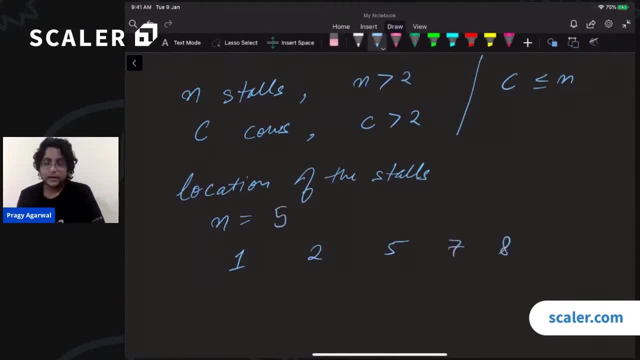 Let us just add one more, And 1 to 5,, 7 and 8. What that means is that the first stall, the first stall, the zeroth stall, is at location 1.. The first stall is at location 2.. 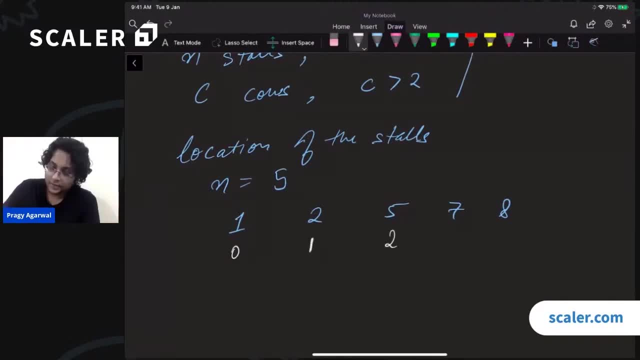 The second stall is at location 5.. Third stall at location 7.. And fourth stall at location 8.. Right, So you can, you can, you can generate BACKFIRST, Right. imagine this, that this one stall, this is the other stall, this is the third stall. 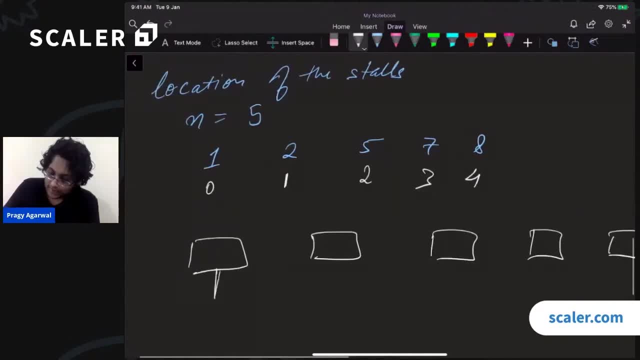 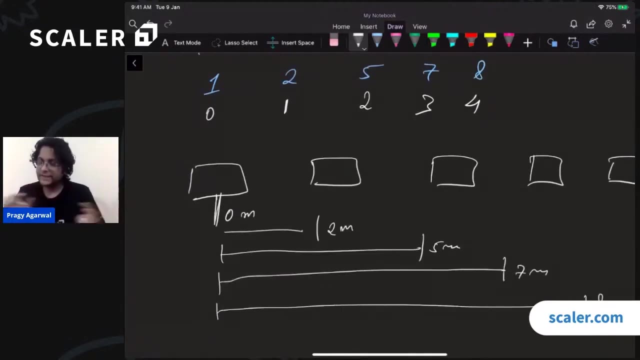 this is the fourth stall and this is the fifth stall, and if this is at zero meters, then perhaps this stall is at two meters, then this stall is at five meters, This stall happens to be at seven meters and this stall happens to be at eight meters, So they are unevenly spaced. These stalls are unevenly. 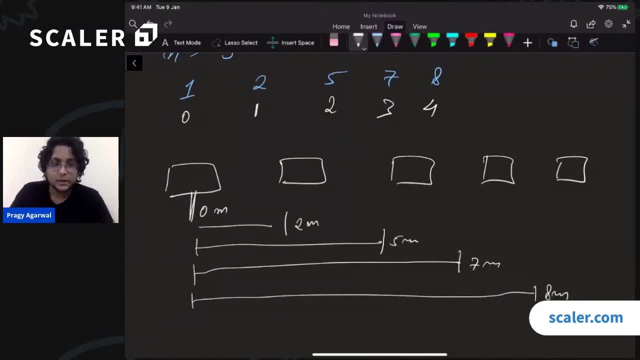 spaced. Now we also have C counts. Suppose for this example, we have suppose for this example, we have three cows right, c equals to three. so now our task is to place these cows, our task is to place these cows into the stores. and one cow one. 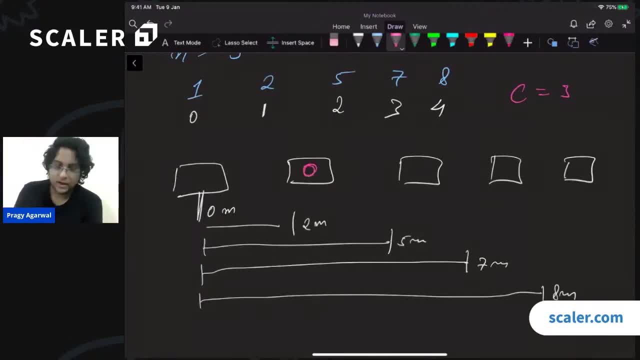 cow can only go in one, so i'll just draw the cow as a circle, right? cows are not sphericals. so i mean, if you were a physicist then you would say that, okay, cow is a. you you would consider a spherical cow in vacuum, right? but we are not physicists over here, so let us just consider. 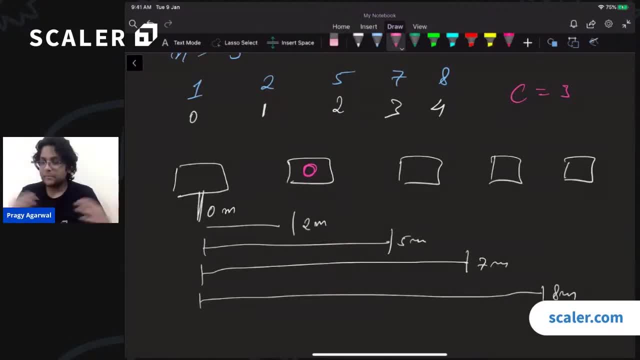 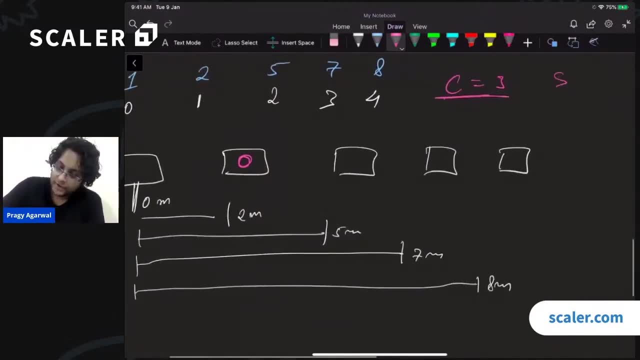 this cow in this particular store. right, so i can, i can put this stall in min. i can put this cow install in many, many different ways if i have three cows and i have five stalls. if i have five stalls and i have three cows, then very quickly, can someone tell me what is the total number of ways i? 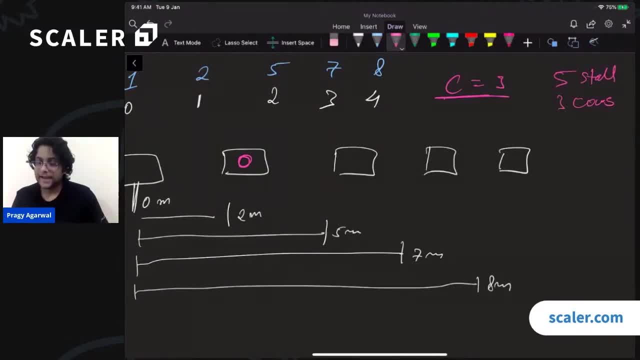 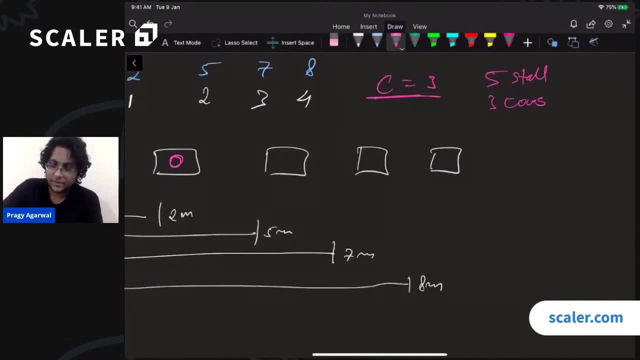 can put them. what is the total number of ways i can take three cows and put them in five stalls. well, that will simply be. that will simply be five. choose three. right, i have to choose three stalls out of five stores to put the cows, and oops. 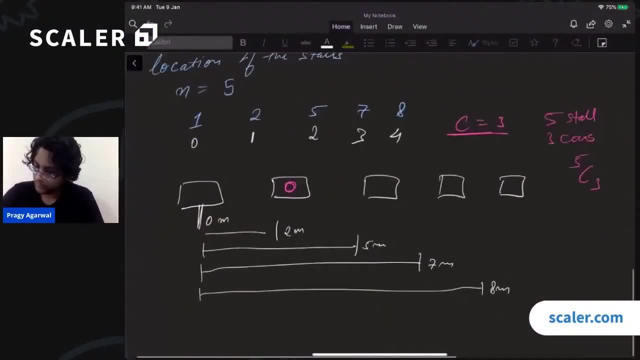 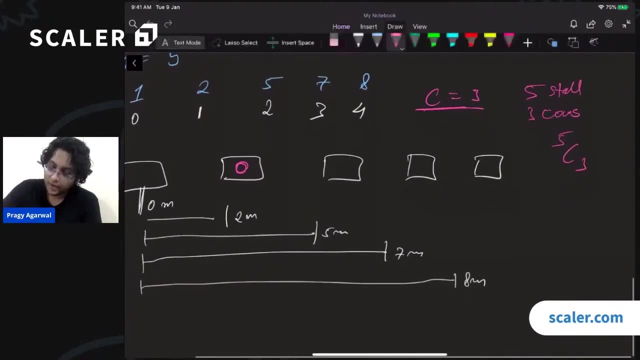 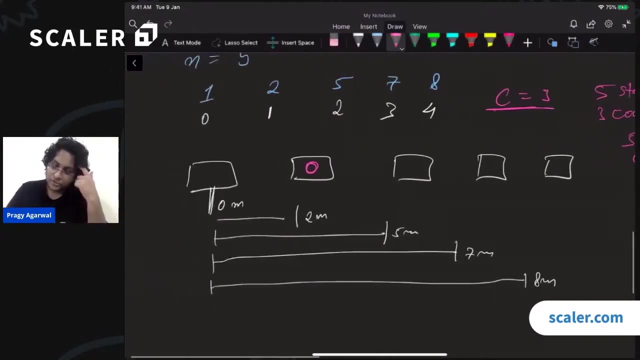 so let us go back. sorry about that, right. and if the cows are distinguishable? if the cows are distinguishable, then i will also have a three factorial factor coming right, that that depends on whether the cows are distinguishable. right, perfect. so suppose i put the first cow over here in this store. i put the. 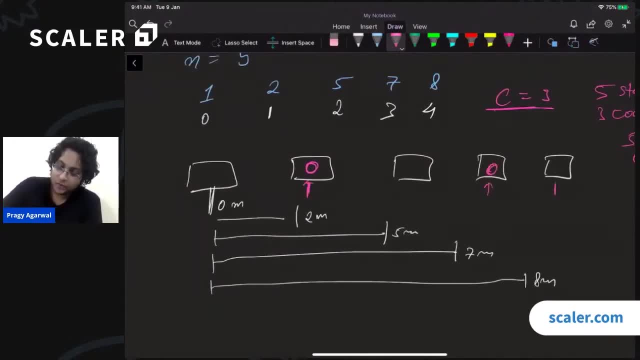 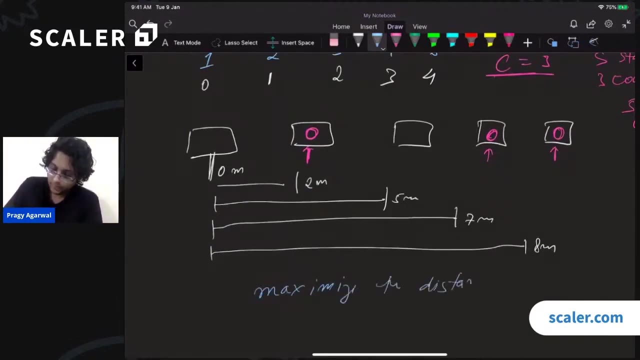 second cow over here in this toy and i put the third cow over here in this store. right now, the cows are aggressive, they want to fight with each of them, right? so we want to maximize. we want to maximize the distance between the cows, between the cows right now, but there are, there are multiple. 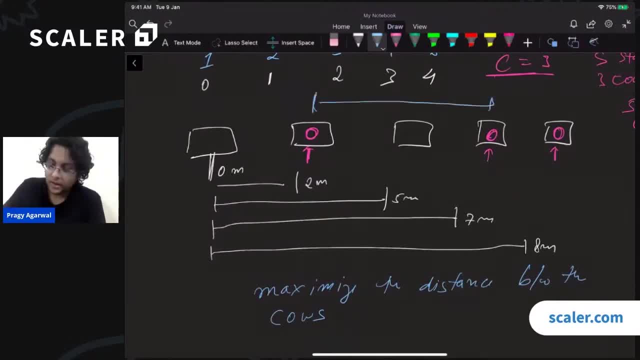 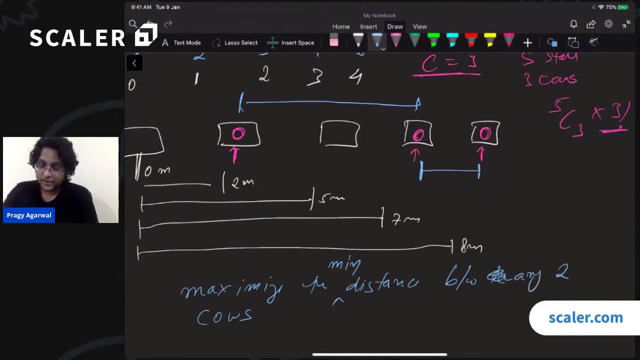 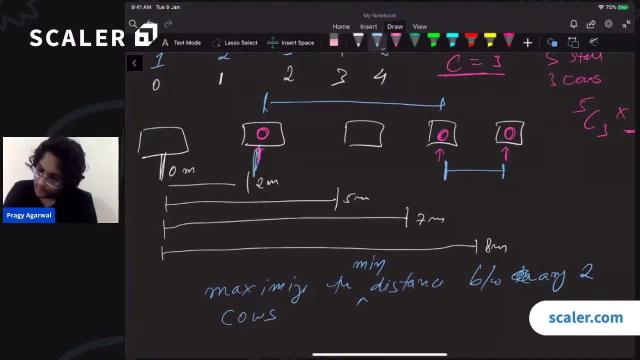 differences, right? so there's. there's one distance between this cow and this cow and there's one distance between the two cows are in between, so the difference between the two ones is six meters. okay, so this one greater distance here is six and the one you have over here, right so? 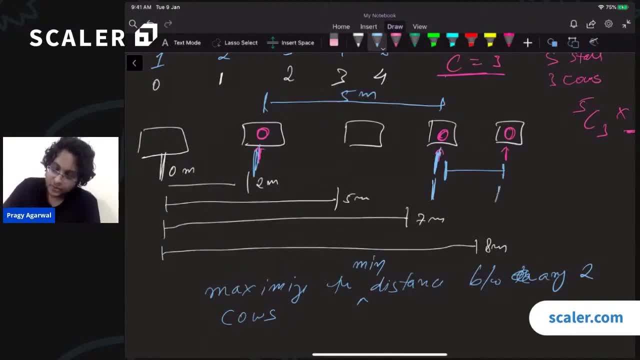 this means that, as a result of all this, we can actually put it anywhere. so it is zero, right? it is six meters. okay, right. so this is the distance between two cows. so now, to which distance are we among these two is? the minimum distance among these two is one meter out of five and one one. 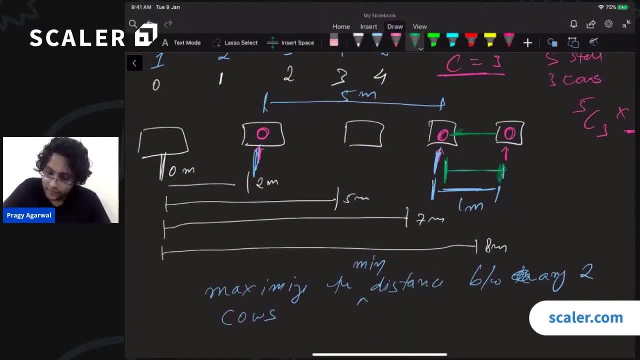 is minimum. so we are saying that this is the minimum distance between two cows in this particular arrangement. we want to maximize this distance, we want to place the cows as far apart as possible, all right. and this distance, mind you, this distance is not in terms of the stall number, this distance, 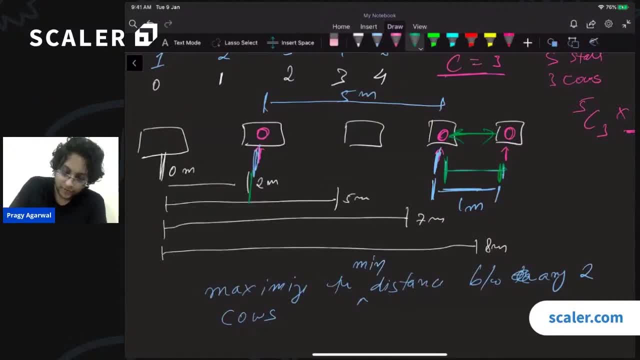 is in term of the location of the stall, right? so we have two things over here. we have the zero- first, second, third, fourth stall. we have the stall number. that is not what we're talking about. we're talking about the distance in terms of the location of the stall. is the question clear? 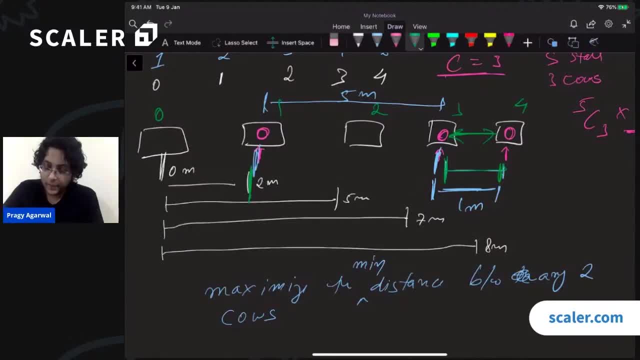 yes, so very quickly, what do you think should the answer for this particular case be? what do you think should the answer for this particular case be? suppose that this is the arrangement. suppose that this is the arrangement. i have stalls at zero meters, two meters, five meters, seven meters and eight meters, and i have three cows. then where should i put these? 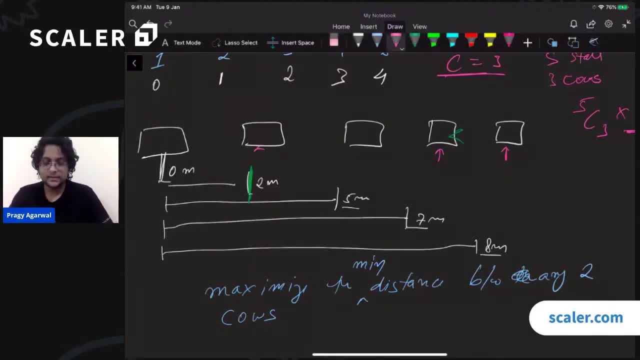 cows. where should i ideally put these cows to maximize the distance? yes, the first cow should go in this particular stall. the first cow should go in this particular stall. all right, then i can put the second cow in this stall and i can put the third cow in this stall. is that clear? yes, so this will be the ideal. 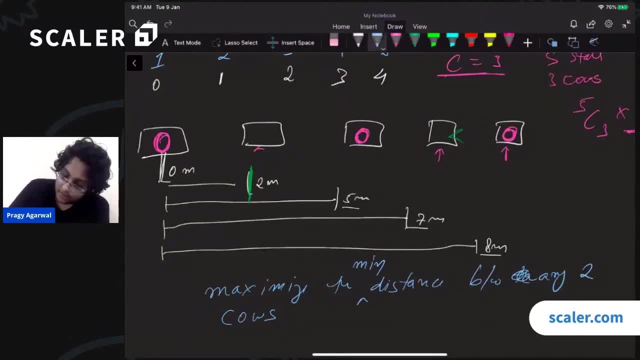 case and what will be the what will be the final distance? the distance will be, so the distance between these two cows happens to be five meters, the distance between these two cows happens to be three meters and the minimum of those distances is three meters. so we are making sure that the cows are. 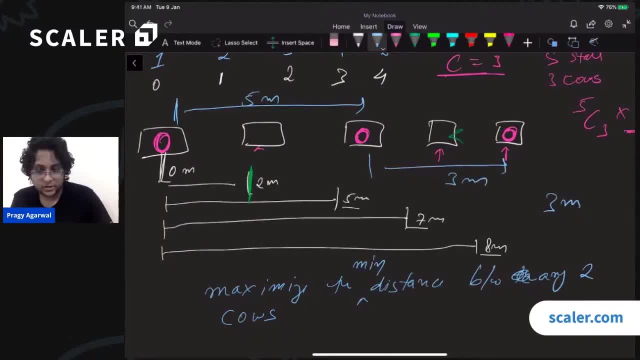 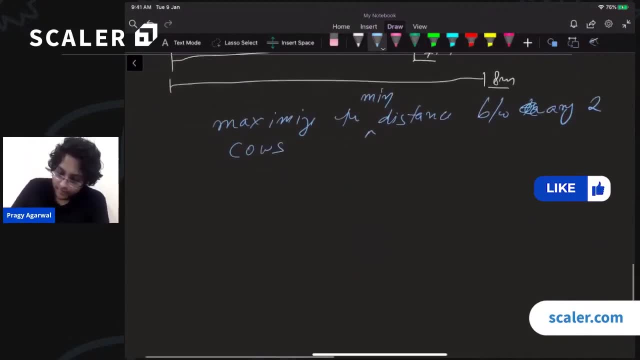 three meters apart from each other. any pair of cows is three meters apart from each other. all right, perfect. so now the question is that, given, you have been given n, you have been given c and you have been given the location of these n stalls, right and right, and you have to tell me. you have to tell me. 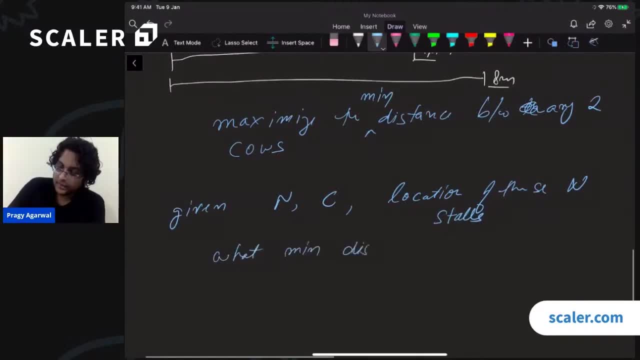 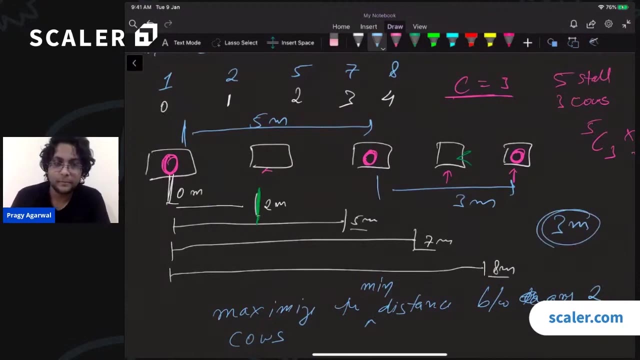 what minimum distance? minimum distance can you achieve? can you achieve by placing the cows as far apart as possible in the different slots? i hope the question is clear. so basically, if this is the input, you have to give me the output three meters. right, you have to give me the output three. 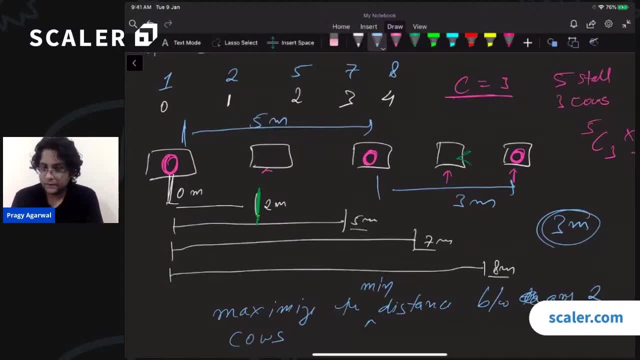 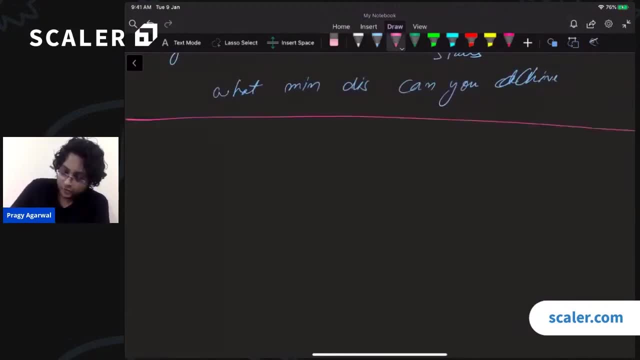 all right now. how will we do this? how can we do this? we have to know the minimum distance, please understand. the minimum distance means minus. all right now. how will we do this? how can we do this? So, once again, let us start with a very, very brute force approach. 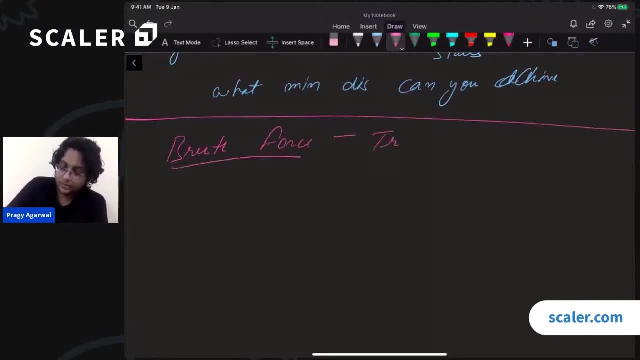 The brute force approach would be to try all possible, try all possible arrangements of the cows, try all possible arrangements. So, as we just saw, so are the cows distinguishable. in this particular case, Does it really matter what the first cow, second cow and third cow is? 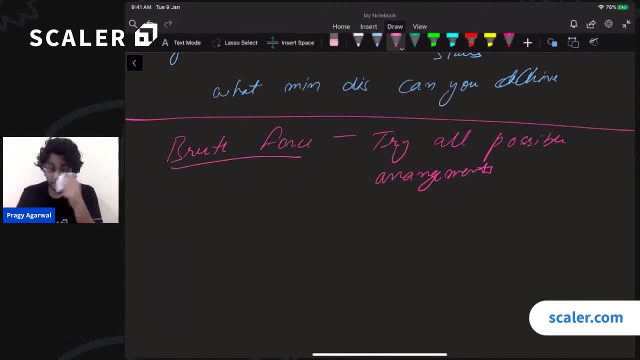 No, it does not. All that matters is what stalls they are in. So, over here, how many possibilities do we have? We have five. see three possibilities, right? or basically, we have n- choose n, choose c possibilities, where n is the number of stalls and c is the number of cows. 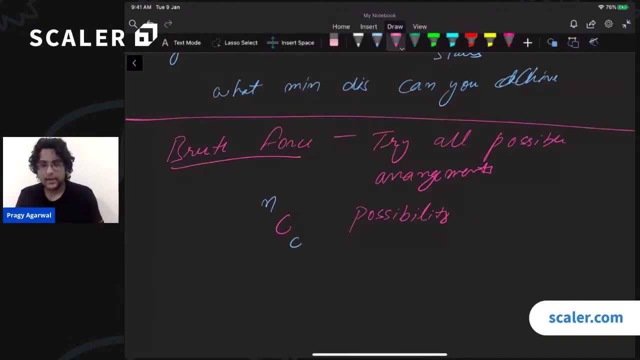 So if we, if we do this brute force, we will check each of the possibilities And then for each possibility we will find the minimum distance. right, we will find the minimum distance. So what will be the overall time complexity of this brute force approach? 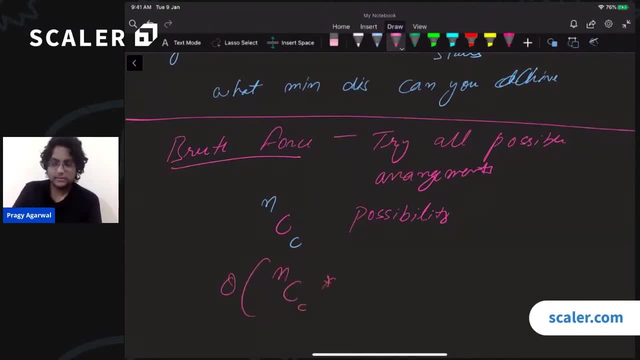 It will be order of n choose c times. So once we have chosen an arrangement, we still have to calculate. so let us say that we have several stalls and we have chosen to put one cow here, one cow here and one cow here. 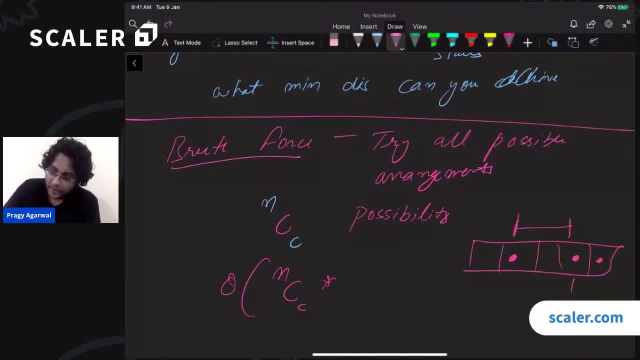 That is not done right. We still have to measure these distances and find the minimum distance between any pair of cows. So that will take us an additional of order of n time because we have to go through every pair of cows Right. 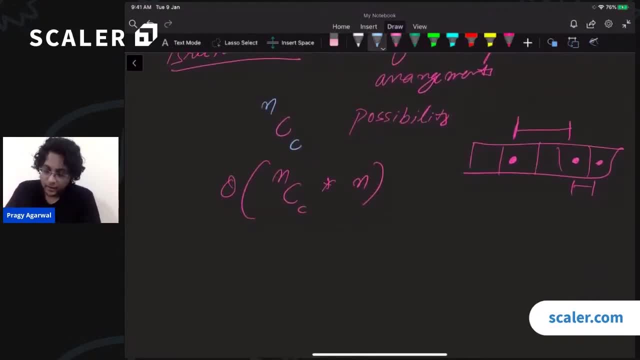 So the total of time complexity will be n choose c times n. Well, how big is n choose c? Can someone tell me how big n choose c is in terms of o n complexity? So what polynomial n to the power? what will it approximately be? 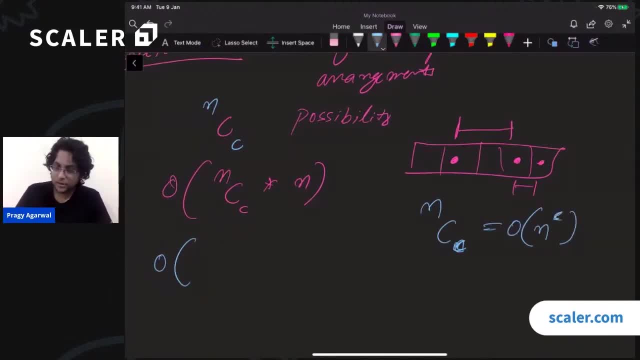 This is the same as n to the power c. right n choose c is the same order as n to the power c. Yes, No, Yes, No. Well, not really, Not really, because binomials flip. From the midpoint, the binomials flip. 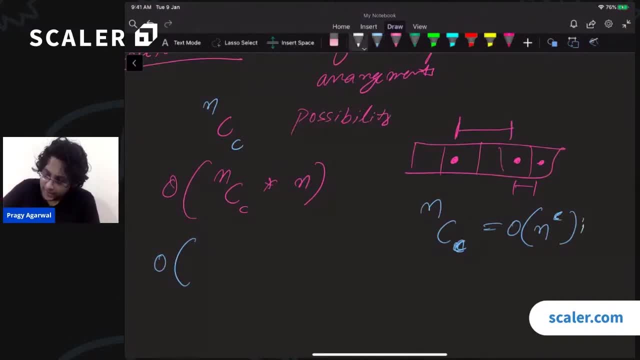 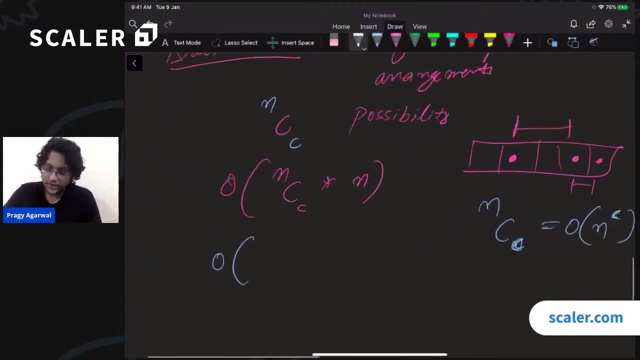 Right, So we are assuming. so this is: if c is less than n by 2, right, c is less than n by 2.. So we can rewrite this as so. let us not, let us not write this complex expression. 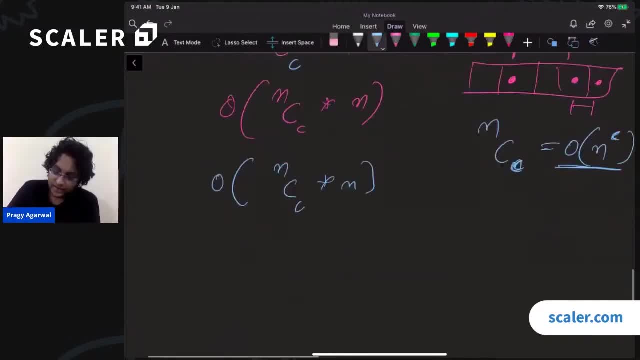 Let us just keep this as n choose c times n, And this is in the worst case. in the worst case, this is equal to order of n to the power. c times n. Right Now, if c is very big, if the number of cows is very big, this complexity is perhaps not. 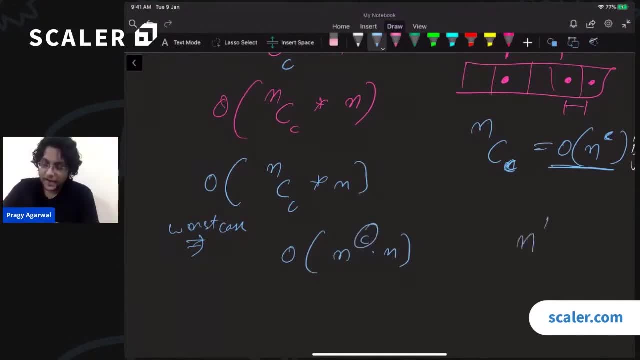 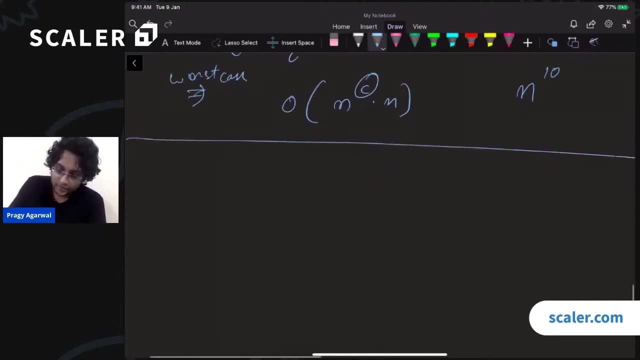 that big Right. If there are 10 cows, then you will have to spend n to the power 10 times. That is very, very bad Right. So let us try to optimize this approach for you. Let us try to optimize this. 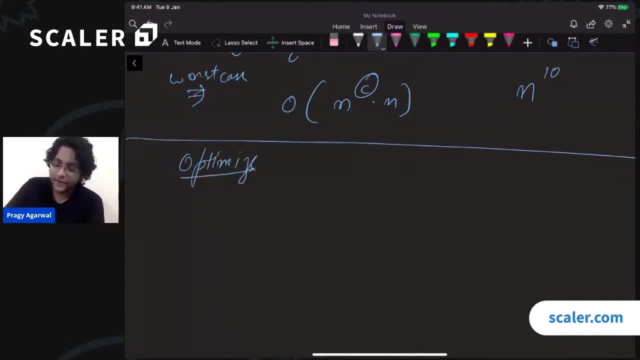 Okay, So those of you who are familiar with dynamic programming, who are familiar with dynamic programming, what would you try to do over here? What would you try to do over here? So anyone who is familiar with dynamic programming would say this: that all right. 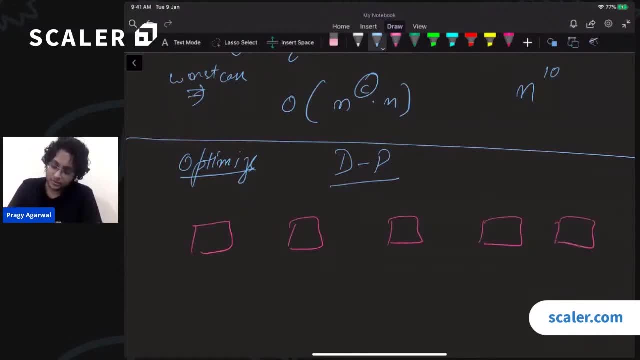 I have several stalls and I have some cows. Right, I have several stalls and I have some cows. That is simple. right. For every stall. I have to make a yes- no decision. I have to make a yes- no decision whether to put this cow in there or whether to not. 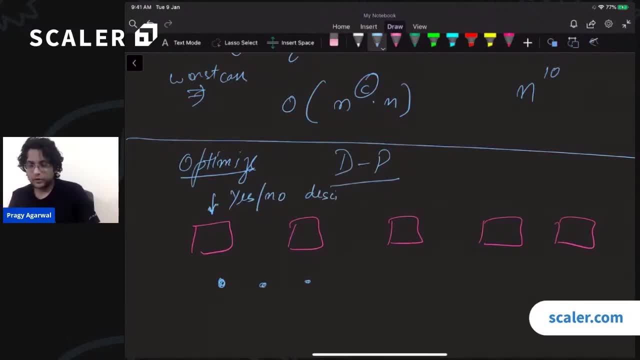 put this cow in there, Right? So people would try to apply DP over here and say that okay, for the first stall, I can choose whether I am going to put the cow in or I am not going to put the cow in. 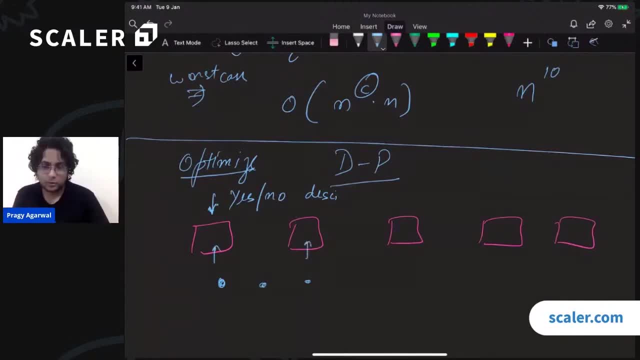 Again for the second stall. I am going to choose whether to put the cow in or not. Okay, And so on and so forth. I will build my choices And by DP I can finally find the answer. Well, that is perfectly valid. 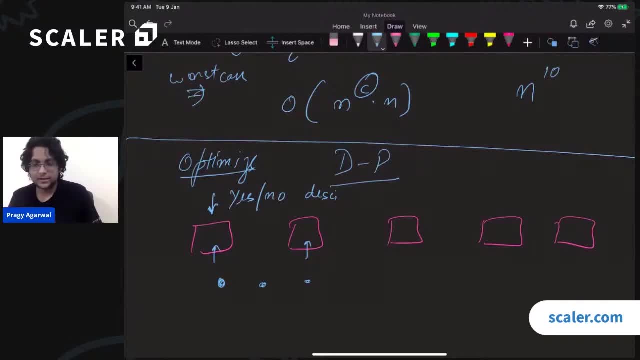 Right, That is perfectly valid. And if you do that, if you do that, your complexity will turn out to the order of n squared, which is not bad right, Which is definitely better than the order of n to the power c times n. 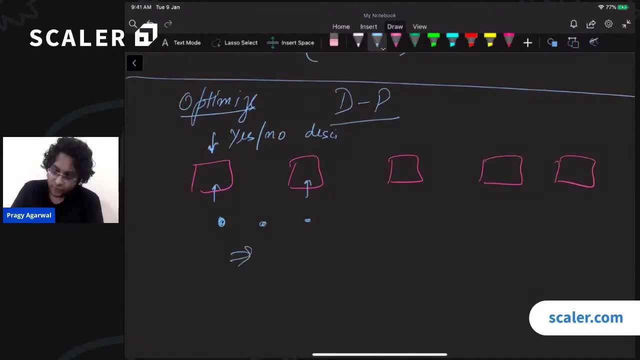 But we can do better, But we can do better. So the moral of this story is that, even if you have come up with a solution, it is important to know that it is not going to be an easy task And you are going to have to do it. 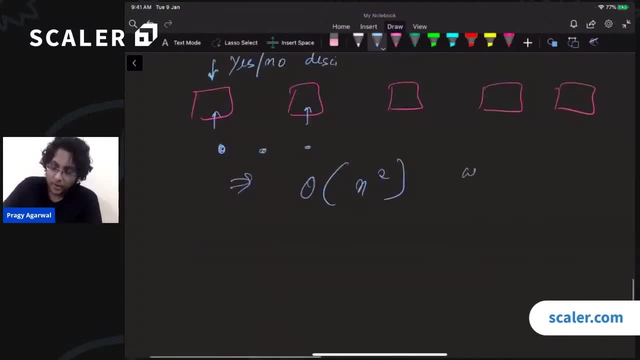 And you are going to have to do it, You are going to have to do it, And you are going to have to do it, And you are going to have to do it. this story is that, even if you have come up with a solution, it is still worth. 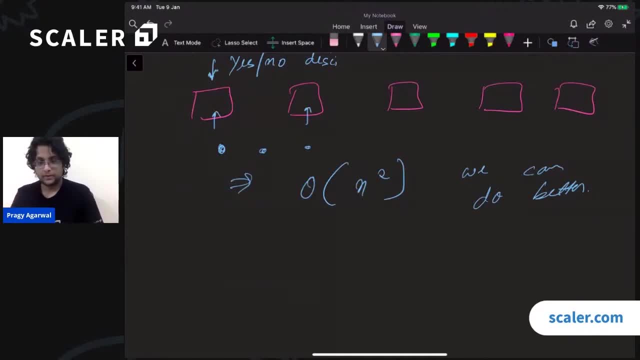 checking if the solution can be optimized or not. all right now let us dive into the most optimized approach, which will be using binary search. binary search- perfect. so if you are supposed to use binary search, we have to have a search base. we have to have a search base. we basically have to decide what we 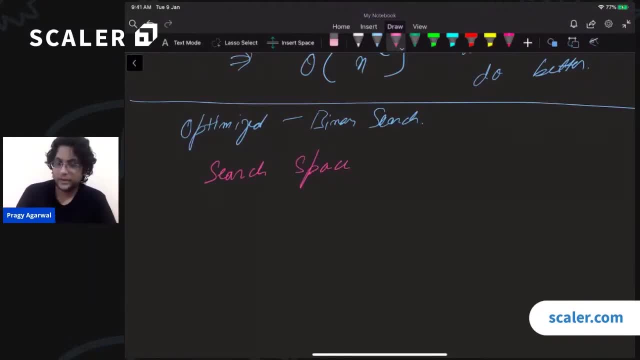 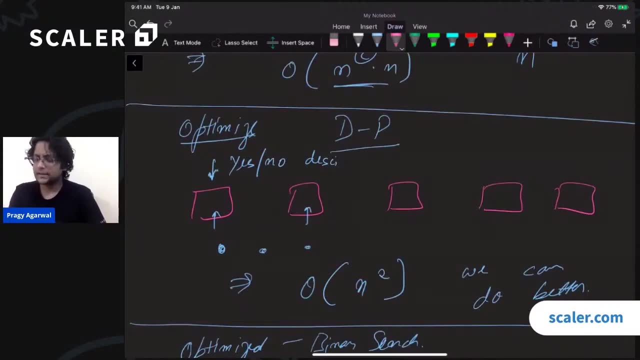 are searching for. what are we really searching for over here? can we search for the location of stalls? can we search for the location of stalls? that does not really make sense, right? because we have to consider multiple stores and there are multiple cows. so how? it doesn't really. 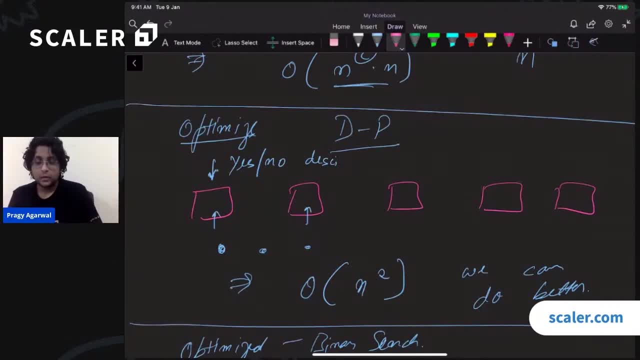 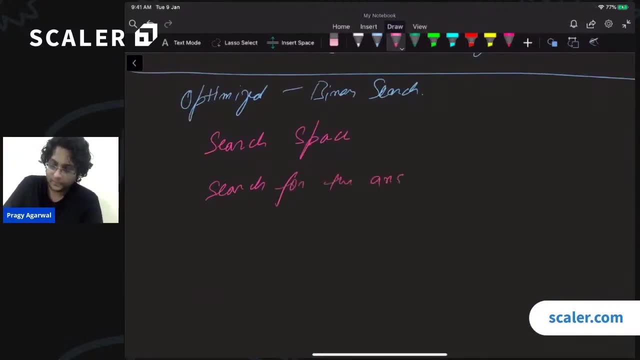 make sense to search for the location of a particular stall. what we can search for is the answer itself. we can search for the answer itself, right? so what is the answer? what we know the answer is the minimum distance. the answer is the minimum distance, and we are trying to maximize this particular answer. minimum distance between any two. 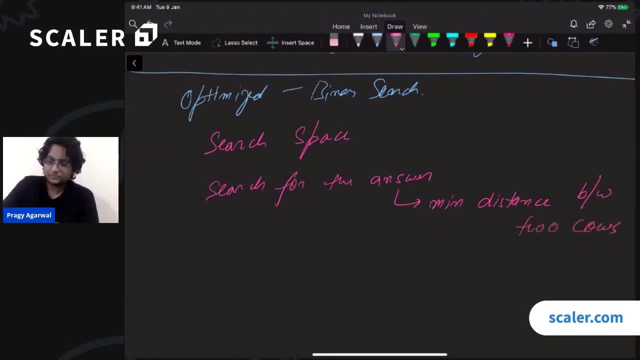 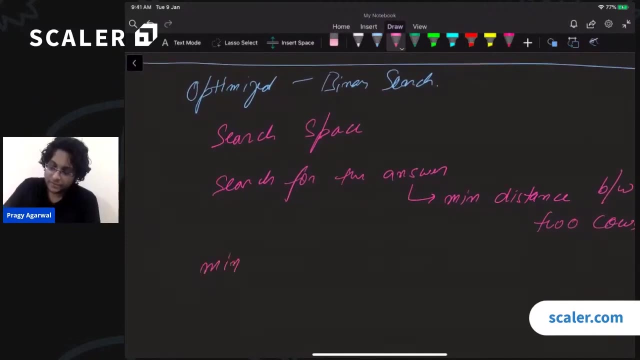 cows between two cows, all right. so now that we have figured out what we have to search over, let us quickly discuss the bounds, let us quickly discuss how large this search space is. so what is the? what is the minimum value for this minimum distance? what is the least possible distance that we can achieve? 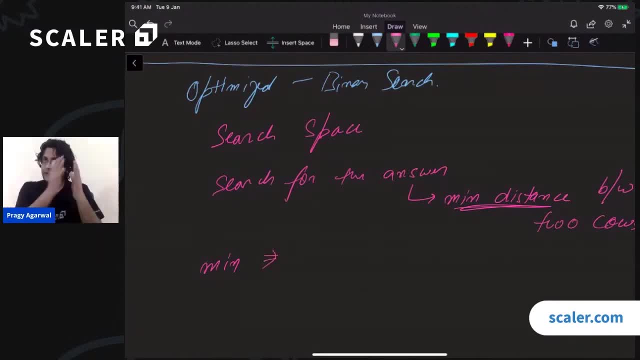 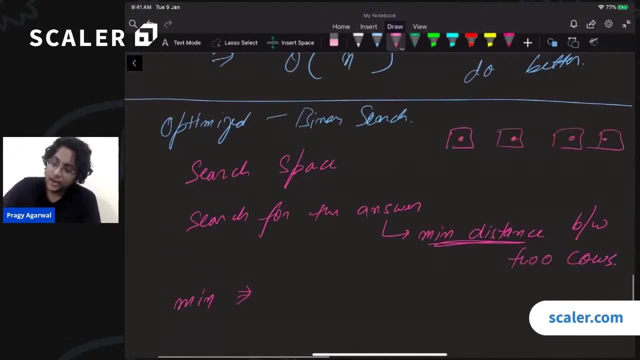 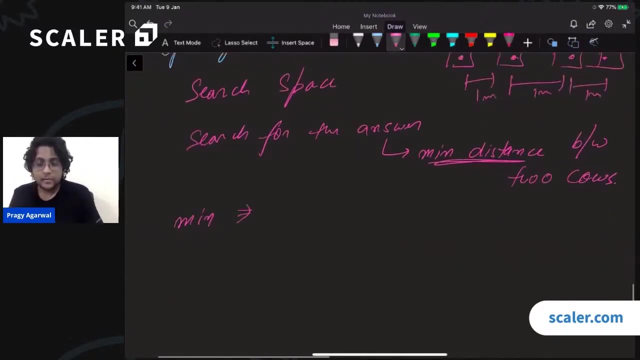 what is the least possible distance when we can achieve? well, if every, if every stall, if we are forced to put one cow in every stall and every stall is one meter apart, right, so they're just next next to with each other, they're just next to each other, then the minimum distance will be just one. do you agree? can the? 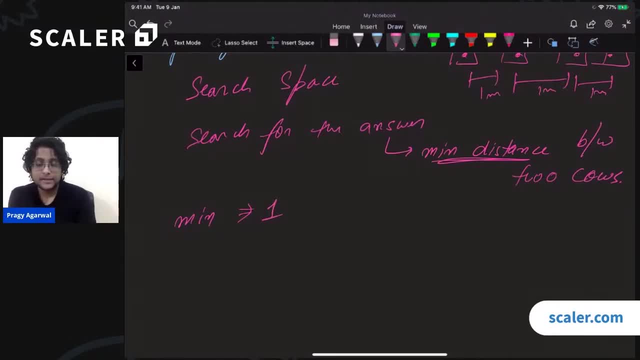 minimum distance be zero. can the minimum distance be zero? not really, right, not really. what is the maximum possible distance that we can achieve? what is the maximum possible distance that we can achieve? well, this is my first stall. this is my zero. it's stall is at location zero. all right, and let us say my nth stall, my n minus one. 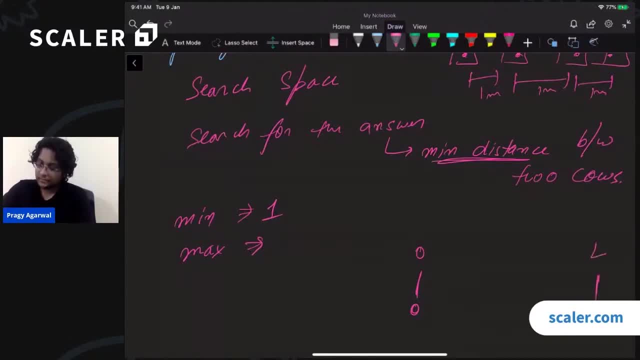 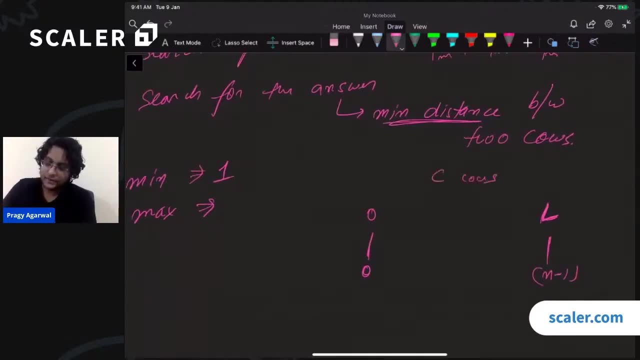 it's stall right, let us say it is at location. let us say: L all right, and I have to place C cows. I have to place C different cows within this distance. so in the worst case, I mean even in the best case, doesn't matter how the stalls are arranged, can I, can I achieve what is the best distance that I? 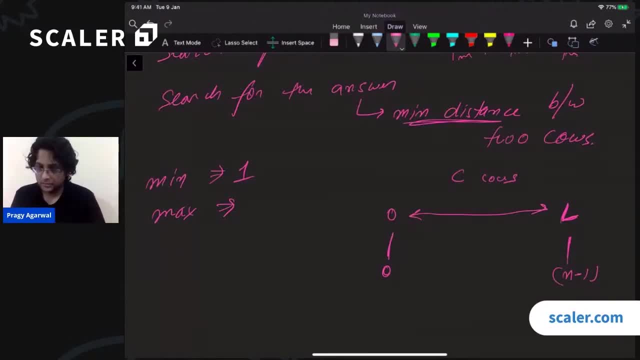 can achieve if all the stalls are equidistant from each other. if all the stalls are equidistant from each other, then I can simply place the cows one in each of them right, and then basically, my distance will be L by C right. this is the. 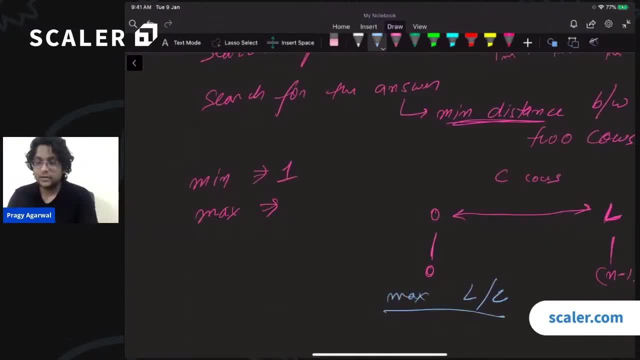 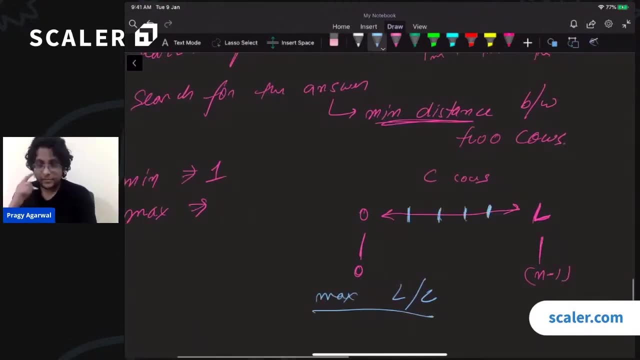 maximum possible distance I can achieve. can I achieve more than that? can I possibly get more than that? no, because once I have placed the cows at equidistant locations, once I have placed the cows at equidistant locations, if I try to move any cow to the left or right, if I try to move any cow to the left or right, then 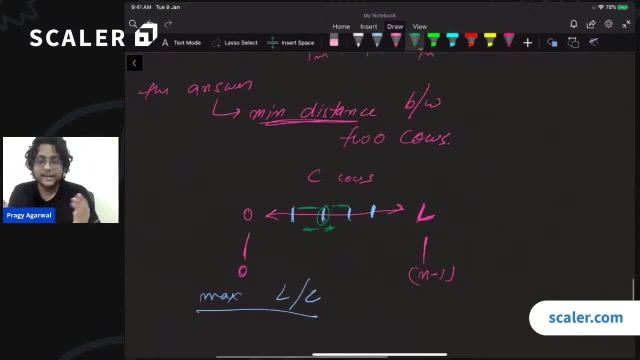 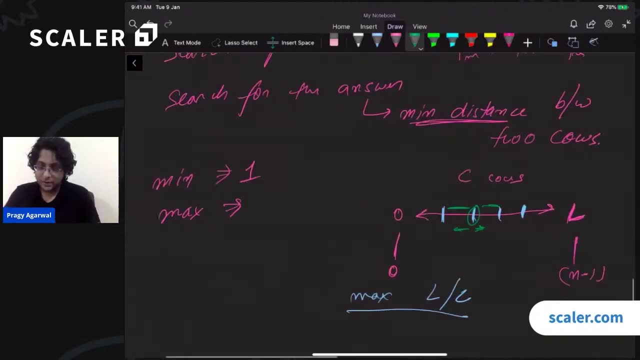 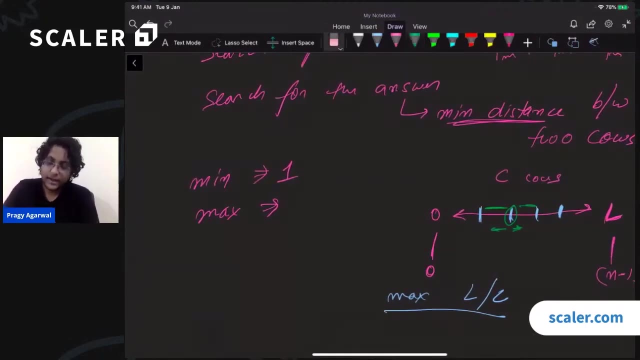 though the distance between the previous cow or the next cow just decreases, and we are supposed to consider the minimum distance between any pair of cows. so the maximum possible distancespeedle BS that we can achieve possibly is L by C, And what is L over here? L is simply the maximum. 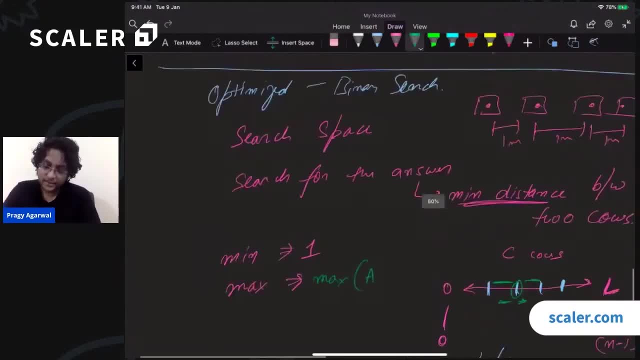 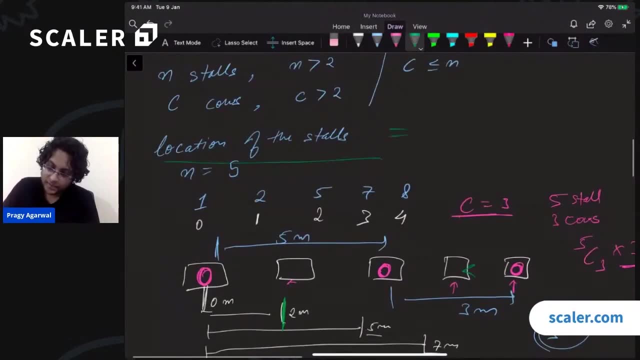 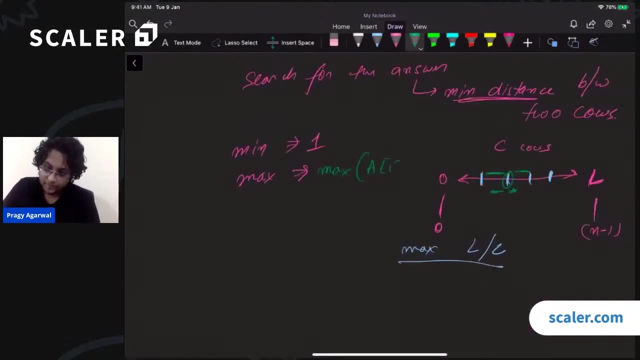 of the array. So let us consider that these distances are given to us in the array. So this location of the stalls, this has been given to us in array of size N. So this is simply max of A, max of A for all A. So we now have the bound, We now know that we are. 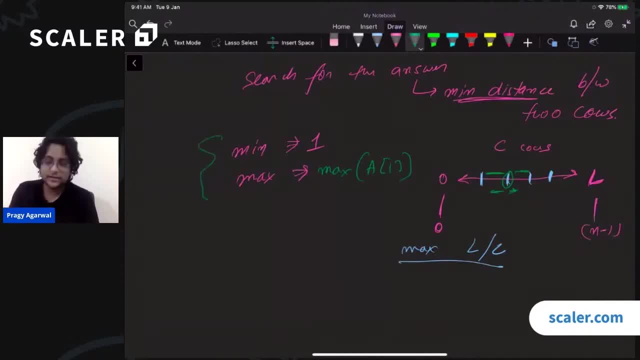 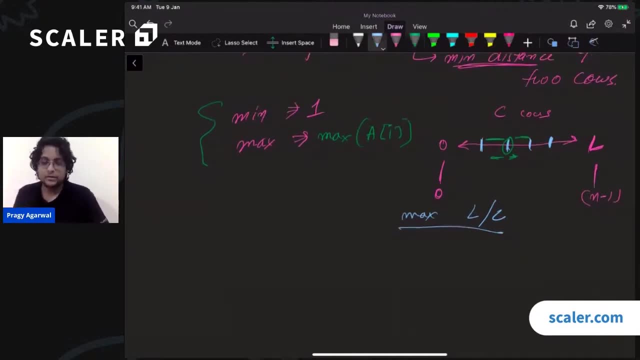 supposed to look for a value in this search space? This search space goes from all the way to max of A of I. Now, what else is required for a binary search? What else is required for a binary search? So, now that I have a low and a high, I have a low and a high. I. 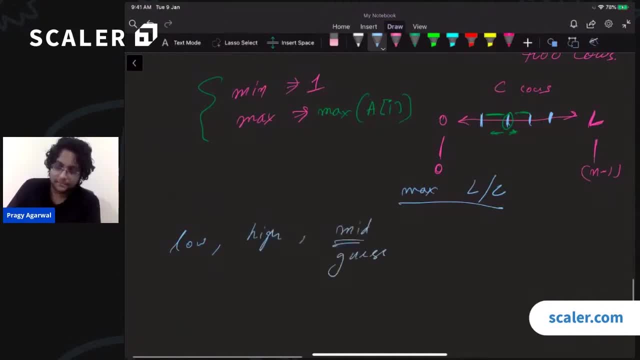 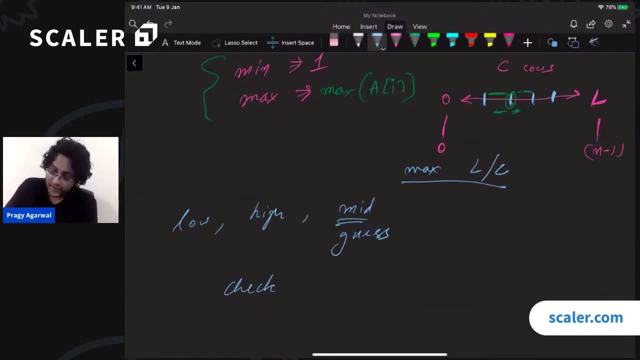 will calculate a mid And this mid is going to be my value. This mid is going to be my guess. Now I have to check. I have to check several things. I have to check: is the guess perfect, Is the guess valid And is this the correct answer? 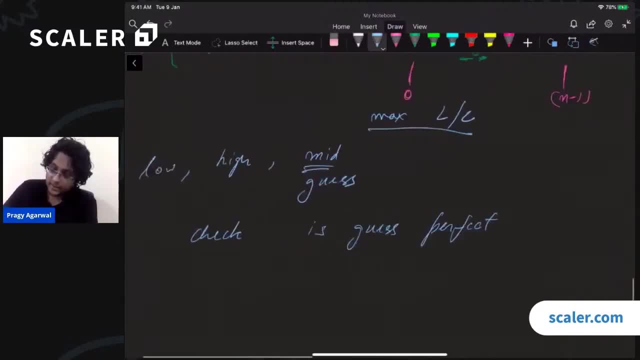 That is one thing I have to check. Or I have to check is the guess too low, Or I have to check: is the guess too high? Because only if I know all these three things, only if I know these three things, answer to these three things, only then can i adjust my search space. do we agree? yes, exactly. 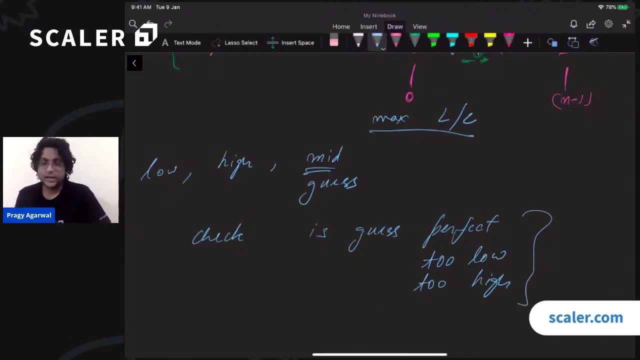 we need a proposition, right? if i don't have these three values, i will not be able to figure out in which direction should i move in the search space. all right, so let us, let us quickly look at how we will do that. so suppose that i tell you, suppose that i have. you have been given this array, a of 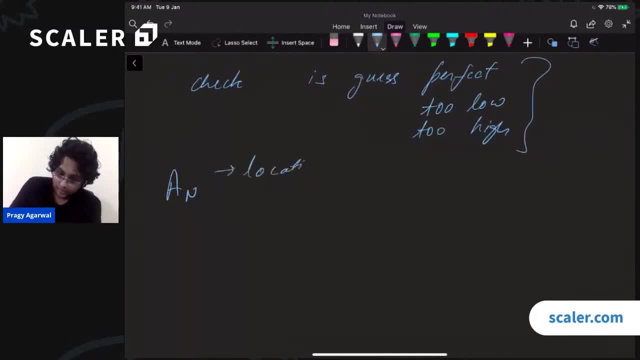 n, size n, and this is the location of stalls, location of stalls, and i am telling you that, okay, you can achieve a distance. you can achieve a distance of, let us say, five meters. right, we have to verify whether this is true or not. so how will we verify that? how can we verify? 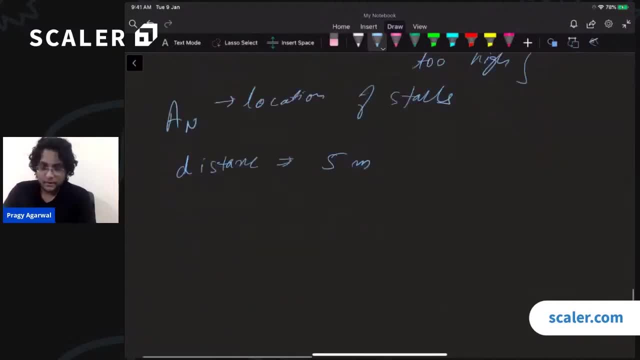 that, well, this is very simple, right? this is very simple. what we can do is so: let us suppose that these are the stalls, right? and let us suppose that this is our location zero. this is our location. five. this is our location. seven, location, eleven, location or sixty. 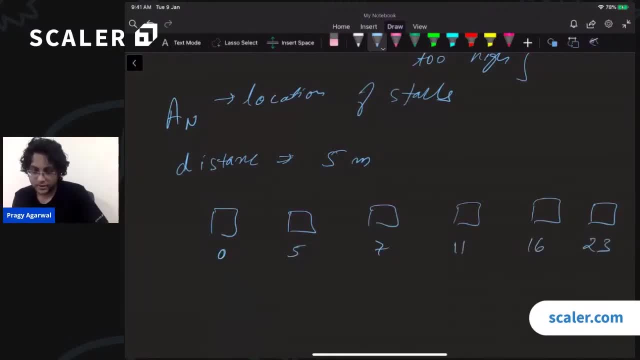 location twenty three, let us suppose these is how this falls. so what we can do is we can place the first cow in here. right, we can always place the first cow in the first one, then we can move on to the next one and we can check what is the current distance. what is the current distance? 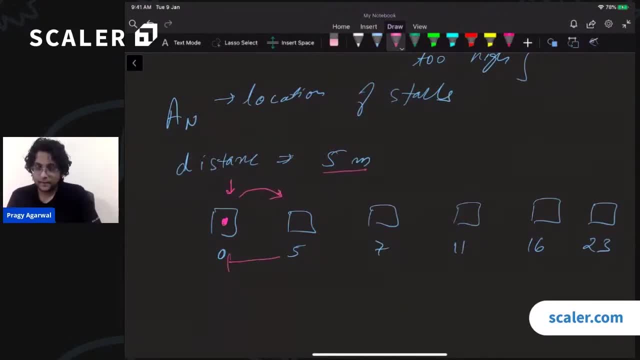 is that distance greater than or equal to five? yes, it is right, so we can see if it is the next cow over here, because we are trying to achieve a distance of at least five. we're trying to achieve a distance of five meters. all right, then we can move on. so when we want to put the third cow, we 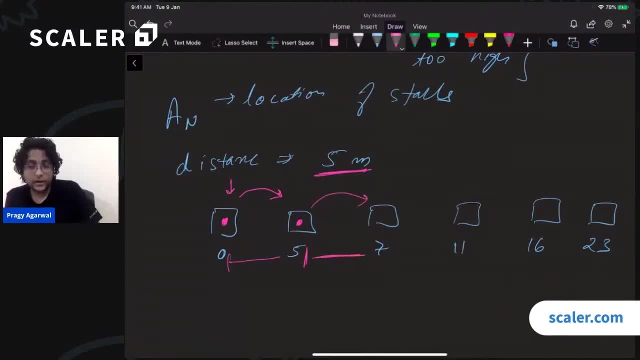 will come to the next one and check: is the distance from the previous cow greater than or equal to five? so is seven minus five greater than or equal to five? no, it is not right. so we cannot. if we have placed the cow in this stall and we are trying to achieve a distance of five meters, then we 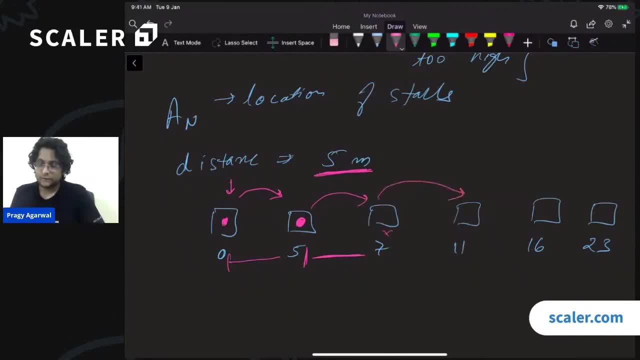 cannot put the next cow in this one, all right. what about the next one? well, the distance from five till eleven is six, so we can safely place the next cow over here. does that make sense? moving on, so we can definitely place the next cow over here and we can also place the next cow over here. right, so we can place the cows in this particular manner. 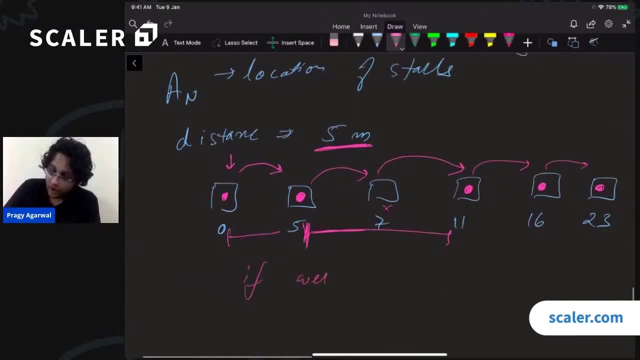 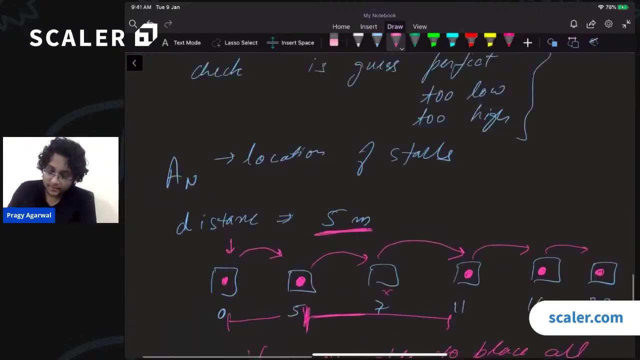 now, if, if we are, we are able to place all the cows, to place all the cows successfully, right. so remember that we have sea cows, right. if we are, if we are able to place all the sea cows successfully and save the 후보 in the right time, then we can also place the next cow on the left moment. 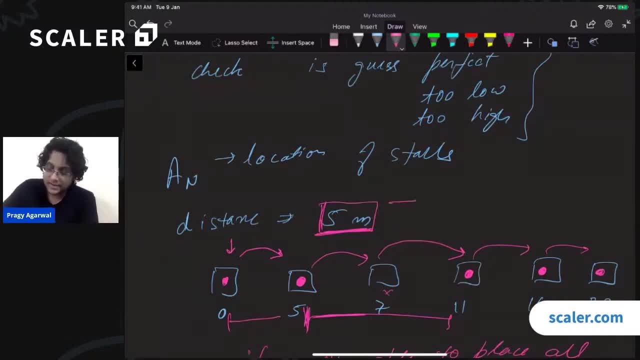 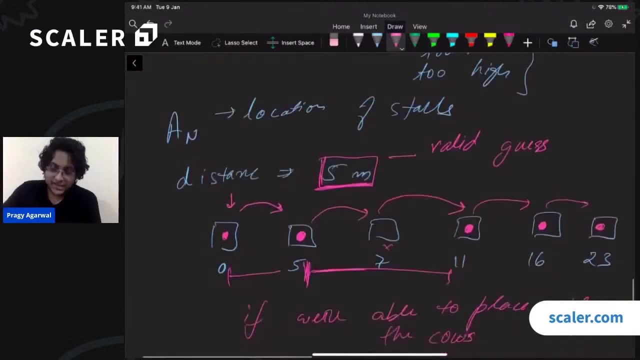 now in this situation, that means this first gray cow goes to the left and we are supposed to place the final cow at the left moment. and now, what you have to keep in mind is that we have many different animals on our sector right. we have different things to do, so there are many. 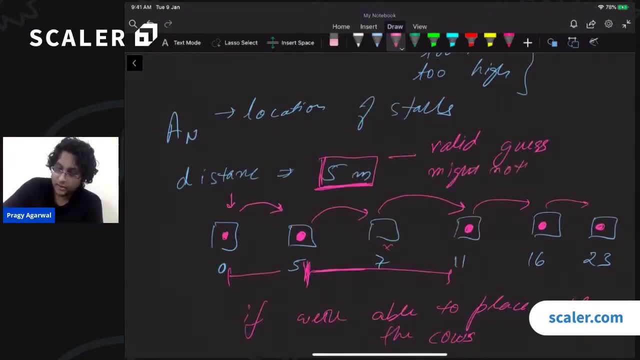 different tools available and one tool we can use to do this, which is the index, add a very criticaluperinkles, and there are many other tools available in the market, or there are many issues available to us that to be engaged in, which are useful and useful things for us. so as it continues. 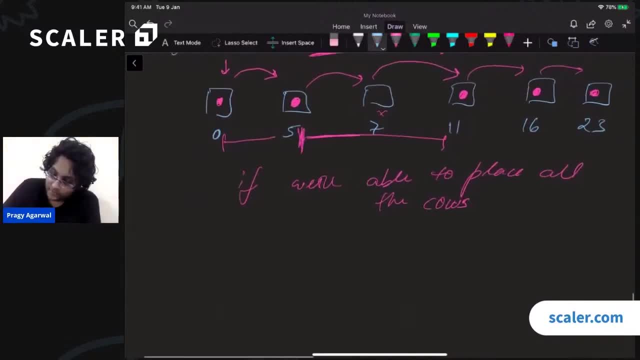 Suppose that we were not. so if this, if we were able to place it, then we have a valid distance By a distance, but the distance can be higher, can be higher, All right. What is the other possibility? The other possibility is we were not able. 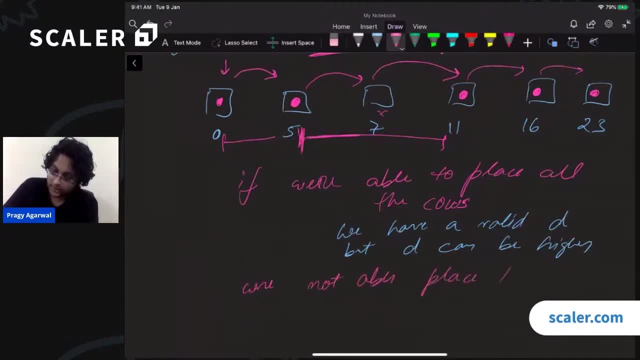 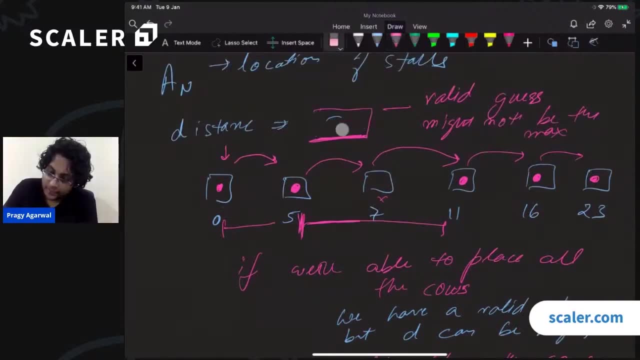 Were not able to place all the cups. To place the cups right, For example. suppose over here, suppose over here. Oh, let us suppose that my distance was my estimate. my guess distance was So just if you just erase this. So let us say that my guess was that, okay, I can achieve a distance of 10 meters. 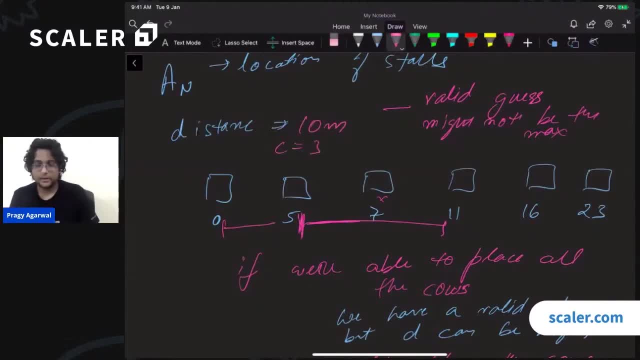 Right, And let us suppose that I had three cups to put. I had three cows, So I will try to put the first cow in this first one. Then I cannot put the second coin, the second stall or in the third stone. I will have to put the second cow over here. 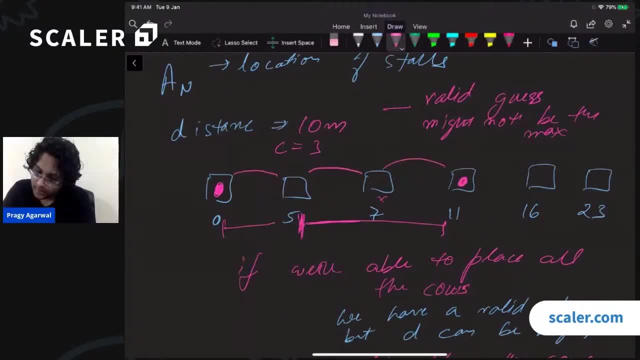 Right, I will have to go In this case. it will be more so Let us let us just say that we had four cups. Let us say that we had four cups, So I will put the second cow in this time. Then I can't put the third cow here. I can put the third cow here, So I will put the third cow over here. 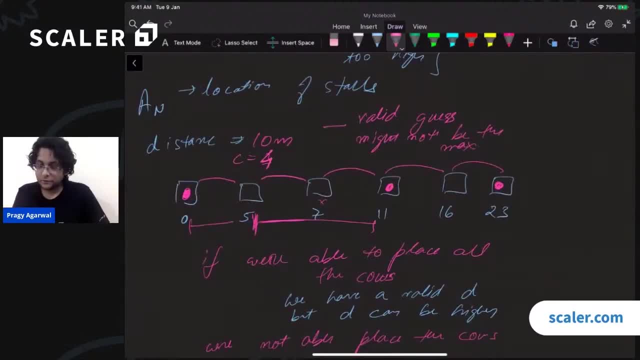 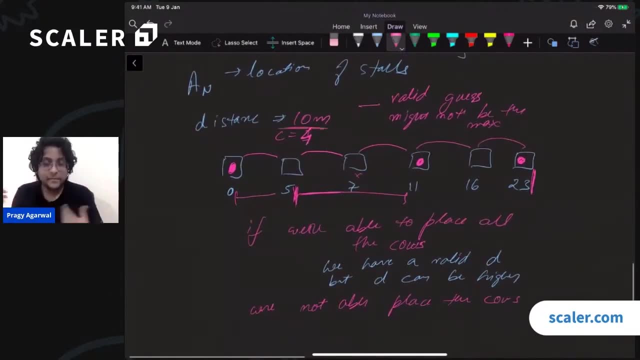 Now, where do I put this fourth, fourth cup? I cannot possibly put the fourth cup because I have exhausted all my stalls right. so in this case We see that we had a guess of 10 meters distance And we try to place the four cows, But we were not able to place all the four cups. 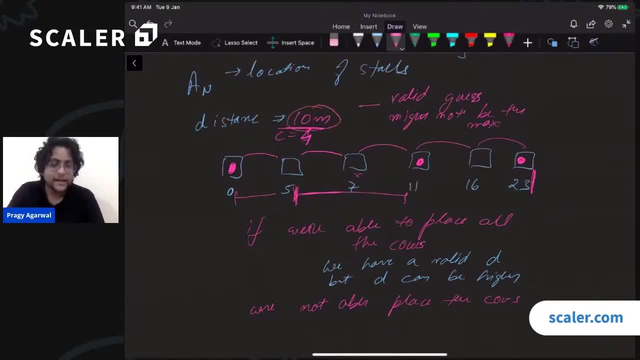 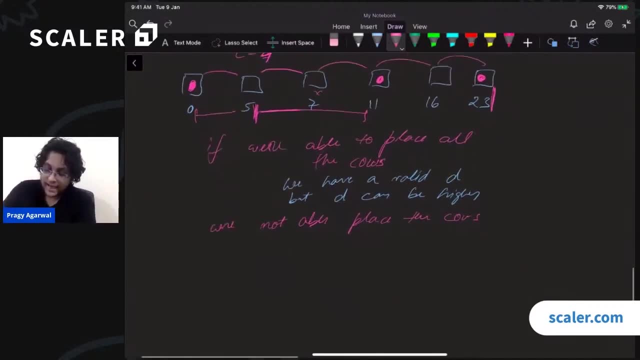 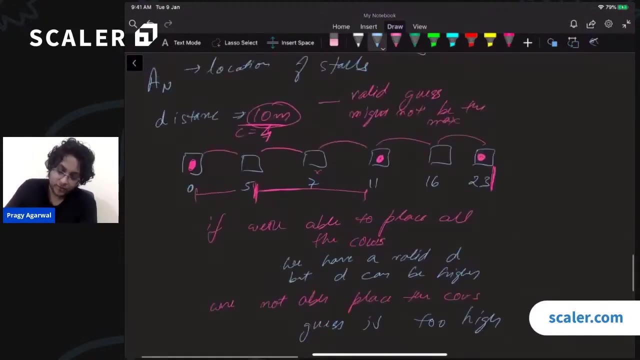 only able to place three cups. So that means that my guess is incorrect, Right, That means that my guess is incorrect. Is there anything else that I know? Is there anything else that I know? I know that my guess is too high, Right, If 10 meters did not work. if 10 meters did not work, then 12. 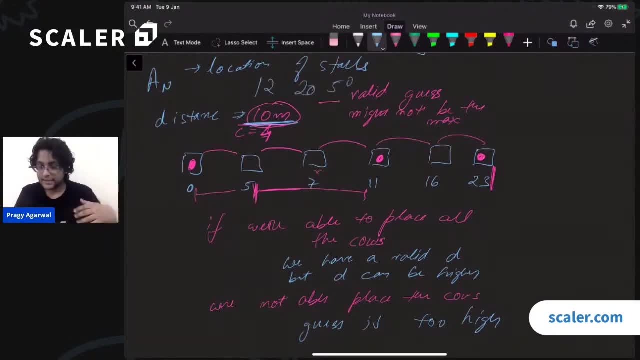 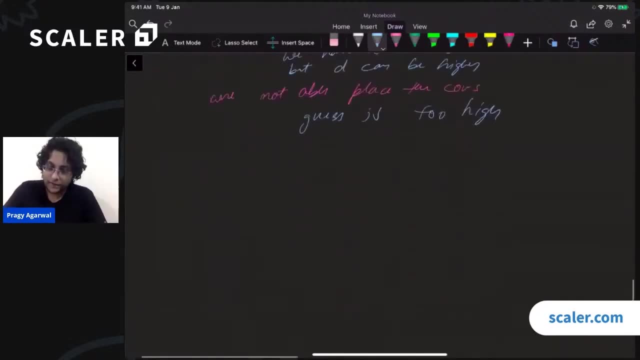 meters or 20 meters or 50 meters will also not work. My guess is too high. I have to reduce my guess. Does that make sense, guys? Yes, So what we are essentially doing is we are saying that let us initialize the low as 1, the high as l by c. So this is maximum of a of i Right, So maximum. 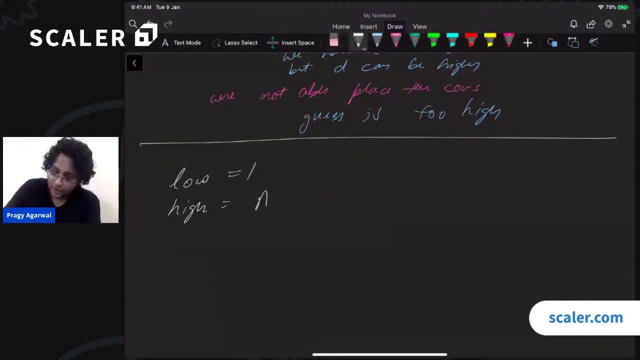 of a of a is just the last location, the location of the last of a of a dot length, or n minus 1.. a of n minus 1 by the number of cows c, Then, while our low is less than equal to high, what we will do is we will calculate a mid. So 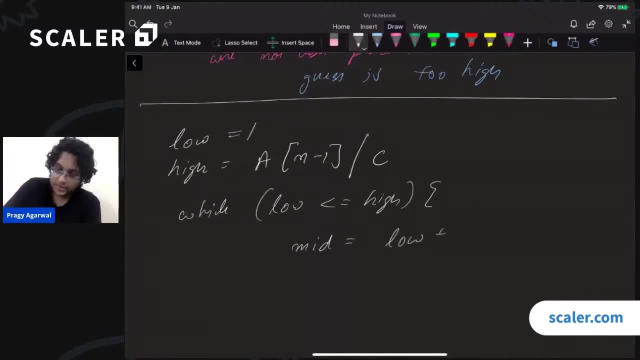 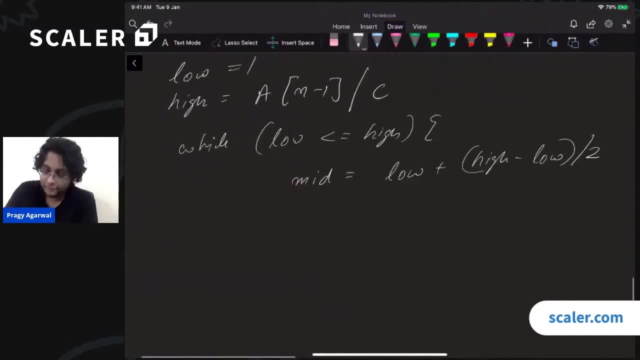 our guess is the mid, which is simply low plus high, minus low by 2.. Do you agree? Now we have to verify the guess. So if works, if this array for this number of cows, for this value, for this guess, if this works, so we will write this function works. 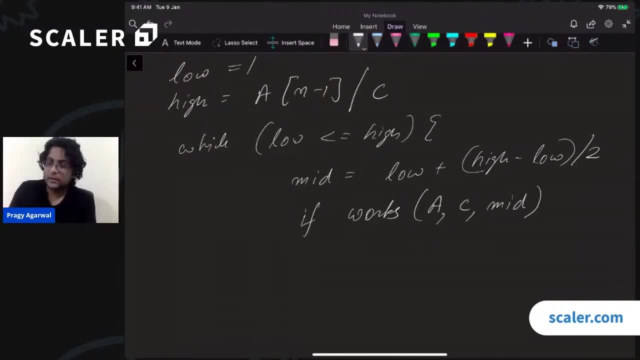 But if this works, then what can we say? If this particular thing works, then what can we say? We can say that, hey, this guess is valid, but it might be too low. This guess is valid, but we could be. we could be doing, we could do better. So we have to increase, we have to increase our guess. 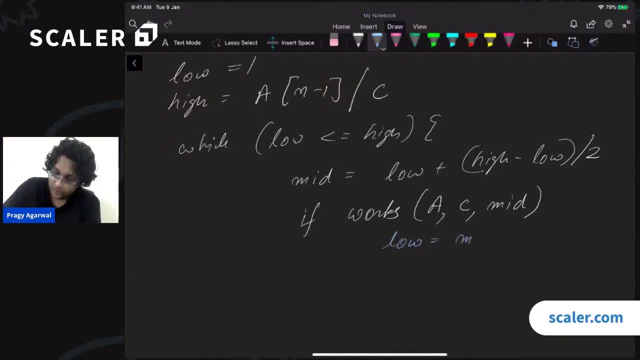 Right, How will we increase our guess? We will say: low equals to mid plus 1.. Right, But this guess works, So we must also save it, right? This was the largest guess that worked, So let me also save a variable over here. largest working guess- right, Let me save a variable. 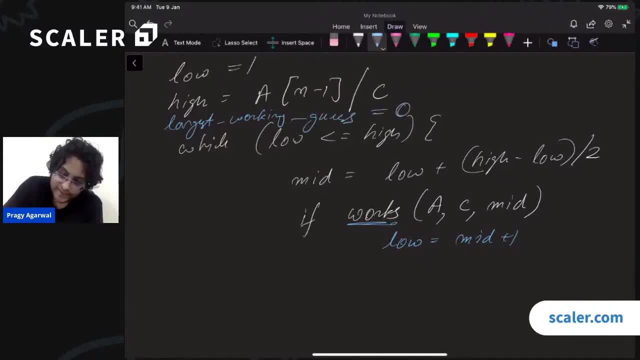 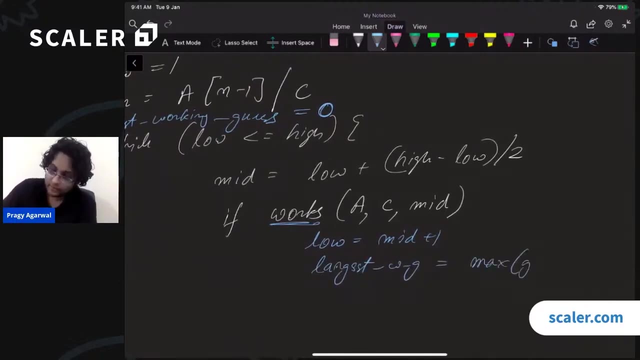 over here, largest working guess, And this was initialized with, let's say, zero or minus, infinity, whatever you want, And I can see over here that largest working guess. largest working guess equals to maximum of my guess, my mid, So it is maximum of mid, the current guess comma, the largest working guess. alright, 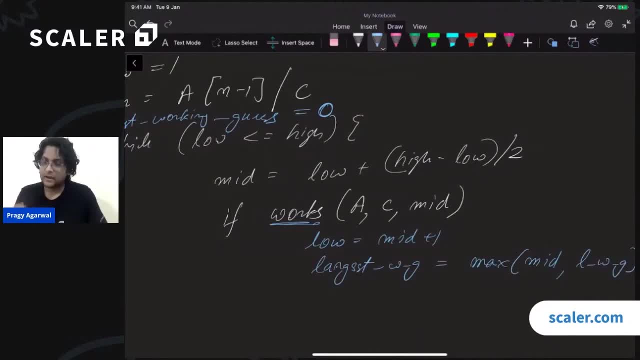 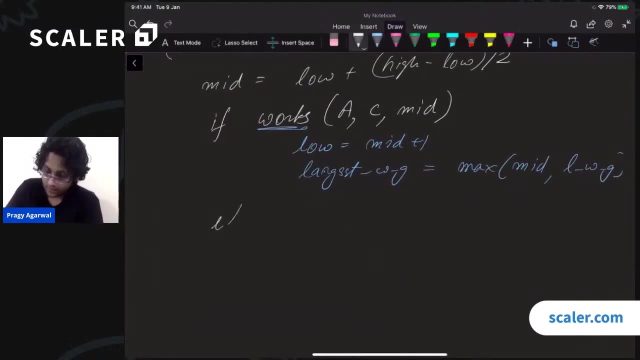 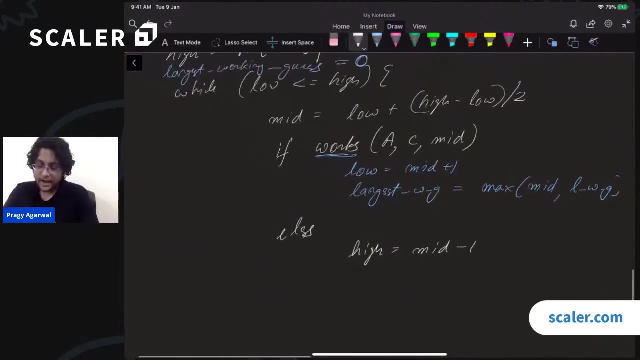 I can make sure that whenever I have a valid guess, I save the largest of those valid guess. Is that clear? On the other hand, if this does not work, if this does not work, then I have to adjust my high High equals to mid minus 1, right. 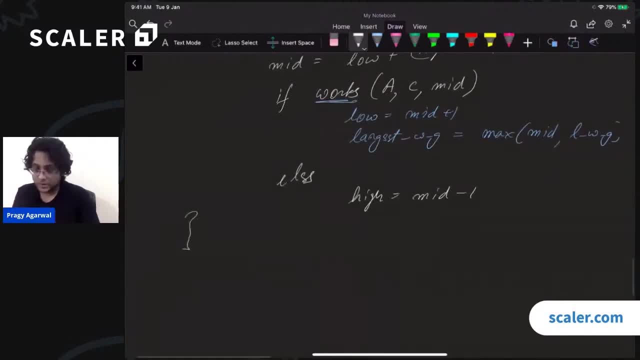 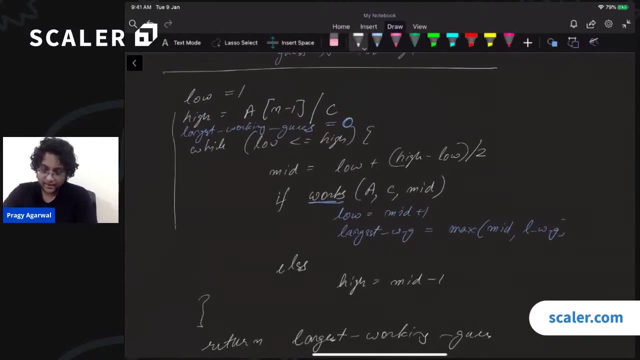 And at the end of this loop, at the end of this loop, when this loop is through, I can simply return whatever maximum guess I have found so far, So largest working guess. Does that make sense, guys? Does this binary search make sense? 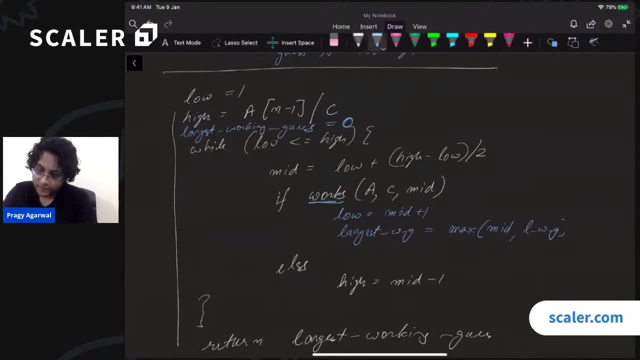 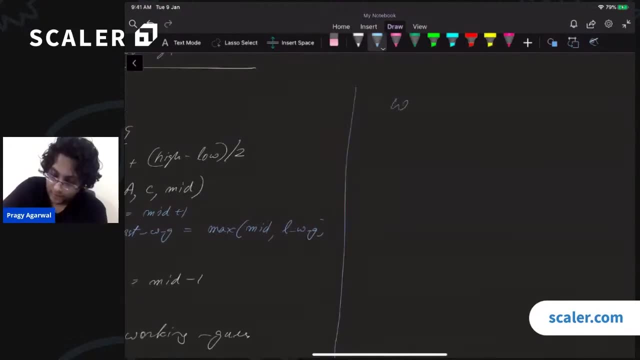 Yes, We still have to write this function. right, We still have to write this works function. Well, this function is very simple, as we saw. How will this function work? So we have to write works. this will take an array. this will take the number of cows. 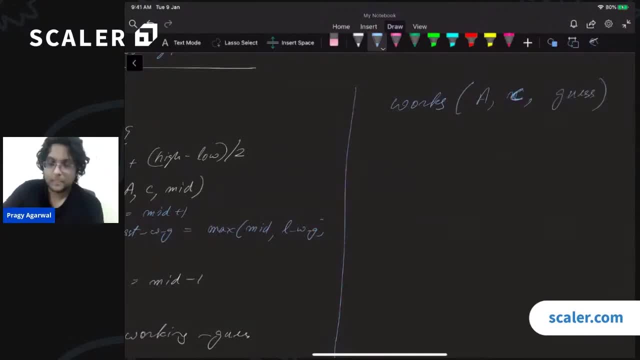 this will take the number of cows and it will take a guess. So what will we do? What will we do? We will start from the location first. right, we will say that the previous stall, previous stall, equals to zero. right, we will place the first cow at location zero. 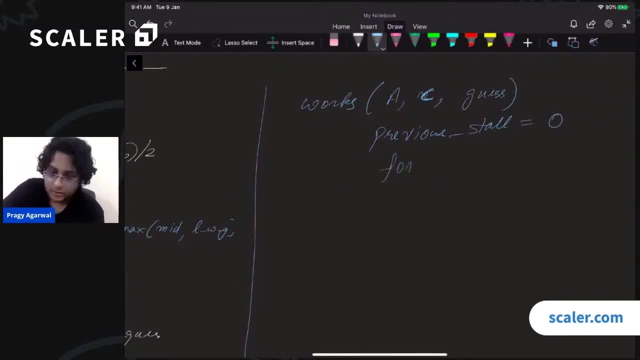 Now, how many cows do we have to place now? So for for i goes from, i goes from 1 to 0.. Okay, We have already placed the 0th cow. now we have c-1 cows remaining to place, so we will. 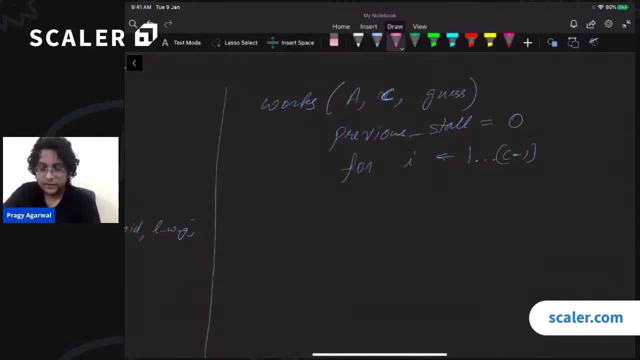 go over each cow, and then what will we do? We'll, what will we do? We will try to place the cow in the next one, So we will also. let me also save a stall number over here. So stall number is 1, I have already used up the stall number 0.. 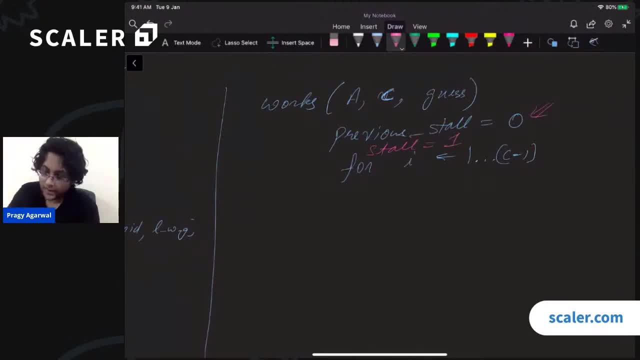 So the current stall number is 1.. Okay, So now what can I do is I can try to. I can try to put this, put the cow in over So I can say: while while the location of the current stall, right while a of stall. 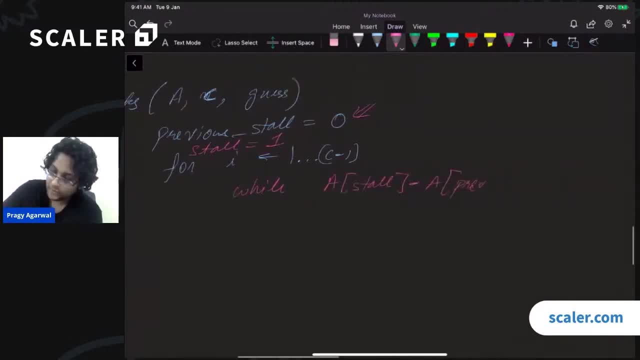 minus a of previous stall, previous stall, if this distance, while this distance is less than my guess, while this distance is less than my guess, I cannot really put this cow in the current stall right. So I must move on to the next stall stall++. 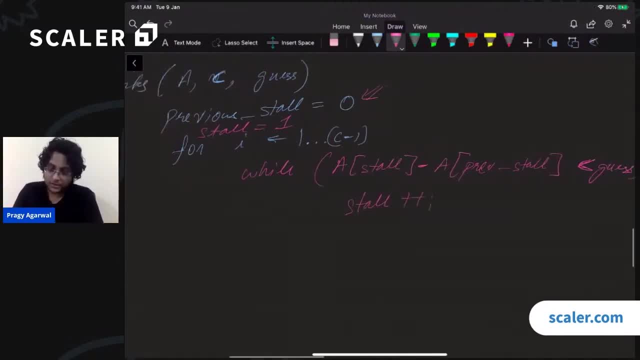 Do you guys agree? While this is true, I will do stall++ right And finally I will say that, all right, once I have this, I will say: previous stall: stall equals to stall, So I will put the cow in there. I will put the cow in there. 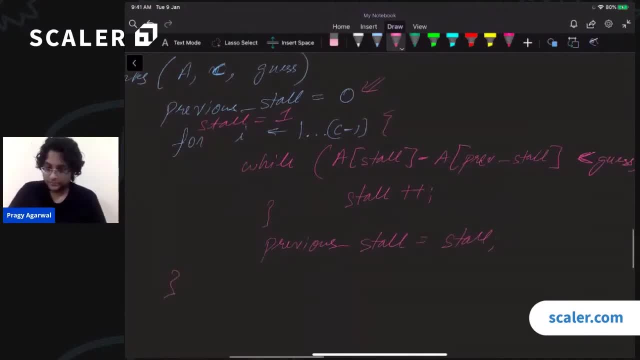 So this is my loop. Now, of course, this loop might not always work, right, this loop might not always work. Basically, when will it fail? When will it fail? When will it fail? When my stall number has become equal to the, equal to the size of the array? 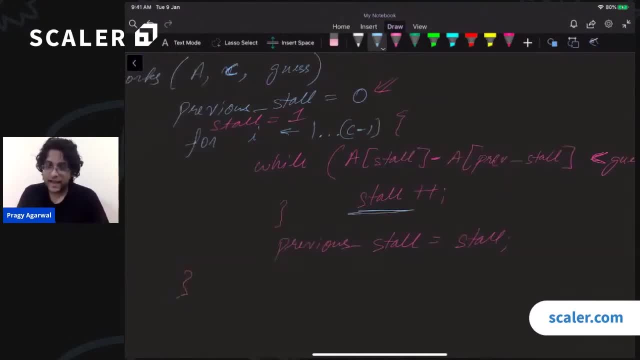 Okay, Okay, When I have reached the last stall, or size of the array, when I have reached the last stall, but my cows have still not been finished. right, my cows have still not been finished. So I can put a condition over here. I can very quickly check over here. 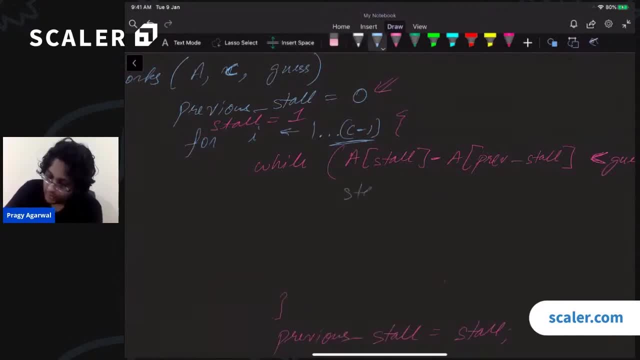 So, instead of directly doing this stall++, let me do a stall++. And now I can check if stall equals to equals to n. If I have already reached the last stall, then I can return false. return false Because this guess did not work. 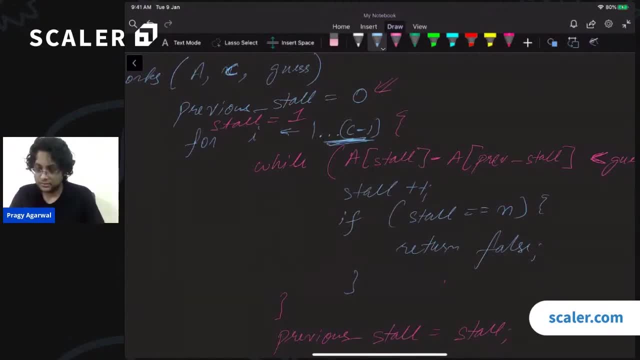 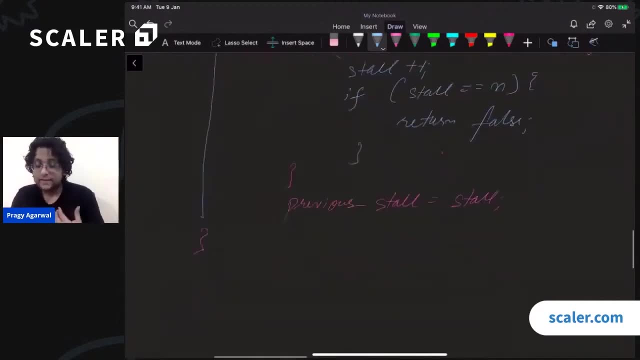 I still have some cows to place, but I have exhausted my stalls, right, So I will return false that, hey, this guess does not work. If I can complete this formula, that means that I was able to place all the three different cows. 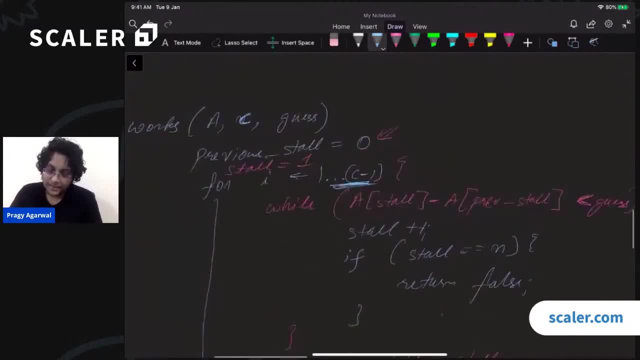 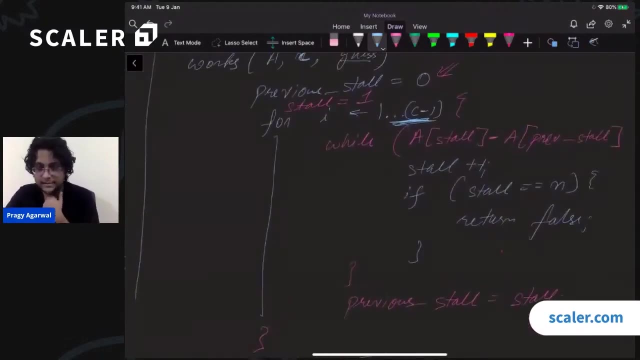 I was able to successfully place all the three different cows at a minimum distance of guess, So over here I can return true, return true. Does that make sense? Does this function? Does this work? Does this works function make sense? Yes, 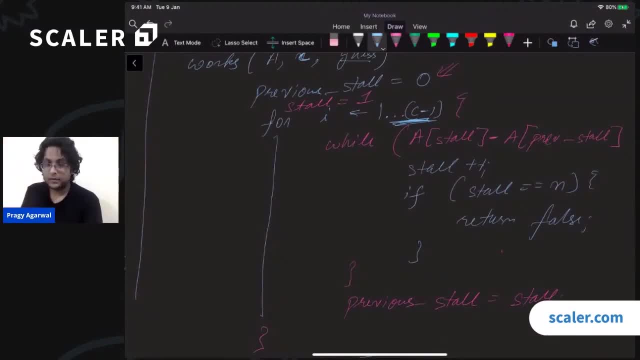 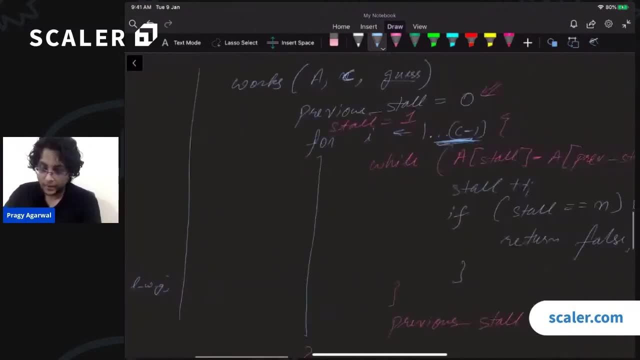 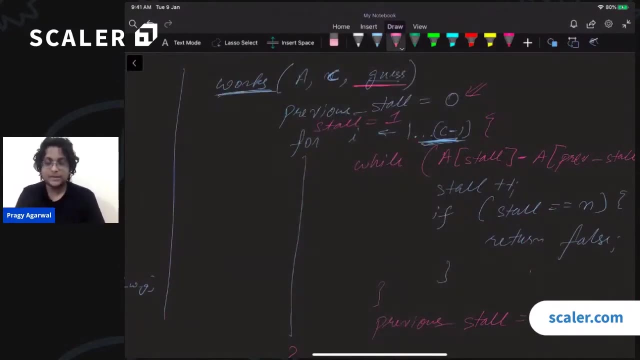 Do you guys agree? Perfect. So what will be the time complexity of this? What will be the time complexity of this entire code? Well, let us take it step by step. How much time does the works function take, Given a particular guess? how much time does it take to verify that guess? 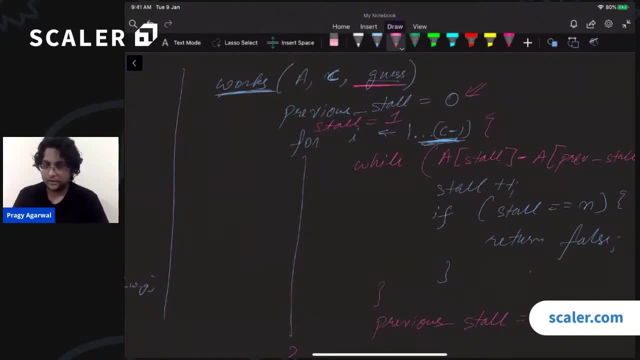 Well, we have to linearly search through the array of stalls. We have to linearly check the array of stalls. So this works takes part of n time, right where n is the number of stalls. Do you agree? Do you guys agree? 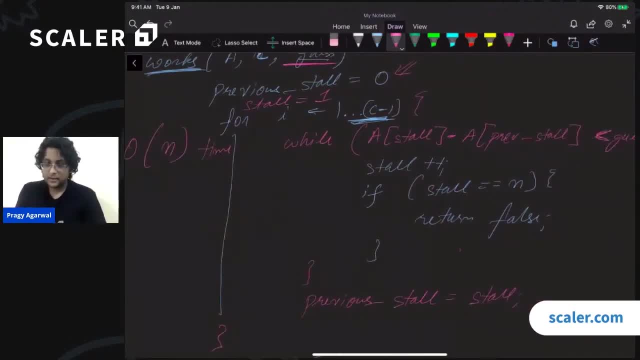 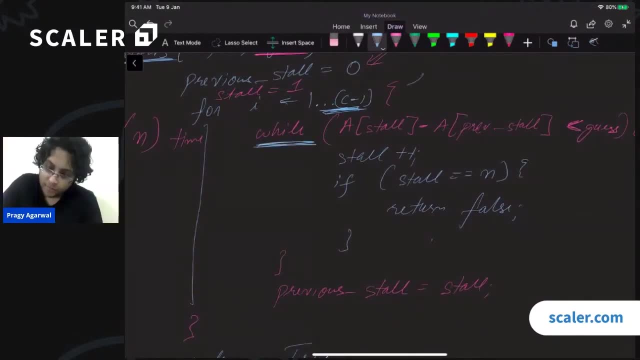 So, okay, some, some people will always say that, okay, you have a while loop, you have a while loop over here and you have a loop that goes c times over here. So isn't the, isn't the complexity going to be c times n? 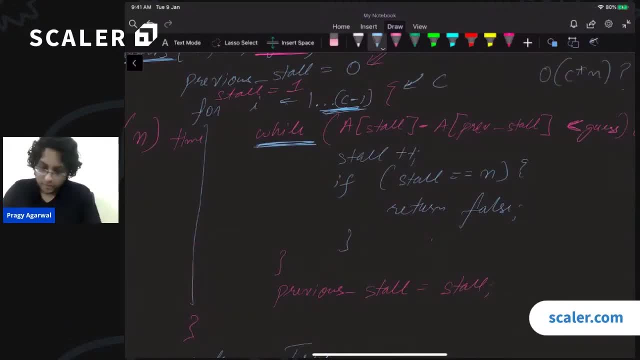 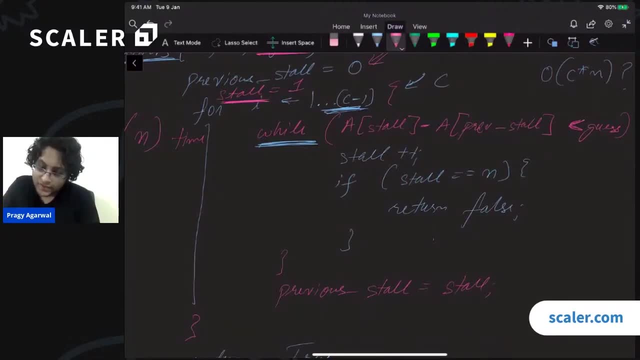 Shouldn't the complexity be c times n? Well, no right. The complexity of this entire for loop is not c times n, Because, as we see, This variable stall, this variable stall is strictly increasing, right, This variable stall is never reset. 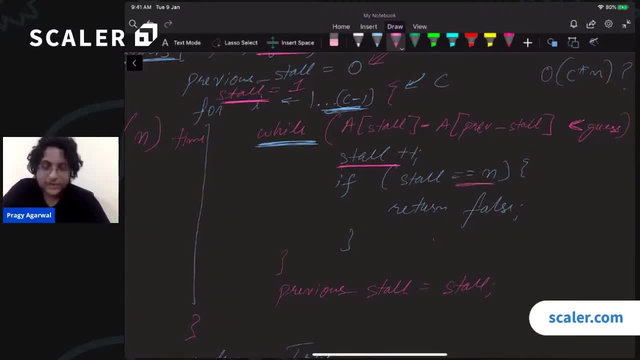 So it can only increase And the maximum possible value of stall can be up to n. It is the complexity of this entire nested loop. It is not C-types, right, It is simply order of n. Is that clear? Yes, perfect. 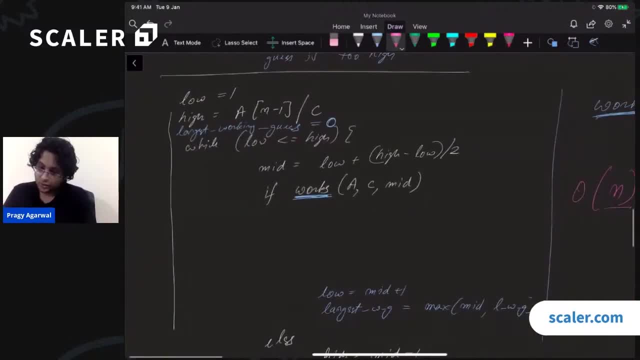 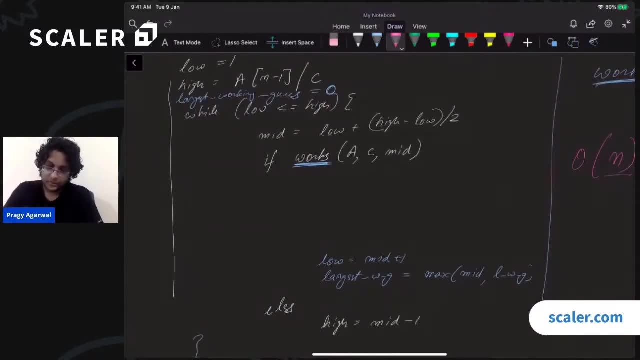 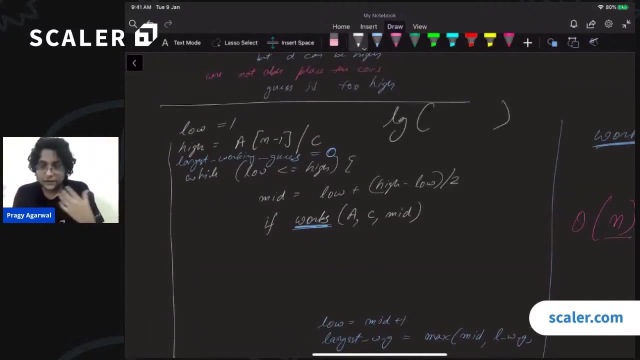 What about this binary search? So I think I deleted it. I'll delete something from here. What about this binary search? So this binary search takes us, how much time It takes us log of the size of search space. What is the size of search space over here? 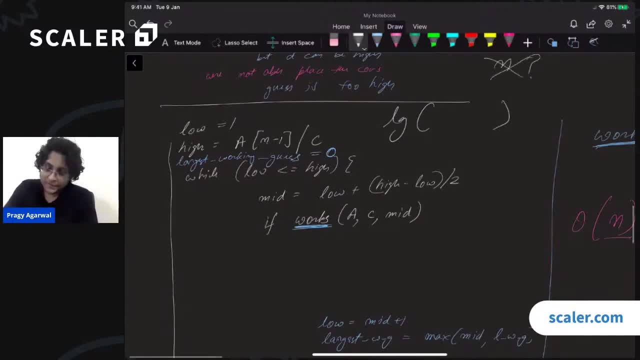 Is the size of search space? n? No, The size of search space. is this value over here, right? This is the size of search space, A of n minus one by C. This is the size of search space. So this will be the number. 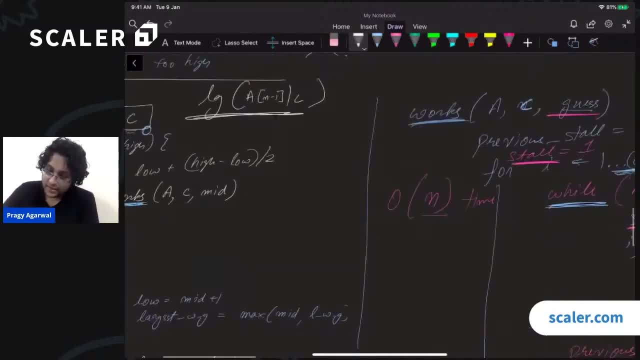 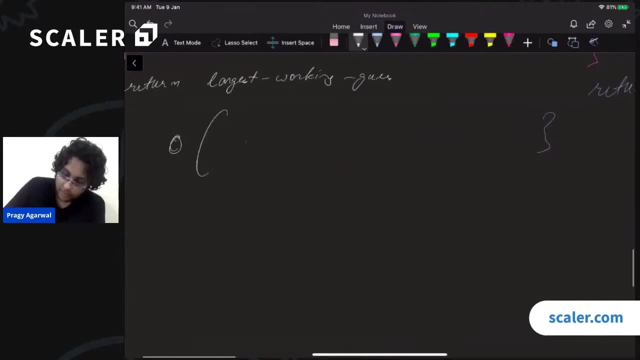 this will be the number of times we will have to do the binary search, And each binary search will take us order of n times. So we can say that the complexity of this is order of log of max of A i. max of A i, the maximum stall location. 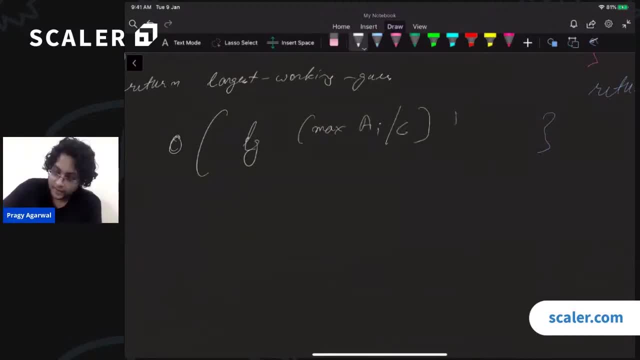 divided by the number of cows right The log of that times n. Is that clear? Yes, Yes or no? Well, C over here, is that clear guys? So C is not a constant, so we can't really ignore it. 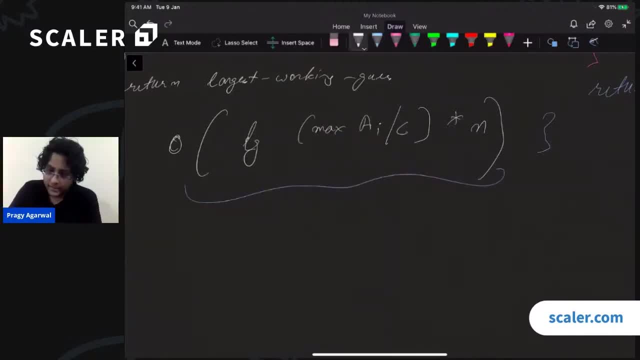 So this will be the final value. This will be the final value. And is this better than? is this better better than n square? So do you guys think that this is better than n square? Well, that will depend. That will depend on how large this A of i is right. 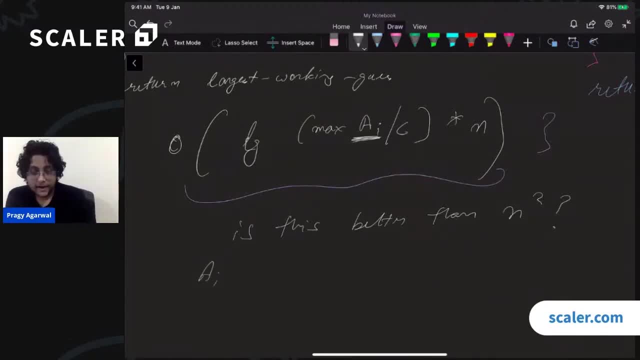 How large this A of i is. Is that clear? So it might be the case that A of i is one trillion. If A of i is a very, very large number, then it might make sense. It might make sense to do this n square solution. 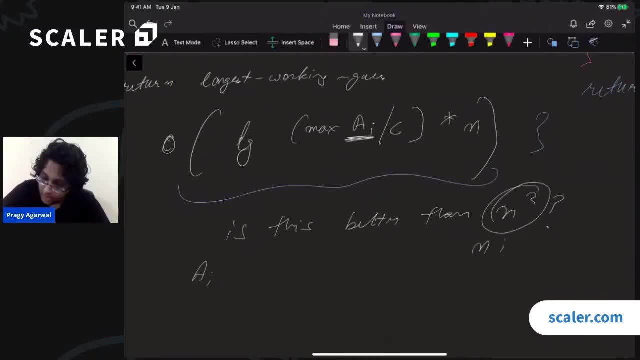 But that is going to be extremely, extremely real right. So if n is large, if n is large, then definitely this log value will be much, much more right. So in general, this approach will work faster. Is it clear? 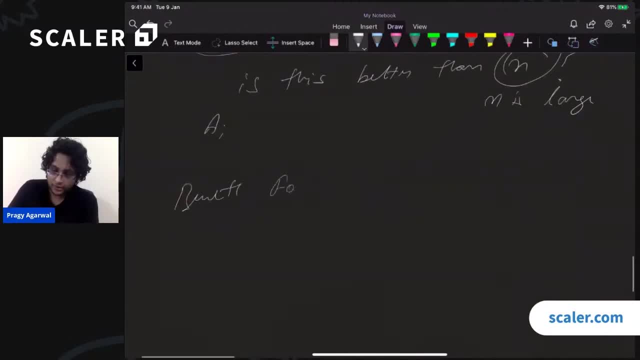 So we saw the brute force approach for this. We saw the brute force approach for this right. That was order of n to the power c plus one right. Then we saw the db approach for this. We did not discuss this in detail. 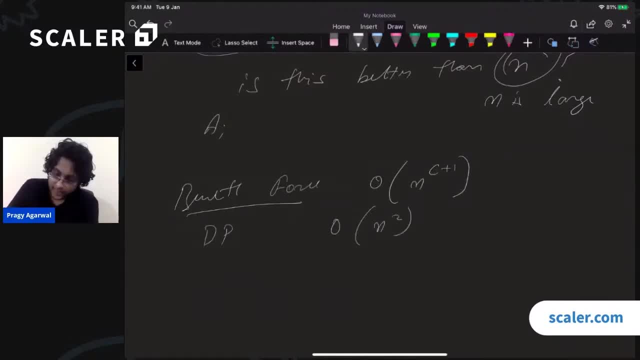 We will discuss this maybe later. So this was order of n square, And then we discussed the binary search approach. Binary search approach, And this turned out to be order of log of max of A by c times n. Is that clear? Yes, Any doubts? 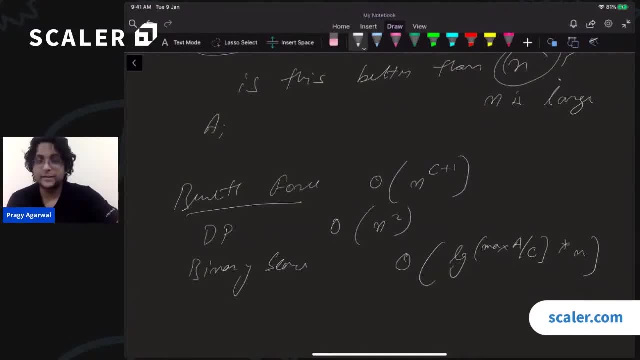 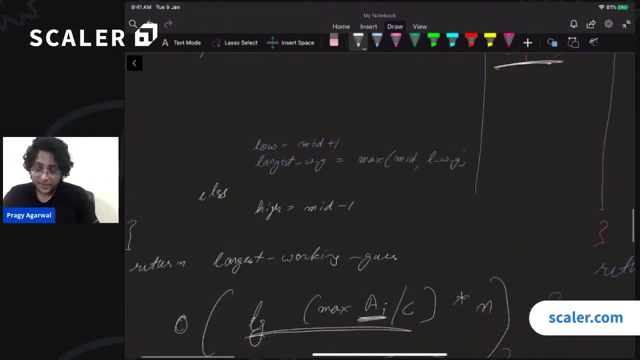 Any questions on this particular question. I hope that you will be able to code it. So this is part of the assignments. So please try and code it. You will actually learn a lot when you implement these solutions right. And one more thing: please, please, try to make sure. 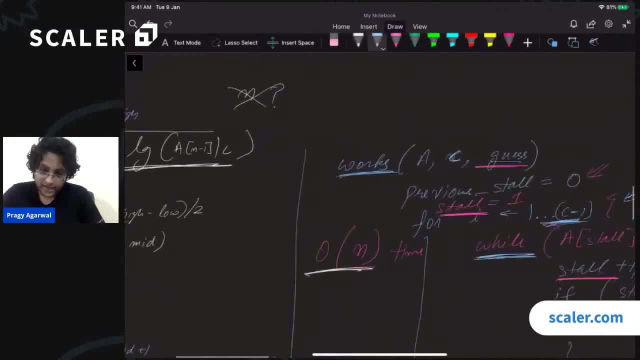 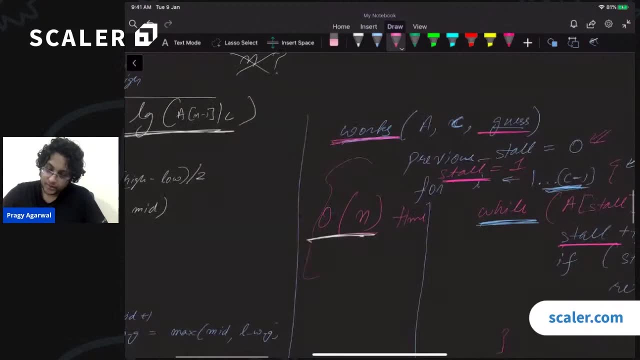 that you make the code modular, right. So, just like we have discussed in the class, please define a separate function. right, That will check the list. You can also write this code over here as well. right, You can also write this code over here as well. 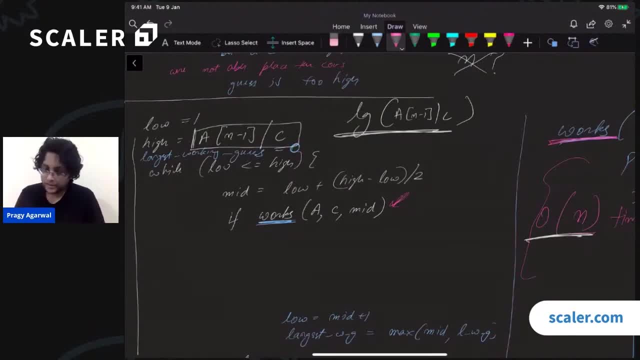 But please do not do that right, Because then your logic will not be clear. You will be mixing the logic of your binary search with the logic of your checking of guess. Let us keep those two logics separate. Binary search is separate. 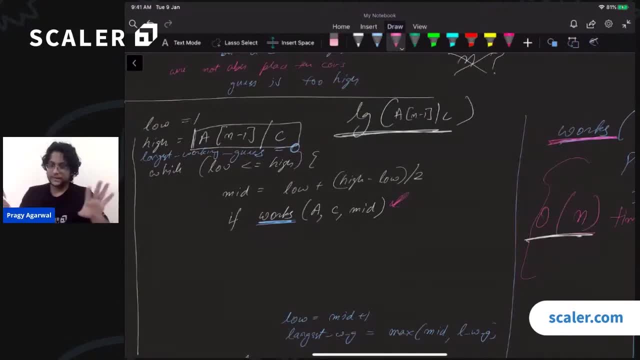 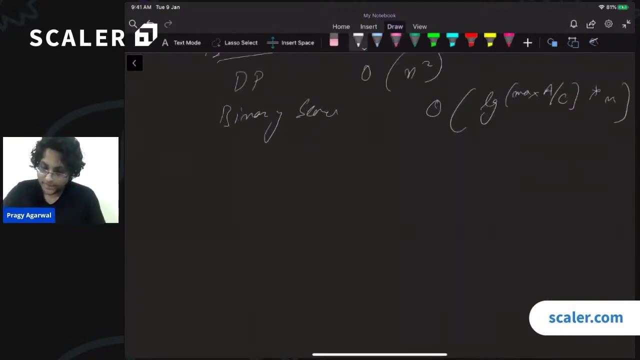 Checking if a particular guess works or not. that is separate. So please let us do the separation of concerns thing and then keep them in different functions, All right, So let us move on to another question. So this is again fairly challenging question. 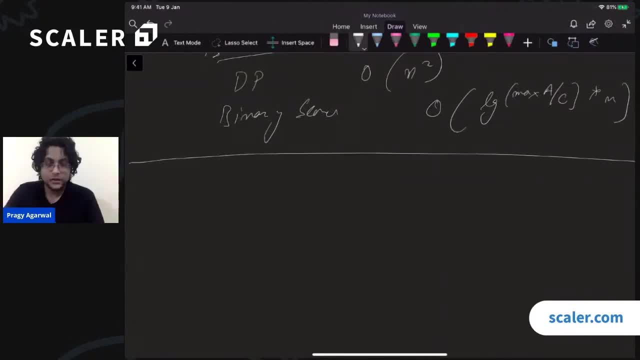 And this is also a very, very interesting question. OK, So the question goes something like this: That you have been given an n, You have been given a number n, And this n is a 64-bit number, 64-bit integer. 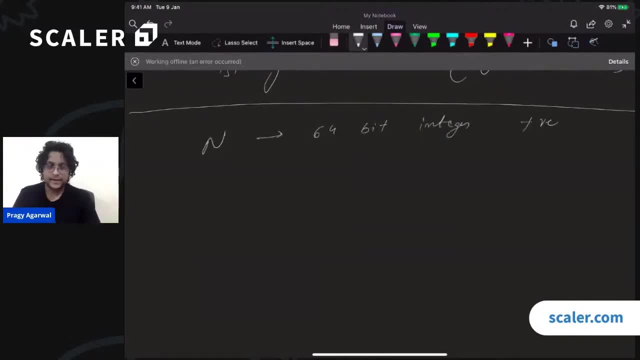 And let us say it is also positive. Let us say it is also positive. Let us also say that n is greater than 2.. Let us also say that n is greater than 2.. So, basically, what values can n take? So n can take a value from, let us say, suppose 3.0.. 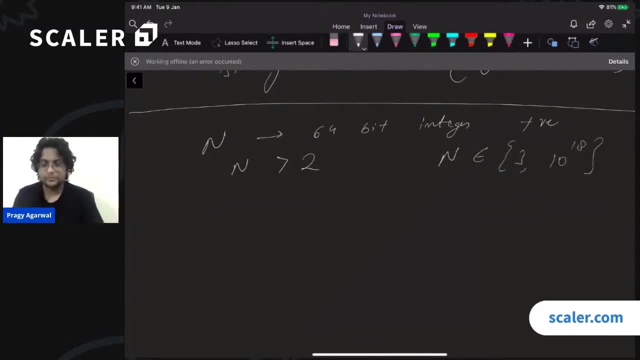 Or the value 10 to the power 18, perhaps right n can take all these different values. So now what we are saying is: let us suppose. let us suppose that n written in the sum base k, n written in sum base k. 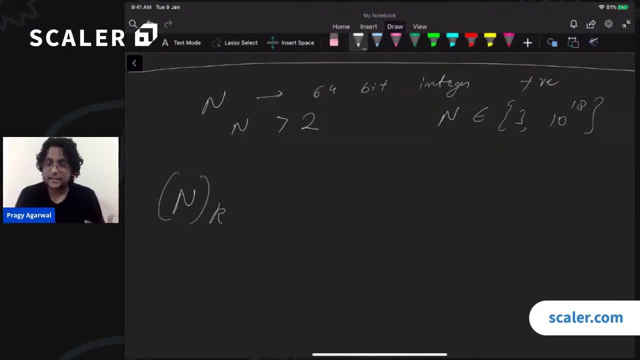 So k can be either 2, in which case we are writing n as a binary number right, Or k can be total, or k can be 3, or k can be 8, in which case we are writing n as an octal number. 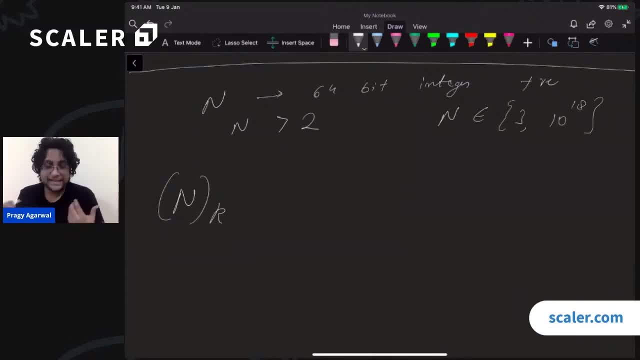 Right. But if we write k, if we have n in sum base k and if this equals to 1, 1, 1, 1, 1,, dot, dot, dot, if this is just a string of 1's, string of 1's right. 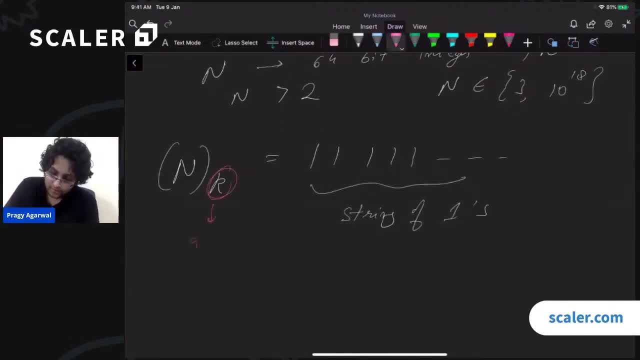 Then we will say that, OK, this k is a good base. Good base, All right. Is that clear, For example? for example, let us say that n equals to 7.. All right, n equals to 7.. Then what different bases will go? 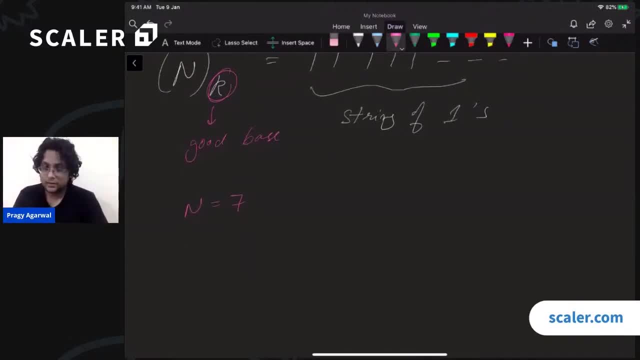 What all different bases can go. So first of all, this k equals to 1 will always go Right, Yes or no. I can always write something in base 1.. A number n in base 1 is just 1, 1, 1, 1, 1, n times. 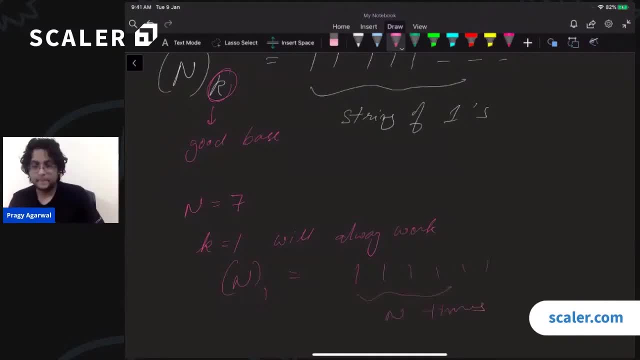 Do you guys agree? Yes, Let us not do that. Let us not do that. Let us ignore. let us ignore this. k equals to 1 thing. All right, Let us ignore this. k equals to 1 thing. So we are also considering that k is greater than 1.. 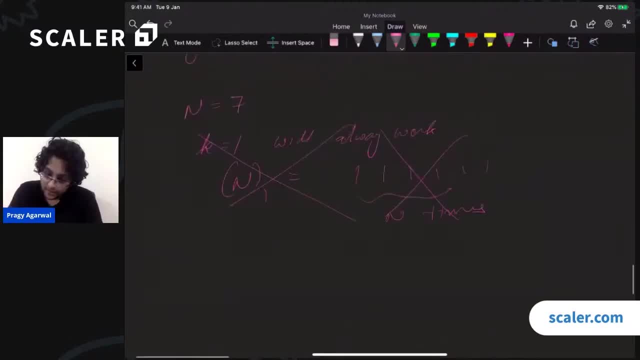 That k is greater than 1.. Now let us try some other base. So 7, 7 written in base 2.. What does this look like? What does 7 in base 2 look like? 7 in base 2 is so this is base 10, my bad. 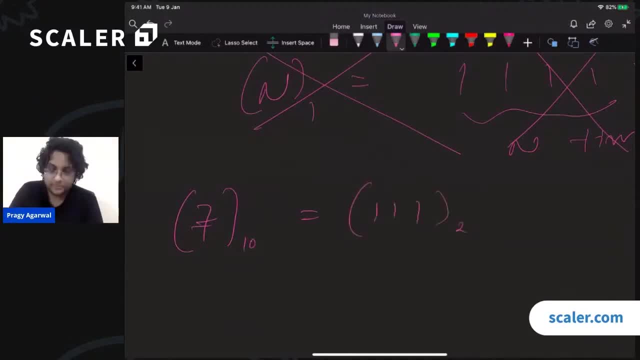 This is base 10.. In base 2, if I write it, then it will be 1,, 1,, 1.. Right, So 2 is a good base. 2 is a good base for 7.. All right. 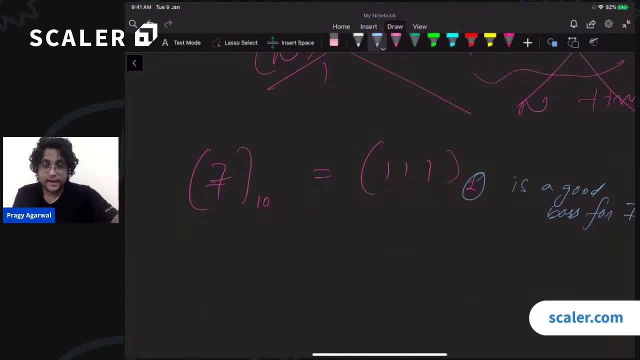 Are there any other good bases? Are there any other good bases? Yes, No. Well, what happens if we write 7 in base? what happens if we write 7 in base 3?? What do we get? So we get 1, then 4 remains. 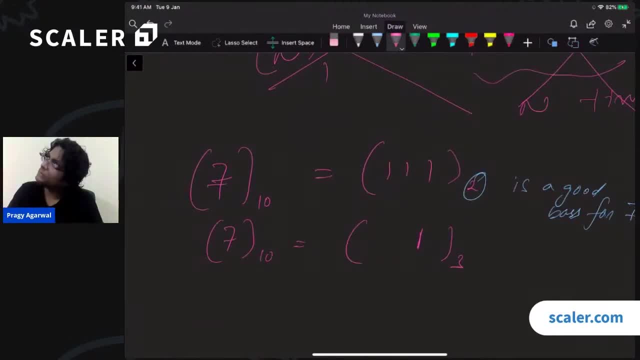 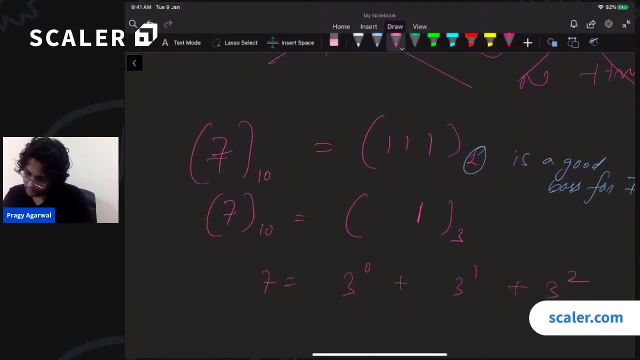 Right, So just give me a second, So the last. so 7 is basically equal to 3 to the power 0, plus 3 to the power 1, plus 3 to the power 2.. So this is going to be 3 to the power 3.. 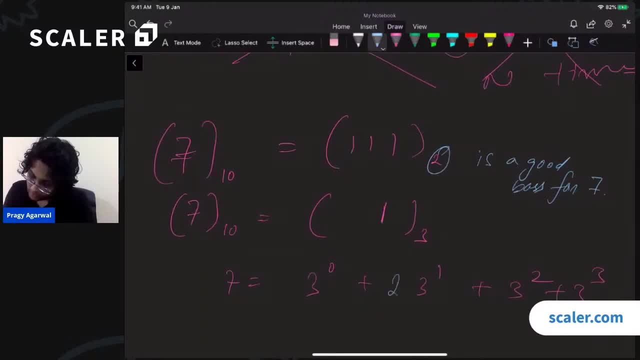 Yes, so this is going to be 2 times 3 to the power 1, plus 1 times 3 to the power 0.. Yes, So this is 7.. This is 7.. So what will 7 look like in base 3?? 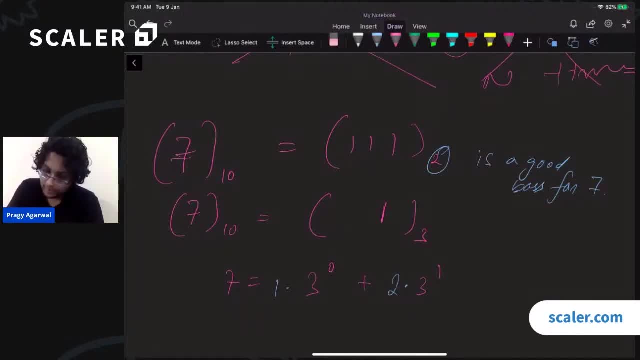 What will 7 look like in base 3?? 7 will look like 2, 1 in base 3.. Right 7 is 2, 1 in base 3.. So is this a string of 1s. 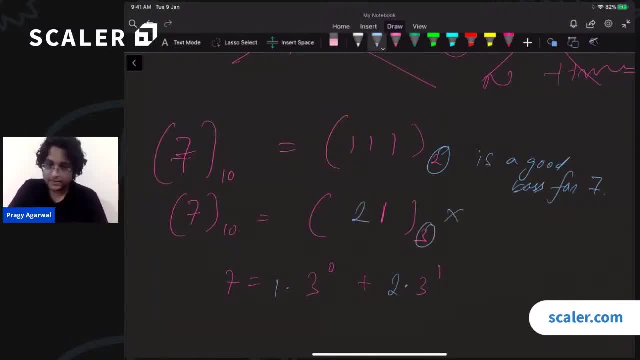 Is this a string of 1s? No, this is not a string of 1s. So 3 is not a good base. 3 is not a good base. All right, Let us continue. Let us continue So we can check the base 4.. 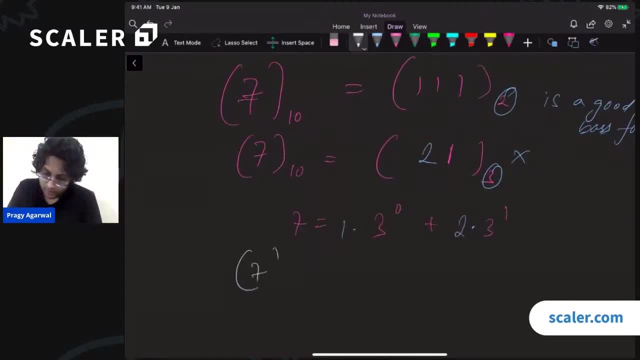 We can check the base 5.. That is also not going to work. There is some other base that is going to work Right. So the base 4 in base 7 is also equal to in base 6, this is going to be equal to 1,. 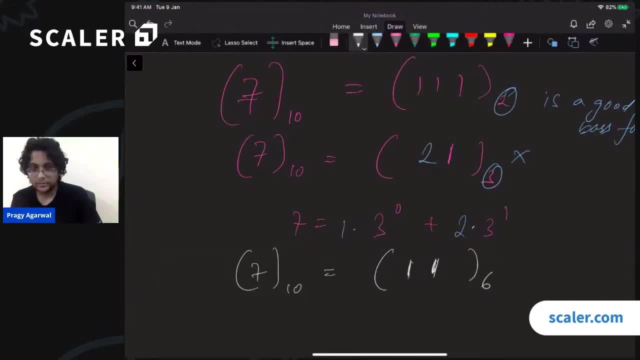 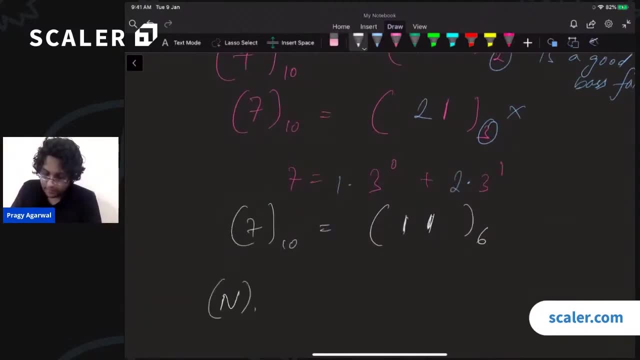 1. In base 6, this is also going to be equal to 1, 1.. Do you guys agree? Yes, In fact, if I have any n in base n, then this is equal to 1, 1 in base n minus 1.. 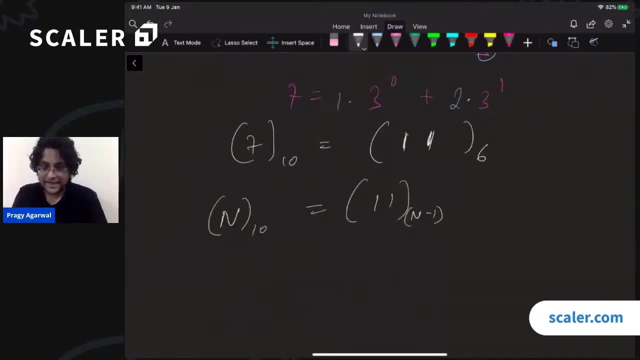 Yes or no? 1, 1 in base n minus 1, that is simply n. Why is that? Because see 1, 1.. in base n minus 1, this is equal to n minus 1 to the power, 0 times 1 plus n minus 1 to the power. 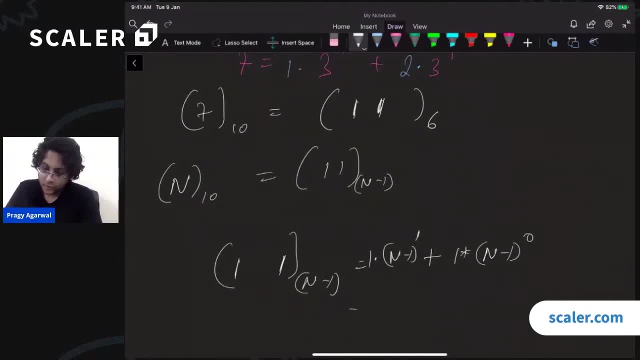 1 times 1, right, And that is equal to what n minus 1 plus 1,, which is just n, right? So any number, any number n that I have, I can always write in one less base and get a string. 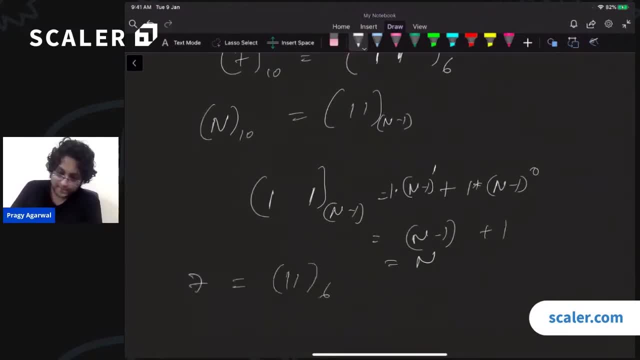 of ones. So 7 equals to 1, 1 in base 6, right 13 equals to 1, 1 in base 12, and so on. Do you guys agree? So n minus 1 is always a good base. right n minus 1 is always a valid base. So 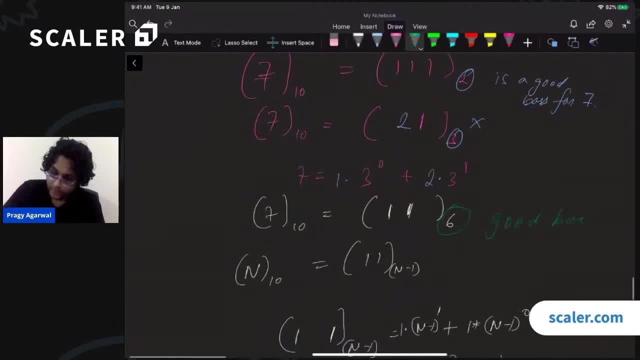 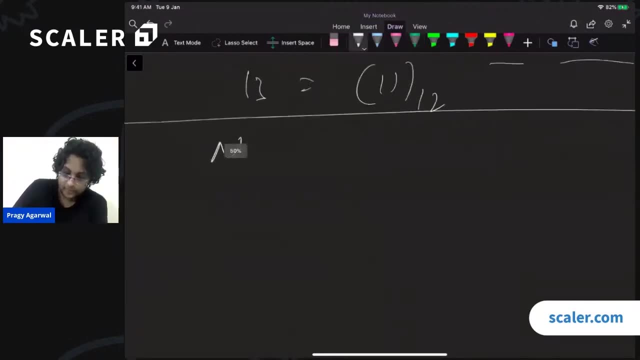 this is also a good base, right, Cool. Now the question once again is that you have been given a value of n, right, Such that n is greater than equal to 3. And n is less than or equal to 10 to the power 18, suppose. So it is a 64-bit integer positive. 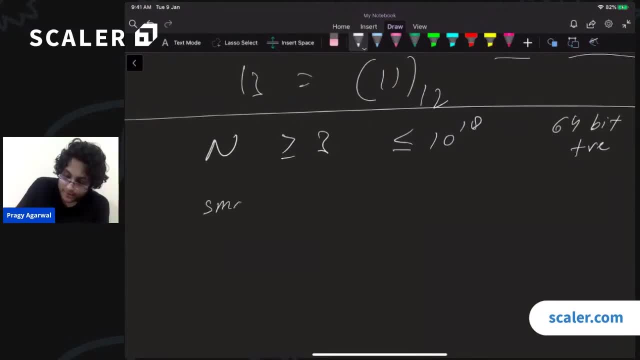 integer. We have to find the smallest base, smallest good base right. So we found several different good bases right For 7, we found that 2 works, So we found that 2 works. 3 does not. 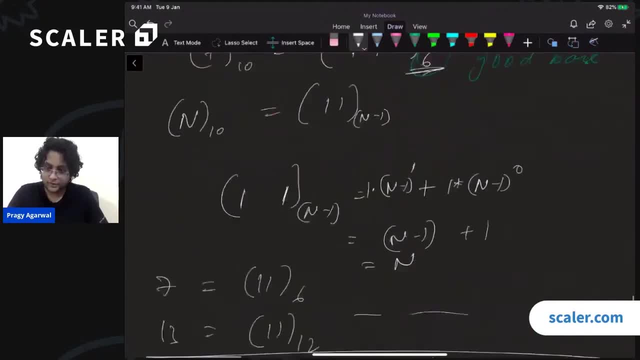 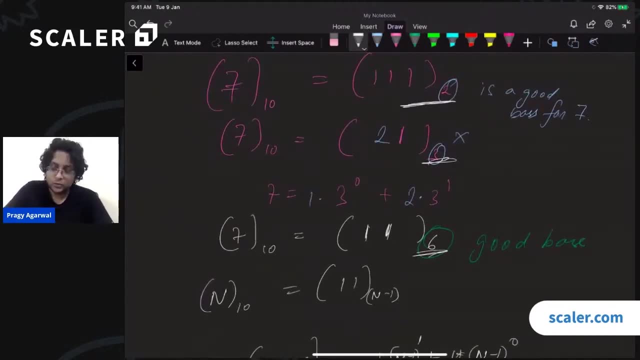 work. 4 does not work. 5 does not work. 6 works. right. That is what we found for 7.. So what will be the smallest good base for 7?? What will be the smallest good base for 7?? It will be 2, right, It will be 2.. So smallest. 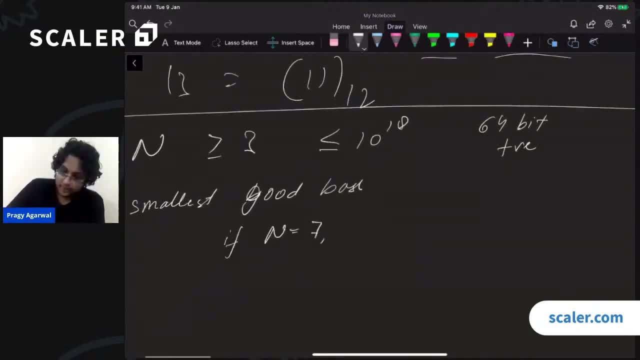 good base. So, for example, if n equals to 7,, then the answer will be 2.. And why 2?? Why not 1?? Because 1 works for everything. If we allow 1,, then for every number the answer. 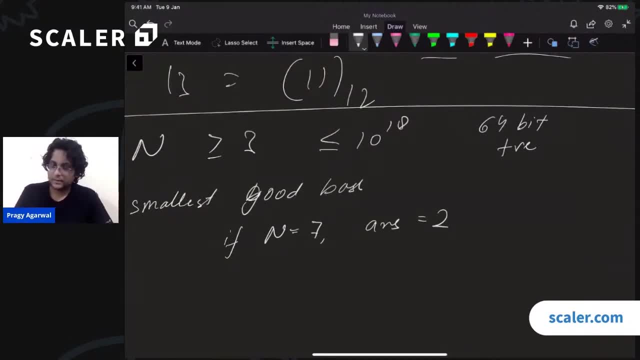 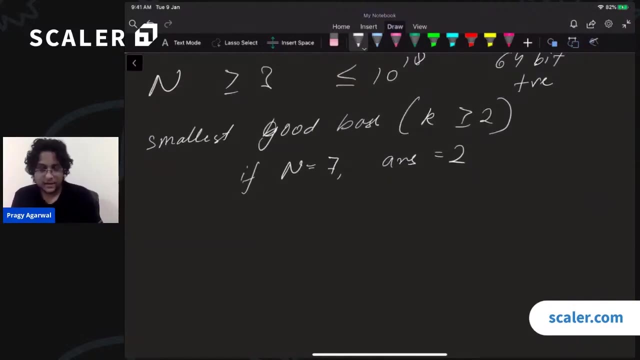 will just be 1, because base 1 works for everything. Is that clear? So we are saying that the smallest good base- let us call this k- is greater than or equal to 2.. So this is the question. I hope the question is clear. Given an integer n return the smallest good base, For example. 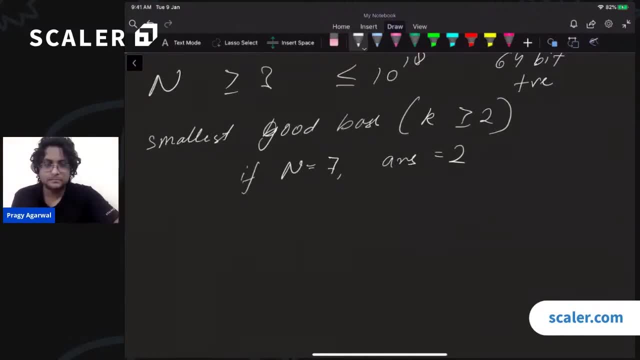 if your value is 7,, then you are supposed to return the value 2.. All right, So what can our approach be over here? What can our approach be over here? Let us start with the most brute force approach: Brute force approach. What will the brute force approach look like? In the brute 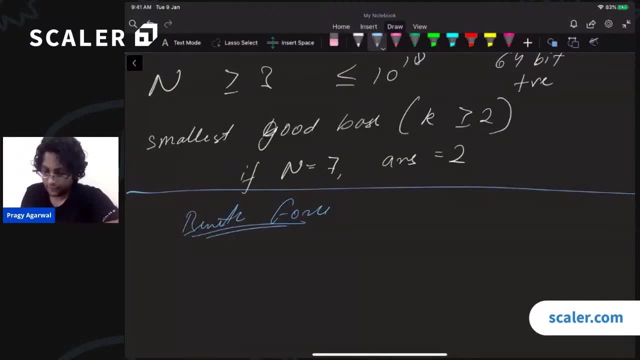 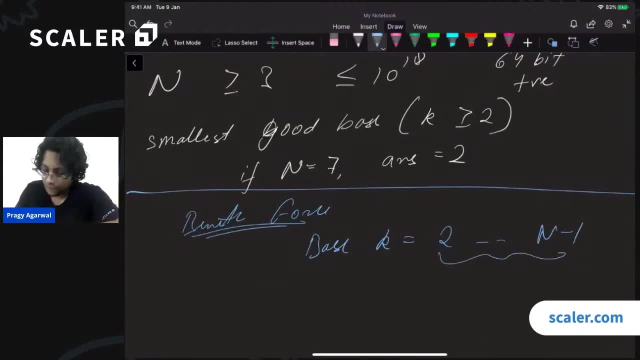 values. Now, once we have a base, once we have a base, we have to convert n into that base, base k, and check if this is a string of 1s. If this is a string of 1s, well, how? 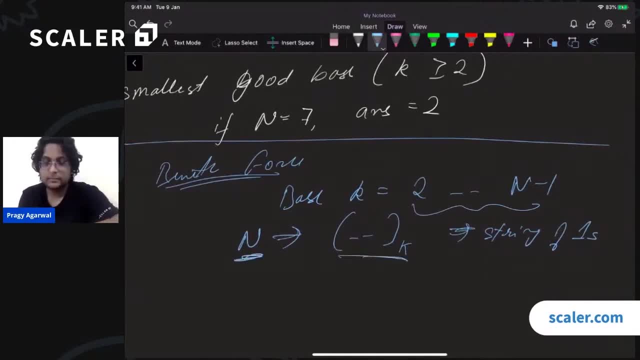 much time does it take to convert a number into base k? How much time does it take to convert a number into base k? Can someone quickly tell me that It will take me log of n time base k? It will take me log n time with a base k. This is how. 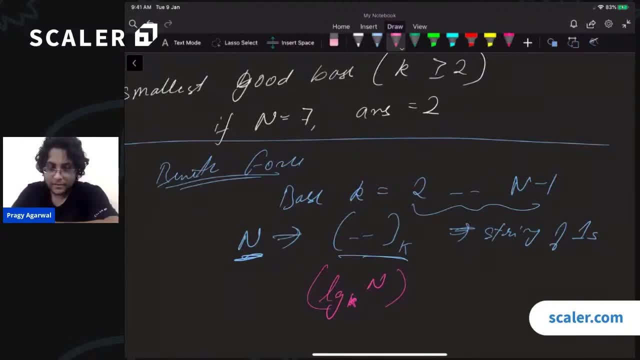 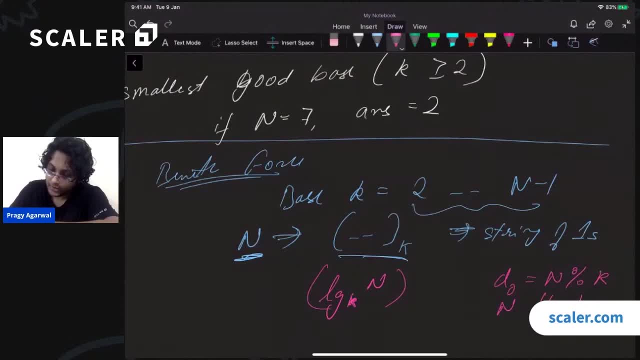 by k. I will say n by k. I will saygi y k. This is not in cost. waited for the current point. The example of this is of simple division Right. Then I will say d1 equals to, once again, n mod k, And then I will again say n equals n. 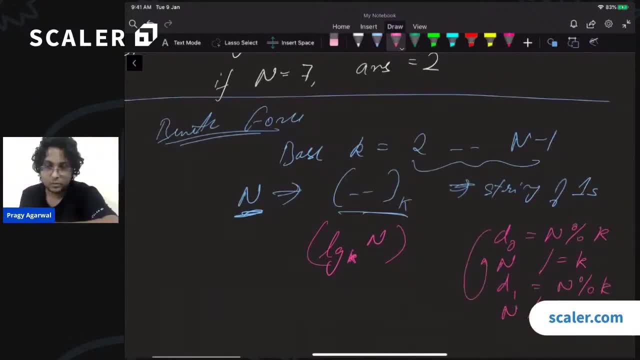 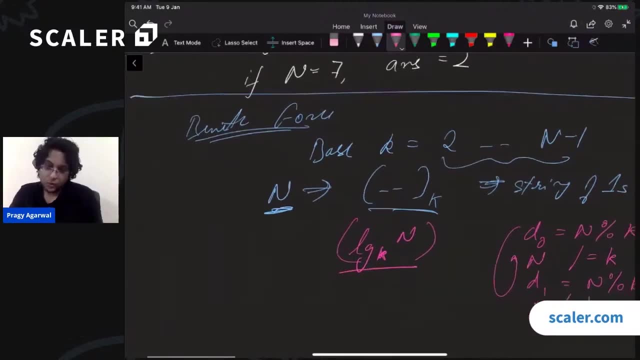 by k And this will be in a loop. This is basically a loop. This is how I convert the base. It will take me log of n time. base k: Alright. So what is the total time complexity over here? I have these many bases to check. I have these many bases to check And it takes 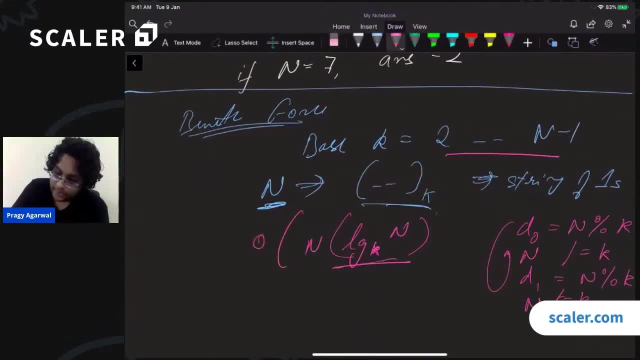 this much time to check each component. This is the number, This is the total time complexity And this is the number. What is the 68th? This is benefactor of that. So again, don't settle case. So it will be order of n times. log n right. So my brute force approach takes me. 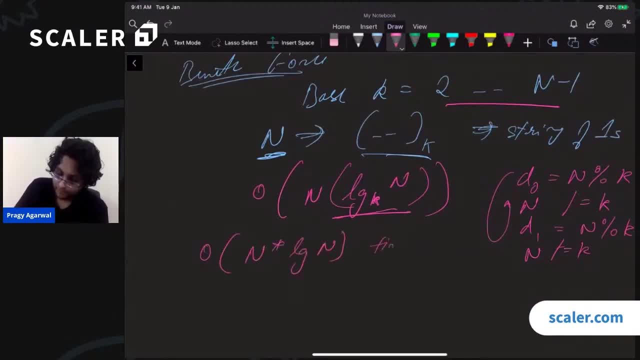 order of n times. log n time. Is that clear? Yes, Now this is not very good, right, This is not very good. If my n is, let us say, 10 to the power 18,, then it will take me 10 to. 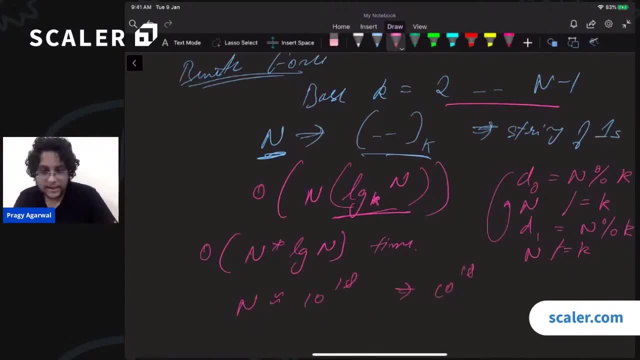 the power 18 steps. That is definitely not possible. I cannot do 10 to the power 18 steps on any computer. Yes, So we should better come up with a faster solution. We should try to come up with a faster solution. Okay, So what can we do over here? What is the first? 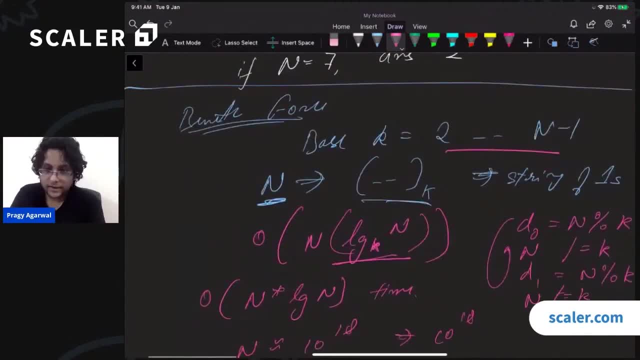 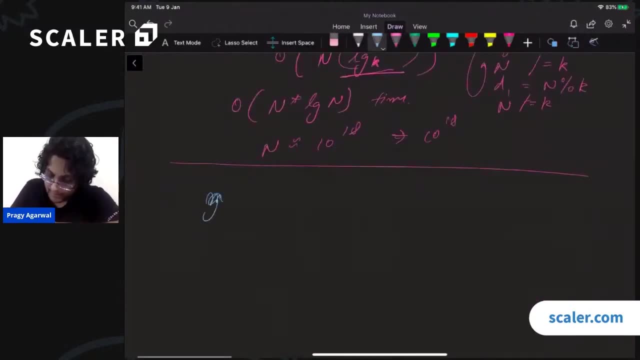 thing that comes to your mind. What is the first thing that comes to your mind? The first thing since we have been doing binary search might be that, okay, let me make a guess. Let me guess base B. Let me guess base B and check if the guess is valid. Let me check. 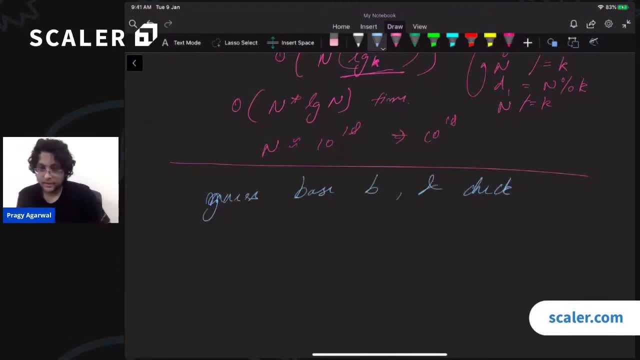 if it is valid or not. Yes, That is what comes to your mind. Let us take a base B, Let us consider a random base B and let us check if it is valid or not. Well, this is not going to work for this case. This is not going to work for this case. Why Suppose? 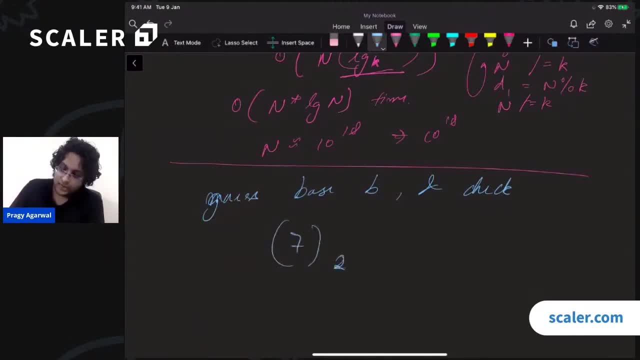 that my number was 7.. I checked the base 2.. I checked the base 2 and it worked. What does that tell me? Does that really tell me anything? That tells me that 2 works, That tells me that 2 works. but that is not enough, right? I also have to understand. I also have to. 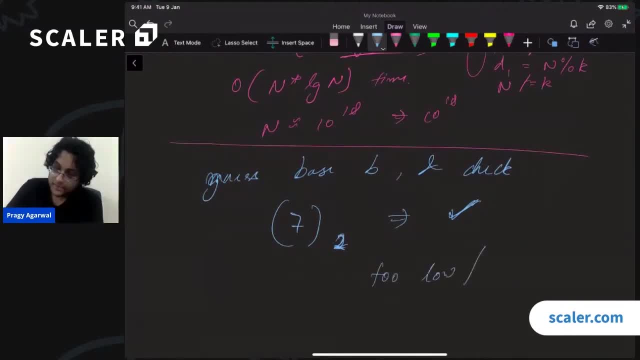 understand. Is my guess too low or is my guess too high? Yes, Just because 2 works, that does not mean that my guess is too low or that my guess is too high. Do you agree? It might be the case that 7 of 6 still works right? So for this, for the base, 7,, 7 of 2. 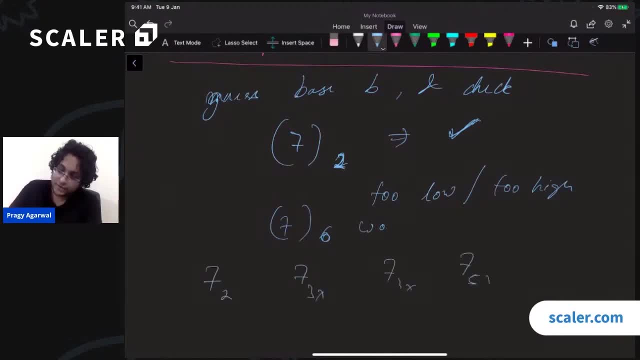 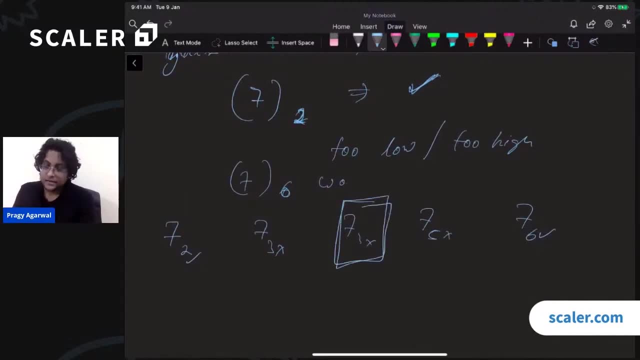 works. 7 of 3 does not work. 7 of 4 does not work. 7 of 5 does not work. 7 of 6 works. This works, Suppose you make a guess. Suppose you make a guess, There is a valid value to the right. 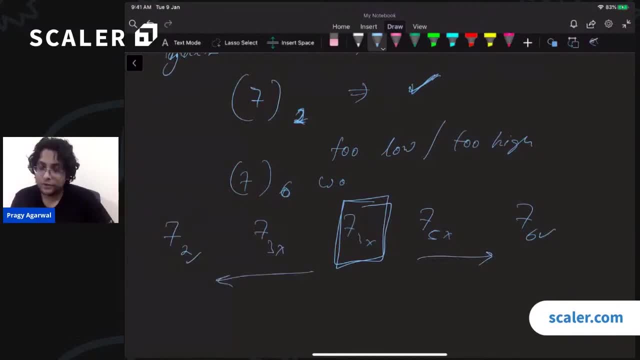 of it as well as to the left of it, And you do not know in which direction you have to go. So, if it, if it turns out to be false, if you figure out that, okay, the guess did not work. did not work. So are you supposed to increase the base, or are you supposed to? 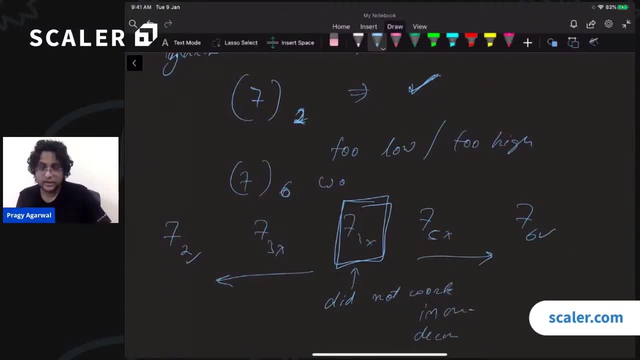 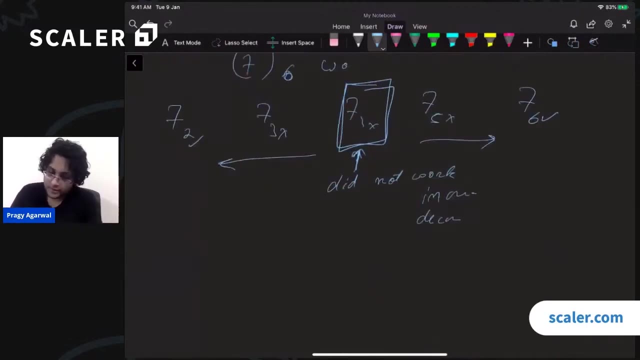 decrease the base? Are you supposed to increase the low or are you supposed to decrease the high? Does that make sense? We have no way of knowing in which direction should we move our guess, So we cannot do the binary search over base. Does that make sense? Because, once again, if we go back to the first class, if this 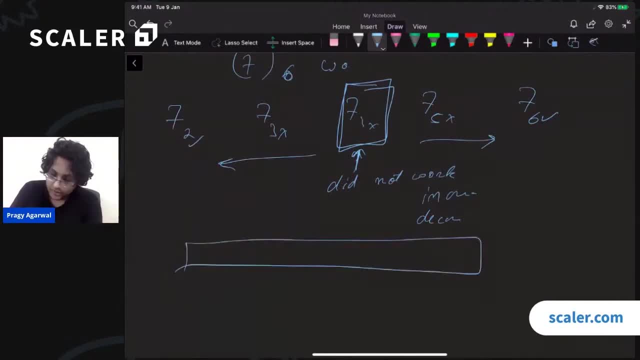 is our search space, then we need to come up with a proposition such that all the answers here are yeses and all the answers here are nos, So that we can search- binary search- for this midpoint, For this particular thing. the answer over here is yes, The answer over 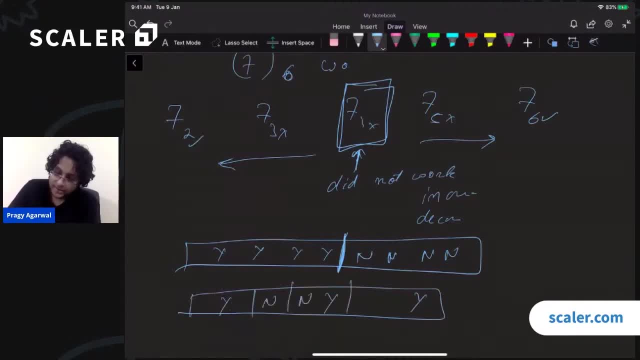 here is yes, The answer over here is yes, But all the other numbers can be no. We do not really know. It can be randomly, It can be in a random manner. So binary search is not going to work for this proposition. Is that clear? Yes, It seems. 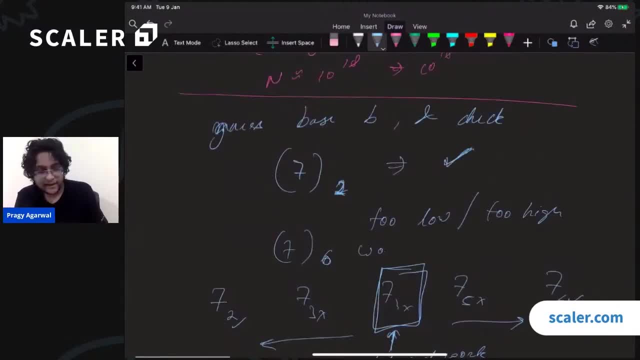 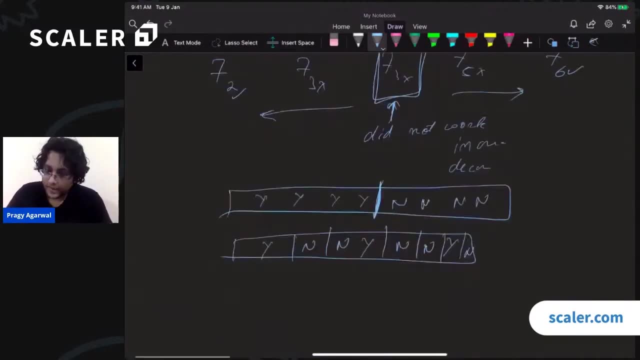 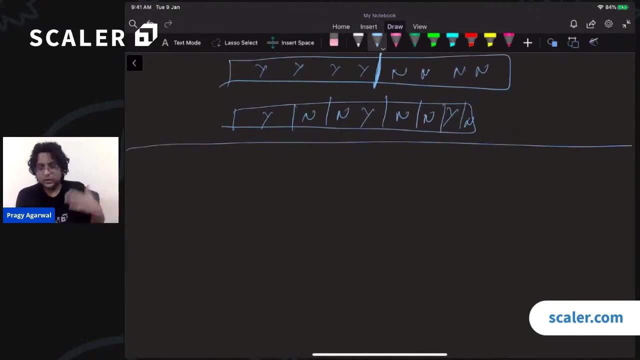 very, very selective to try to apply binary search over here. I have a base. I can verify if it is a valid base or not, So let me just binary search over the base. That is not going to work, unfortunately, So what else can we do? What else can we do? So we have to look. 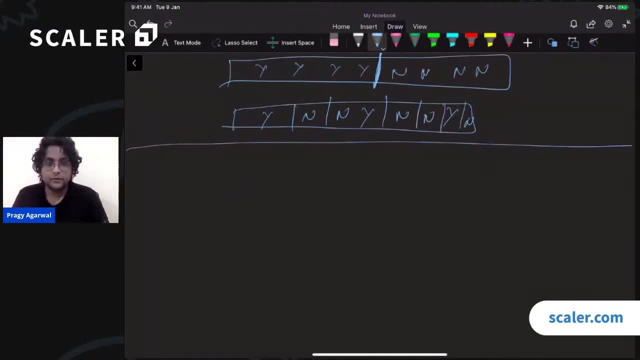 at the question from a different perspective. over here We have to look at the question from a different perspective. We have to look at the question from a different perspective. So let us suppose that we are talking in base B. Suppose we are talking about in base. 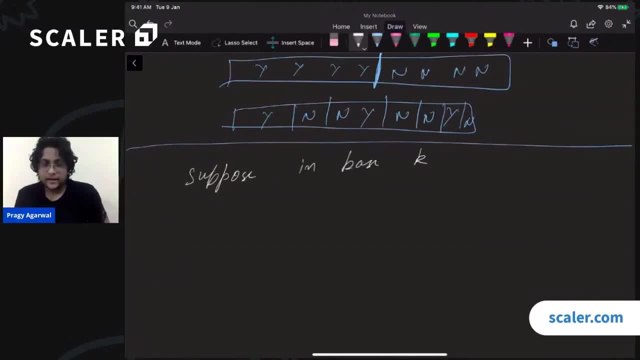 K, Suppose base K, Then if basically my number n in base A is a string of ones, I already know what the string of ones is. I can construct this string of ones. I know that this is in base K. I know that this is a string of ones. I can construct this string of ones, I know. 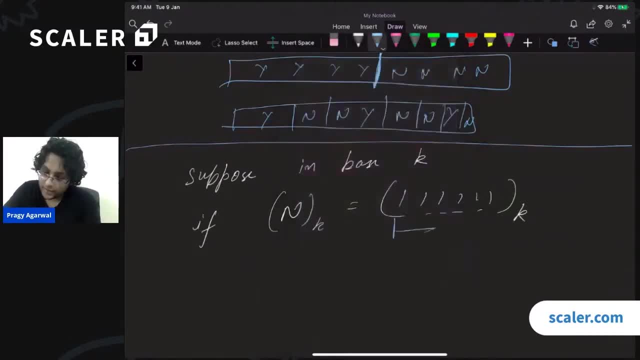 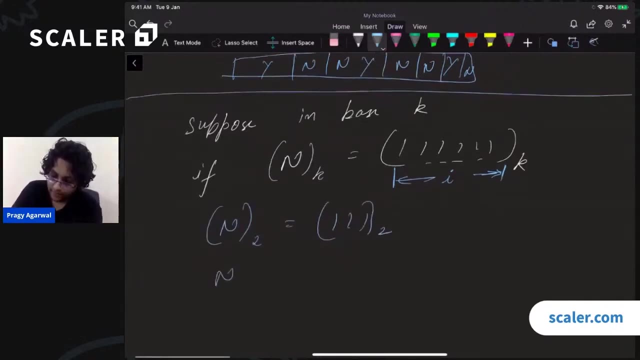 that this is a string of ones. The only thing I don't know is how many ones there are over here. Yes, How many ones there are over here. Let us call this value. I Does that make sense? So n written in base 2 will have 3 ones. n written in base 6 will have 2 ones. So instead, 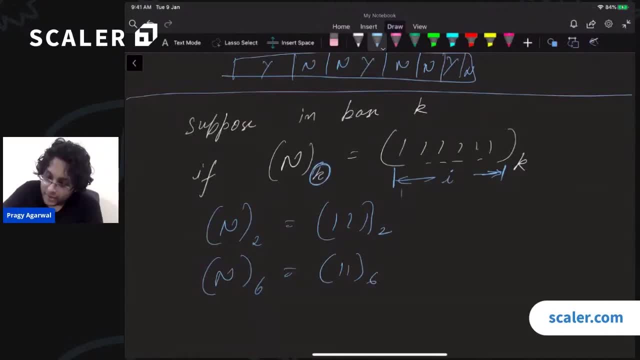 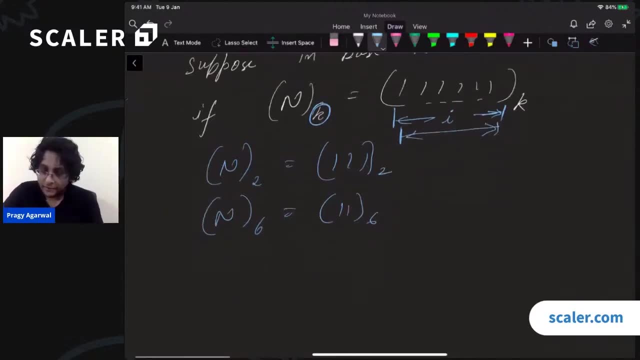 of trying to binary search over the value of K, let me try to binary search over the value of I. Let me try to binary search over the value of I. But let me first establish a relation between these two. Let me first establish a relation. 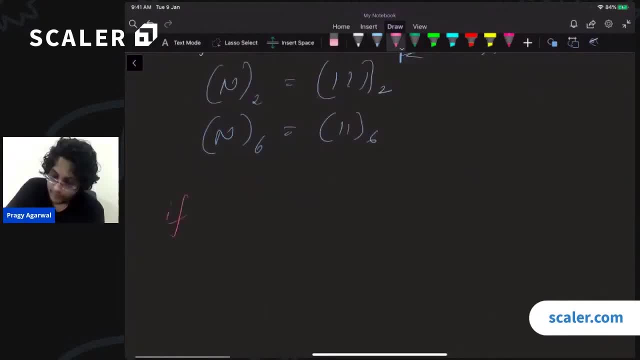 between these two. So if n in base K is a string of ones in base K, So n is equal to a string of ones in base K. And let us say that there are I ones over here. Then what can I say? Is there any relationship between n and K? Is there any relationship between? 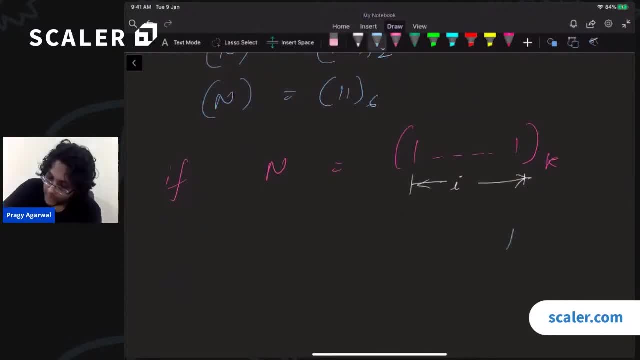 n and K. Yes, there is. What is the relationship? I know that 1 times K to the power 0 plus 1 times K to the power 1, plus 1 times K to the power 2, plus all the way till 1 times K to the power i, This thing equals to n. 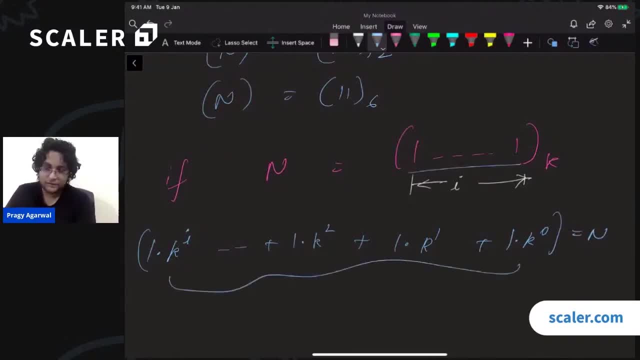 If I have this number in base K, then this is the expansion of it, And I know that this must be equal to n. So what can I say? n equals to summation of K to the power. i for K to the power. let us say x. 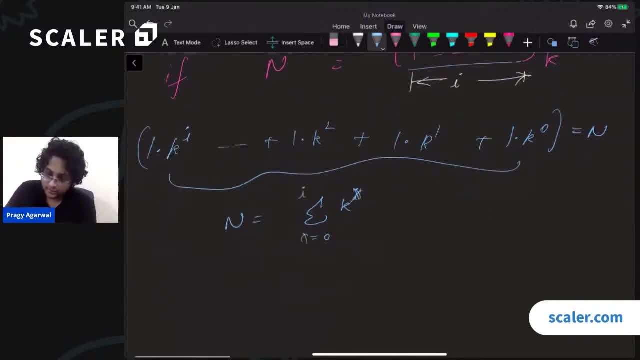 x equals to 0 till i. So this is a. what is this? This is a geometric progression, This is a GP. So can I write the sum of it? The sum of it is simply K to the power. i plus 1 minus 1. by what? By K minus 1.. Right, So the sum of a GP, summation of R to the power. 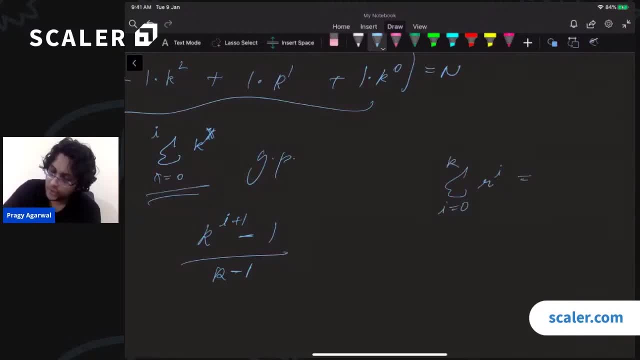 n plus 1 for i equals to 0 till K. this is equal to what? 0 till n? This is equal to R to the power n plus 1 minus R to the power 0 by R minus 1.. Right, Yes, So just notice. 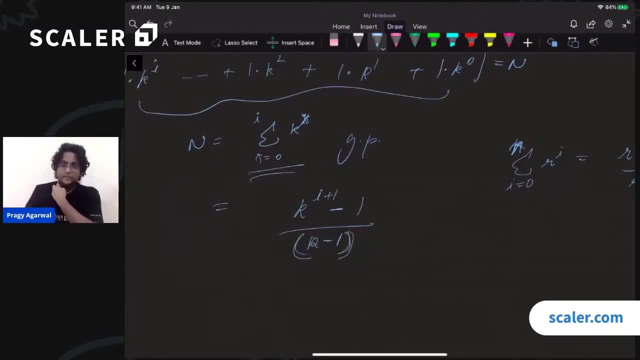 that there is this denominator over here, Right? You cannot simply say that the denominator is 1. Right, Sajiya, So Sajiya. there is a small mistake in your formula. You have to make sure that this denominator is also dependent on K, Right. 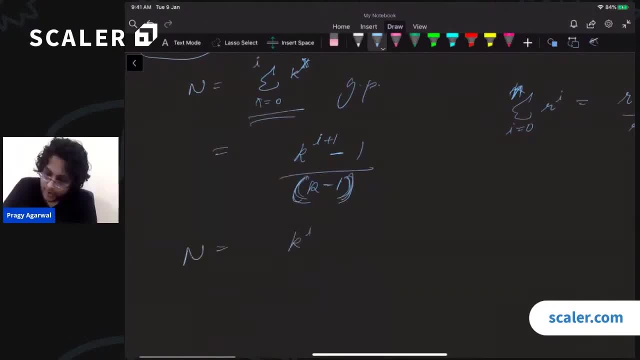 So we can say that n equals to K, to the power i plus 1 minus 1 by K minus 1.. This is the relation that we have established between n, K and i. Now I know that i cannot really binary search over K, But that's okay, Let me binary search over i. Let me binary search. 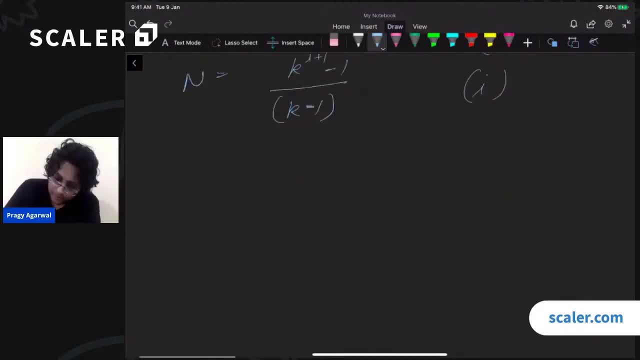 over the value of i. All right, Now let us suppose. let us suppose that I have i ones over here. Let us say that I have i ones over here, Right, And this is equal to n. This is equal to n. Then what if I'm trying to minimize? 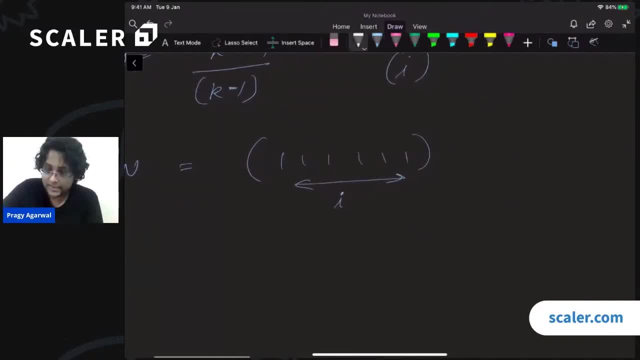 if I'm trying to minimize, so remember that I have to find the smallest good base. I'm trying to minimize the value of K. I'm trying to minimize the value of K. So what am I trying to do with the value of i? If n is my constant? n is my constant. I'm trying to minimize the. 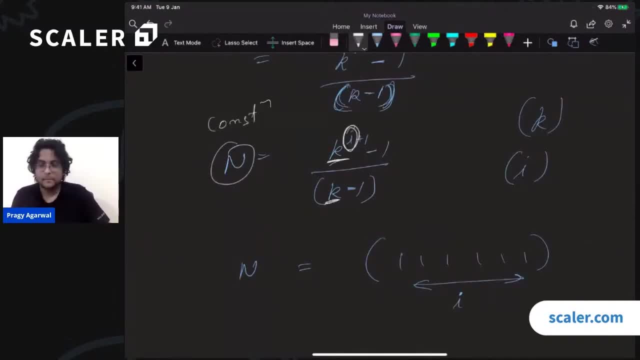 value of K. So what am I doing with i? I'm trying to maximize the value of i, Right, I'm trying to maximize the value of i. Do you agree, Yes or no, Right? Yes or no, guys? So that is one thing we know, Perfect, We. 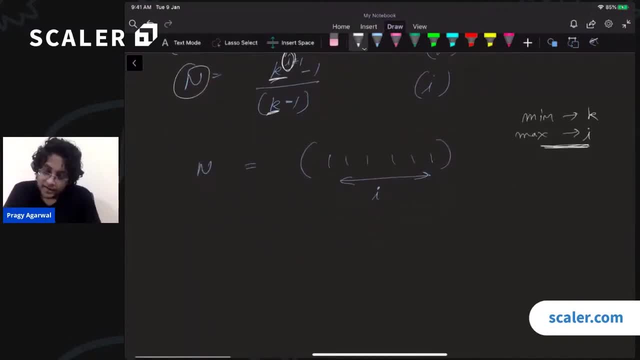 know that we are trying to maximize the value of i. All right, Let us also. let us also consider: what is the search space of i, Search space of i. What is the search space of i, So i can be, i can be, so this can be. so let us suppose. 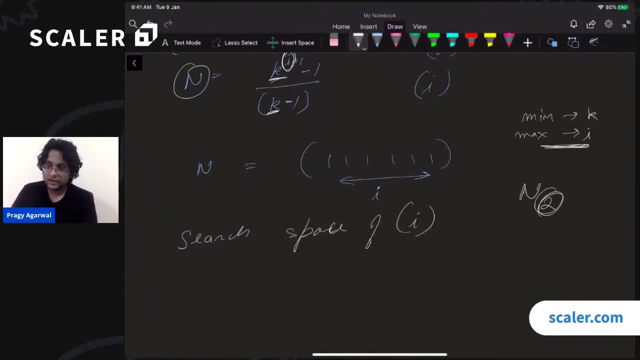 that I write n in base 2.. Right, This is the smallest base that I can possibly have, So that will give me the largest possible string of ones. Largest possible string of ones. How many ones will I get when I write n in base 2?? I know that n is a 64 bit integer. 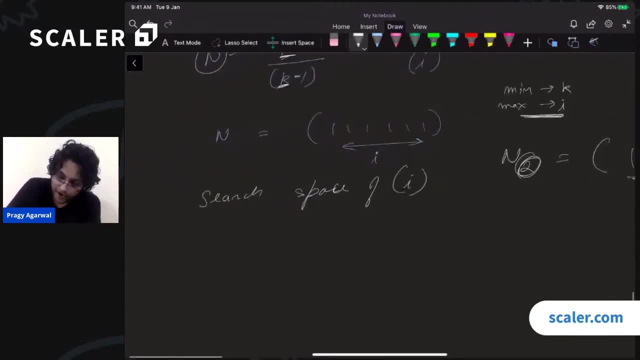 64 bit integer. Right, So I will. the maximum search space, the maximum value of i can be 64.. Right, All the way from 2, all the way to 64 ones in my string, In my string. All right Now. 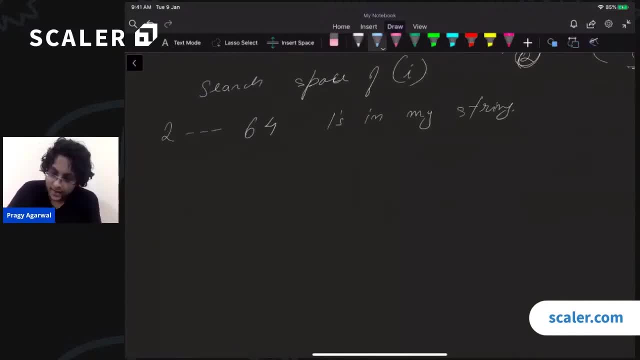 once again, the problem over here arises. Once again, the problem over here arises. If I know, if I know that this sequence of i works, does that tell me anything about this sequence of i or about this sequence of i? Does that tell me anything about this? 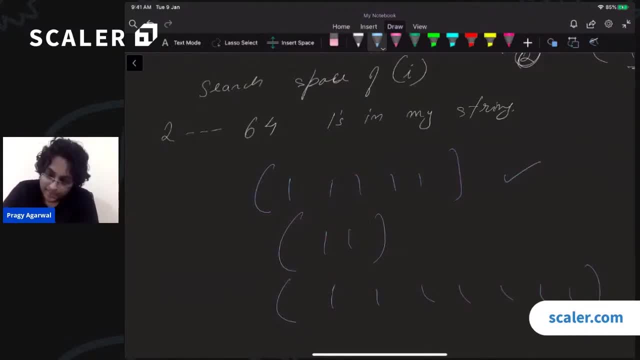 sequence of i or this sequence of i. It does not. I know that I have to maximize the number of ones, But if this works or if this does not work, it doesn't tell me whether I should increase it or decrease it. So I cannot really binary search. I cannot really binary search over 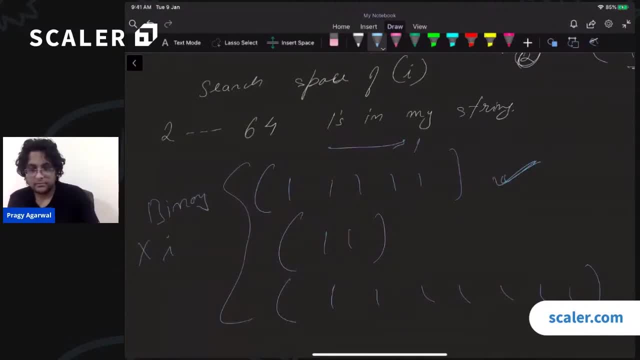 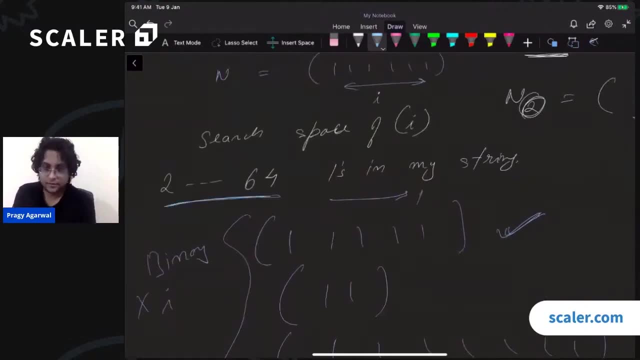 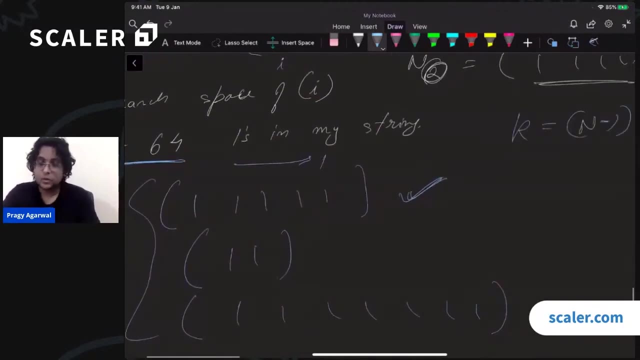 the value of i either. That's sad, But how many i's can they be? We just established that the maximum possible value of i can be 64.. On the other hand, when we were talking about k, we established that a maximum possible value of k can be up to n minus 1.. So what would we rather search? 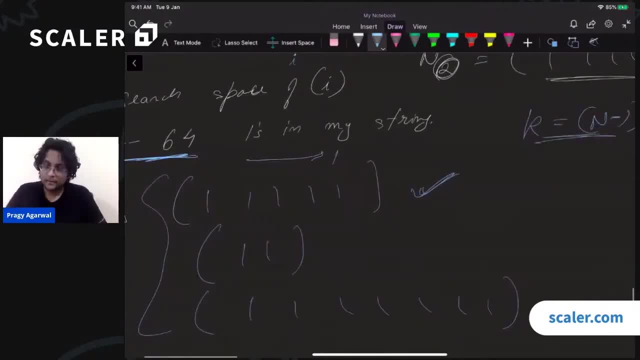 over? search over k or should we search over i? this can be up till n minus 1. this can only be up till 64, right? so this is much better, right, do you guys agree? searching over i is much better. so i can simply check for every possible i, for i goes from 2 till 64. let me check for all the possible. 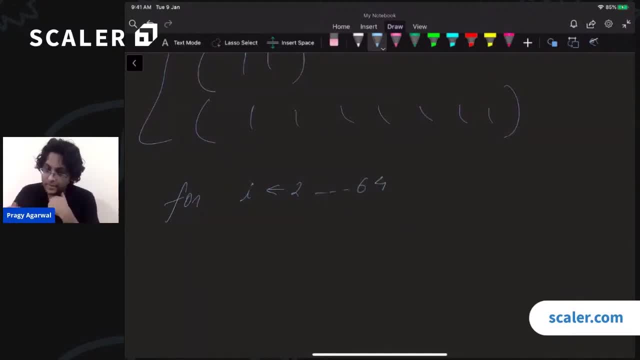 let me check for all the possible strings of 1. let me check all the possible strings of 1. now, what i will check now, i will see. now i will see whether n can be written in the form of 1, 1, 1, 1, i, 1s to the base k, whether i will try to see whether such, whether any such base k exists, that 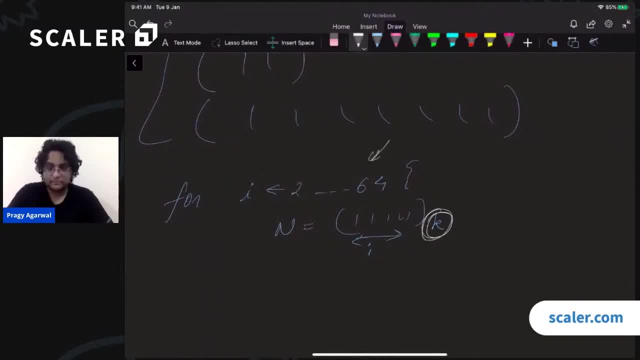 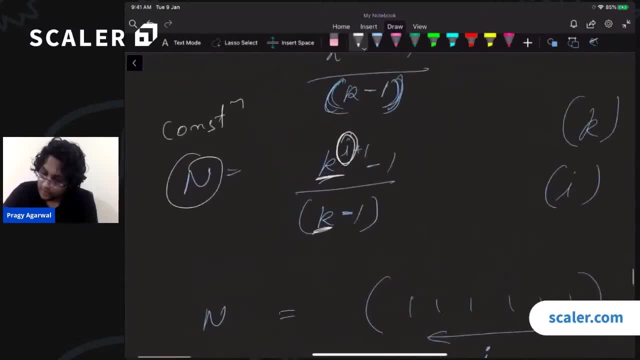 i know the relationship between these two right. i know the relationship between these two right. there is a relationship between all these numbers. I know that. I know that n equals to k to the power i plus 1, right n equals to k to the power i plus 1 minus 1 by k minus 1.. I know this. 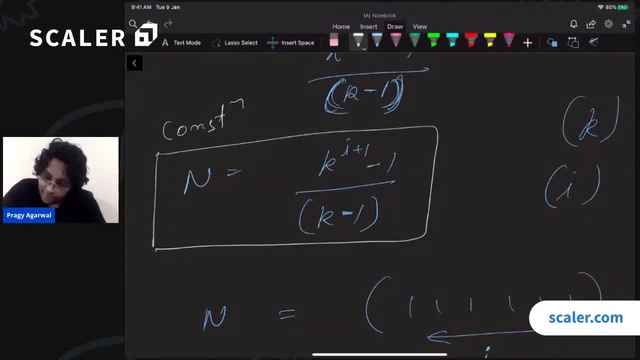 relationship. So now, if I have the value of i and if I have the value of n, can I find the value of k? Can I find the value of k? Yes, How will I find the value of k? That is difficult, right. 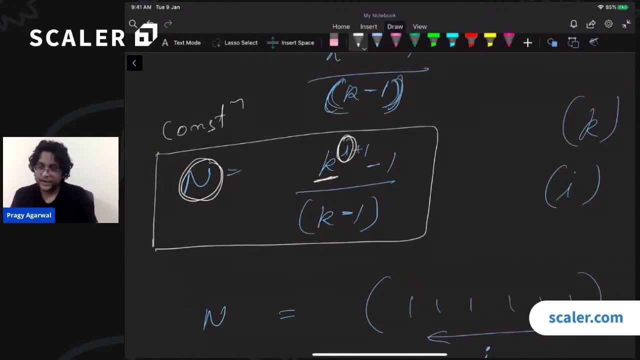 I will have to. I will have to manipulate the formula. right, If I want to find the value of k. I will have to manipulate the formula. I will have to extract k out of it. I will have to extract k out of it. So can someone solve this equation for me very quickly? Can someone solve? 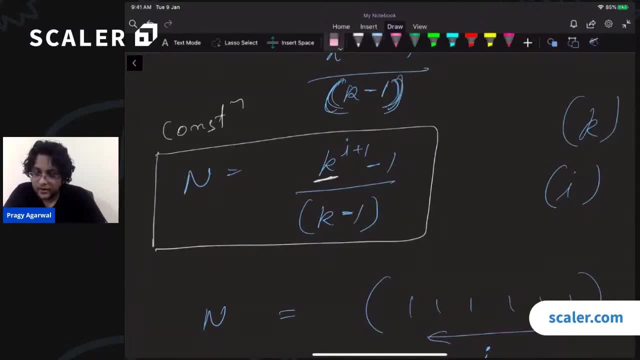 this equation for me very quickly. Well, you can't really. you can't really do that right, Because this k, this, i, might be a very, very large number and you don't. for higher degree polynomials. you don't always have a way of solving an equation, So you can always solve a quadratic. 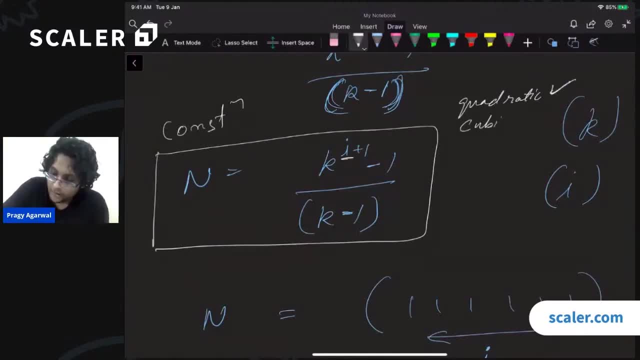 If you have a quadratic equation, you can always solve it. If you have a cubic equation, you can always solve it right. But for higher equations- I'm not sure for the fourth power, but I know that from fifth power and above right- It is not always solvable. It is not always possible to solve a. 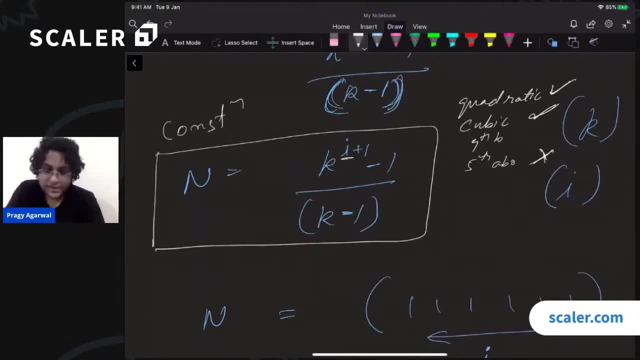 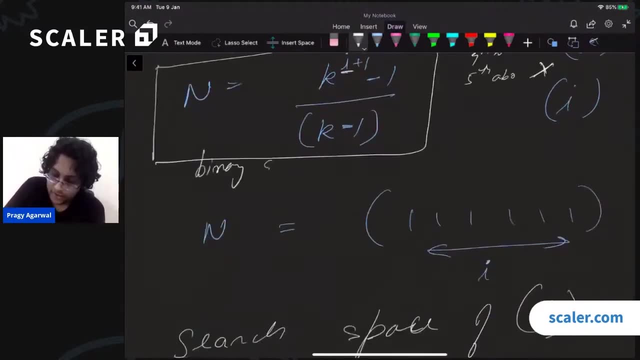 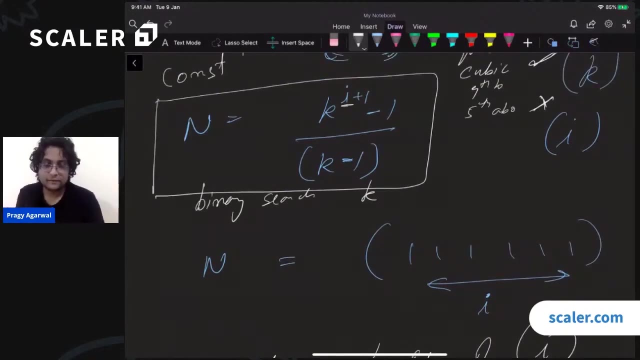 higher degree polynomial right. So this equation might not be solved. So what can we do? Do we have to give up? No, Here is where we can binary search. We can binary search for the value of k. we can try to plug in the value of k and try to binary search for an answer that works. 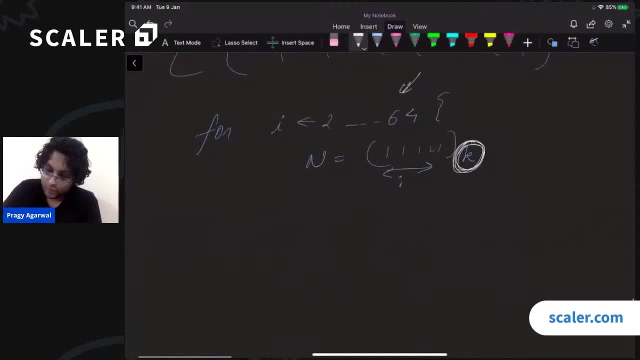 Is that clear? So what we will do now is what we will do now is we now have to find a k that works. What is the maximum possible value of? what is the maximum possible value of k? The maximum possible value of k? so the low. the minimum possible value of k is 2. The high maximum. 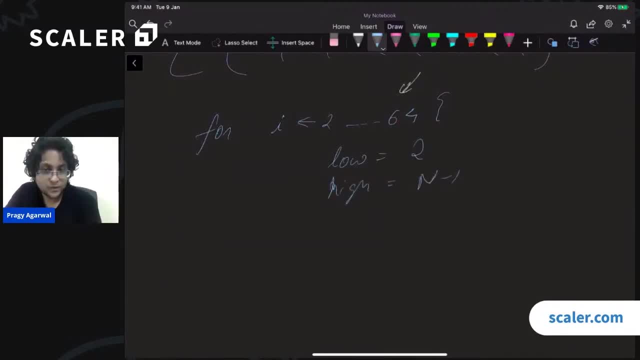 possible value is n minus 1.. And now I can binary search over this value of k. I just have to find 1k that works. I can binary search, binary search for k which satisfies this equation, which satisfies the equation n, n equals to k, to the power i plus 1 minus 1 by k minus 1.. Is that clear? So just like. 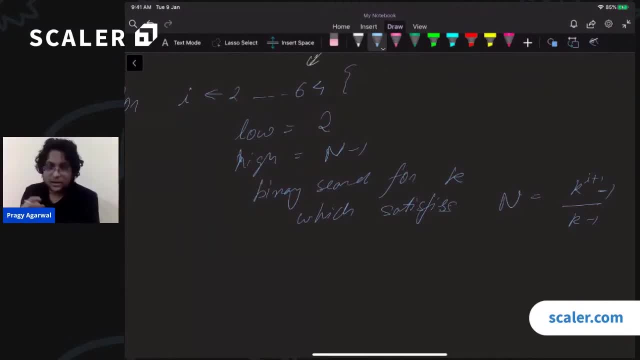 in the first class we tried to binary search. So we did not do it in the class but it was part of your assignment. So in the assignment you had to do a binary search for the square root of a particular number. For the square root of a particular number, Yes, So n minus 1.. This is 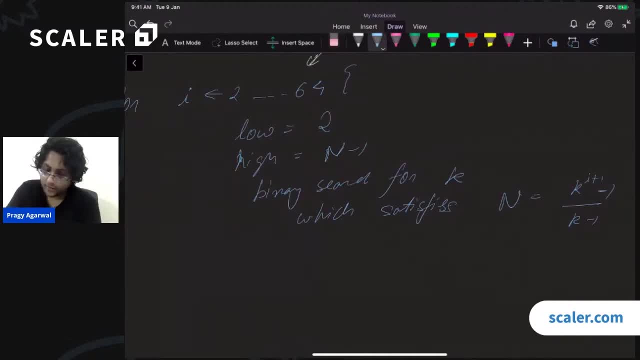 n minus 1.. So we can binary search over the value of k. Is that clear? So how much time will this binary search take? How much time will the binary search for k take? This is my search space. This is my search space. My search space has size of n And I am doing a binary search, so it will take me. 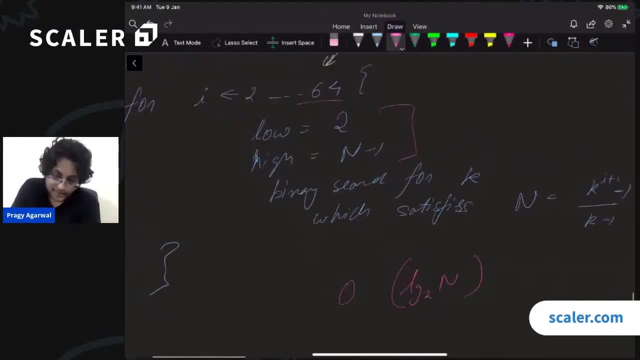 log n time to binary search for a value of k. But I have to do this 64 times. I have to do this for all values of n, So this will be times 64. So the overall time complexity of my approach will. 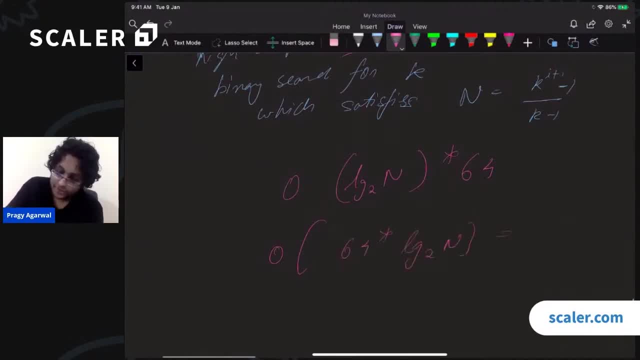 just be 64 times log base 2 of n, which will just be log n. That is amazing. We went from an n log n solution, We went from a n log n. what happened over here? n log n brute force and we reduce it. 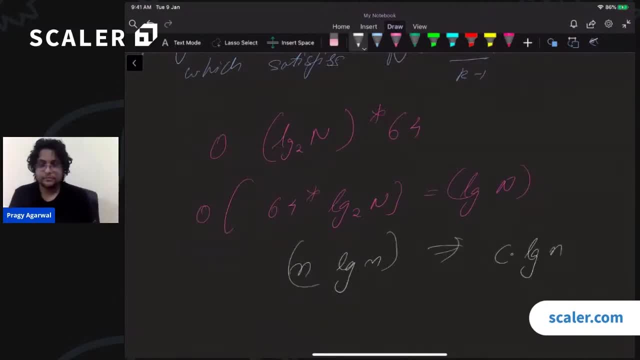 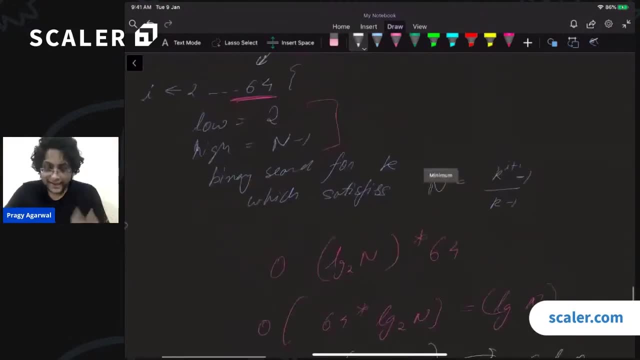 down to a constant times log n, So we can do a binary search for a value of k, But I have to do a binary search for a value of k. Is that clear? Yes, So, even though the question does not directly, 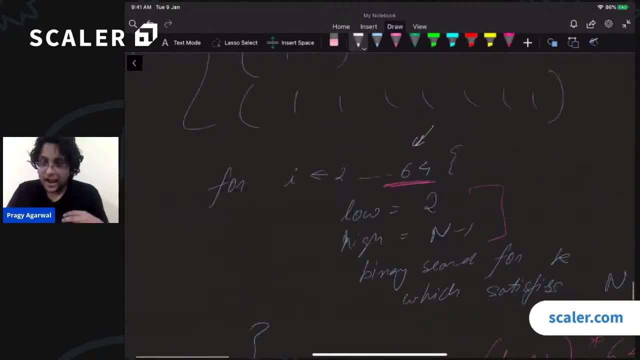 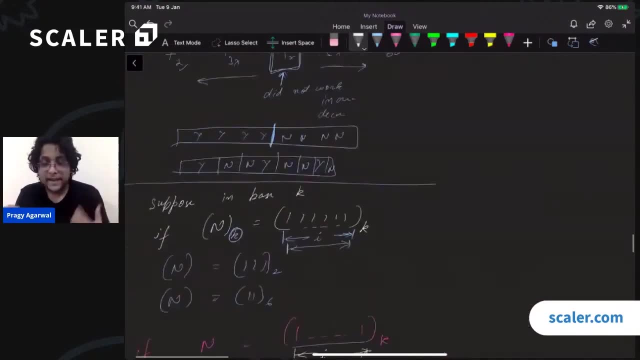 involve binary search. there is still an involvement of binary search And the moral of this particular question is that be very, very careful. Be very, very careful For binary search. you just don't have to make and verify a guess. You also have to understand, given the guess, if that guess worked. 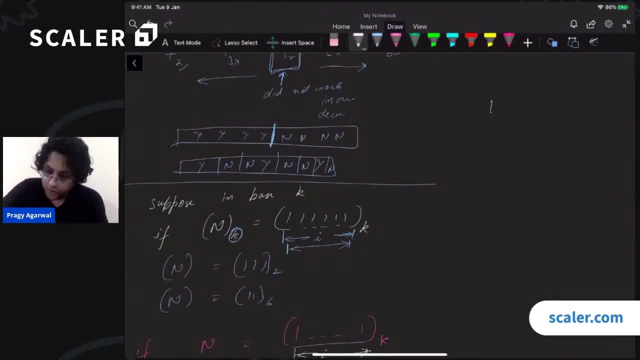 then: is the guess too high or too low? If the guess worked or if it did not work, this is not enough. Establish: is the guess too high or too low, Because if you cannot do that, then you will not be able to binary search for your answer. Is that clear, Perfect? 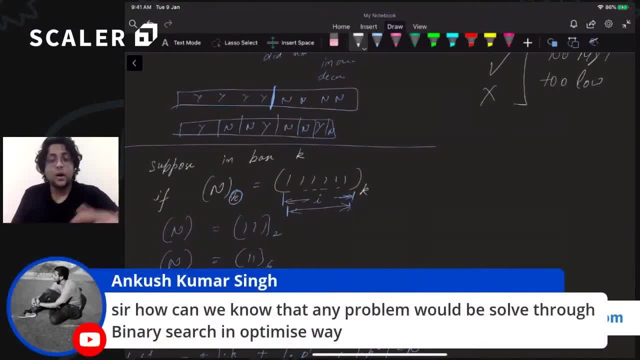 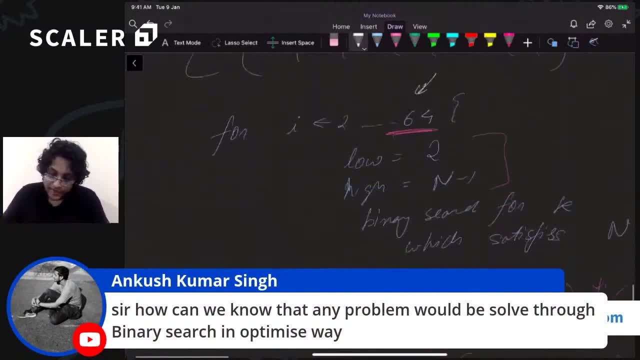 Ankush has asked a very good question. Ankush is saying: how can we know whether binary search will be applicable for this particular question? Now, that is a very, very tricky question. So, basically, the most common answer you will find to this is practice, The most common answer that you will. 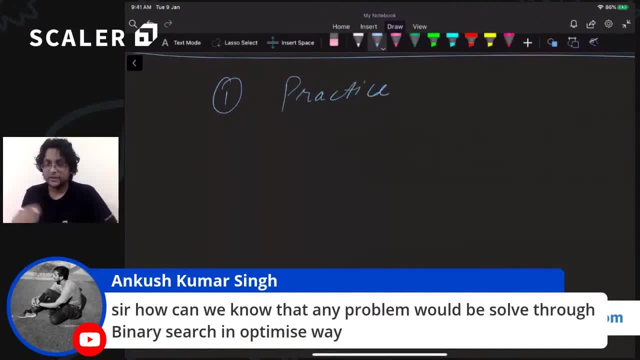 find to it. is that okay? if you just practice, then practice will make you perfect. You will get to know which way, which approach you have to apply. But that is not the entire truth. There is a separate way as well. So there is a systematic way. There is a systematic way of approaching. 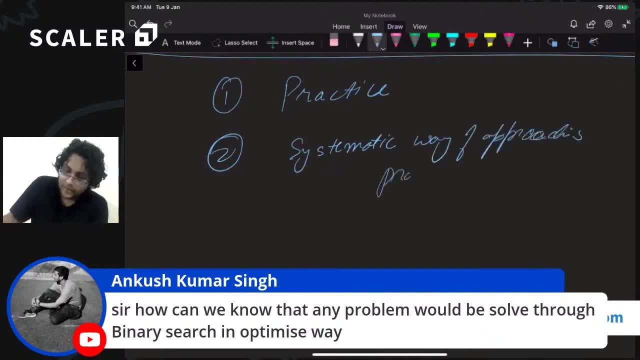 problems, Approaching problems. Now, unfortunately, I cannot teach this systematic way in a YouTube class. I can only be taught in a one hour class. So the entire scale, or the scalar curriculum, the entire scalar curriculum of these algorithms is based on, is trying to teach you this. 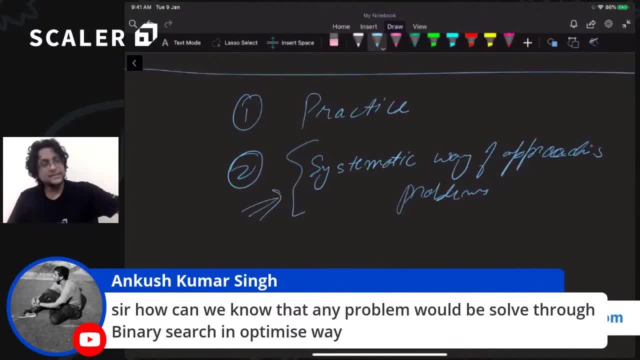 systematic way, So that whenever you get a new problem, you can just apply the systematic algorithm and try to come up with a solution for that. That is what we teach in the scalar process. So I mean we could cover this, but this is going to take a very, very long time. You will have to. 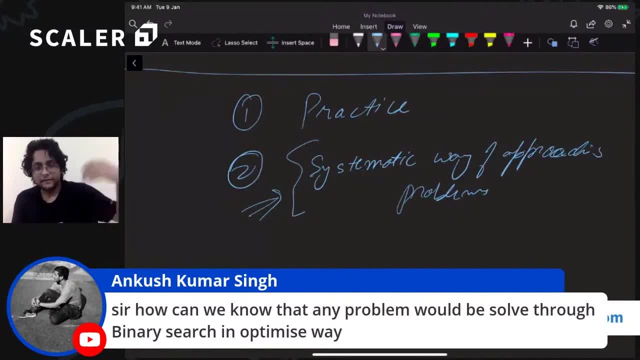 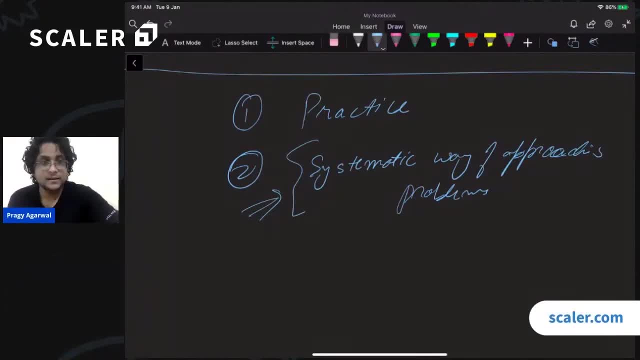 take a very long time. You will have to consider all the DS algorithms and then we will have to tell you the approach. Perfect. So that is it for today's class. Let us end the lecture now And see you then. So, once again, you can find the assignment set in the video description. Please make sure that you attend the problem set. Okay, then have a nice day, guys. 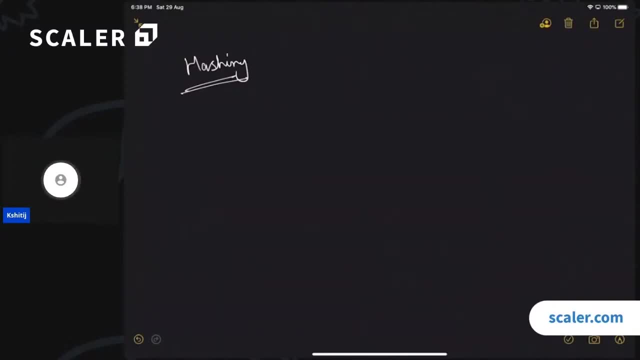 Okay, so today we are going to study a very, very, very important data structure. This is going to be very handy, which can reduce the time complexities of many problems significantly, just by adding a little bit on the space side. Okay, And this is called a hash map or a hash table. Okay, And the whole process is called hashing. 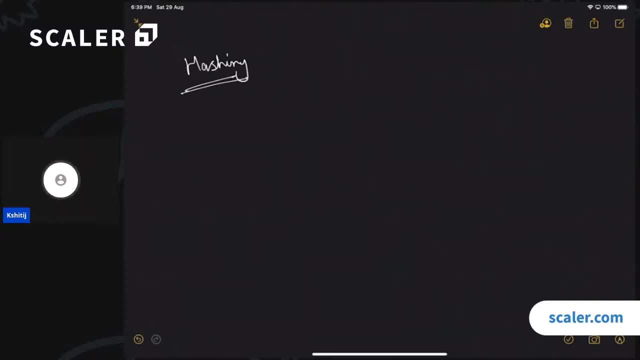 In today's class we are going to study some basics of hashing, how a hash table functions, And we'll also discuss some problems which have been asked in the interviews And we'll see how you can solve these problems optimally using a hash map or hash table. Okay, 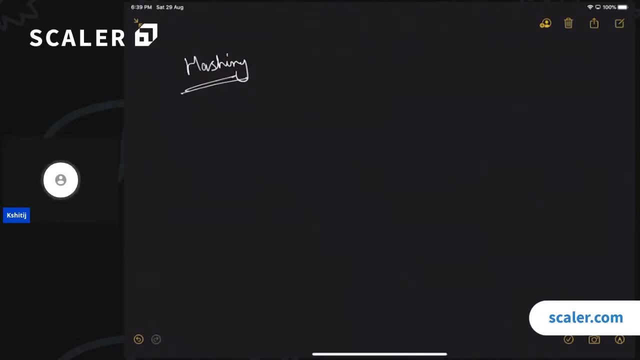 I have a question, I guess: Have you ever encountered hashing in your real life Hashing? Have you ever faced any practical scenario where you have used hashing? Let's talk about those days when there was no corona, or let's call it the pre-COVID era. 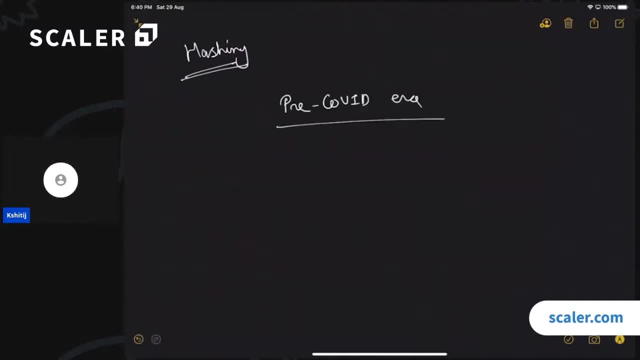 Let's talk about the pre-COVID era. So during the pre-COVID era, we used to go out on holidays- right. We used to go for trekking. We used to go to visit different places- Right, And whenever you go to a different place, you need to stay in a hotel. 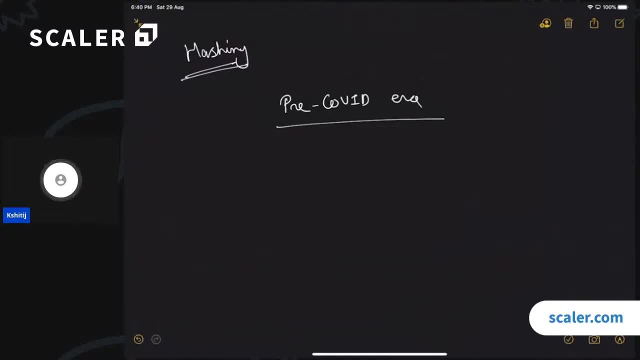 Right. So let's say that if you go to a hotel and you want, if you want to look for a room, right. You go to the receptionist and ask whether a room is free or not. Now the job of the receptionist is that he will take all your preferences. 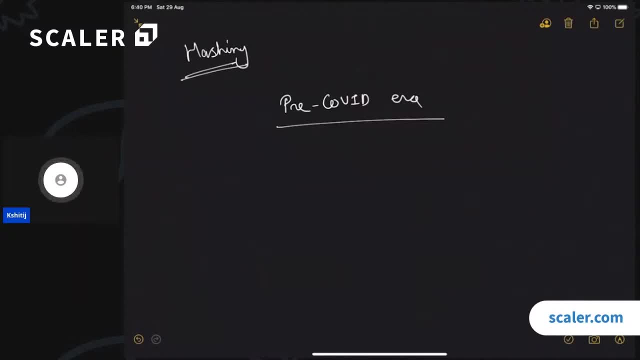 He will ask you what type of room you want And then, based on your preferences, he will just check whether a room of those Is free or not. Right? So you go to a hotel and in this hotel you have a receptionist, right? 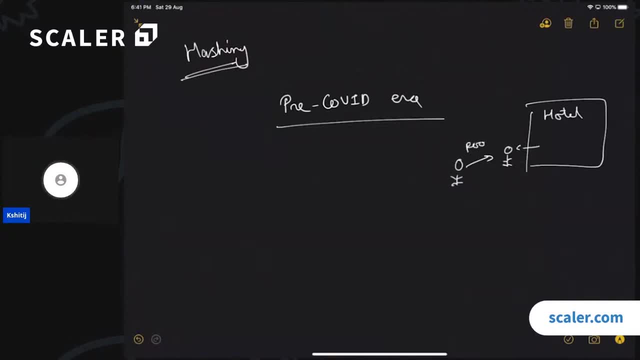 And you go to the receptionist and you ask for a room. Give me a room which, let's say, is a single bedded room, has a AC, has a balcony and all Right, And this guy will just check whether a room is free or not. 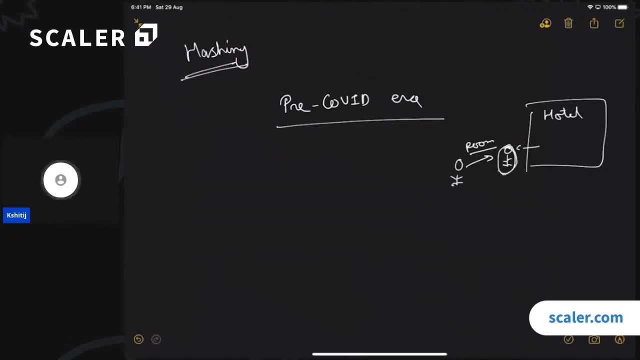 Now this guy has got two ways to check the room. First is that he can actually go and he can visit all the rooms of the hotel and check whether such a room is present or not. Right, He will go, he will knock each and every door. 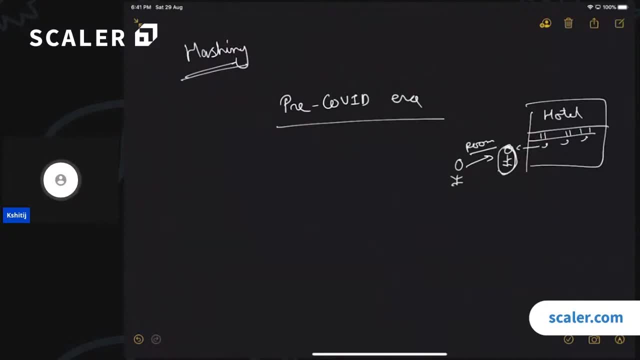 He will check whether the door is closed or whether the door is open, whether the key is with him or whether the key is with the person who has taken the room Right. So this is one way. Now, as, as all of you can see, that this is a very, very unoptimized way of finding a. 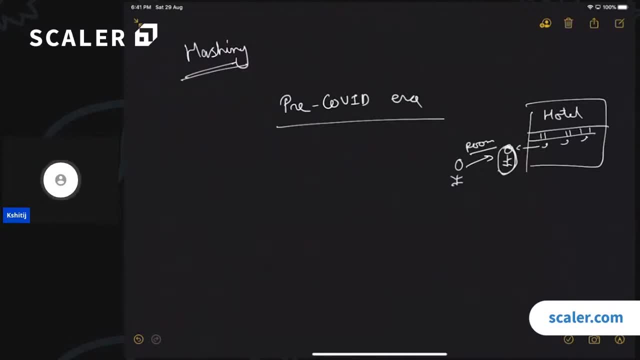 room, right? Because if there are, let's say, 200 rooms in this hotel- this is a very big hotel- Then he's going to check each and every room For each and every customer, Right? So if there are N customers and if there are M rooms, then how many checks is he going? 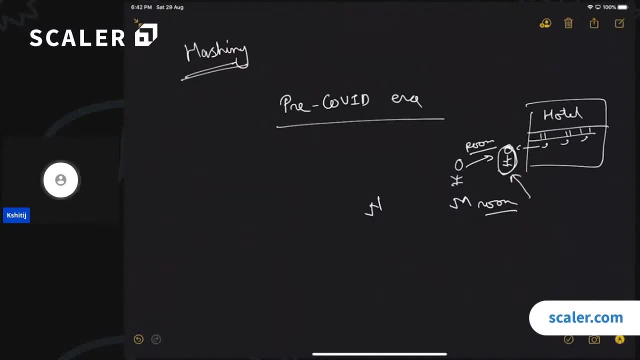 to make. This unoptimized receptionist is going to make N into M checks. This is not going to be profitable for the hotel business. Whoever is the owner of the hotel, he will fire him the next day, Right. The other way that this guy can use is he can maintain a. 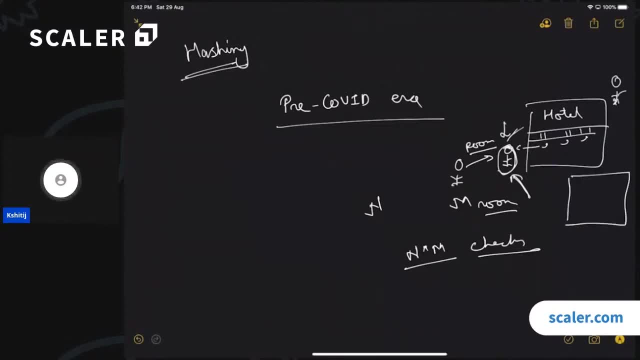 Map, Right. He can just uh against each and every room, Right, Let's say room number 1: 0 1 1 0, 2. He can maintain whether this room is occupied or whether this room is empty. 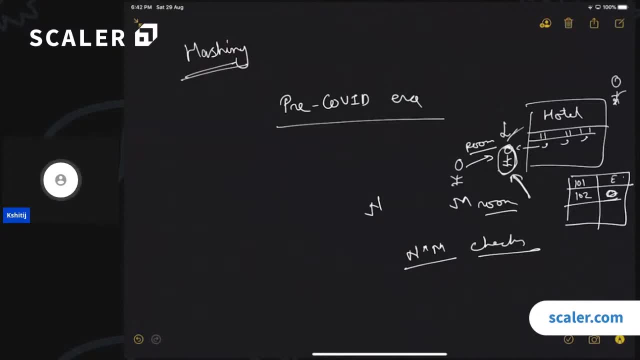 Right, Or he can also, uh, have, uh, the keys in the key holder itself. He can also have the room number written Right. So now, whether he has the key or not, that is also visible here. Whether the room is empty or not, that is also visible here. 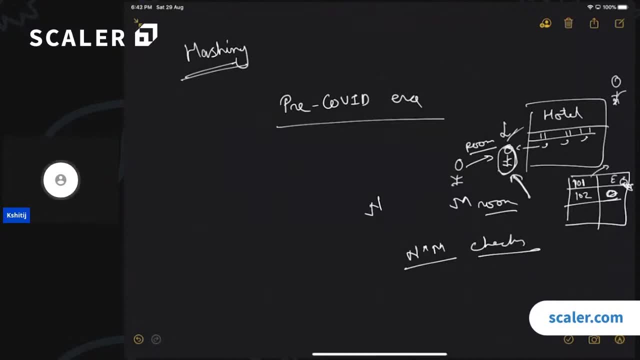 He can also have Uh the type of the room written here, So he can have uh that 1 0 1 is a single bedroom which is empty. 1 0 2 is a single bedroom which is non-empty. 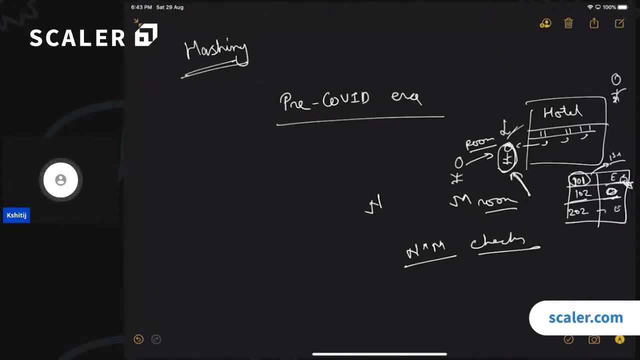 Let's say 2 0. 2 is a double bedroom which is empty. Right, So he can have each and every information regarding the room stored against the room number. Okay, Is this going to be a better choice? Yes, Right. 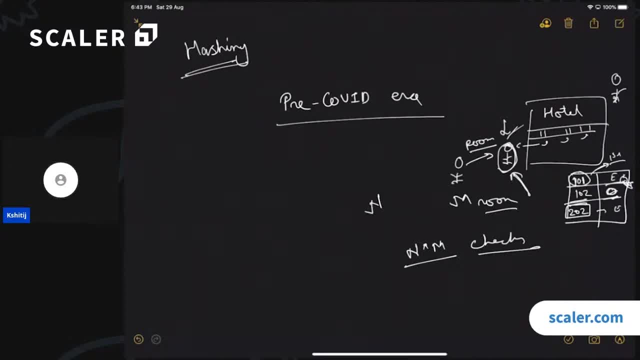 That is why each and every receptionist actually does this. You must not have seen any receptionist who actually go and check all the rooms, Right? But this is something which you all must have seen, Correct? Uh, let's talk about another example. 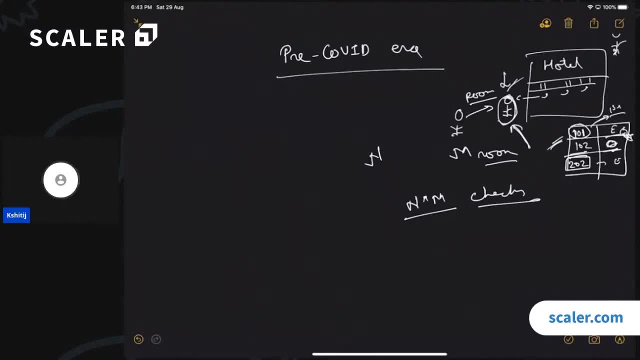 Okay. So let's say that in those days, you also used to go to shopping malls, right? So this was an example where we want to stay on a hotel. Another example would be that if I want to go to a shopping mall, Okay. 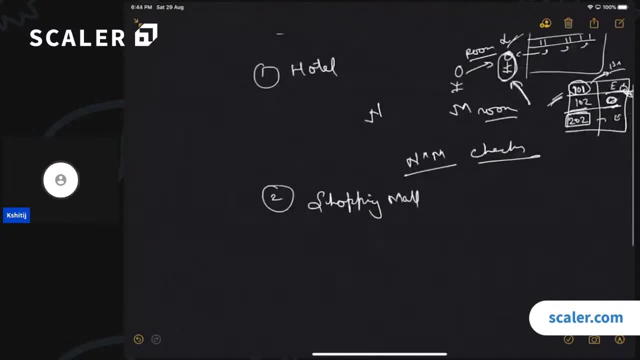 Now, if I want to go to a specific shop in the shopping mall again, there are two ways that either I go And check each and every shop in that mall, Right, So there are going to be multiple floors in that mall. 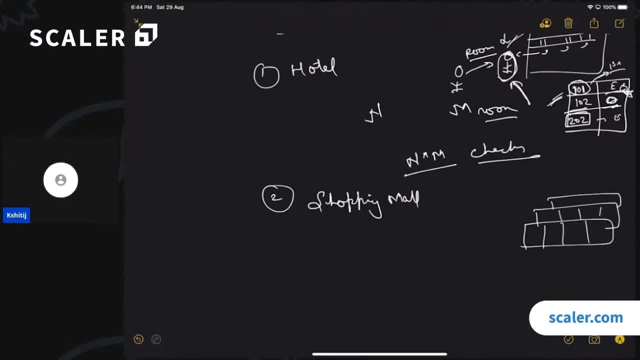 Right, Each floor will have different shops, Right, And let's say I'm looking for a specific shop, Okay, Let's say I want to buy, uh, the magical drug Coronel. Okay, I have a perception- I have read on on WhatsApp- that if I take Coronel then Corona is not going to catch. 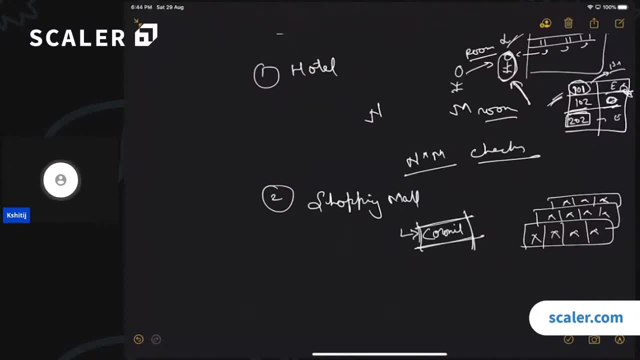 me Right. So what I would want is I would want to search this shop which is selling this drug, Coronel, right now. again, I have got two ways to do this. First thing, that I go to each and every floor and I take each and every shop one by one. 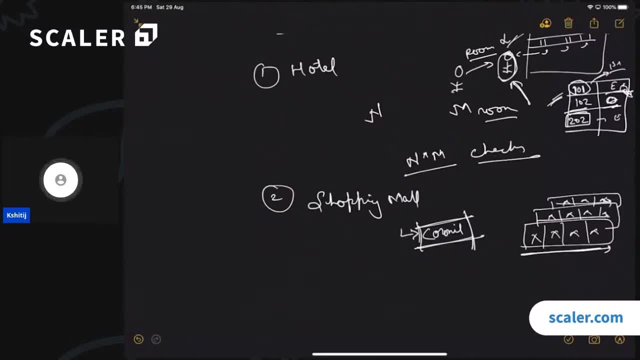 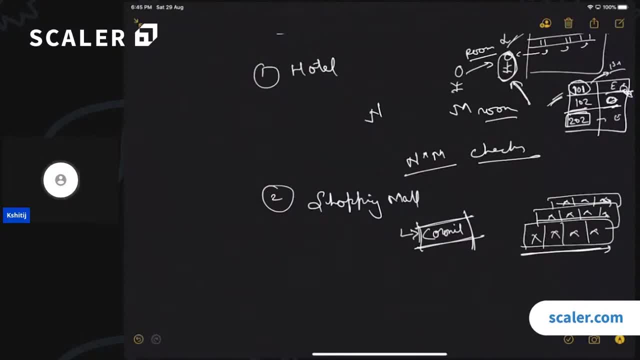 uh, uh, uh uh. shop number: Uh, they, they give the complete address of the shop. Uh, floor-wise, they will say that in the first floor these are the shops which are there in this order, right. 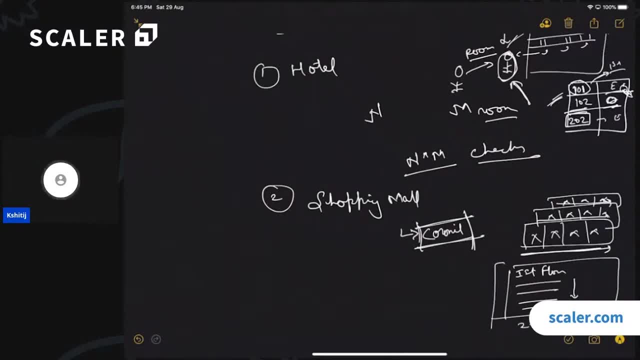 And in the second floor these are. these are also. what I can do is I can use this map and I can find the exact location of the train And then I can go to the shop. by this, I can make sure that Corona is not affected. 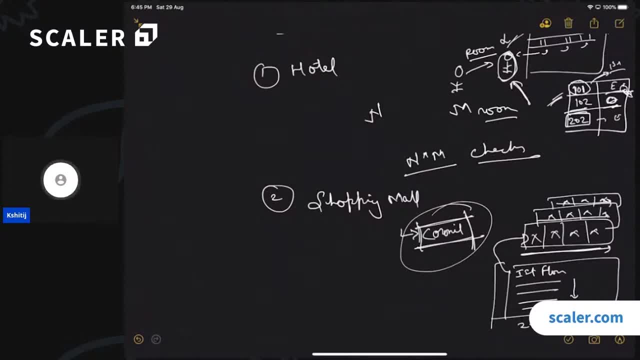 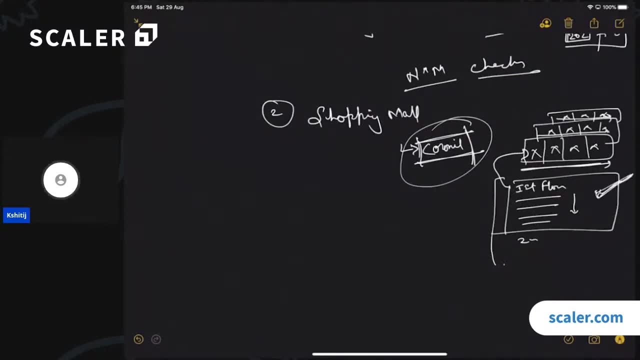 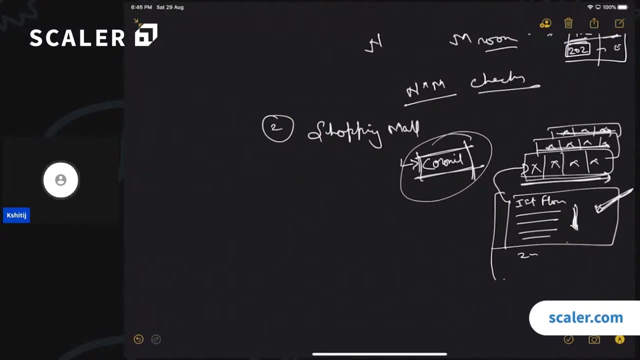 But since this was a knowledge that I gained from WhatsApp, this might not be true, right, but this way of searching the shop, this definitely is a better approach, right? instead of visiting each and every shop, what i am going to do is i am going to check this map and then find the exact location of the shop. okay, does this make sense to everyone? 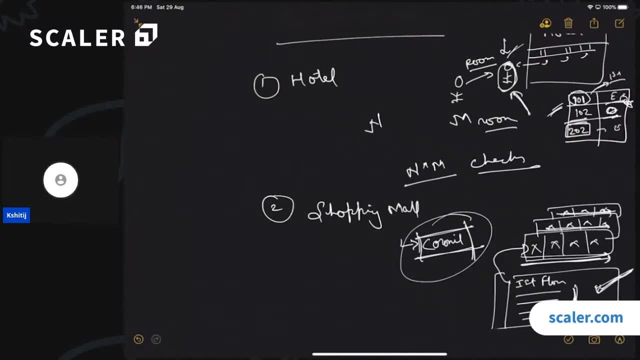 these are two examples which all of you must have used like these or something like this in your real life, right where you have to keep track of things and you just create a table, or you create some entries and just mark profiles, or you just the attendance register that we have. 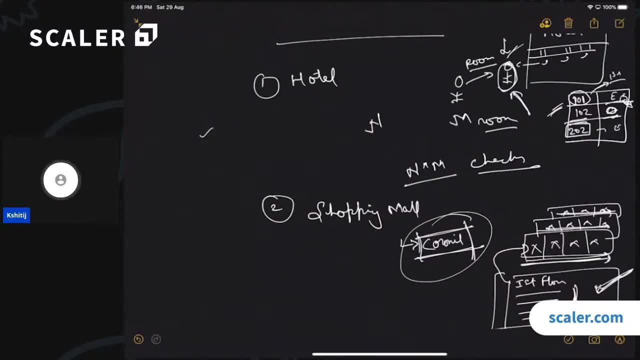 that we used to have in our school classes. right, that was also an example of hashing. if, let's say, a teacher wants to know whether a student is present in the class or not, right, what he will do is he will just do a linear scan on all the students, and doing this linear scan, 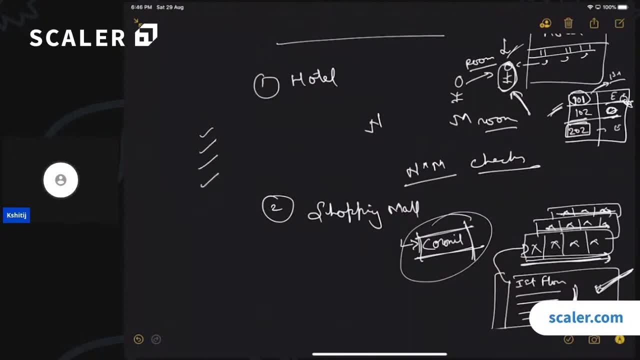 while taking the attendance he also keeps, he also marks the attendance right. so if there are the students, let's say in our class we have aman, then we have monica, then we have and more right. so if i have to check whether all of these guys are present in the class or not, 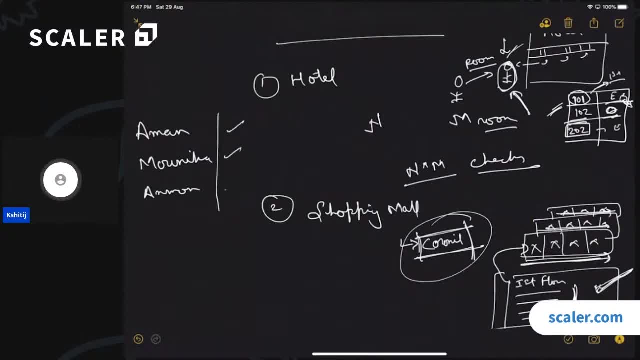 what i can do is just before beginning the class, i can just mark their attendance right now. if, let's say, after some time i want to know who all were present in the class, i will not do another. i will just check whether monica is present, whether aman was present or not, right so? 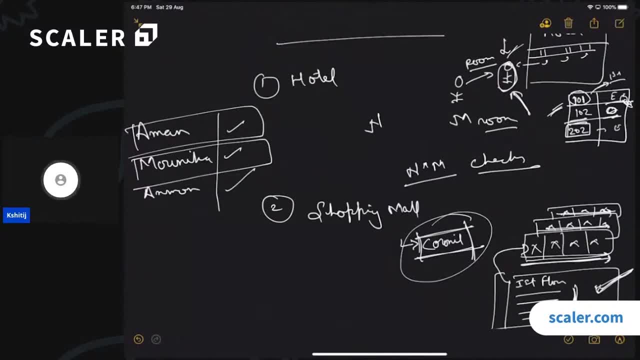 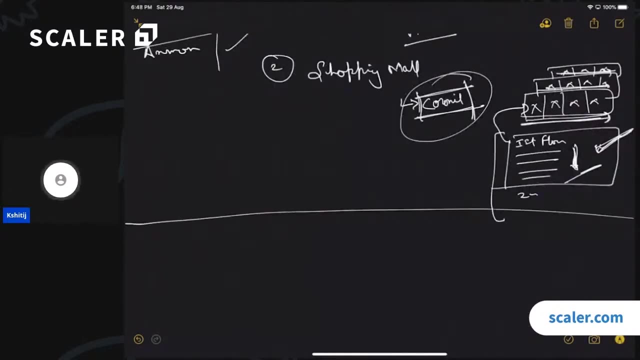 this again is another example of hashing which we have been seeing from the school days. right, okay, is oyo also used concept of hashing? yes, oh, you must also have used this same concept, right, okay? so this is. this is the general idea of hashing. now let us see how it actually functions. 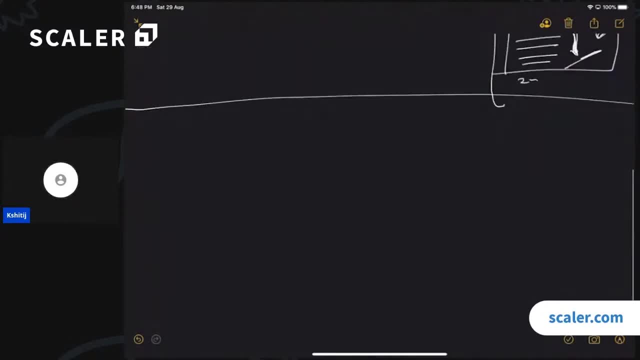 in the- uh, in the world of computer science. okay, so let's try to understand this whole process using an example. so let's say that, uh, we are given an array and this is just to understand how hashing is going to function. okay, this is going to be a very easy example to understand. 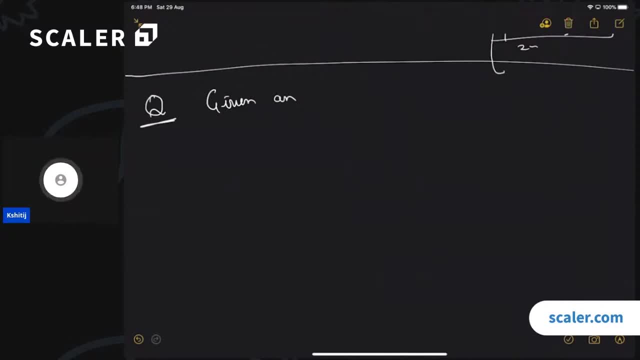 the working of hash maps and hash tables. okay, so let's say that you are given an array and in this array you have all the numbers from range one to thousand. so you know that any number in this array is going to be from, or let's say from, zero to thousand. 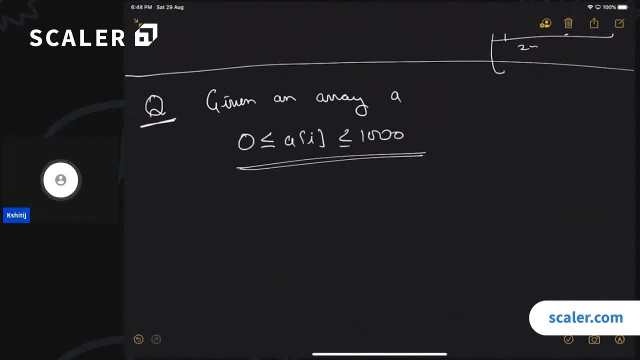 okay, so you're given an array of size n and each and every number of this array ranges from zero to thousand. okay, you have to return the frequency of frequency of every number. let's say you have got queries about the numbers. okay, so you have this array and now you are getting multiple queries. 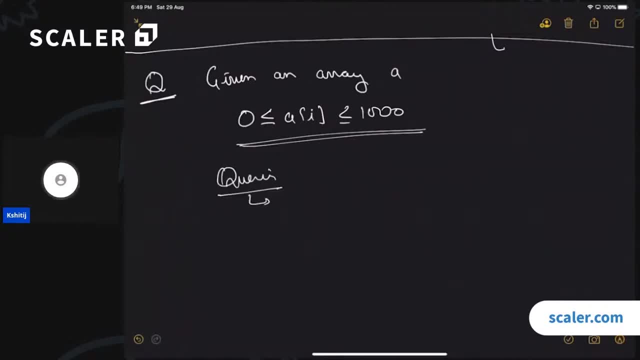 you have to answer these queries and each query asks you the frequency of a number. okay. so, for example, if the array is something like this, okay, if this is the array. after getting this array, you will get different multiple queries and you have to answer what is the frequency of the given number in that query. so, for example, if your query 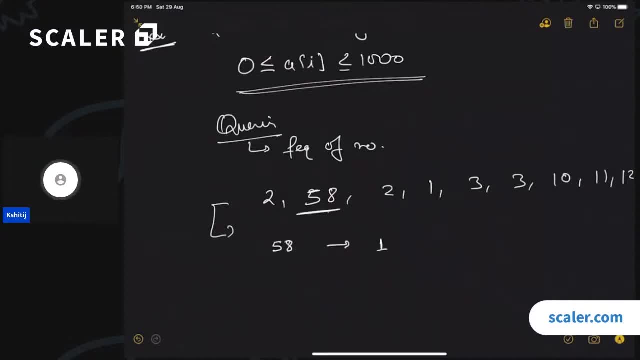 has 58, you will return one, because 58 occurs only single time. then if let's say: uh, you get three in the query, then you will be returning two because three is operating twice in this array. if you get two, you will again be returning two because two again depends twice in the야. Okay, 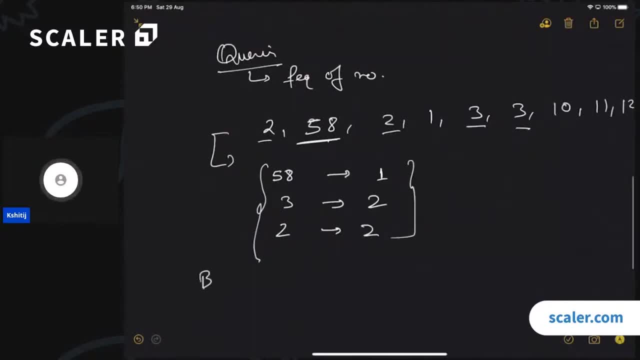 okay, let us, let us start from the brute force. okay, what is the brute force way to solve each and every query? the brute force way to solve each and every query is that, whenever you get a number in the query, you iterate over this complete array and you count the. 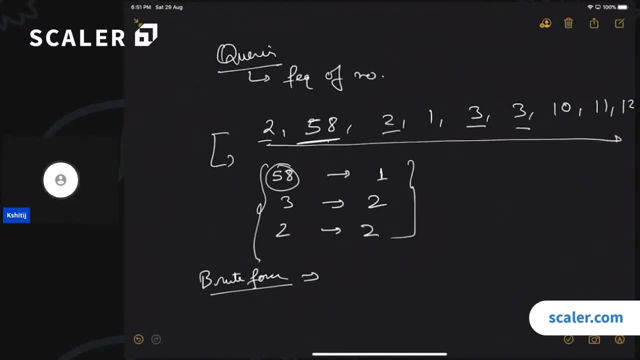 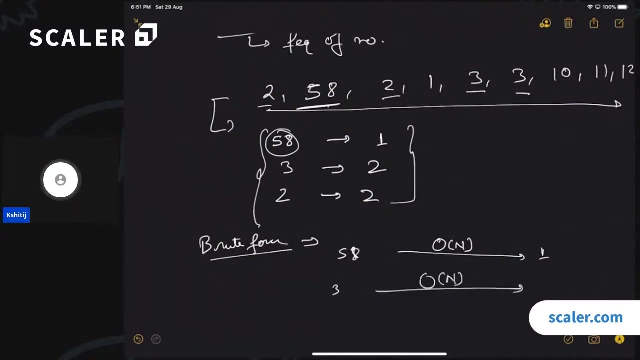 complete array and you count the operances of that number right. so if i get 58, i will do an iteration over the complete array, which is going to be an order n operation, and then i will return 1. if i get 3, i will again do another order n operation over the complete array and i will 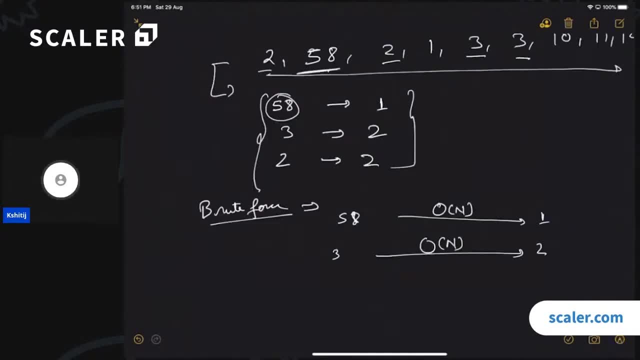 return 2. okay, so what is the total time complexity of if i go by this approach? let's say there are q queries, solving each query takes order n time, so the total time complexity is going to be q into n. right now this q can be very, very large, okay, so this is something which is not optimal. 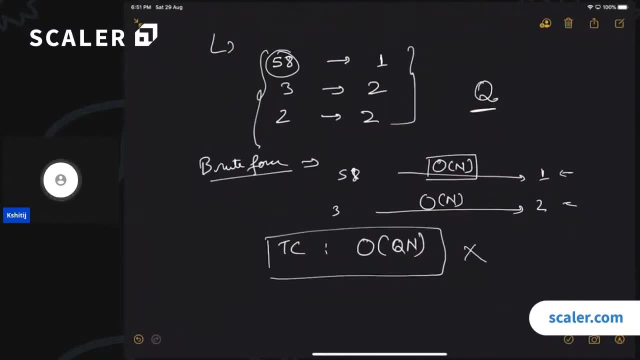 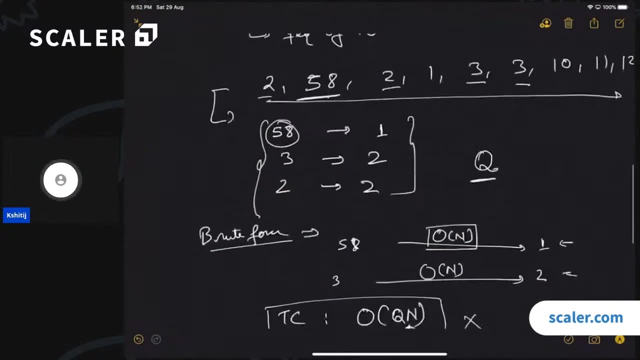 right any other approach that we can use in this case that you might have studied in the previous classes. can we optimize this order and factor here? let us say, if i do some pre-processing, okay, if i solve the array, if i sort the array, what happens to the order now? the order is the array sorted in. 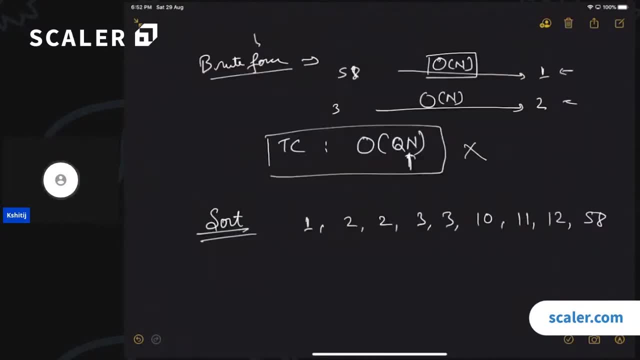 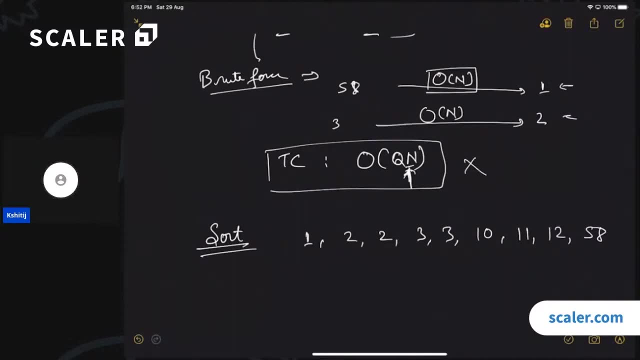 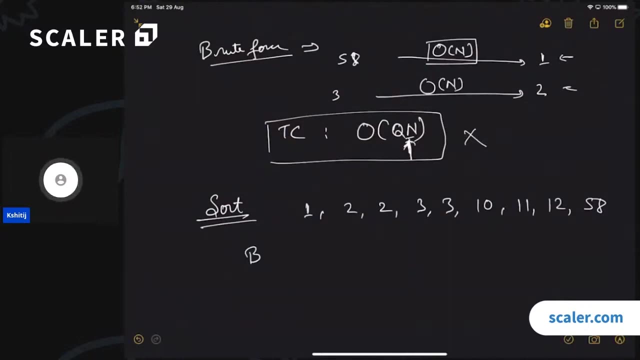 ascending order right now. can i find the frequency in a more optimal time? can i reduce this factor of n? yes, now, how can we count the frequencies? now we can use binary sets. you must have studied this, you must have learned it in the previous sessions, that, given a sorted array, you can count the number. 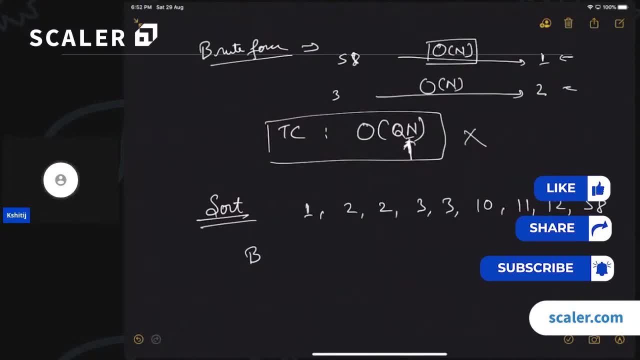 of operances of any element using binary sets right. you can just find what is the first occurrence of that number using the binary cells, then you can also find what is the last occurrence of the number and then you can get the length of this server right. so if you 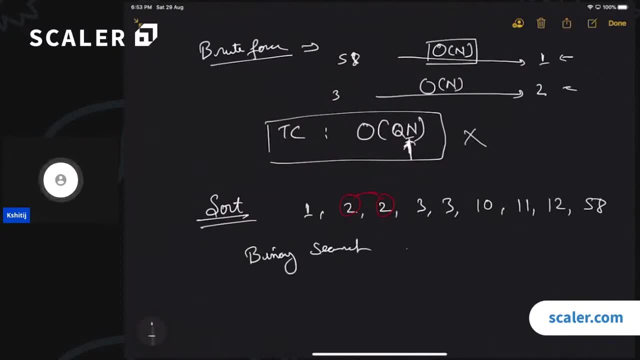 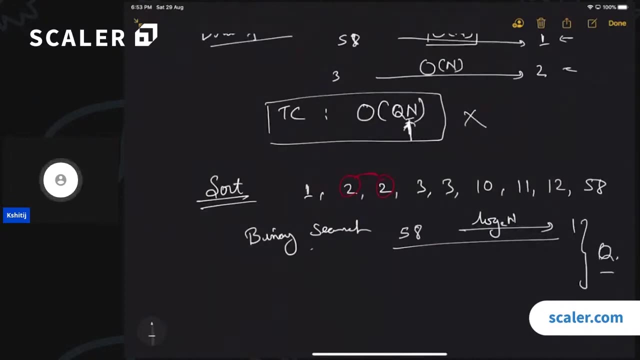 use binary search after sorting, then each and every query is going to take how much time? only login time, right. so now what is the total time complexity of finding all the frequencies? so if you have q queries, then solving all the queries is going to take you q into log base to n time. this much is the time that. 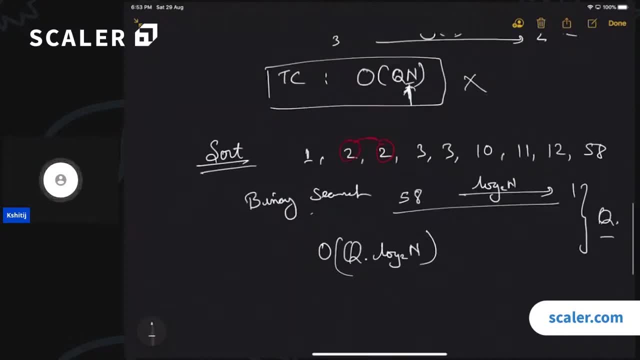 you will invest in resolving each and every query, but before this you have also sorted the array right, so that amount will also be counted. now, whichever is the greater of these two will be the overall time complexity right. this is still is a lot because, again, n can be very large, q can also. 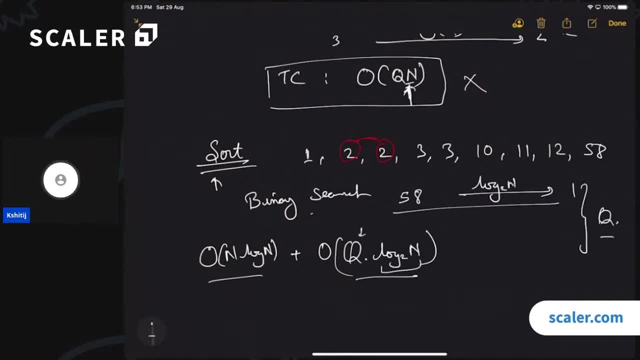 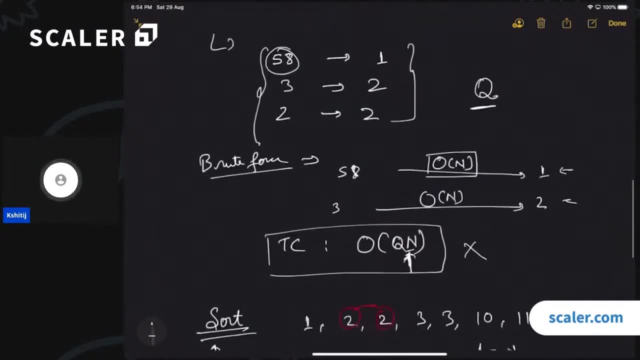 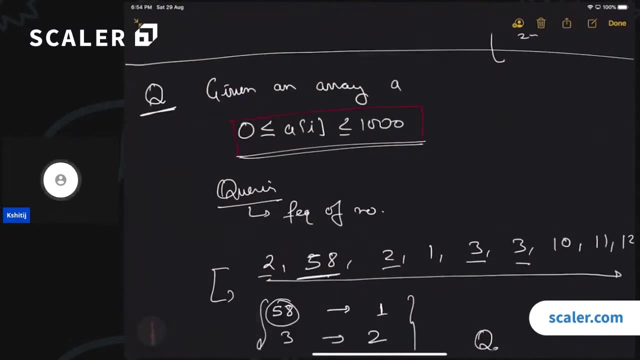 be very large, right, so can we further optimize this? right? so, as many of you have already already suggested, what if i have another array? right, so i can see here, if i focus on the constraint of the problem, the problem says that any array value is going to be in this range. strictly right, any 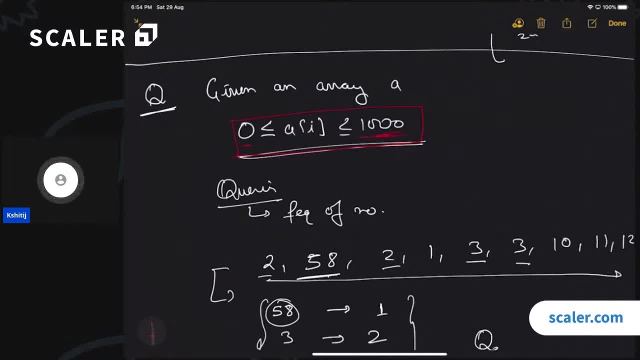 array value cannot be more than thousand and it cannot be less than zero, right? what if i just have another array where each and every index of the array represent the numbers and the value in the array represents the frequency of a number in this original array? so what if I have another array? just call it a frequency array. 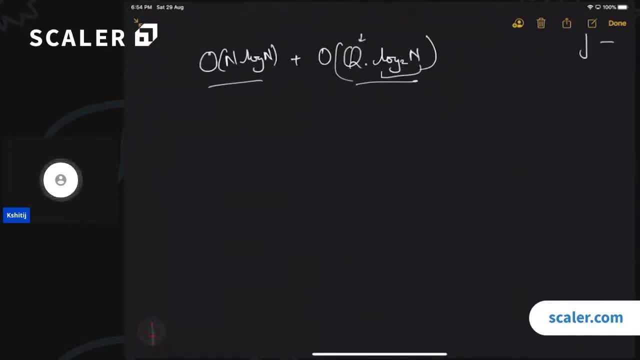 right and and store and count the frequency of each and every original array element in this array right, so I can have another, let's say, frequency array of size. what should be the size of this array? what should be the optimal size of my frequency array, if I know that all the numbers are going to be in? 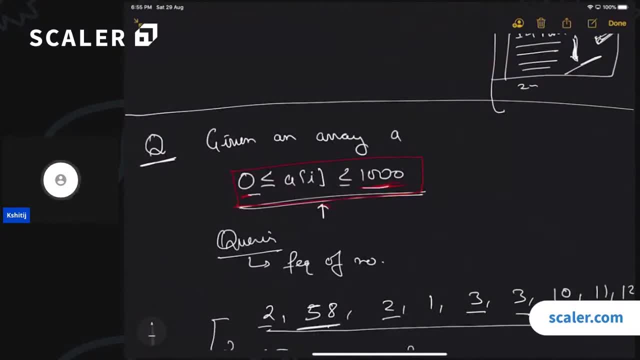 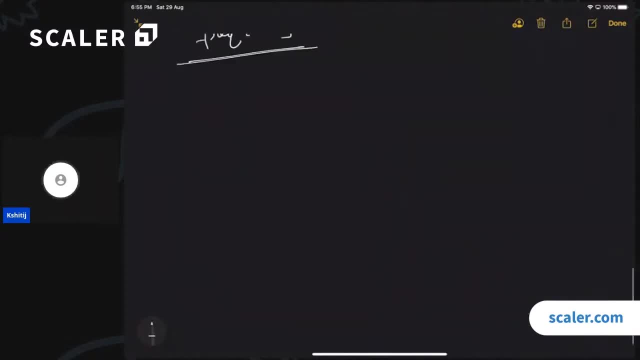 the range from zero to thousand. I know that the maximum number that I can have is thousand. to have thousand as an index, I need an array of size: one zero, zero, one right, one thousand one. this this array is going to be. this array can accommodate all the numbers of this array, right, so I can have another array. 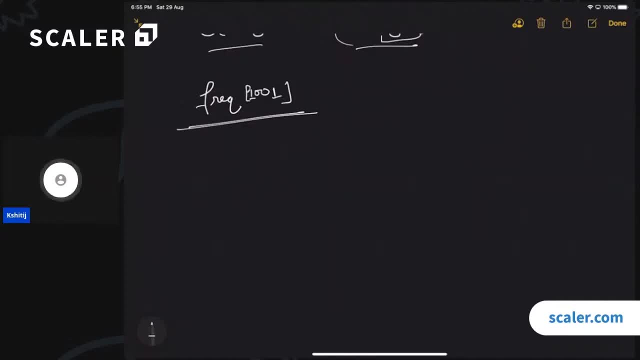 number from zero to thousand in index right. so now what I will do is whenever I am iterating over this array. so initially I initialize this complete thousand sized array by a zero. so in this array, initially I have thousand zeros in every index right and then whenever I visit a number, I will just 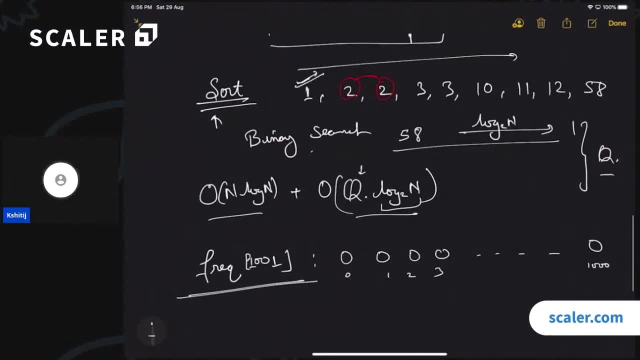 loop over this array. whenever I visit a number, I will increase. I will increase the value here because this denotes the frequency. so so initially I am assuming I infinite, I am assuming that frequency of each and every number is zero. whenever I am counter a number, I will increase the frequency. 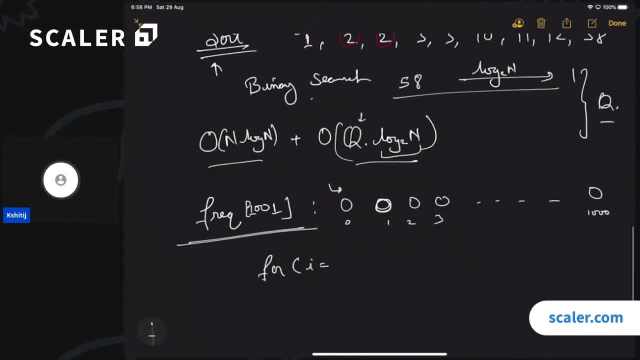 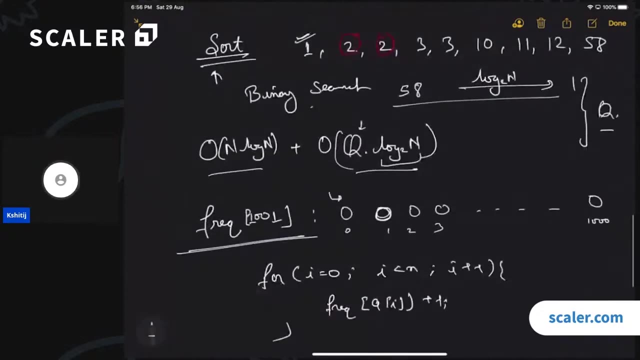 right. so I will just loop over this array. I will say, for i equals to 0, i less than n, which is the size of the given array, i plus plus, and I will say: frequency of A of i plus plus right. if I just do this, what will I get in this array, frequency of one will be increase to one right and then 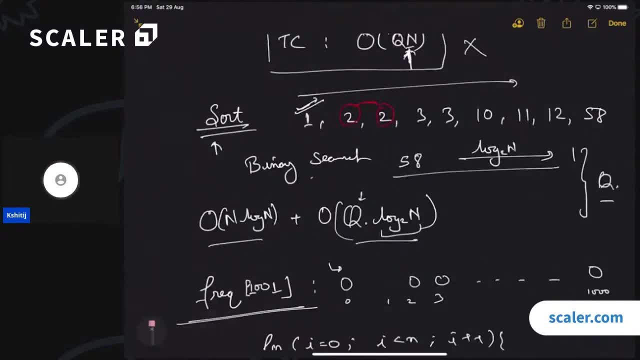 if I just do this, what will I get? in this array, frequency of one will be increase to 1, right, and then frequency of 2 will also be increased and it will be 2, frequency of 3 will also be 2, and so on, right. 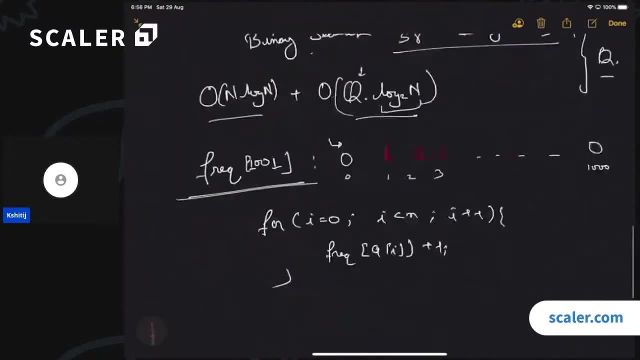 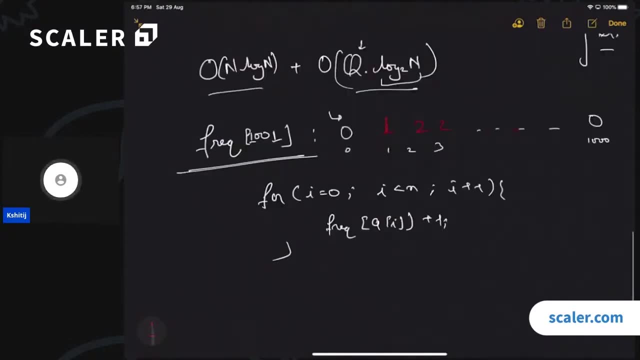 so now, after i have built this array, if i have to return, what is the frequency of any given number, right? what is the operation that i have to do after i have built this array for any number i, for any given number i, if i have to return, what is the frequency? frequency is nothing but. 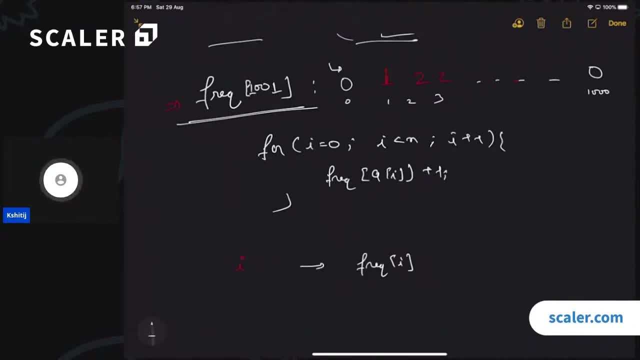 frequency of 5. so if i have to return, what is the frequency of 58? i will quickly do frequency 58. if i have to return, what is the frequency of 2? that is going to be frequency of 2, and that's it, right. so what is? what is the time? complexity of this operation. time complexity of this operation. 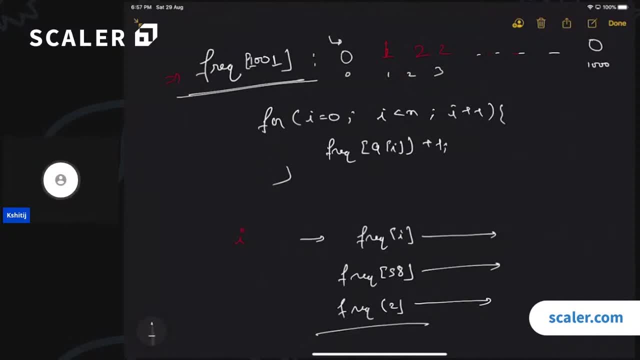 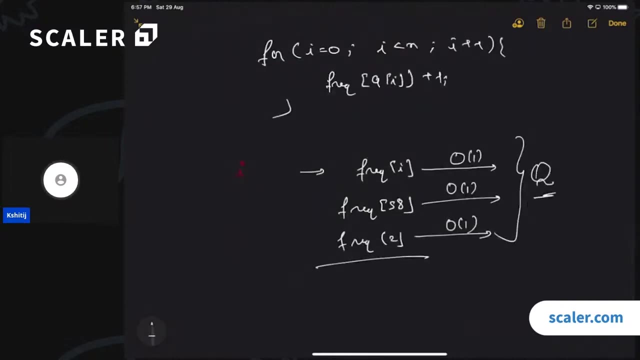 is constant, right, this is a constant time operation. i'm just retrieving a value from the array, right? so this is going to take order one time, correct. now i have a few queries and each query is being solved in order one time, correct. so what is the overall time complexity of solving all these queries? overall time complexity becomes order. 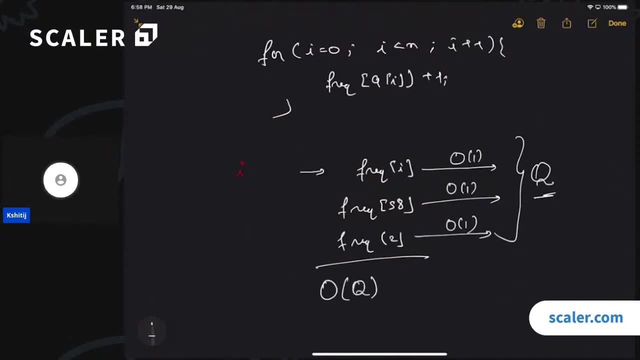 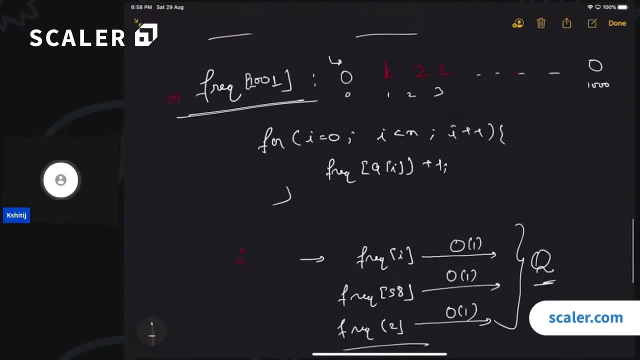 q, because each and every uh query is taking how much time? only order one time right. so this is the time to resolve each and every query, and then we have also built this array right. so we have iterated over the given original array and then we have also built that query and now we have 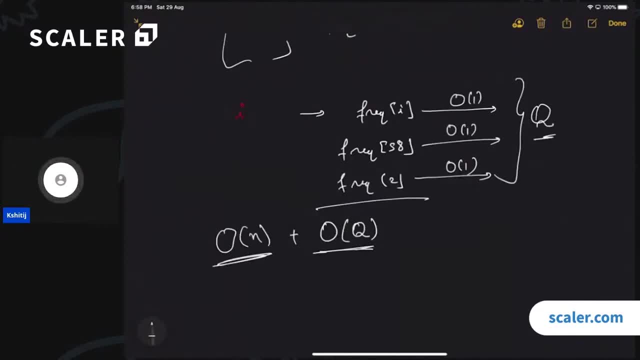 that array. so this takes order and time: order n plus whichever is greater will be the final time. complexity: okay, does this make sense to everyone? how we have solved this like: optimize the time complexity from n square to n log n plus q, log n to order n plus q. okay, now one of you just asked: 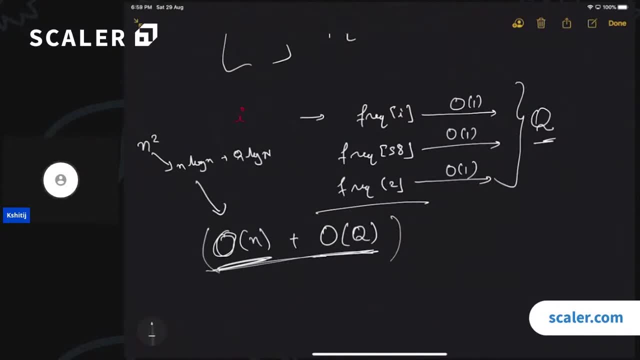 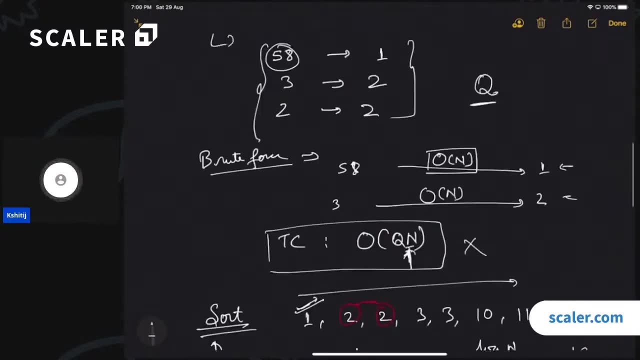 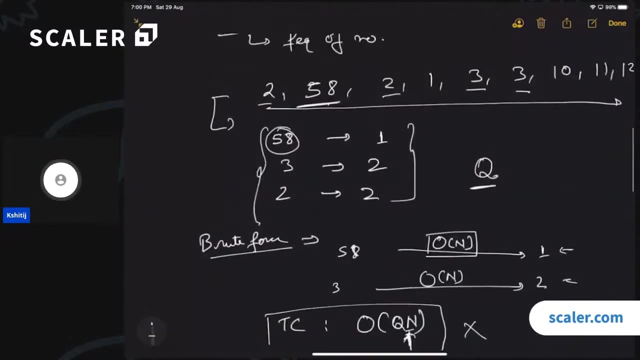 what happens when array elements range from one to one raise to power, or 10 raise to power, 18? okay, what, if so? in in this problem, it was given to us that the numbers are going to range from 0 to 1000. that is the reason why we are able to create an array. right, i can create an. 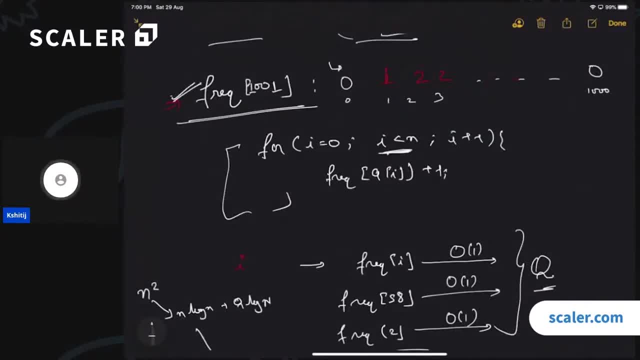 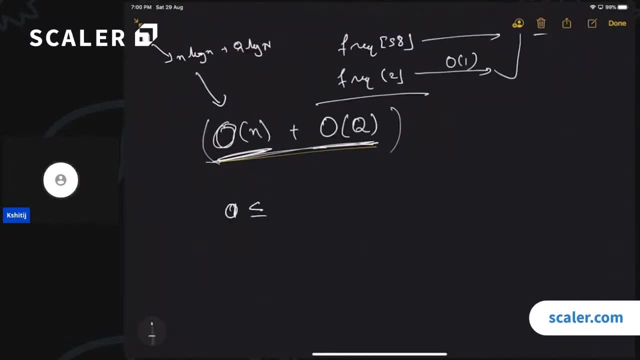 array, because i know that indexes can be in this range, correct. now what if the numbers are going to be very large? okay, a of i, as asked by lucky movies. what if the range is this: can i use the exact same approach? so now i cannot use the. 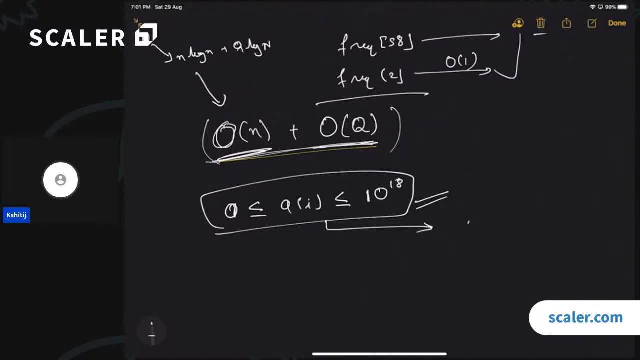 exact same technique, because i cannot have an array. i cannot create a frequency array which has a size 10. raise to power 18. right, because this is going to cost me a lot of memory. right? how much memory is it is it going to cost if this is an array of integers, one integer? 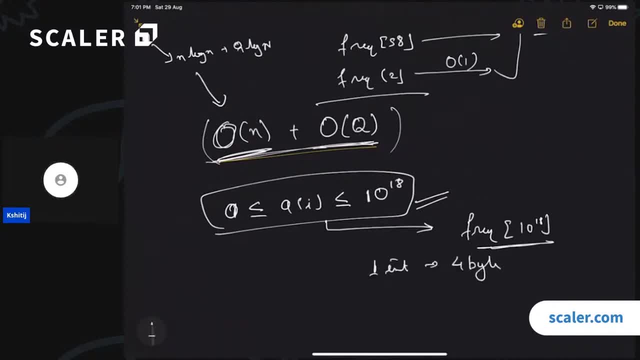 takes. how much memory four bytes, right? so if you want to create an array of size 10, raise to power 18, this is going to cost how much time. how much memory 4 into 10, raise to power 18 bytes. can anyone quickly tell me how much? 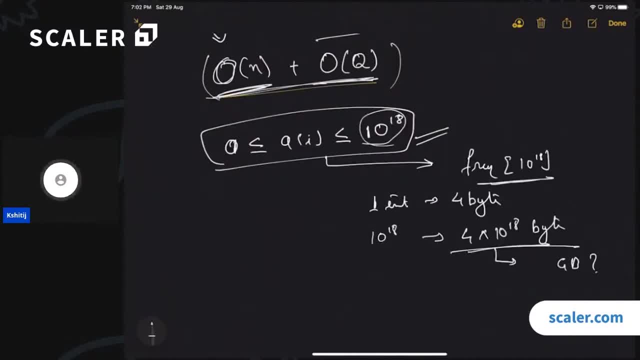 is this in gb's? 4 into 10, raise to power 18 bytes. how much is it in gb's? so if you want to create an array of that size, you need to have this much of memory. you need to have this much of memory in. 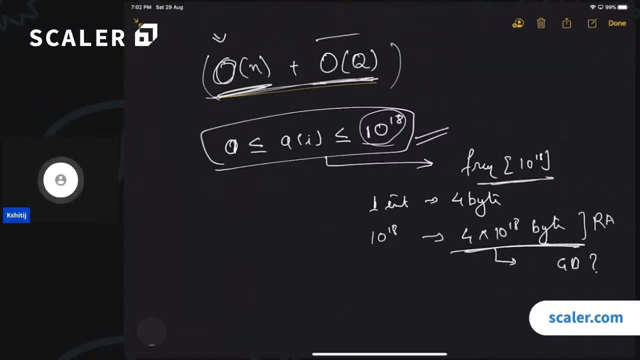 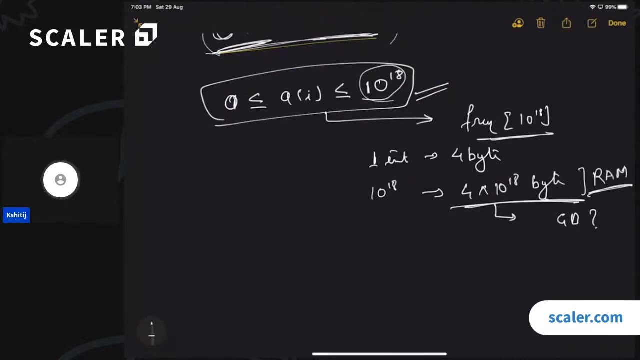 the ram, right? so this much of memory in the ram is definitely not going to be possible for an ordinary computer, right? so what we are going to do is now we'll have to be a little more logical and we'll have to apply a little more mind, right? unlike, uh, mumbai police. so let let us be a little. 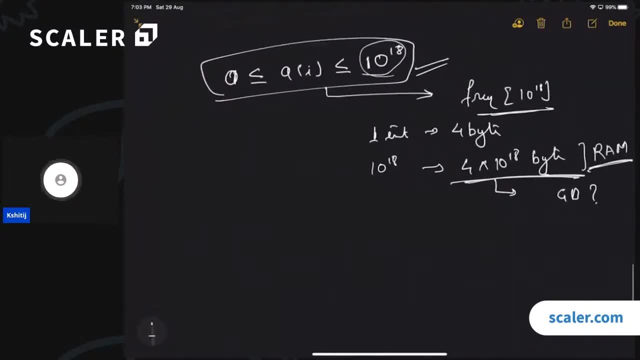 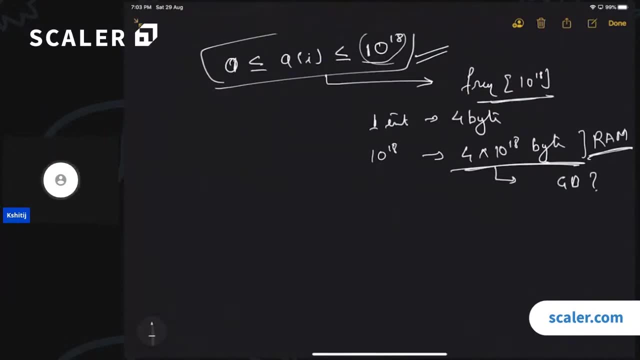 more logical and let us try to see if, if we have an upper limit on the memory, right. if let's say, let us say, let us take a smaller example, and let's say that the numbers are ranging again, ranging from, just to understand, let's take this smaller example, that the numbers are. 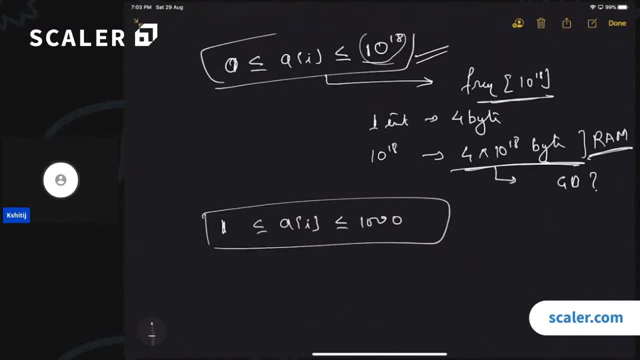 again, ranging from one to thousand, but the largest array that i that i can have can have a size of 100. this is the upper limit on the size of array. okay, similar example. so what we are doing is is numbers are ranging from these grades, ok, and that is why we have to. 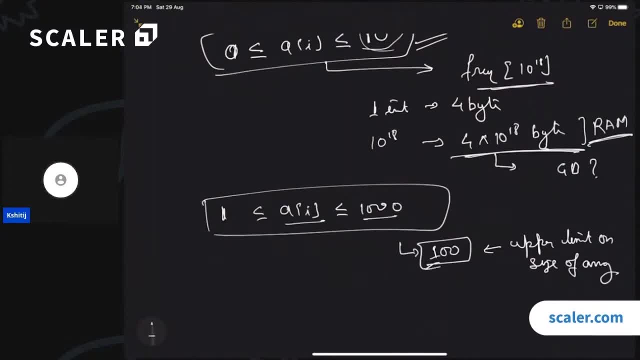 be bit careful- are ranging from a garlic. the numbers are ranging from one to thousand. alright, okay, and now let's see if we can have some significance from what we have. a high limit, 1 to 1000, but the maximum size of the array can only be 100. right now, again, i cannot use. 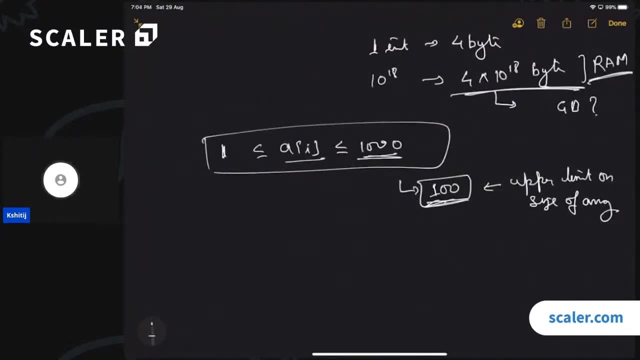 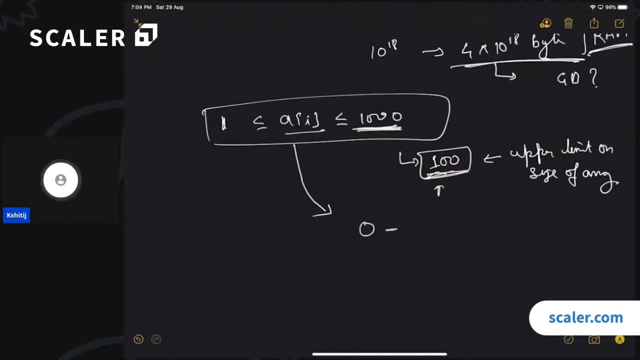 the exact same method. why? because having an array of size 1000 is not possible, right? so if i want to store the numbers as an index in the array, then i can only store till 100. is there a way using which i can map all these numbers from in this range from 0 to 99? because the maximum size 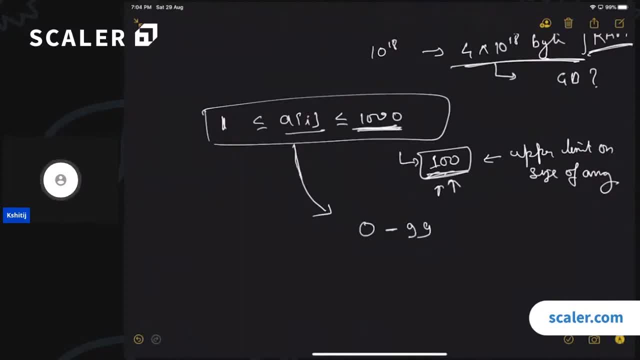 that i can have is 100, so can i map all these numbers in this range? is there a way? have we seen any way? or let's say that all these numbers are ranging from 0 to 1000, right, yes, what can we do? we can simply take modulo, right? is everyone familiar about what is a modulo operator? this? 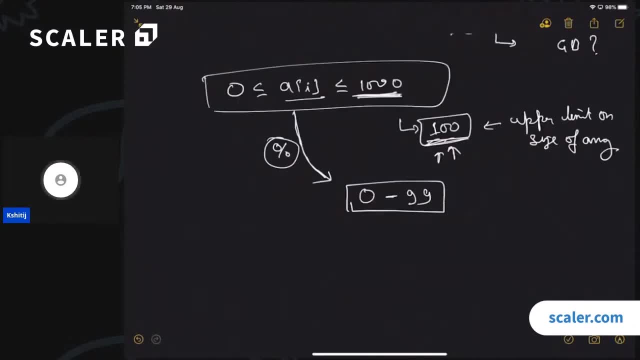 gives you the remainder right. so if, if i take modulo of any number ai with 100, which is the maximum size of the array, then i can have 100 right. so if i take modulo of any number ai with 100, which is the maximum size of the array that i can have, can i say that this number, which 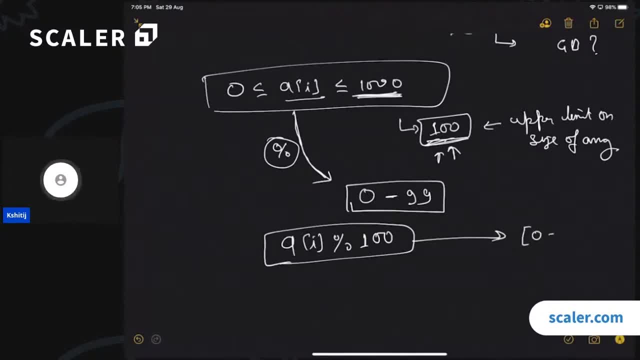 is ai modulo 100, will always lie in the range from 0 to 99. can i say this? yes, correct. so i have got one way to map these numbers which are in this range from 0 to 1000, to a range which is very, very. 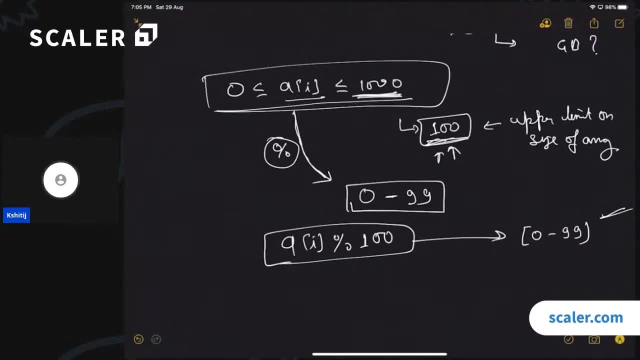 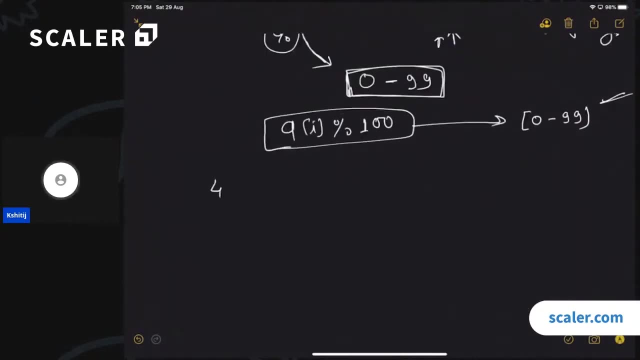 small, right? this? this range has a length, length, uh, thousand thousand one, and now the resulting length is 100, right? so i am mapping these thousand numbers to 100 numbers. okay, if this is the case, how am i going to store the numbers? let's have, uh, an example. let's say i have 492, 5, 8, 23, 15, 142. 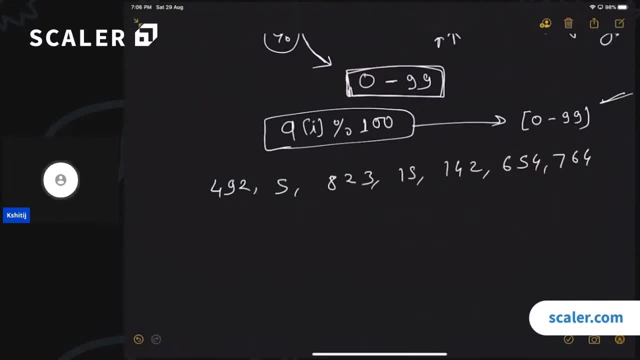 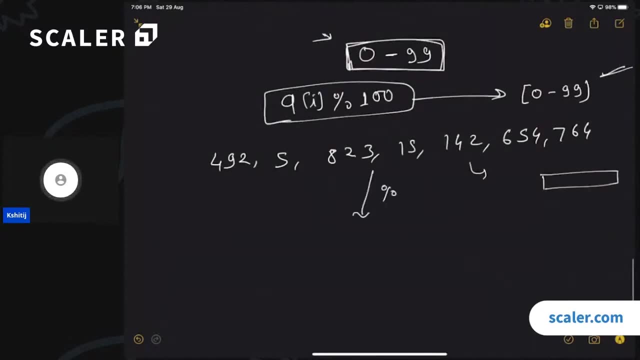 and some random numbers. okay, and now, if i, uh, if i can only afford an array of size 100, right, how can i map these numbers? i will first take the modulo of these numbers with 100 and then, whatever number i get by using, by doing this operation, i will store these numbers in that index, so i get 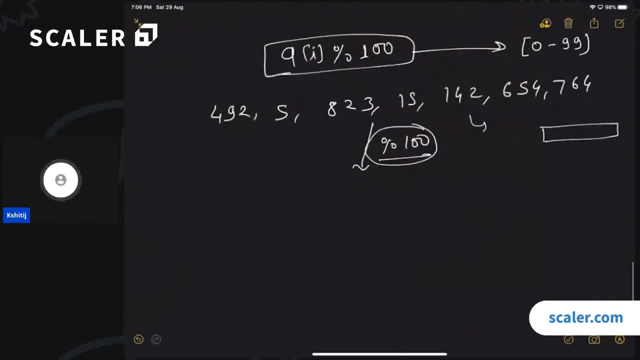 the index by taking modulo of these numbers by 100. so first number will be stored against index 92. this will be stored against index 5. this will be against 23, 15, 42, 54 and 64, right? so if, if i have these as the array, index 54 and so on till till 99. 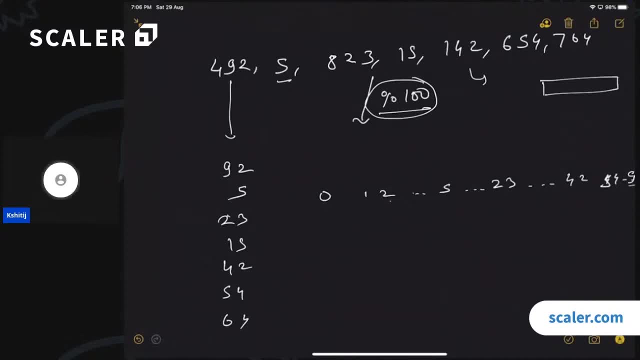 then at 0 is going to be empty, 1 is empty, uh, 2 is empty. at 5, i am going to have 5. at 23, i will be having 8, 23. at 42, i will be having 142, and then 6, 54, 7, 64 and so on. right, so now is this going to? 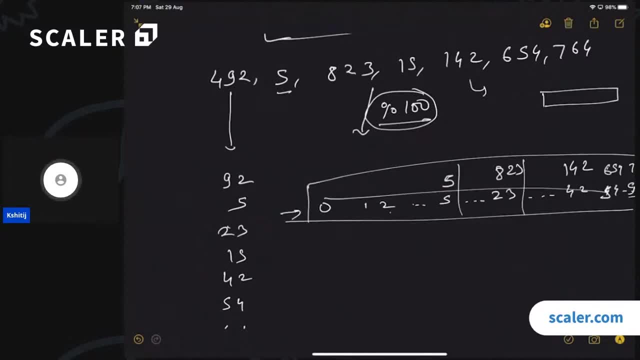 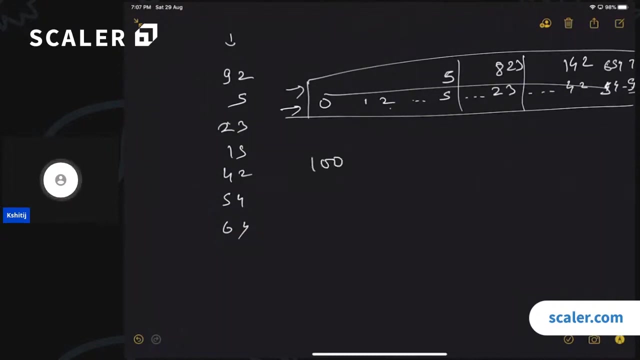 work. is this going to work correctly if these are the indices, and these are, and i keep the values in array element mod 100 index. okay, now of you are saying that this is going to work, but there can be collisions, right, what are collisions? okay, so let us say, let us say that in the array, in the original array, i have these numbers 100. 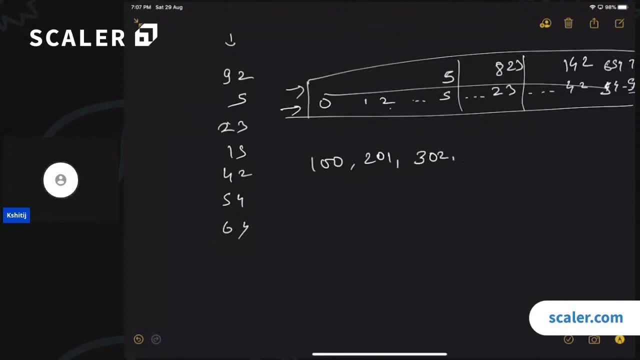 or 201, then i have 302, then maybe 300, 401, 200, right if i have these numbers right. so in which index should a number belong? in index zero? how many numbers am i going to have in index zero? i am going to have 100. 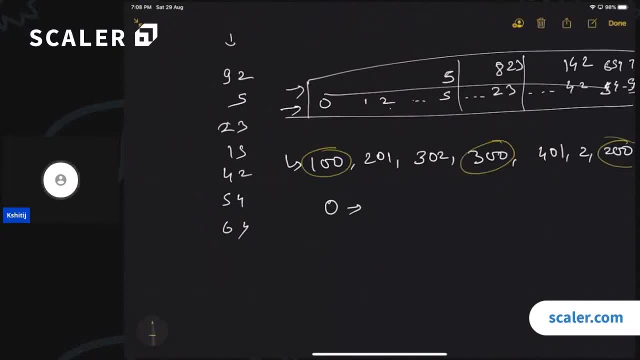 then i am also going to have 300 and i am also going to have 200, right. all these numbers will try to get inserted against a single index right. these are called collisions when there are multiple prospects, candidates for a single index right. so uh, index one will try to accommodate 201, then 401. 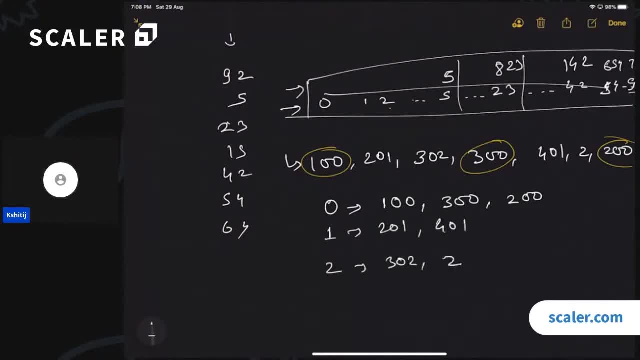 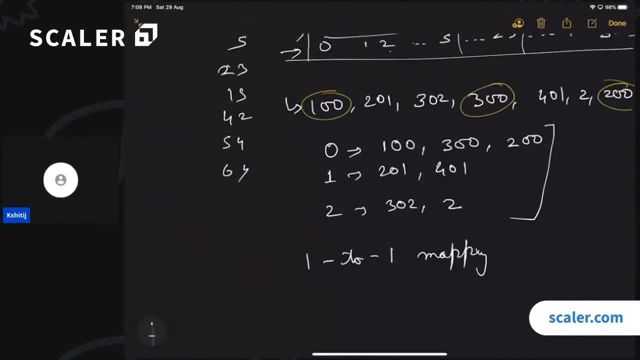 have 302 and then two, also right. so there is no one-to-one mapping, right? a one-to-one mapping does not exist, correct? if a one-to-one mapping does not exist, is this even possible? to use this technique are are we going in the wrong direction? is this a correct way? is this the correct path? 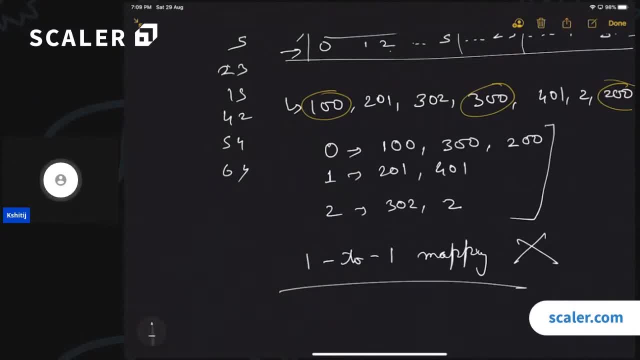 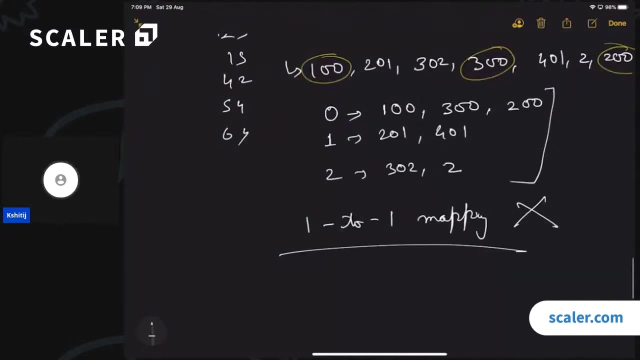 that we are taking, maybe right, we we have also studied a data structure called linked list, right, if? if you know about a linked list, what if we have an array of linked lists? i i have, if i keep an array of the linked list nodes right, can i say that this can work in that case, right? so currently, 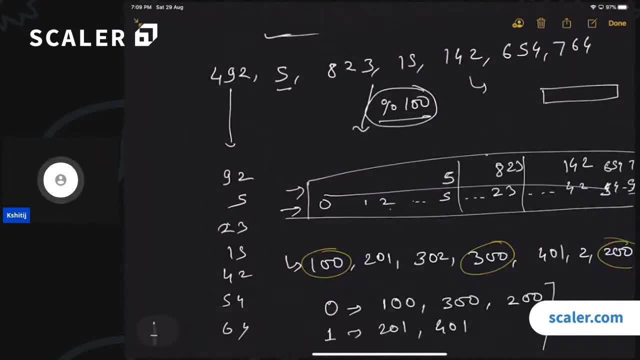 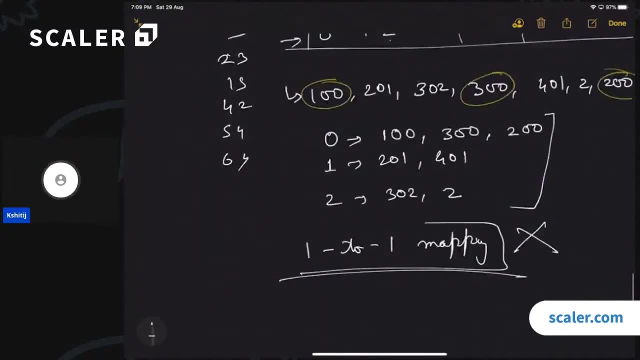 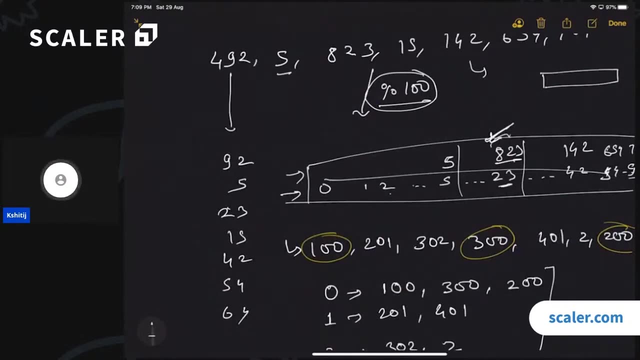 if, if you are only storing a single element- if you are, if you are only trying to store a single element against one index, then, since there is no one is to one mapping, this will definitely fail. we are going to lose some data right, because every time you have a collision, the previous number will be. 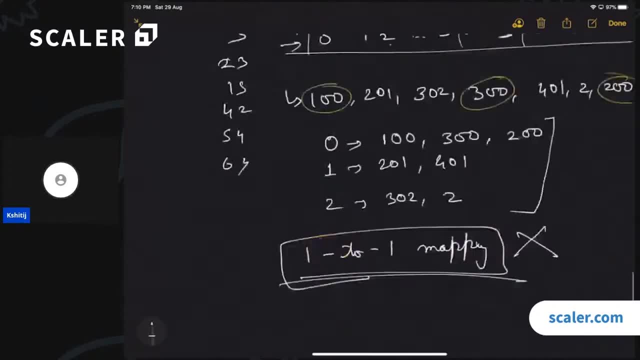 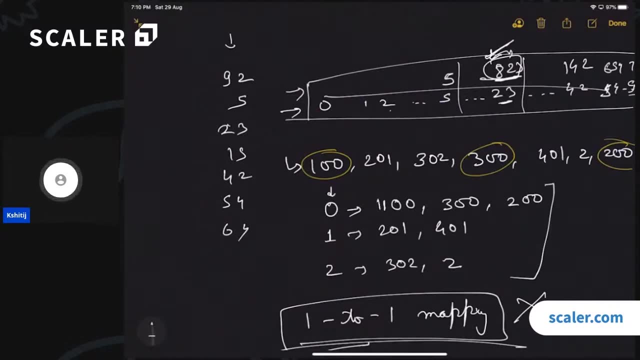 overwritten. but what if i use a linked list? so instead of having, uh, these integers, right if at index 0 i have this complete linked list store. so if i have to create an array of linked lists, what? what do i need? i only need the pointer to the head stored in the in that correct index, right only if, if i have an 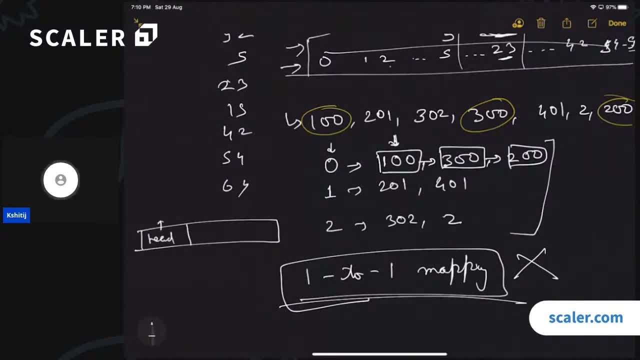 array like this where i have this head pointer, then using this head pointer we can have the complete linked list right. so we don't need to actually store this complete linked list in the array, we only need to store the head pointer right. similarly, at index 1 we can have: 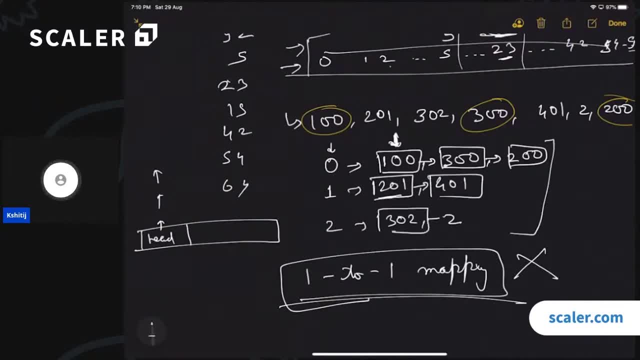 the head pointer of 201 at index 2, we can have the head pointer to 302. does this make sense to everyone? so we can still manage doing hashing in this case, even though the the range which we have to store is very large. the size of the array is very small, but we are making sure using the modulus operation. 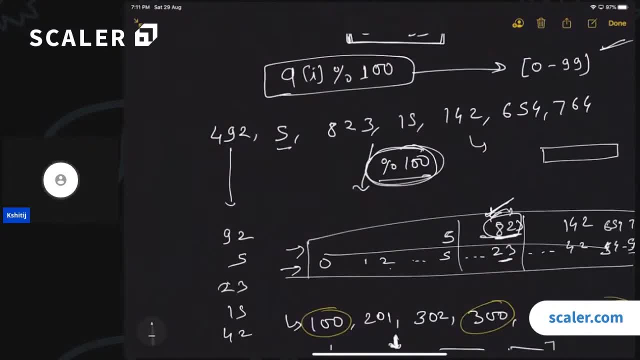 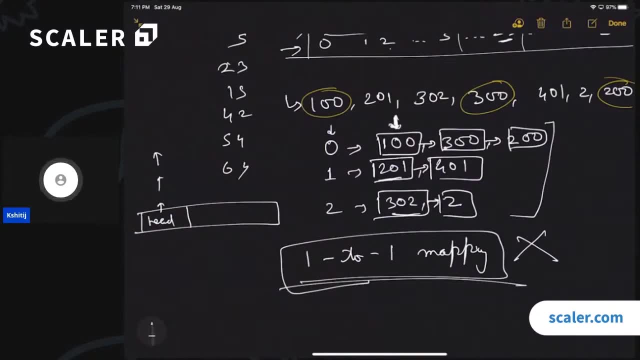 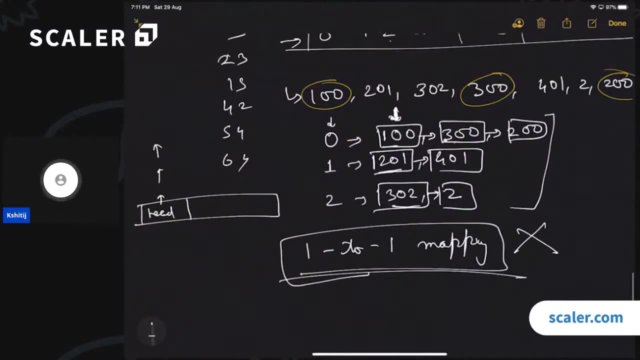 that we are mapping these numbers to the available size and then using a linked list. we can also make sure that we are not losing out any data and we are storing all these numbers using the chaining. okay, now, if, if i am storing the values like this, now, if i have to find what is the 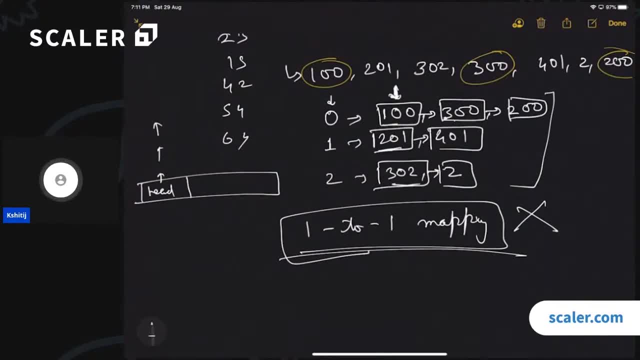 number of frequency or, let us say, if i just want to check whether a number is present or not, right, what is the worst case? time complexity of this case. if i am going by this approach, if i am storing linked list, if i am having an array of linked list nodes. 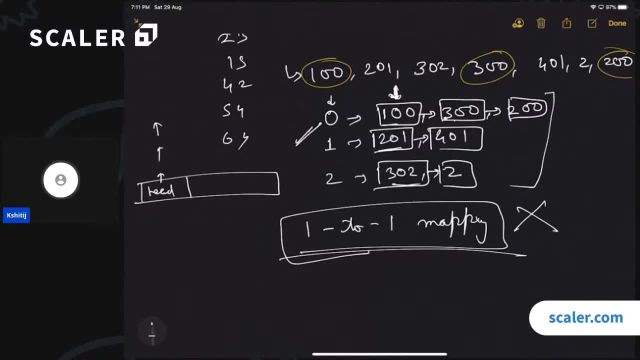 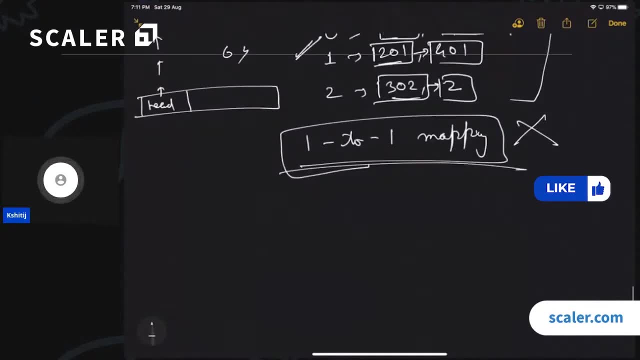 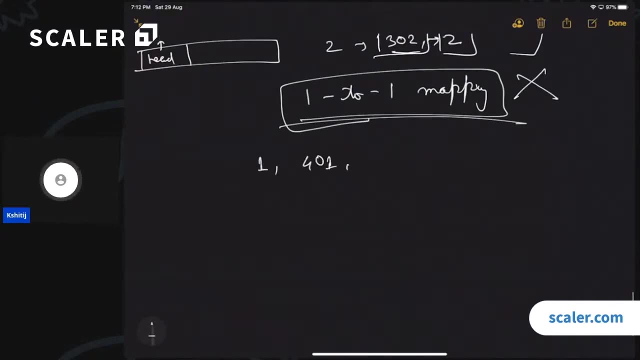 what is the worst case? time complexity of finding whether a number is present in the area or not. so the worst case is going to be if all the numbers are mapping to a single index, right? so if let us say that the numbers are these one, then you have 401, then you have 101, then you have 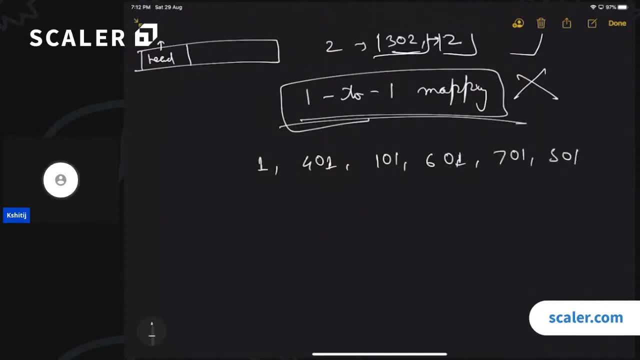 601, right 701 and 501 correct. if i take mod of all these numbers with 100, all of them are going to take the exact same key, so all of them are going to map against one. if i have to search whether a specific number is present in this array or not, i will be traversing. 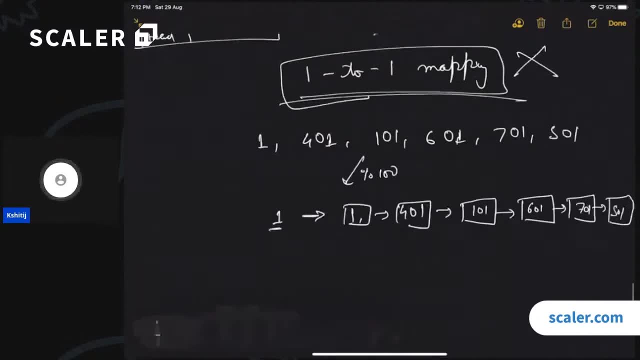 this complete linked list, right? so first let us say i get a query. i get a query of, let's say, 801. i have to check whether this number is present or not. so first of all i will try to see in which index is this number is stored. so i will just do 801 mod 100, which is going to be 1. so i go to. 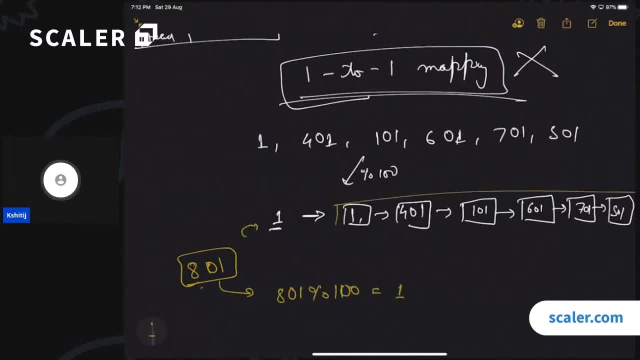 index 1 of my array, and now i have a linked list of size n. i will iterate over this linked list and since this is also not in sorted order right, i will have to check each and every element and i will then figure out whether i have 801 or not, right? so this is going to be a order n time. 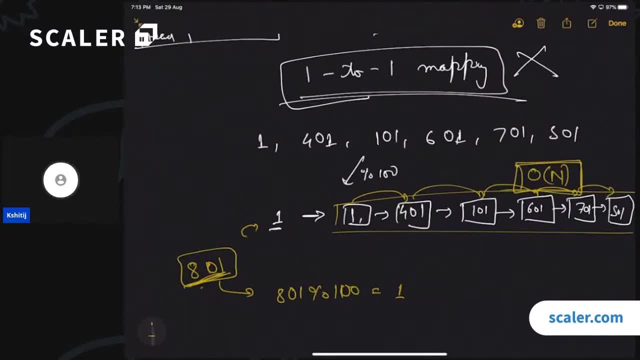 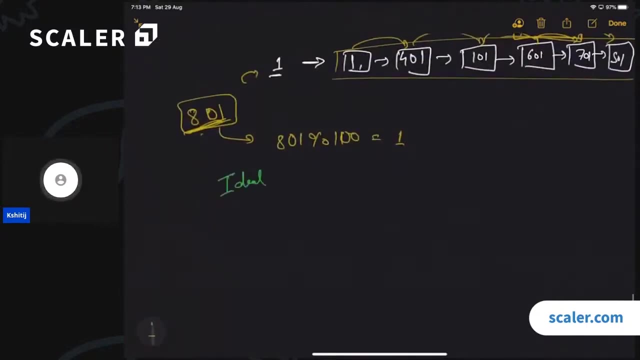 complexity operation. does this make sense to everyone? this is the worst case time. complexity of checking whether the number is present in this list or not. right, okay, so this is the worst case. what could have been an ideal case. when can i say that that this is the best thing, that that i want? what is the ideal case in? 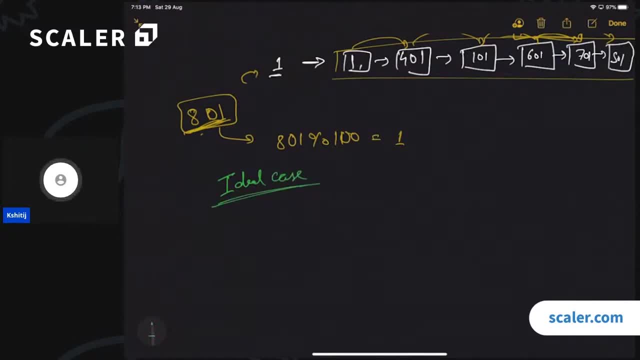 this. in this scenario, the ideal case would be that if all the numbers are mapping to different index, if all the numbers, if i have a data and like, if i have the data in such a way that all the numbers, all the index, right. so if i, let's say, have 401 against one, then i have two, so let's say i have. 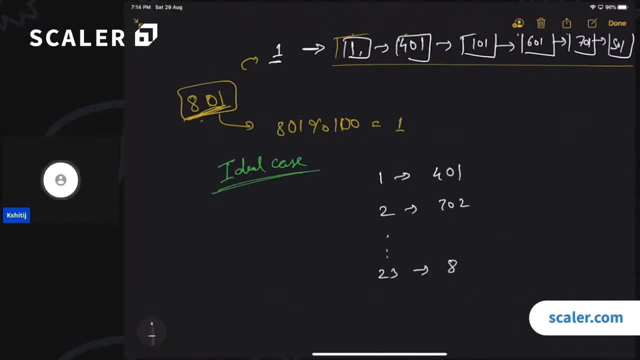 702, and then i have 23, so i have 823 and i have exactly one element for each and every index. this is going to be the ideal case and what is going to be the time. complexity, in this case, of just finding whether a number is present or not, since the list size in each and every case is exactly. 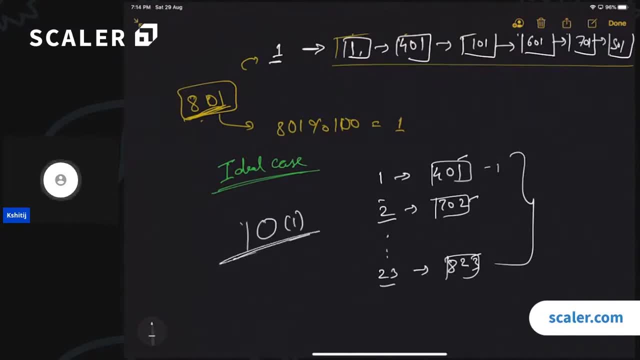 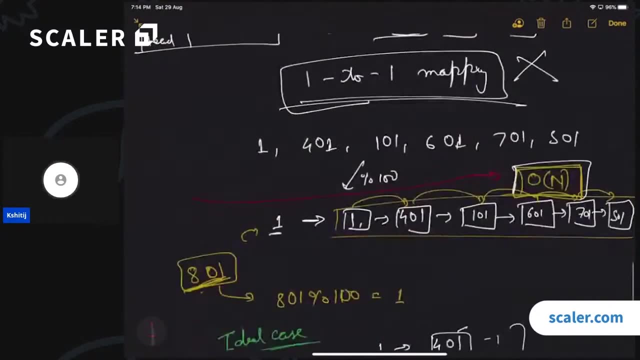 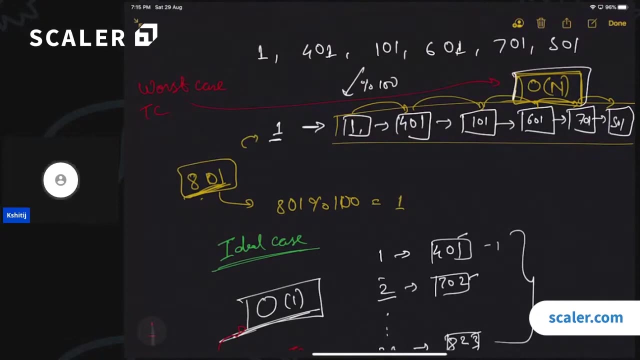 one the time complexity is going to be constant, right? so this is the best case time- complexity- and this is the worst case time- complexity. is everyone clear about these two? okay, great. so the aim is that the mapping function that we are using right. currently, the mapping function is: 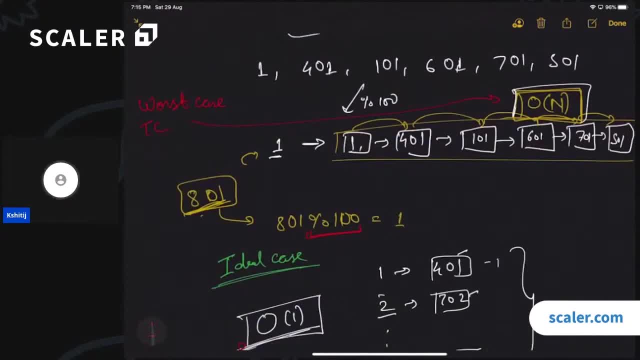 mod by the size of the array, right? so the aim should be that whichever mapping function we are using should try to evenly distribute the load amongst all the possible indices, right? so this, this function, this, the mapping function that we are using, this is called. what is it called? anyone knows what is the. 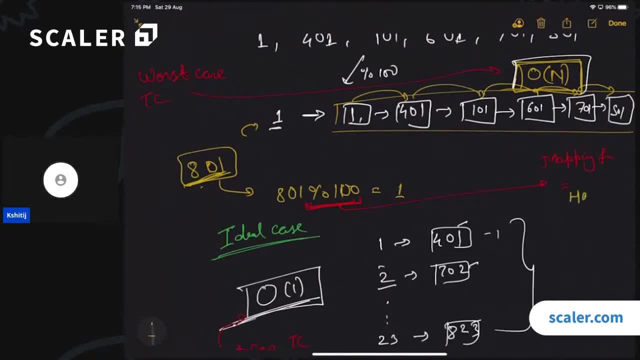 name of this function. this is called the hash function. okay, and hash function is is a very, very big topic in itself. there is a lot of research going on. there has been a lot of research already done on what could be a better hash function or for what case. right, so you can just go and google. 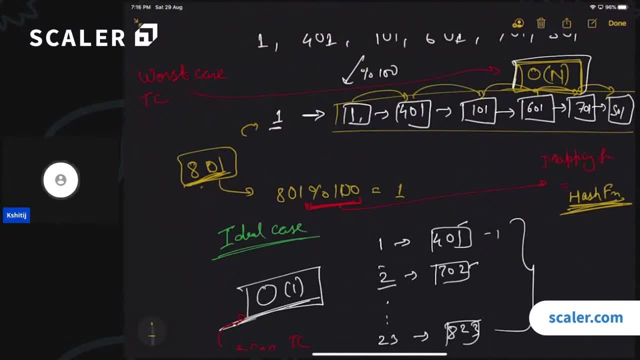 and read about hash functions. there are multiple publications on these. you can read, you can go through some of the publications if you are interested. right, but taking a mod, this is the most simple hash function that you can have, but not the most optimal, and this was just for the example. you have very complex, very optimally written hash. 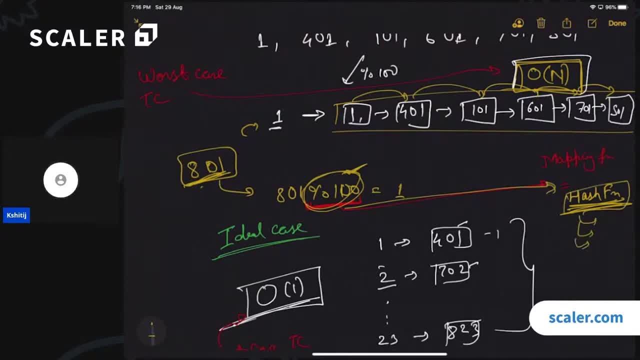 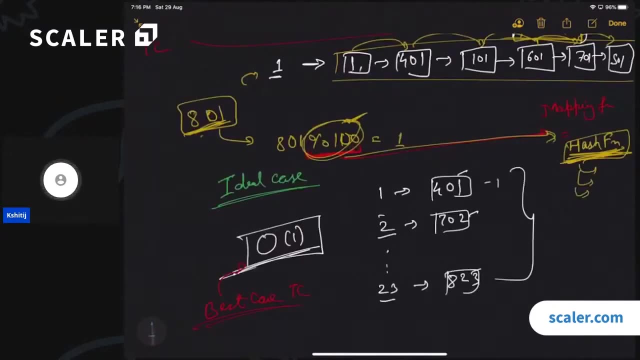 functions which try to distribute the load evenly. okay, so you can just go back and read about what are hash functions and you can also read about some of the common hash functions. okay, cool now if if i write one of the best hash function even which is the best possible hash function currently present in this world. 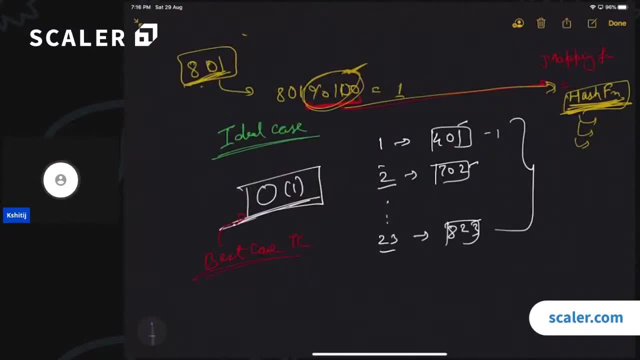 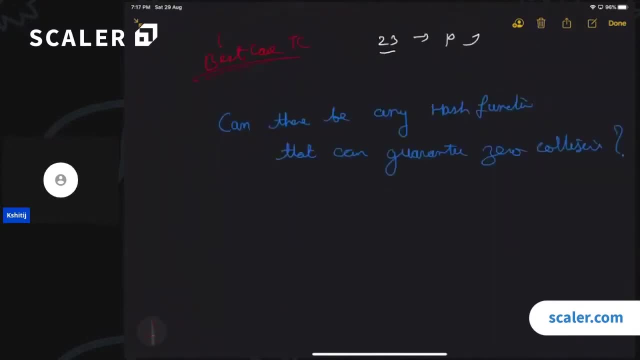 can i say that that hash function will guarantee zero collision? can there be any hash function which can guarantee zero collisions? no, why, why? no? you have got a very big range of numbers, right. you have to map numbers from, let's say, zero to thousand. you have got only hundred slots. 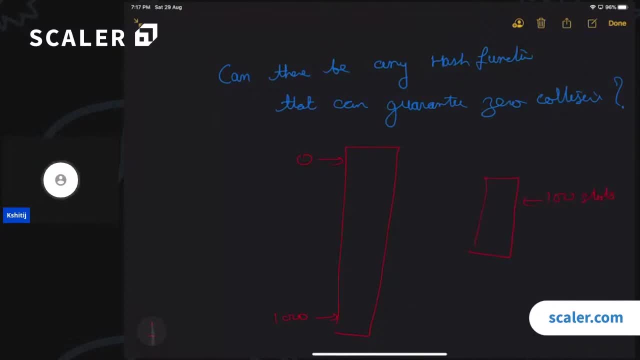 is: are you? are you aware about the pigeonhole principle? you have hundred slots and you have to put thousand things. when you put the first hundred things, and if your hash function is guaranteeing zero collision, hundred slots are filled right now when you pick the 101 index. 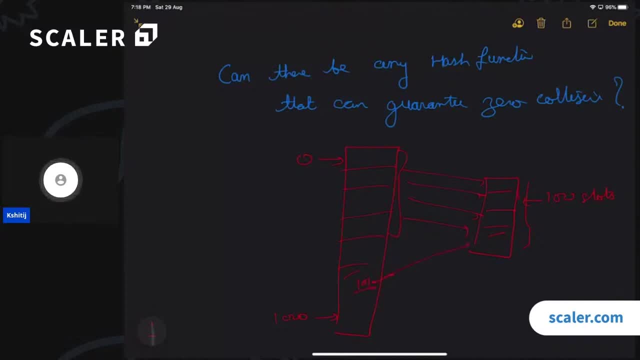 number. this is definitely going to collide with at least one of the pre-existing slots, right? so since you are mapping a lot of the hash functions, you have to put a lot of the hash functions, so it is not possible to just put the whole hash function into a bigger list of numbers to a smaller. 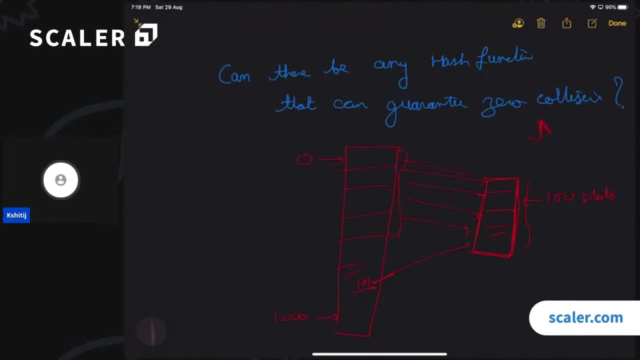 list. you will always have collision, so there cannot be any hash function which can guarantee zero collisions- okay. however, there are hash functions which try to distribute the load evenly. that is possible. there has been a lot of research done on that. you can google and read: okay, cool, so this is. 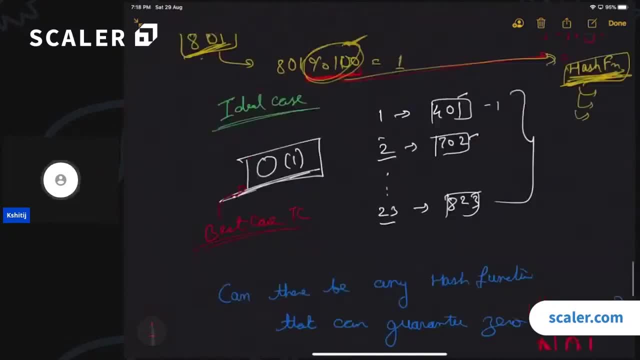 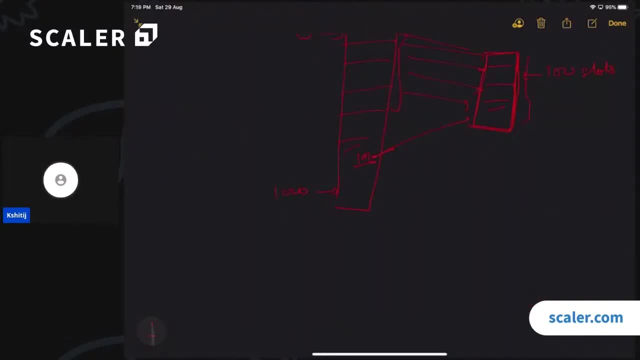 this is, uh, the basics of hashing, right? uh, you can read about hashing and you can read about hash function functions. you can also read about hash tables. hash table is nothing but key and value, right? so you, you must have seen whatever dictionary. if you use python, you must have used hash maps. so hash maps. 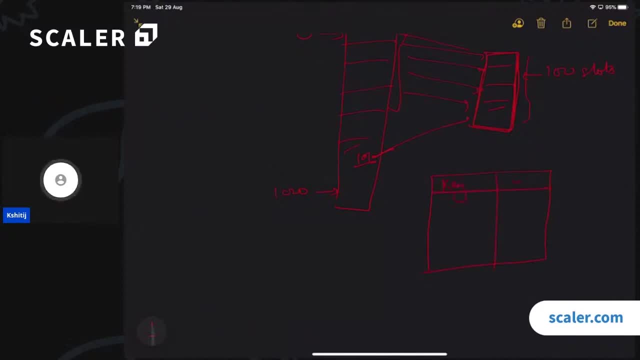 or hash tables. they are nothing but a key value pair. this key is is the result that you get from the hash function. this is a hash code of of any value and in the value you can store it. anything right. so the key, as you all now should understand, these keys in this case are this: are the index. 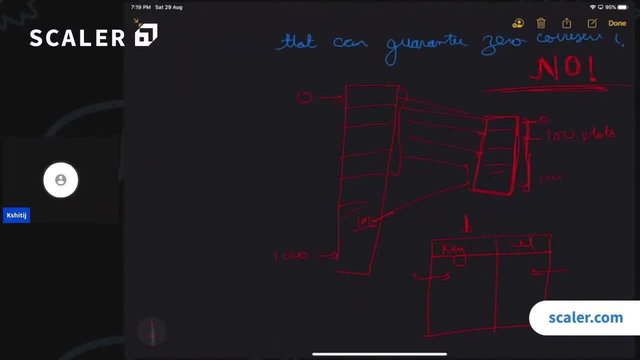 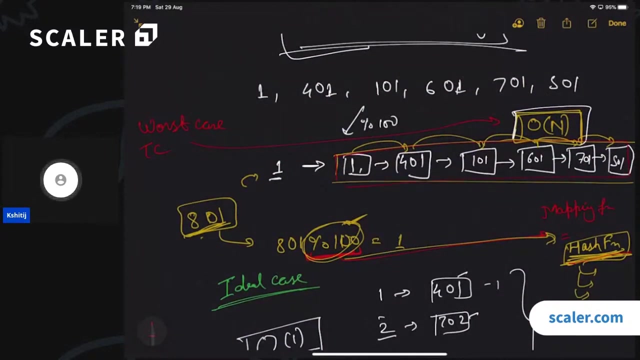 from zero to hundred. right, so keys are always and always going to be unique values. can repeat, you can store the values, uh, in list or maybe in some other data structure, but keys are always going to be unique. okay, now there was a question that if, if you are using a list, is there any specific reason? 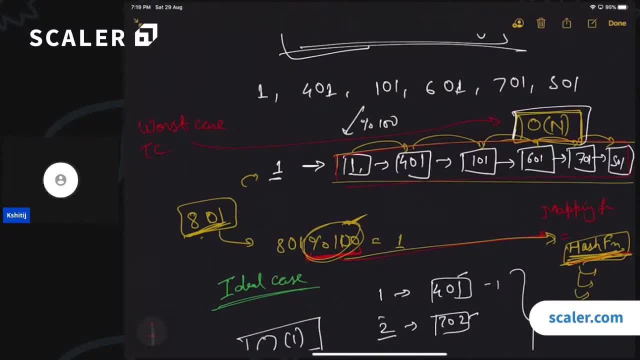 of using a list, or can we have any other data structure here? what do you guys think can you? Can we have any other data structure in place of list? So Surit is asking why we use linked list. Is there any specific criteria? Correct, Komal has got a good solution to that. 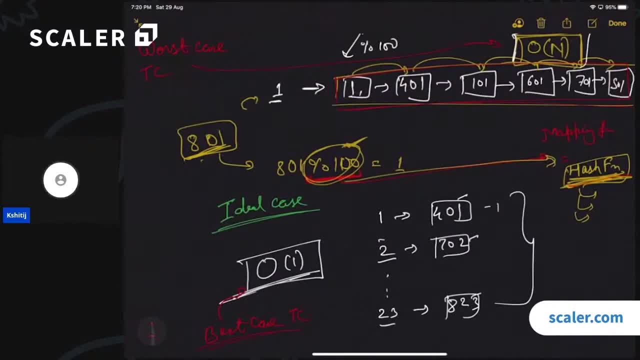 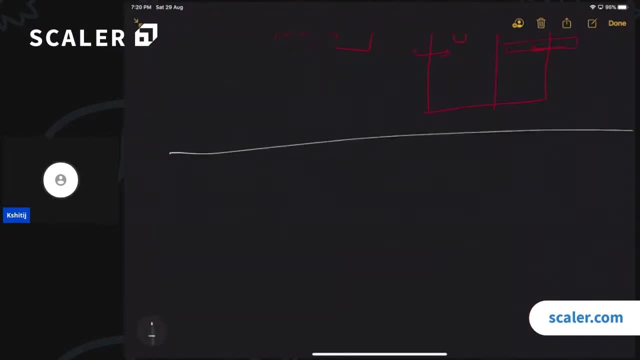 If I'm using a list, what is the worst case time complexity of searching a list in? if you have a list which is not sorted and which is a linear linked list, what is the worst case time complexity of searching in this list? Worst case time complexity of searching in list. 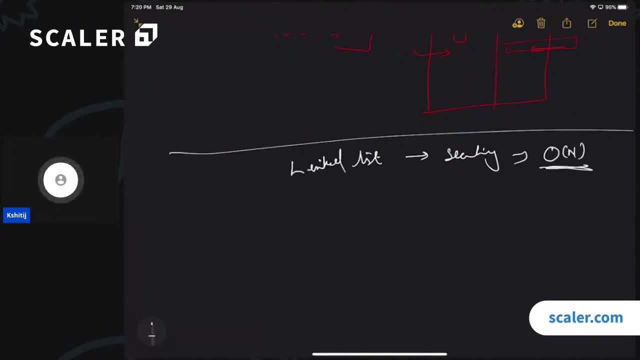 is order n. okay, Now do we know any data structure which provides a better searching time? complexity: Is there any data structure which can store the numbers, maybe in some order, and then can give us a better time? complexity: Do you guys know about binary search trees? 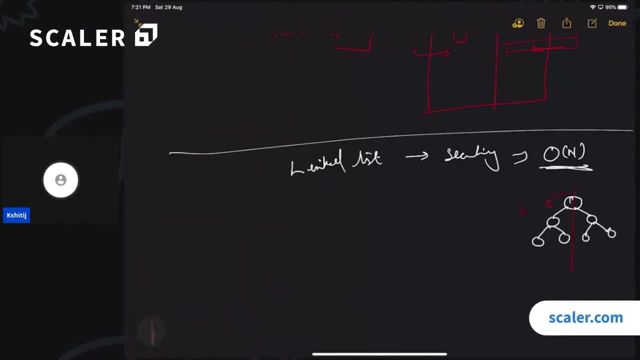 In a binary search tree. all the values on the left sub-tree are going to be less than or equal to the value of the root. All the values of the right sub-tree are going to be greater than the value of the root right. 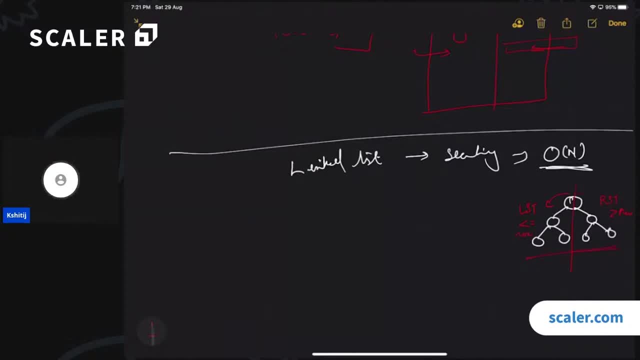 So just by using a technique like binary search, it can always discard. while searching for a number, it can always discard half of the search space, right? So what is going to be the time complexity to search a number? It's going to be log base two n. 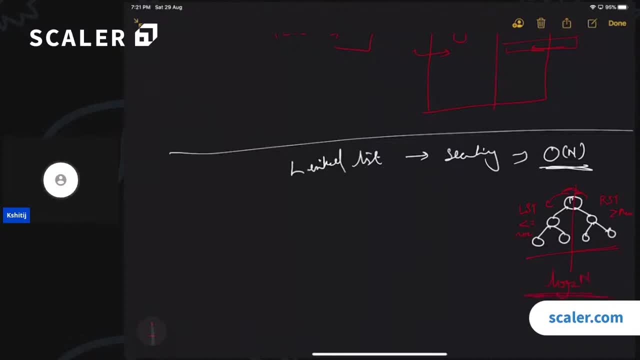 If you are using Java 8, one of you who is using Java 8 must know this- that in Java 8, they optimize this worst case time complexity of retrieving from a hash map using a balanced binary search tree In a normal binary search tree. 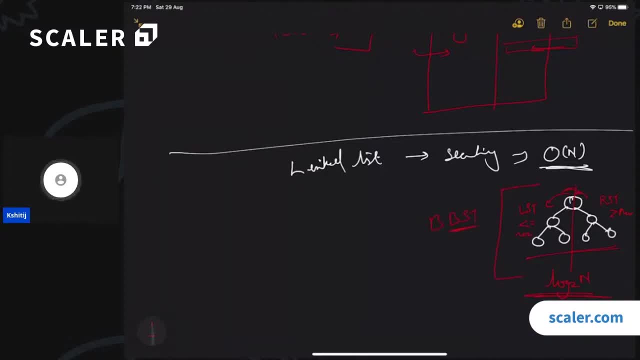 in worst case you can also have in time complexity of n if the tree is skewed, But if the tree is always balanced then you are always going to have a searching time. complexity of log base two, n. So in Java 8, what the hash map does it? 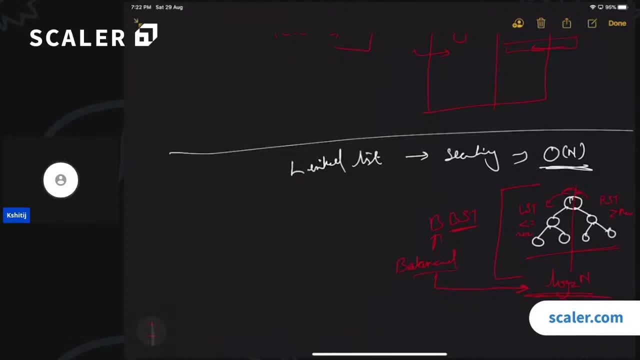 if the size of the list is till a threshold number which I don't remember correctly- I guess it's five or six till- then it maintains a list. If the size exceeds the threshold value, then it converts the list to a balanced binary search tree. 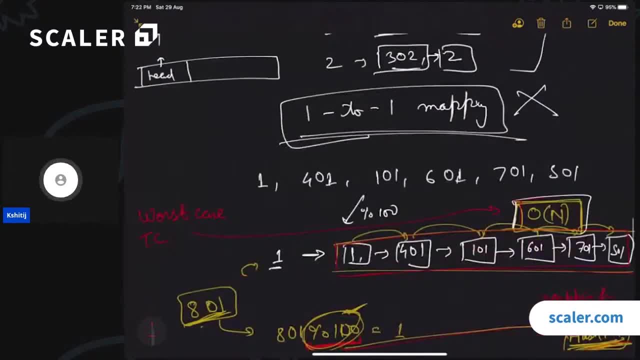 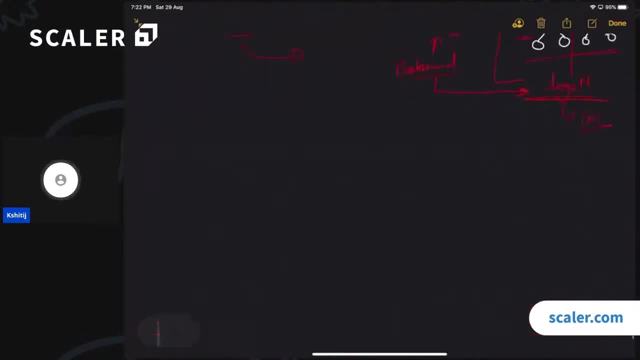 So the worst case time complexity that we have seen to be order n will reduce to order log n- okay, Cool. So, guys, this is, in brief, about hash maps and how they work. okay, Let us quickly solve a problem also okay. 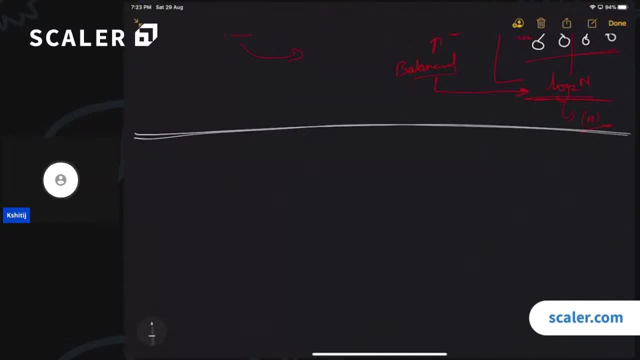 In this type of questions, can we blindly use hash functions? Okay, in any question if it talks about the frequency or counting the numbers, or maybe checking whether a number is present or not, or checking the presence of anything, then you can use hash function. 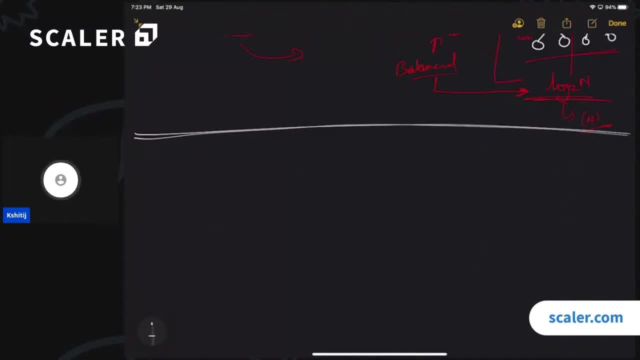 then you can use hashing. okay, Let's quickly solve a problem. You will get a better idea of when to use hashing, okay? So the problem says that you are given an array and you have to check whether there exists a subarray which has sum equals to zero. okay, 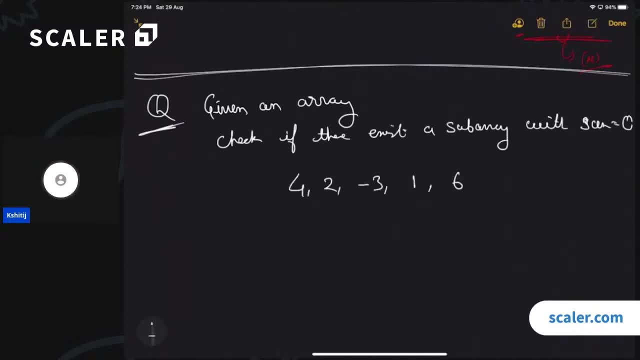 So, for example, if your array is this, in this case does there exist such a subarray? Yes, right, If you see the sum of this subarray, what is the sum of this subarray? It's exactly zero. So, if you see the sum of this subarray, what is the sum of this subarray? 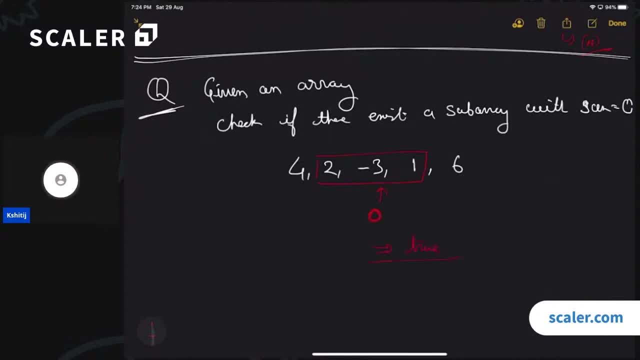 It's exactly zero, So you can return two. If there exists a subarray which has a sum equal to zero, the subarray can start from any index, it can end at any index, it can have any length which is possible. but if there exists any type of subarray, 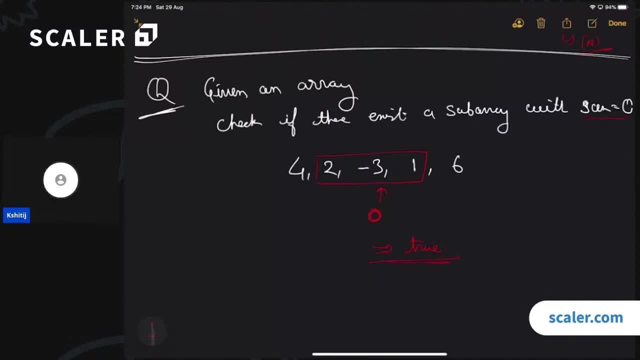 which has sum equals to zero, then you can return two, else false. okay, Modify cadence algorithm. okay, How will you do that? Remember that the subarray can start from any point. This subarray is starting from this point. There might be an input where your subarray 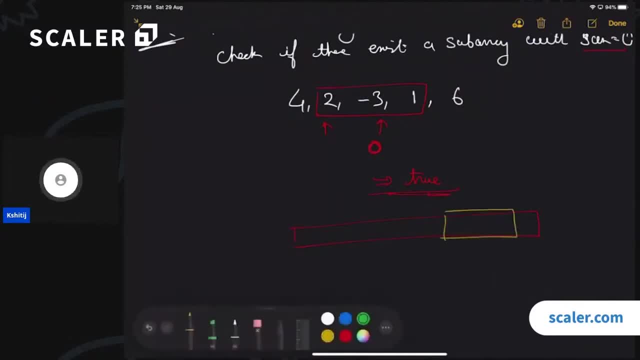 which is causing a zero sum can be present, let's say here, Or the subarray can be present here, or maybe the complete array can also be the subarray. What is a brute force way If you're not getting any solution? 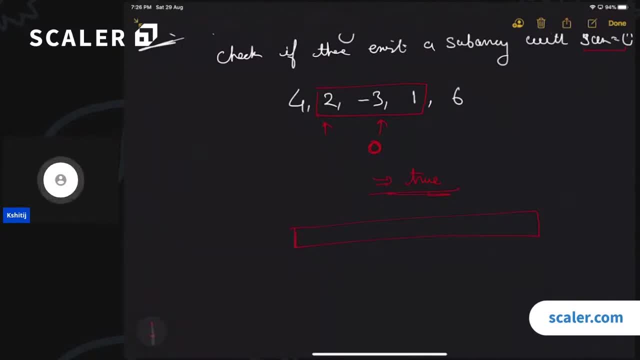 can you quickly write down what is the brute force way? The brute force way is going to be that that you actually try to calculate the sum of each and every possible sub array. right, so you? you first check all the sub arrays of size one, then you can check all the sub arrays of size two, then you can check. 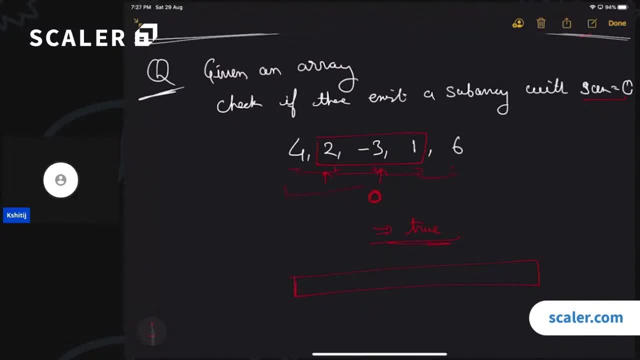 all the sub arrays of size three and so on. right, how many sub arrays are possible? and square sub arrays are possible- to calculate the sum. what is going to be the time complexity for every separate, you will also run another loop to calculate the sum. so it's going to be an. 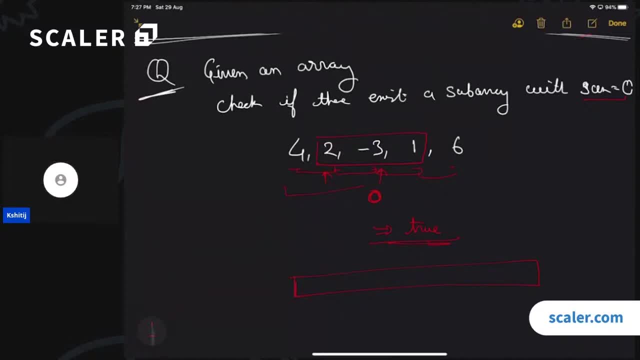 n cube solution, right, which is highly unoptimized. how can we come up with a optimized approach? and we have also studied hashing. hashing doesn't seem to contribute in this question, right? okay, let us let us assume that there exists a sub array. okay, there exists a sub array. 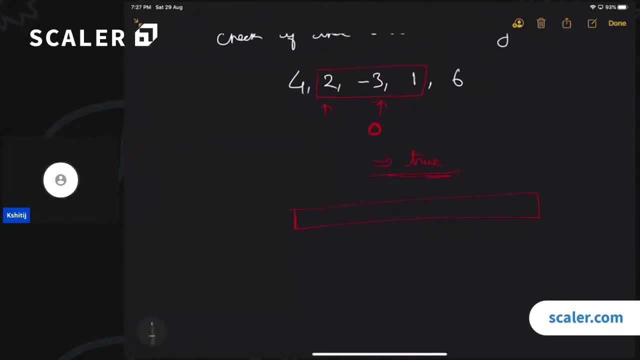 which has got sum equals to zero. okay, so let us say this is the initial area that we have and there is a sub array- let's say this part- which has a sum equals to zero. how do we define a sub array? we always define a sub array using a range of 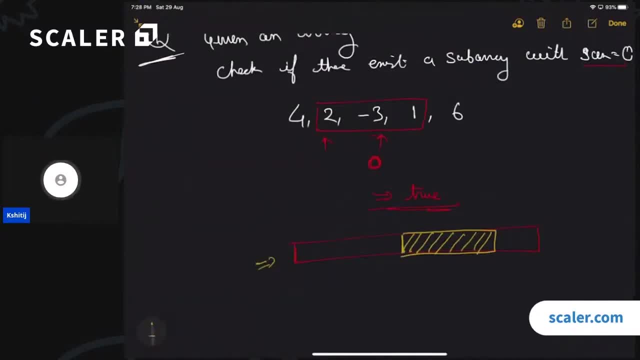 indices. right, because, as i said, this array can start at any point, it can end at any point. right? let us say it starts at a point l and ends at an index r, and i am saying that we are just assuming that the sum of this sub array, starting from l to r, is 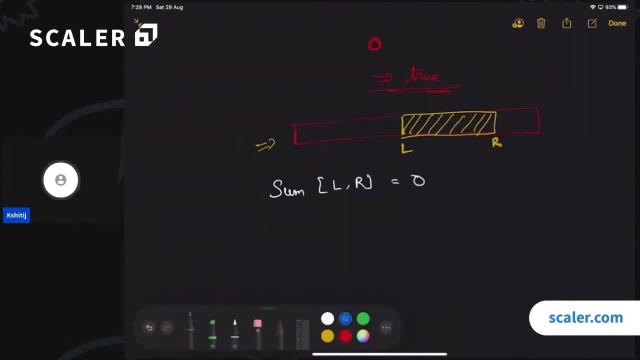 zero. okay, now, if this sub array has got sum equals to zero, right, if, if i also have the sum of all the sub arrays starting from zero stored with me, okay, what? what can we say about this part, this part which is in the blue dotted line? what is going to be the sum of this part, the sum of this part? 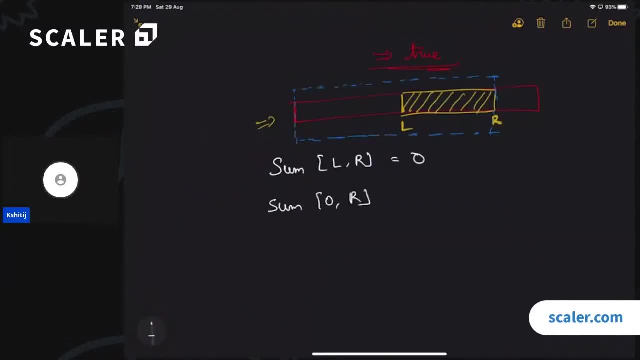 is nothing but sum from zero to r, right, and this sum from zero to r can be broken down as sum from the range 0 to l minus 1 right, plus sum of the range from l to r. does this make sense to everyone, right? so sum of any sub array can actually be written in terms of this prefix sum, right, i can write. 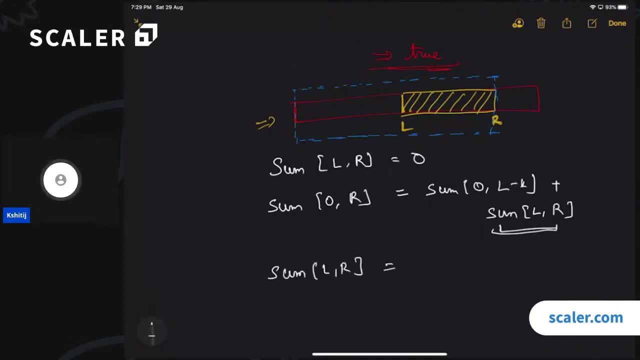 sum from l to r is equal to sum from 0 to r minus sum from 0 to l minus 1 index. i can write the sum of any sub array which starts at index l ends at index r in the form of the sum of sub array starting from 0, which is nothing but the prefix sum. 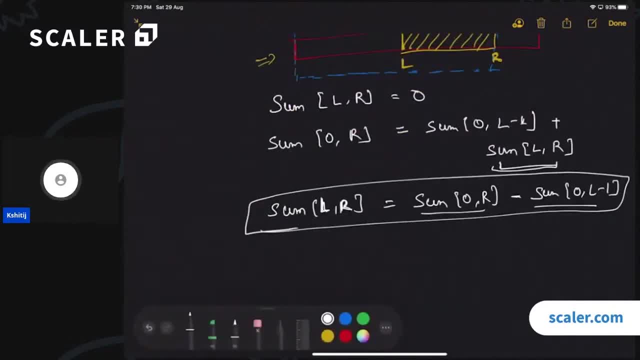 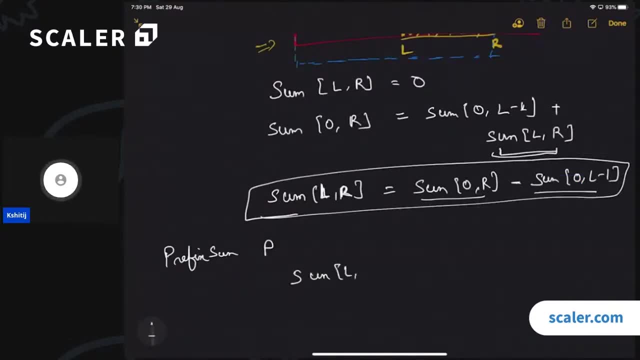 everyone here understands what is a prefix sum, right. so if, if i have a prefix summary, then i can say that a sum of the sub array starting from and ending at r is nothing but p of r minus p of l minus 1, does this make sense to everyone? prefix sum is nothing but prefix sum. 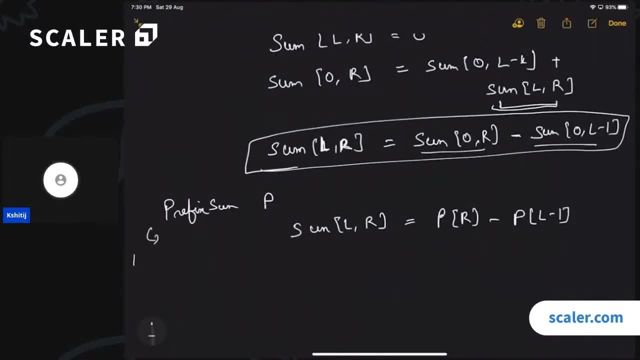 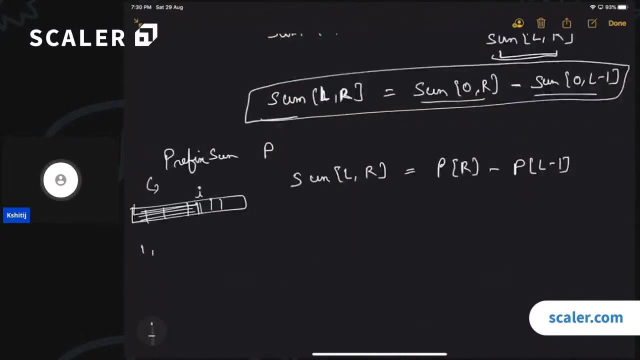 is the sum of all the indices till this, till that index. so if i have an array, right prefix sum at at any index, i is nothing but it is the sum of all the elements, including the i and all the elements before the i. okay, so if let's say i have an array one, two, 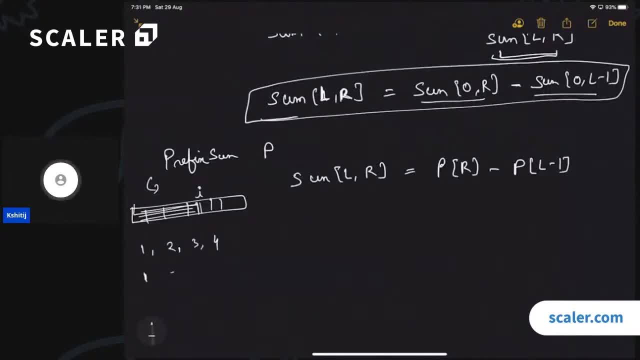 three, four. the prefix sum array would be one, and then this will store the sum of these two is three, then this will store the sum of all of them, which is six, and then this will store the sum of all of them, which is ten. so this is the prefix sum array for this array, if i have all. 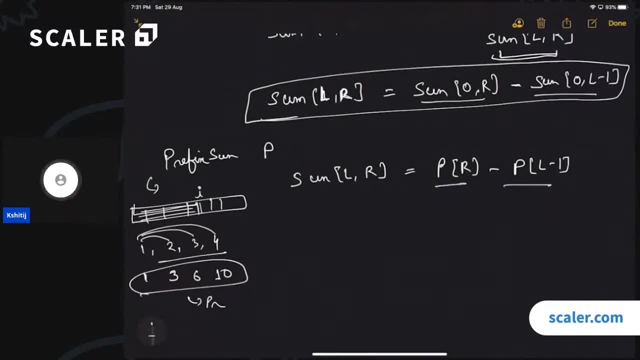 these numbers stored with me already in this array prefix. now i can represent the sum of any subarray in the form of prefix: sums, right, and if i'm saying that this sum is equal to zero? if this sum is equal to zero, can i make any comment about these two values? 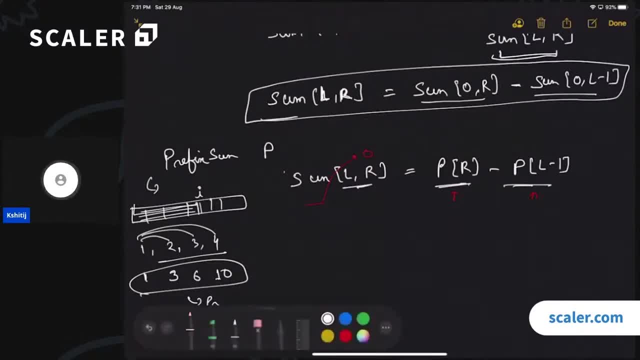 if this sum is equal to zero, this means that prefix sum of r should definitely be equal to prefix sum of l, minus one right. let us visualize this in this diagram. and then, if i have all these numbers stored with me already in the form of prefix sum array, 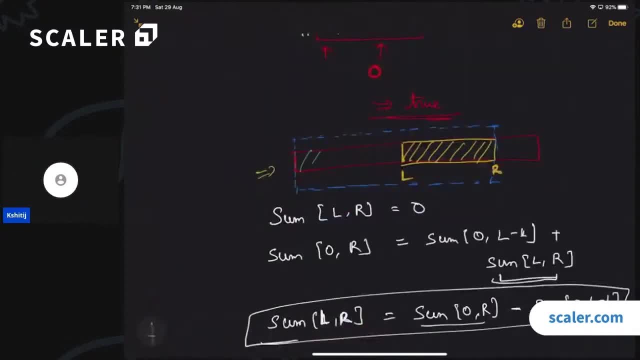 will be more clear. so I have these two parts right now. I am saying that this, this represent. this blue box represent the prefix sum of R. this is the sum of all these elements from 0 to R. okay, this we this yellow box. this represents the sum of all the numbers in the range L to R. correct? and what about this green? 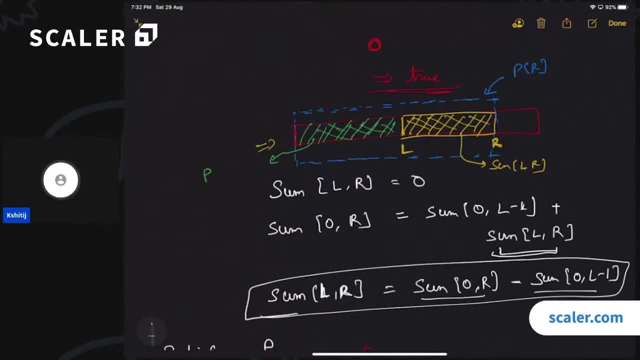 box. this green shaded box represent the prefix sum of the index L minus 1, the sum of all these numbers. can I say that if, if this is going to be 0, right, if I'm adding the sum of all the index from left to right, and and if this part is: 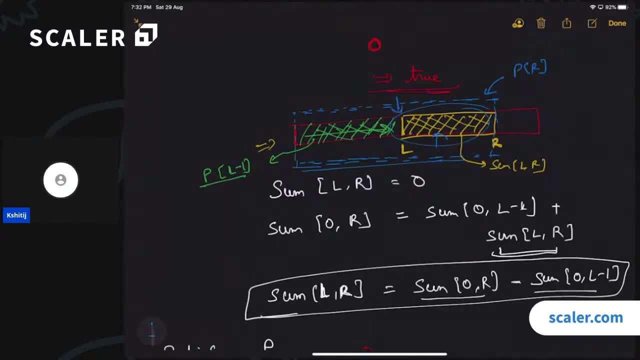 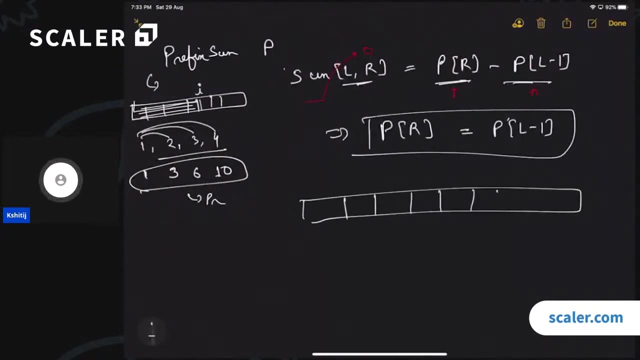 equal to 0, then whatever sum I get at this point, the exact same sum will also be present after this, because the contribution of this is zero. does this work or not make sense to everyone, right? so, if, if i have an array right and if i'm just calculating the sum, 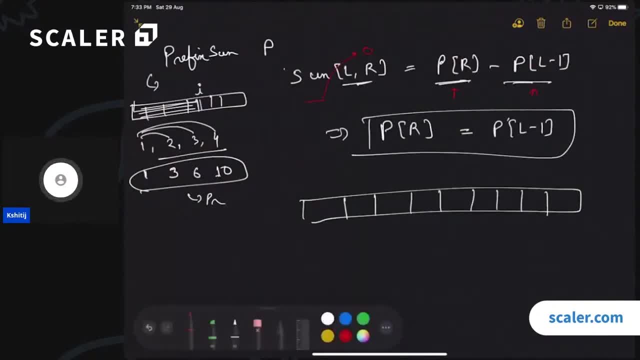 of all the array elements till that index, and then there is a part which is contributing exactly zero amount, right? so this will give some some sum, right? let's say s, then this gives s dash, and then, if i add this as well, this gives s double dash, this gives s triple dash, and then this gives something. 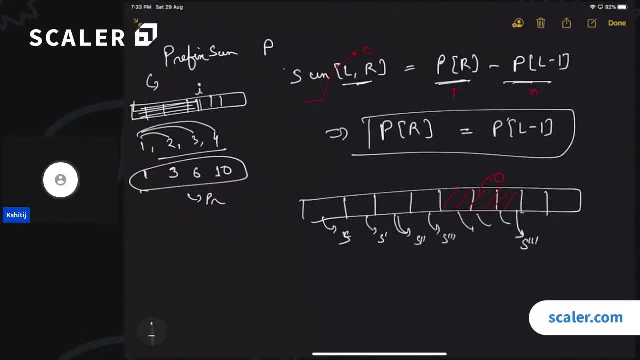 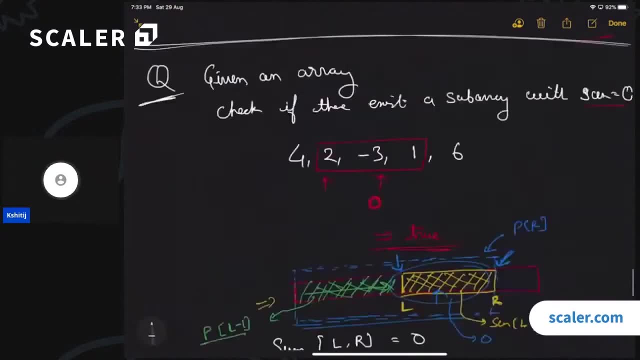 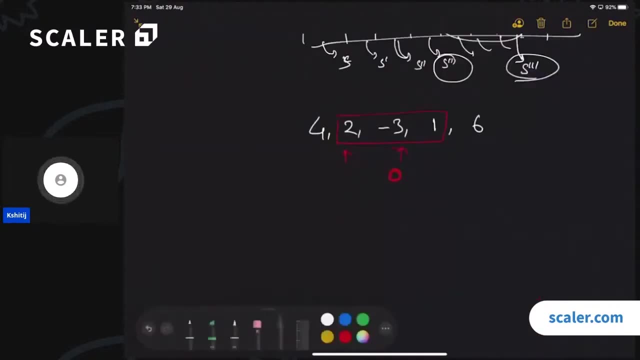 something, something. after i am here i will again get s triple dash, because the overall sum of this part is zero. does this make sense to everyone? let us take the example as well, and then this will be crystal clear. so i will just copy this thing. so if, if i just calculate the prefix sum of 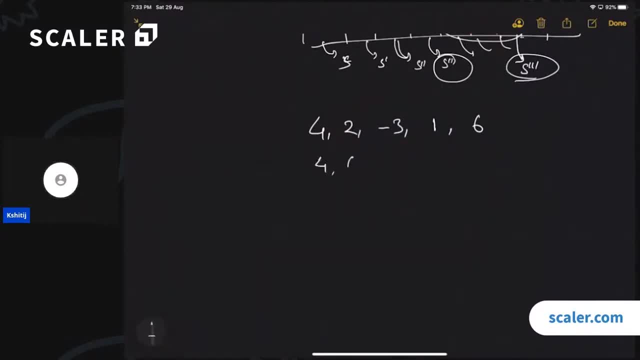 this array- i will be getting four right, six, six minus three again is three, then four and then ten. okay, now what i was explaining is, since the sum of this part is exactly zero, this part, the contribution of this part, in the sum of all these numbers is going to remain zero, right? that is why, whatever, 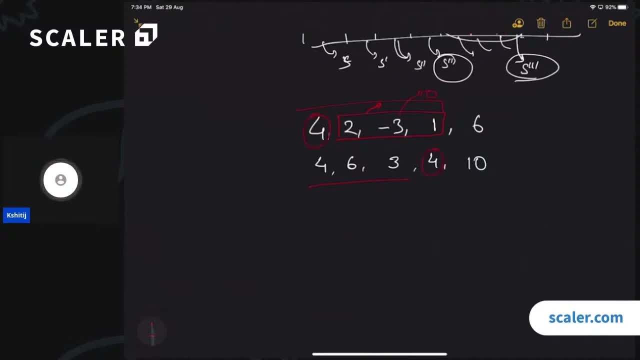 number i am getting here will also be repeated here, right? so whatever sum i am getting at this point, which is this point, is l minus one, right, because i am assuming that this summary starts from l. so the previous is l minus one and this is the r. these two have to be equal. if these two are equal, this means that this: 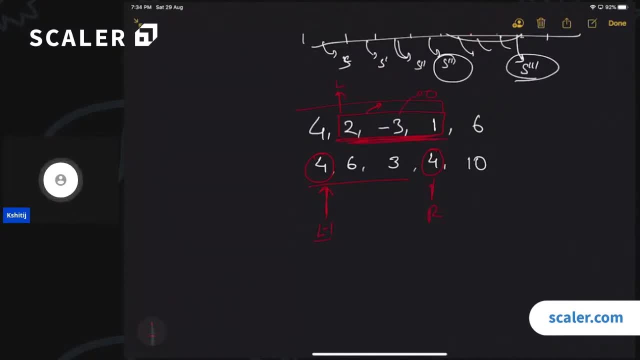 summary. the contribution of this summary was exactly zero. all the values cancelled out each other and we are remaining with whatever we had before starting this summary right? so how can we now solve this problem? if we calculate the prefix sum of the array and then if we, if we observe that 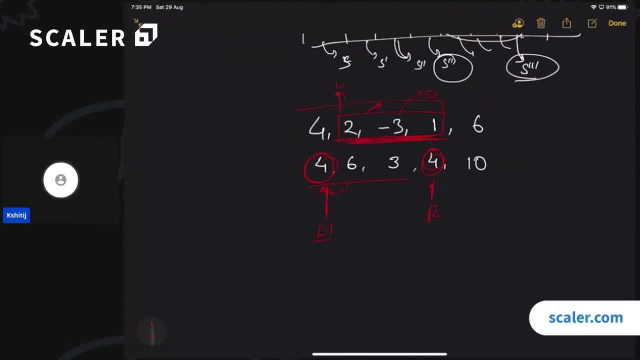 there is a number repeating in the prefix sum. can i say that the contribution of all the elements between these two numbers is going to be zero, which means that this summary is adding to zero. okay, is the idea clear to everyone, guys? is the idea clear, right, let's? let's take another example. let's say i have four, two zero, one, six. okay, now, if i take 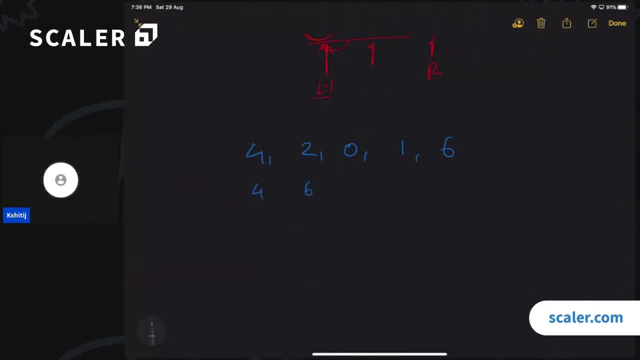 the prefix sums. i will be getting four, six, then again six, and then seven and twelve. so again i can see that a number is repeating in the prefix sum, which means that whatever comes in between these two, this is if i said that first number should be l minus one. this- 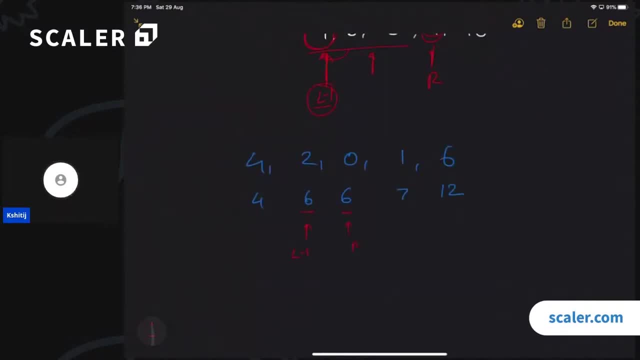 is l minus one, right, and this number is r. so whatever is from l to r is going to give me a sum equal to zero. l to r here has exactly one element, which is zero. now some one of you asked what if a same number is repeating twice? right that. 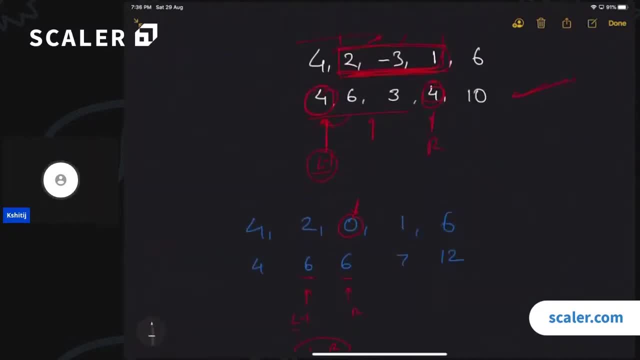 can also be possible. you will have to understand what is the physical significance of this thing, right? so even in this case, if i just modify this array here, i got four, then i have zero, then let's say again zero, then i get uh two and then minus two, and then something. right now, what will be the 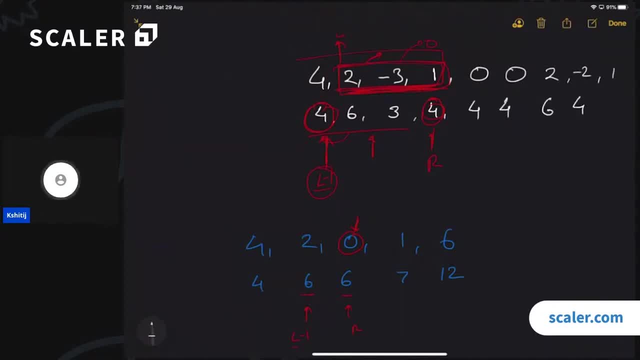 prefix sum: here again four, four, six, again four and then five, right. so this means that all these numbers which are repeating, they all are forming a subarray which is going to give a zero sum. if these two are repeating, this means that we have a sum zero here. if these two are repeating, this means we have a sum zero here. from this: 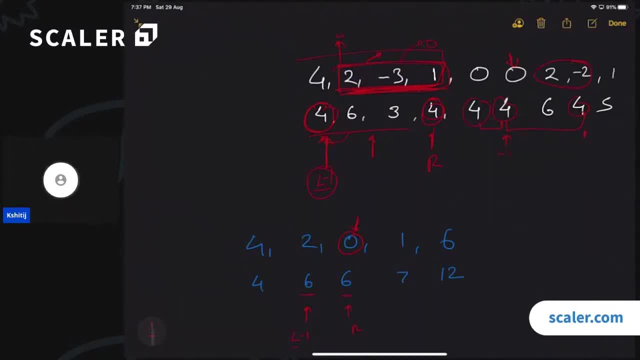 plus one to this right, because this has to be the l minus one index. so even if you have multiple repetitions, that points to only one thing: that the subarray between them is giving a zero sum. okay, now how do we solve this problem? so one thing should be clear to everyone: that 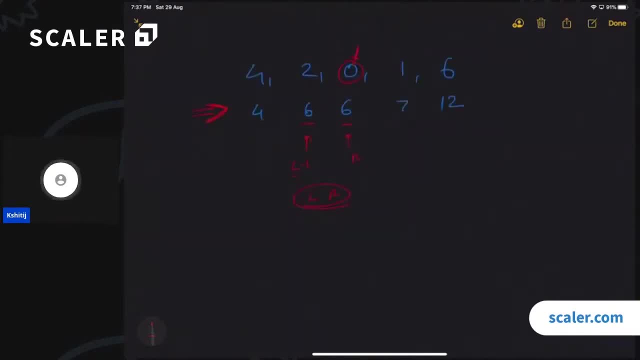 first step is that you create the prefix summary. how can we create the prefix summary? this is very easy task. you can have p0 equals to a of zero, because the first number is going to be the exactly the same, and then, for building the rest of the error, you can just keep calculating you. 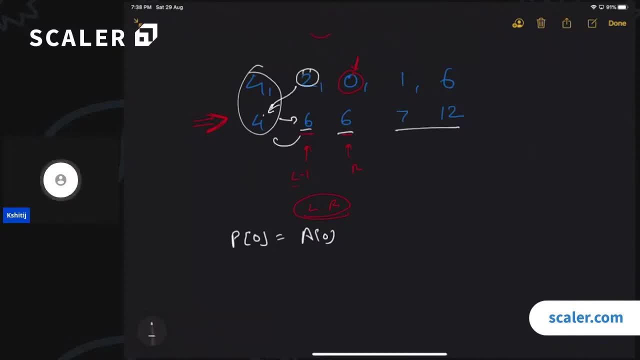 can just keep adding the current value to the previous prefix sum. right prefix sum of i is the previous prefix sum, whatever is the sum tilling. the prefix sum of z is a subarray. and this is now plus whatever is the sum of the current element. so now we can run a loop from: i equals. 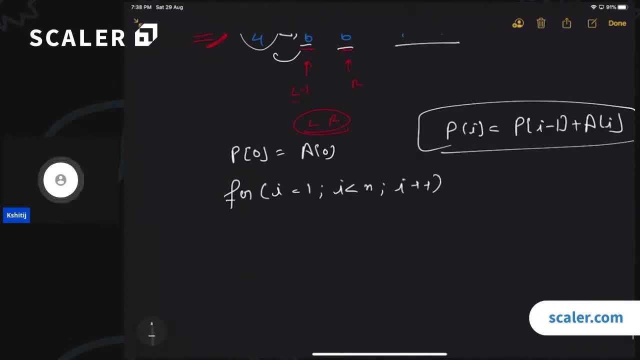 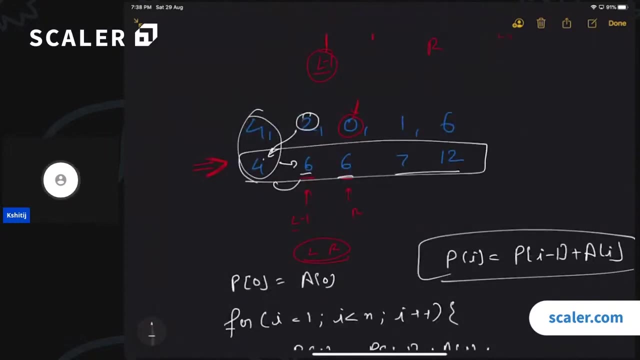 to 1 i less than n, i plus plus, and then you can say: p of i is equals to p of i minus 1 plus a of i. this gives you your complete prefix sum. now, in this prefix sum you just have to check whether there are two numbers which are repeating or not. is there any data structure? let me know which can. 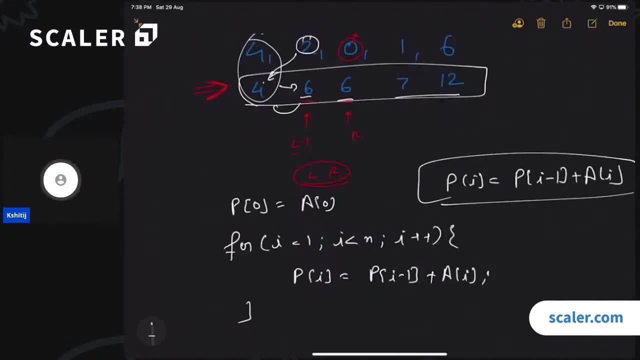 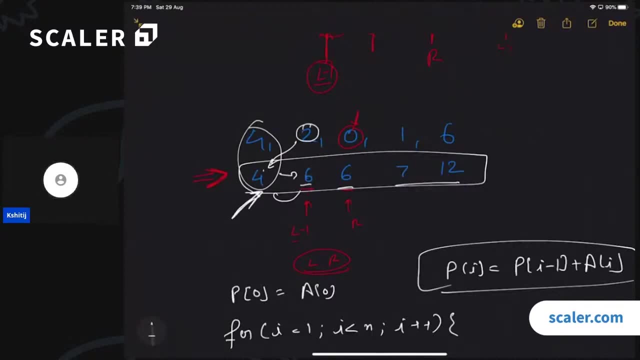 solve this problem very optimally. you just have to check whether there are two numbers which are repeating or not. how do you check for a repetition of a number? you can have a hash map, right. maybe you can have an integer here and a boolean, right. then you get 4, you store true. when you get 6, you 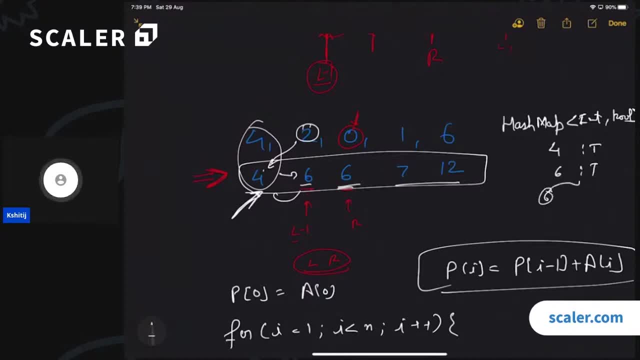 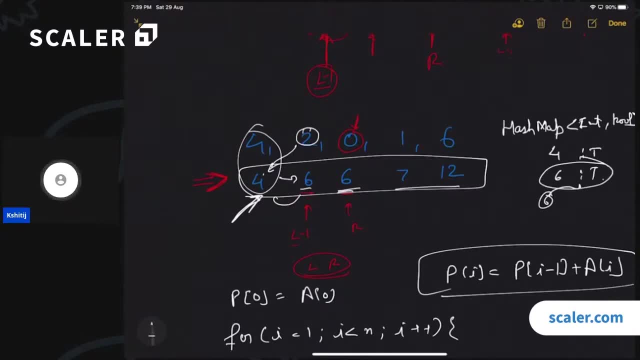 store. true. when you get another 6, you know that 6 has already occurred. if 6 has already occurred, this means that there is a subarray which is giving a zero sum. if you also want to find out, is the length of the subarray, instead of, instead of having the boolean, you can try to store the index here. this also. 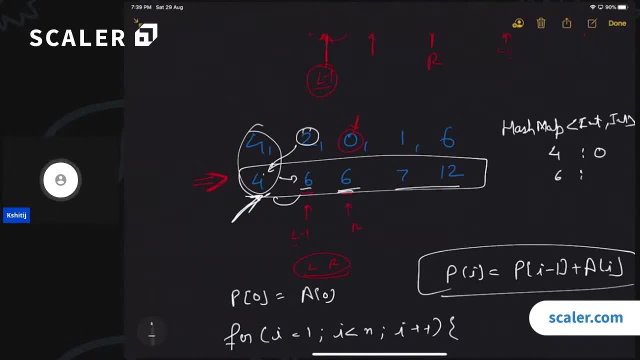 becomes integer and now you can say that 4 occurs at index 0, 6 occurs at index 1, then 6 again occurs at index 2. this means that from this index, this plus 1 to 2, we have got a subarray which is giving a sum equals. 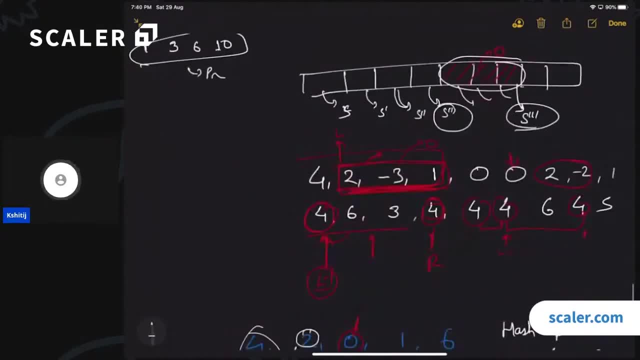 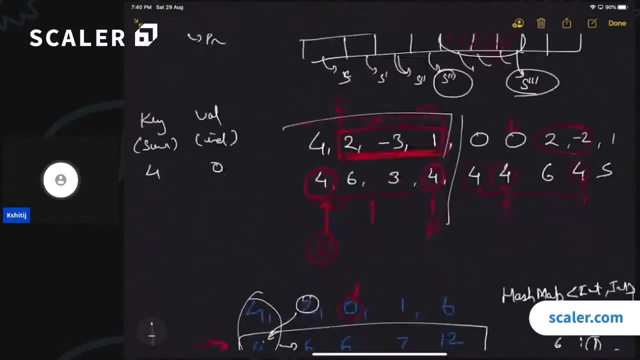 to 0. okay, let's take this example which we initially had, this one. right, you can have your key and value. key is the sum, value is the index in the hash map. you get 4 sum at index 0, then you get 6 sum at index 1, 3 at 2. 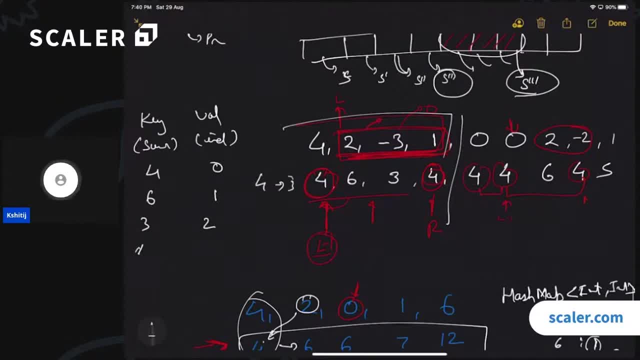 and then you again get 4 at index 3. right now. we had discussed right that keys are going to be unique. so once you get another same key you can just check that this key is already present in the hash map and the starting index was 0. this means from 1 to 3. i have an array which is giving sum. 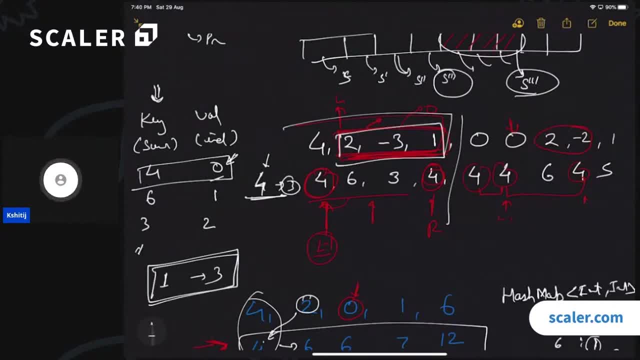 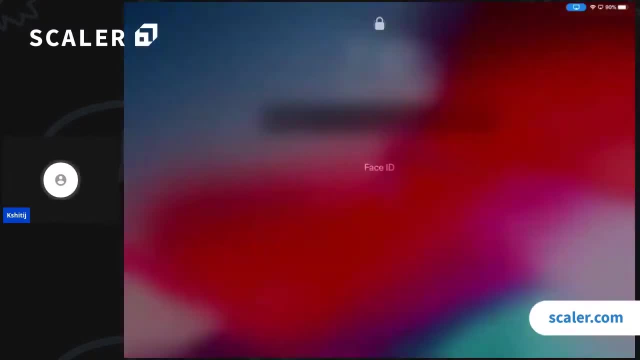 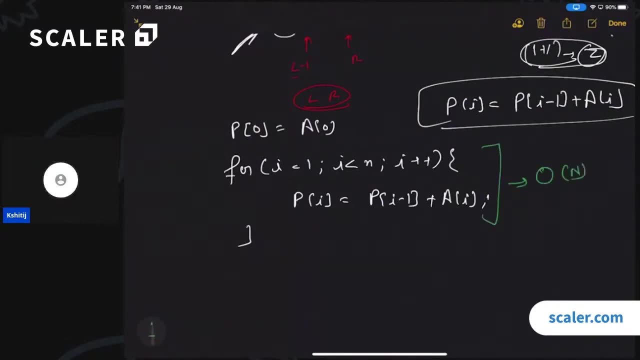 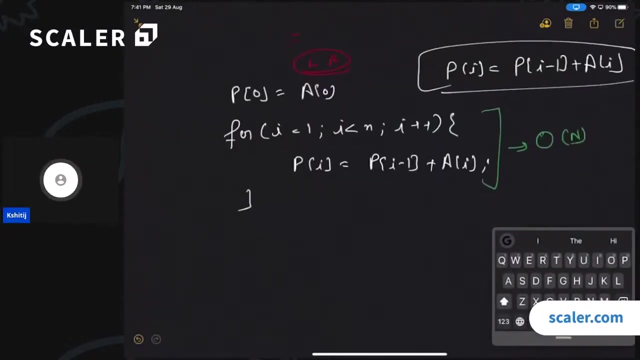 equals to 0. okay, does this make sense to everyone? what is the time complexity of this complete problem, of this, this complete algorithm? first of all, we have calculated the prefix sum. this cost us order and while calculating the prefix sum only, you can just also enter in the hash map right here. 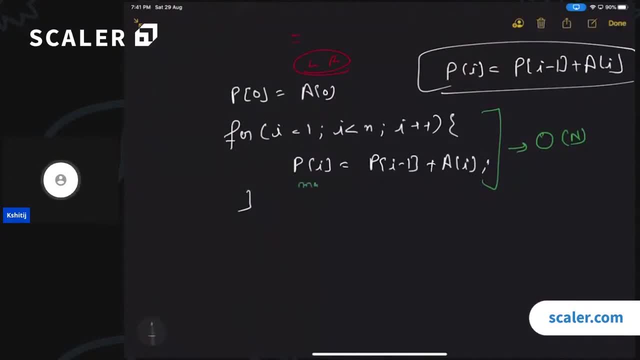 only you. what you can do is you can do your map dot put, or first maybe you can check if, if map dot put bi, this means that you have found a sub array. you can directly return true, right. else you can say map dot put bi and comma. whatever you, you are storing, whether it is index or or whether it is. 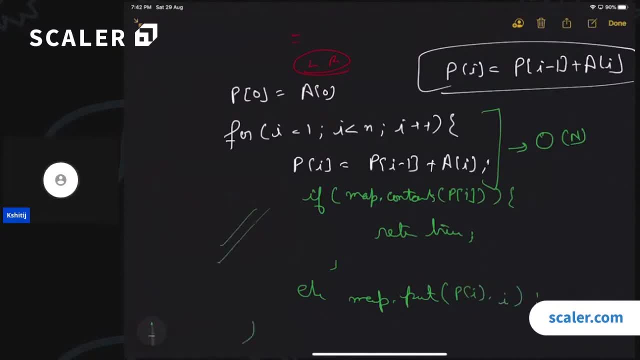 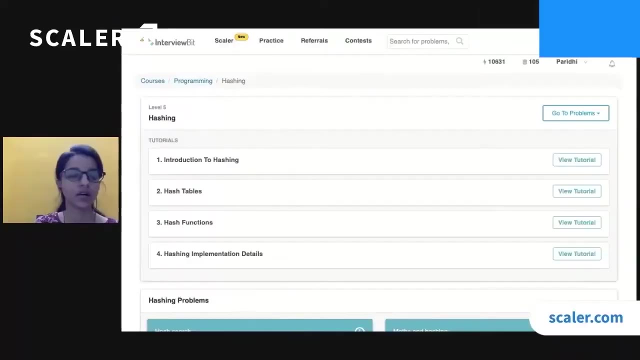 your true or false right and this is going to solve the problem. overall time complexity. here is order and okay. so, guys, i will now end this session. please, please, do solve all the problems. thank you, guys. hello everyone. so today we have the topic as hashing and i am pardi, i am a software developer at interview bit, so today i have 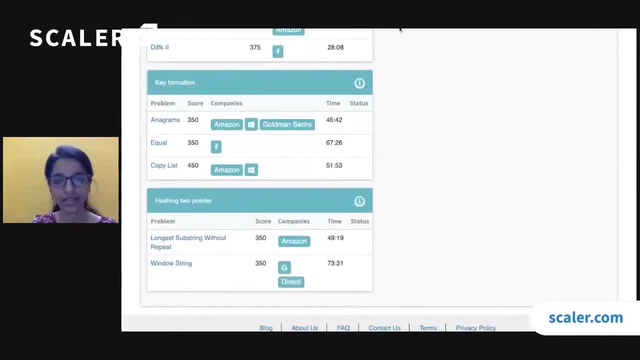 selected two, three questions, two questions basically that i'm going to discuss here and it's it's basically how important there are, they are from interview point of view, so i have selected them and, uh, so today we are going to do. first question is anagram. so let's quickly dive. 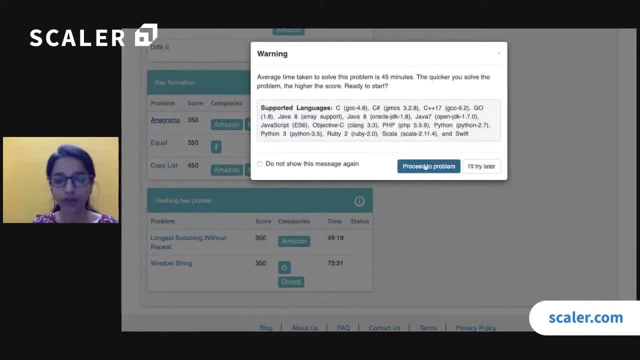 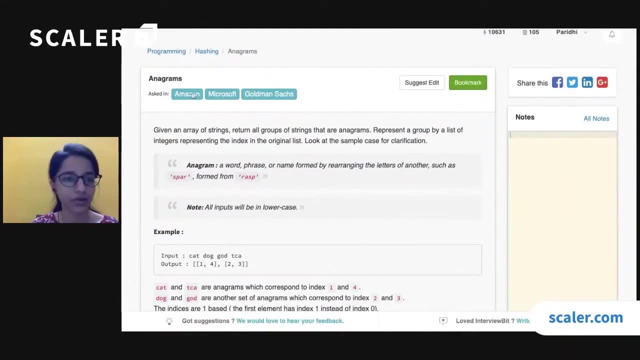 into that? okay, so today we are going to do our first question and that problem is anagram. this is very famous problem. this has been asked in amazon, microsoft, goldman, as you guys can see, very important from the interview point of view. let's let's quickly see what it says. okay, so, given an 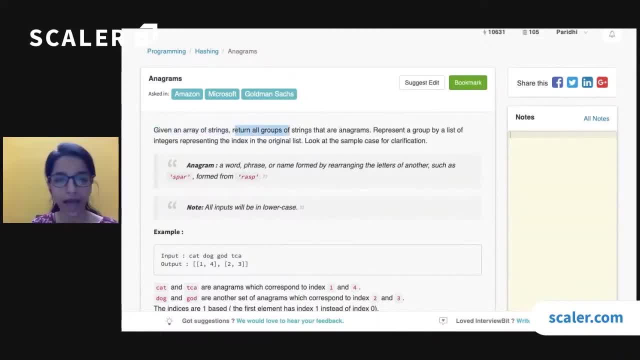 array of strings to return all groups of strings that are anagrams. okay so, represent a group by a list of integers representing the index in the original list. fine, so we are given a group of anagrams and basically we have to group the same, basically the anagrams together. okay, so let's see the example for: 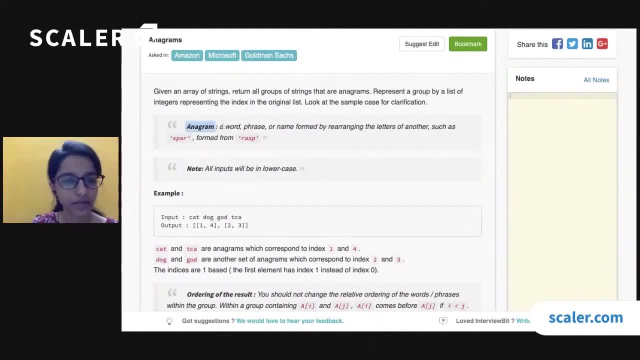 clarification. first of all, what is an anagram? so it's a word, a phrase or name formed by rearranging the letters of anagrams. another, such as spar, is there, formed from rasp. okay, so basically, an anagram is a word in which so uh, two, two, uh strings can be said as anagrams if they have same characters. right, and the 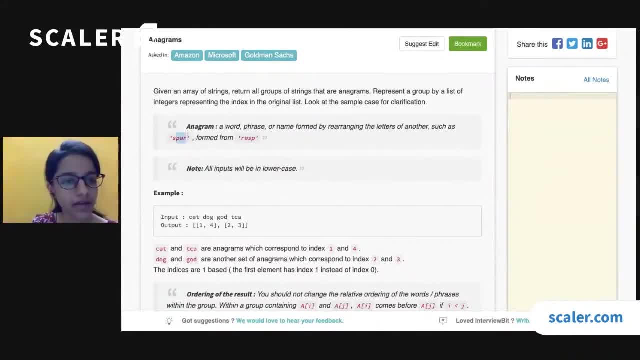 frequency of the characters is also same, but their order is different. okay, so here as we can see that s is present in spar and s is also present in rasp, then p is present in r and p is present in rasp. likewise, a is present in spar and a is present in rasp and r is present in. 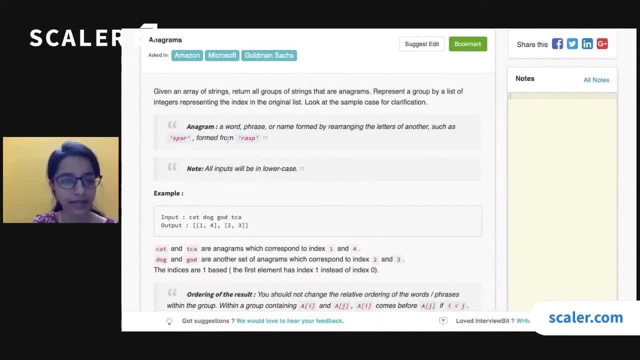 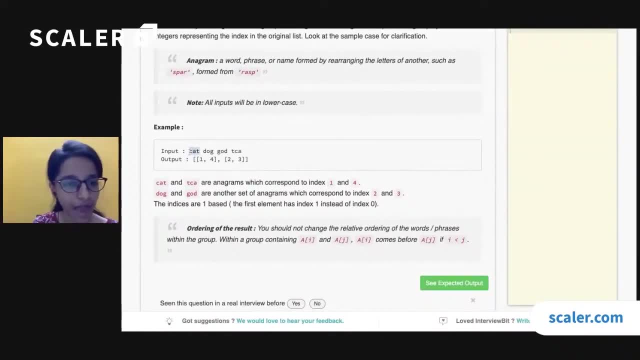 spar and r is present in rasp, fine, and these are the only characters. so these characters are basically jumbled right. so these are known as anagrams. now, given the example, we have cat dog, uh, god and tca, fine. so these are the anagrams and we have to group the anagrams together, right, okay, fine, so 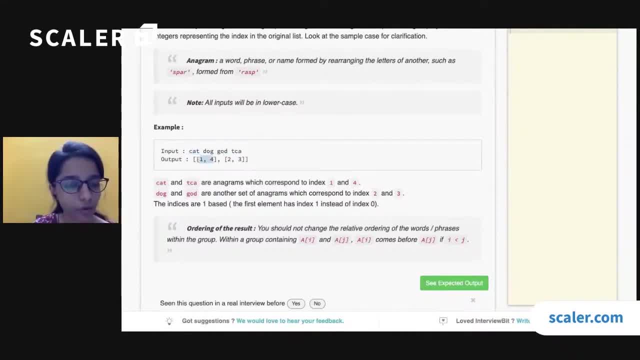 uh, we have cat and i can see that one and four are anagram. that means cat and tc are anagrams. okay, fine, they have same set of characters and frequencies also same, makes sense. and dog is there and god is there. they both are anagrams. fine, makes sense. so, uh, they have same. 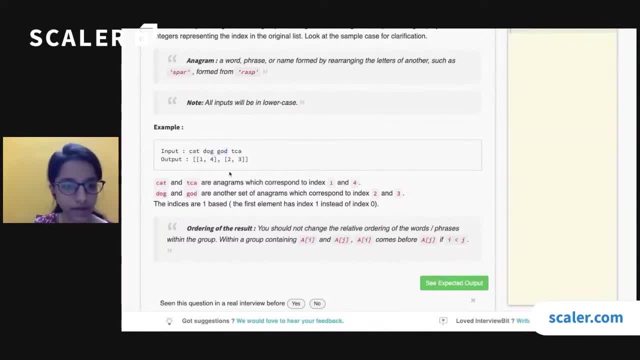 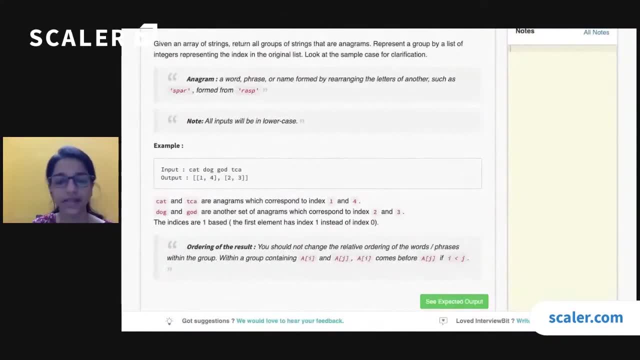 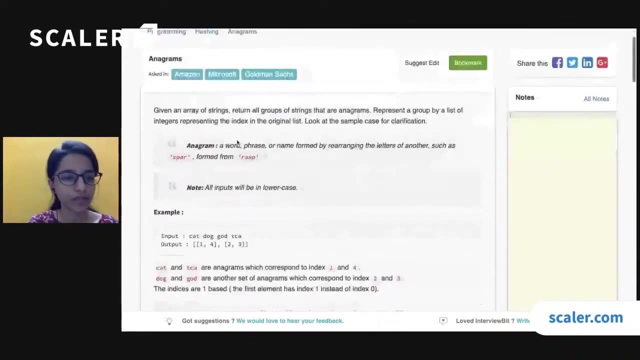 uh, basically, characters and frequencies also same, fine, okay. so, uh, what do you think we can do? what is the first thing that comes to your mind? so what i can think of is that, um, these two, from these two anagrams, as given in the example over here, the spar and rasp, right, they have same. 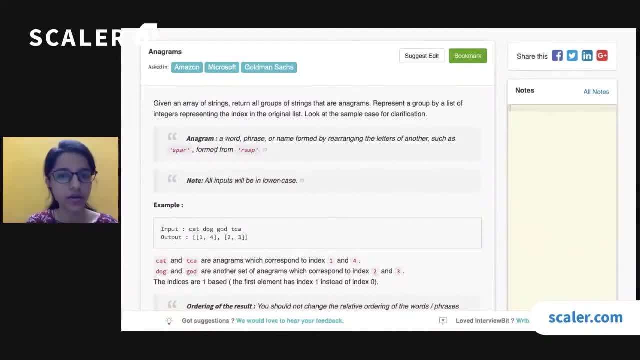 characters and also the frequency same. so maybe if i like sort them, they should give the same result, right? so if i sort spar i should get the same result as if i spot a sort right? does that make sense exactly? so you guys have started to reply and you are on the right. 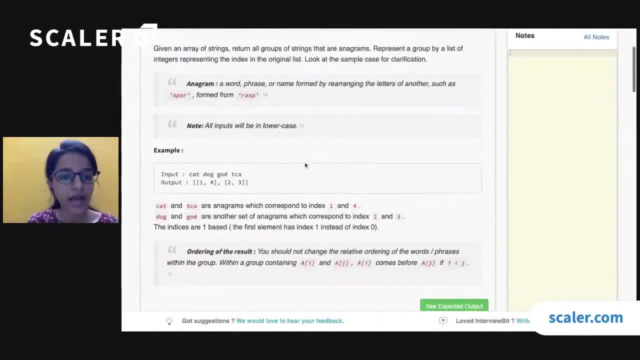 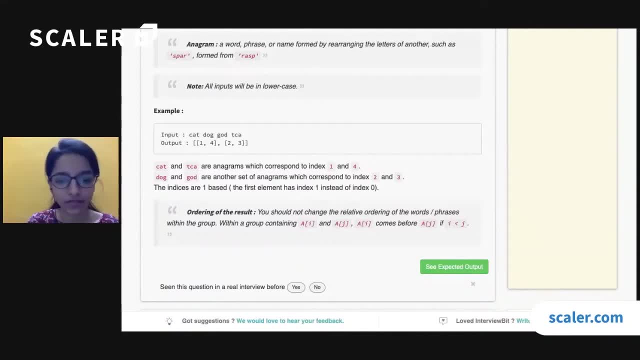 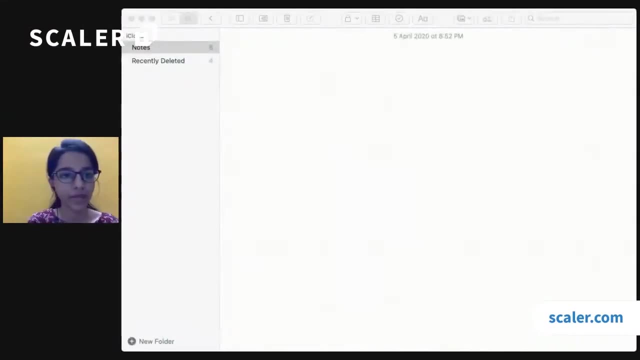 track that we can sort them, and after sorting, what is the thing that we are going to get? let's see. so let me share my screen. first of all, the notepad screen. so, uh, here we have. so in the example we have fine, so let me just copy it down. so we have cat dog and god and tca. so we have cat dog. 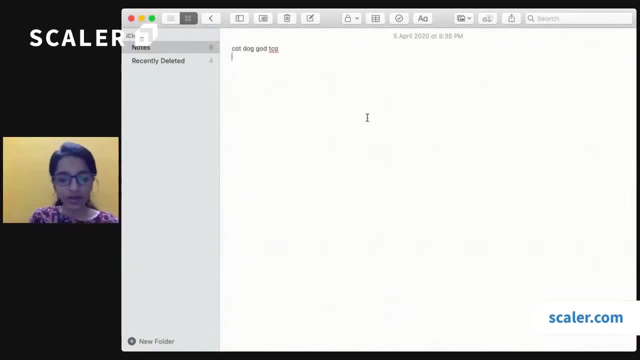 so i'm just copying it down on here, so okay. so if i sort them, this will become a c t right. and if i sought, so if if i sought dog, i will get d g o right. if i sought god, i will again get dgo. and if i saw tca, i will okay. so wait a minute, it just got auto corrected. uh, d g a. oh sorry, d g o. and. 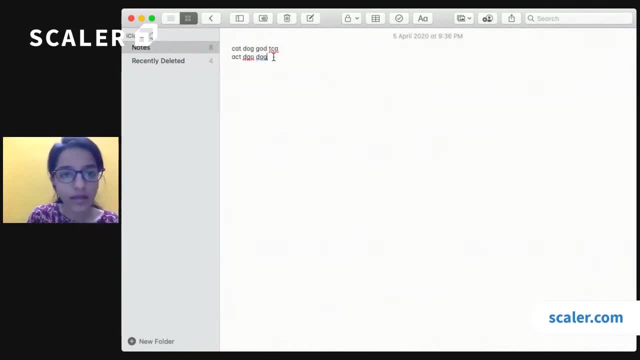 this will also be b g, o and this will be: uh, this will be act. right, so that means here we know that cat, as in the example, cat and tca are anagrams and when we sort them out, then act and act, we have got the same string, right, okay, that means anagrams will get, will have the same string. 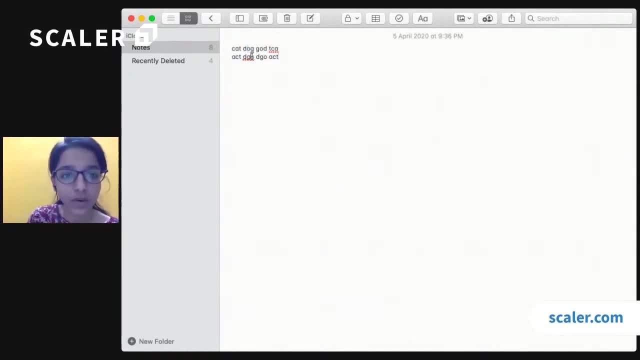 makes sense. and likewise in dog and god, dgo and dgo, they have the same string. now what can we do to sort them out, so we can actually group them up, so, as someone of you has have said that we can hash them up correctly, that perfectly makes sense, that, uh, basically, here the sorted string can act. 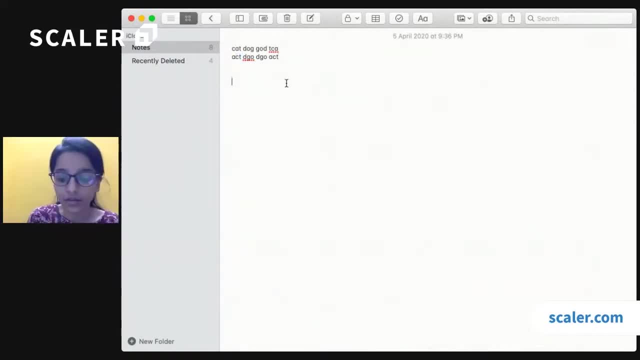 as a. so here the sorted string can act as a. the key, right? the key is the sorted string, and the value are going to be the indices of the anagrams. does that make sense? so here the so let's, let's. so we have one, this is one, this is two, this is three, this is four and we want the indices only. 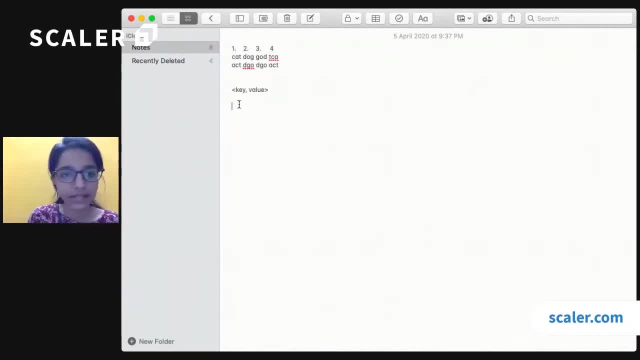 right. so indices are starting from one in this case. so basically the key here for c uh cat is going to be a cp and here we are going to have the value will be a. we can see a vector where we can store the indices of the anagrams. so a, c, t is a string and c at is an. 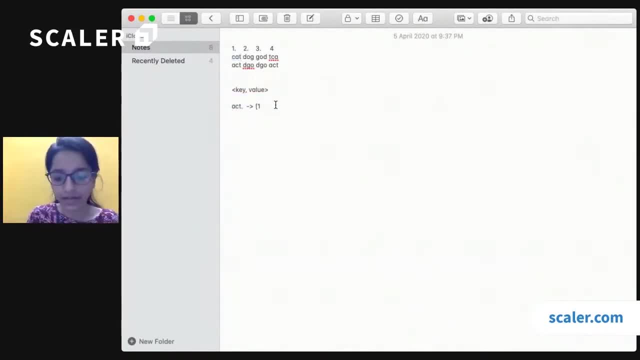 anagram for that. so that means we can have uh in a vector, we can have one, and also this pca is also: if we sort it up, we will get act right. so that means the same string and so the value is going to be four over here, right? so that means we have actually paired up the anagrams. the main task. 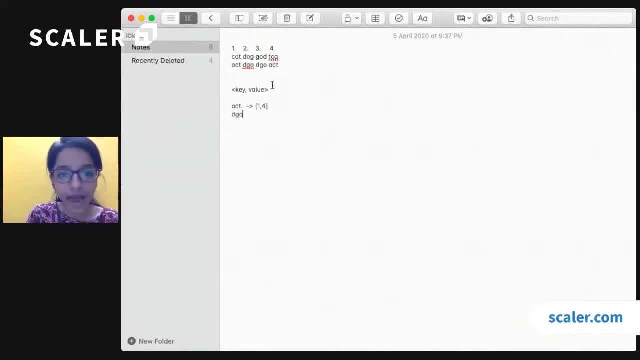 right now, the second string is dgo. right, and uh, we can pair the strings that are forming the anagrams. that means two and three. does that make sense? so right, we can do it in various ways. we can even hash them up in various ways. we can use frequency arrays as well, so we can do it in. 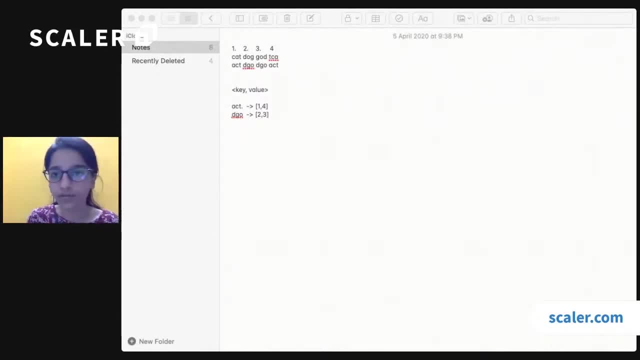 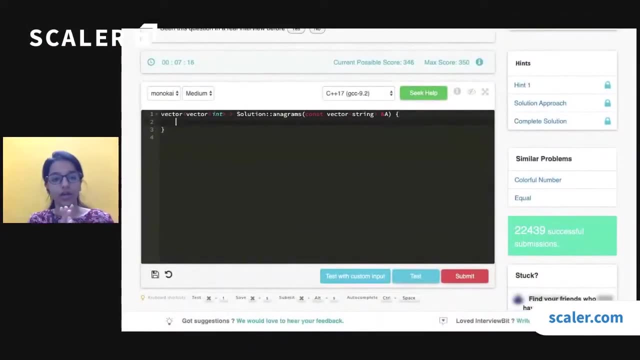 any way, right? so let's just code it up. so i think most of you are ready for this, let's code it up. so here we have the screen and let's quickly code it up, right, okay? so, uh, basically, we will be keeping. first of all, we need a vector. 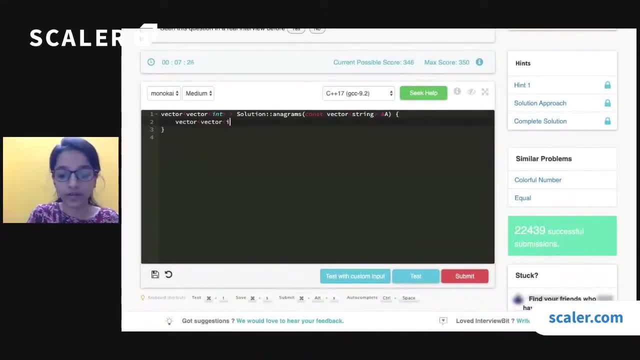 of vector for um, for the answer thing, for storing the answer, right. so vector of vector of n. and also we need the map- sorry, we need a map, unordered map. so we basically do int comma, okay, no, sorry, not. we need string, right, we need string. and we need a vector of int. let's call it maybe group, right. 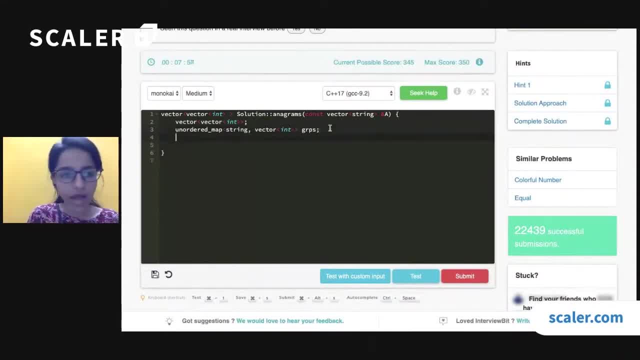 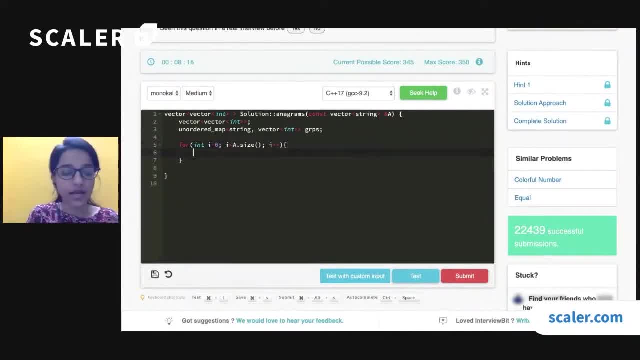 right, and i plus plus now. okay, so we will take the first string. let's take it in. let's say, we will actually have to generate the copy of the string because we have to sort them up and also we need the original string, right? so therefore we are. 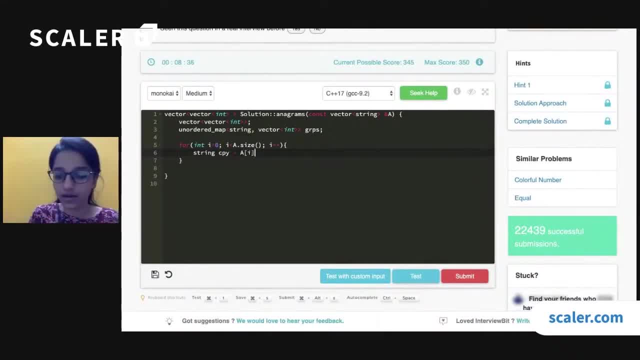 maintaining a copy. so let's take it in here and this will create a copy. now let's sort the string. so let's sort the copy string. so cpy dot begin, then um, cpy dot end. right, so we have sorted, and now the task is that we can actually, you know, hash it. 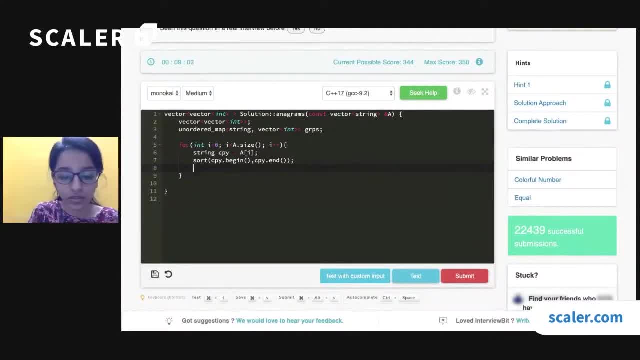 so that's what we are doing, so let's hash it. so the groups is the map that we have taken and this is copy, right, the string is copy. that we have sorted. okay, so we have sorted it and let me see if there are some comments. okay, so, um, now, now, what should i do? 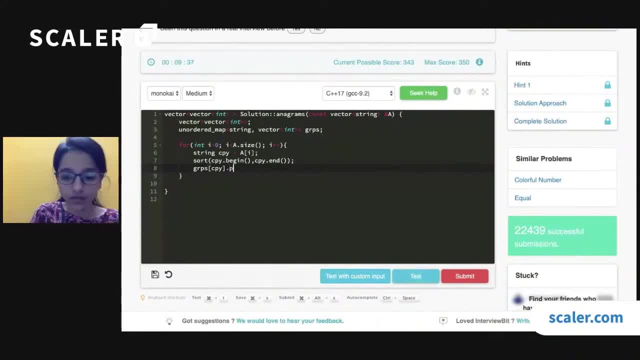 may i get it in the comments? what shall i write? so basically, i can push. if that copy is present, i can push the index value right. so after sorting this copy string, the string at ai, if after sorting we get a string which is there in the hash right, which is present, 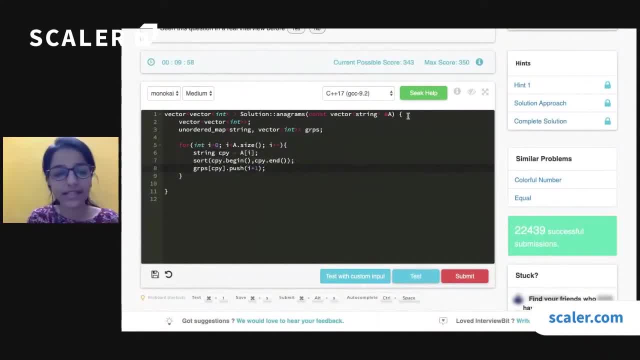 in the key we can actually push. i plus one to that. it's exactly what we have done in our notepad right, so we will do it for all the strings. and finally, after doing it, we actually have to iterate through the map. does that make sense, that we have to iterate through the map? so let's do it. oh, groups is the map. 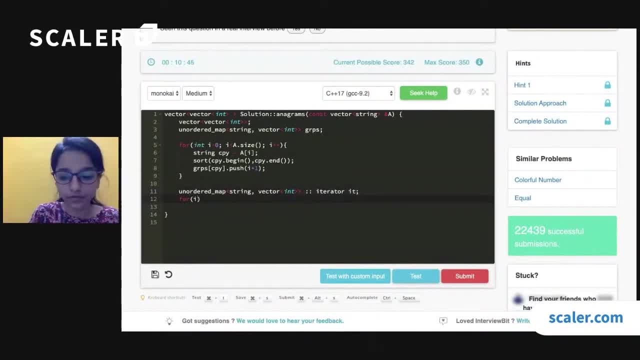 a creator. let's say it now, we will simply move through it. so that means it equal to that is groups dot begin, then it is not equal to groups dot end and it plus plus, right? so if so we have to just take the value right. so here we have actually maintained an answer variable. 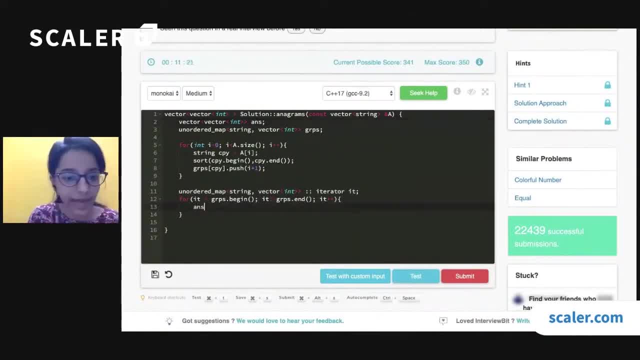 answer array and we have to basically push the entire vector that we have created into the group. so that is groups dot begin. then it is not equal to groups dot end and it is not our answer in the main. answer right, so basically we will be pushing back ip. that means the iterator. 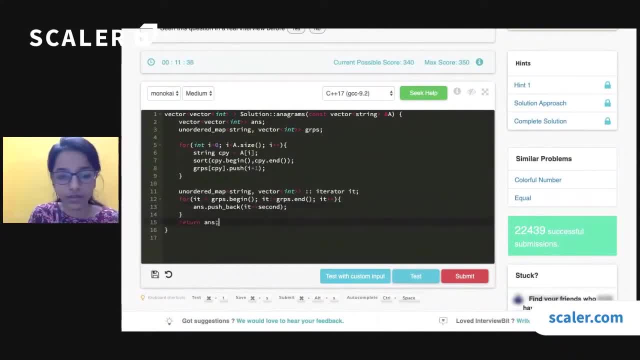 dot second, and here we can simply return the answer array: right, so does this look fine? please check everyone. are you guys coding with me? yes, so basically for that? um, we are. we are actually storing the indices only, right. so, nilesh, we are storing the indices only we. 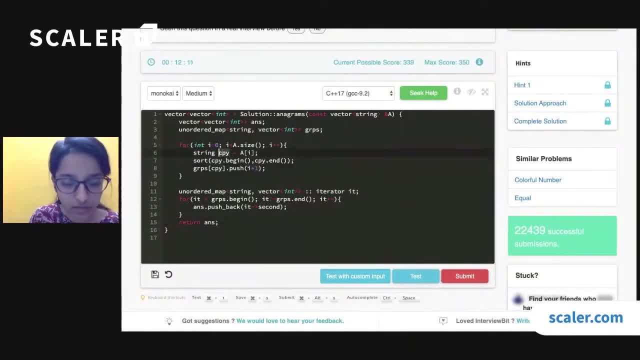 actually have taken the string in the copy string, that means the extra string. then we have actually uh sorted this copy, uh string and here we need not maintain the main string. basically, we just want the index of that right. so here we are pushing the index right, just as we have seen. 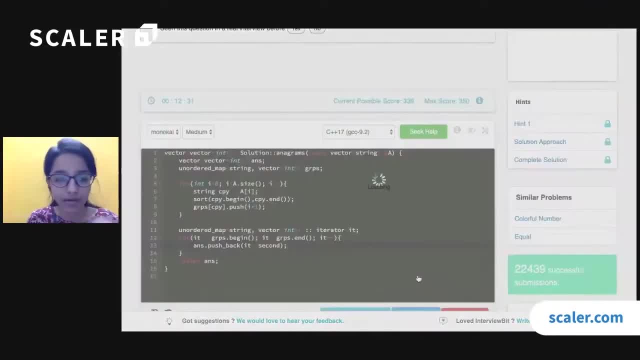 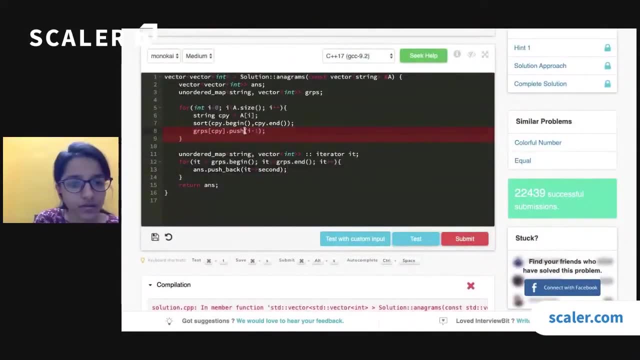 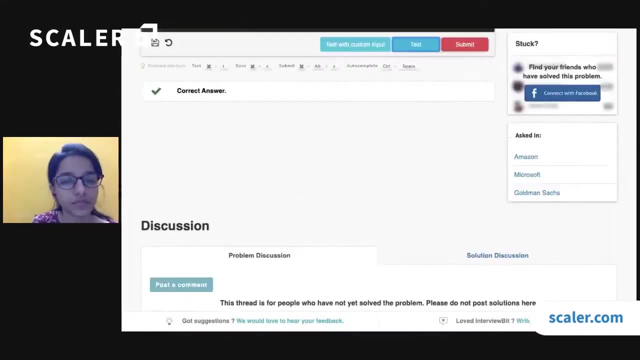 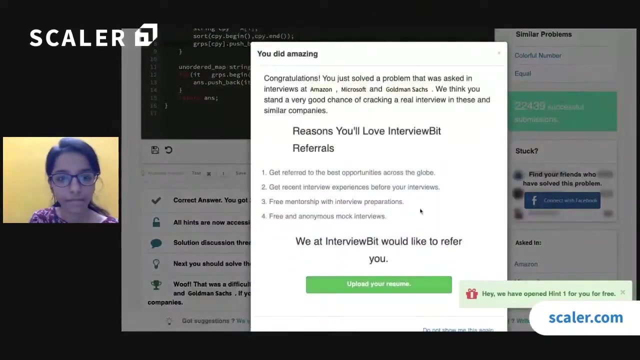 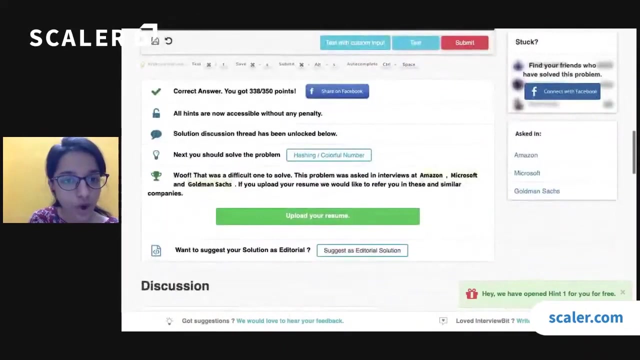 in the notepad. so that's what we are doing. let's try it now. let's see if it passes. oh sorry, so this should be pushed back. great, let's see if it gets submitted. cool, so we have done a good job and, uh, we have scored 338 out of 330, not bad. 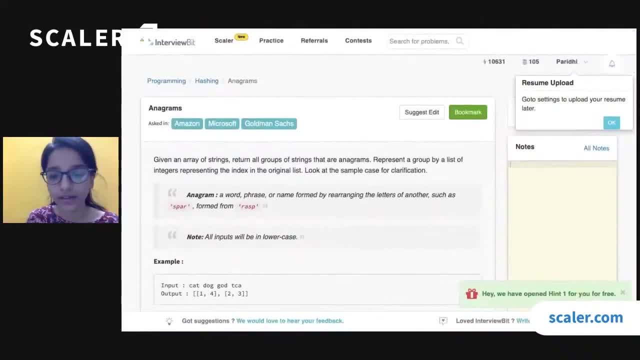 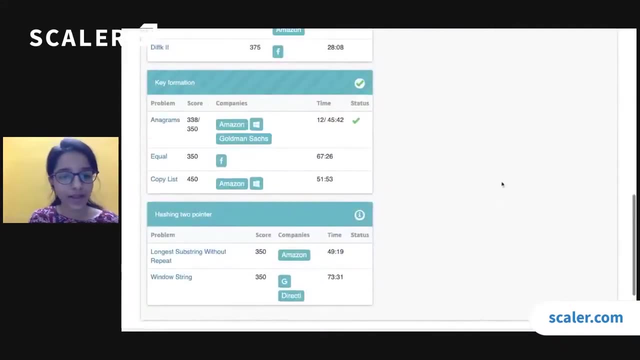 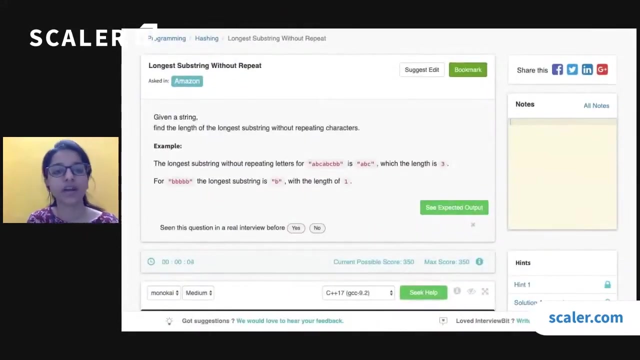 okay. so have you guys got it? have you guys got it? are you guys with me? is it clear? sure, now do submit it with me, any, ah, okay, so now let's do the next question of the day. asked in various other companies as well. can't remember the name right now, but yes, this is a. 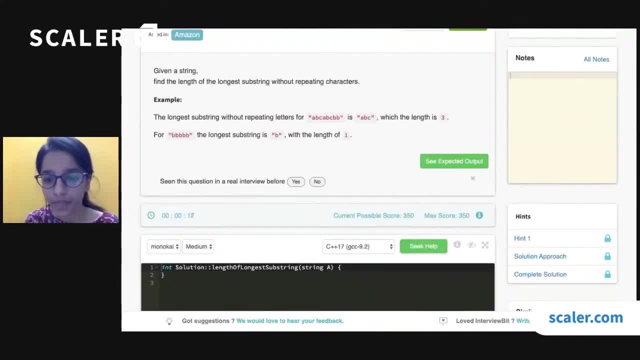 very important question, so let's get to it, okay. so ashish says he has a question in interview. we are, we are we allowed to use inbuilt function? okay. so basically, it's like when you are asked to implement something or which is, let's say, you are asked to implement a substring function, 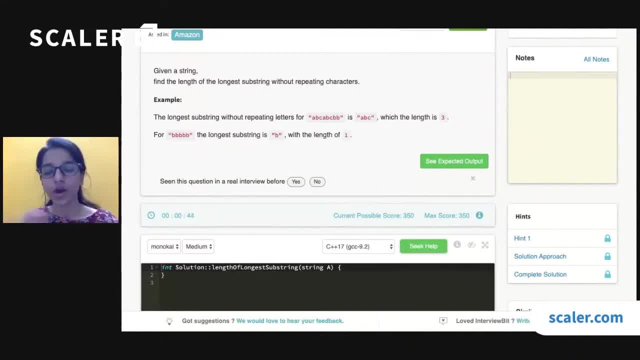 in that case you cannot, you know- use it. or let's say you are asked to sort the array, so the trivial question is that. so the main question here is that you have asked to sort it, so how can you use a given the inbuilt function? right, in that case you have to actually perform. 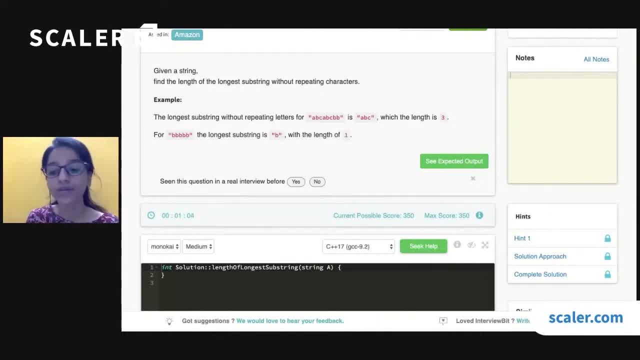 the sorting with the various algorithms you have. you can't use inbuilt function in that case, right? so here the question is different. you can use the inbuilt function in this case if it's not mentioned. if it's mentioned that you cannot use, then you cannot use, right? 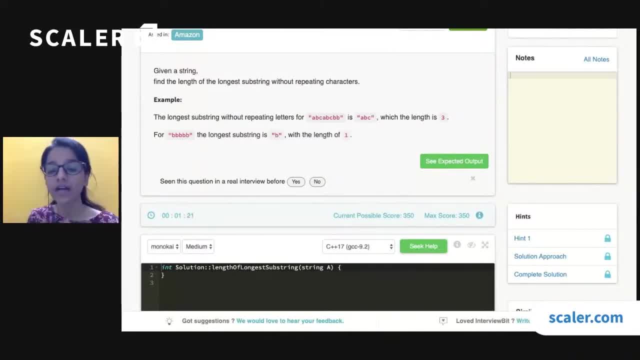 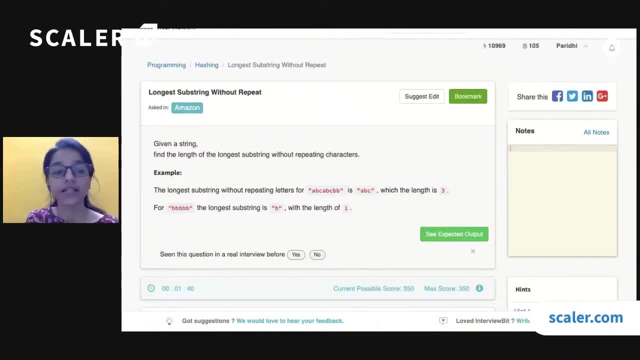 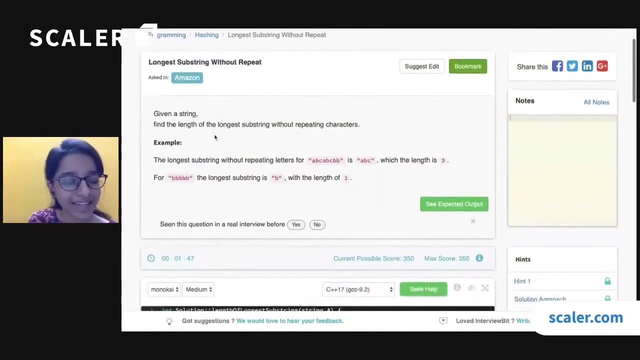 so it actually depends- you can actually ask your interviewer about it- that if you can use it or not, make sense, cool, okay, great. so guys, let's move on to the next question. and the next question is longest substring without repeat. okay, so, uh, let's see. so the 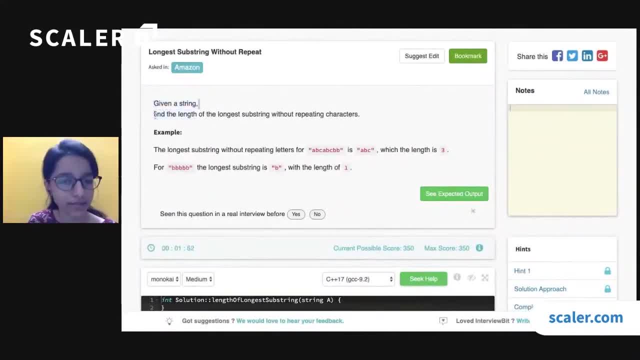 question says that, given a string, find the length of the longest substring without a repeating character. okay, so here we are, given a string, or this is the string, let's say, and here it says that abc is the longest string and the length is three. that means abc is the longest such substring. 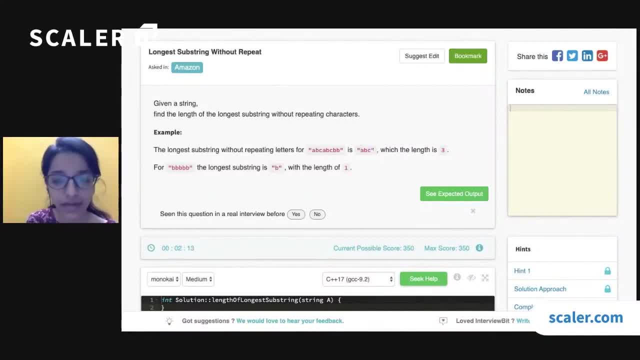 in which there are no repeating characters, as you can see that, okay, abc has unique characters, okay, so, basically, we want a substring out of a long string which which has only the unique characters, right, which doesn't have a non, which doesn't have a repeating character. basically, in the second example, as you see, 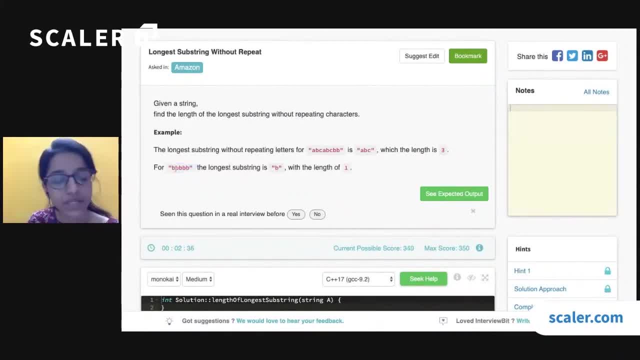 that we have so many b's over here and that means here the substring is just a. b that means of length, one that has a unique character. if we try to extend this up, that means if we try to take um, try to make the length two, then definitely we will get bb and length. 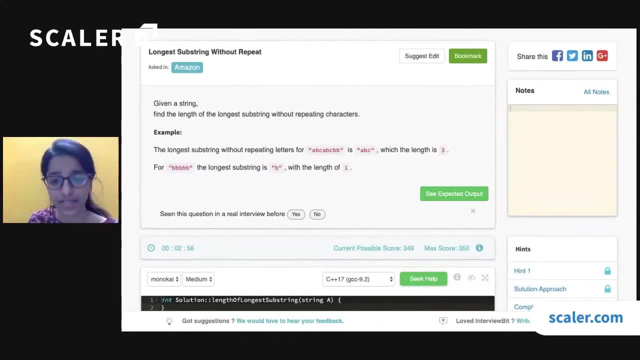 of two doesn't have unique characters. does the question make sense to everyone? yes, so everyone. okay, could you elaborate more that? what would you do, guys? please at least come up with the brute force approach. i would like to discuss it with you all. that, what do you? 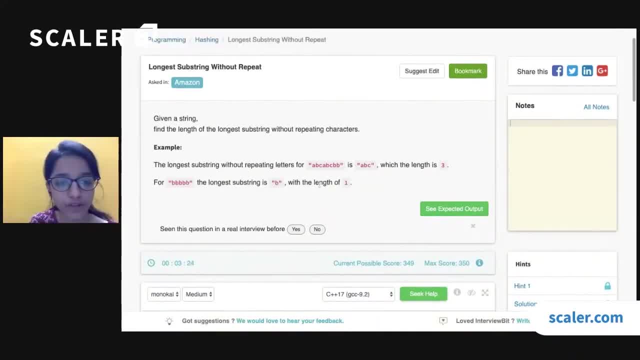 have in your minds. can you guys think of the brute force approach for this question? is the question clear to you all? okay? so, guys, please think on this question. okay, and then in a minute we are going to proceed with the solution. okay, so garima says that. please explain. 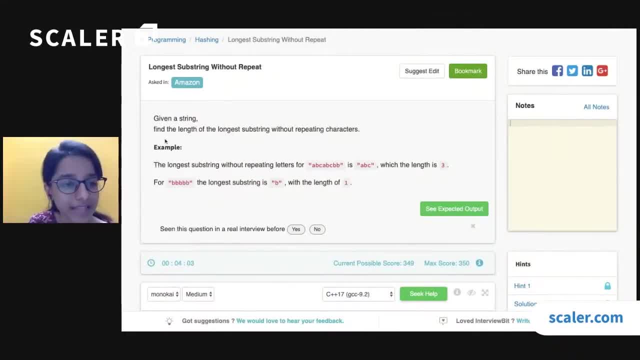 the question again. sure, garima. so here we have the solution. okay, so garima says that we have a string. okay, so here it says that you are given a string. okay, you are given a string and you have to find the length of the longest substring without repeating characters. 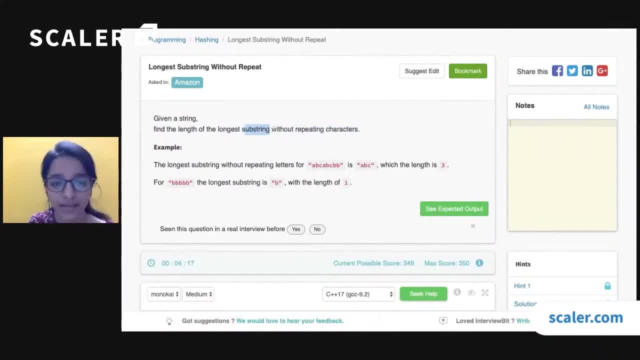 now, first of all, do you guys understand what a substring is? so a substring is that when you take, uh, so here, if i say that this is a string, right, so what are the substrings of this string? so let me actually, um, show you my screen, cool. so here is my notepad screen. 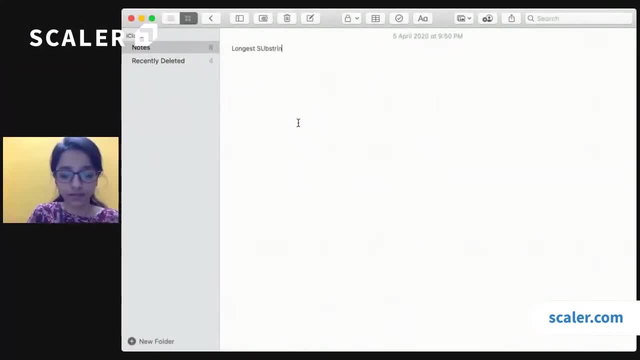 okay, so here we are discussing the longest um substring without repeating characters. okay, so let's say, i have a string a, b, c, d and or b c. okay, a, b, c, d, d, now how? first of all, what are the substrings of this string? so a is a substring, then a, b is a substring. 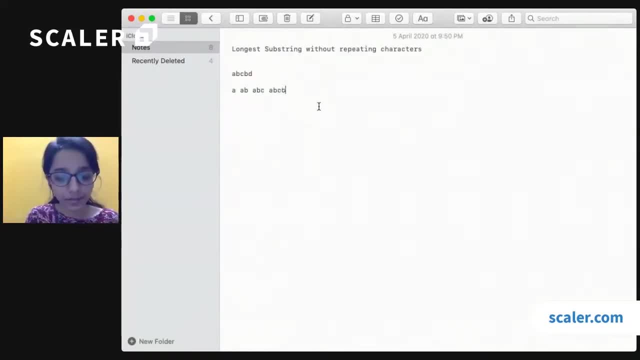 then a, b, c is a substring, maybe c, b is a substring. then a, b, c is a substring. a, b, c, be is a substring. A, B, C, B, B is a substring. okay, Then starting from B, we have just B, then B, C, then B. 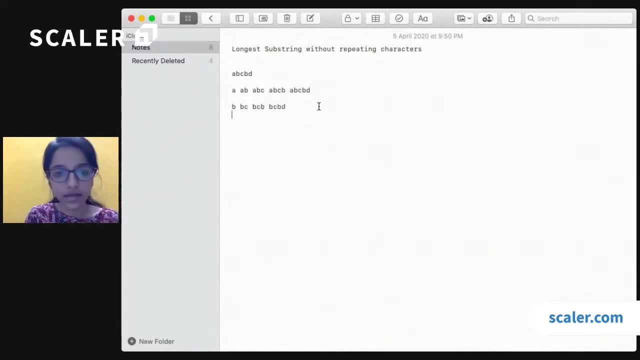 C, B, then we have B, C, B, B, right. Then, starting from C, we have C, then C, B, then C, B, C, B, D, and starting from D, we have just B, then B, D and then, starting from D, 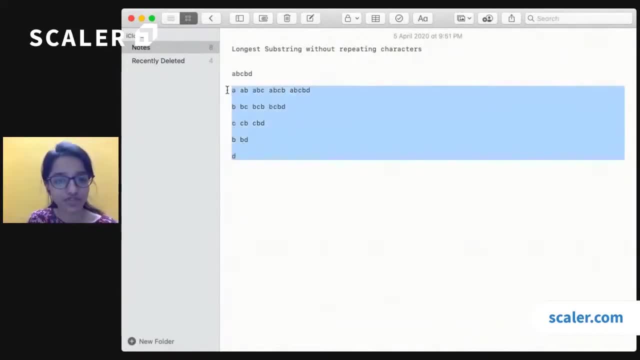 we just have D. Does that make sense? that these are the substrings of this string, the consecutive characters? Garima is the question, so the question says that once. So basically, you have to find the longest length of the substring that has unique characters Here. 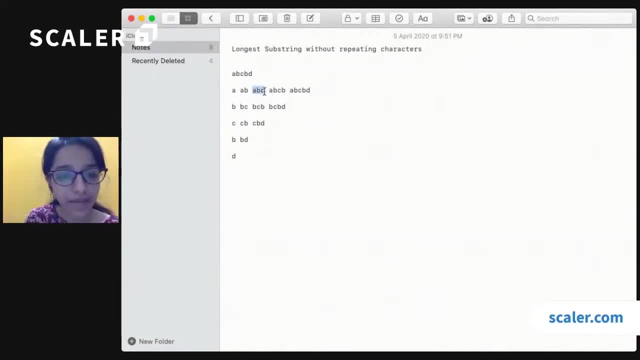 such a longest length is just A, B, C, because if we consider any length which is beyond 3, then that has a repeating character. So if we have, let's say, A, B, C, B, right, So in this case also we have two repeating characters, as in one repeating character. 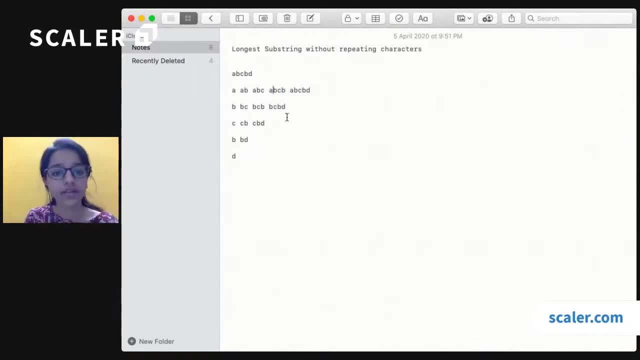 that is the longest length of the substring. So if we have a, let's say A, B, C, B, that is B, right. So B occurs two times, which we don't want. So the question says that: 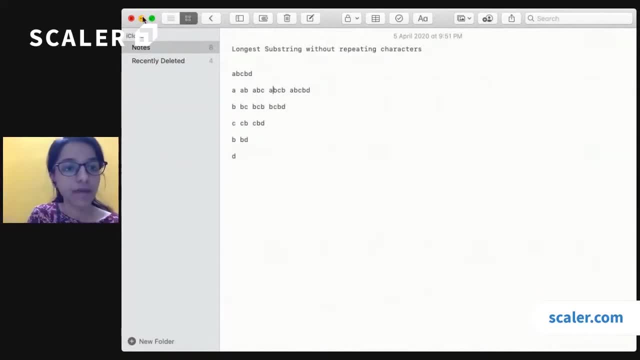 you have to find the longest substring without repeating characters. Am I clear with the question, guys? Am I clear with the question? Okay, great, Okay, so let me clear this up, right. Okay, so let me actually build your solution, then you will be more clear, Okay. 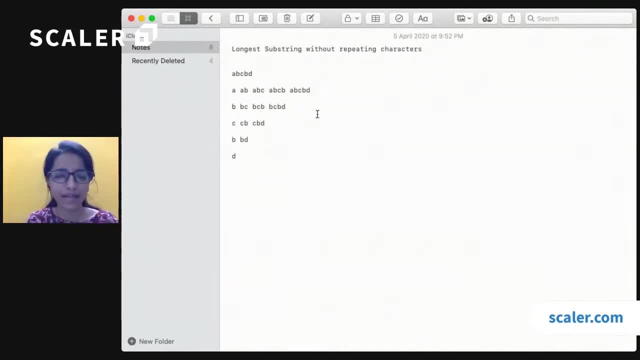 so the brute force approach that comes to my mind is that we can generate all the substrings- right, We can generate all these substrings. and we can generate all the substrings and we can check if the substring consists of unique characters or not, right? So how to check if that? 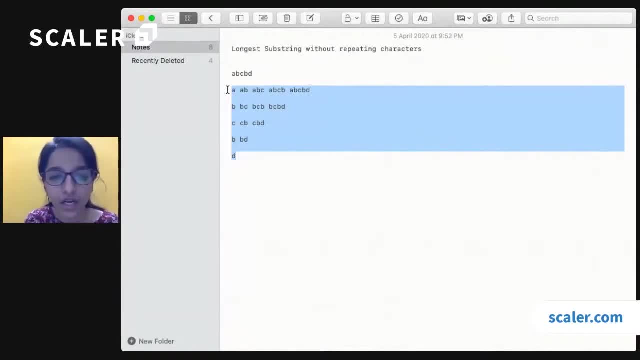 if a substring consists of unique characters or not. So, basically, for that purpose, we can maintain a hash map. what's it So? we can maintain a hash map that will tell us that if some character is already present in our string or not, Does that make sense? that we can use a? 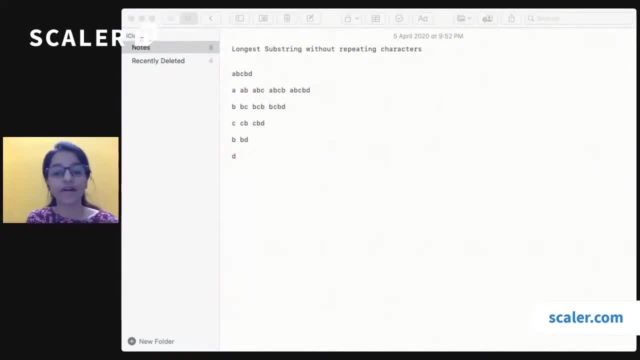 hash map, because it tells us in just order of one time that, okay, if some character exists or not, already exists or not, right, So this is the brute force approach. So does anyone know that how many total substrings we can create out of a string? How many total substrings are there? 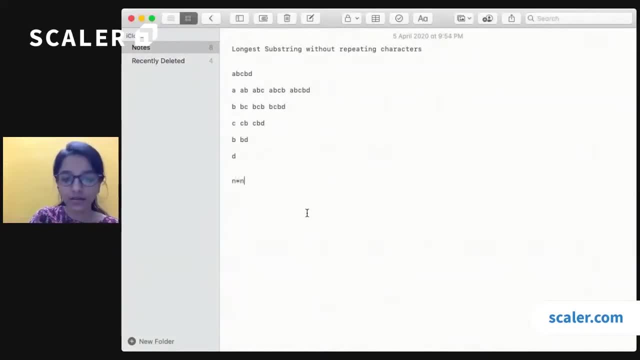 Okay, so total substrings are: n into n- wait a minute- n into n plus 1 by 2.. Okay, these are the total number of substring that we can create, and where n is the number of characters in the string. Now, so, once we generate all the substrings and then if we check with the help of a hash map, 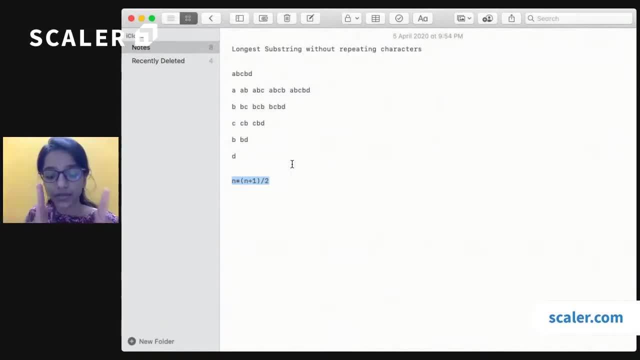 that if that particular substring has unique characters or not, then the time complexity for first of all for generating the substring is going to be order of n, square. okay, Because total we have n into n plus 1 by 2 number of substring, therefore the time complexity of generating these. 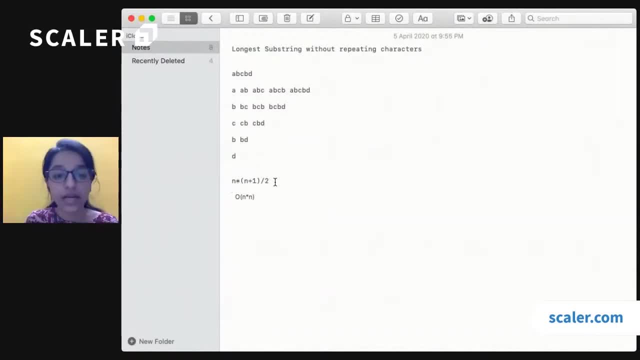 many substrings is order of n, So we can generate all the substrings. and then if we check with the help of n square now we have, we also have to check it with the help of a map if it consists of unique characters or not. So for that it's again going to take order of n. because why? Because, 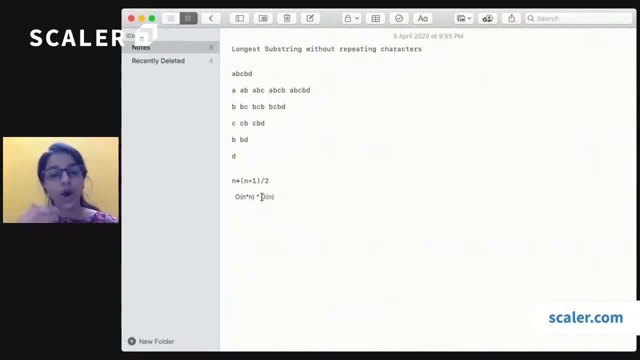 for maintaining the hash map. it's going to take again: order of n. So the total number of time complexity, the total time complexity, is going to be order of n. Does that make sense to everyone? Cool, So the time complexity is going to be n? cube, but it can be further. 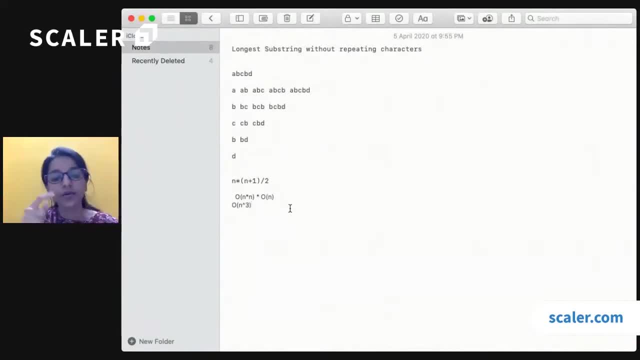 optimized if, while going through our second loop, we can actually check on that base only if we are getting the unique characters or not. So what I'm saying is that while maintaining the second for loop, in the second for loop itself we can check that that substring from i till j has unique. 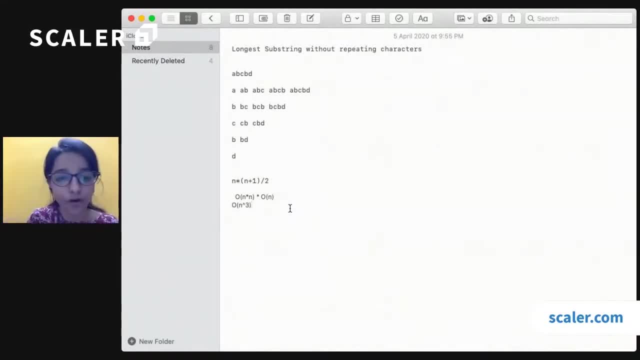 characters or not, And this we can do in our for loop only, the checking part. We don't have to do it separately For checking the unique string. Okay, So then the time complexity will reduce to order of n square right, Because here we will be doing it in our second for loop, only We will be checking it in. 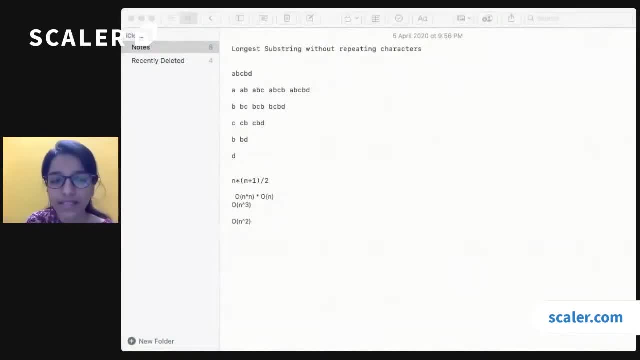 the second for loop only. Does that make sense, guys? Is it clear now that why n square? So n square is because while generating a string, let's say I am at a, so the string is. wait a minute. let's say the string is a, b. 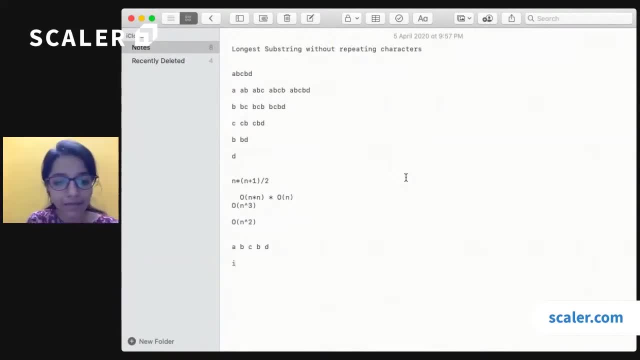 c, b, d. Right, this is our string. Now I'll keep my i pointer here and initially the j pointer will also be here. Okay, Now we will also maintain a map side by side and we will put the character in the map that 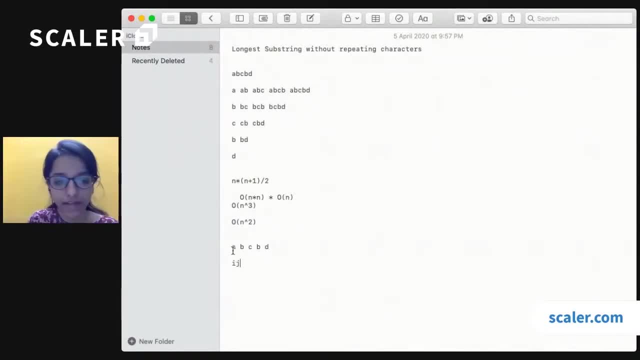 if so, for checking if it's unique or not, Right now in our map a is not there, Right, So we will put that. okay, a is not there, That means a is unique. let's put it in our map. So first we will check that, if some. 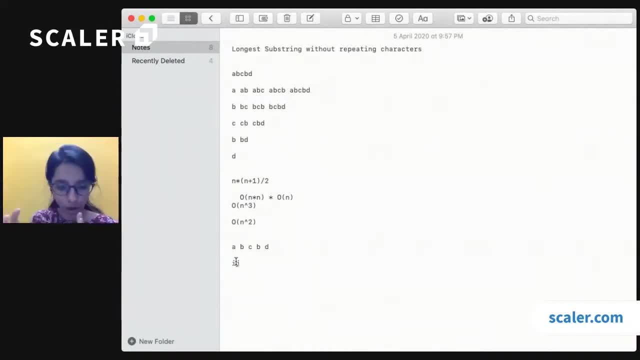 that okay. a is not there, that means a is unique. let's put it in our map. So first we will check that if some exists in the map or not. if it doesn't exist, that means that character is unique. once we get in, get 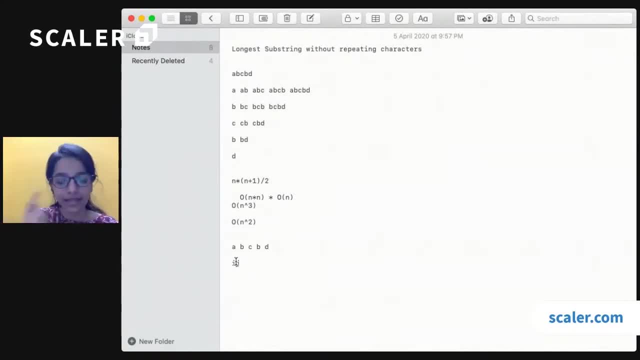 to know if that character is unique, then we can add that character in the map, okay, so, okay, now we have done it. so we have checked for string a, now we will move. so now we have ab, so we have in the map. we just have a till now. right now we will check that if the character at b is in our 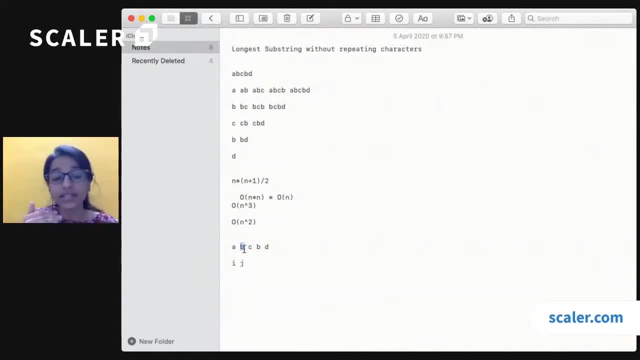 map or not. if it's not present, that means we it's a unique right. that means it's unique. but once we have checked that if it's unique, we will add it to our map because we have already taken it. so are you guys able to relate that how, in the second loop only, that is, while moving our j we 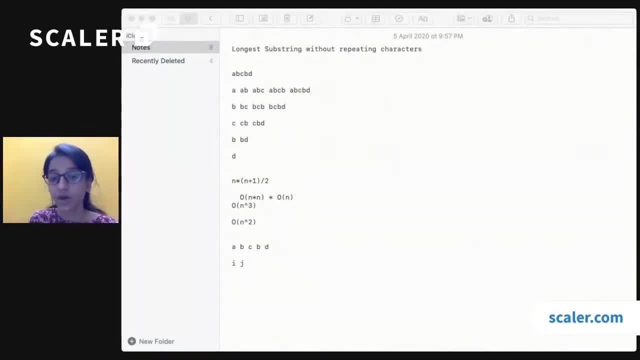 are able to check in the map. that's why the complexity is order of n square. okay, do try to dry run it on your own right, and then i am sure that you are going to get it. and if you are still confused, then you should definitely try to code that up now. i would try to, so okay, so here we are. 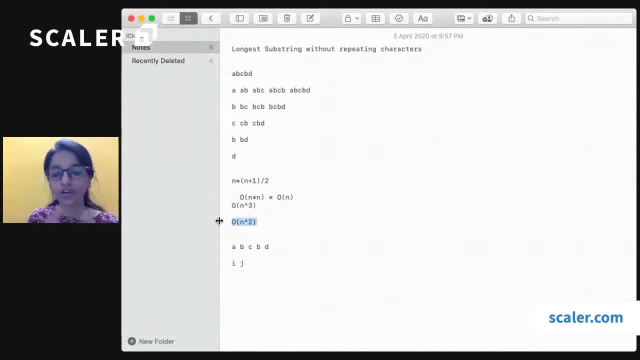 now. so the time complexity of the brute force solution is order of n square. right, or i would say a little optimized solution is order of n square, but here we are generating all the substrings. do we really need to generate all the substrings? so let me make my point clear from here. so we have. 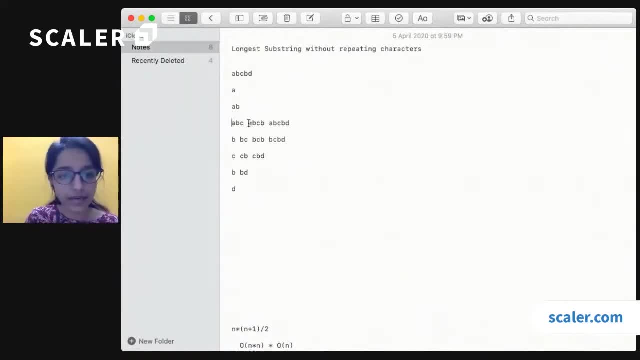 we have a, then a b, then a, b, c, a, b, c, b, a, b, c, b, b, right? so here we are actually generating all the substrings here. i am trying to make my point here that we actually don't need it. so i can figure it out. 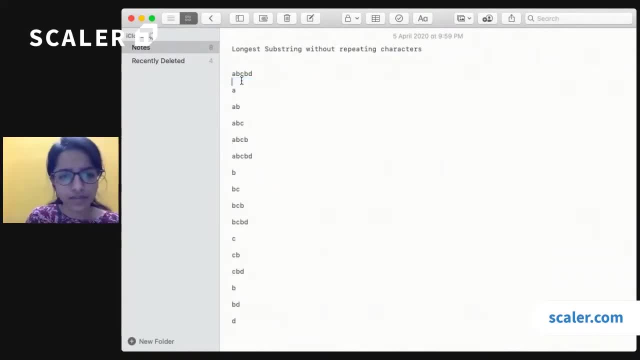 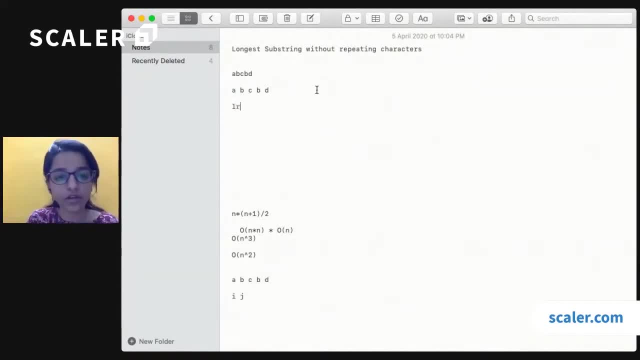 so we have to maintain the length as well. so we have to maintain the length as well. do it from the map, right, so we are also keeping the map. so let's keep a map. a has a. i can, so we can maintain a index. okay, so we can maintain our index. let's also put the indices one, two, three. 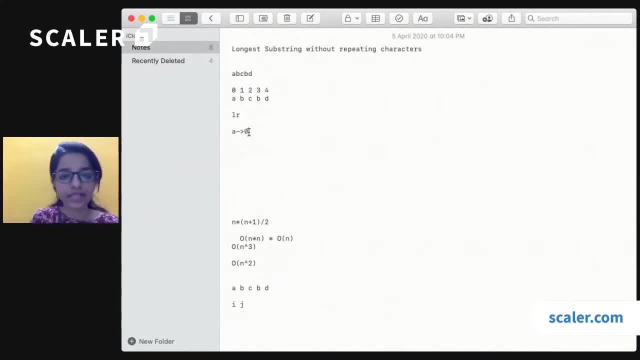 four: right, we can put an index over here. that means a is at index zero and a we have already taken. now let's try to expand the window. before that we will also keep a length variable which will keep the track of length. length right now is a, now we will move our r, so now the window has. 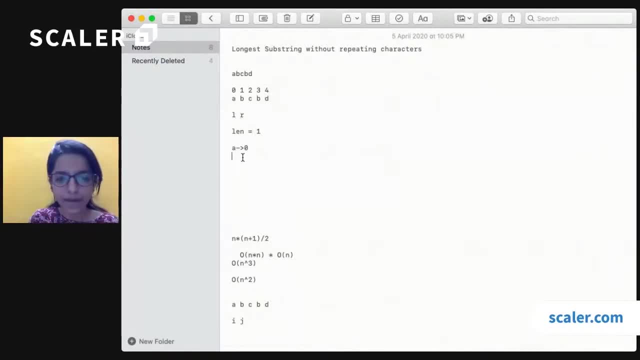 become from a to b. b is also not present in the map. let's make the length two right and add b to the map. index of b is one right now. let's increase r, so r is at c. so c is not there in our map. let's: 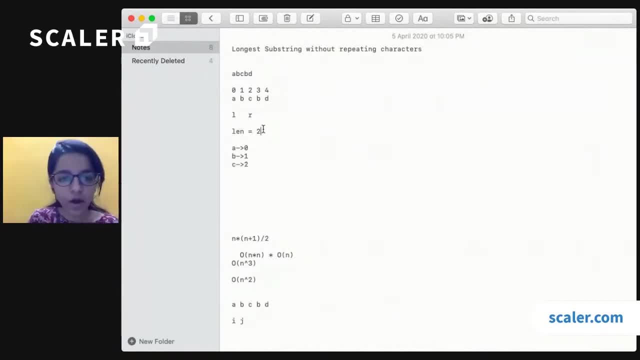 include c in the map with the index right, although the length has become three. now let's move r, okay, okay. okay, we saw that now the we don't have any unique characters, so that means length will remain same, and now we will move our left pointer so that we can actually remove the previous occurrence of b. 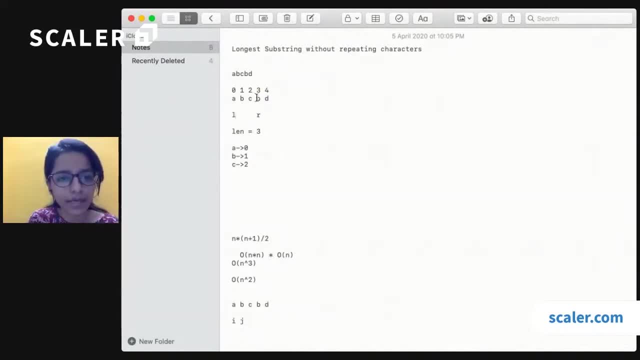 right, we will move our l till the point the b- the occurrence of b- becomes, becomes one. only right. does that make sense that we will move it till the point the occurrence of one becomes one? okay, so let's move our l now. so as i move my l, l moves to b. right, l moves to b and r is still at three. okay. 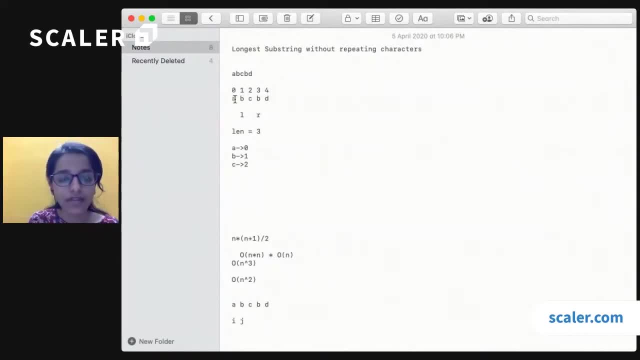 l is at one and r is at three. now we will. so a has gone out of window. that means l to r is the window. a has gone out of the window, so remove a from map. okay, we will be removing a from map now. we will check. that still is the element. is the character at r still present in the map? well, yes, it's still. 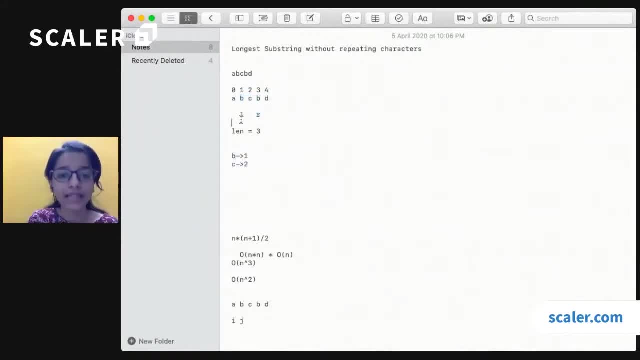 present. it means that it's still the part of the window and in that case we will again move our l. so let's move the l and l comes over here and b will remain at three. now b will be gone. that means here. so we actually remove this, this b, from the window. let's remove it from here now. we will check. 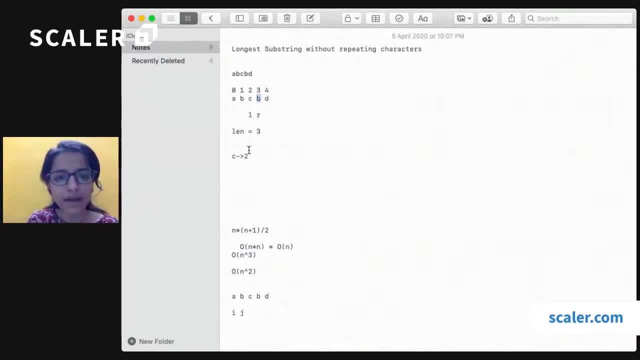 that, okay, is b present? now is b present now. we will check that. okay, is b present? now is b present. now is b present in the map. well, yes, it's. it's not present now. right, it's not present. that means we can include this b in our map. now. we can include this b with its current index, which is: 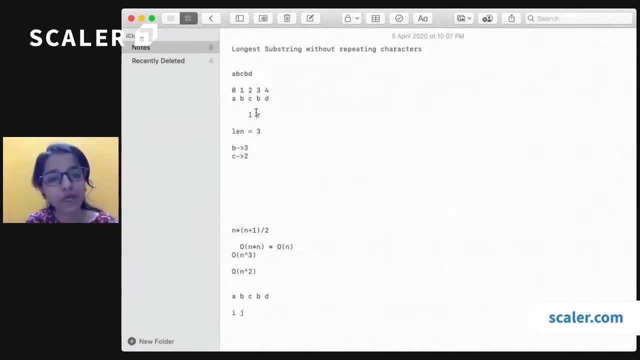 three, okay, which is three. now we can start moving our r again. so let's move our r now. r comes to four and b is not present in the map. length will remain three only because l to r, the other length is still three. let's include d in the map now b becomes so. 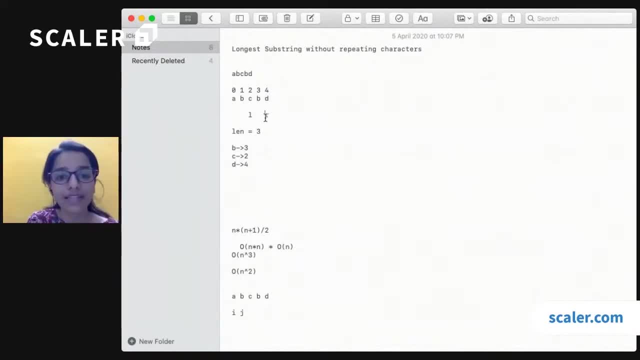 d is at position four. okay, and now let's move our r and now r. there are no more characters. therefore, we will simply stop and whatever will be the length, we will simply return it. so this is how we can process it: using sliding window, the time complexity of this approach is. 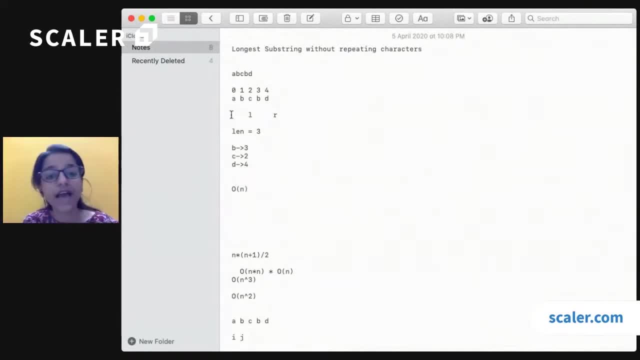 going to be just order of n, because we are iterating to each character not more than twice, because one with the left point of the window and the other with the left point of the window right. so as we are moving our left pointer and as we are moving our right pointer, so we are not. 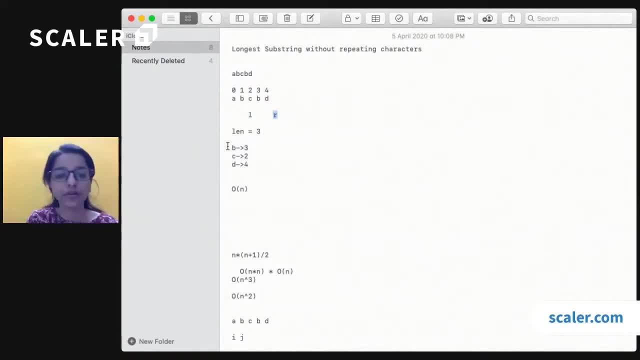 coming to any character more than twice. therefore, the time complexity is going to be two into n, which is nothing but order of n. right, we don't consider constant and the space complexity is order of n, again, because here we are using a hash map. does that make sense how we have? 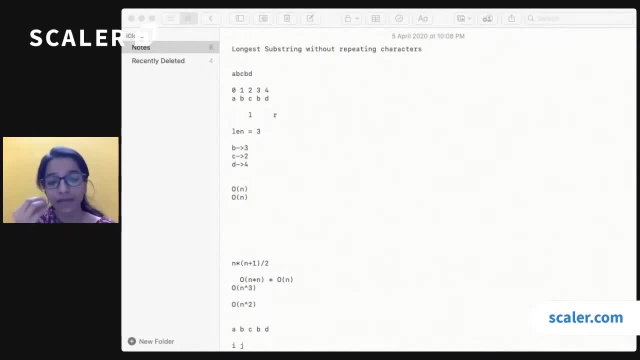 beautifully come across a good just by building some. you know order of n. right, so we are moving our r and we have come to this solution. does that make sense, guys? shall we code it? great, cool, so let's code it up. here we are now. let's quickly do this, okay, so um, first of all, i have to maintain 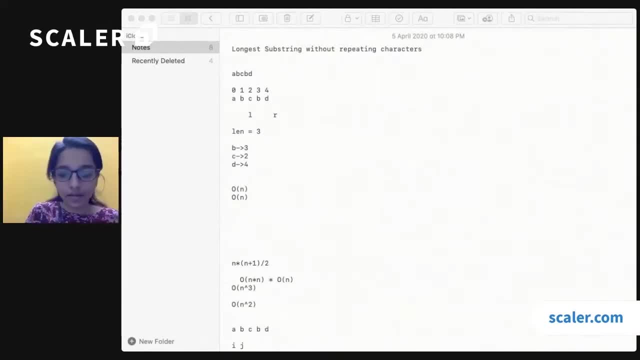 an answer which is, let's say, at present, int min, right, we want the maximum value, so we will initialize it to int min, or we can initialize it to zero as well, it doesn't matter, right? okay, so we can. the left pointer we will keep, which is initialized to 0, and also. 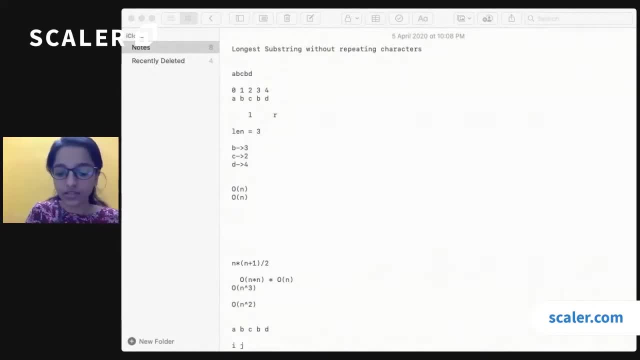 we will keep a right pointer right which is initialized to 0, and also we will keep a length right, which is again 0. now we will be move it rating through our string or we will be trading it with the help of right pointer, right pointer. so 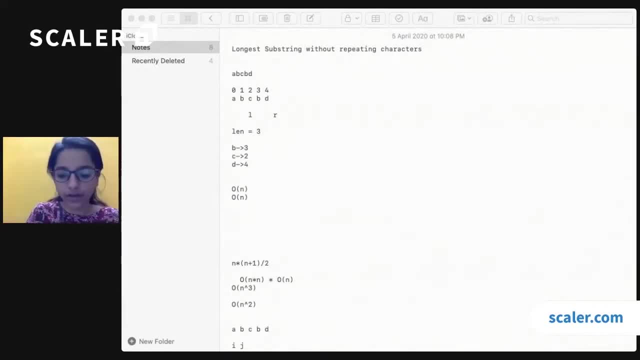 let's keep the right pointer in the loop. so let initialize the right pointer here, only to make it more readable for you guys. so right is less than a dot length, then right, plus plus okay and even okay. so we have to take a map as well, right? 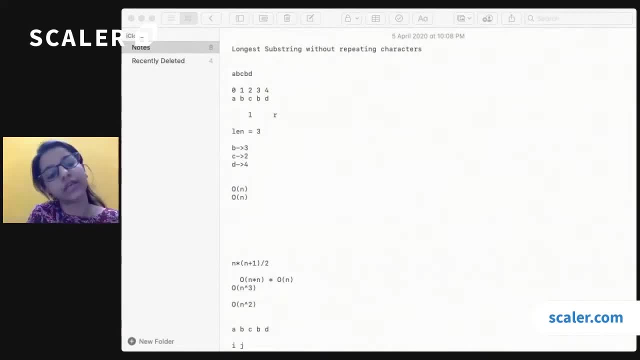 so we will take a map and that will be a map. will be off care comma inter, because we will be maintaining the index. make sense, you? you be maintaining the index with each character. now, okay, so if the character, so if the character at right, is present in the, so it's not present in the map, right? so how we will check that. 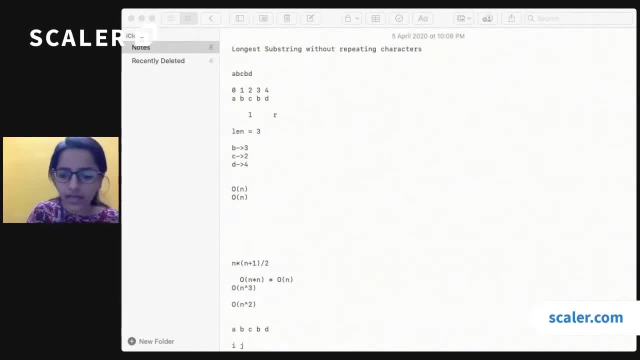 uh, m dot fine right. m dot fine is equal to is equal to m dot n. that's how we will be checking that a character is not present in the map. so if it's not present, we will simply do what we will simply do. m at a of right is equal to. i sorry, right here we are actually assigning. 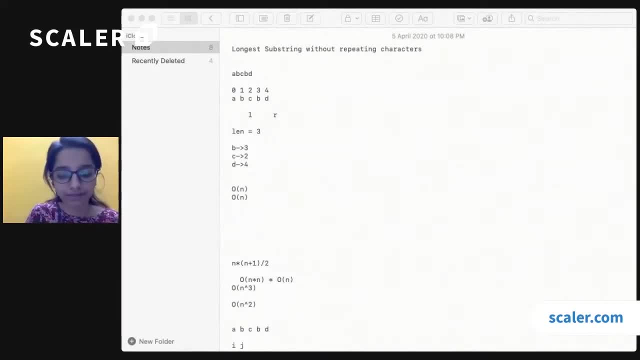 so here we are doing nothing. but, uh, let's say we have um, we have a, b, c, b, d, right? so here we are doing nothing. in the map we will be storing a mapped to zero. that means the index of a. okay, that's how we will be storing it now. uh, after storing, 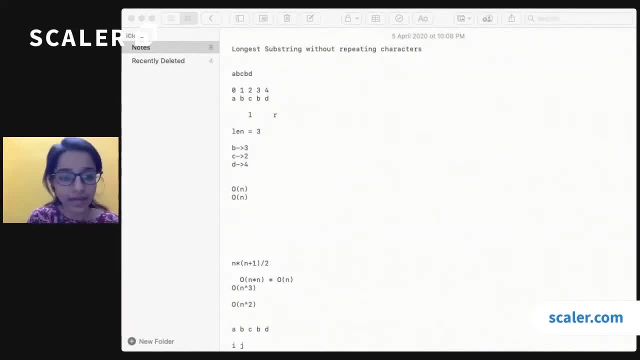 it like this: what to do? let's increment the length, right, because we have actually found a new character we have included in our map. let's increment the length. so, after incrementing the length, we are done till this point. now, what if the character is already already present? right, so for. 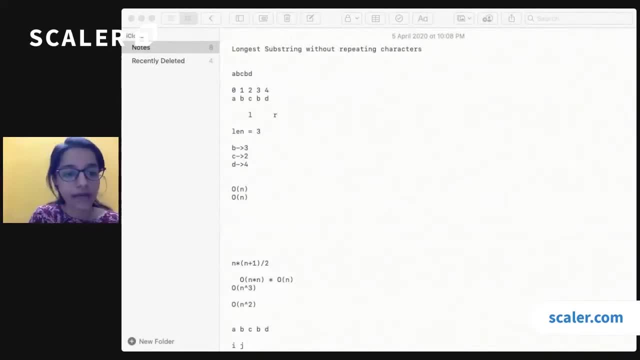 that we will use a else else block and in the else block we will be actually moving a left pointer. we will be moving the left pointer till the point. so let me, uh, just write it and then i'll make it clear, maybe, uh, okay, so let me make it clear first. so here what my point is: that i have let's. 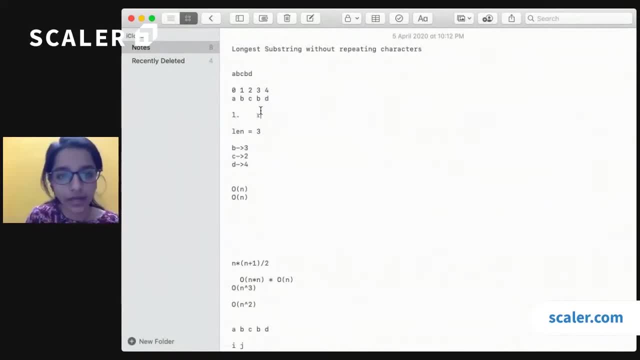 say l here and my r is here. okay, and now a. so let me actually change the map. the map will be: a for a, it's zero, for b it's one. for c, it's two and again b comes right. so i will be moving my l till. 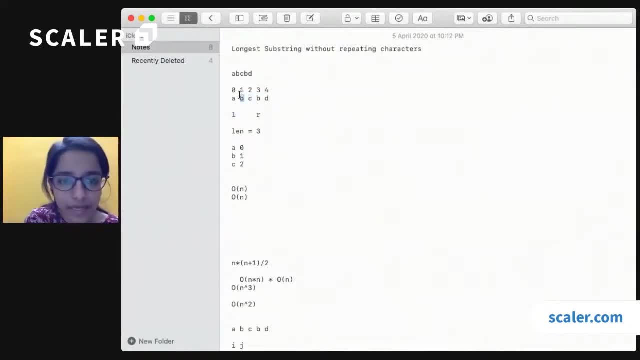 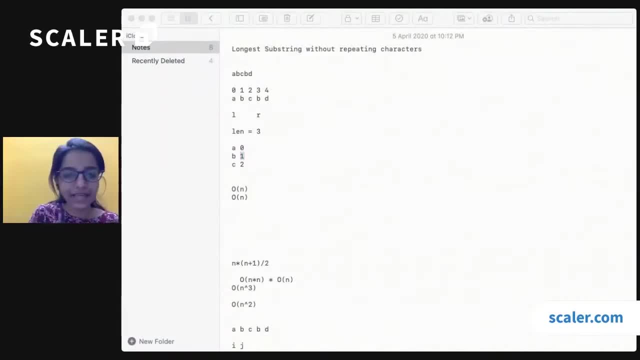 so, while left, left is less than equal to a sorry m at a at right, we will be moving our left pointer- and what more do we have to do? moving our left pointer and we have to erase the occurrence of whatever is left behind right. so that means m dot erase a at right, okay, and 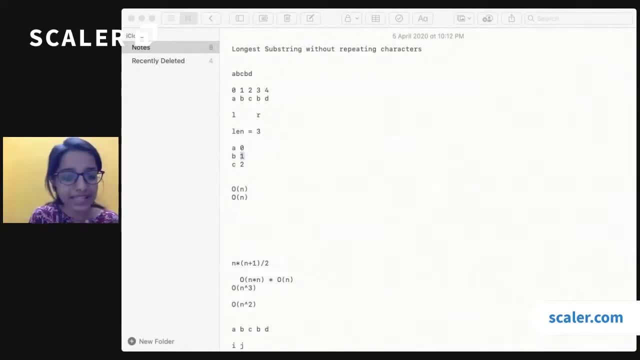 also, we have to do one more thing, so we have to reset the length. okay, we will be resetting the length. we have maintained a global variable. that means this is, let's say, this is the answer. but as our left and right shifts to this place, that means l comes over here and r comes over here. 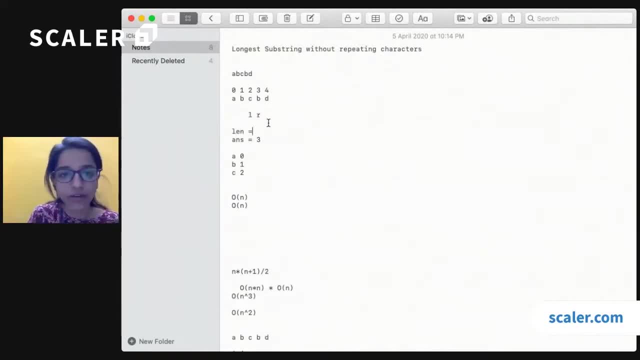 again the length, so we will also maintain a variable length. so now it will become 2. okay, it will become 2. that means the current window size and that is given by what? that is given by right, mine- sorry, right minus left, plus one. okay, and also we will be updating our answer to max of. 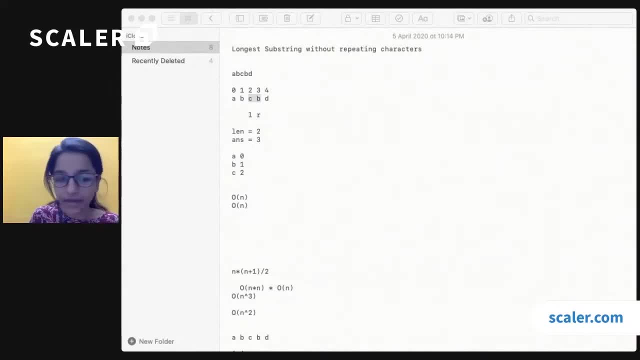 max of answer comma length. and finally we will minus our answer comma length. okay, and then finally we will will update the length to max whites of ones row left. this means that the current window level size will cover this function. we will return the answer. let's see if it works. are we missing on something? does this look fine? 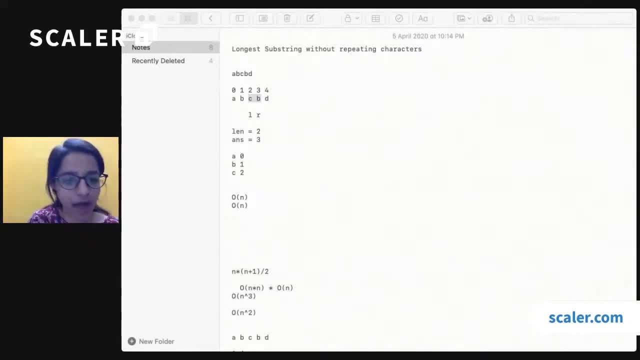 okay. so we actually, uh, have to do one more thing over here, and that thing is that we actually have to write the new index, right? so here let's say, a was gone and now the new index of b is equal to three, right, so that means it's equal to nothing. but m at a at right is equal to right, and that's. 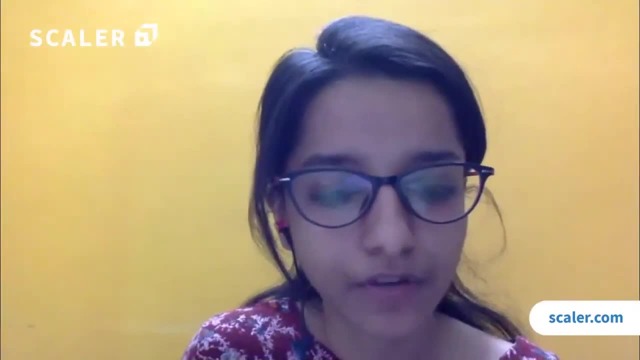 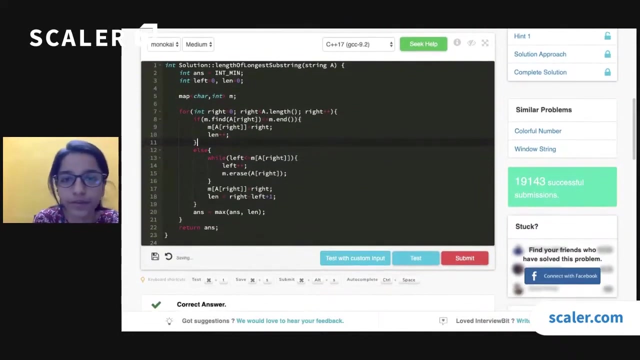 all, let's test it. um, i'm really sorry, i didn't uh see that. let me share it again. don't worry, i will explain the code. okay, so you guys want me to just explain it? cool, it's good that you have understood the logic and i'm sure that you will all will be able to code it, let's see. so here i am maintaining: 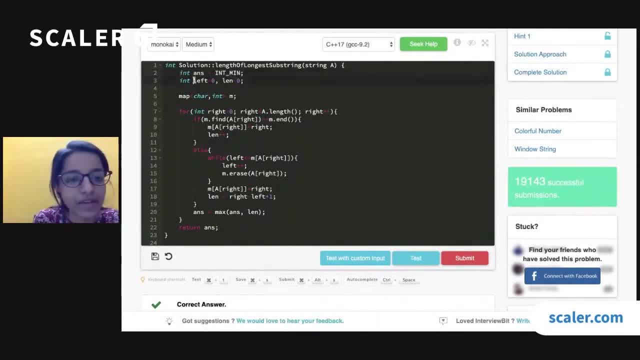 the answer, which is initialized to int min. okay, then we have a left, that is the left window, and this length is basically the uh to keep track of the length. we have right, this length is actually from left to right. okay, now we also have a map that is from map to character to int that character, map to the. 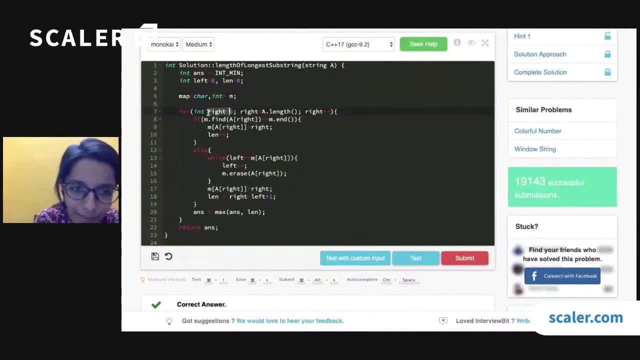 index. okay, now we, with the help of this right pointer, we will actually be iterating through our string. okay, and while iterating through the string, we will check that if the character is already present or not. so here we are actually checking. if the character is not present, okay, so the character is. 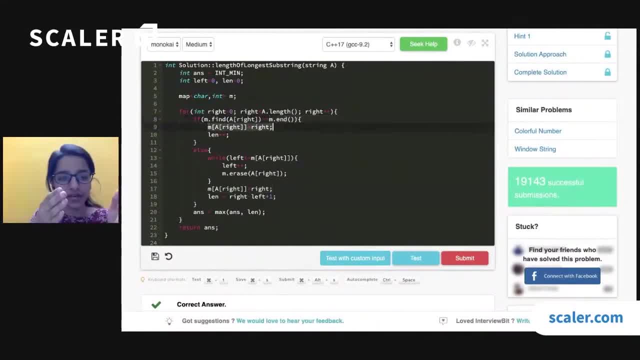 not present. so we will actually put the character with the index in the map, okay, and also we will increment the length. so this is when character is not present. but if character is present, in that case we will be moving the left pointer. okay, we will be moving the left pointer till the point. 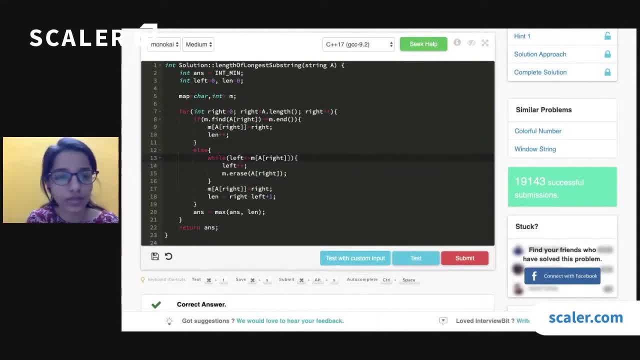 uh, so actually i i have shown it to to you in the editor. i think you have seen it there. right, you have seen it there. so we are actually moving our left pointer till the first occurrence of the repeating character in is gone. okay, it's gone. so then we will do left plus plus. 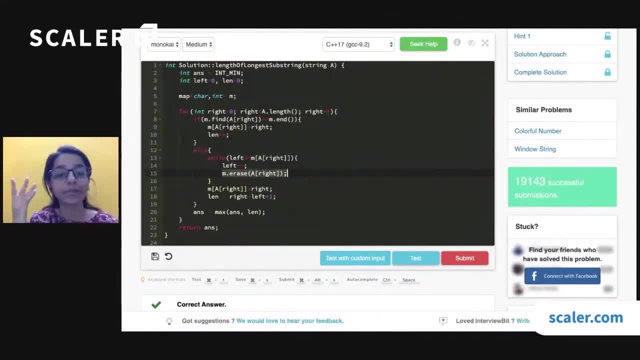 and we will erase the character that we have left behind. okay, and then we will do it till the character at right pointer which we found repeating in the current window. so till the repeating character is no more repeating, we will then add the new index of that character. 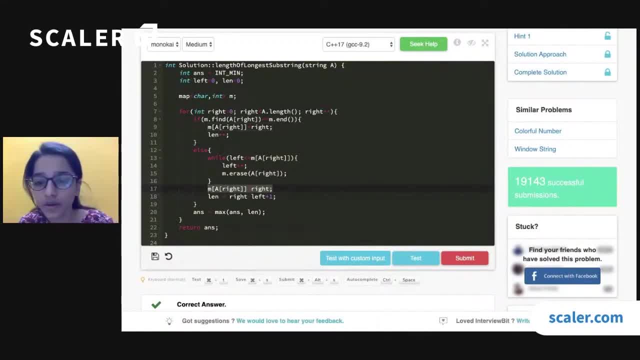 in our map make sense, we will add the new index of that character in the map. does that make sense? okay? so, okay, okay, let me complete it and then i'll get back to your questions. okay, so here we have the character with its new index, and also now we will reset the length to the length of the. 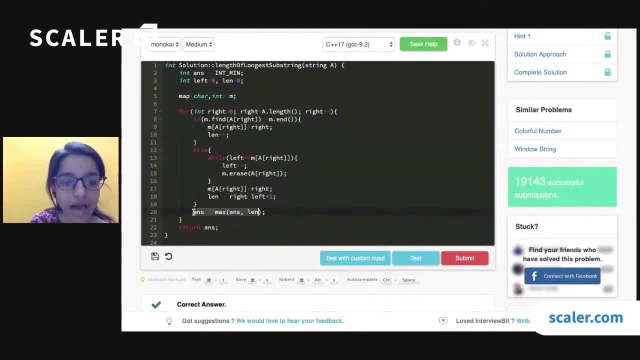 current window right to the length of the current window, and then we will update our answer. we will update our answer. we will keep on doing this right. so length will have the size of the current window and this answer is the global answer that we have. so whichever is maximum and our answer will have a 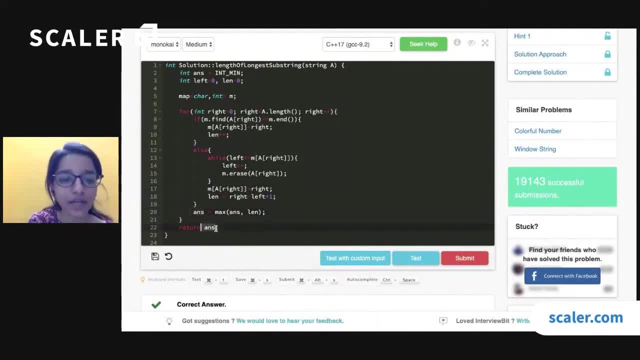 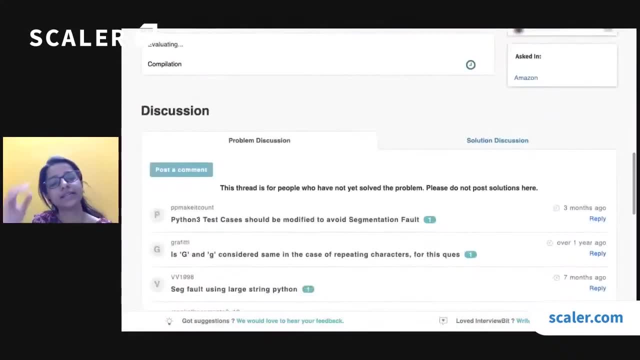 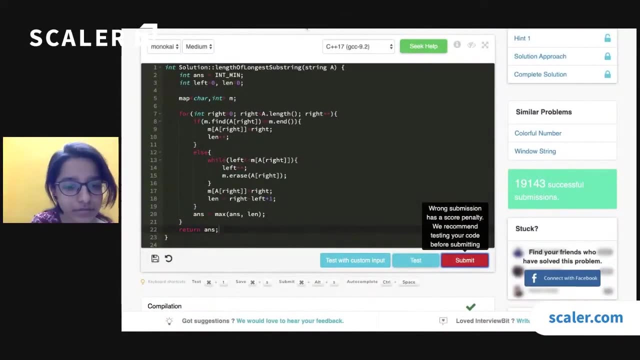 that will come in our answer and we will return the answer. okay, we will return the answer. let me try to submit it. let's see if I get summited. okay, it failed there. did it fail? oh sorry, we here. we need to erase the left, not right, okay, 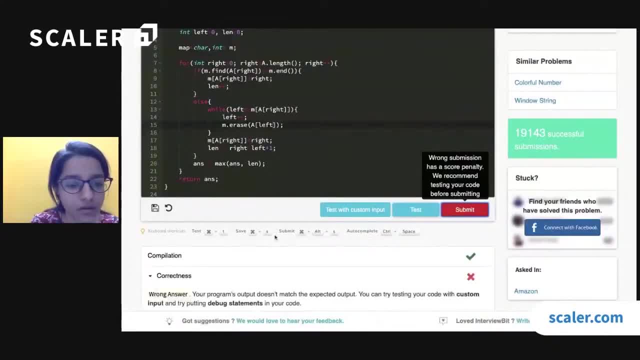 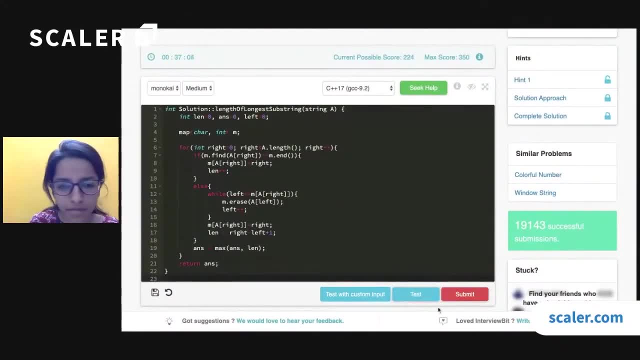 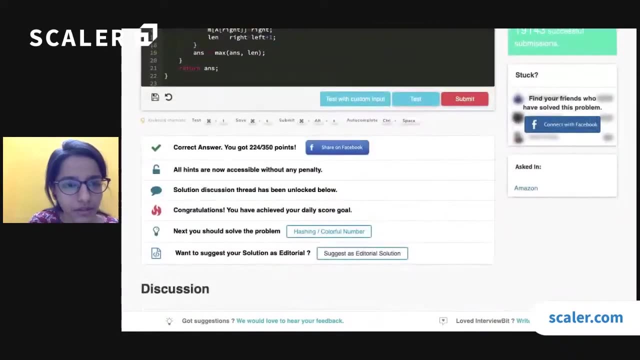 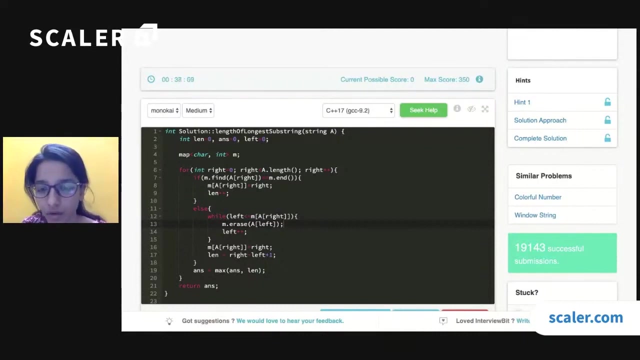 and let's see it now. it's still not passing. let's see if this works. yes, it worked. so first we have to basically erase and then we have to do left plus plus right. okay, so there was just a little bug. okay, so is everyone fine with this? okay, so let's see if we can do it. okay, so, let's see if we can do it. 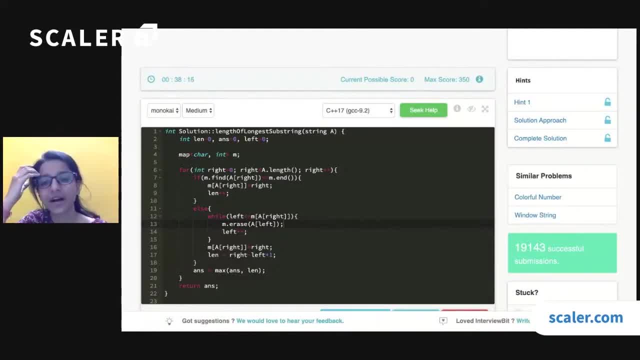 fine with this thing, okay. so basically, you should use set when you have just, you just have to keep track of that particular character only, or I would say that particular data only, as in when you don't have to map, anything, right? so here we see that we actually map the character to the index, right? so that's why we used. 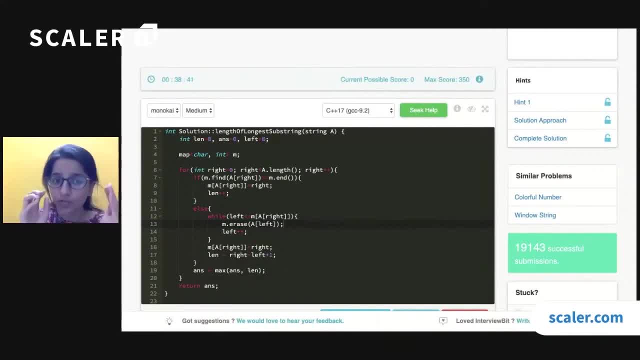 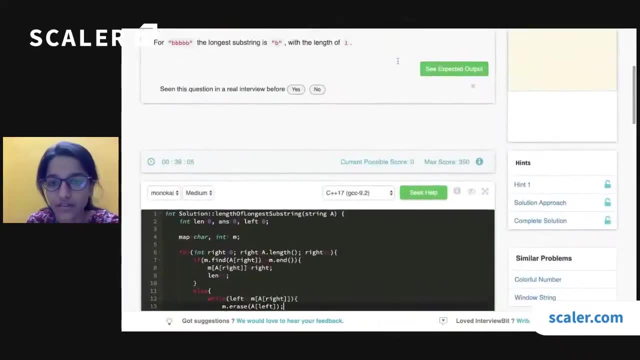 a map because keeping the index also was necessary to move our left pointer and therefore we preferred map over set right S. does that make sense? execute now that. why do we need to keep map over here? why not set? we actually made a streak today, right? so, Pawandip, I would say that. 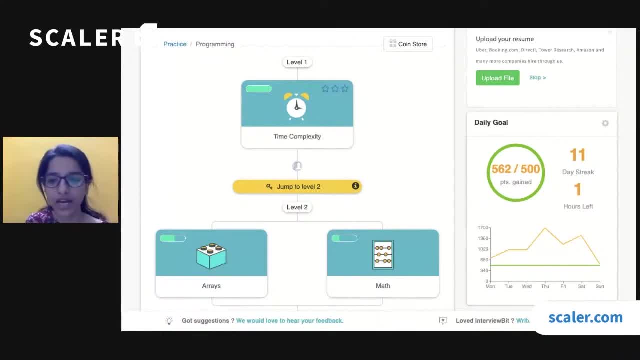 yes, maths is important, but competitor, competitive programming is more than maths Olympiad, right? so it's, it's more than max Olympiad, that I would say. but yes, it will definitely help you, right, because in competitive programming we can see maths a lot. so, yes, that's a good question, pavandeep, that you brought up. so this was it from my side. 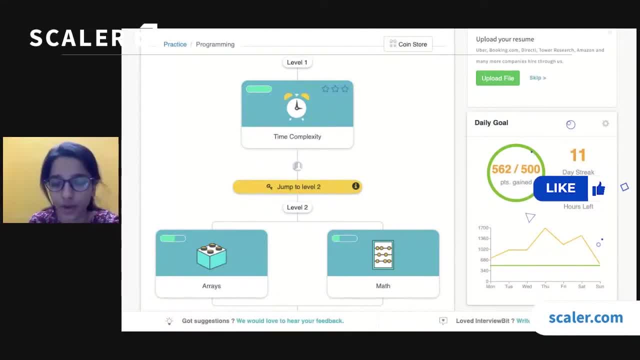 these were the questions and i hope that you enjoyed them right. so see ya. bye, bye, take care, stay safe. 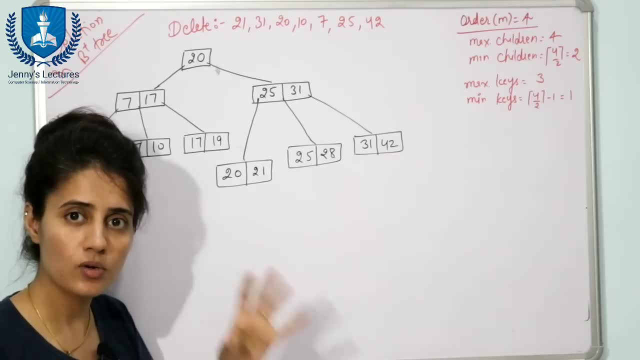 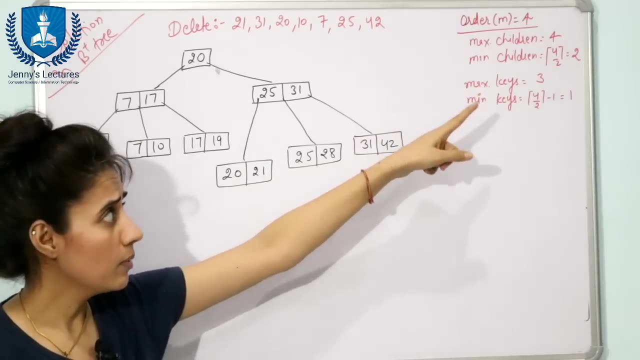 Now in this video we will see how to delete data from B tree. We will discuss all the cases of deletion right. The order of this tree is 4.. So maximum children can be 4,. minimum can be 2,. 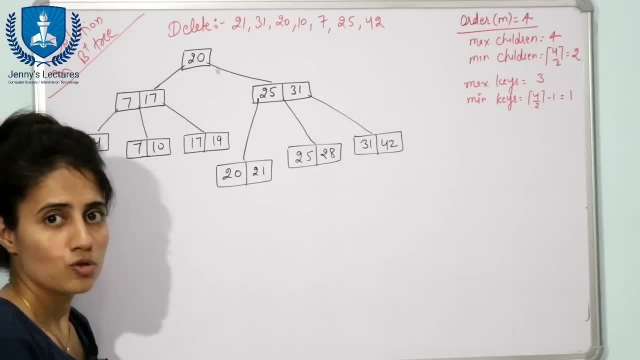 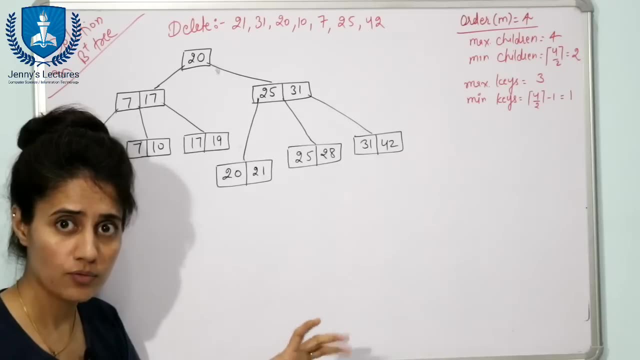 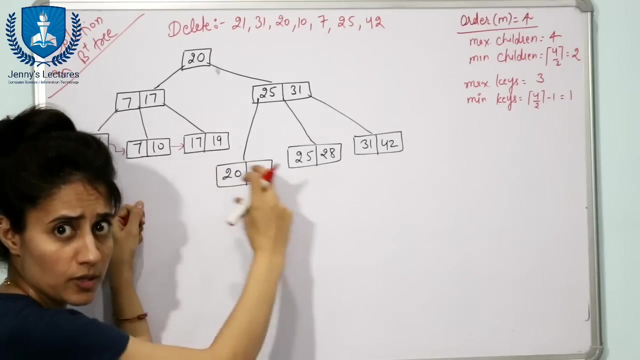 maximum case can be 3 and minimum case can be 1.. So first, suppose you want to delete 21.. See, as we know, the data in the B plus tree is present in leaf node only. fine. And see these leaf node are also connected like this: like this right, These data is present in a. 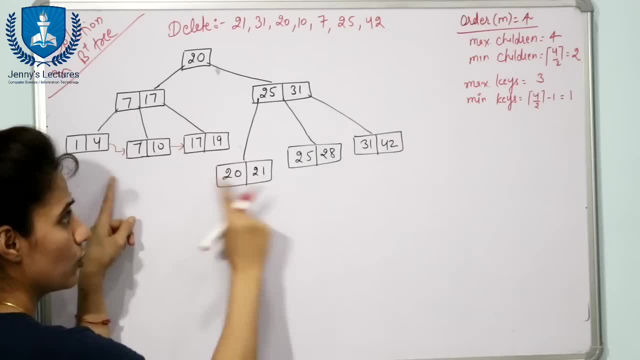 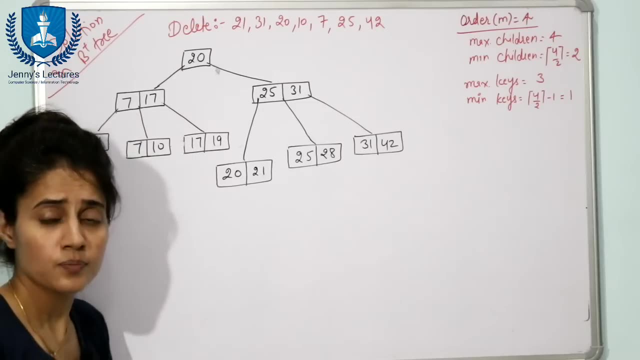 form of link list. These leaf nodes are also connected with each other, right? So I am not going to show that thing here, but you have to take care of that thing. fine, Now, data is present in leaf node and in internal nodes. only we have indexes. fine, See, now suppose you want to.